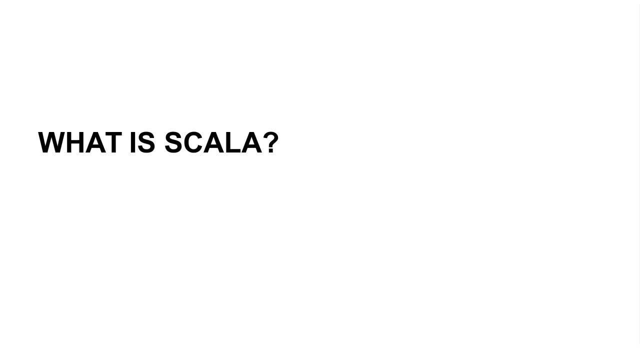 The language is supported by a large and growing community with varying backgrounds and disciplines. Today, Scala is one of the most well-known and respected alternative languages on the Java Virtual Machine. In this session we discuss the positives of Scala. Scala's strengths you'll find not. 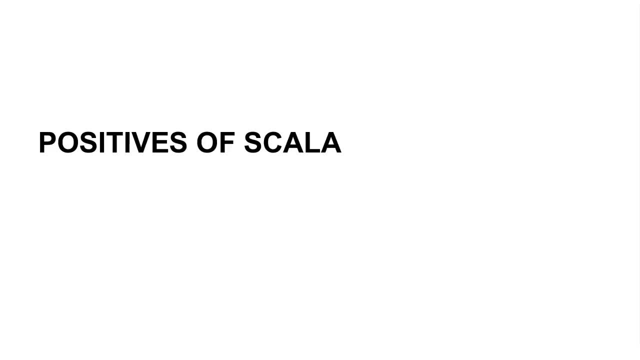 only in this series, but as you progress are many For one. Scala has type inferencing, so that you don't need to declare everything explicitly And although you don't type much, it is also statically typed, where you know the type associated with every reference. 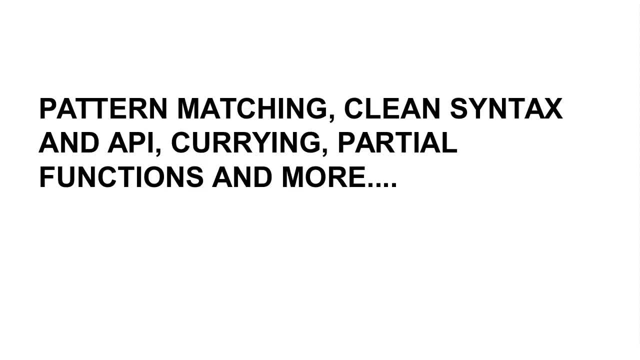 Scala is also a language that offers other features like functions, pattern matching, clean syntax and API curring, partial functions, partially applied functions, implicits, operator overloading, infix operators and more, And some of which we'll find in this particular. 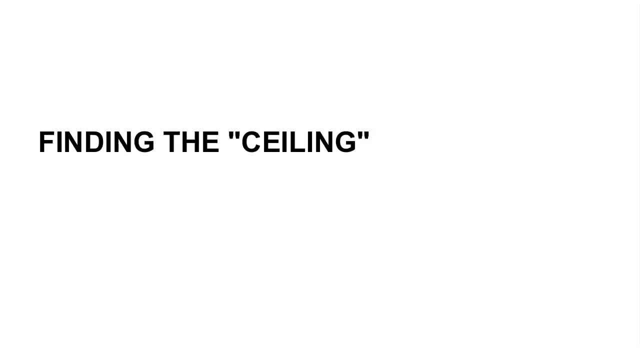 video series. Now, as someone who has knowledge of currently 10 different languages, I find Scala very complete without much aggravation. It'll be tough to reach what I call the ceiling with this language, And what I mean by the ceiling is the point where things become either weird. 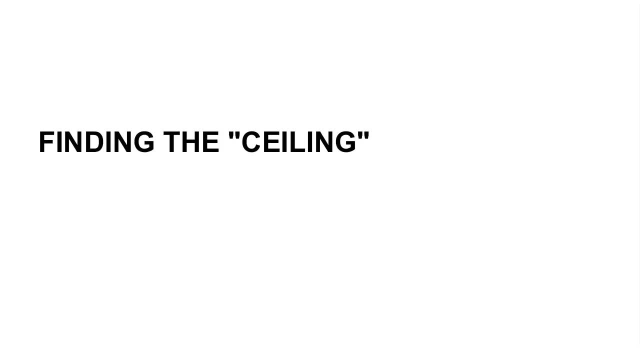 or awkward for the programmer. Although every language has its strengths and weaknesses, it'll be very tough to find that ceiling in the Scala programming language. It wouldn't be fair to the viewer if I didn't cover the negatives of Scala First off. let's 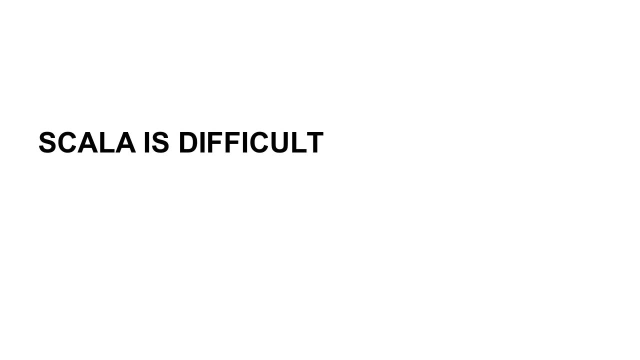 start with one of the obvious. Scala is difficult. It is an extremely powerful tool and because of such, there are many that find this language hard to understand and to use it. The analogy I use is moving center blocks up to the top of the building In order to move that center. 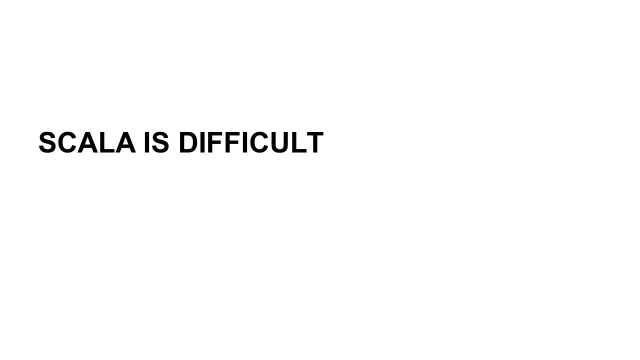 block. you could either do the simple thing: take those blocks, put them on your shoulder and start walking up the stairs, or you can put the investment of learning how to use a crane. With a crane, though, you will have to learn the mechanics, wind tension, safety. 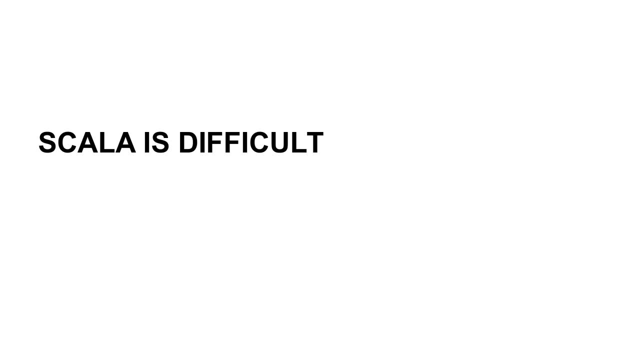 and weight capacity. The rewards for accumulating that knowledge are immense. Another issue is that Scala currently suffers from a soft skill issue, and that is finding talent. There are many jobs and often there are not many that can fill it. If you are interested. 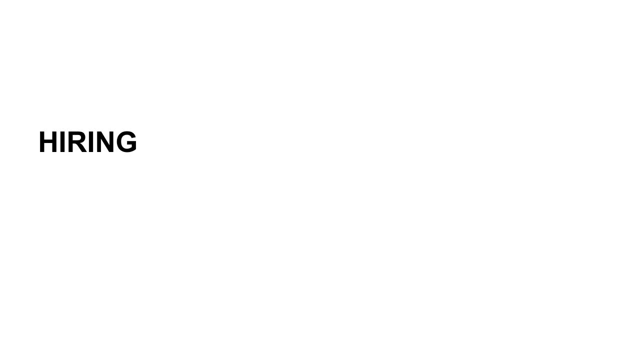 in either creating or migrating a project to Scala. it is worth investigating your team options before proceeding, And although I find this more of a positive than a negative, is that while language engineers do care about backwards compatibility, they will not hold up the next release of the language. 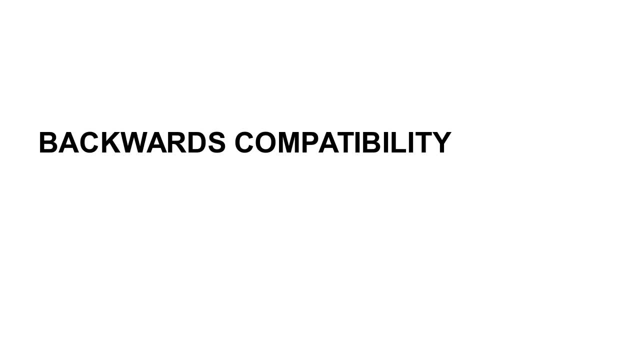 over it. In other words, Scala again cares about backwards compatibility, But not that much. It isn't going to be like Java. So what effect does this have on the community and how they work with Scala projects? Well, let's take a look at a very popular Scala-based library called Acca. 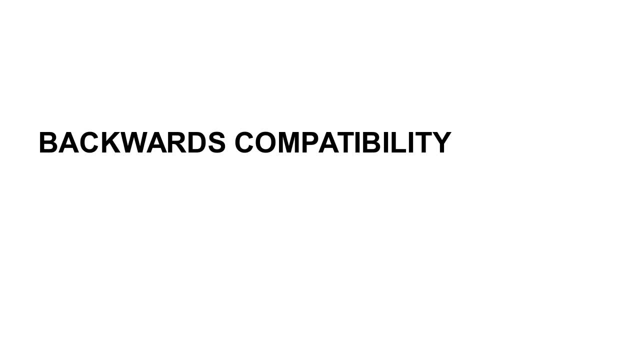 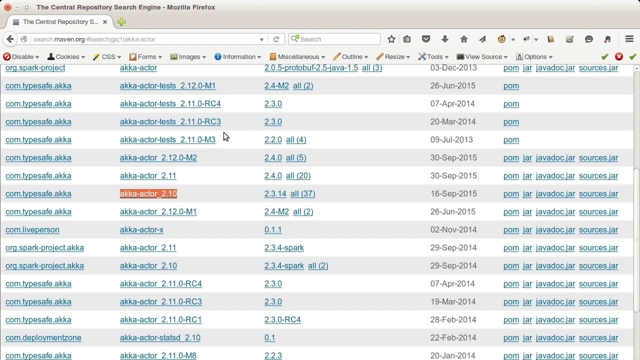 And what I'm going to do is I'm going to go over to searchmavenorg on the browser And let's take a look at some of those dependencies. Okay, so here we are Now. if you want to use actors within Scala, you'll notice that. 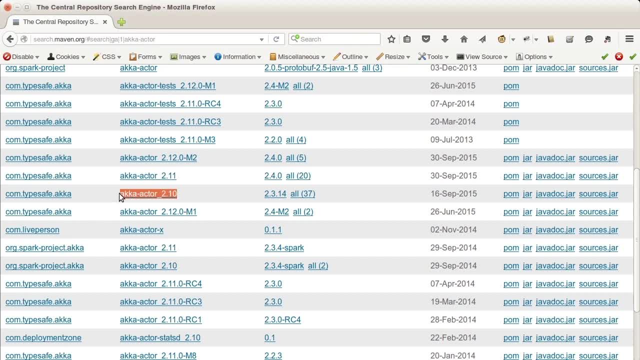 something like this, where I have Acca actor 2.10.. All the while I have a version like 2.3.14. And over here I have Acca actor 2.11.. Now, the 2.10 and the 2.11 are Scala versions. 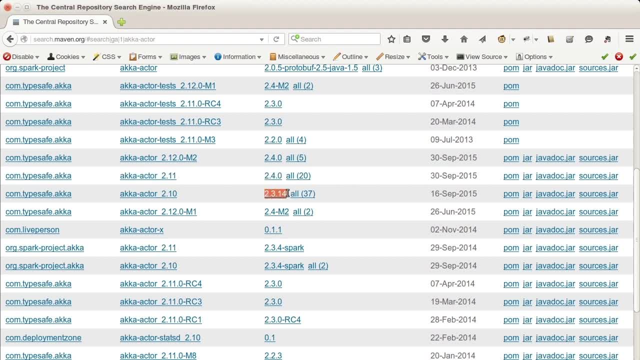 And these versions over here are the versions for the library itself. So you have this divergence. One is they have to maintain the version of Scala And for every library. So this one has a 2.11. And a 2.10 version. 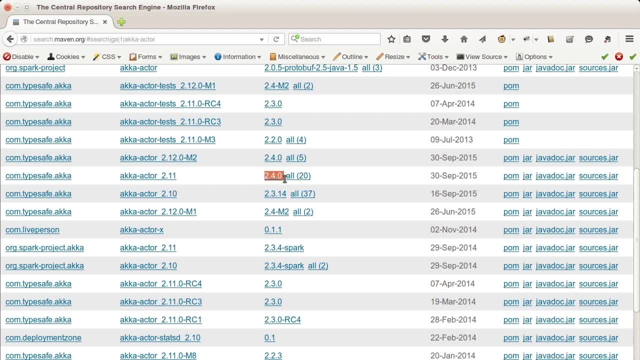 But that library itself has versions of its own, So this is a side effect that you would have to be aware of. Now again, is this truly a negative? I do not think so personally, But it would be something that you should be aware of before engaging in the Scala programming. 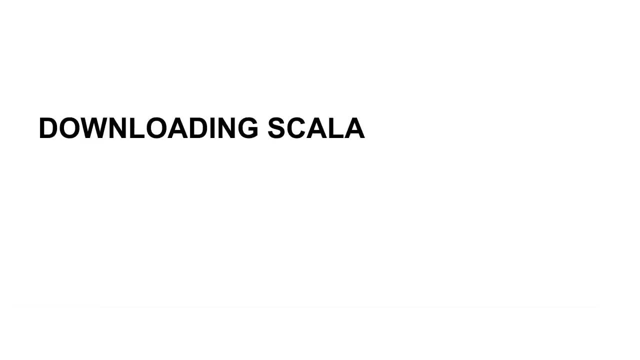 language. In this session, we discuss where to download the Scala programming language. Before we talk about downloading, Scala is a JVM-based language. It's a JVM-based language, So a Java is required, In particular, a JDK or Java Development Kit. 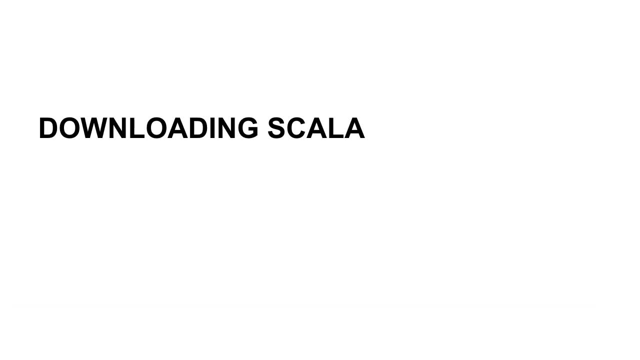 And this is required before proceeding, And because the Java Development Kit has the compiler, all that is needed As of Scala 2.11.7,, JDK 6,, 7, or 8 is required. JDK 8.0 is preferred. 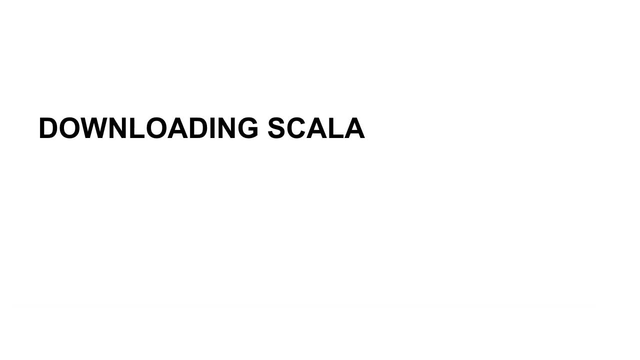 And not only that. as of April 2015,, JDK 8 is the only version supported by Oracle. To download the JDK 8.0 version, you need to download the JDK 8.0 version. You need to download the JDK 8.0 version. 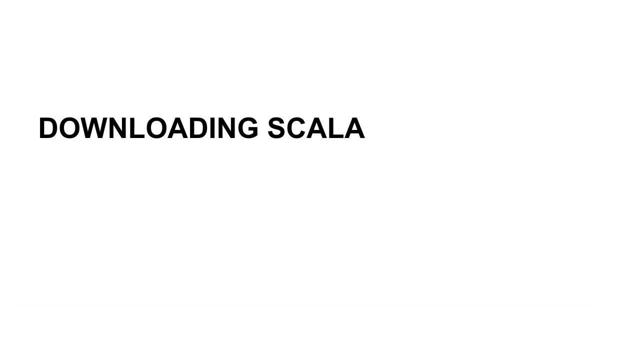 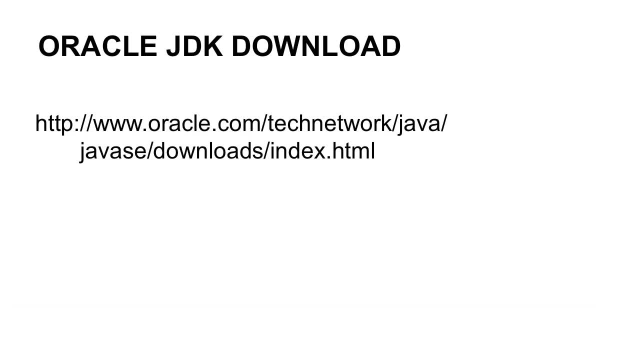 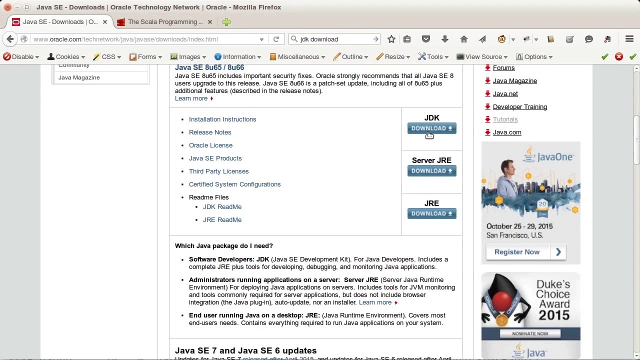 or JDK download, or you can go to this website: oraclecom slash tech network, slash Java, slash Java SE slash download, slash index HTML. This is what the page looks like. I'm going to scroll down a bit And here I'll find the JDK download button. 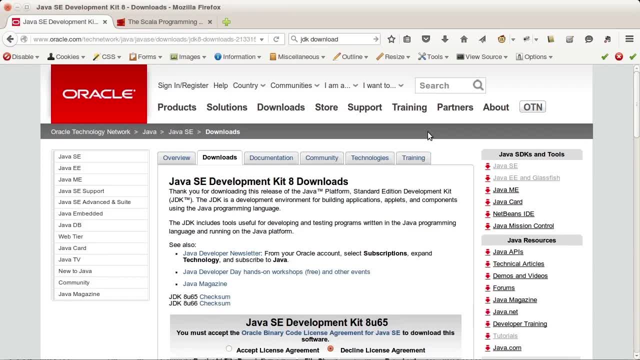 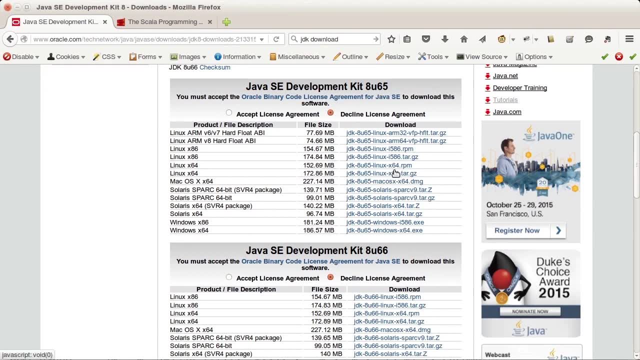 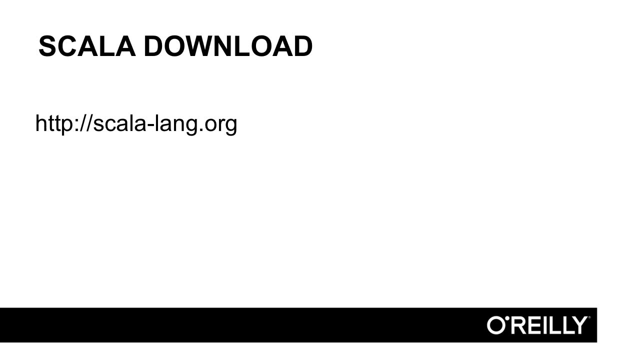 I'm going to click on the JDK download button And this takes me to the download page. Choose your flavor and architecture and install per the directions. I'll be running my examples on Linux. Next we must download Scala, And this can be found at scala-langorg. 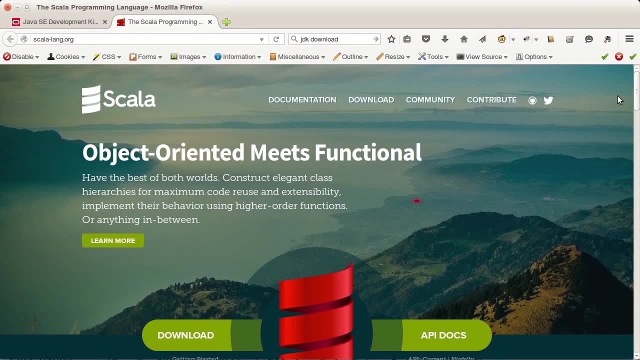 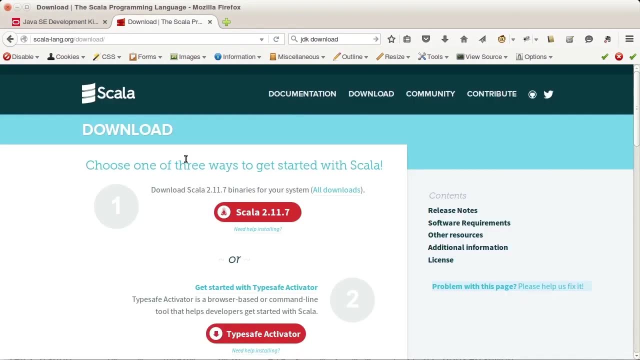 Let's see what that looks like. Here's the scala-langorg website And here I will click on the download link. Now here's the page for the Scala download And we'll select the button that states download. And here it states Scala 2.11.7.. 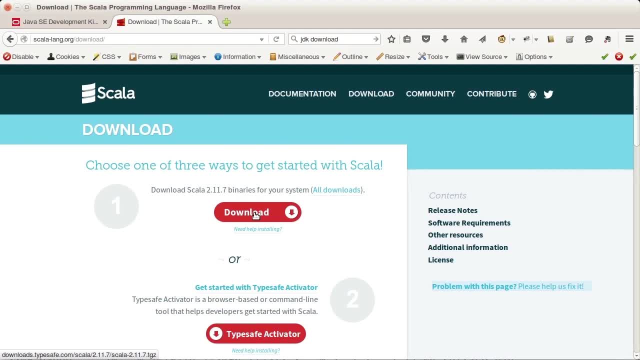 For Mac OS X and Linux. this will be a TGZ file or a targz file, and it'll be up to you to expand the file in whatever location you desire on your home directory. Please make note of the location, since we'll need that later when we set up our environment. 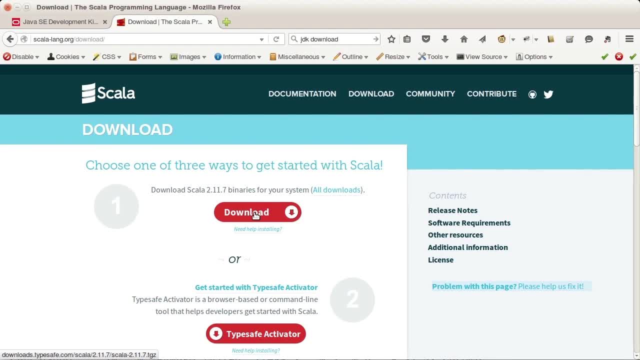 variables. Windows users, this will download an executable msi file. Once that is downloaded, double click the msi file Now, as a note for Linux and Mac users, there are package installers that you can use if. 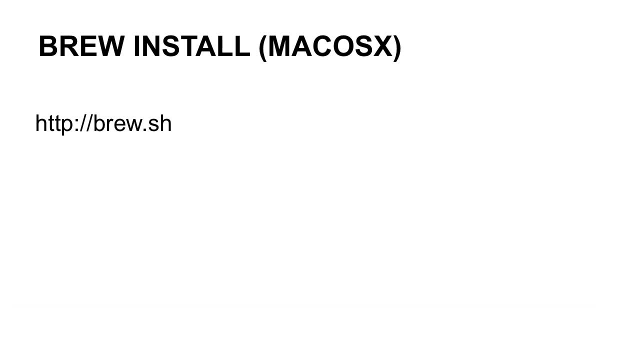 you so desire to. What we've just described is adequate enough. but if you want to use the package manager instead, then you can do so. For Mac OS X, you have a magnificent installer called brew, And to install brew, just follow the directions at brewsh. 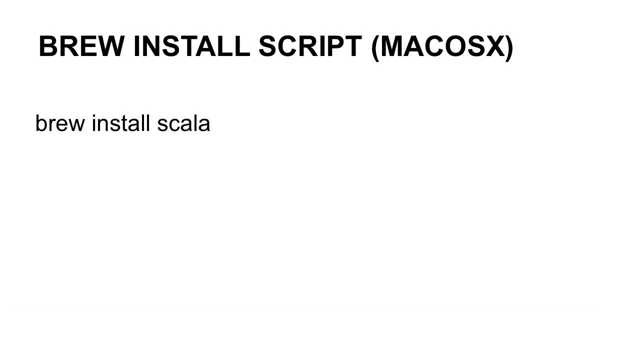 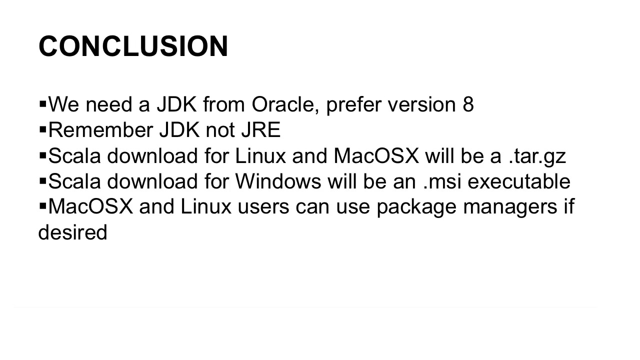 This is a website. Once brew is installed, you can install brew with a command called brew install, And that's it. Thanks for watching. I'll see you next time. Bye, If you're viewing this recording much into the future and there's a version 9, then use. 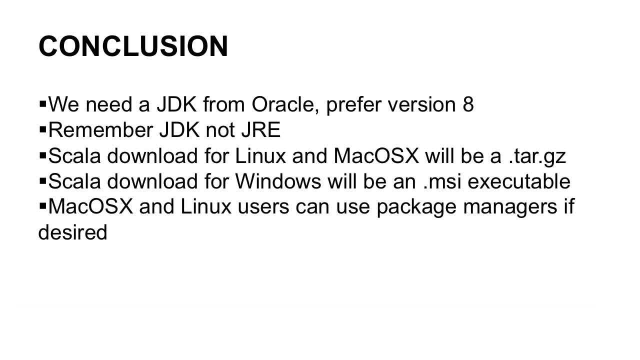 the latest one. Remember: use the JDK, not the JRE. JDK has the compiler. JRE is just a runtime for the end user. For Linux and Mac OS X, this would be a targz file. For Windows. this would be an msi. 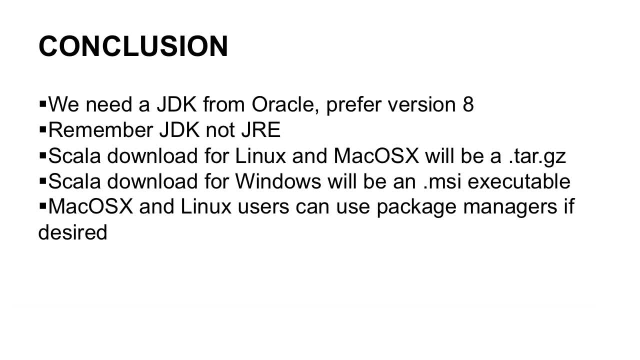 You can double click on that msi file And, if you'd like, you can use package managers installed on your machine, and this is only applicable for Mac OS X and Linux. And, if you'd like, you can use package managers installed on your machine, and this is only. 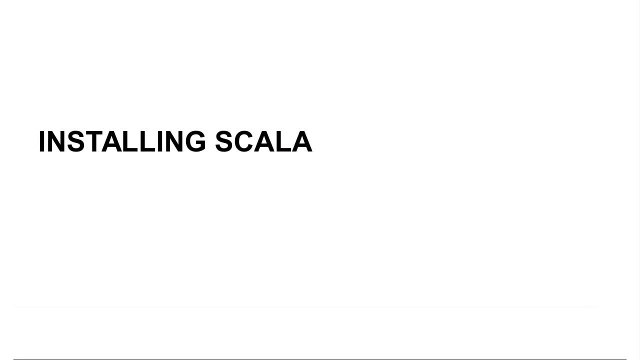 applicable for Mac OS X and Linux. In this session we're going to make sure that Java and Scala are mapped correctly in our environment variables, So our goal in this session is to make sure that all of this works in a terminal or command prompt. 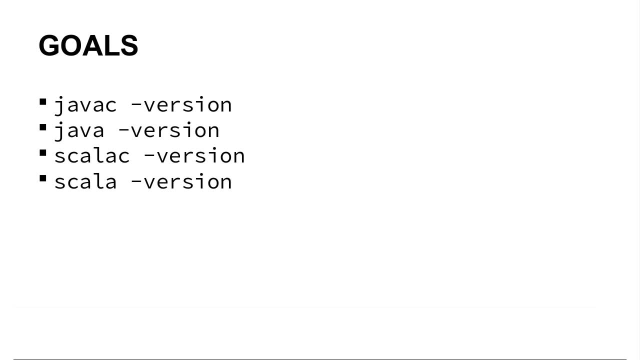 Java C space dash version, Java space dash version, Scala C space dash version and Scala space dash version. We're going to start things off in the Windows operating system Here. I am in Windows And I'm going to open up the command line by hitting the Windows. 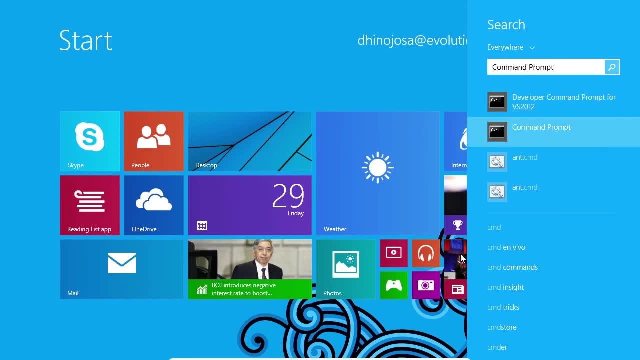 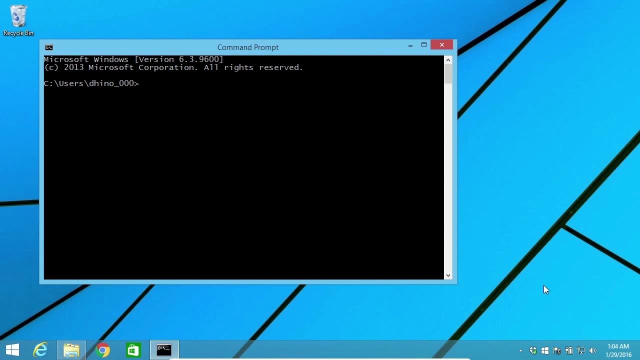 key and typing in CMD, And I'm going to open up the regular command prompt that comes with Windows. If you have a specialized command prompt, open that. Now let us try our set of goals. Java C space dash version. That didn't work. 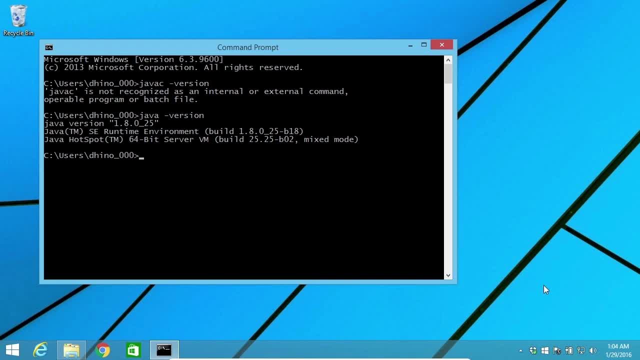 Java space dash version That one did. Now that worked because the Windows installation by default will always make this runtime Java executable work. It won't make Java C, which is the compiler, work, So we need to do a little bit of work. 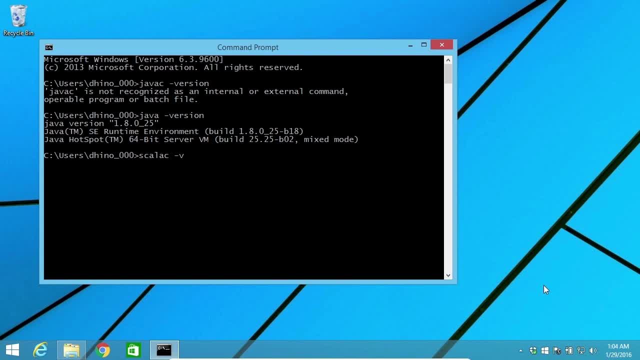 In order to get that working. So Scala C space dash version is the other goal that we were looking for. That did not work And I'm going to assume that neither does this one, So we need to go to the environment variables and set up Java home and Scala home. 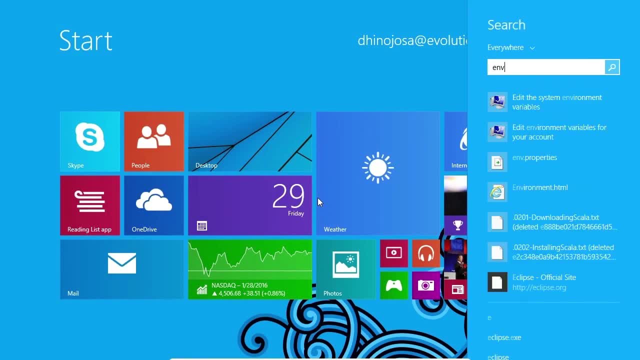 I'm going to hit the Windows key and type ENV So you can see. I have two entries here on the right hand side: Edit the system environment variables and edit the variables for my account. Now, the edit environment variables for your account might be your only choice. 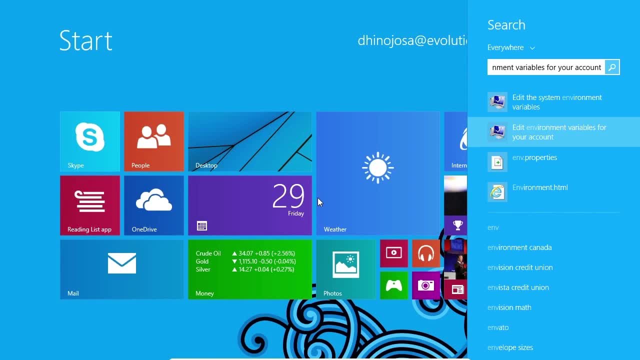 Since many users are on work machines and they don't have the full access to their machines, I am going to select edit the system environment variables. I have complete control of my machine. What I'm going to do here is, once I have this box open, I'm going to click on environment. 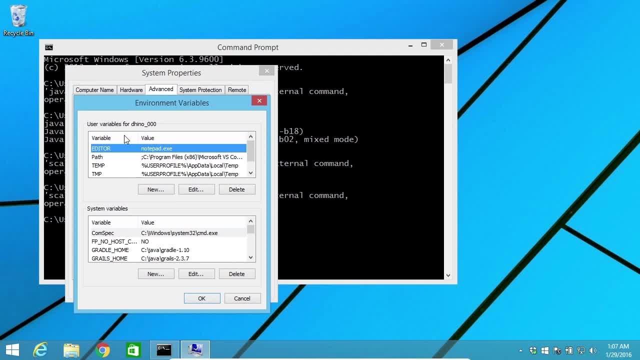 variables. Now I have user variables for my account up here. That's the first box- And I have system variables down below. Now, down here, what I'm going to do is I'm going to create an entry, and this entry is going to be called. 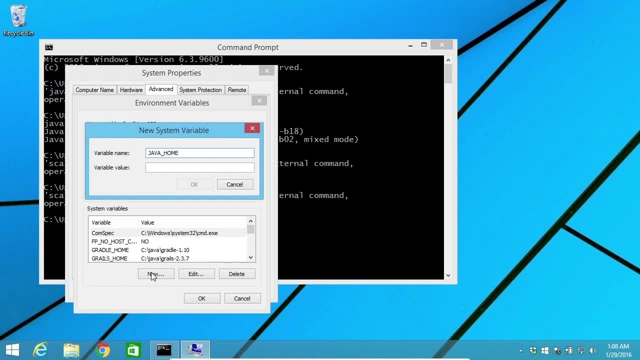 Java underscore home, all in caps with an underscore. This is a standard name And what this is going to do is it's going to point to a location of my Java install. So what I'm going to do is I'm going to go down over here and load up the Explorer and 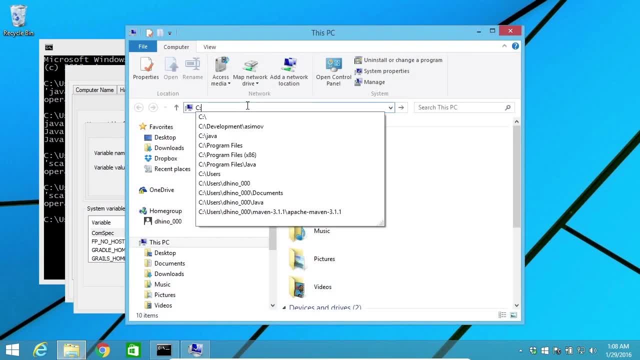 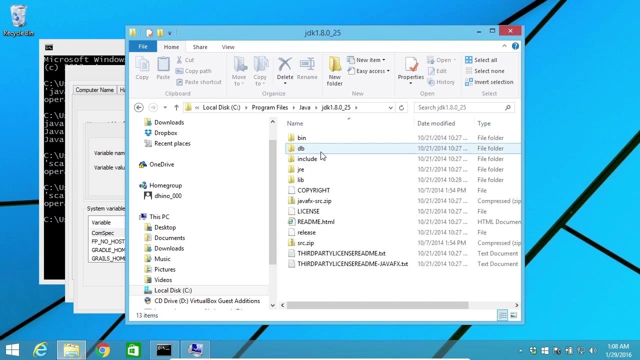 look for the location of my Java install. Now, if you went ahead and accepted all the defaults when you installed Java, this in all likelihood is going to be inside of program files and Java. So I have JDK one eight. So I'm going to go ahead and click on that, and then I'm going to go ahead and click on. 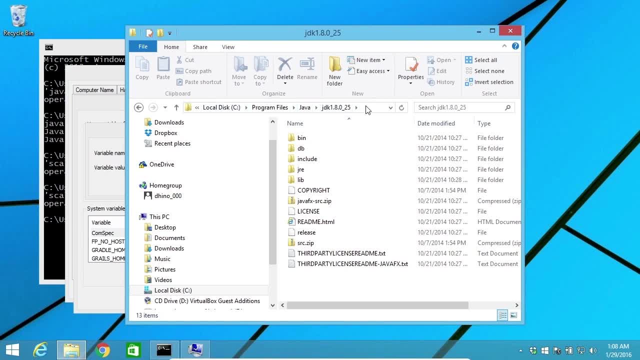 this box right up here that shows the file structure, and I'm going to just use my mouse and click on that. Now I get to see there's the complete path. I'm going to copy that and I'm going to go over here to the system variable and I'm going 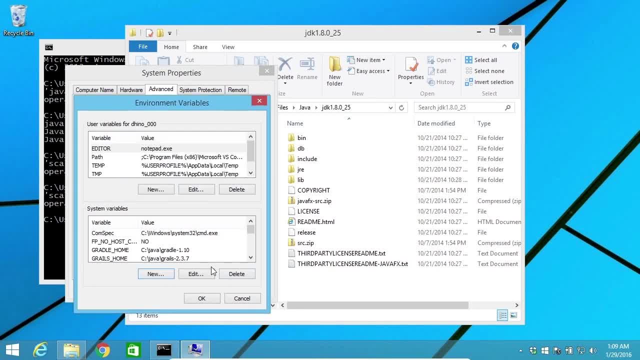 to paste that location in here. All right, so we've established the Java home. now, inside of my system variables, I'm going to include Scala home, And now let's go to the Explorer and find out where this is located. Now, if you downloaded the MSI, which is in all likelihood, that's what you did. 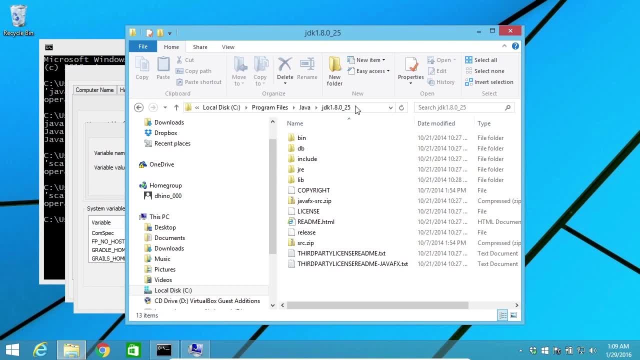 This will be located in somewhere around C program files x86, backslash Scala, but let's verify that first. So we're going to be looking for C backslash program files x86, and somewhere within here we're going to look for Scala. and here's Scala, right in here, and here are all the folders. 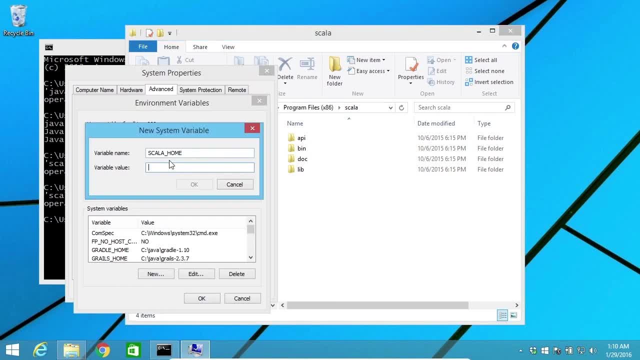 that we're concerned with. So I'm going to copy this location And I'm going to paste that onto here. So variable value in here will be C program files, x86 backslash Scala. Let me go ahead and click OK, And next is the path. 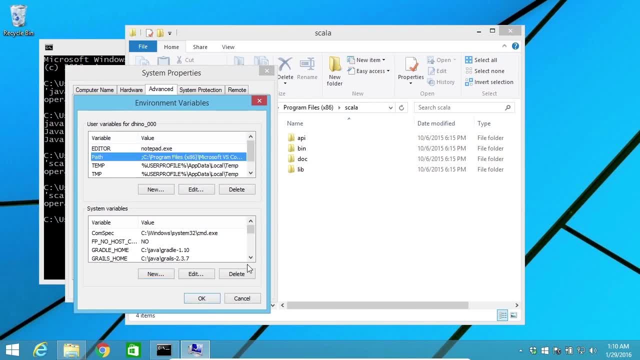 Now, as you can see here under user variables, I have a path here. I also have a path here for the system. I have access to the system, so I'm going to edit this one. So I'm going to highlight path and click on edit. 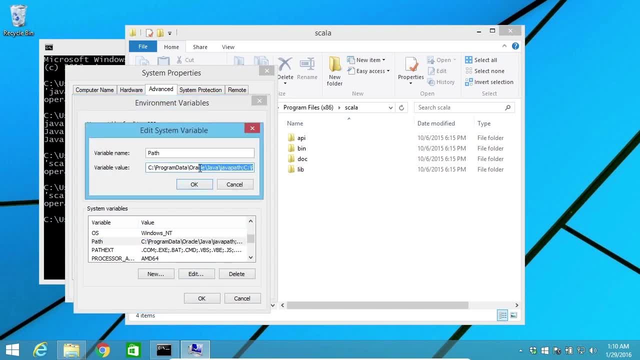 Now, once I'm in here. now there are some entries that are already available, and I don't want to mess around with what has already been established. So what I'm going to do is I'm going to merely append or add Java underscore: home backslash. 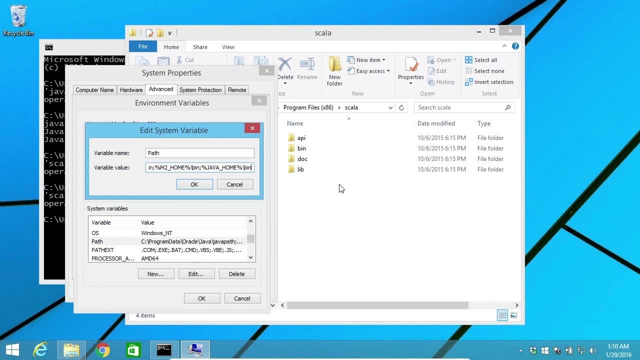 BIN. Make sure it's a backslash and not a forward slash. another semicolon: percent Scala, underscore home. percent, backslash BIN. and here I'll click OK. Now let me open up the path just so, that way you can get a quick review again of what this. 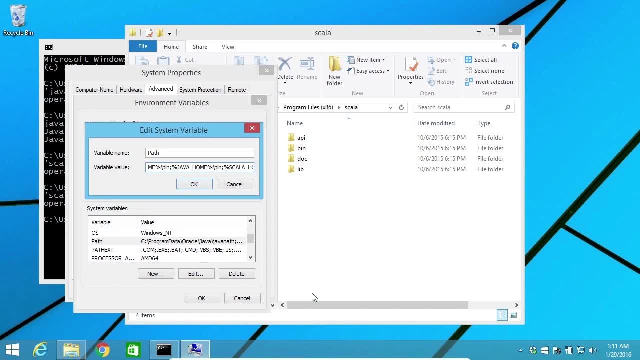 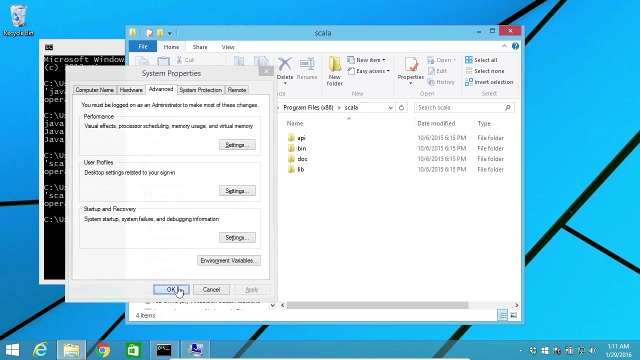 looks like So again, This is semicolon percent- Java: underscore: home percent, backslash BIN. semicolon percent Scala: underscore, home percent, backslash BIN. Now I'm going to click OK all the way out of these settings. OK, OK and OK. I could even close this Explorer now and I am going to close out of the command prompt. 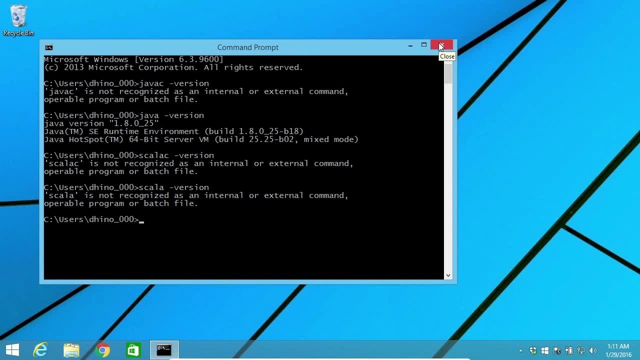 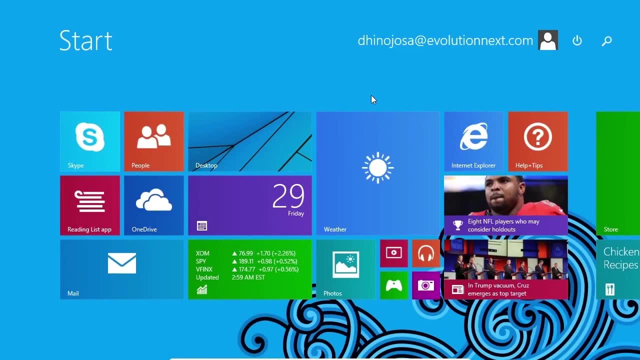 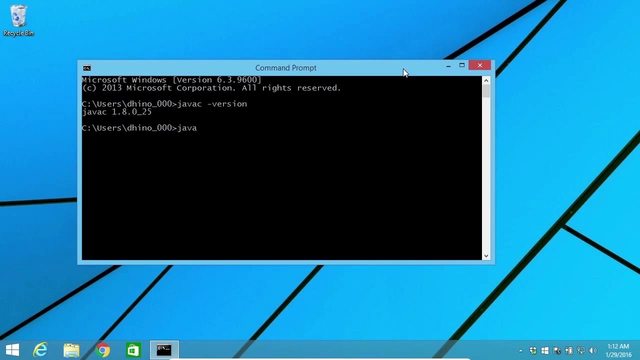 because any settings that I have made for my environment variables will not take hold for any command prompts that are already open. Therefore, I'm going to close it and I'm going to open up a new one. Now let's review our goals. Java C space dash version- great. Java space dash version- great. 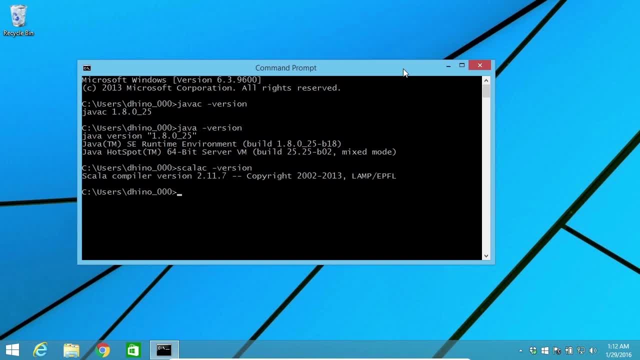 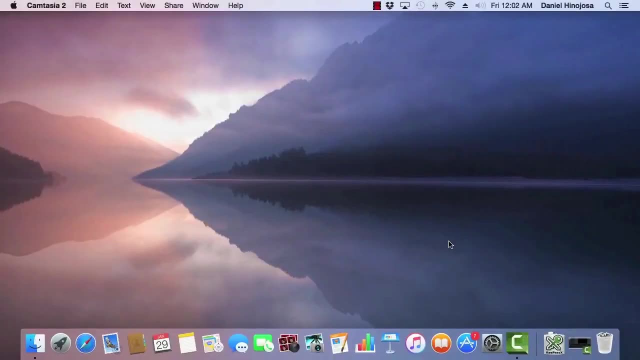 Scala C space dash version- great. and finally Scala space dash version- fantastic. All four pass, everything looks good and we are ready to use Scala in Windows. Here We are in Mac OS X. This is a standard install where bash is the default shell. I already installed the JDK DMG and Java works just fine. In fact, what's great about the Mac installation is that Java C and Java already work, So let's take that for a spin. I'm going to hit command space and locate terminal. 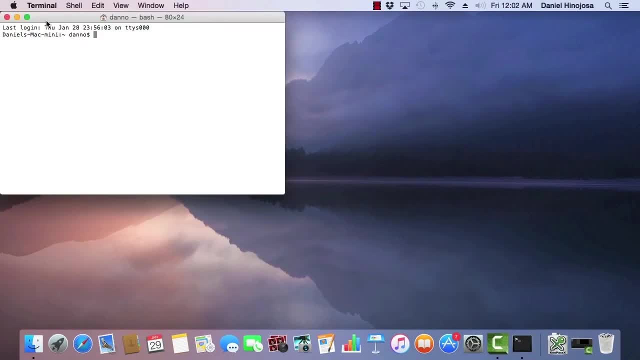 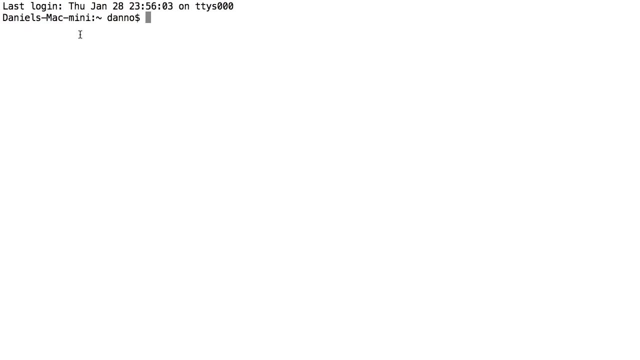 Well, I already had that there, Here's terminal, and let me go ahead and maximize this and let me increase the font. I'm going to do a command plus to increase the font a bit. That should be a good size for it- And I'm going to try out the following: Java C space dash version. there it is and Java. 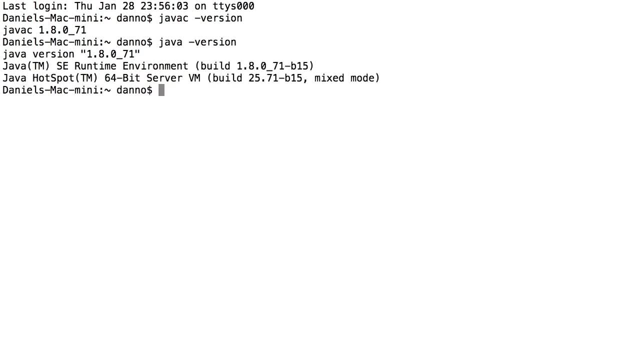 dash version. This should be automatic for us, But what doesn't work is Scala. Now I downloaded a tar file from Scala lang org and I already expanded it, and here it is. It's right over here: Scala 2.11.7.. 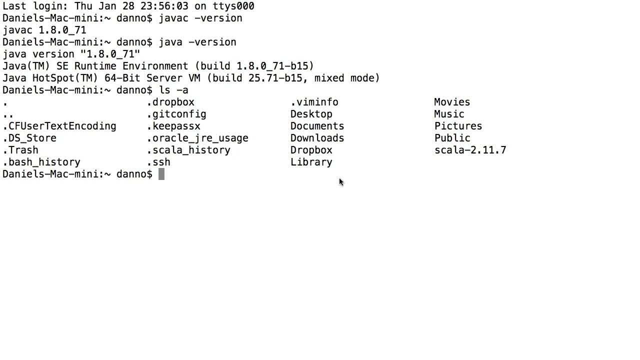 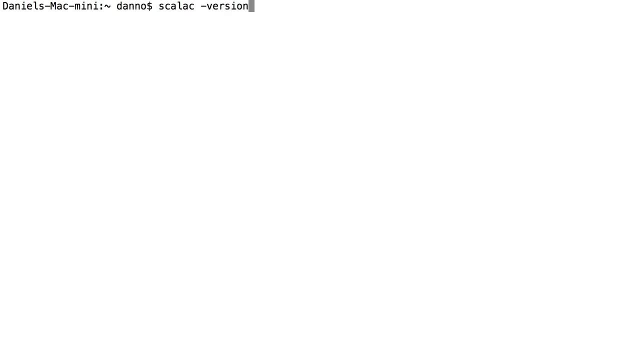 So that works pretty good. What I'm going to do- Let me hit a control L just to start off with a clean screen- Is that once I downloaded this by default this will not show up. This will say command not found. And if I do a Scala space dash version, this will also say command not found. 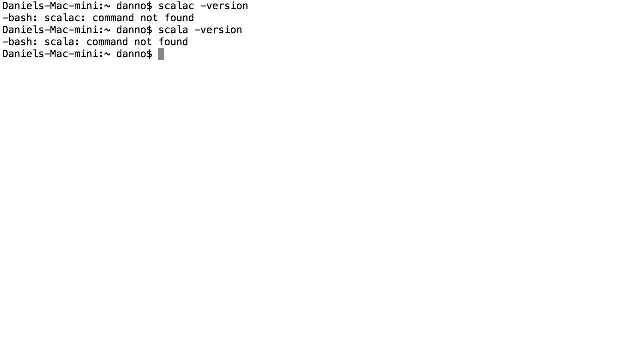 Now, if I install this using brew, like I mentioned in the previous session, everything should be good to go and all your goals should be met. But if you're not seeing the Scala C space dash version or Scala space dash version working, then we'll need to create either a dot bash underscore profile. 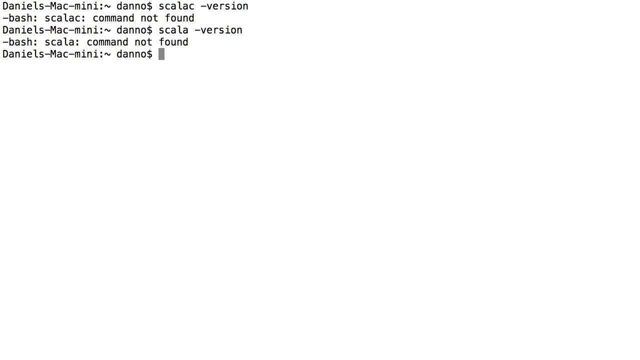 Or In this example, we'll be using a dot bash underscore profile and we will add some entries. So let me get started with that. So what I'm going to do is I'm going to use my favorite editor, Vi. you could use emacs. you could use whatever type of editor is your favorite. 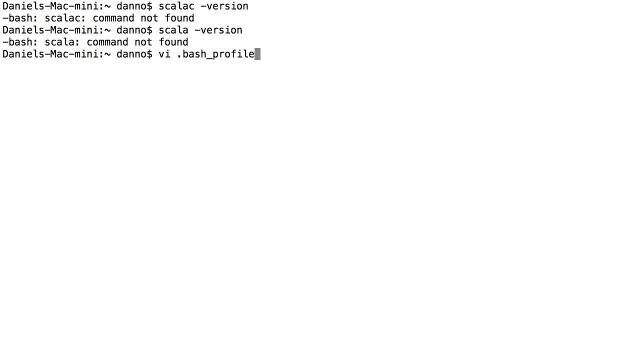 And I am going to create a file called dot bash underscore profile and edit that file. And here we are. I'm going to add the following entries: I'm going to Export Scala underscore home. And again, please use your favorite editor here. doesn't have to be the same one I'm using. 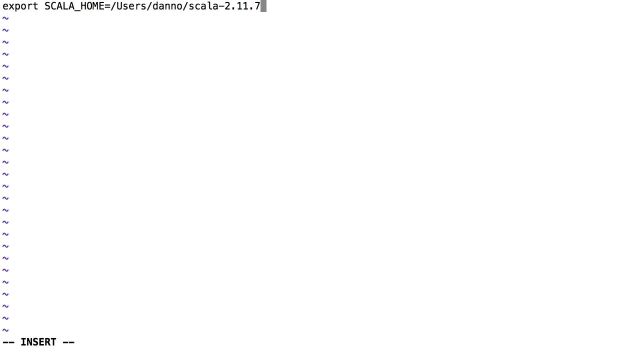 And I'm going to put the location of where I expanded my tar file And it just happens to be under slash user: slash Dano, which is my name. Slash Scala, dash two, eleven, seven. For the next line I'm going to add export path. 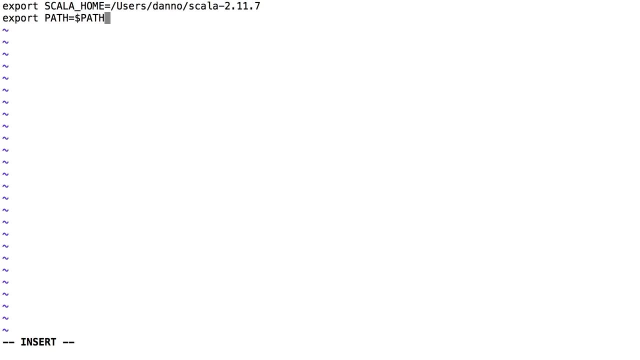 And I'm going to set that equal to dollar sign path. Now that path Is Going to retrieve the path that has already been established on your operating system And bring this in, and what I'd like to do is bring the already established path and 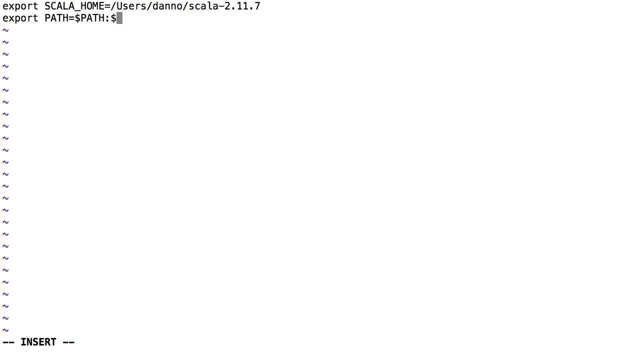 append to it, and I'm going to use a colon, in this case Dollar sign Scala, underscore home forward slash bin b i n. That is it. Now. what I'm going to do is I'm going to save and close this file, And now, on my terminal, I'm going to type the following for the changes: 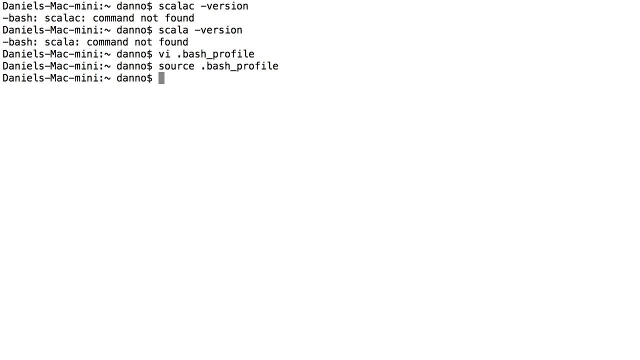 To take In effect Now. let's try our four commands in our shell To ensure that we are ready course. Java C dash version works. Java dash version should work as well. And now Scala C dash version. That works out great. And Scala dash version. 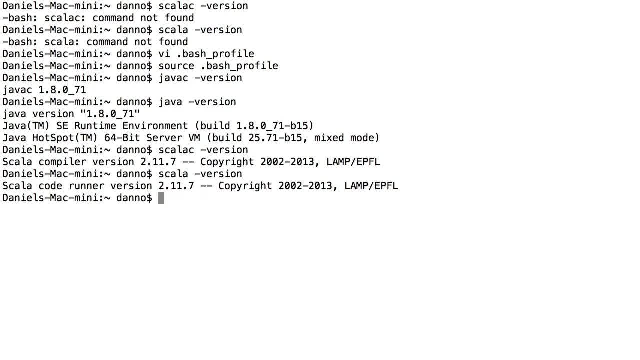 And that'll work out great as well. We are ready to go Now. I want to call what I just did a full on recommendation. Every shell has a set of files met for different reasons and could very well be that dot bash RC is your preferred file. 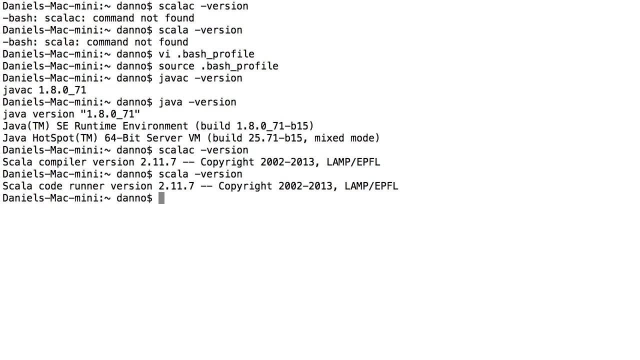 All this depends on your machine, how it was set up, how it is administered. look up any documentation for your OS and your shell. usually there are two different documentations. discuss it with your system administrator as to the best place where to store your environment variables on Mac OS X. if you're the master of your own machine, dot bash underscore profile. 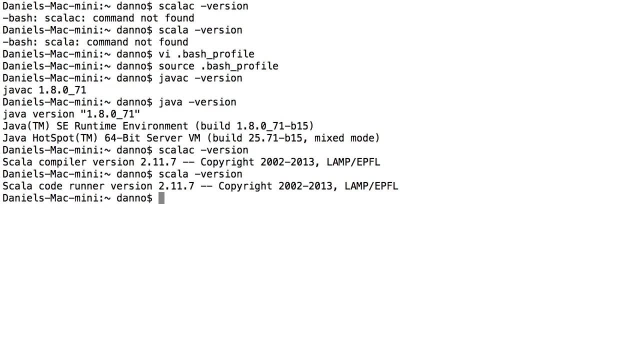 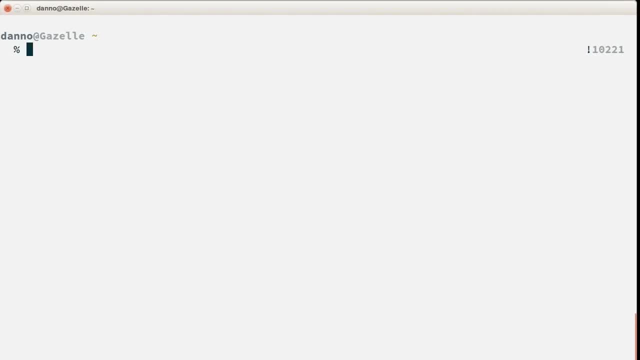 just as we shown here ought to work just fine For the duration of the video series. I'll be using Linux, for Linux users will be nearly the same setup as the Mac. So what I'm going to do is I'm going to open up a terminal- and here it is already- and see: 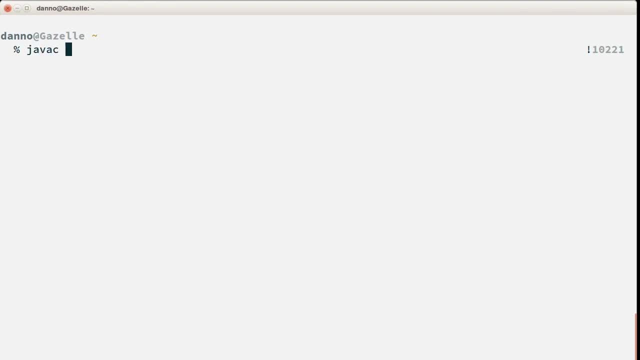 where I am with my four commands. what my goal is: Java C space dash version that works, Java space dash version that works, Scala C space dash version that does not work and Scala space dash version that does not work. So I have two out of four. 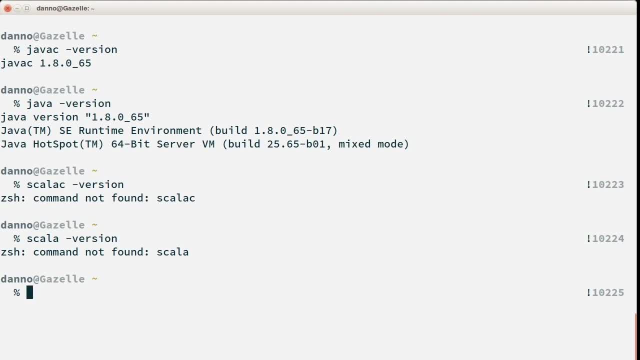 Now for the Linux users. These Java C or the Java may not work. on my particular machine. it is already mapped to Java C and Java using something called update alternatives. check it out. it's a really great way to set up Java and you're able to choose which version you want. 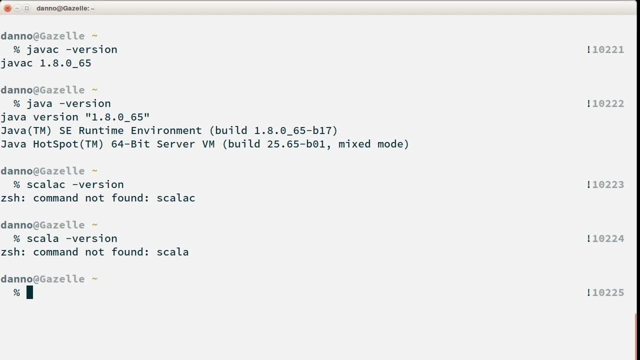 Now for my example. while it is working well, I'll still have to map Java home in order for everything to work correctly And, as you can see, my Scala C space dash version and my Scala space dash version does not work, So I need to fix that. on my Linux machine, I'm using Z shell. 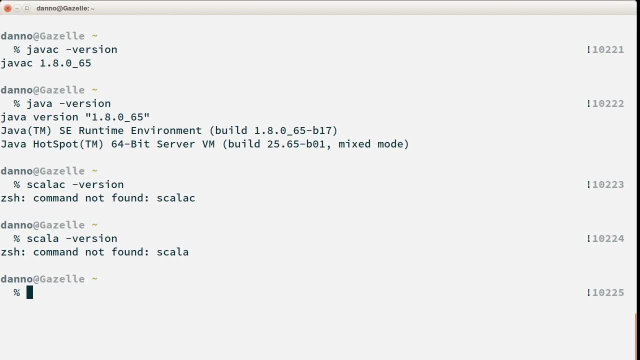 So what I'll need to edit is my dot zsh RC file to add my environment variables. Now you could use whatever shell you want. The most popular shell that is in use, of course, is bash, followed by, I believe, Z shell, and either one of those are going to have their own particular files that you need to edit. 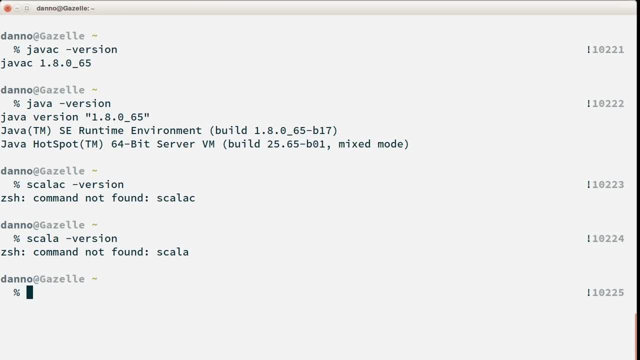 to set up the environment variable. So, if you're using bash, edit your dot bash underscore profile or your dot bash RC. If you're using zsh, I'm going to be editing my zsh RC Now. I just told you the names of two popular shells that you can use with Linux. 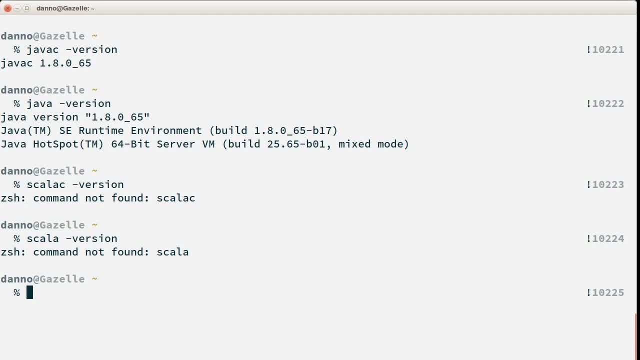 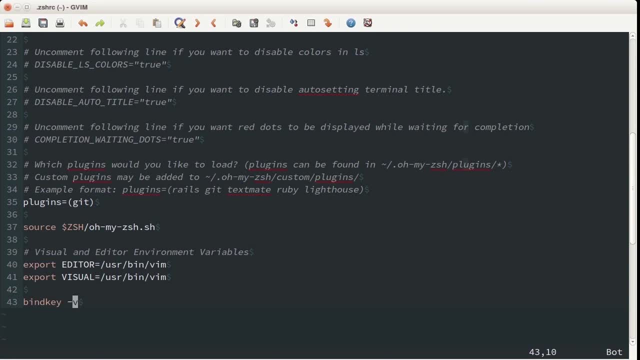 There are a lot more. Now I'm going to open up my zsh RC, and here it is, And in this file I'm going to add my Java underscore home with the location of the version of Java that I wish to use, And I'm also going to create a Scala underscore home with the location of where my preferred. 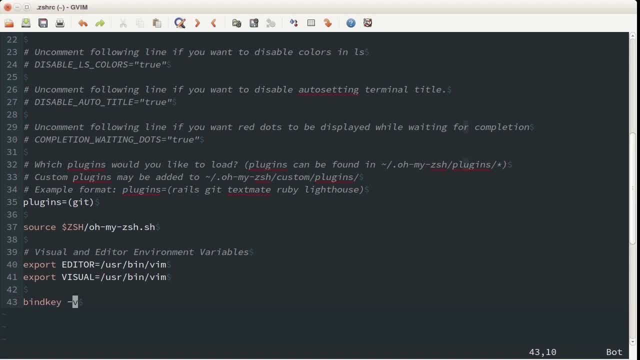 Scala will be located, And then I'm going to take the location of all those and add them to my path. So here's a zsh RC and already has some information that zsh needs, and I'm going to add the following. First off, I'm going to add the Java home, which is user lib JVM. 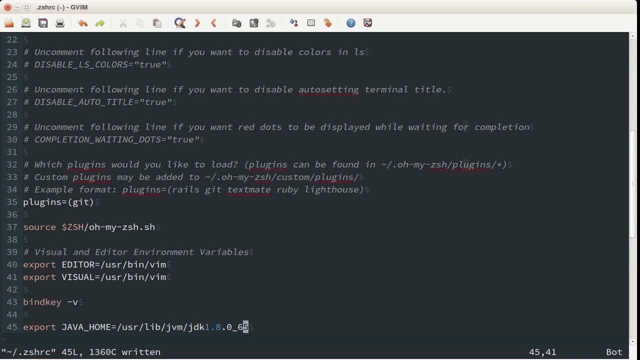 Now this is going to be different for everyone. This just happens to be the location on my machine. it could just very well be that this would be in your home directory And you can add whatever path your JDK is located on, So I'm going to go ahead and do that. 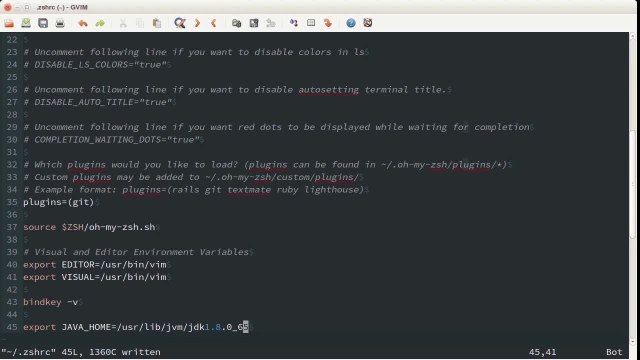 So I'm going to go ahead and do that. And you can add whatever path your JDK is located on. So I'm going to go ahead and do that. The path that is located on to this line. So export Java home and then the location of your JDK. add a few lines here. I'm also. 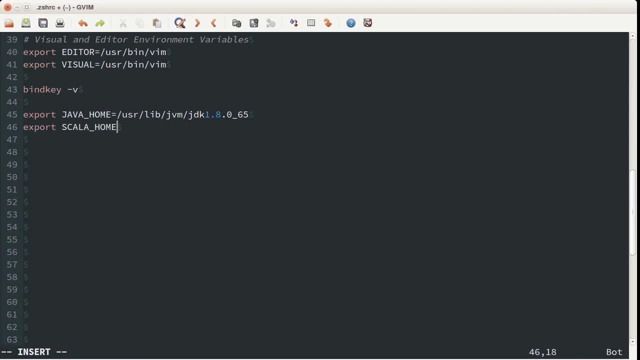 going to add export And I'm going to include my Scala home, So be located under home: Dano, Java and Scala two dot 11.7.. And then, finally, I'm going to export a path and very much like we did with the Mac, I'm 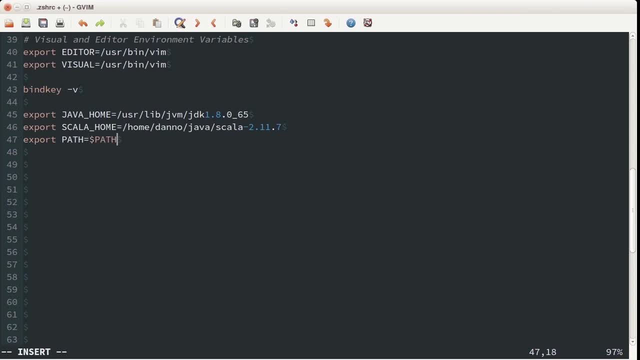 going to set this equal to the path that is already established. colon dollar sign java underscore- home forward slash bin. that's different than windows. make sure it's a forward slash. colon scala underscore- home forward slash bin. now i will save the file and now i will. 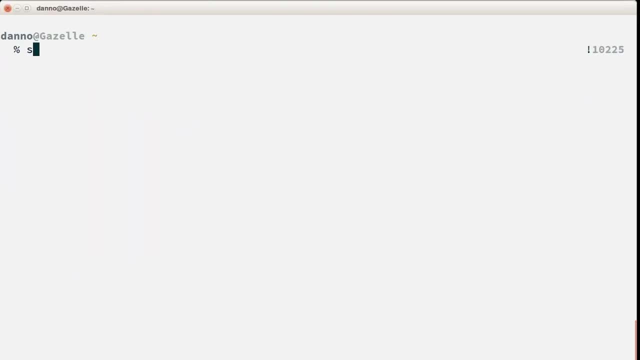 go to my terminal, i'm going to hit control l and i'm going to run source with that file, zshrc. that way, all those changes will take effect. you can either type sourcezshrc if you're using zshrc. if you are using bash, then you would type in sourcebash underscore profile. i just happen to. 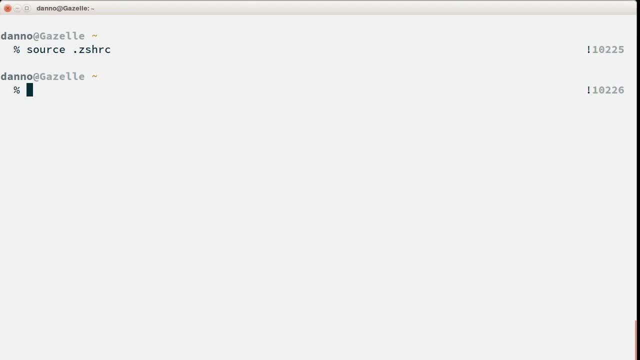 be using a different shell for this example. the other alternative is to close out the terminal and open up a brand new one. so let's go through our goals. control l. java c dash version. okay, we already knew that one worked, at least it did on my machine. java dash version. scala c dash version. 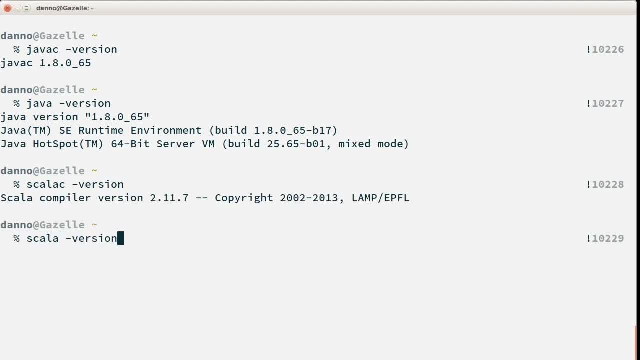 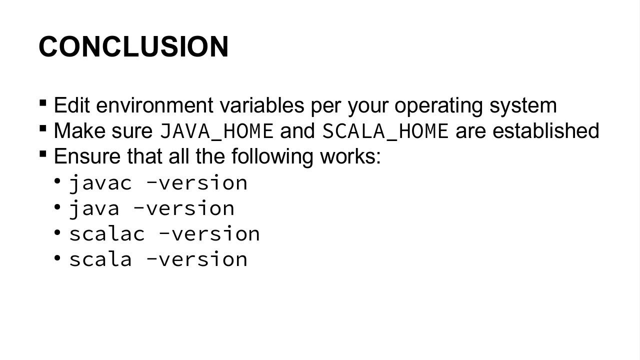 fantastic. and then finally you, and if it all works, we're good to go. and we showed you how this is set up in windows, mac osx and linux. so, in conclusion, edit the environment variables per your operating system, make sure your java home and scala home are established and ensure that the following works: java c: 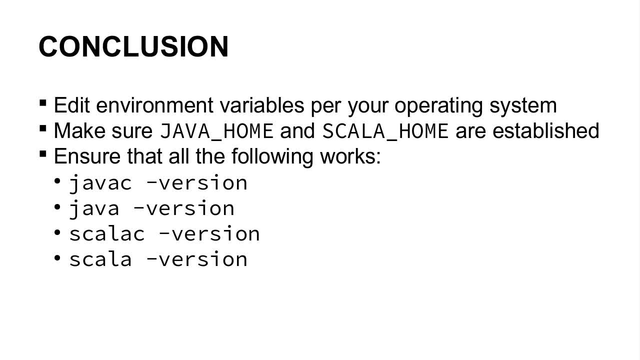 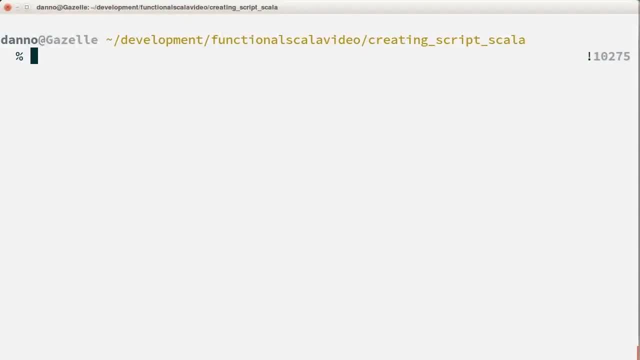 space dash version. java space dash version, scala c space dash version and scala space dash version. build full custom java and create a java file. in this section we're going to talk about how to create a script in scala. for many java programmers out there. you may not be quite as familiar with scripting. 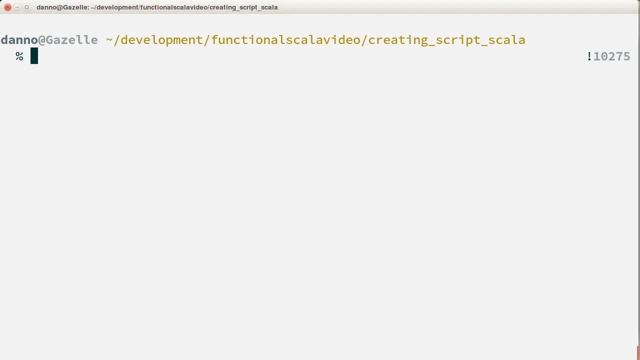 although you may have played with a little bit of scripting in other programming languages, but in scala there's no need for a compilation or a public static void main string args. although scala programmers tend to compile their code just to make it fast, there is no requirement to do so. 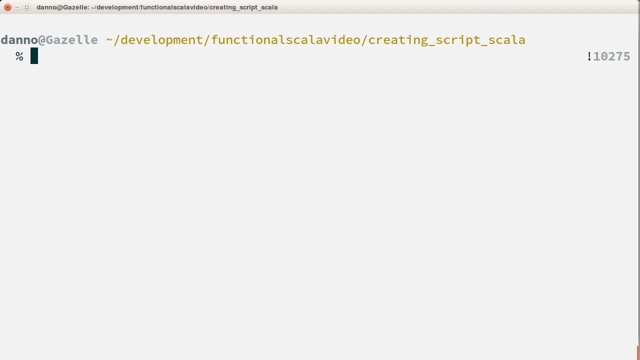 so what we're going to be doing in this section is we're going to be creating a file, a script- script, again, without a public static void, mainstream args and without compilation. For this you'll just need an editor. There are plenty of great ones out there. 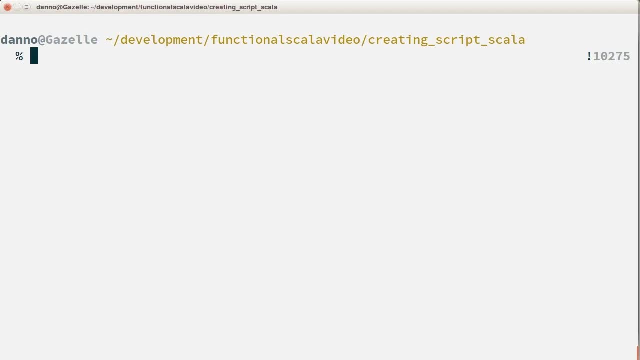 There's Sublime, which has Scala syntax highlighting. There are some other editors that don't have syntax highlighting, but they're great nonetheless, like Notepad++, TextPad, UltraEdit, Visual Studio Code. For those who enjoy the classics, there's always Vim and Emacs, and there's plenty of. 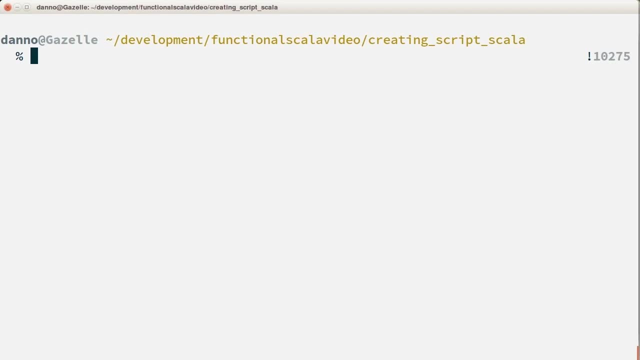 syntax highlighting for Scala for both of those editors. If you want to add a code with any IDE, there's some great ones out there. There's Eclipse and you can download Eclipse with a plugin called Scala IDE which you can get at ScalaIDEorg, or you could go to ScalaIDEorg and download an actual full-blown. 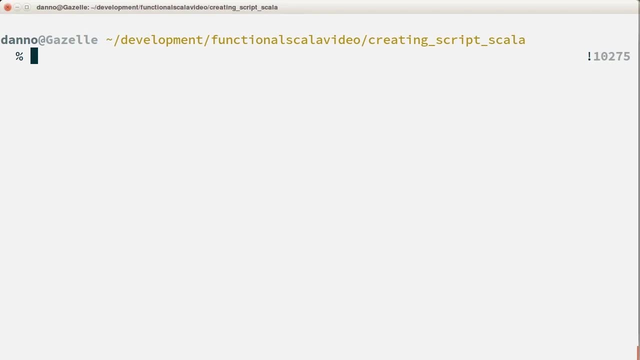 IDE, with all the plugins readily available. There's also IntelliJ. Once you download IntelliJ, go to the plugins and you can download the Scala plugin from there and edit files. There's NetBeans, which also has a Scala plugin, And if you want to stay with Visual Studio Code, you can download the Scala plugin from. 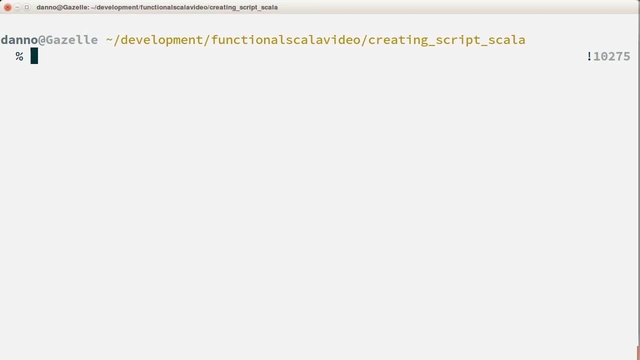 there and edit files. If you want to use Visual Studio, then you can use Visual Studio, but there won't be any syntax highlighting for Scala. What I'm going to do is I'm going to start off with a script And I have a folder here called CreatingScript- Scala, delimited by underscores. 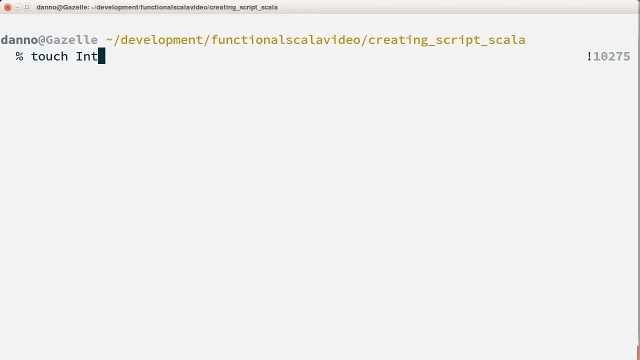 And what I'm going to do is use touch to create a script called introscriptscala. Once there, I'm going to bring this up in my editor, Just so you know. there's no touch in Windows, So if you want to create this in the Windows operating system, then you can just go ahead. 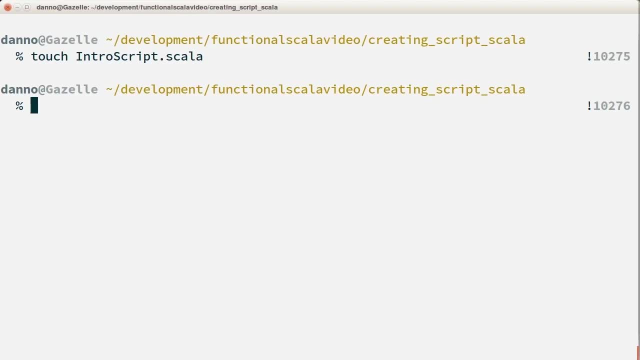 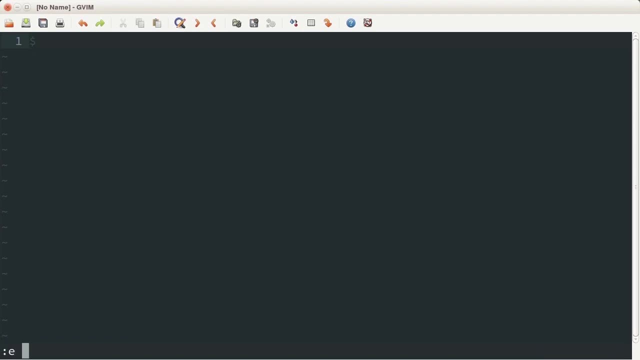 and fire up an editor and create the file from there. Once I have this available, I'm going to hop over to my editor alt tab. Now, once I'm here in my editor, what I'm going to do is I'm going to go ahead and open up. 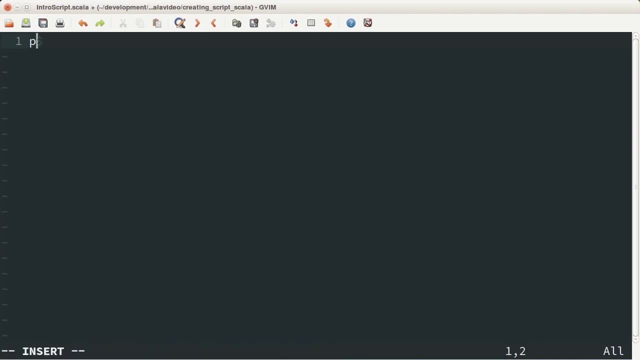 that file that I just recently created, And I'm going to get started with something very simple. I'm going to do a print line for all the Java programmers coming in. There's no systemoutprintln, We just head straight towards it and do a print line. 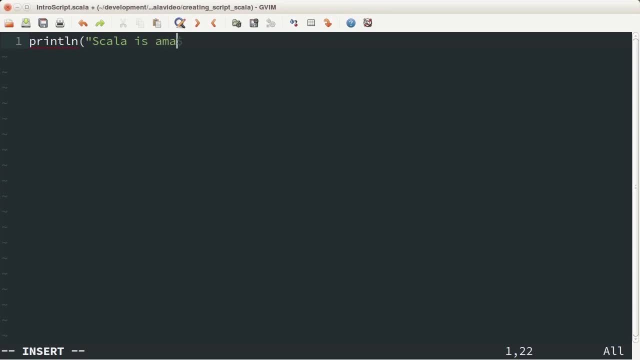 I'm going to do an open paren and a quote and stay here That Scala is amazing, Amazingly concise. Close the quote, Close the paren And we're good to go For Java programmers. you'll notice something is missing: The semicolon. 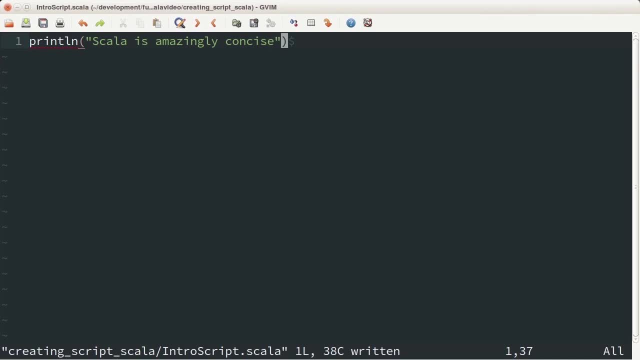 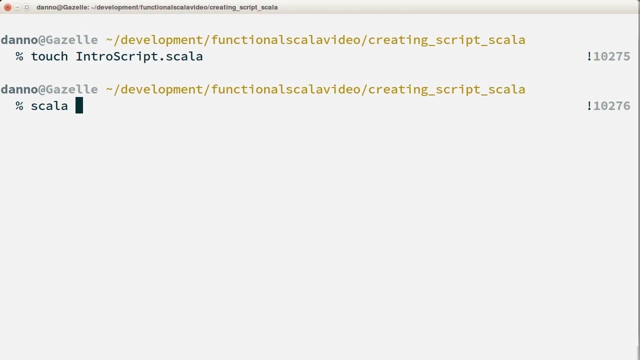 No need for a semicolon in Scala. I save the file and we're good to go. I'm going to alt tab over to the terminal Once I'm here in the terminal. now I can just type in: Scala- introscript- Scala. Again, there's no compilation involved with this. 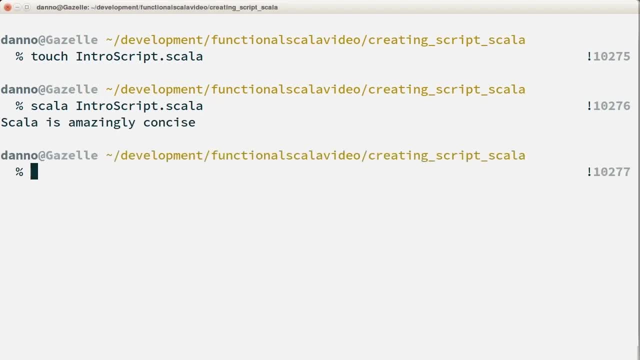 It is going to be interpreted, It is going to run quickly And we'll get a. Scala is amazingly concise. That's how easy it is. Again, no compilation involved. Now what if I want to create a shell script that I could run on Mac OS X or on Linux? 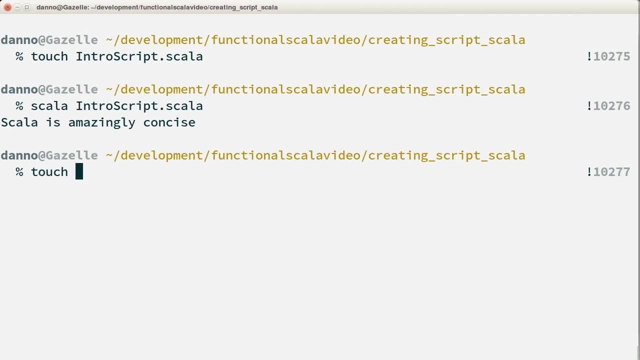 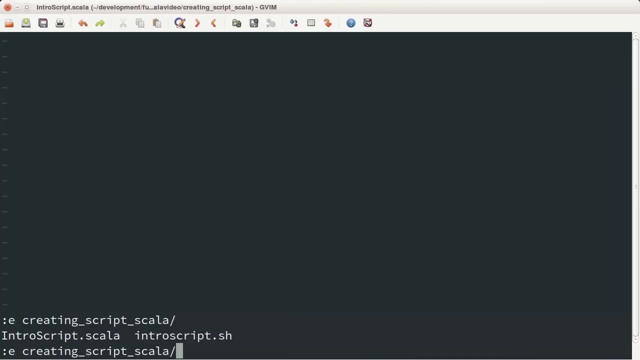 Let's go ahead and get started with that. I'm going to create a script called introscriptsh, Not a Scala extension, but a sh extension. Now I'm going to head to my editor. Here in my editor, I'm going to edit the file. 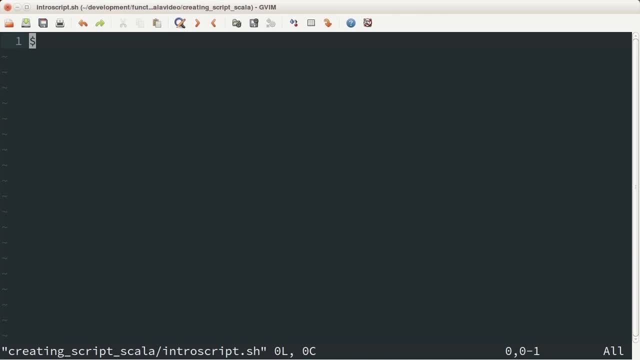 Called introscriptsh, And for the first line, I'm going to include a hash and a bang And I'm going to specify that I want to use sh for the shell script. The next line, I'm going to specify that for this particular script, I wish to execute. 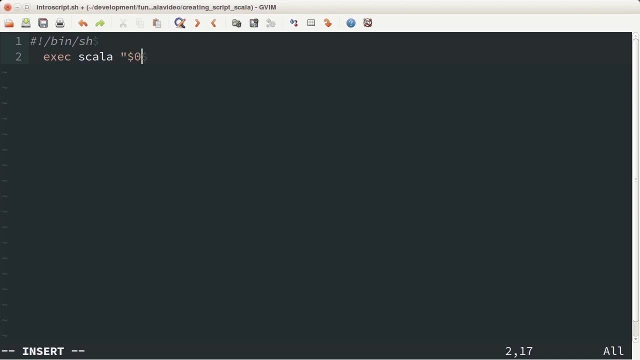 Scala. This funny argument that I'm going to type here, specifies the name of the file. And this next funny argument that I have here is going to be for all of the arguments for Scala, For this particular script. I'm going to close things up with bang and hash. 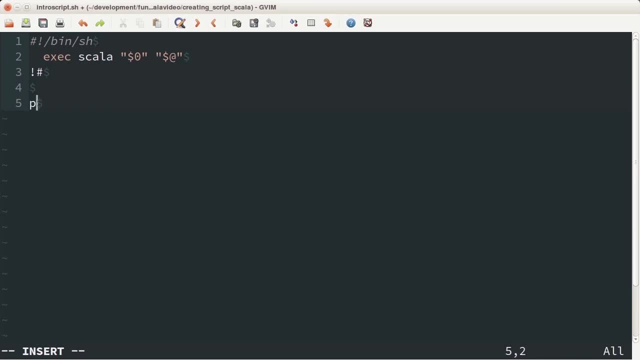 Once I'm done with this three line prefix, I'm going to go about this using just plain Scala. So I'm going to do a print line and again specify that Scala is amazingly concise. Close the quote, close the paren and I'm going to save the file. 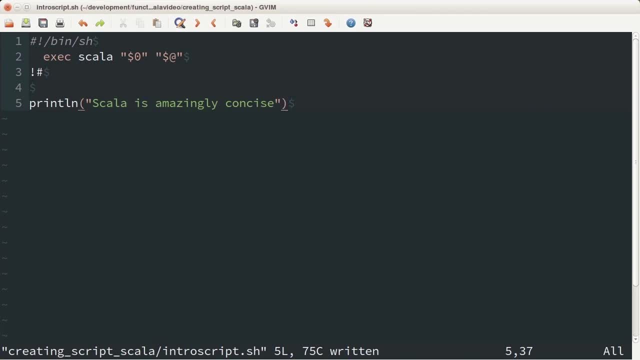 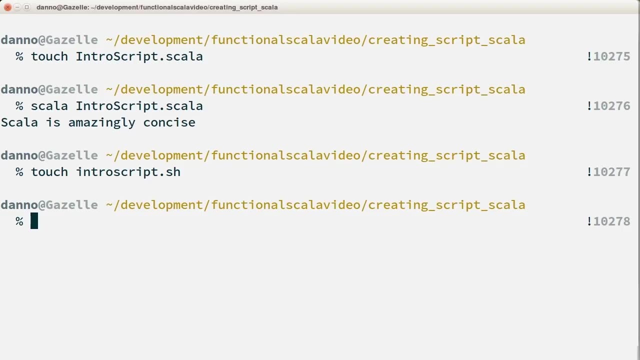 And that's all there is to it. With that three line header, that's enough information to provide for our shell script to run as a script. So let me head over to the terminal. Now that I'm here, there's one adjustment I need to make. 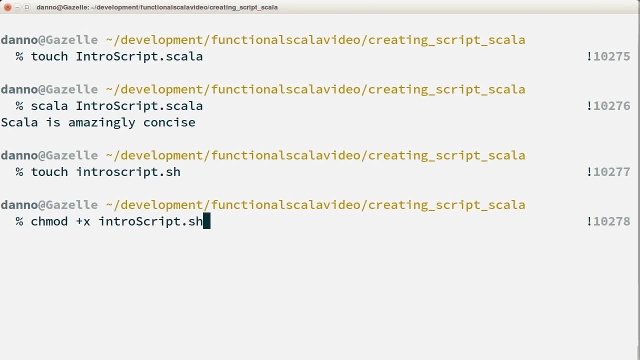 I need to make sure that this particular file that I just wrote is executable, So I'm going to chmod plus x, which turns the flag on, to make it executable. introscriptsh. Now I can just run this just like any other shell script. 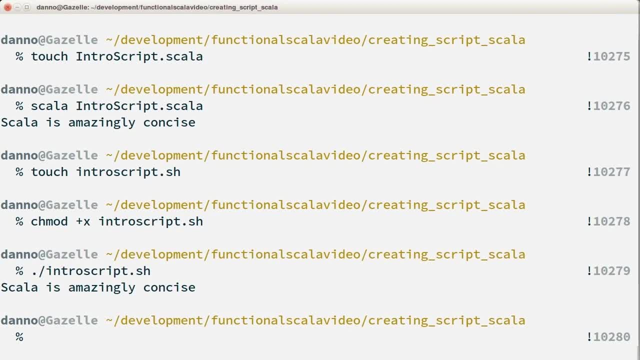 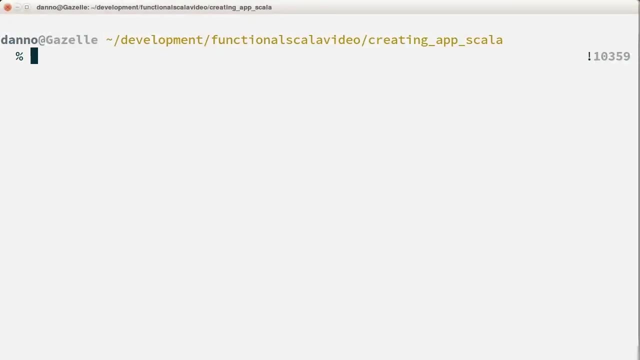 And, as we see here, it specifies that Scala is amazingly concise. That's how easy it is. It's fast setup And once you become familiar with the language, This might be your preferred scripting language for days to come. In this section, we're going to talk about how to create an app in Scala. 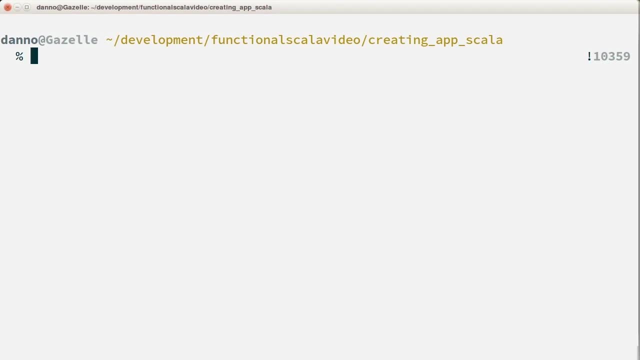 The previous section, we created a script which was interpreted. Now we're going to be creating and compiling source code, which then becomes JVM bytecode, which then we can use to run or make it a part of a library. Now, for this section, we're going to need an editor. 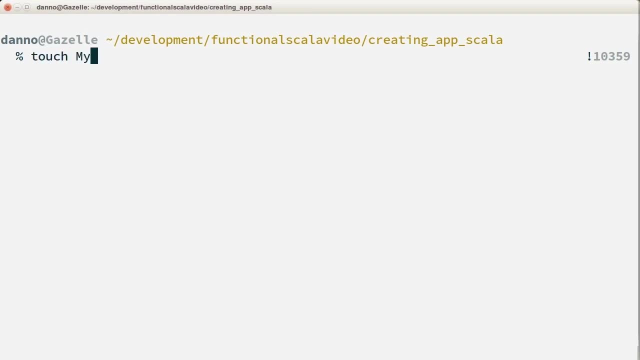 And what I'm going to do here in the terminal is I'm going to start off by creating a file called App dot Scala. Now I'm going to bring this up inside of an editor, Alt tab. inside the editor, Let me bring up creating app Scala, which is the folder where I'm placing this Scala. 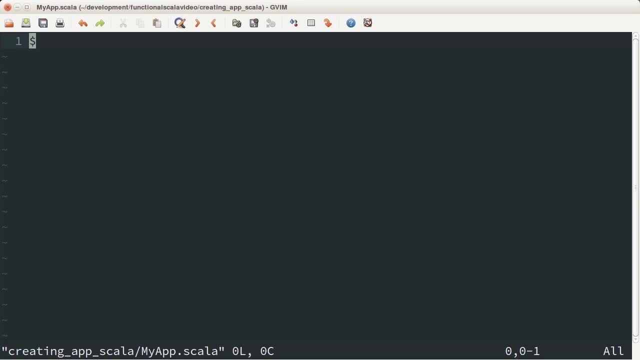 file I'm going to bring up my app dot Scala. So inside of this file I'm going to start off with a very basic class. I'm going to call this class employee. There's no need for public. Everything is public by default. 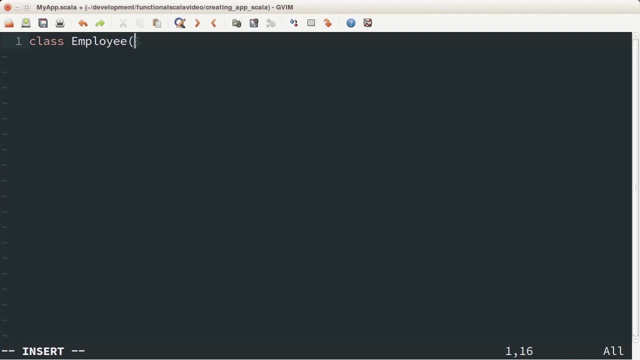 And I'm going to start with an open paren. I'm going to start adding the properties. First property I'm going to add is first name, followed by a colon, then the type. If you're coming in from Java, this is reverse of what you expect. 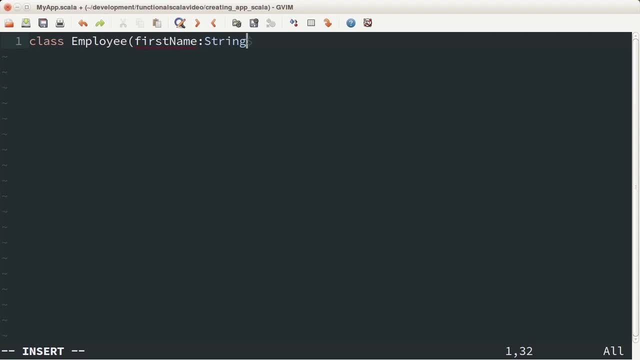 In Java you expect to do a type first than the name of the property or variable name inside of Scala. We'll do the property name first colon, then the type and I'm going to add last name followed by the type. at the very basic level. 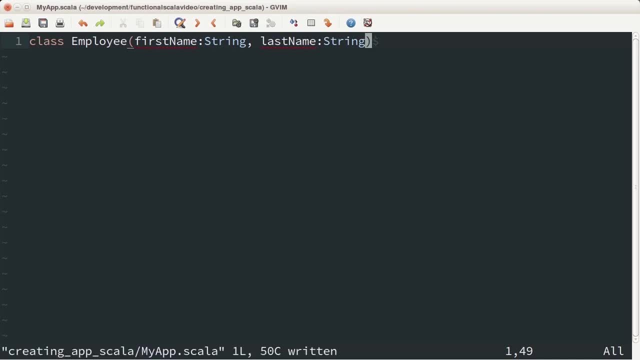 This is not all we need, but it's sufficient, So I'm going to save this file. Now, if you're coming in from Java, you're going to notice something a little bit alarming: The class name is called employee, but the file name is called my app, dot Scala. 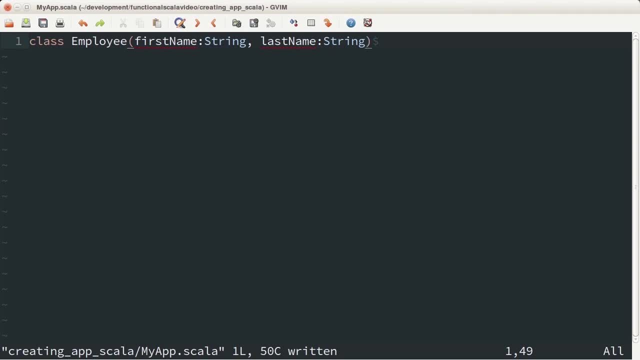 The Scala compiler is going to allow. this Scala compiler is going to do a lot of things for you that you don't have to particularly think about all that much. In fact, you could even create multiple classes within the same file. Let me show you an example. 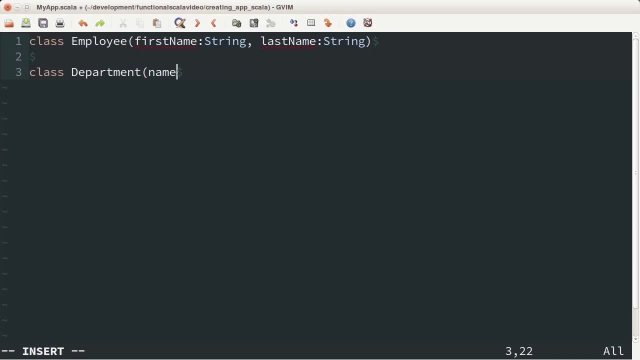 Let's say I want to create a class called department And the department has a property. I'm going to create a class called department And the department has a property. I'm going to create a class called department And the department has a property called name, with the type string. 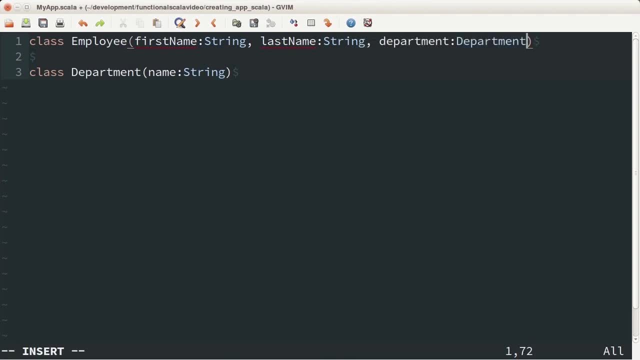 In fact, I could also make it a part of this employee class. So now this employee has three properties: first name, last name and department. I have two classes within one file- Pretty amazing. I'm going to go ahead and save the file. 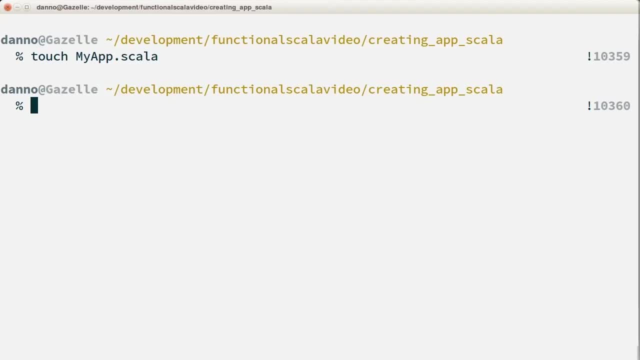 And now I'm going to switch over back to the terminal. So back in the terminal, I have one file. Let's take a look There. it is my app dot Scala. Now what I'd like to do is I'd like to compile this file, and I'm going to do so with Scala C, which stands for Scala compiler. 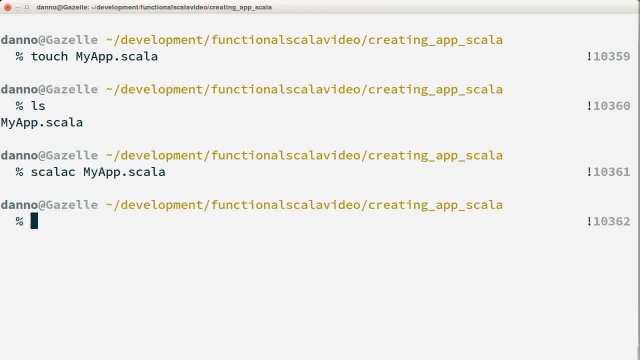 And I'm going to specify the Scala file that I wish to compile. Now that I'm done, let's take a look at what is inside my folder. Now I created two classes inside of my app, dot Scala, And when I compile it, what it's going to do is it's going to create two Java class. 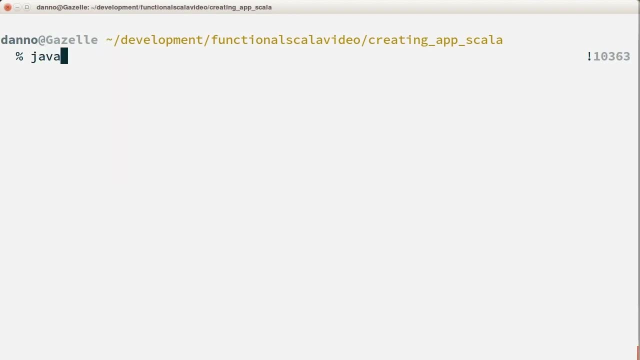 files. Now, if I want to take a look at the class files, I can use Java P, And Java P will allow me to introspect these class files. I'm going to use Java P, space dash P. Dash P allows me to view a lot of private information. 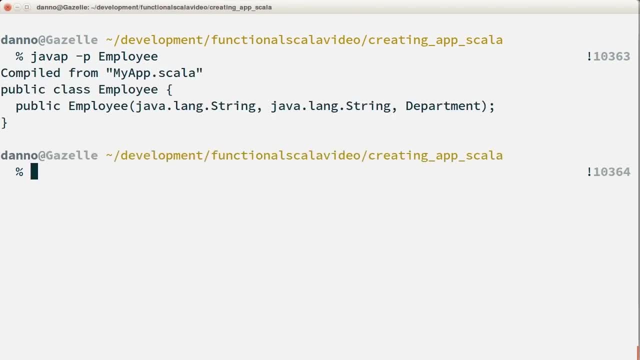 within this particular class file, And I'm going to specify employee, And when I do so, I could take a look at the internals of the employee class that I created. This is Java, And this says that I have a class called employee. 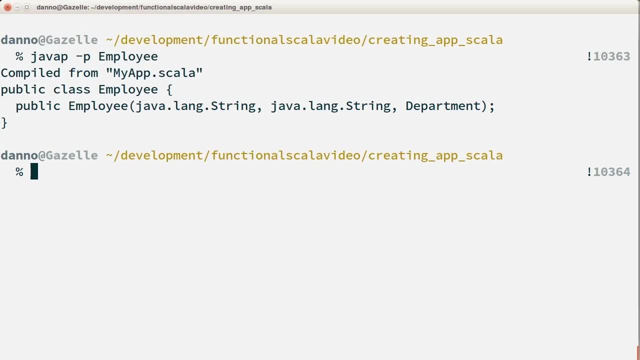 And I have a constructor called employee, with three arguments: First one's a string, which represents the first name. Second, one's the last name, which is a string, And then finally a department. Again, this is all JVM bytecode. Now, let's say I wanted to get organized. 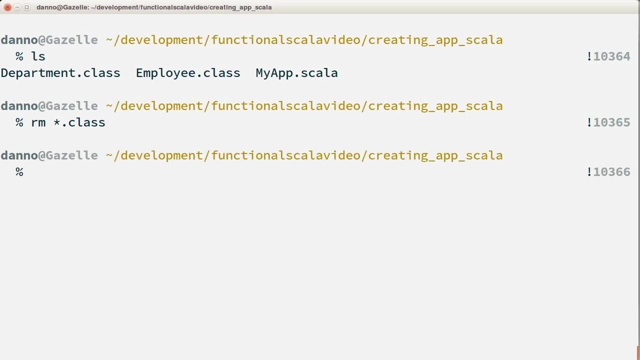 What I'd like to do is I'd like to remove the class files from here. They could always be regenerated using the compiler, And here's my, my app, dot Scala. What I'd like to do? let's say I want to create a source folder and I want to create a classes. 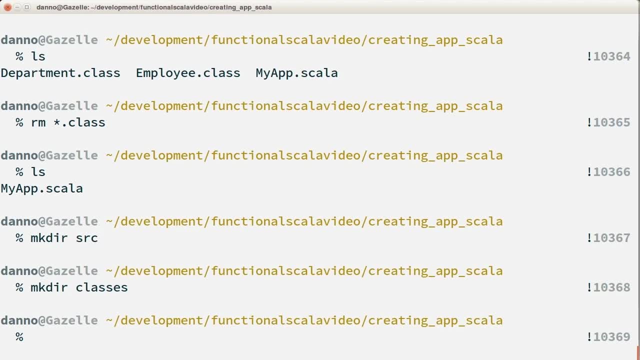 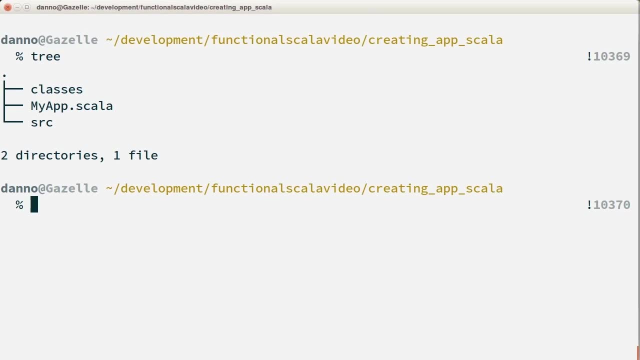 folder where all the compiled classes will be placed. Let me do a tree to show you what that looks like. Now, tree is freely available for Mac OS X and Linux. For Windows, there's also a tree. The only thing that you would have to do is make sure that you specify that you want to. 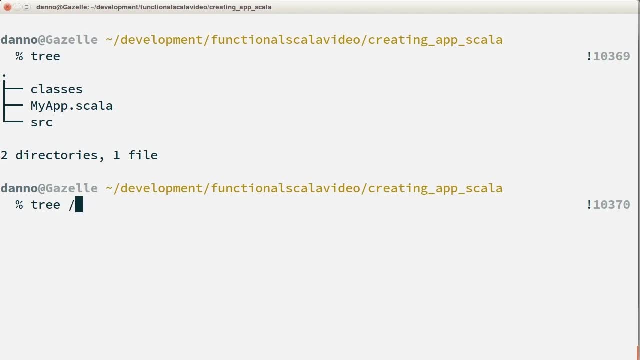 see files as well, But this is available to all Windows users, So what I'd like to do is move my app dot Scala, into the source folder. I'll go ahead and do that right now and do a tree to see where we're at. 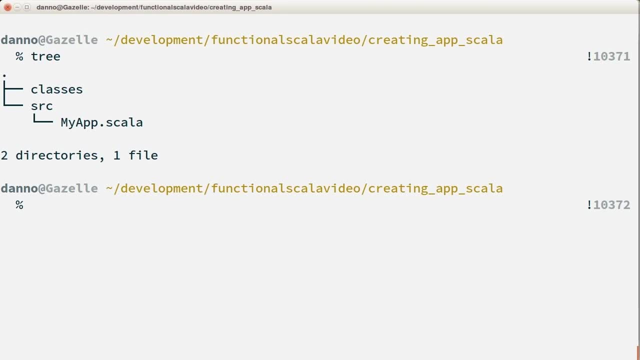 So I have my app dot Scala inside of the source folder and I have a classes folder to compile to. Now, if I want to compile my app dot Scala, I can use the Scala compiler, And I'm going to use a switch called D which will allow me to specify where the class files. 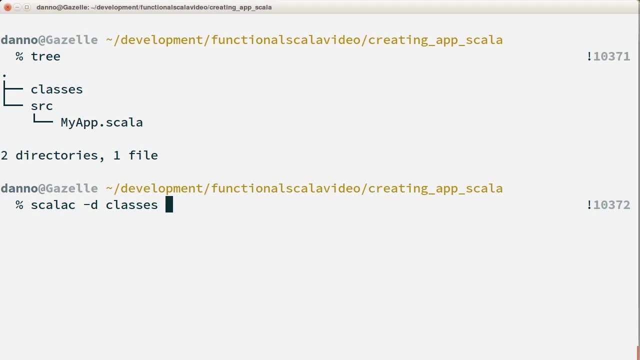 will be sent to. I'm going to specify that this should go into the folder called classes. And now I'm going to state that for the source files, I want you to look inside of the source folder and look at any Scala file within it. 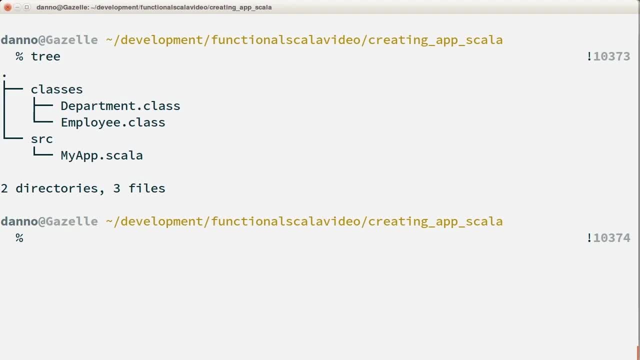 Now let's take a look at the tree. All the class files are inside of the class, So I'm going to go ahead and do a tree. All the class files are inside of the class folder and the source files still stay within the source folder. 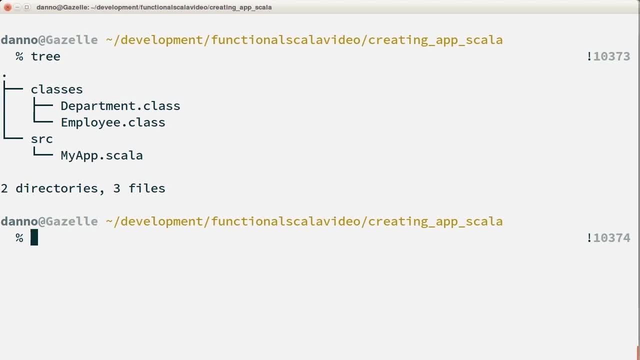 And that's using the Scala compiler. Now I have to warn you this: my app dot Scala is for compiler use only. If you're going to compile it, you cannot run it as a script. Let me show you an example of that. 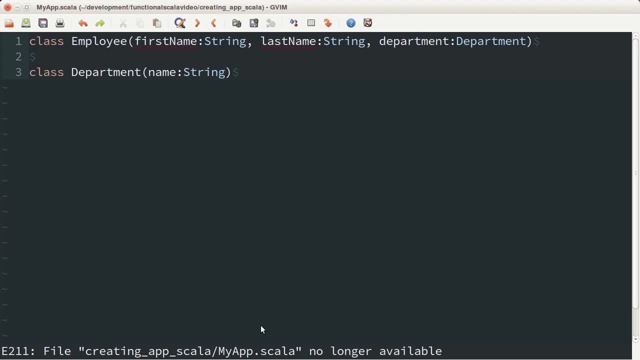 I'm going to go back to my editor. This says right down here that the file is no longer available, which is true, So let me go ahead and bring this up. This is now under the source directory under my app, Scala. Make sure we're editing the right one. 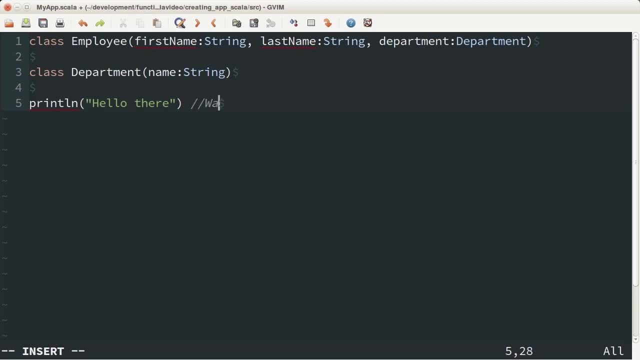 But let's say I want to treat this like a script. Again, warning this will not work Because I have two classes here. that's fine, I can compile that, But the print line right here is now going to be treated as a script. 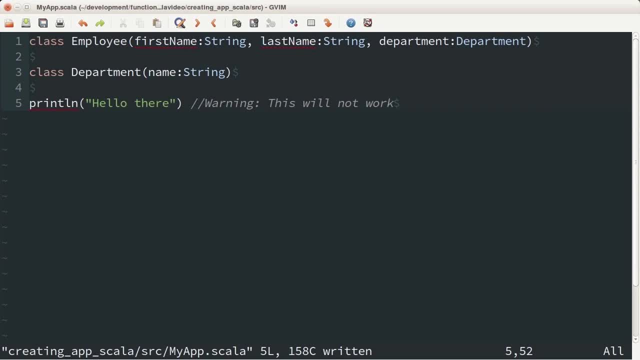 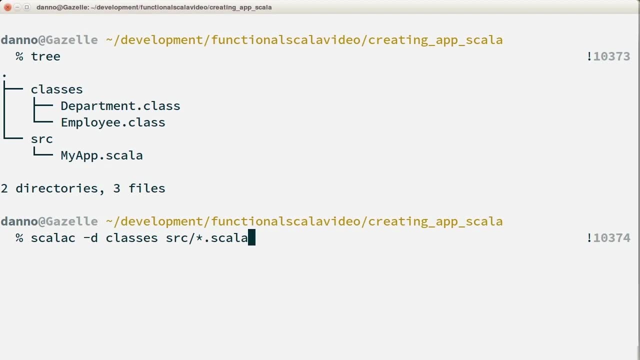 Now. I could run this as a script, but I cannot compile it. Let me show you what that looks like. I'm going to bring up the previous command that I had before. Again, my app is inside of the source folder and inside of the class file. 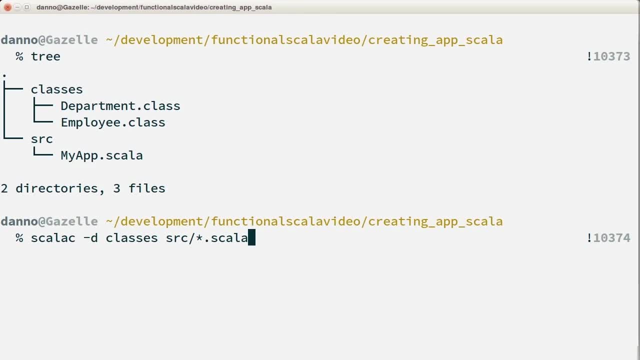 This is where everything is going to be compiled. If I'm going to compile a Scala file which is modeled as a script, I will get this expected class or object definition. It doesn't know what to do with that print line. I can run it as a script and there's nothing wrong with doing that. 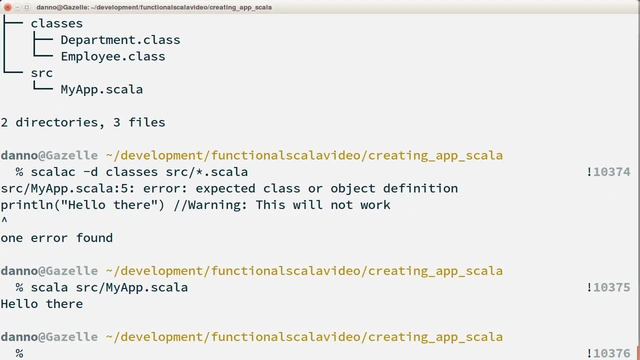 I just can't compile it, So you'll have to know the difference. And this sums up how to create an app inside of Scala. So you could either choose compilation Or you could choose interpretation. But when you choose compilation, be sure you compile code that is not a script. 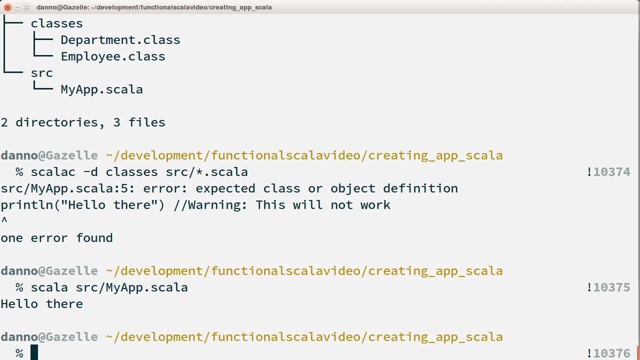 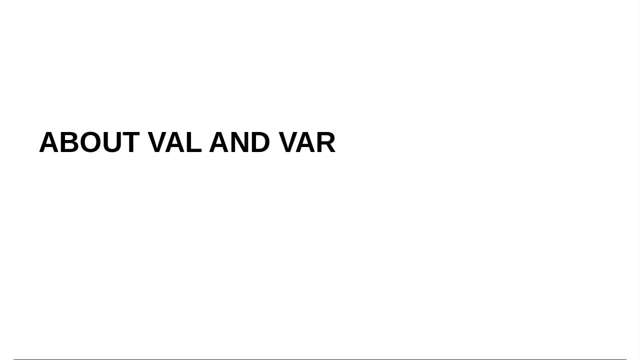 To recap, source code can be compiled or can be interpreted. If you are going to compile, use Scala C. If you're merely going to interpret it as a script, then just run Scala on that file. In this section we're going to talk about Val and Var. 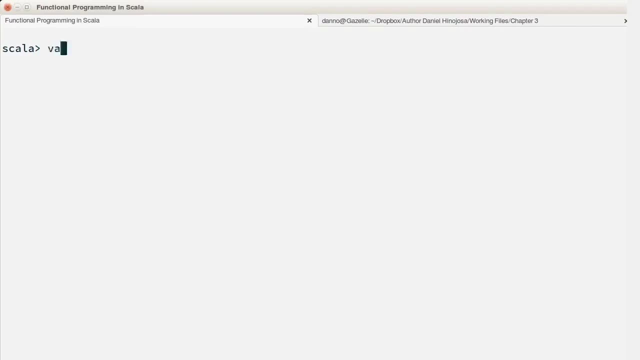 In order to do so, I'm going to head over to the REPL And here on the REPL, what I'm going to do is I'm going to declare val and var, Then I'm going to run the file. So let me run this. 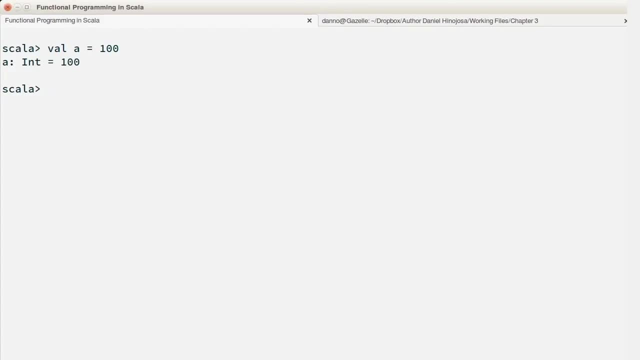 And here on the REPL, what I'm going to do is I'm going to declare val and var is equal to 100. I am declaring what's called a value, and a value is not reassignable. This is analogous to final in the Java programming language. Let me show you what happens if you. 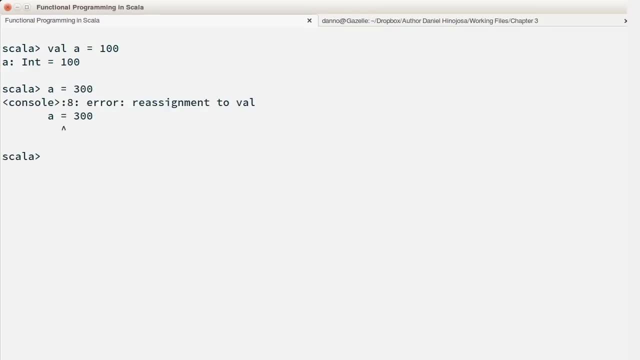 try to do a reassignment, you'll get a reassignment to Val. Now, opposite of this is a variable. It's a variable because it varies. you can change the content. So if I have rb is equal to 400, I can reassign that at any time. I cannot, however, change the type. This is a static. 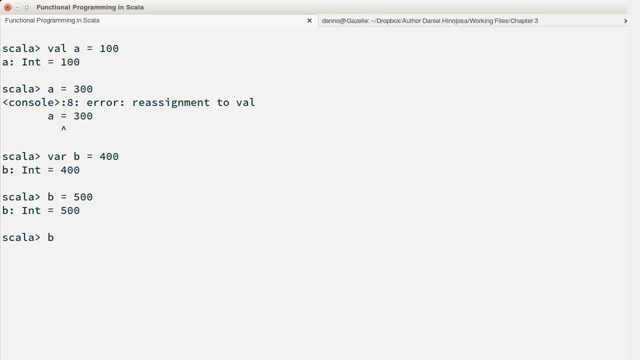 type programming language. So once it's already been established that B is of type int, I cannot make it a string. Scala programmers will prefer the use of Val over var, And var are used in things like actors and other controlled environments, like in a single method, where 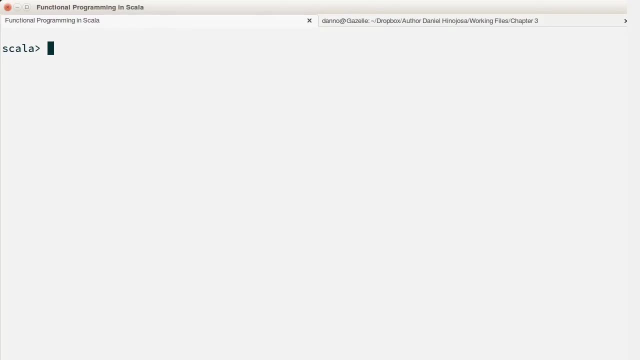 there's only one thread and it's being used to create an object, A lot of projects. you'll need to reassign that at any time. So if I have rb is equal to 100, I can reassign that at any time. 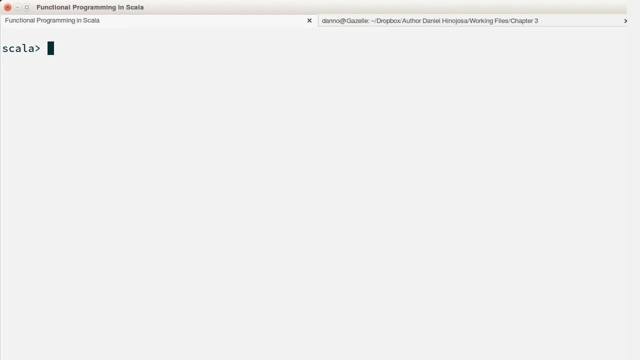 reflect why it is you're using a var and having a fairly good reason as to why you want to use it. Let's show another example. Let's say I have Val a is equal to 400.. Once again, and we'll see here. 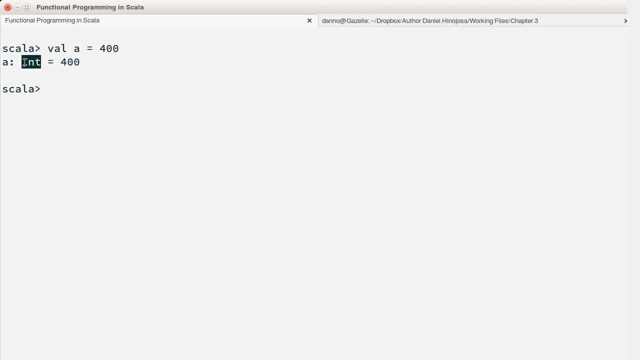 is. something else happened. This says that this is of type int, But did I declare so? No, What happened here is that Scala inferred the type for us. we could be explicit, if we want to, by stating that a is of type int and then specify the integer: But the type int is of type int, And. 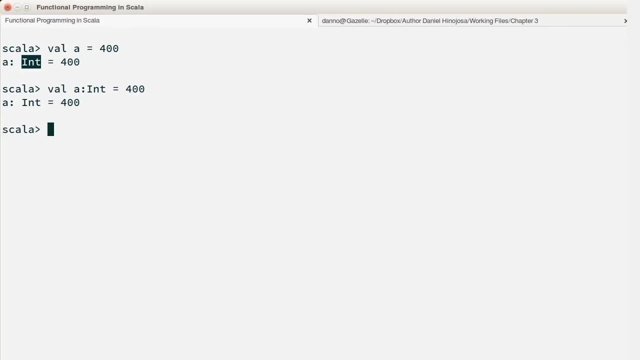 type inference does a fairly good job of knowing what type this is before declaring it. Now, if I wanted to change the type- let's say, instead of Val a of type int, I wanted to make it a double- it will then make the appropriate actions to make sure that the type for a is of type double, And 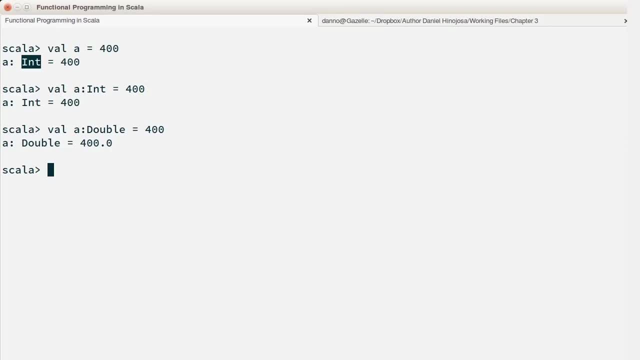 in fact, the content now is changed to 400.0, which is of type double. it is not an integer, it is a floating point. That is one way to change the type. Now, both of these are declaring types explicitly. the Val a colon double is not only declaring a type explicitly, but it's also 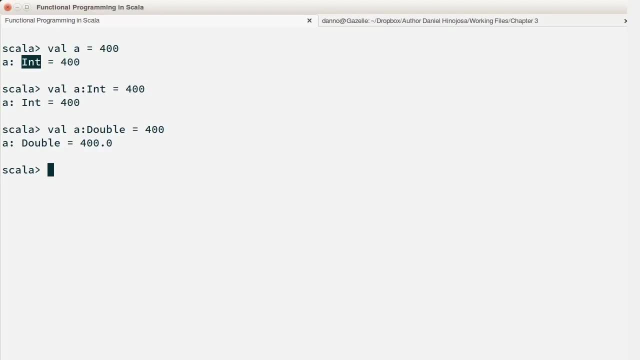 coercing that 400, which is of a type integer, and coercing that into a type double. We could also do a coercion. if I specify something like: Val a is equal to 400, colon double. This is essentially after the fact. what's happening here is we are creating an integer of 400, then we're placing 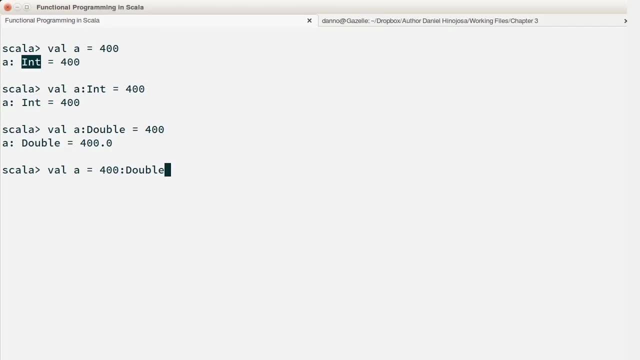 in the colon double, which in turn is going to coerce this into a double. And we're going to create an integer of 400, colon double, which in turn is going to coerce this into a type integer. And when this double is assigned to a, therefore the type inferencer is going to make sure that a 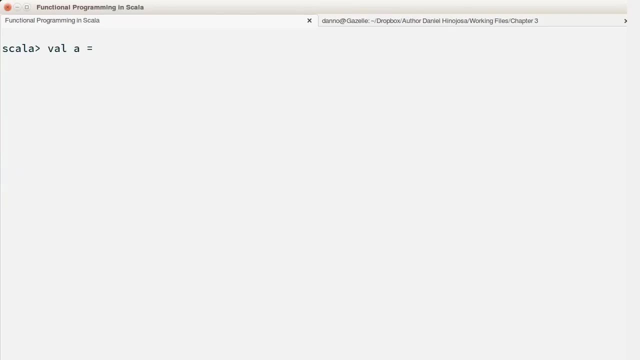 is of type double, two different ways to go about this. Let's show another example for type inferencing. Let's say that I have Val a is equal to 100. And let's say I'm going to declare Val b is equal to. Hello, The type inferencer is going to see B as of type string. Now what I'd like to do. 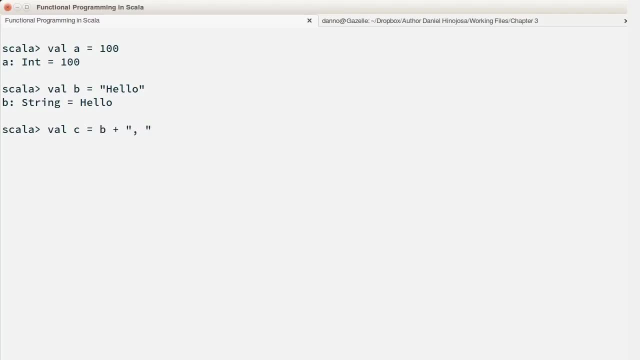 is declare another value called C. I'm going to add a string with a comma to it and I'm going to add a. Now the type inferencer is going to figure all this out And therefore the type system is going to declare in an. 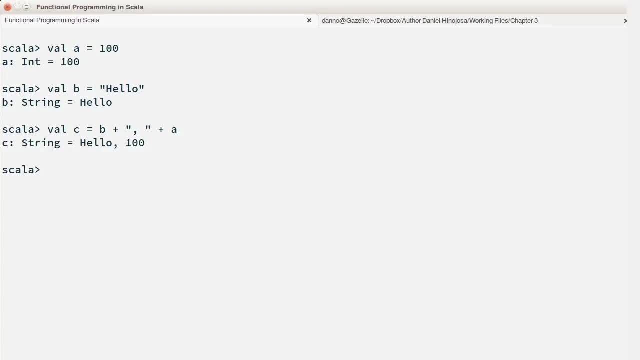 inferred way that C is of type string. Now types are needed to satisfy the type systems And at times you will need to add your own type just to make sure that the type system gets it right. It does a pretty good job in inferring the type you want, But sometimes 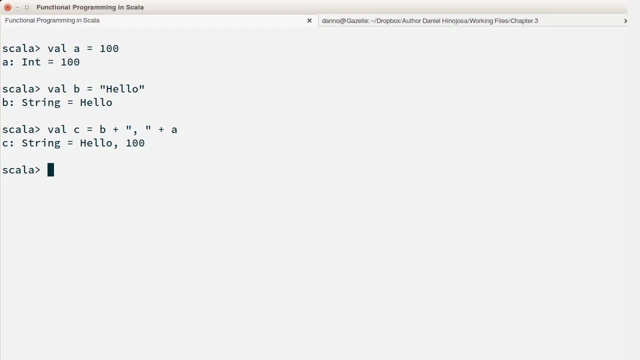 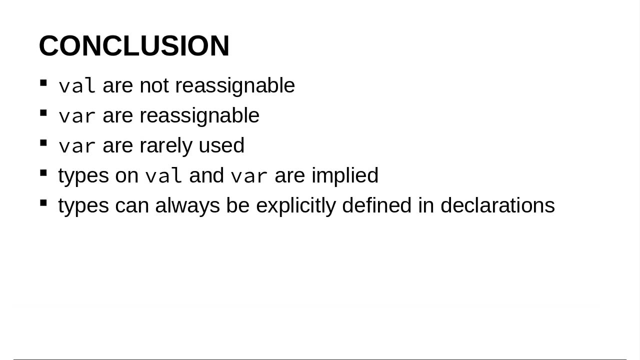 it will make mistakes And you'll have to explicitly state what type it is that you're meaning to do So. in conclusion, vowels are not reassignable but vars are reassignable. But vars are rarely used And we usually have to think about why it is we're using a var and what's the reason. 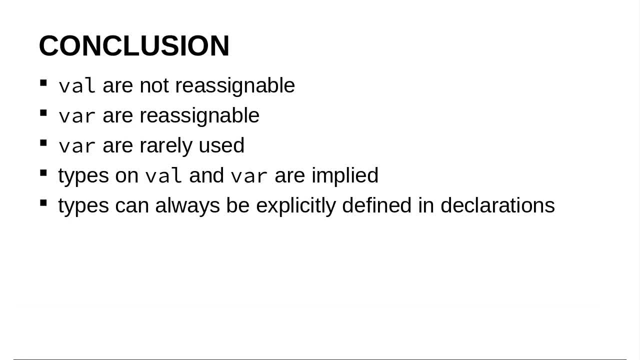 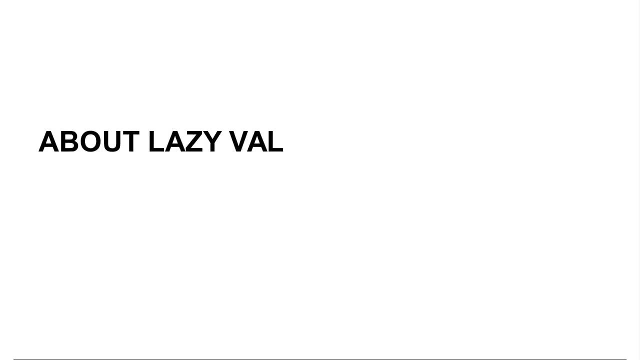 for it. Types on both Val and var are implied. you will be given types by the type system called inferred typing. But in case it gets it wrong or it doesn't understand your intent, types can always be explicitly defined in your declarations. In this session we discussed 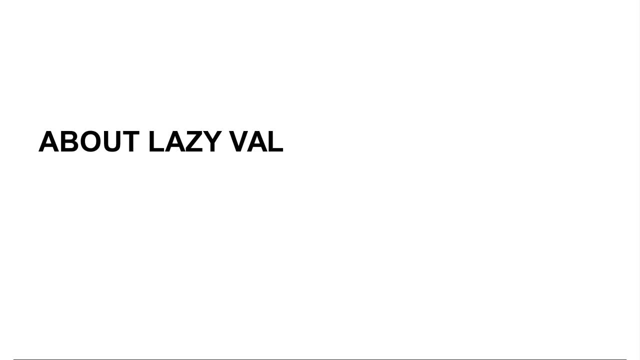 lazy Val. A lazy Val is just like a Val we just covered, with the exception that a lazy Val will not be evaluated until it is called. Let's try the following as an example: in the REPL: Here we are in the REPL and what I'd like to do is just try out a lazy Val. Here I have lazy. 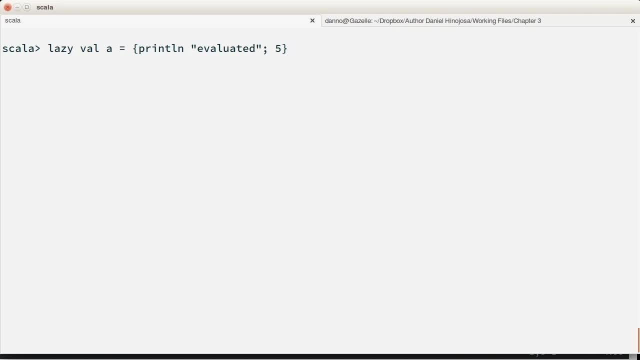 Val A- A is going to be the name of the value- And I have a block And a block is just multiple statements. Let me correct this. First statement is: I'm going to print line evaluated. The second statement is: I'm going to print line evaluated. And the second statement is: I'm 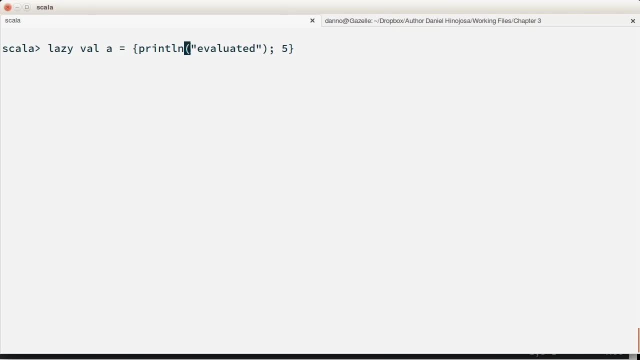 going to print line evaluated. The third statement is: 3 will be validated into A. Let's try out some Americans this morning: NASA Andes Free June June June June January, July, August, Mar. and if I do this again, we will no longer get the print line evaluated, but we will see that it is. 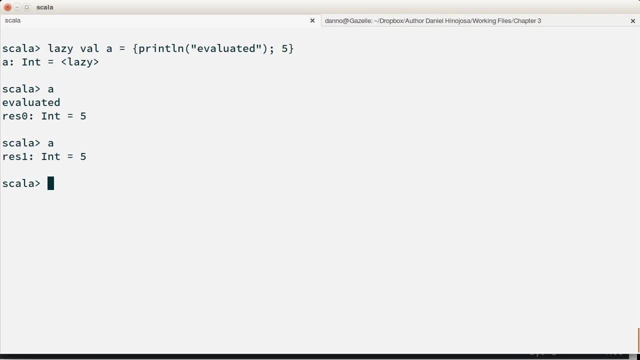 five. because five is now fixed to a. it only takes one invocation, and thereafter every subsequent call will have that assignment made again and again. every call just shows the evaluator result the first time we referenced a. now there is no such thing as a lazy var, only lazy vowels. now one thing. 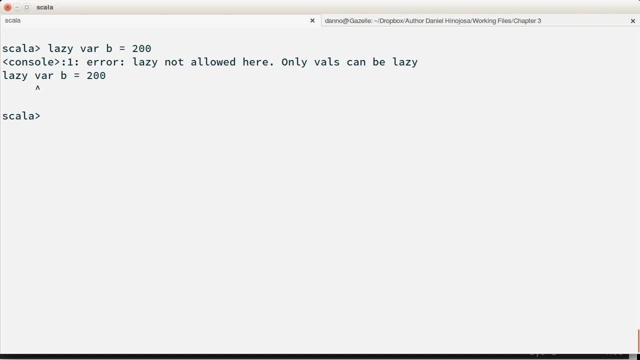 that it is possible is, with lazy vowel, is the ability to forward reference a vowel, particularly without a warning. so let's give this a try in a script called lazy vowels dot scholar. so here I am, inside of lazy vowels dot scholar and I'm going to add three lines. 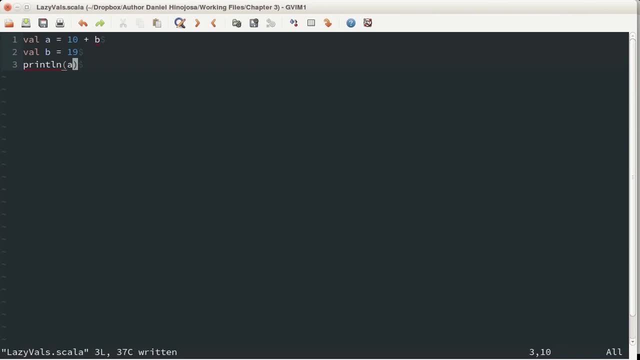 val a is equal to 10 plus b, but b is not established yet as of line one. then on line two I have vowel b is equal to 19 and finally we'll print line in a. so I will print line in a. went ahead and saved this file already. I'm going to run the script And what we will see is a. 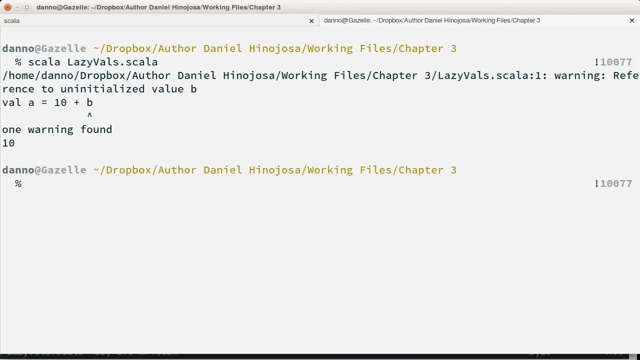 warning. Our warning will state reference to uninitialized value B. Scala was able to kind of wire things together- was, after all, a simple script. sometimes it will be a warning, sometimes it will not, But, as it's stated right here, at of this moment, B has not been initialized. Now, if we 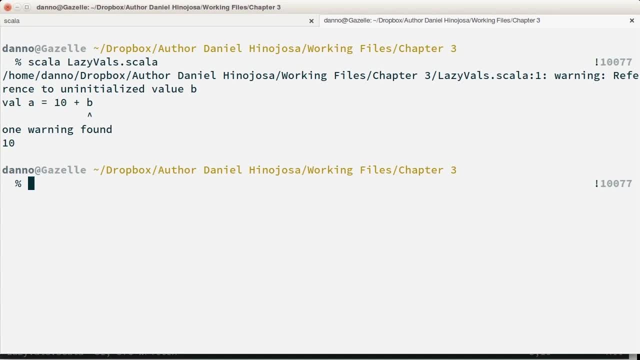 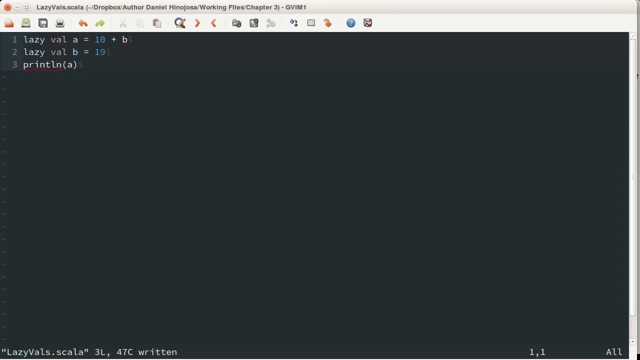 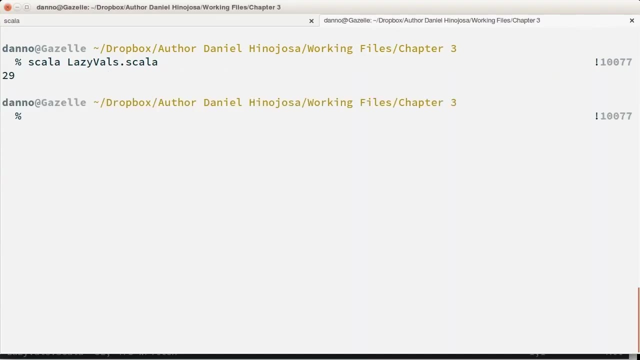 retrofit those assignments with lazy, we could find that these warnings will go away and we can make that code snippet work. So let's head back to our code. There we go. I've added lazy in front of those valves. Now, if we run the script, warnings go away And we prove that this is. 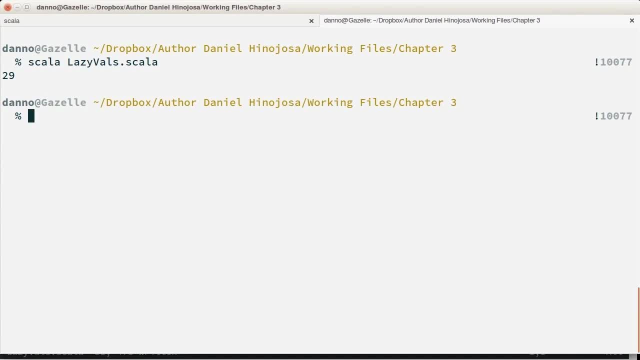 particularly useful for wiring components together, And if we're stuck with a component, that comes first dilemma, lazy valve gives us that power to defer that until it is needed. Now let's talk about another fascinating side effect when it comes to lazy valves, And that is: 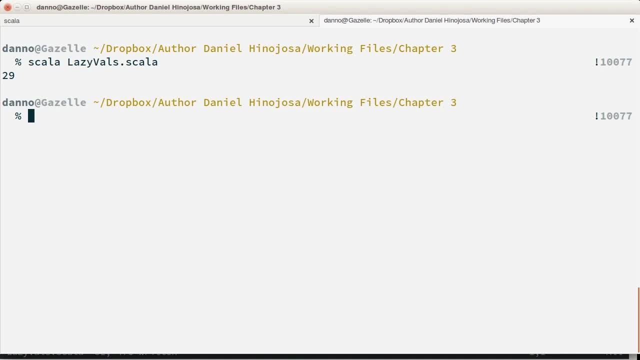 when exceptions occur. So we'll turn to our REPL this time for our next example. Here I'll have a divisor And here I'll have a lazy valve with a quotient, And this quotient will be 40 divided by that particular divisor. As you can see, here quotient is lazy. Now if I print line that quotient, 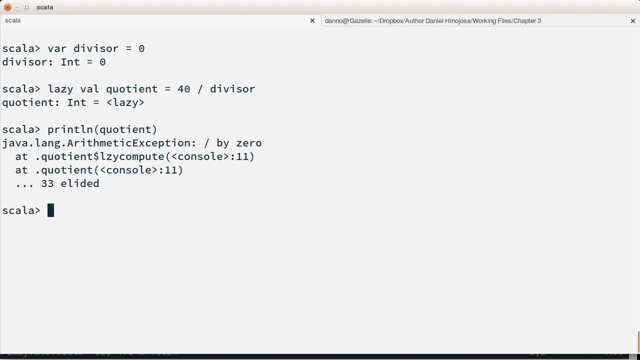 quotient is being referenced. we get of course division by zero arithmetic exception. But since the first invocation failed, Scala is forgiving and gives you an attempt to do it again correctly And if successful, it will then lock the valve quotient to that value. So if I change divisor to two, 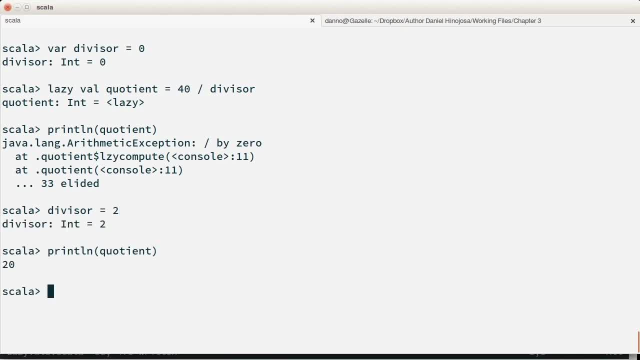 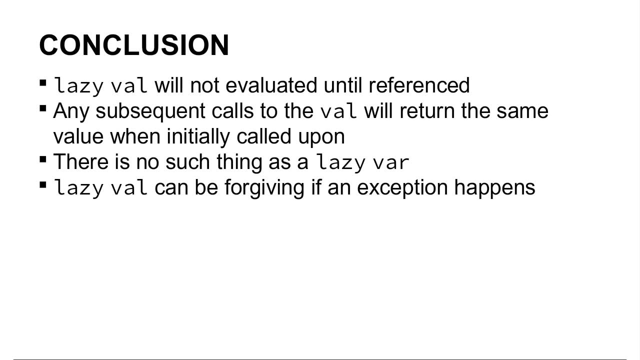 and finally do a print line quotient. once again, we will get 20.. So, in conclusion, lazy valves, do not evaluate until it is called upon And the subsequent calls will return the already established quotient. And that's what we're going to do here. So let's go ahead and 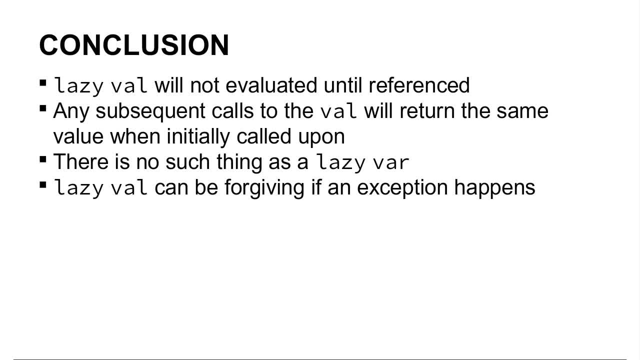 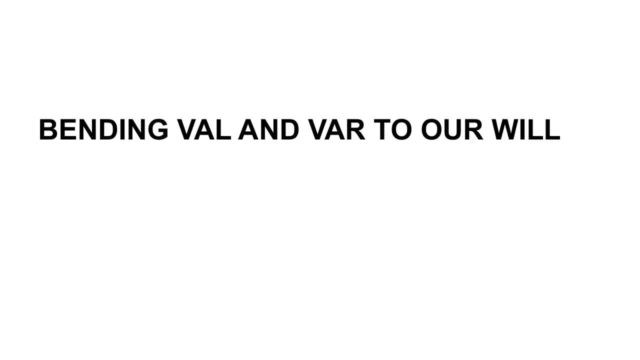 see how we can solve this problem And we'll have a lazy valve result. There's no such thing as lazy var. Also, lazy Val is forgiven if an exception happens the first or second time, or third or fourth, until it is able to make the assignment. That's when it will lock In this section. we'll. 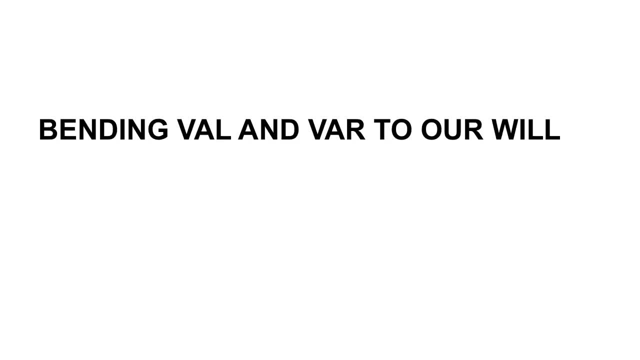 be discussing how to bend values and variables to our will. Scala offers several tricks that allows us to be expressive in a flexible way. There is a concept called internal DSL, where you can make a host language, have a look in front and a back end where you can Jingle your game and see what can. 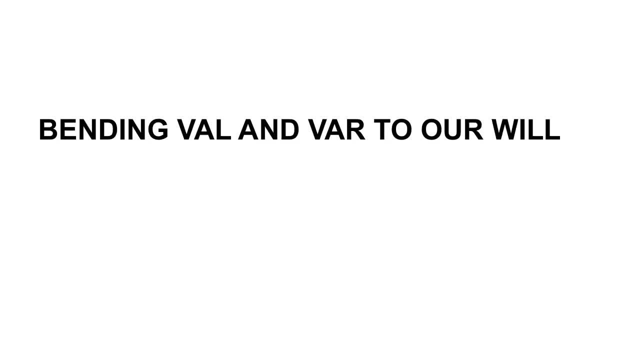 be done in the end right and just leave a link on the bottom corner to the end of your game and feel of another language. As you increase your knowledge in Scala, you'll be introduced to other libraries and tools that will make Scala look like an entirely different language. This section 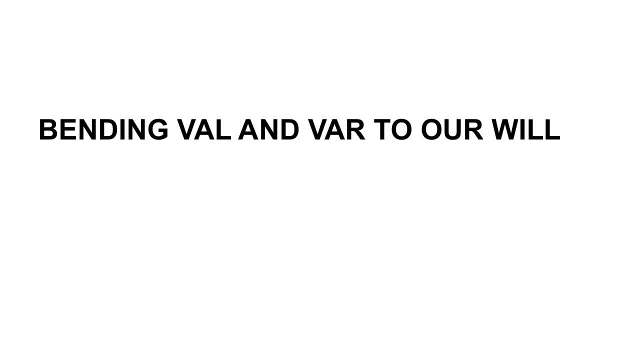 presents some of those neat little tricks. We start off on the REPL with the following: I'm going to start off with a VAL and then I'm going to start off with a back tick. This is the key that's usually right next to the one and above the tab. I'm going to enter in my greatest gift in. 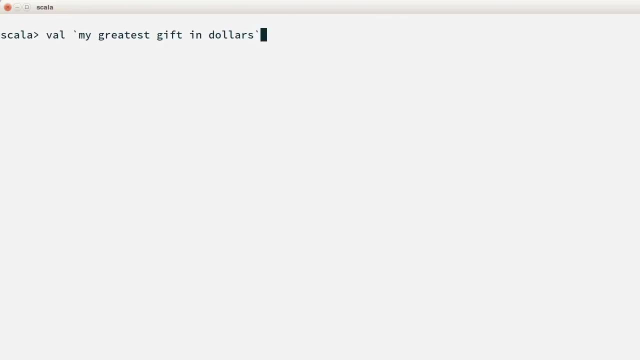 dollars. I'm going to close things off with a back tick and I'm going to assign that to 500.. As you can see, I've created a value with spaces in between words. For those with Java experience, this is welcoming, since there are no spaces in any of the variables in the Java programming language. 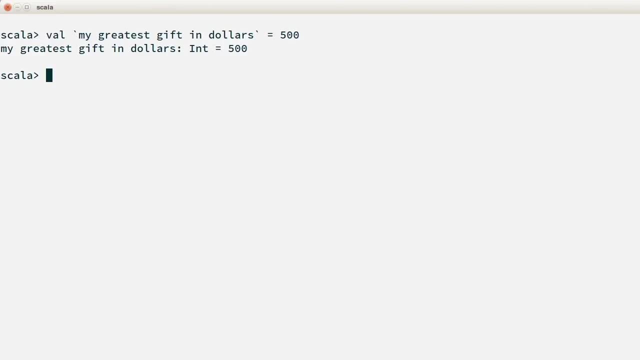 Now, before we go on to the next example, we need to learn what an OPCHAR is. In the Scala specification, Scala has a definition for an OPCHAR. OPCHAR is any Unicode character from U0020 to U007F. For more information on these Unicode characters, visit unicodeorg. slash- charge slash. 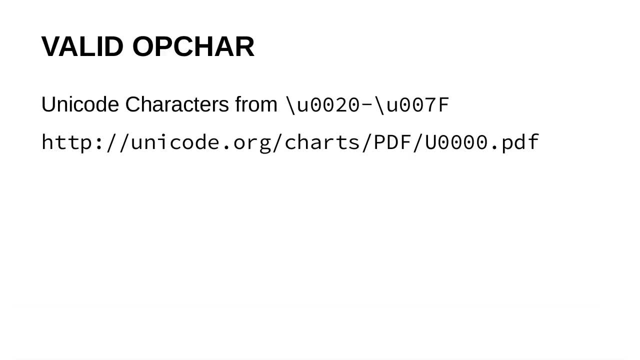 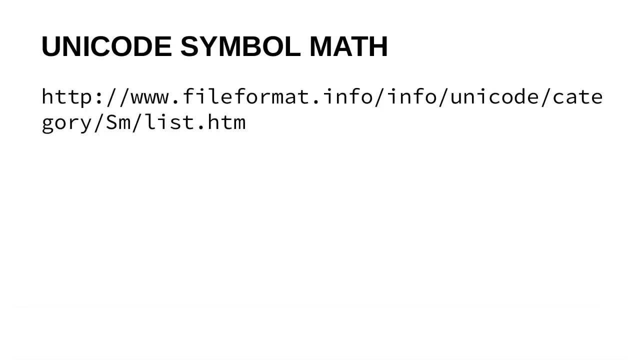 pdf slash- U0000.pdf. Now for the next opchar. we have Unicode symbol math. These are mathematical symbols that we can place in a variable or a value, And for a list of these mathematical symbols, go to the following link. Finally, you can use Unicode symbol other. These are other symbols. 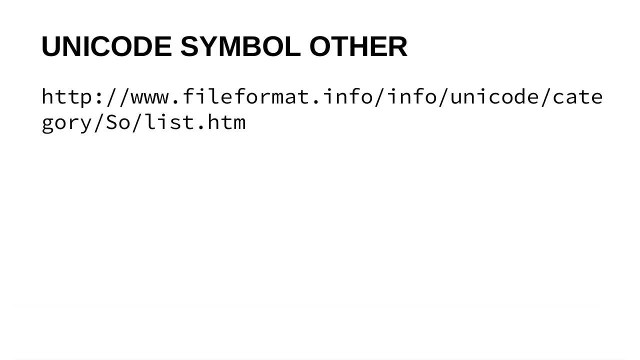 that you can place within a value or a variable, And for more information, visit this following link. And what can we do with some of these strange characters? Well, let's go back to the REPL. In a val or var, you can put any opchar after you establish an underscore. Let's try it. 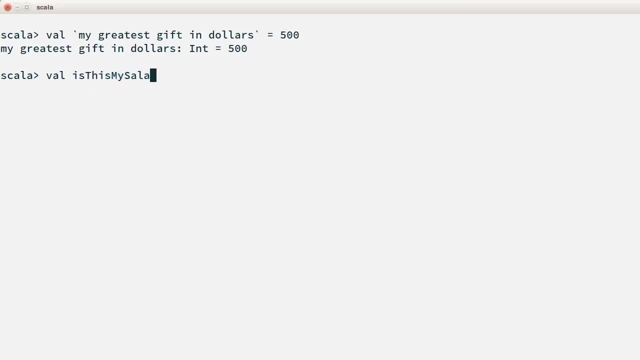 out. I'm going to create a val called is this my salary per year underscore? And this time I'm going to use a question mark. May seem strange, but this allows us to be flexible. Now, if I want to reference it, let's do it. 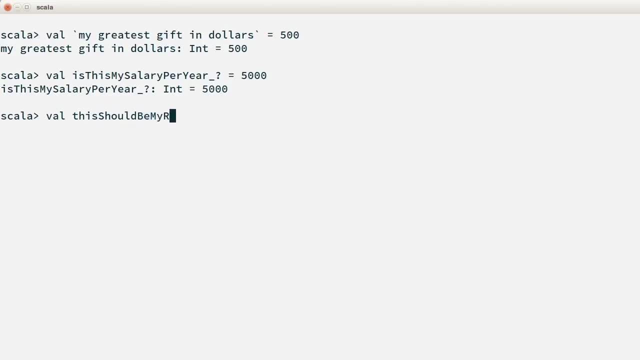 Let's try this out. Let's say: this should be my raise, underscore with an exclamation point. Now I'm going to reference the previous value that I've just created And I'm going to add 50,000.. I just gave myself a raise. Now let's go back to backticks. Backticks can also be used to create a value, or? 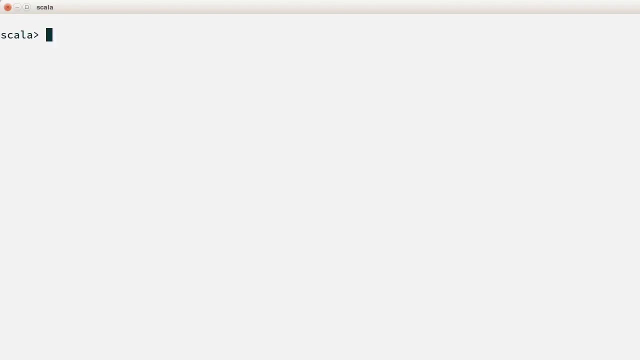 variable that are reserved keywords in either the Scala or Java programming languages. As you can see here, import is a reserved word for Java And it just happens to be a reserved word in Scala. If you wish to reference keywords in backticks, be careful. 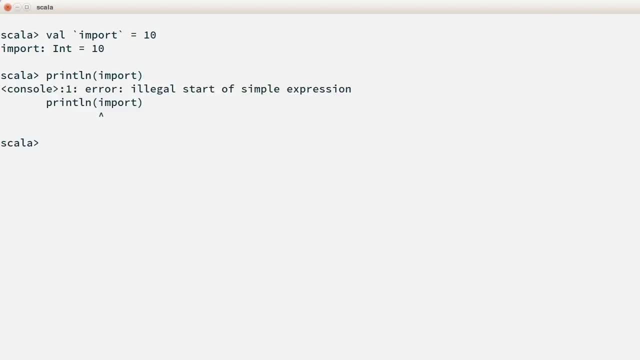 For example. this will not work. It doesn't work because import is a keyword and the parser will first recognize that as something that it should import. You'll have to make sure that any subsequent reference also has the backtick, So in order to do this correctly, I need to include the: 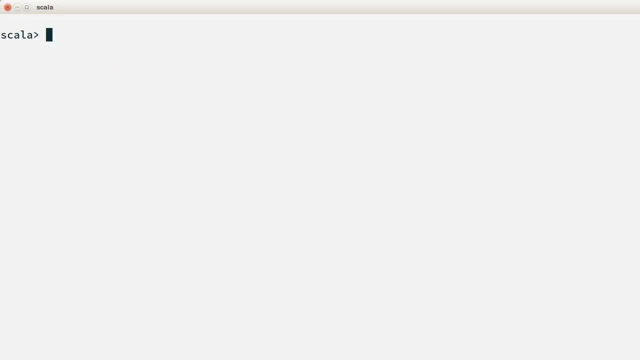 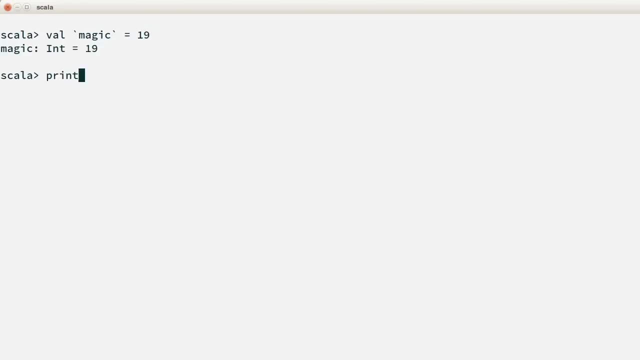 reserved keyword in either Java or Scala, then I can safely reference that value or variable without the backticks Of course. don't go nuts. You still have to work with your coworkers And for our next example we're just going to do something silly, But you'll get the point. how flexible the 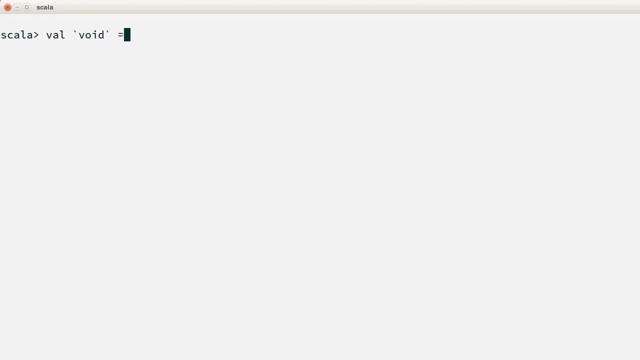 Scala programming language can be. Let's try that. we want to include a val void and set that equal to 100.. I'm also going to create another val called false, and set this to true, And I'm also going to set return and set that equal to 90.. What do you think the answer is going to be for? 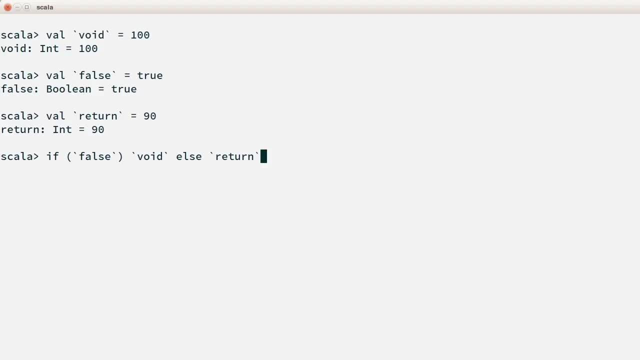 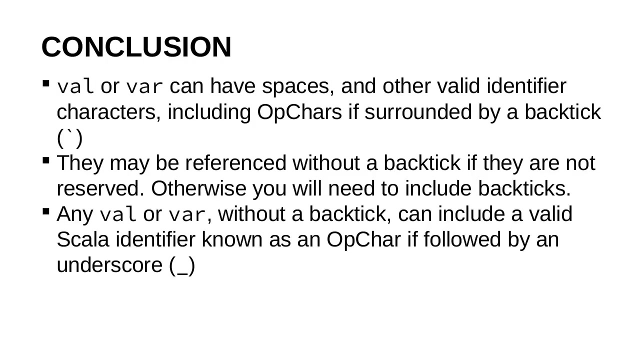 this statement: If false, which is true, then return void, which is actually 100.. Otherwise, return return, which is actually 90.. Again a silly example. I wouldn't recommend this for production code. So, in conclusion, val or var have spaces and other valid identifier characters. 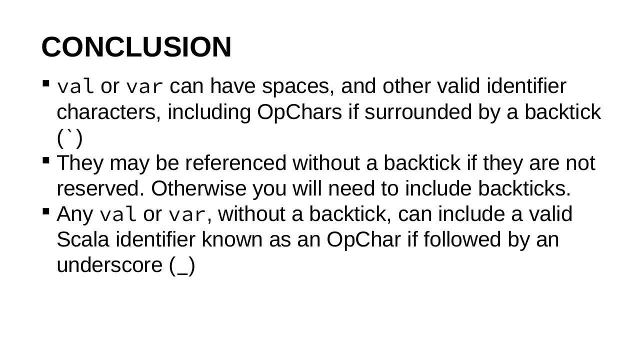 including opchars, if surrounded by a backtick. They may be referenced without a backtick if they are not reserved. Otherwise, they are not a backtick. Any val or var without a backtick can include a valid Scala identifier known as an opchar, if. 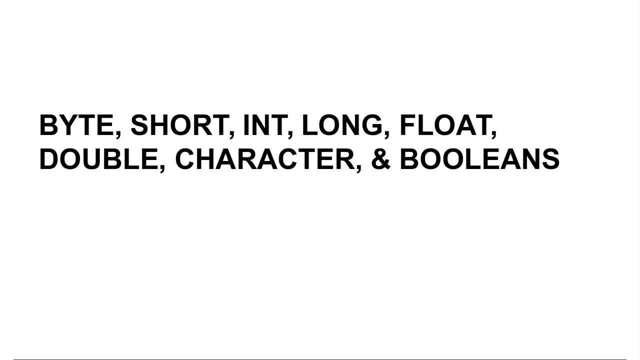 followed by an underscore. In this section we're going to talk about primitives by short and long float, double character and booleans. Now I think for the most part many programmers already know the basics of these items, So I'm going to run down fairly quickly with this, But also 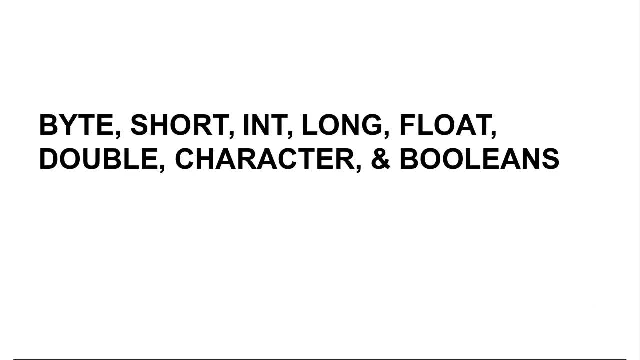 I'm going to do this with a twist, Of course. that twist is we're using a different program. So let's go to the REPL and play around. Let's start off by creating a byte. I'm going to do so by creating a, val, b and specifying that the type here is of a type byte. A byte is an 8-bit number. 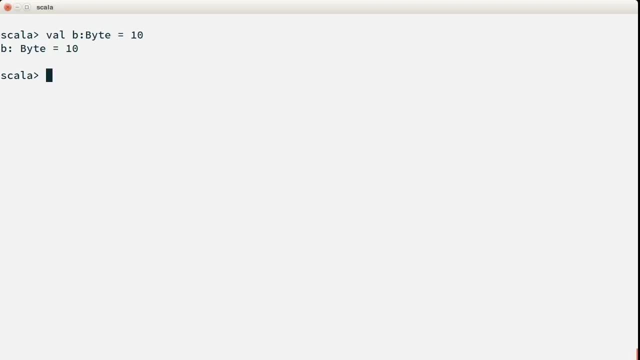 which is the same as it is in Java. The maximum formula as defined in Java is the same as it is in Scala: 2 to the n minus 1 minus 1.. Therefore, the maximum number you can have as far as a byte, 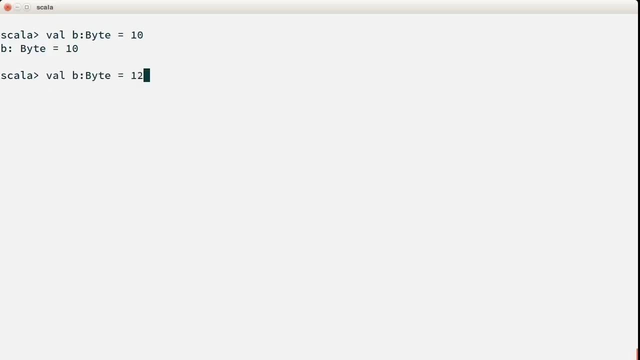 is concerned, is 127. If you go much larger, you can have a maximum of 127. So let's go to the REPL. If you go much larger than that, you'll end up with either a type mismatch or what's called an overflow In specifying a type. I could either do so at the value declaration or I could coerce. 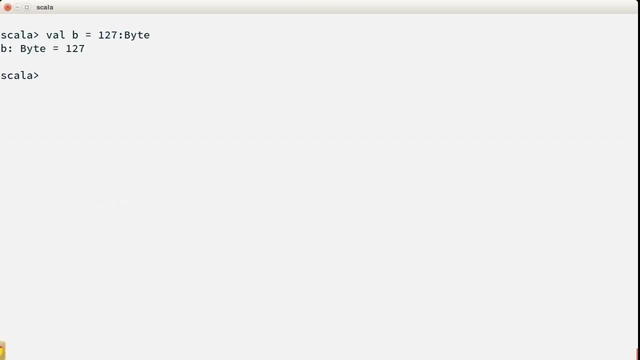 it after the number. Now a short is 16 bits. Therefore the maximum is 2 to the 15th minus 1 minus 1, or 32,767.. And the minimum is negative, 2 to the 15th. 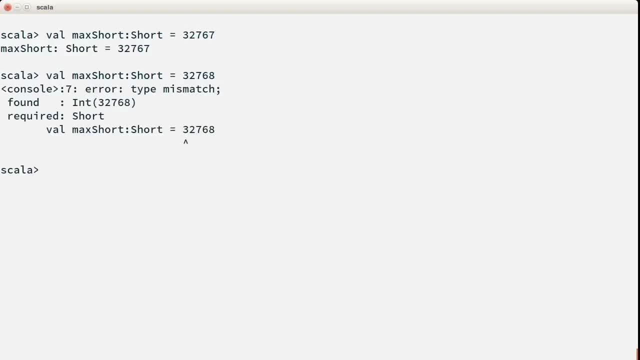 And if we go just one more over the bounds, we'll end up with a type mismatch Again. I could also do this, specifying the type after the number. Now integers are the default in Scala. I don't have to specify an int. I can specify the type, just like anything else next to the value, or I could. 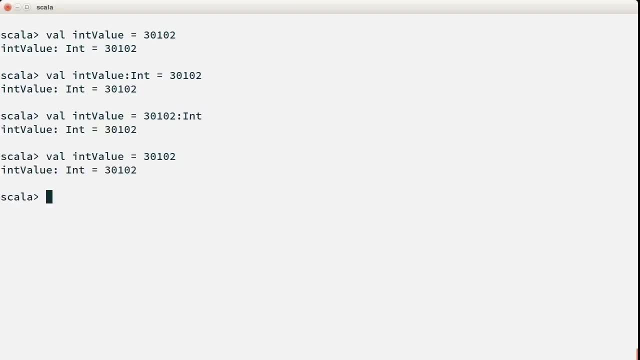 specify the type after the number. Oftentimes that is unnecessary. Now. longs are 64-bit and either require the type mismatch or the type mismatch, So I'm going to go with the type mismatch, The type definition or the type after the number using coercion. 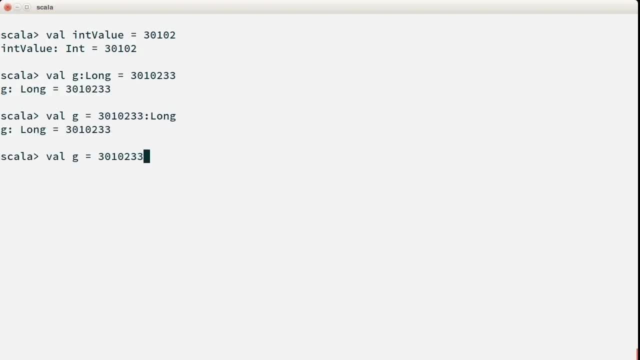 Here it is using coercion. If you don't want to use either one of those, you could specify an L at the end of the number. This is using Java style. You could also use a small L, but I don't recommend that because that looks too much like a 1. And, depending on your font, that could get. 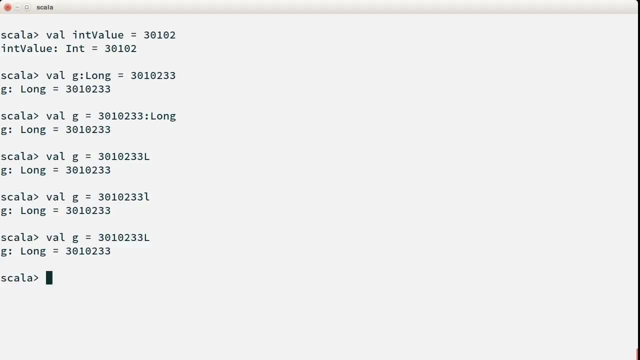 easily confusing. Floats and doubles are IEEE 754 standards, same as it is in Java, And floats can be explicitly stated by type. But this can get kind of tricky. Let's specify a float value And what we're going to do is add the suffix F. Therefore it's going to be listed as a float. 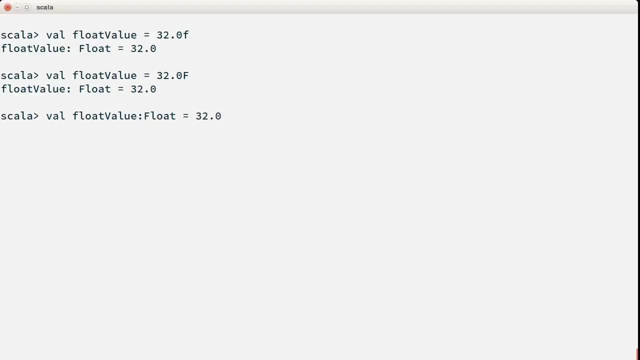 or a capital F. If I specify the type here as a float but forget the F, this would be listed as a type mismatch because it's going to be assumed to be a double. So what I have to do is make sure that I add an F. If I add the coercion without the F, that is still considered a double. So I'm going to. 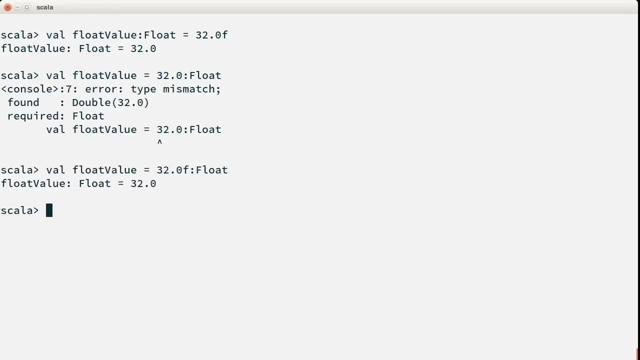 specify the type mismatch. So again, I need to make sure that I either have the small F or the capital F. Now doubles, on the other hand, are the default when dealing with decimal points. Without specifying a D, without specifying a type of double, this is going to be understood to be a. 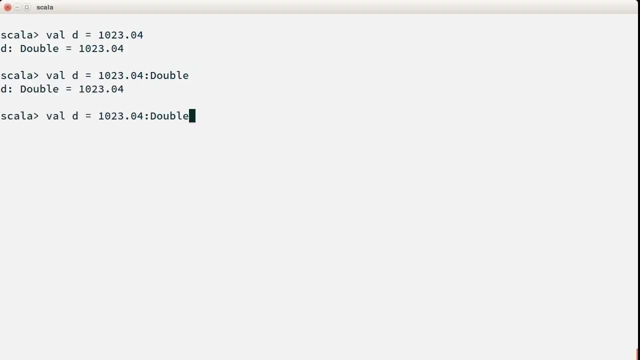 double. It's going to be type inferred to be a double. I can add types wherever I need to, either by coercion or by adding it to the value. I could also explicitly add a D to the end of that number or a small d. Doubles have more precision than its float counterparts. Doubles are 64-bit and floats. 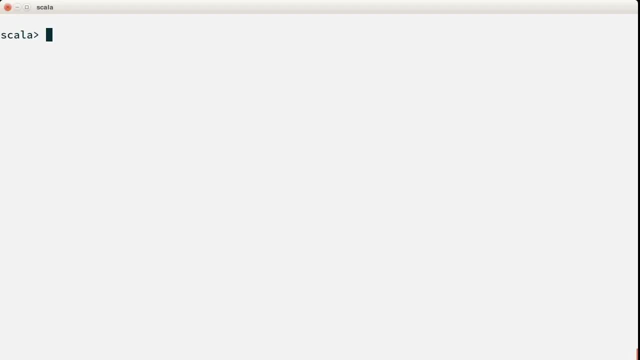 are 32-bit. Now let's talk about characters. Characters are very much like in Java, where when you have to specify a character, you put single tick marks around it. Now, if you wish to specify a Unicode character, you can do so with a single tick mark backslash U and then enter the Unicode value of what. 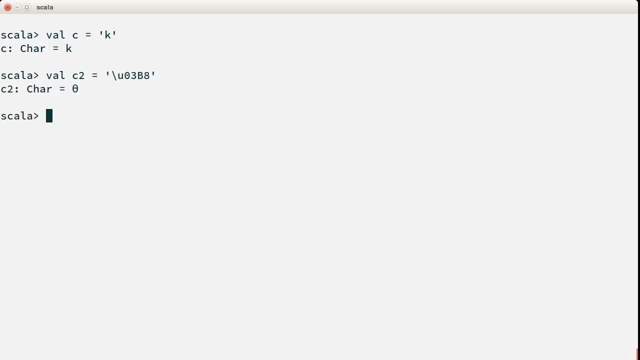 you're trying to represent. This will be a theta. Now, booleans are the same basic construct as it is in Java. We have true and we have false. They do not correspond to ones or zeros. They are values onto their own. Now, last thing to mention is that, unlike Java, Scala's primitives may be treated like objects. 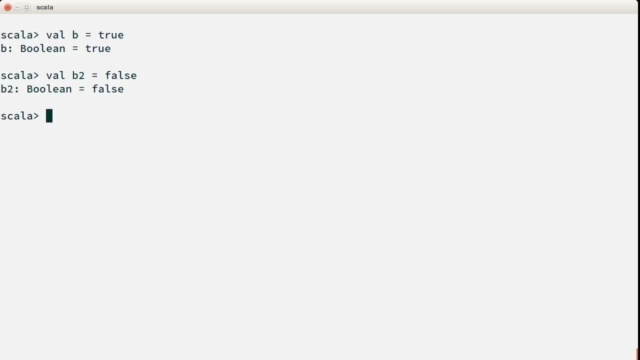 I'm careful when mentioning that they may be treated like objects. When calling an operation that works perfectly fine as primitives, Scala will not box or wrap the primitives up in another object. Only when calling a method that requires an object will an object be created. 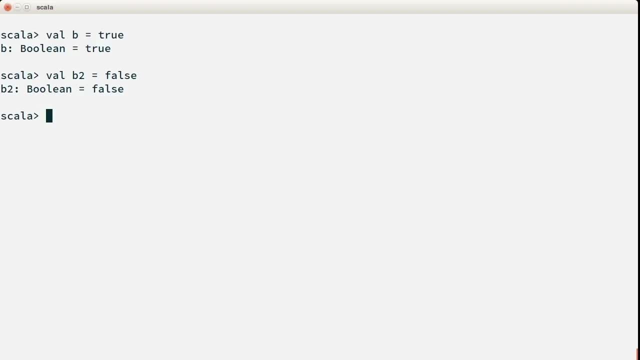 Best thing about Scala is that you don't have to concern yourself how or when this wrapping occurs, since a compiler will typically do that for you. Now consider the following statement: 1 plus 4.. Obviously, it's going to return 5. Now, when you're actually running this, what's happening? 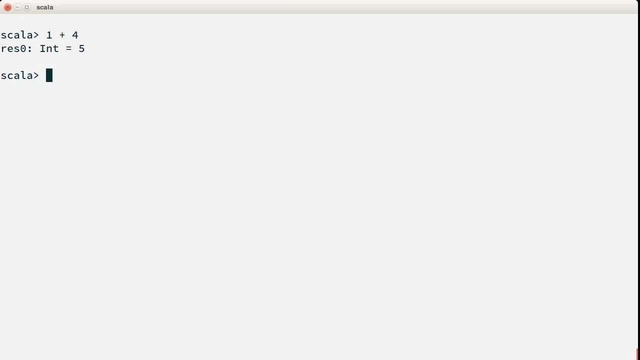 is, you're actually adding two primitives together, And while that in itself is not exciting, knowing that you could also express that addition as a method on an object will allow developers to maintain an object-oriented frame of mind. In other words, this operation looks just like an add. 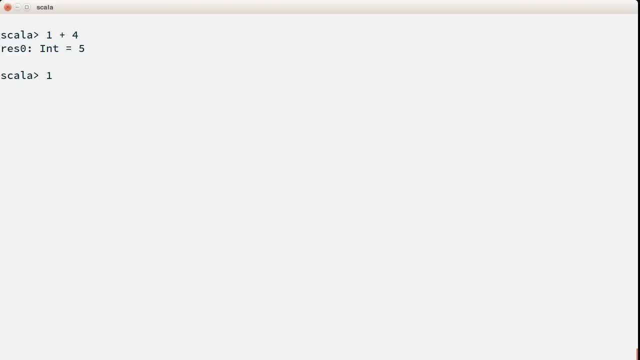 which is a method on an object with a parameter 4.. So let's say I have 1, and let's say I just want to treat it like an object And I'm going to call the method plus. There is operator overloading in. 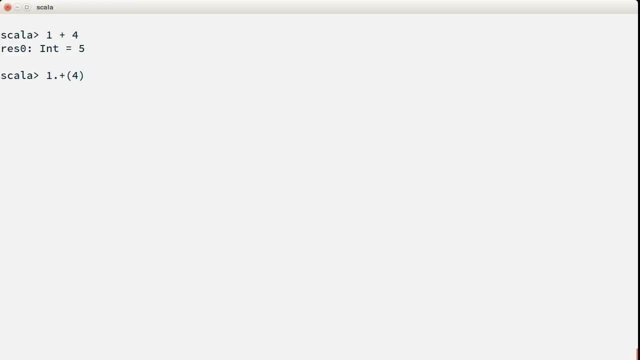 Scala, And I'm going to call plus and I'm going to give it the parameter of 4.. Now these two end up with the same values. They're the same values. They're the same values. They're the same values. 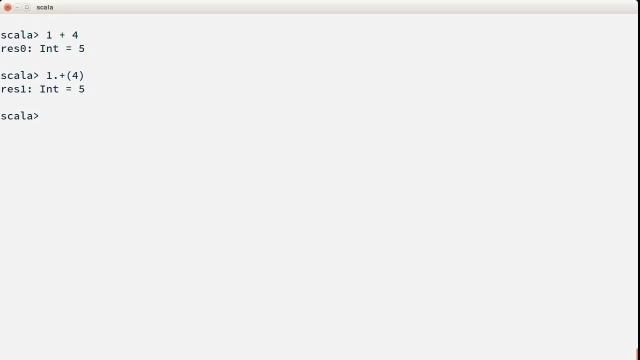 Again, in Scala we can treat everything like an object. That doesn't mean everything will be an object when it comes to compile time or runtime, just only that we can treat it as an object. Now there are times in Scala where there are actually objects being wrapped up in order to 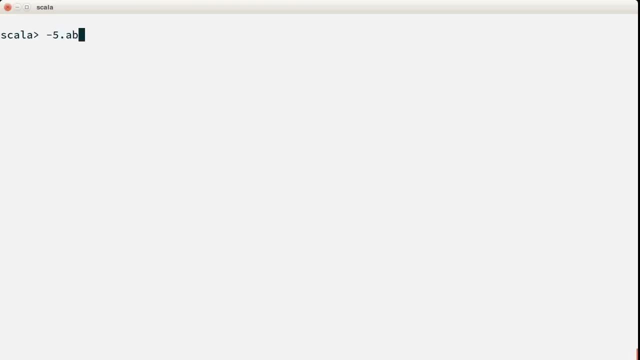 add certain functionality. Let's take the following as an example. This looks very clean. I have negative 5 dot abs, And abs is a method on int that calculates the absolute value of this int. Now, this requires a little bit of history knowledge when it comes to Java. 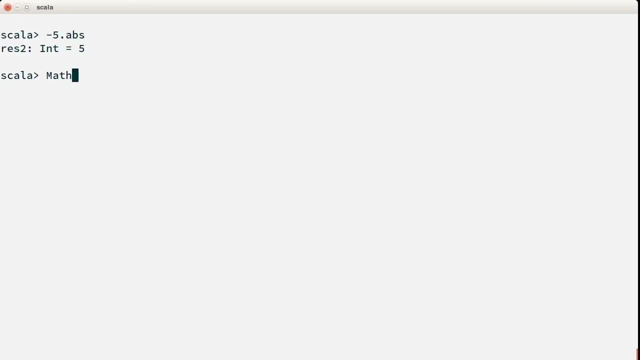 Now for those coming in from Java, you know that in order to get the absolute value, you have to bring up this annoying little method called math dot abs, math being the class and abs being the static method. as you give it the value, you're trying to calculate the absolute value for. 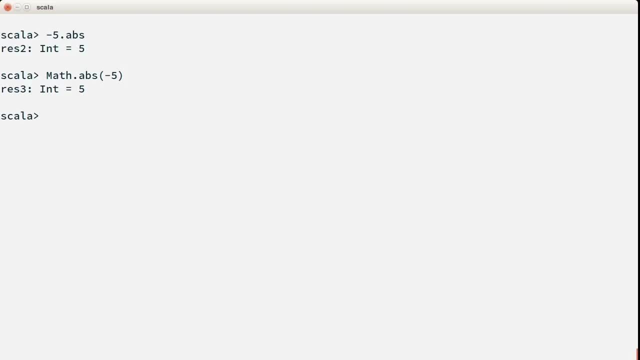 Scala has cleaned most of this up. I'd rather do negative 5 dot abs rather than math dot abs, For one reason: if you're using an IDE, you can have code completion, give you all the necessary functions you need pertaining to an int without having to look up some kind of static method in 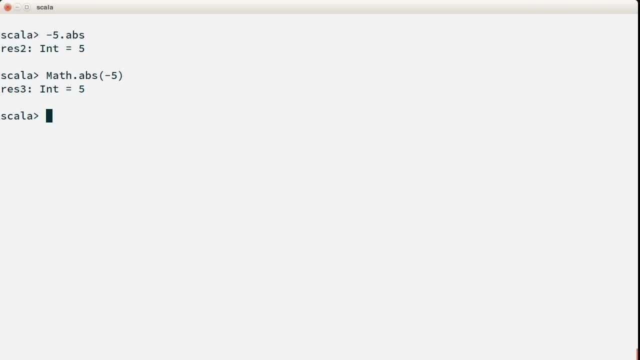 some other class. Now in Scala it looks like abs is an inherited part of int and it's doing so through a trick called an implicit wrapper, And notice how the abs function here just seems like it's a natural method for that number. In this case there's an adapter, a class that wraps around an. 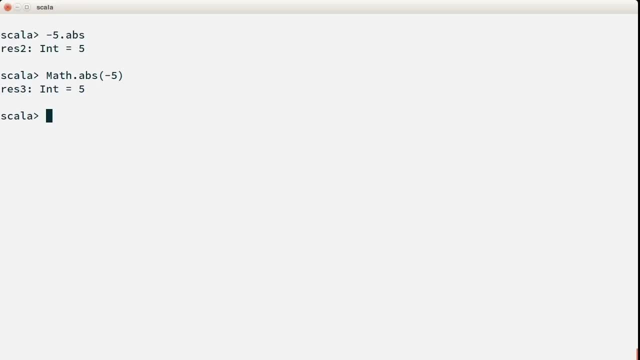 int, called rich int, And it provides nice little methods like abs, among others. Every primitive type in Scala has a corresponding wrapper: For car: there is rich car. For boolean, there's rich boolean. For long, there is rich long, and so on. Scala will convert any primitive into an object. 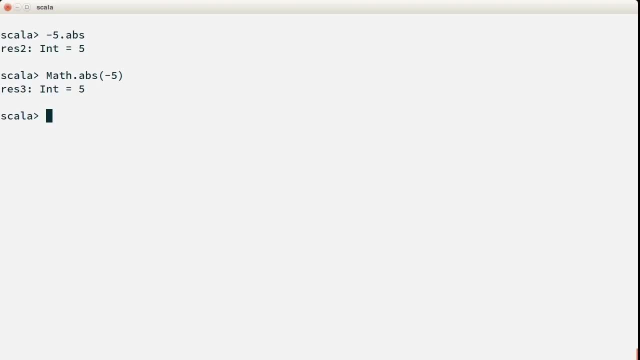 on a as-needed basis automatically, which is good. Scala will always work to our benefit and we could just go on thinking in a functional and an object-oriented way. So, in conclusion, all of this stuff is very useful and I hope you enjoyed this video. If you did, please like, comment and subscribe to the channel and I'll see you in the next one. See you in the next one, Bye-bye. 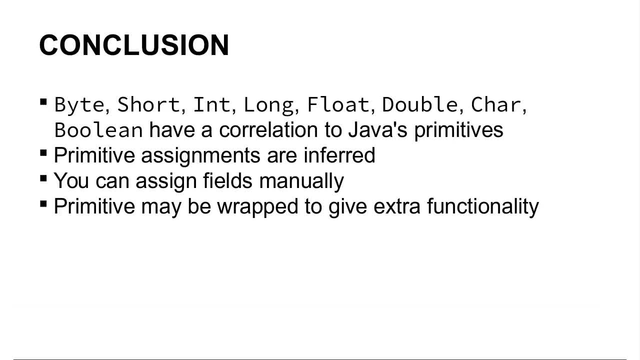 All primitives work just like in Java, with varying differences. Primitive assignments can be inferred by the type system, or you can add types manually as you see fit. Primitives may be wrapped by a rich wrapper, depending on which method is called, and this gives a primitive more methods and more functionality than it originally had with Java. 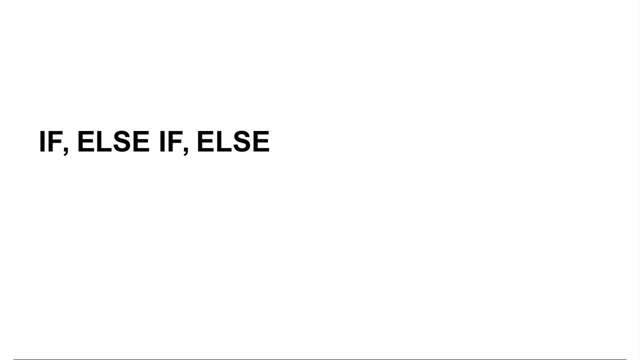 In this section we'll be showing if else, if and else in Scala and some of the differences to expect when working in a functional programming language. For the most part, I think we understand to this day and age that if else, if and else statements. 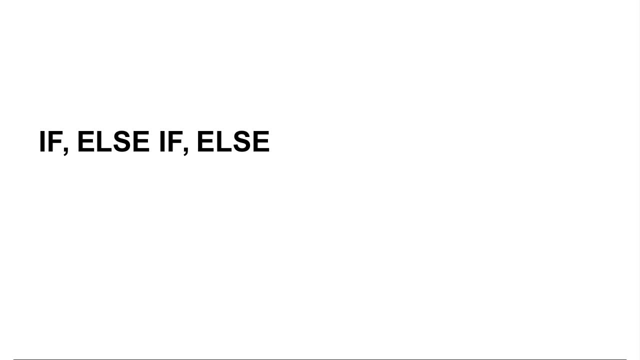 are fairly predominant. We know what they are and, given the knowledge of previous programming languages, we would expect someone new to Scala to know how to write if statements with some minor differences. So let's get started with a file called old if statements. 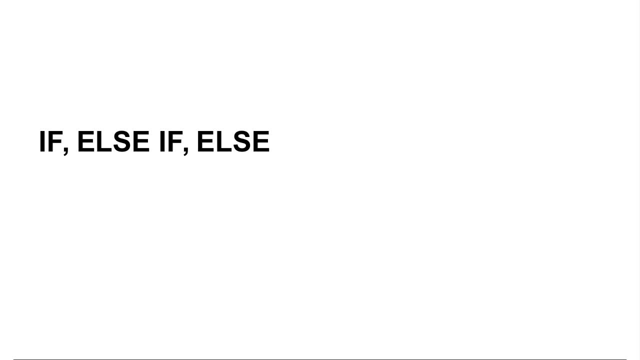 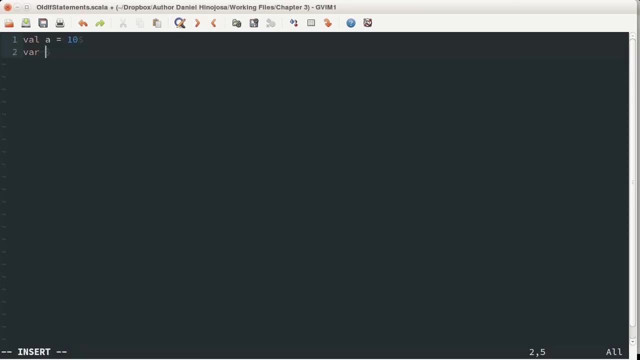 and let's mock up something that a programmer first coming to Scala would write. Here's our file: oldifstatementsscala. Let's get started. My first two lines: val a is equal to 10 and var result is equal to an empty string. 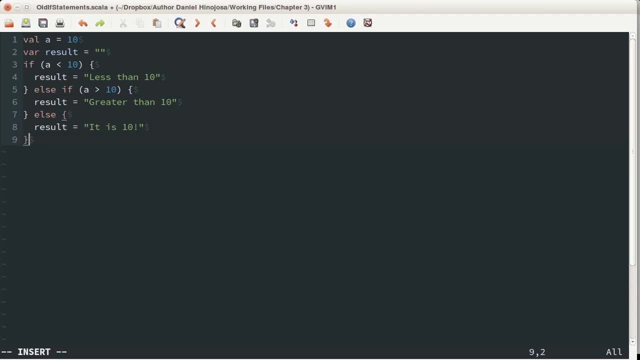 So we have: if a is less than 10, then the result will be less than 10.. Else, if a is greater than 10, then it'll be greater than 10.. Otherwise, we will state that it is 10.. Therefore, less than 10, if a is indeed less than 10,. 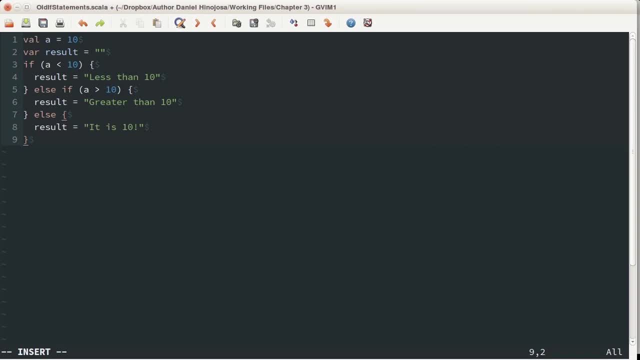 result will be greater than 10. if a is greater than 10. And if nothing else is valid, then we'll assign that to it is 10.. All right, so we'll go ahead and save that And let's go ahead and print out the result and see what we are looking at Again. this is all. 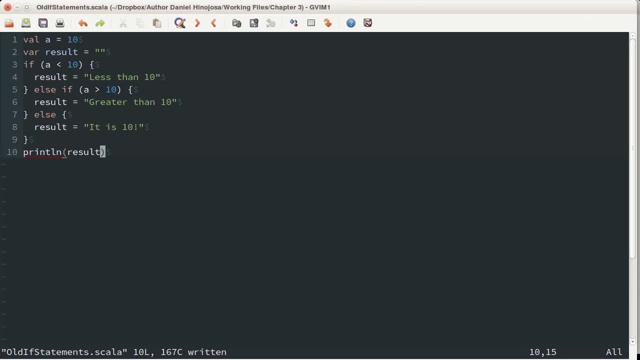 under a file called oldifstatementsscala. Let's go to run it. Great, it says it is 10.. Let's go back, And here we had that a is equal to 10. And the result is going to have the ending string of the. 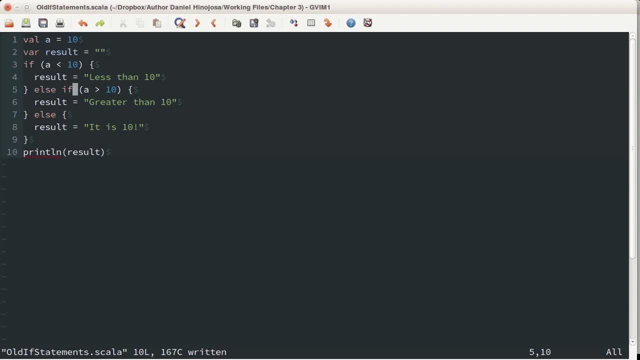 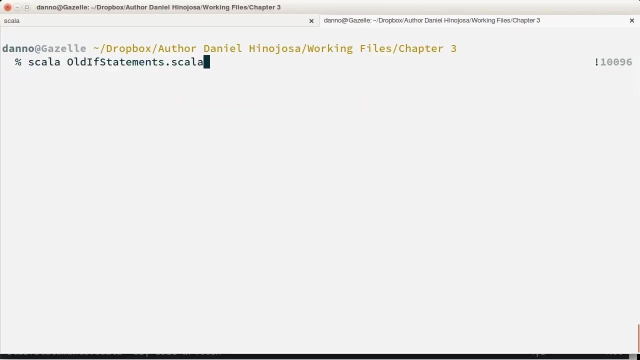 result which is assigned with each subsequent if statement. Now, if we didn't want to, we could just go ahead and get rid of some of these brackets here For it to be a little bit cleaner. let's go ahead and save that and run it. There we go. This still says that this is still 10.. 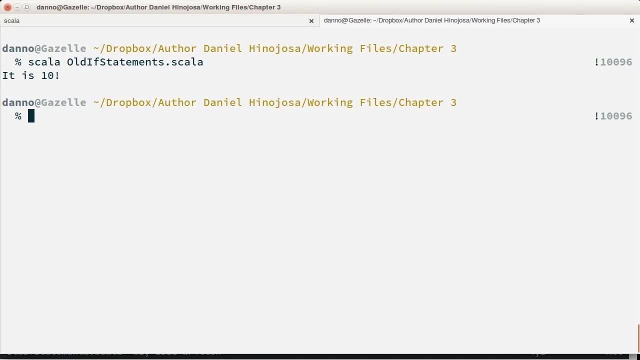 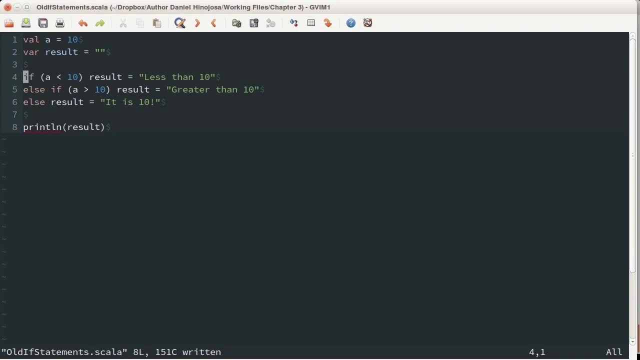 Now, these lines of code work just fine in Scala, but it is imperative, So let's go back, And that means that all computations are done in a series of statements. There is also this var right here under line two And, as we mentioned, the video section about val. 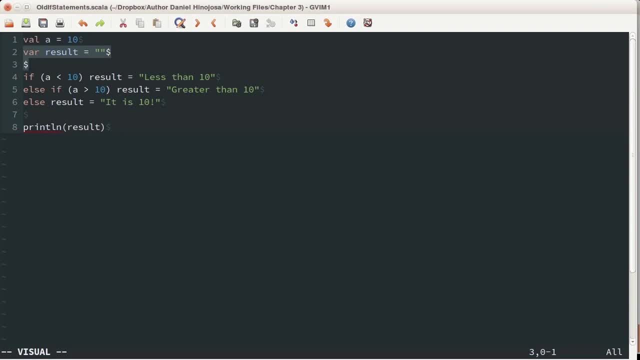 and var. we like to avoid vars. The solution to this is to change this code into a functional style. So I'm going to rewrite this in a file called new if statements, And that way we can contrast the differences. So here's our file: new if statements. let's begin. 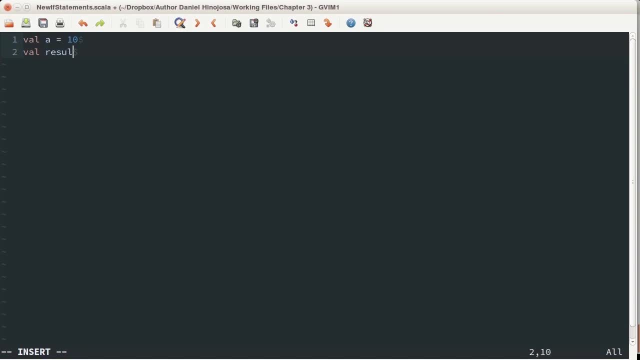 Now, this time the result is going to be assigned to the if statement. Perfect. Now let's print the result. Now, that is a little bit different. compare this to this. we don't have a var, So this is from our old file. we don't have a var And we can essentially inline everything. And here's how it. 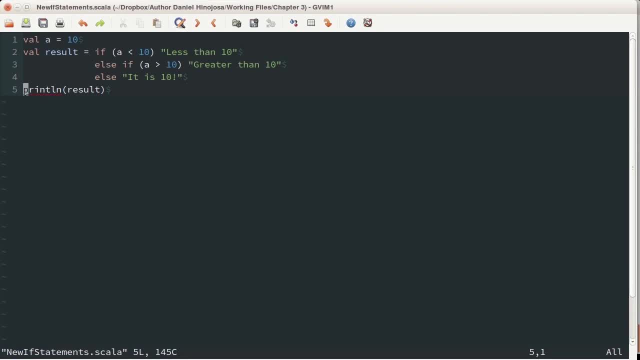 looks under new if statements. Now, this idea may be a little bit new, but soon you'll become somewhat natural in your daily Scala development to do this sort of thing. Again, we can assign an if statement to a value And in this case the value is the result. Because we could do that. 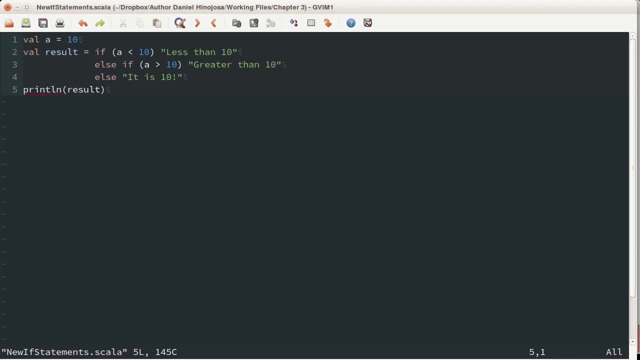 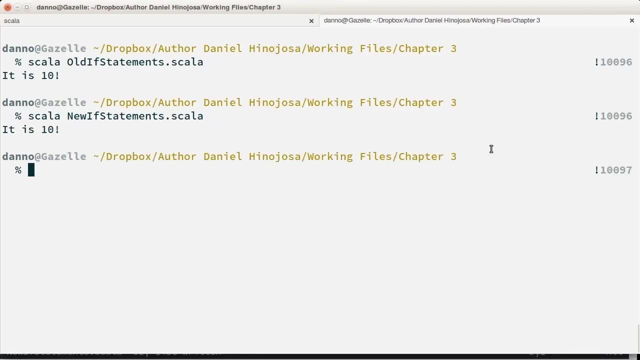 we can get rid of all the assignments to the results, since the end result of all this will inevitably be assigned. Now let's go ahead and run this, Let's go back to our new if statements, And I'd argue that this is cleaner, easier to read and 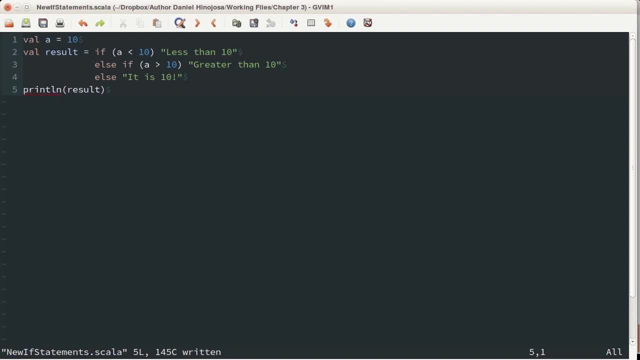 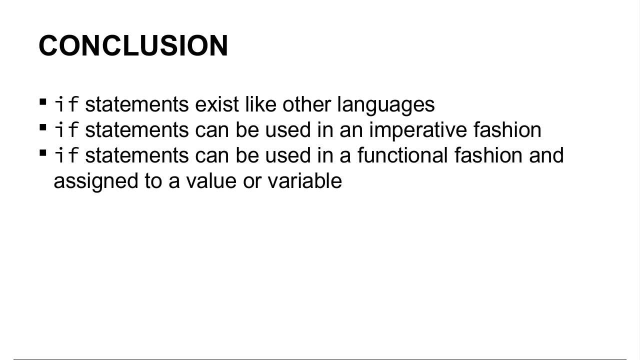 understand and avoids any kind of immutable reassignments, in other words varbs. So, in conclusion, if statements exist, just like in any other programming language, they could be used in an imperative fashion or they can assignable to a vowel in a more functional fashion. 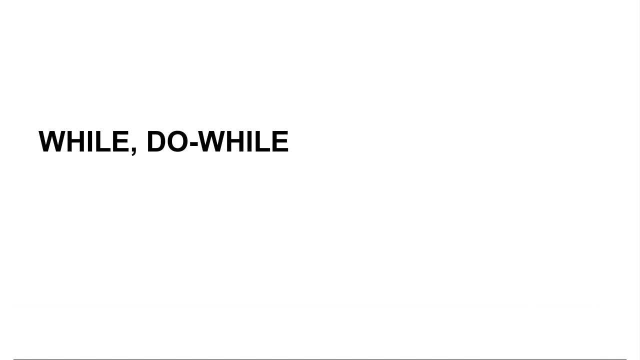 In this section we'll be showing while loops and discuss its use and the migration to a functional style of programming. While loops are nearly the same as they are in Java and many other programming languages. It will run the code within a block as long as the condition for the while loop is met. 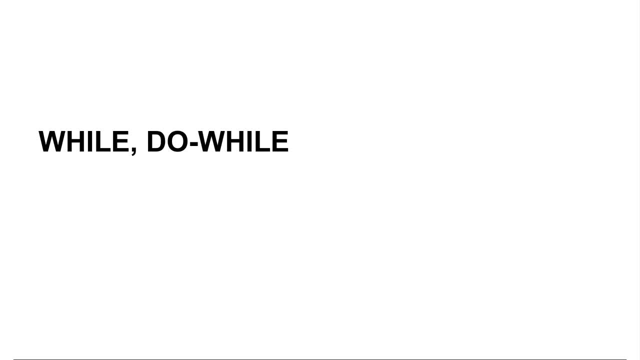 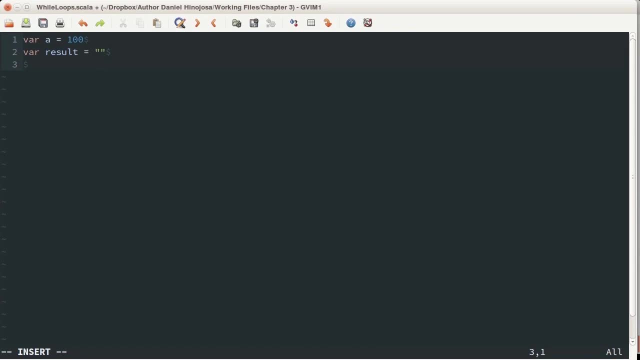 So let's give this a try in a file called while loops dot Scala. Okay, here we are at while loops dot Scala. Let's get started Here. I set up var a is equal to 100 and var result is equal to an empty string. Keep in mind I am using a var, something that is able to change, and not a vowel. 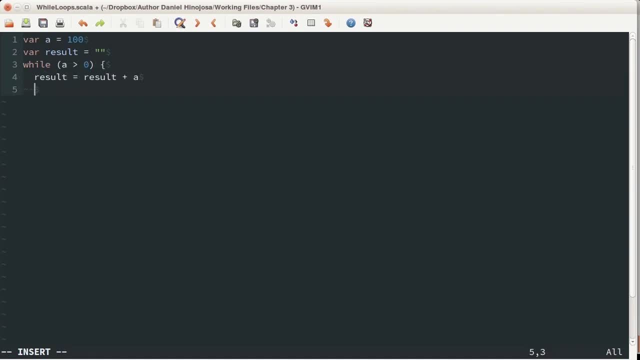 We continue. Okay, we're done So. while a is greater than zero, we will continue along with this loop. we will set result equal to the number or we will append that number to the result. If a is greater than one, we'll add a comma. 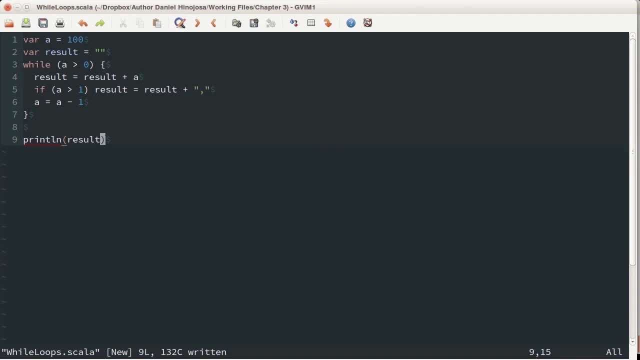 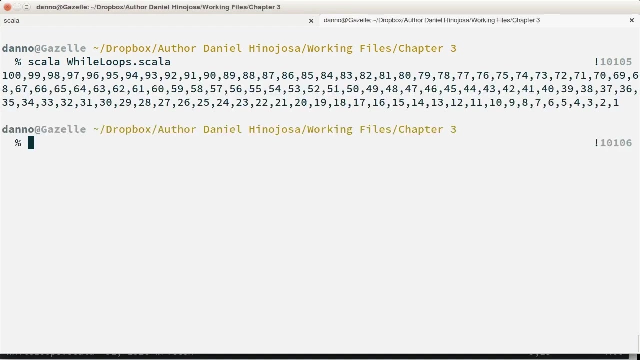 to that, And afterwards we will deduct one after each iteration of the loop. So let's see if this works. This should be somewhat very familiar to many programmers. Let's go over to the command line And there we go: 199, 98,, all the way down to zero. So let's go back to our code Now. this is: 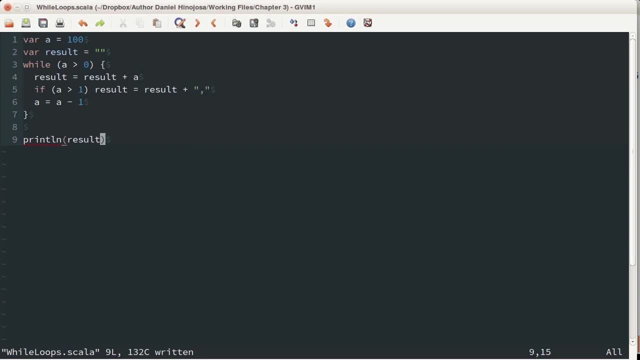 not only imperative code but it has mutability with the A and the result. Remember I mentioned we are starting off with var for a and result, Not to mention this is also a lot of work. The same result can be achieved through more functional means. to give you a taste of functionally, putting a comma after each number. 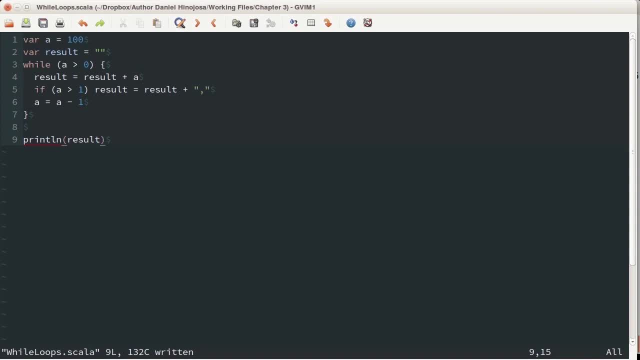 from 100 to one. let's try something different. I'm going to start off with a file called functional loops, dot. Scala. Okay, here we are inside of functional loops, dot Scala, And there we are. This will create a range from one to 100.. We will take that range, reverse it and 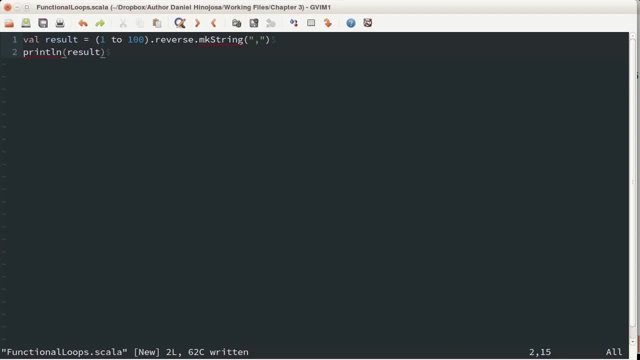 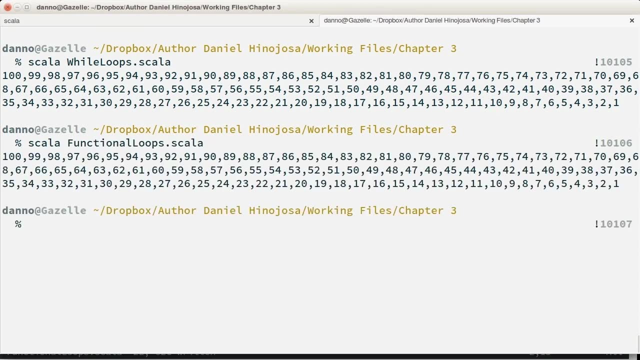 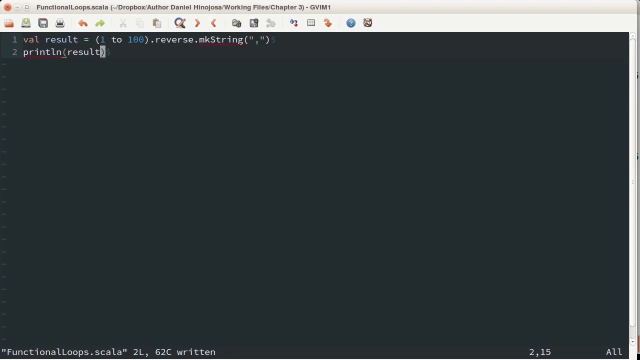 we'll call a method called make string, which will put a comma after each element within that range. Let's run it. Great, It's the same thing. Let's go back to our code Again. this is a range from one to 100, reverses it and creates a string delimited by commas. We could have also rewritten this by doing the. 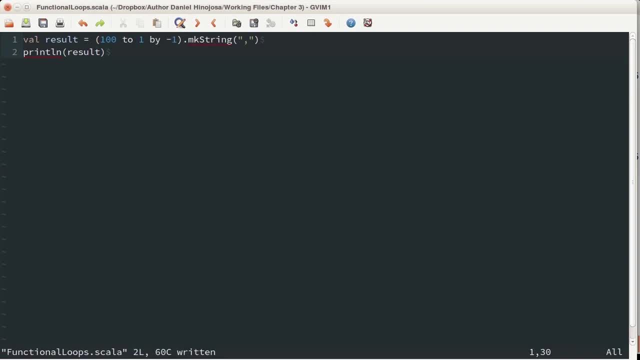 following: We could have also rewritten this by doing the following: We could have also rewritten this by doing the following: This is now arranged from 100 to one, with each step decreasing by negative one, then creating a string where everything will be delimited by a comma, Since the result is so lightweight as opposed to the full featured while loop. we could also do the following: 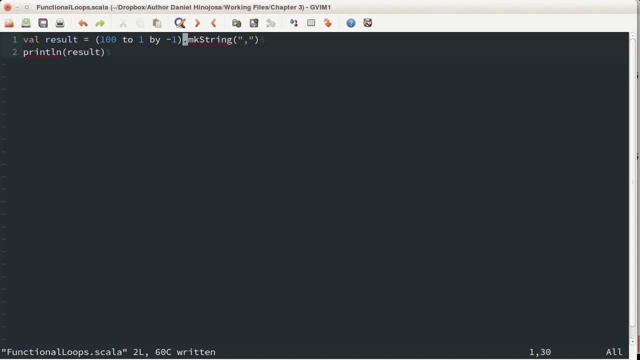 Then creating a string where everything will be delimited by a comma. Since the result is so lightweight as opposed to the full featured while loop, We could also do the following: Now let's run Great, Let's go back to our code. Now, this requires a retraining of our minds to think functionally. we essentially have to make sure that every step of the way is correct. 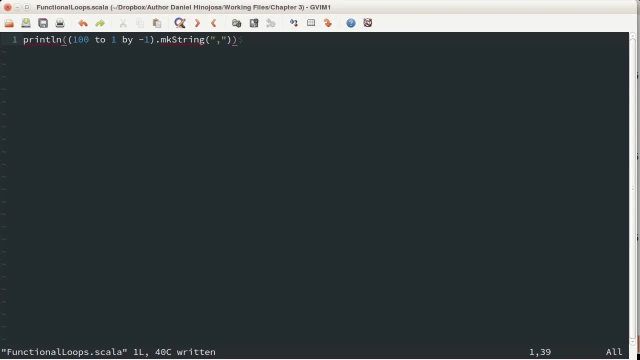 essentially have to usurp years of imperative programming knowledge to do it. And maybe usurp is too strong of a word, since we don't want you to intentionally forget things. We want you to build upon your years of imperative programming knowledge. but the rewards and efficiency 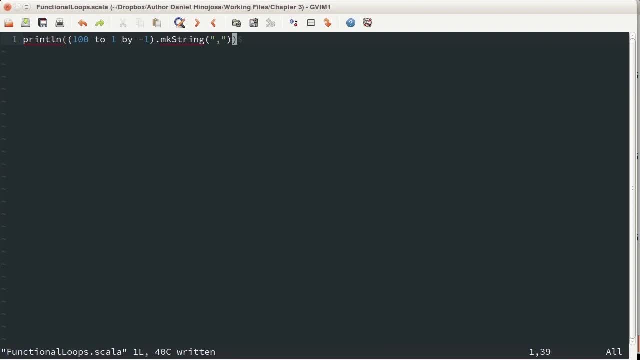 readability and maintainability in functional programming will be revealing over time. So the verdict of while loops: not use that often, There's usually some sort of programming that you can do functionally in place of the imperative programming, And there may be situations where 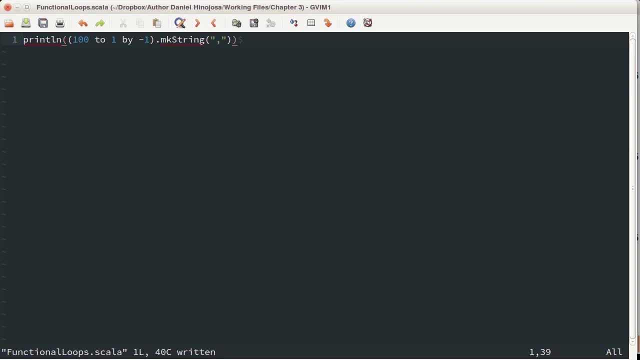 you have no choice or intentionally require a while loop. but its use in Scala is going to be limited, And that goes for its crazy cousin, the do while loop. So let's refresh our memory with a do while loop. I'm going to create a file called do while loops- dot Scala. Here we are in the file. 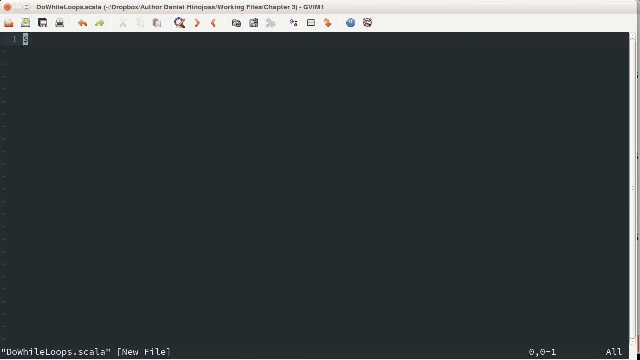 do while loops, dot Scala, And we're essentially going to write the imperative programming example we did at the beginning of this session, But this time with a do while loop. Now let's add a print line. Okay, same thing. This is a do while loop while a is greater than zero. 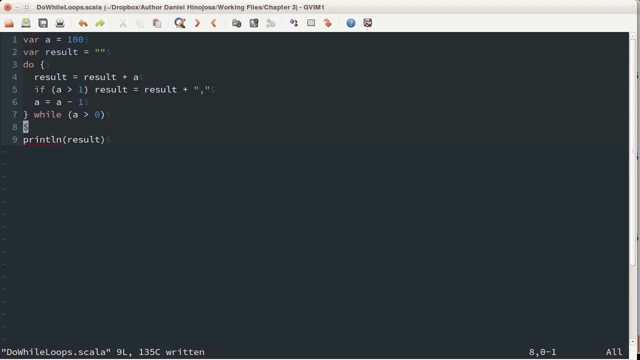 we are going to append to it. If a is greater than one, we'll add a comma to it. That way we can delineate between all the different numbers. And again, the do while loop- for those I forgot, same as the while loop, except it will always go through, at least. 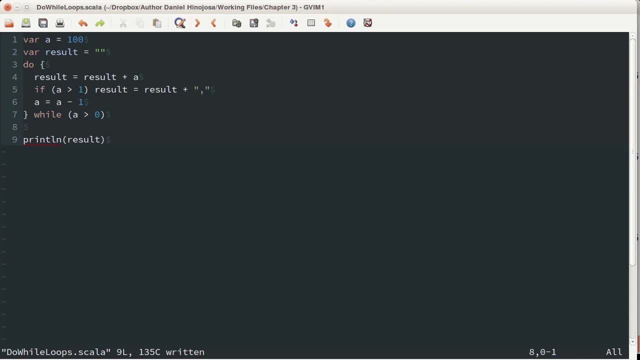 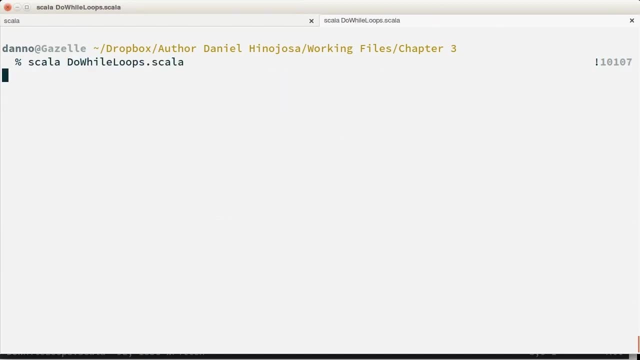 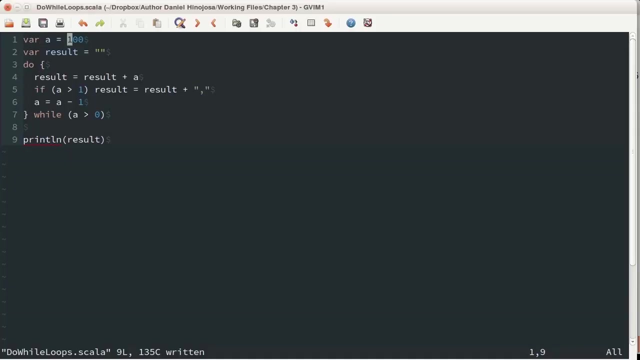 15. One iteration, And if the variable a was zero in this example, it would at least just print out the first number. But let's give this a try. Works out very well. But now let's change things around, Because this is a do while loop. let's say we changed a to zero, Now let's run it again. 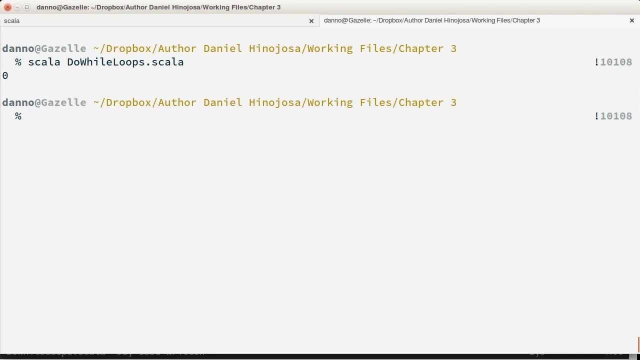 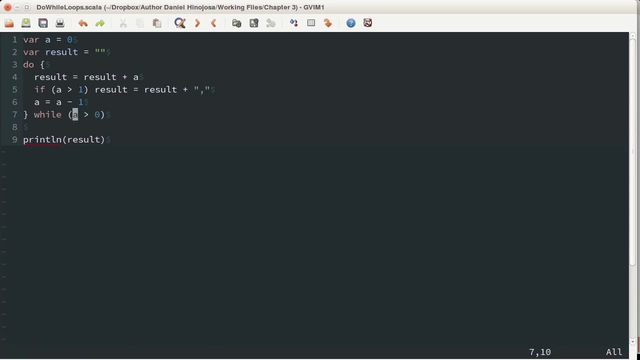 As you can see here, we get a zero because a is established as zero. Let's go back: a is established as zero And our while loop has a greater than zero, But a is not greater than zero. So therefore our do while loop is going to iterate at least once. So, in conclusion, while do while exists just like any. 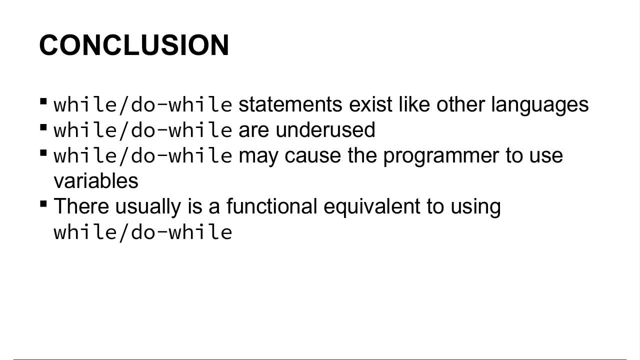 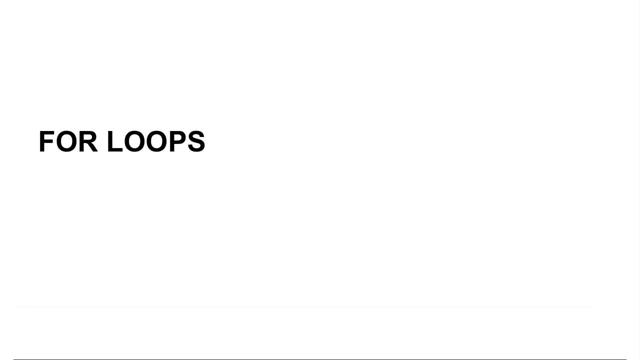 other programming language but that's rarely used in Scala. While in do while may cause the programmer to resort to variables and mutable state And there will always be a functional equivalent for a while or a do while loop. In this session we'll be showing for loops in Scala and contrast them with for. 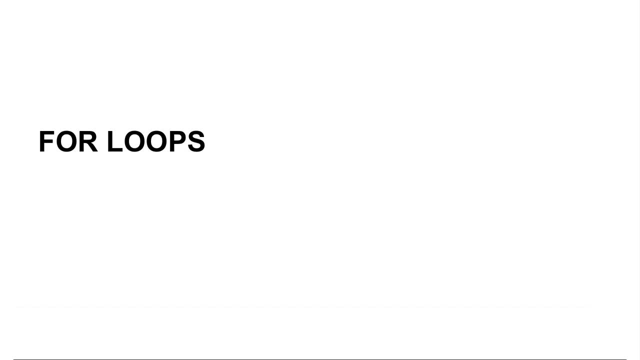 comprehensions For loops are going to be interesting, for loops are also underused in Scala And, to be clear, I did say for loops. In other words, the way we knew for loops will be underused will be migraine for the most part to a concept called for comprehensions And that is an 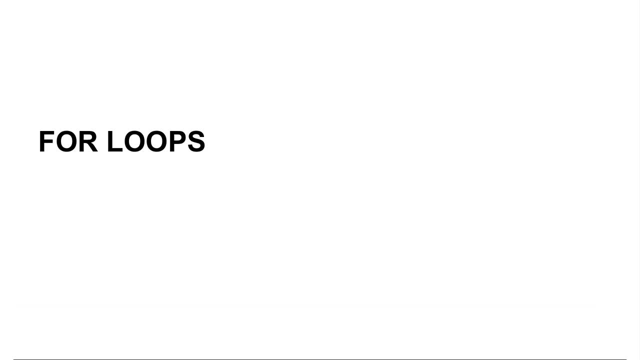 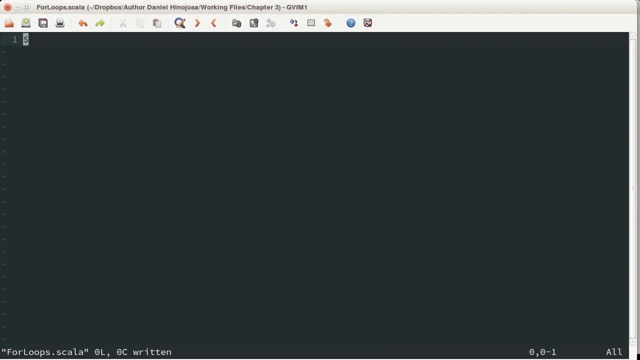 idea that is consistently used. But first let's start off with a review of a for loop, And we start off inside of a file called for loops dot Scala. Here we are inside of for loops dot Scala And we're going to get started with a result, And we're 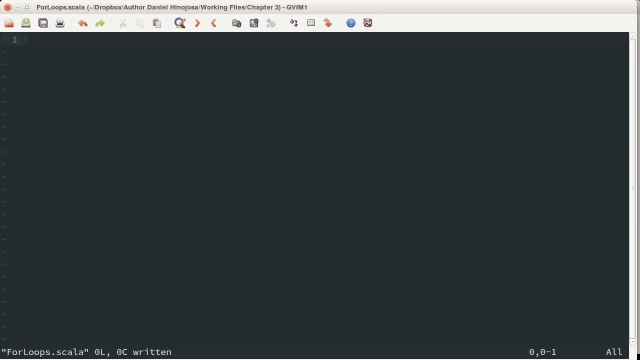 going to this time count from one to 100. And we're going to print the results with a comma between each number. This is very much like our while do while example, but this time using a for loop, And that way we can become reacquainted to what a for loop looks like. Let's get started, And here's our 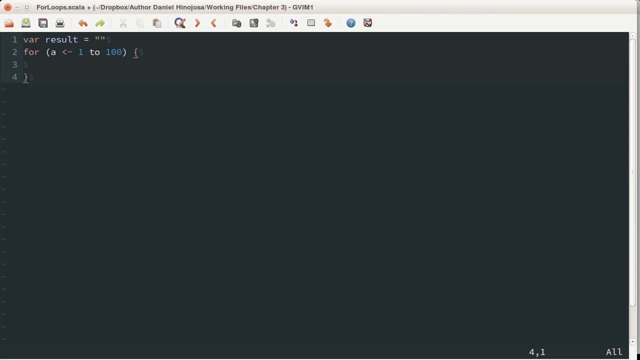 for loop. It should have looked similar from one to 100.. For each iteration, we're going to assign that to a and within the block inside of the for loop, we can use that a, however we would like to Right. So for one to 100, we are going to assign each iteration to a and we will append it to the. 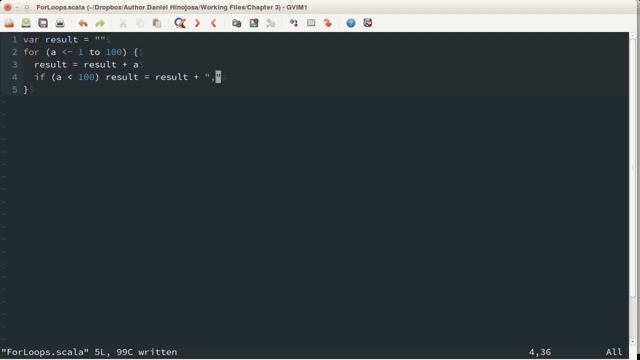 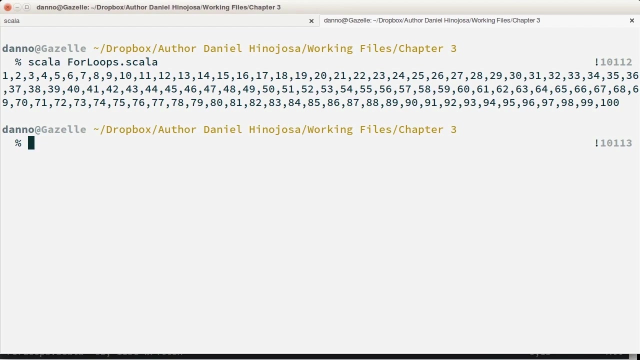 string And during this time, if a is less than 100, then we will go ahead and make sure that there is a comma. Now, at the end of all this, let's go ahead and print Out the result. Let's go to run it. There we go: 12345, all the way up to 100, with a comma between each. 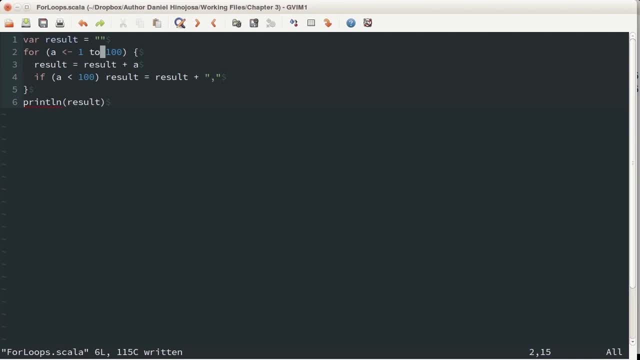 number. Let's go back to the code Now. this is a typical for loop, the way you've known it for many years, And just like the while and do while. in order to use it, you typically have to have some sort of mutable variable- typically, but not always- And you have to have that set up in order. 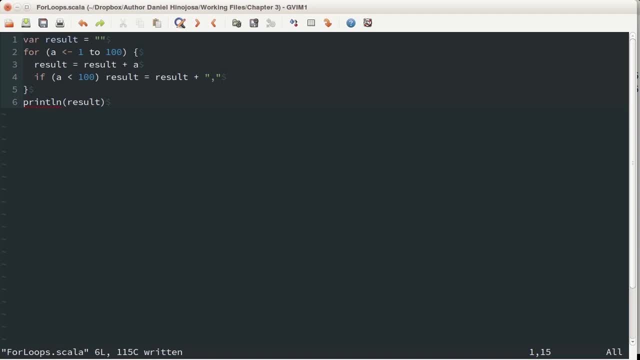 to use it. Now, this code example again is much like the while and do while example, And you can see that the first two examples we've had before. Now, again, this is an imperative style. What we're going to be looking at in this session is more of a functional style as well. Now we mentioned four. 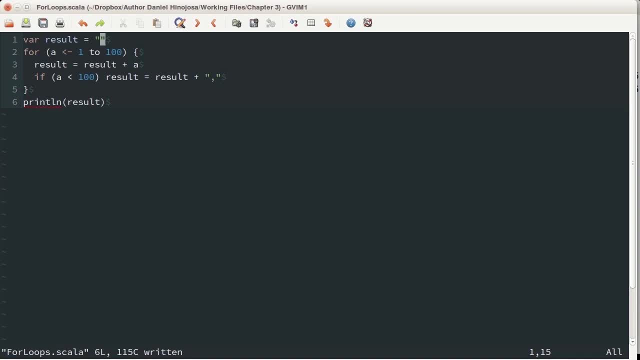 comprehensions already, And since Pandora's box is already open, we might as well serve it to you up as an appetizer. But first let's go about this the long, imperative way. So we've seen this example, And this is just a typical for loop example. But now let's do something where we want to do some. 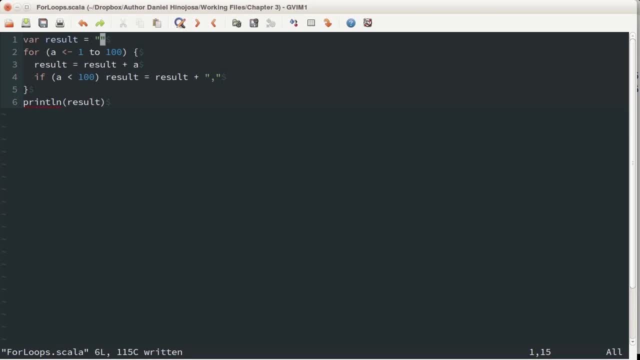 sort of computation for every item within a list And we want to create a resultant list based on that computation. And we're going to start off with a file called for loops to dot Scala. Let's begin, Okay, and here we are, inside of a new file called. 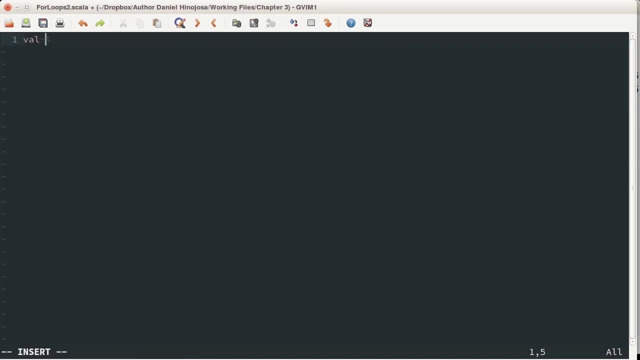 for loops to dot Scala, And we begin Now in Scala. this is a list, list of 123. And for this is a list of int. And what I want is: I want to create a list of int, which will be the result. And what do I want in result? I want every element inside of X s to be added by one and placed inside of this. 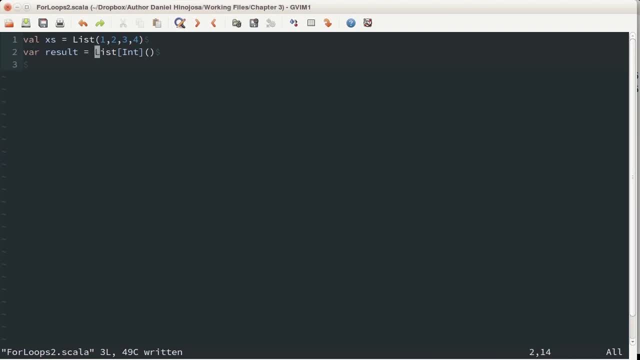 new result list. Now, what is this bracket here? we'll talk about this in another session when it comes to collections, but this right here is a parameterized type or a generic type. This just says this is a list event And because this list is empty, I have to declare that this is a list event. I could 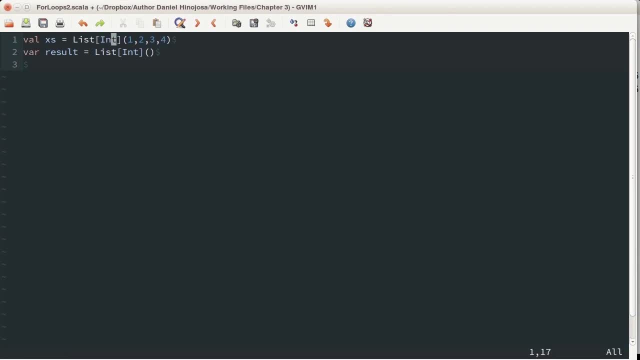 have done the same thing over here, But have something called type inference, so i don't actually need this here and again for more information. we have a few sessions for collections and how all this works. okay, but there it is. so we have a list of one, two, three, four. i have a resultant collection that is going to hold. 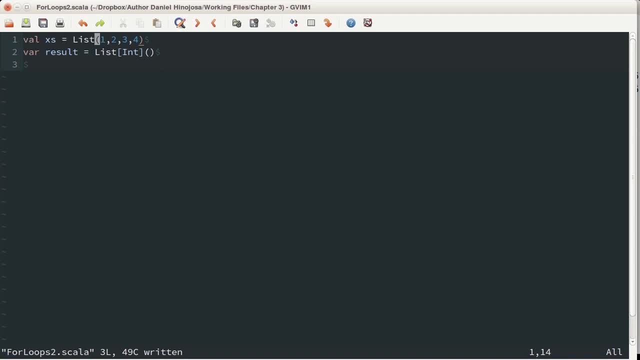 the same elements as xs, but we're going to add one to each element. now. let's create the for loop now. this may be a little bit mysterious here, so let me stop right here. this is actually just a method on a list and this is just a way that we could append an item to a list and that's all. 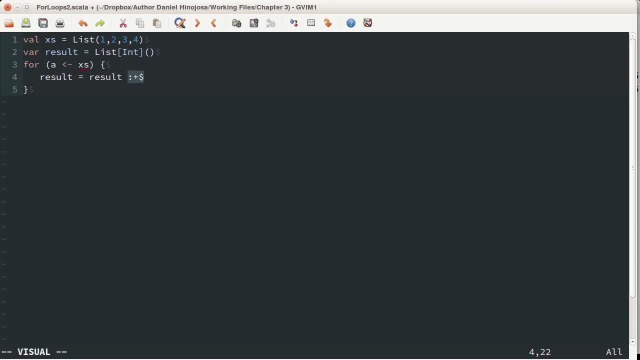 that means there is something called operator overloading, and we have more on that topic a little later. and what we're going to append to this result? well, we're going to append whatever a is, but we're going to add one to it now. we'll print out the result. now let's run it. 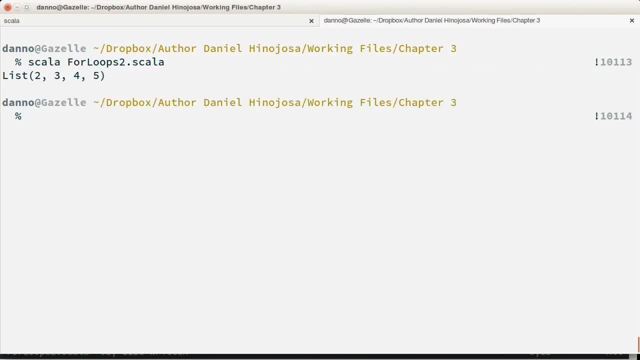 great list: two, three, four, five. that is the list of one, two, three, four, but we're adding one to each individual element. not so bad. again, we took each element, added one to it, created a new list. we got what we wanted. of course, the pain point is that var, let's go back. 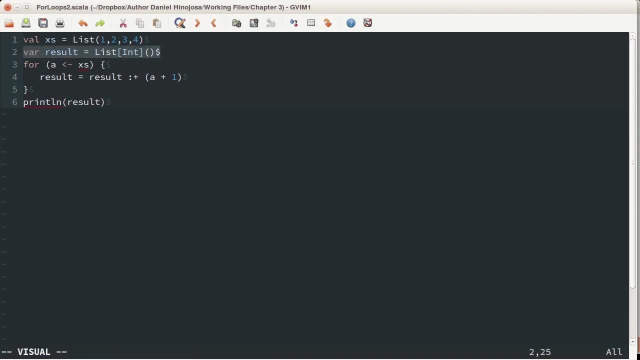 so here's that var. once again, remember we don't like that var and we want to try to avoid it again. it's worth reiterating: sometimes there's no way around it, but we want to try to avoid it. again, it's worth reiterating: sometimes there's no way around it. 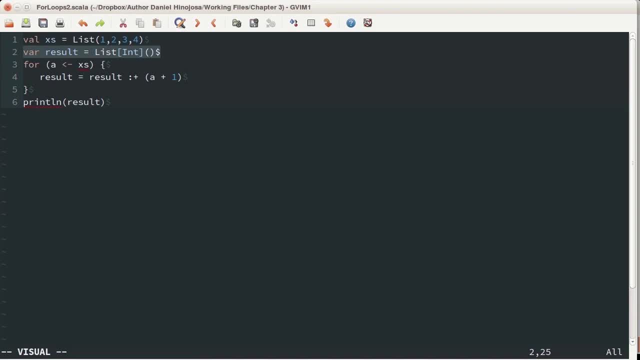 we'd like to keep this as a val, if we can do so. so let's try this again in a functional way, using a for comprehension, and this time i'm going to create a file called functional for loops. okay, here we are, inside of functional for loops and we're going to do nearly the same setup now. 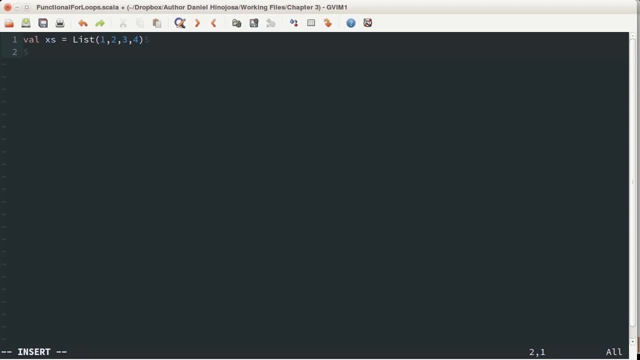 we are setting the result to the. for comprehension, this should look kind of similar to that functional if statement we had a couple of sessions ago, where we take the result and apply it to a value. so we're going to do that, and we're going to do that, and we're going to do that, and we're going to. 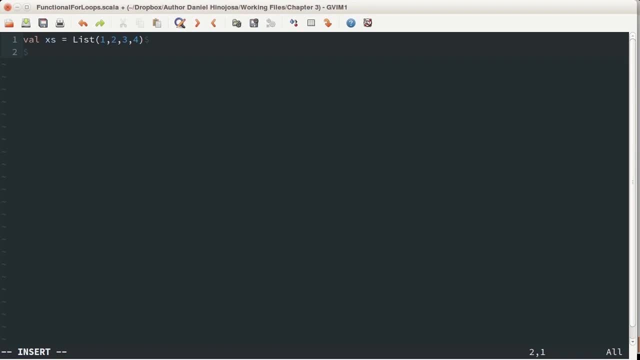 the only difference now is we're also going to be using a keyword called yield, and yield will essentially yield a new collection that will be created and the value is calculated, and in this case this would be a plus one. but let's see what it looks like first, and then we'll describe it. 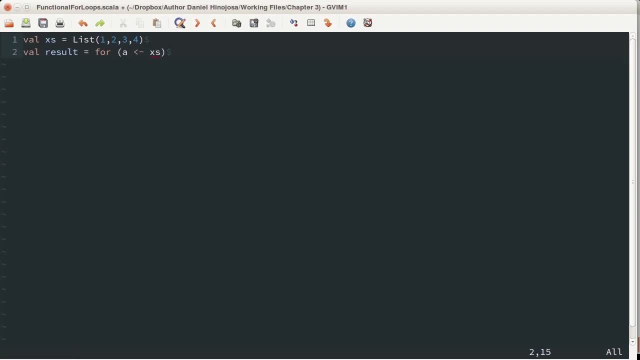 now this right here is what i was talking about, where it looks very similar to if. if you remember, a couple of sessions ago we had the if statement. but what was really weird about doing it functionally is that we can take that if statement and assign it to a function that is. 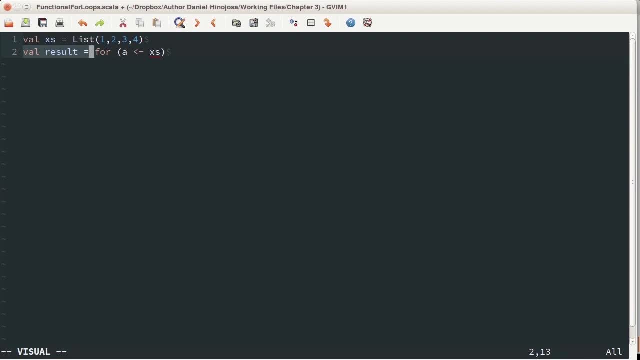 assigned it to a value. well, this time we could take a for loop- or what we seem to think is a for loop, it's actually a for comprehension- and assign that to a value. and remember, it says val result, it does not say var result. and now i'm going to call yield. yield again just means that for every item. 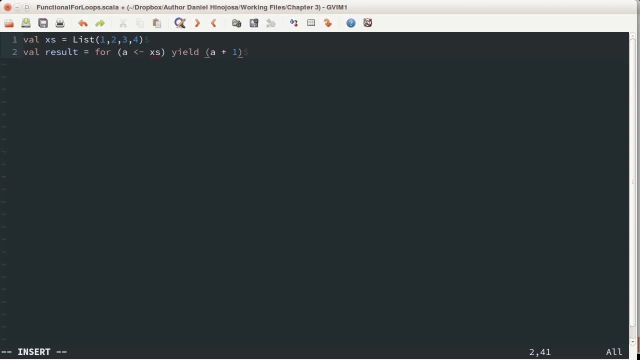 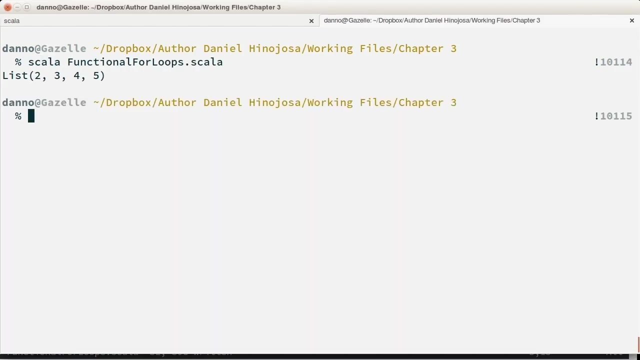 that we get. i want to add one to it and yield it back to a new collection, and now we will print the result. okay, that looks like a good idea, so let's go ahead and do that, and let's go ahead and run it. we're going to run. functional for loops, dot scala. it looks the same, doesn't it? let's go. 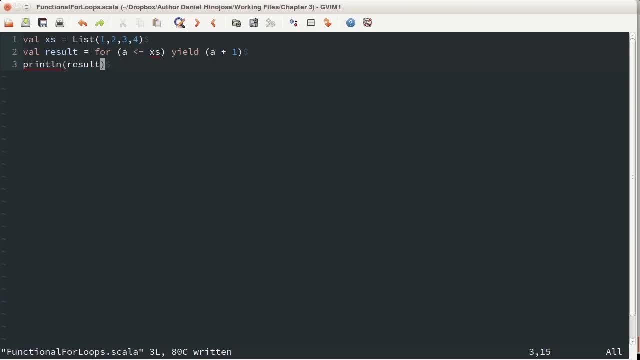 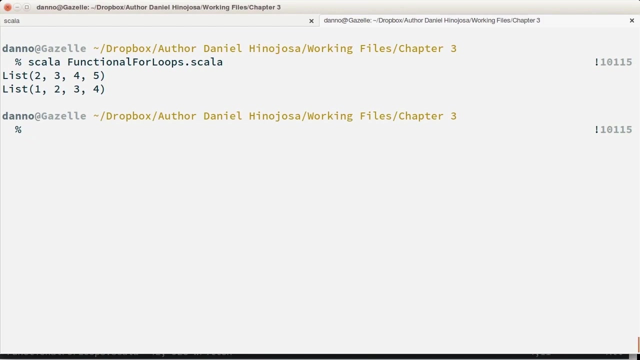 back to our code, we see that this created a new list and if we wanted to, we could do just to verify that we have an actually a new collection out of this. so let's save this and let's go to run it. first one is the new result. the second one was the original xs that we created. so 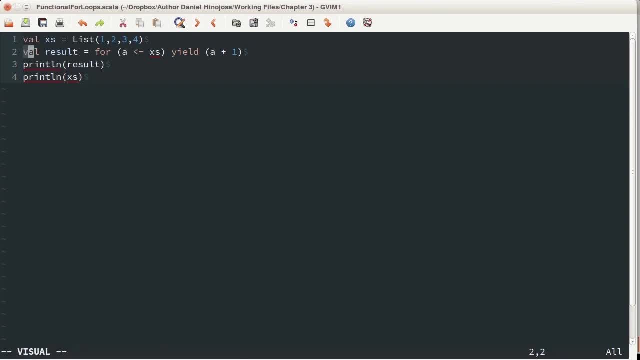 what we can do is we can reset the list to the new one and once we have it, we'll be able to see how it works, and then we'll be able to check out if it's still on. and if the current one is still on, i'm going to go back into the fadeoblack via setup and going to the 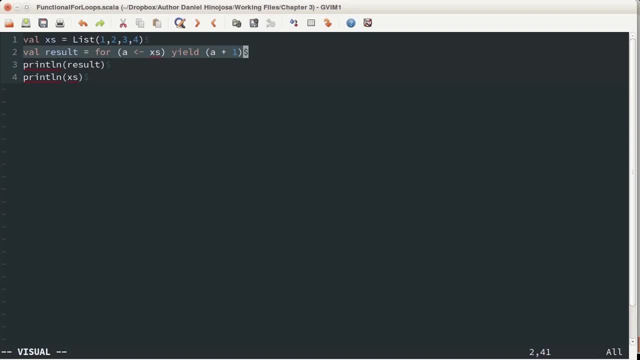 file editor to fix that. and let's go ahead and go to our class, our class. we will do a very small update now. it'll just be like the previous example, except this part is now in one glorious one line and without mutability in the form of a var and imperativeness. we could just make that assignment. 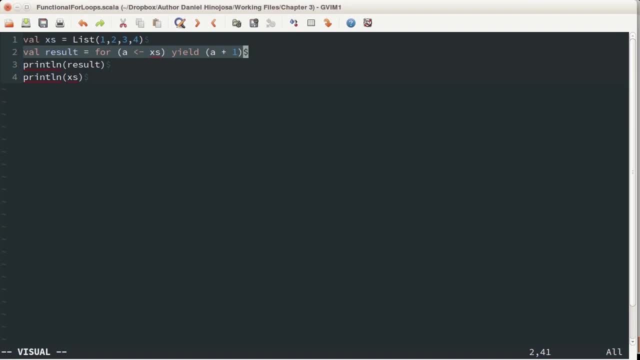 so there's more to what's going on. we'll revisit this topic when we discuss maps and flat maps. for now, just notice that the result is also a list. now again, the access stays the same and by default, every operation and scala will return a different, different collection from the original, since the original collection is likely immutable and in 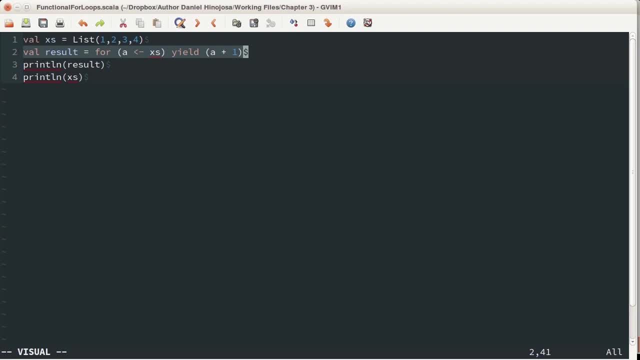 this case, that list one, two, three, four is an immutable collection. I did say likely because there are ways to work with mutable data structures in Scala, but for now we're just focusing on the immutable data structure. So it is important to stress again also that with a for comprehension, 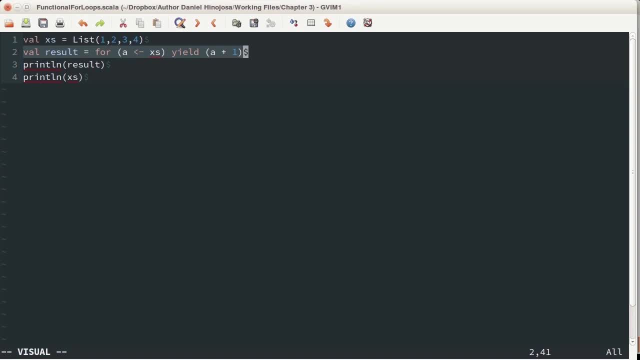 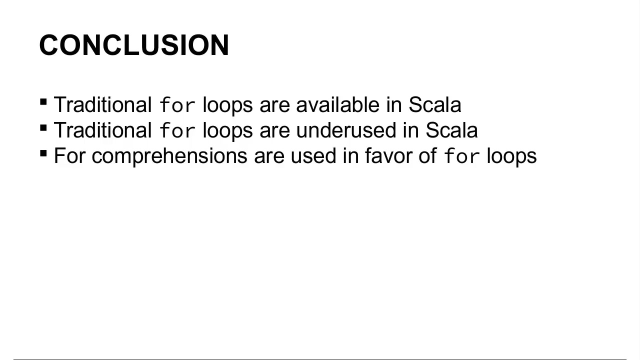 the collection type that we get from yielding will typically be the same type as the collection we first started with, and in this case it is a list. Result here is of a type list and, to be more precise, a list of int. So, in conclusion, for loops are available in Scala and you can use them just 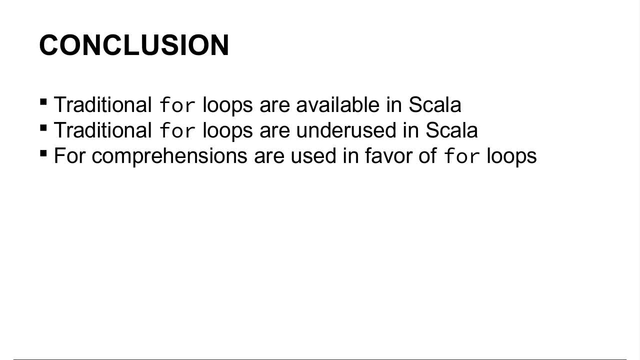 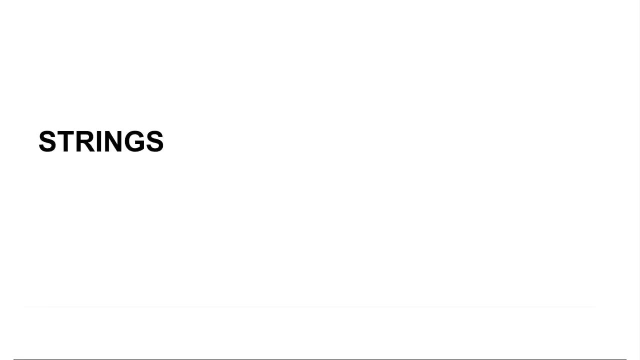 like you've used for loops in other programming languages. Now the traditional for loops are actually underused in Scala. Scala programmers, the more advanced they get with the language, will start using for comprehensions more in favor than the traditional. In this section we'll be talking about strings. Strings retain the same basic structure from Java. 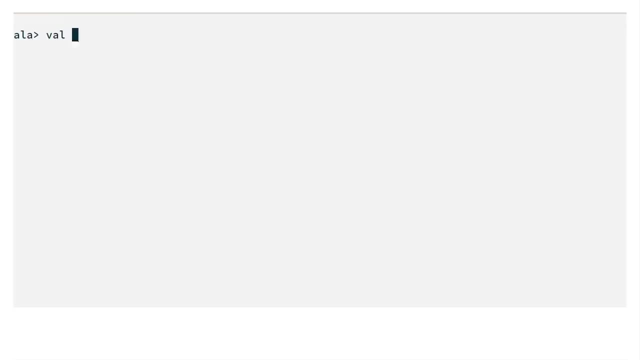 Java lang string. So let's start with a REPL. Let's get started with a very simple declaration. Valet is equal to Scala. As you can see, here, the string is surrounded by quotation marks. If you want to specify a type, you can. of course, you can always place it in the beginning, or you can always. 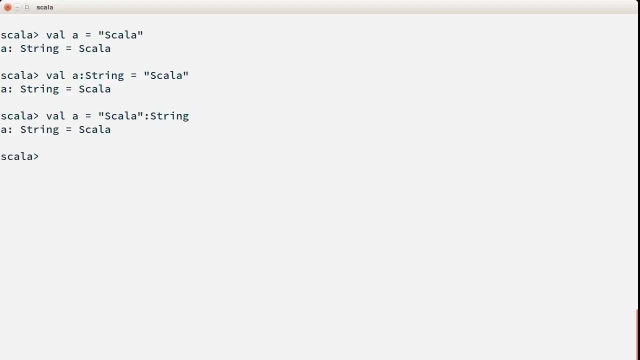 place that in the beginning. If you want to specify a type, you can, of course you can always place it in the beginning, or you can always place that in the beginning. If you want to specify a type, you can, of course you can always place that in the beginning, or you can always place that in the end. 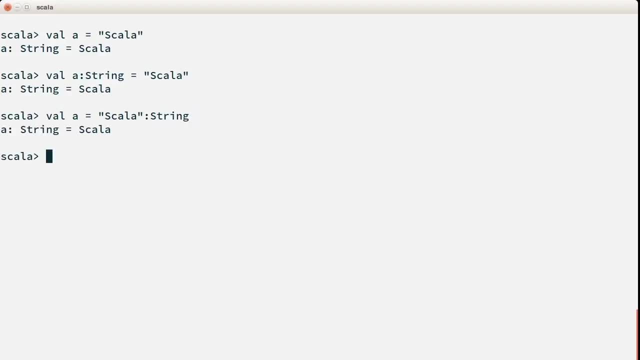 But this is usually unnecessary, since the type has already been inferred. Strings are not primitives like numbers, boolean and characters. For Java programmers they contain nearly all the same methods as you'd expect from Java- lang string, but with more functionality: All the methods that are available in other collections in Scala. 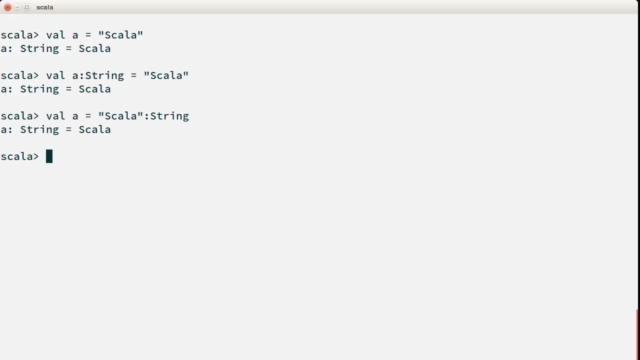 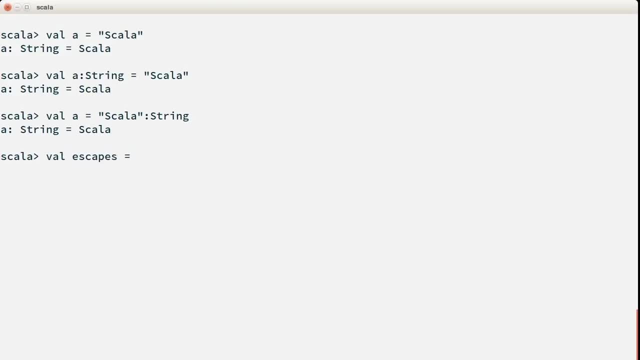 Strings can also have escape characters like tab, new line, carriage return, and so on. Let's try one. I'm going to create a string called escapes. Here's a tab, Here's a new line, Here's a carriage return. 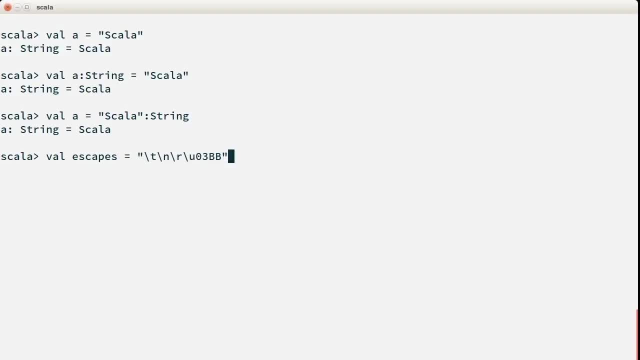 And finally, here is a unicode. And finally, here is a unicode. That should be a lambda. So we have our tab, We have our new line, We have a carriage return somewhere in here, We have a carriage return somewhere in here And we have a lambda. 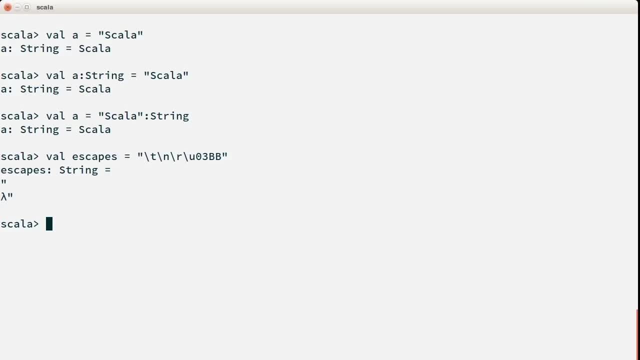 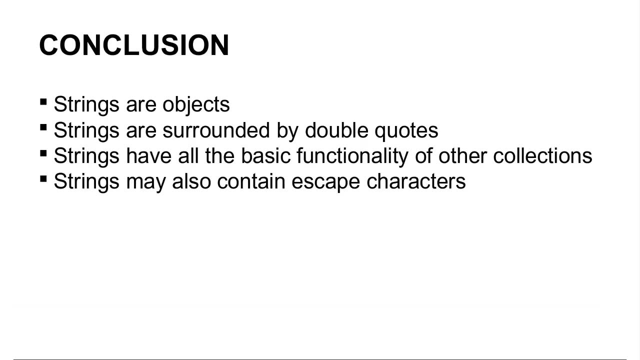 This has been a very trivial section on strings. In the next section we'll show different types of strings, called a smart string. In conclusion, strings are objects. They are surrounded by double quotes and they have the basic functionality of other collections. Strings can also contain: 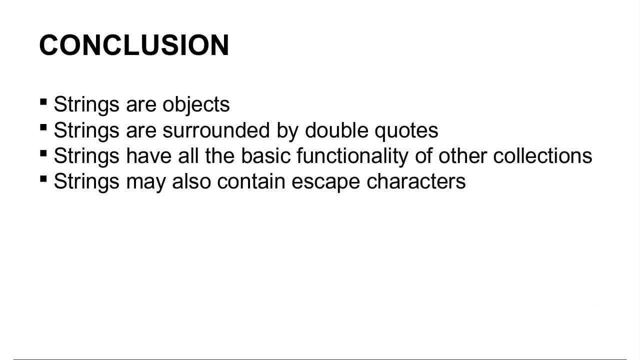 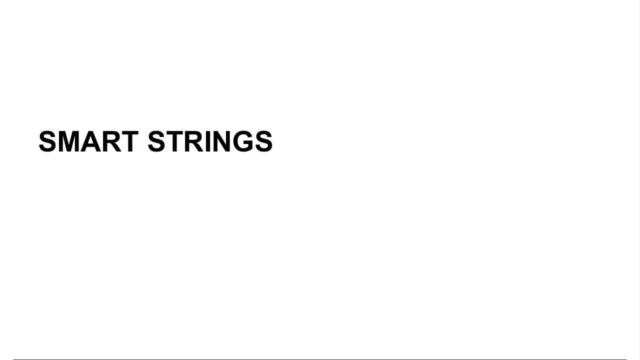 your escape characters like tab, new line, carriage, return and any kind of unicode escape and any kind of unicode escape. In this section we'll be discussing Scala smart strings. Smart strings are a wonderful string construct that makes development a pleasure to work with in the Scala programming language. 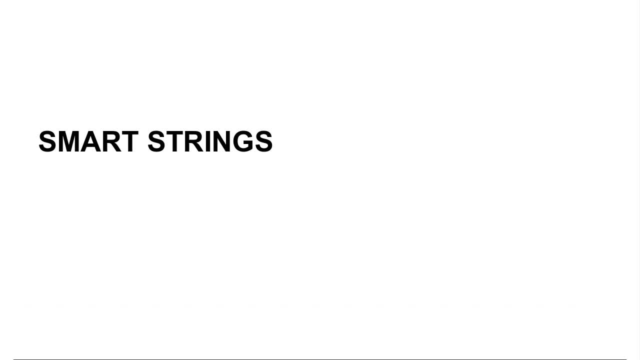 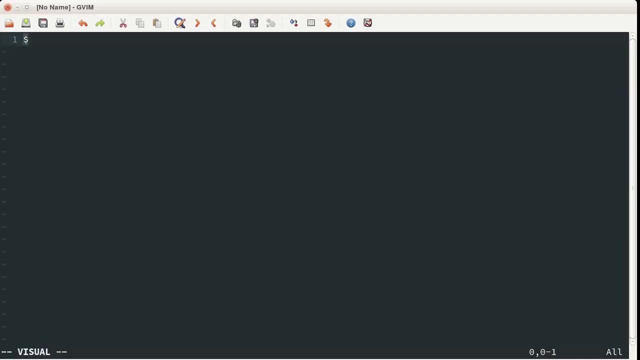 Mostly because it gives us things like multi-lines and sane regular expressions. So let's start off with a file called Smart String Scala, where we'll create a multi-line string in the old classical way. So let's jump over to our editor. Now let's get started here. 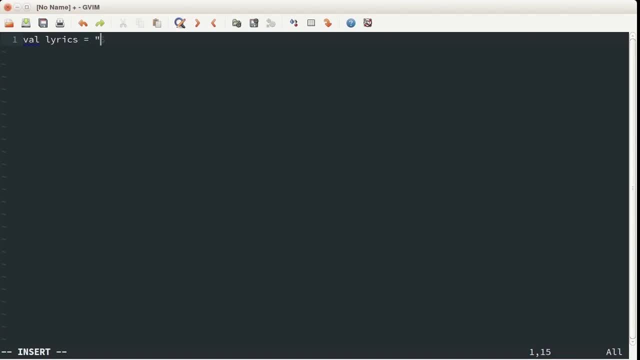 And we'll get started with some lyrics. So let's create some lyrics, Let's break out the Louis Armstrong. So we'll start off here with: I see trees of green, Red roses too. I see them bloom for me and you, And I think to myself. 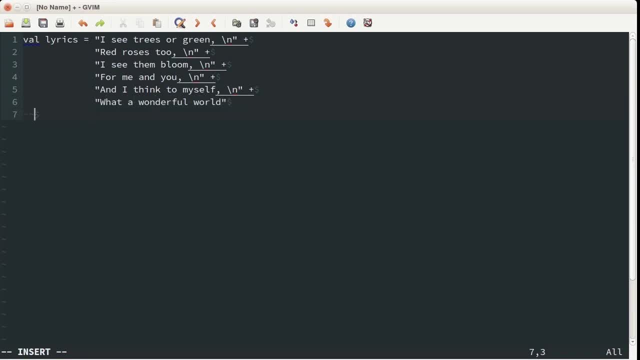 what a wonderful world. Let's go ahead and save this as smartstringsscala and let's finally do a print line on this, And we should be good to go. So there is our multi-line. This is the old, classic Java way of creating. 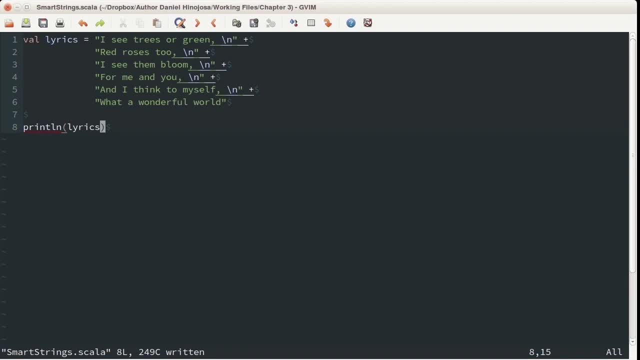 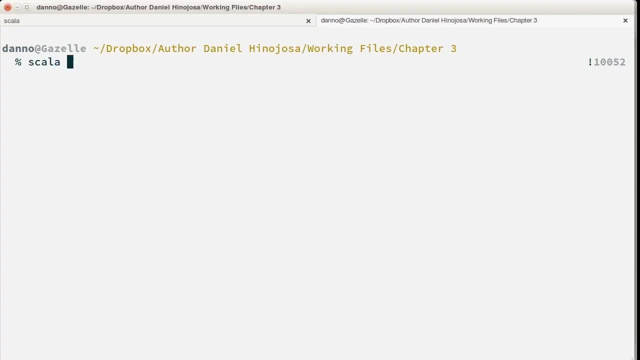 a line each. We have to put carriage returns on this. We have to add plus at the end of each line. It can get kind of messy. So let's run this at the command line and smartstringsscala and looks fantastic. The only problem is it doesn't look quite as 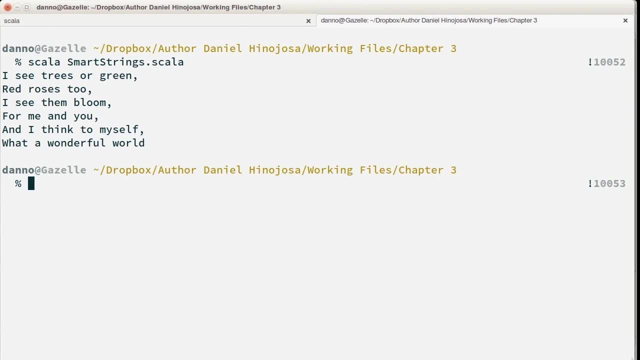 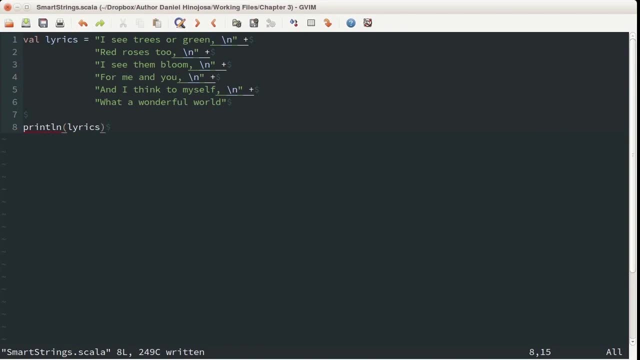 fantastic. on the Scala source code itself, There are a lot of quotes. Again, there are a lot of new lines. So let's clean this up using a smart string. Now, with smart strings, the only role you have to pay is that you need triple quotes at. 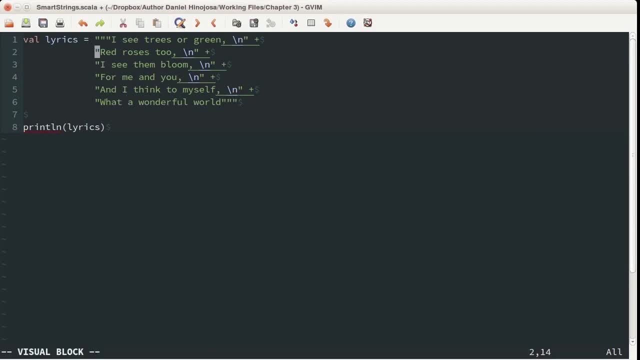 the end of the line. But you can get rid of these quotation marks and you could also get rid of, so let's do a quick search here of all the new lines with the quote and the plus. There we go. So we have. I see trees. 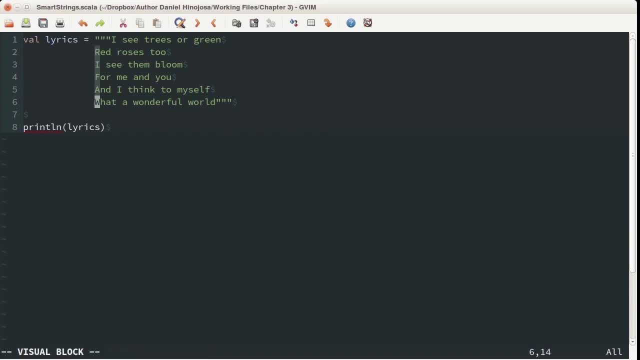 of green, red roses too. Let's make this a little bit more inline. What I'm using here is a visual block. There's something similar in IntelliJ and Eclipse. It's called insert mode. Take a look at your documentation and do something like this. It really 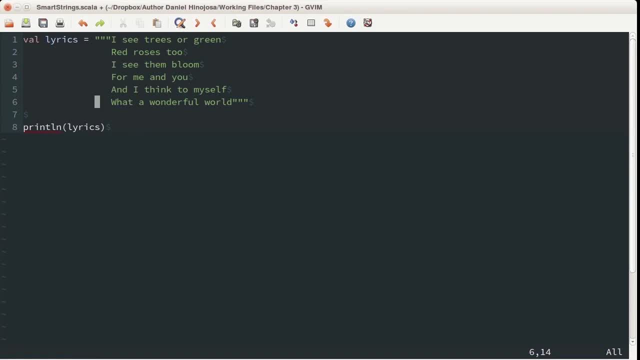 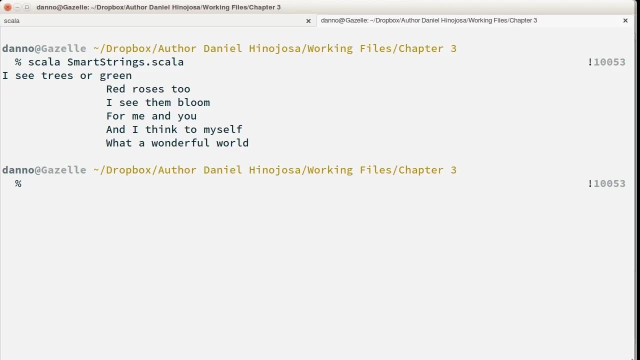 makes programming a lot easier. Okay, There's our smart string A little bit cleaner. Let's run it Now, as we see, with the result I see trees of green is flush to the left border, but we have some space before the red roses too and all the other subsequent. 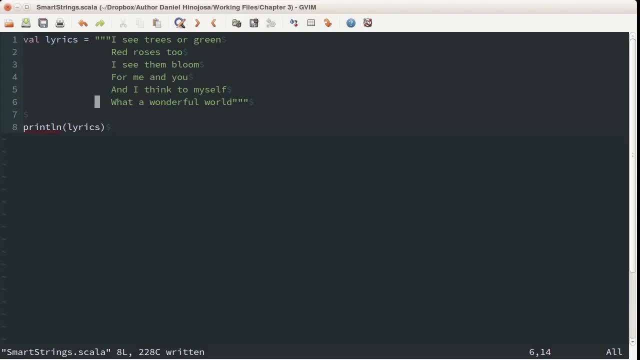 lines. So let's go back to the code. We have an issue, And the issue is that Scala is merely doing what we told it to, And we have this large block of line and all Scala is doing is interpreting these blank lines and putting them. 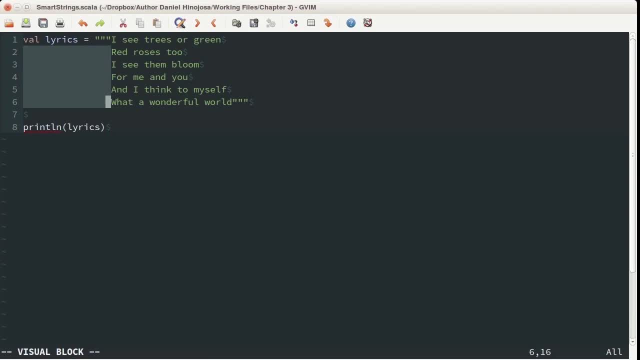 at the command line whenever we run our code. So my attempt to make my code look nice in the editor caused it to look different on the command line. Instead of cutting all this space out, leaving my code ugly on the editor, let's tell the smart string where the margins. 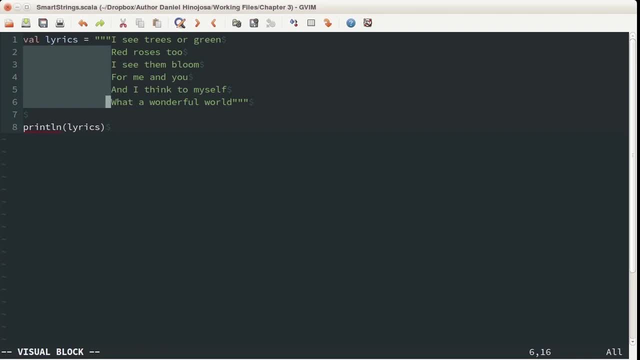 truly began. and let's add a method to the end of smart string called strip margin. Let me use that column mode again, just because it makes things a little easier. I'm going to put a pipe in front of all this and at the end I'm going to call strip. 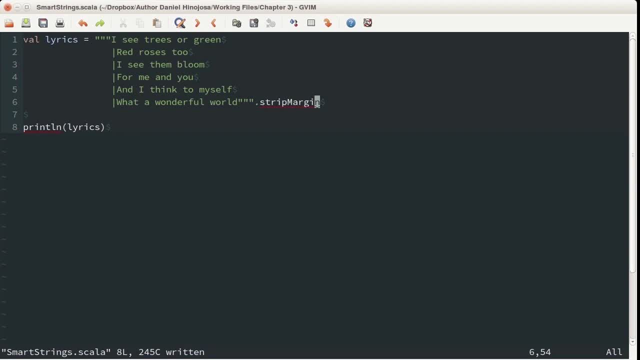 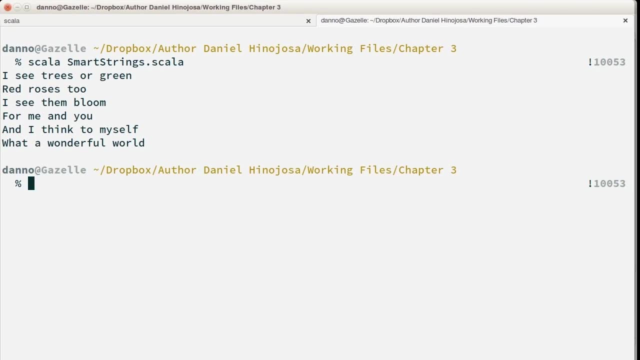 margin Strip margin will use that pipe or the or symbol as the default indicator of margin. Let's go ahead and run this. Great Everything is now flushed to the left hand side. Now I can enjoy beautiful code in both my editor and my command line. 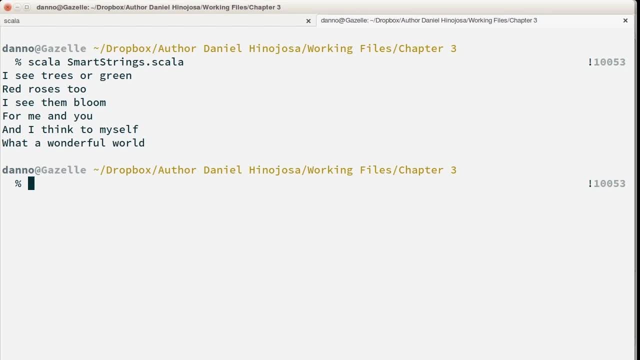 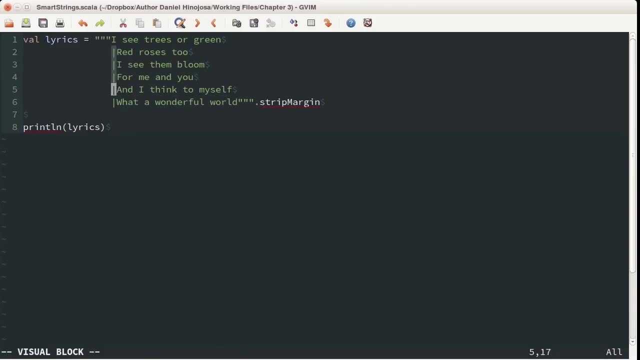 Now what if I wanted to try a different delimiter for the margin instead of the pipe or the or symbol Strip margin will accept any character that you give it. Let's say we wanted to replace all of these with an at sign and what we can do is add that. 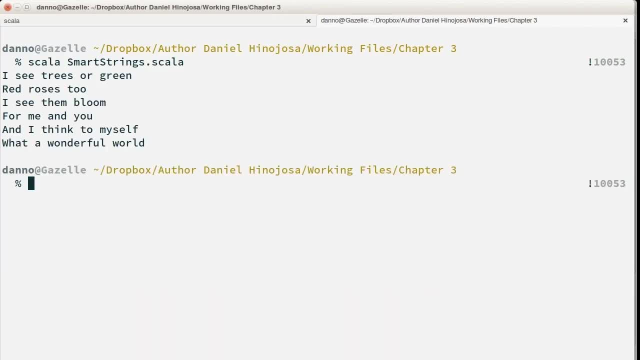 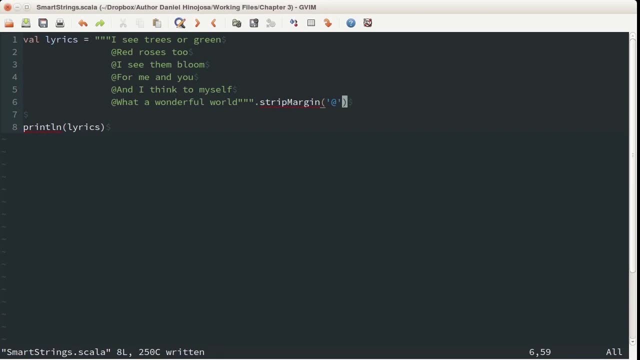 character as a parameter to strip margin. Let's run this Good stuff. Let's go back to the source code and take a good look at it. So, instead of a pipe, again, I am using the at sign. All I have to do is just specify as a method. 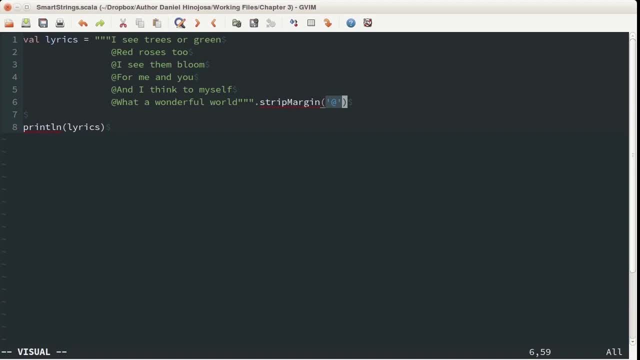 parameter to strip margin that I wish to use the at sign. There is an additional bonus when using smart string, and that has to do with regular expressions, So let's do up a regular expression. I am going to create a message and the message will be: we are. 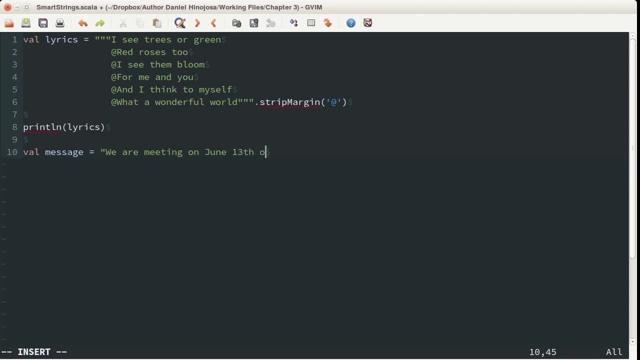 meeting on June 13th of this year and having lunch at 1230 pm. Now what I would like to do is I would like to create a regular expression, and what I want to do is I want to pluck out of this string the 1230. 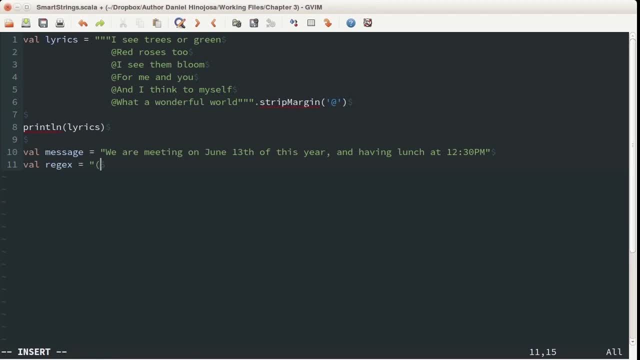 pm the time. So we start off with something optional. So let's say that any space or 0-9 for the hour, the hour might be optional. in case it's like 1 o'clock or 2 o'clock, that's optional and we have 0-9. 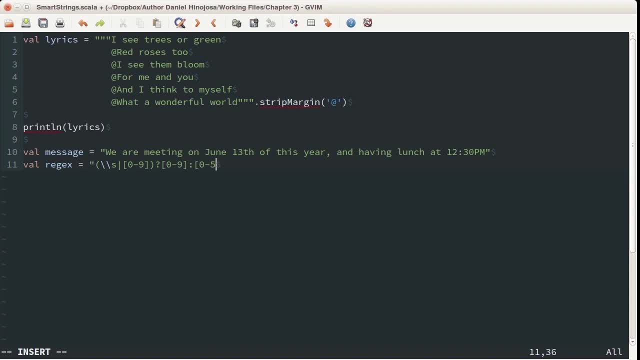 of course we need a colon. and now for the minutes. that could be 0-5 for the first number and let's say 0-9 for the second. We'll need a space, perhaps 0 or more spaces, followed by whether it's am or. 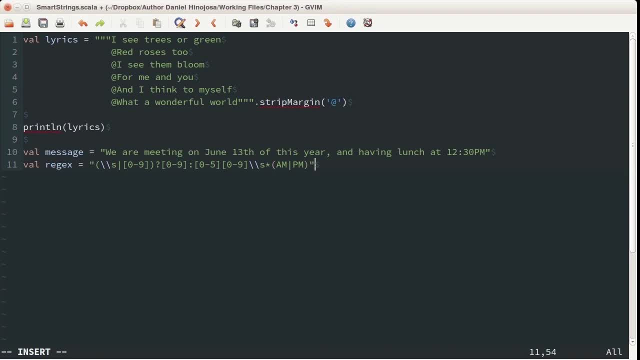 pm. So there's our regular expression to extract the time from the string. To make a regular expression out of a string, we are only going to call a method called R, which stands for regular expression. The problem with this, though, and the problem with a lot of strings in Java: 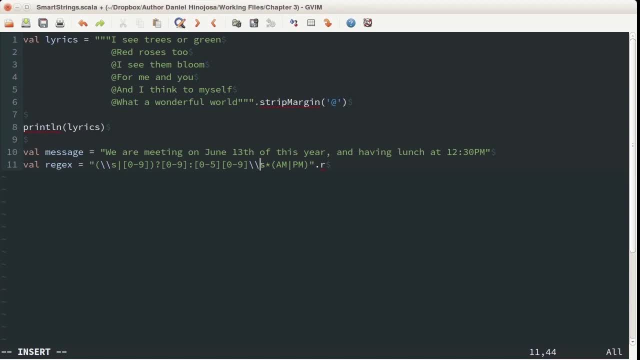 is, we have these double backslides and by nature within a Java string. if we want to create a backslash, we have to do two of them With smart strings. let's go ahead and convert this over to a smart string. we can get rid of the. 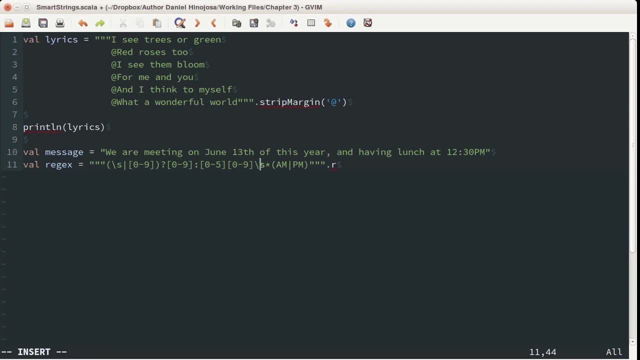 extra backslashes. We can now just focus on the pure regular expression without any extra annoyances. If you're curious about how to use this as a regular expression, let's print out the match. We're calling this regex: find all in within this particular. 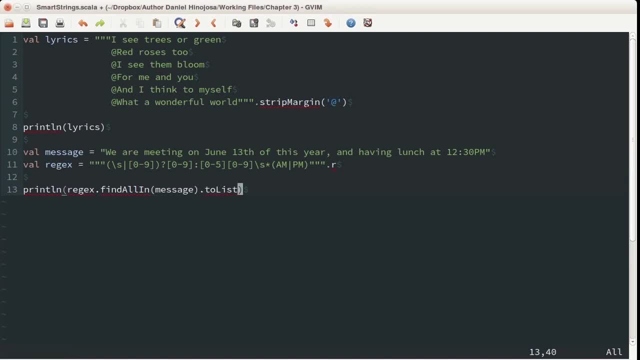 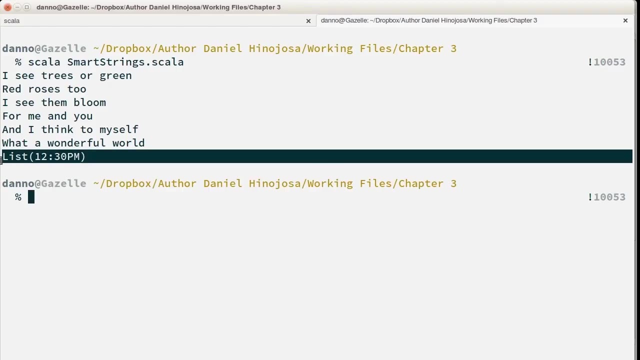 message And let's convert it to a list. You need to list. that way everything is displayed out in a nice way. Find all in will take that regex and find all instances within a particular string. When we run this, you'll see here at the bottom line. 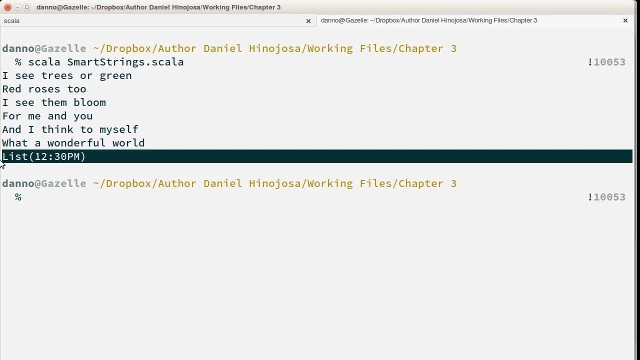 this says list 1230 pm. there was only one instance of a time within this sentence. With Scholar, we can focus on what we want and we don't have to tip toe through a bunch of different rules like the double backslash escape in regular expressions. 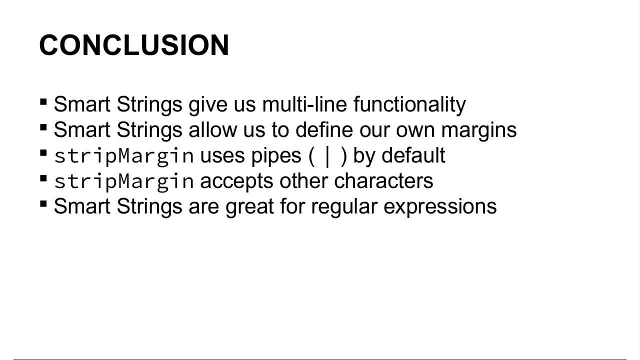 Smart strings gives us multi-line functionality without breaking up this string and putting a bunch of new line characters. Smart strings also gives us the ability to add margins into our code with a method called strip margin. Strip margin uses a pipe or an or operator, if you want to call it that. 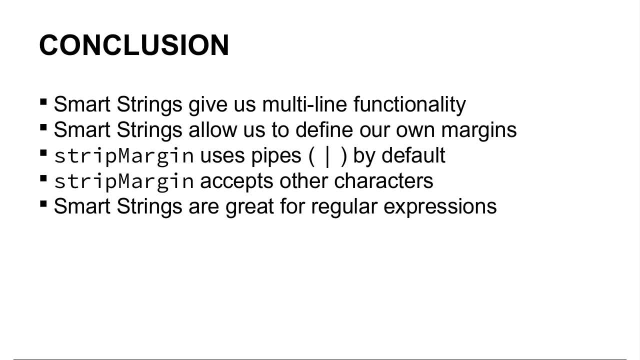 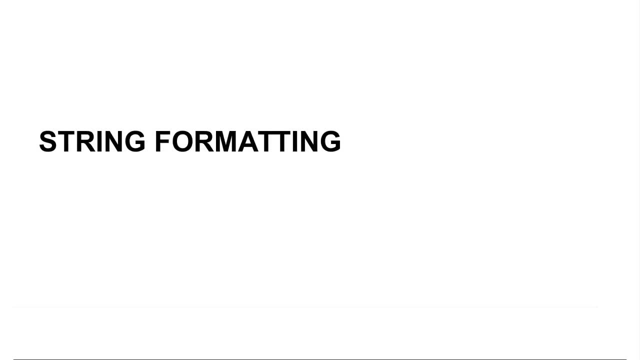 by default, Strip margin also uses another character. if we wish, we just need to provide that with strip margin. Smart strings are absolutely amazing for things like regular expressions by making it easier to escape characters. In this section, we're going to talk about string formatting. 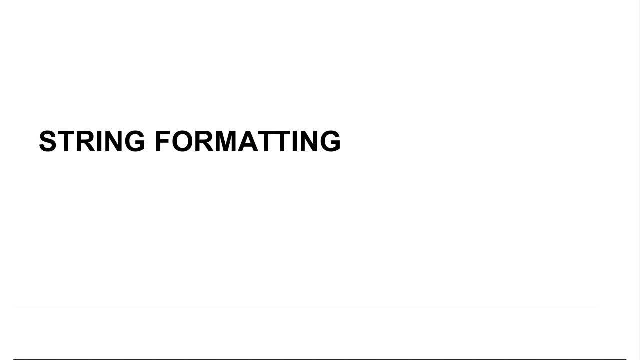 Scholar provides a quick and easy means to do C style or Java style formatting of a string, much in the way that you expect in string format in Java, but with a few changes. Let's go in an editor and try out some of these changes. First off, I'm going to start off. 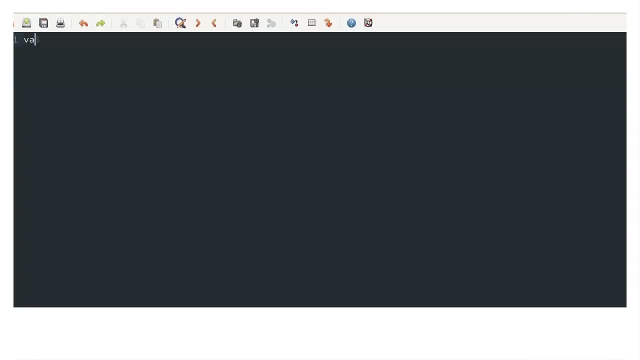 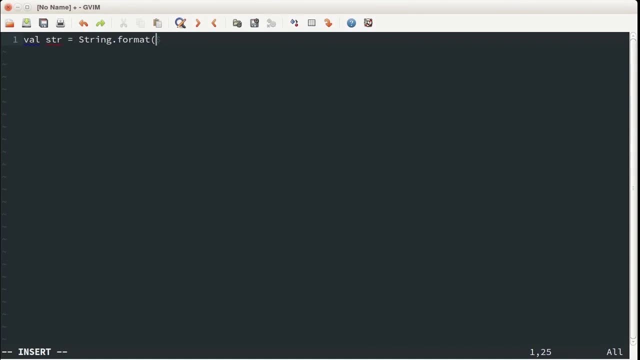 the classic way, using string format. Let's go over to the editor. Let's create a string and we're using the Java style string dot format, using a static method call and we are going to state that this is a percent s and afterwards we are. 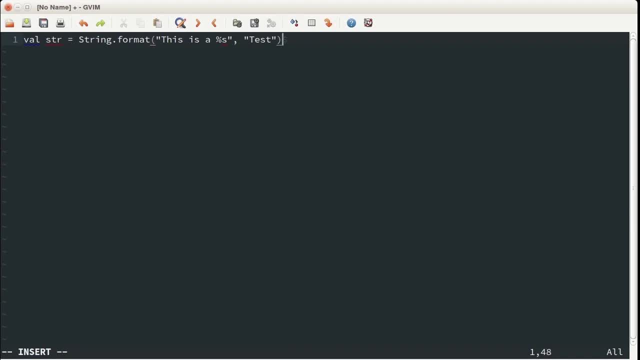 going to state that percent s will need to be replaced by the string test. Let's print it out and let's save this in a file called string format, dot scholar. So we have val str, which is equal to the static method call. this comes from: 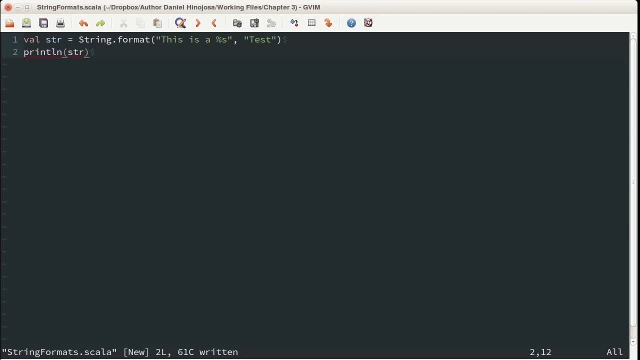 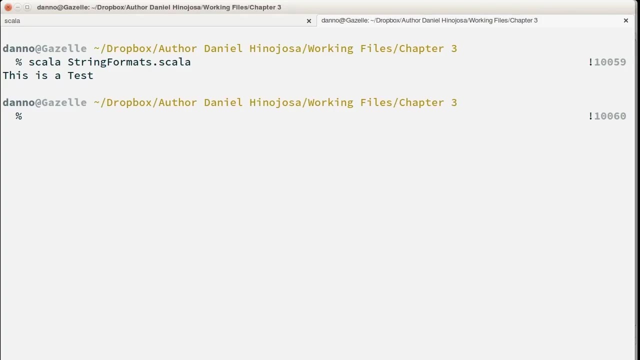 java lang string. there's a static method call called format which brings in a string. we have that percent s and that percent s is going to be replaced by test. We'll print, line the string and see what happens. As we can see, this prints out just fine. 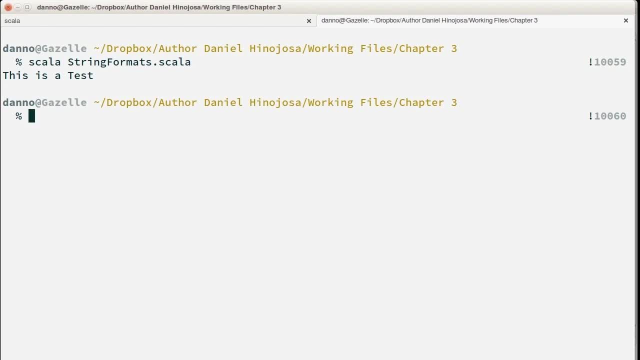 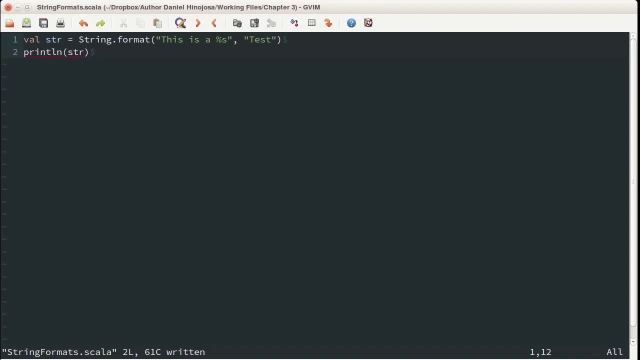 this says: this is a test. Problem is: let's go back to the source code. the problem is that this is a static method call and what would have been preferred is that we just call a method from a string. a string is already an object and it would have been nice and very clean. 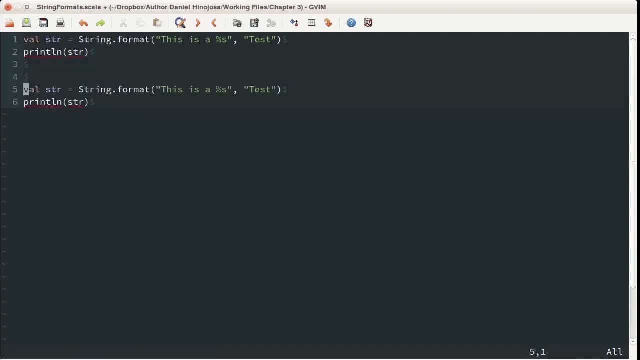 to call it up that way. that's what scholar gives us, so let's take this string and create a different one, but instead of using the java style for it, let's go ahead and use scholar's style this time. I'm going to create a string called this is a percent s. 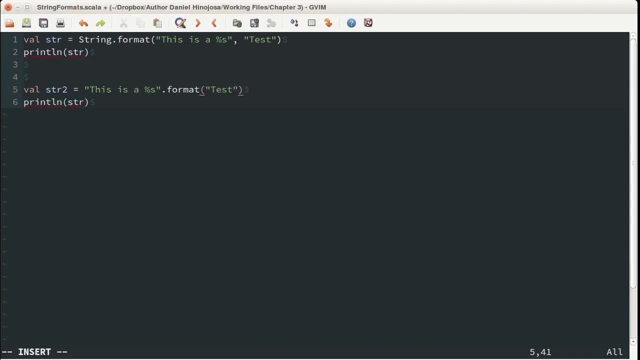 that is what's inevitably going to be replaced, and we're going to call format with test and let's save this. keep this here for a bit so we can take a look at it again. we have a string. this is a percent s dot. format and test. 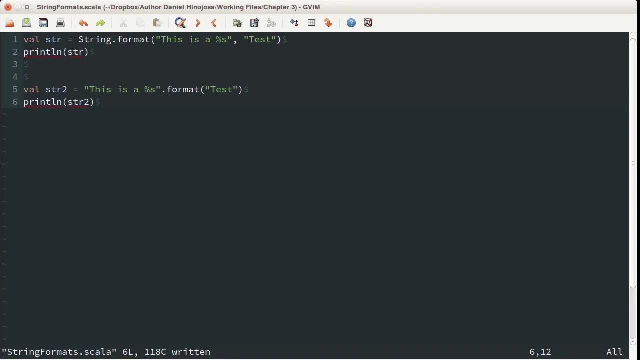 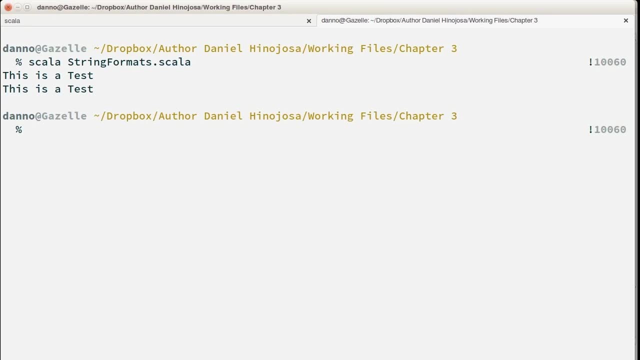 is going to be the argument which will be replacing the percent s. we saved it. let's go to the command line. they're the same thing just a little cleaner. on the second one, using scholar's style string formatting, java and scholar formatting variables can be found at this address. 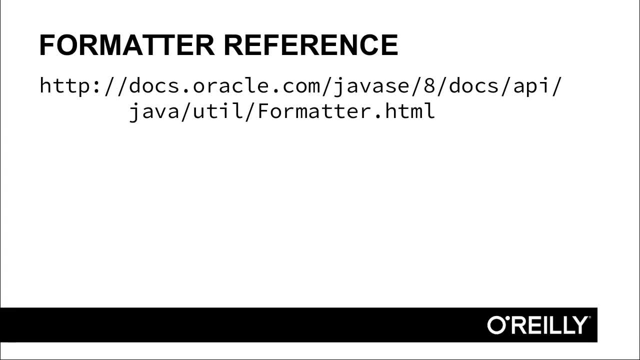 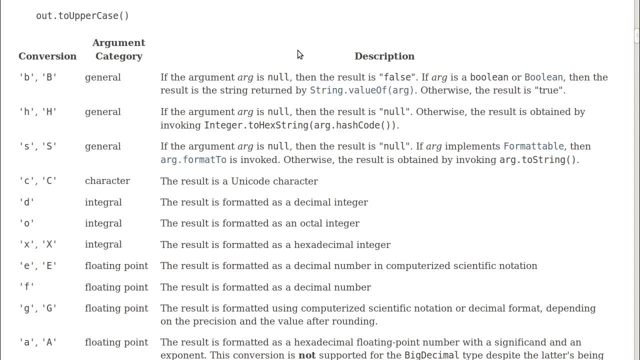 docs dot oracle com. java se eight. we are in java eight. currently docs api java util formatter dot html. let's take a look at an example of what is at this website. we will see that there are different characters representing different types that can be replaced in a formatted string. 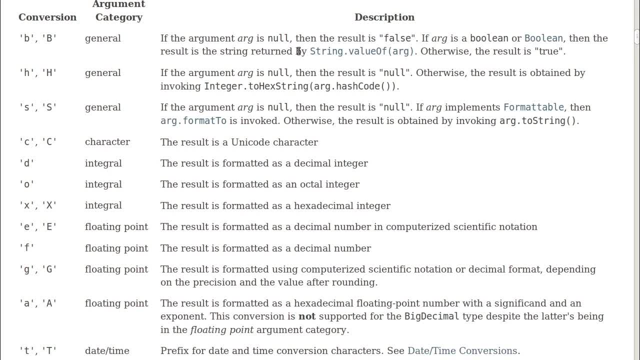 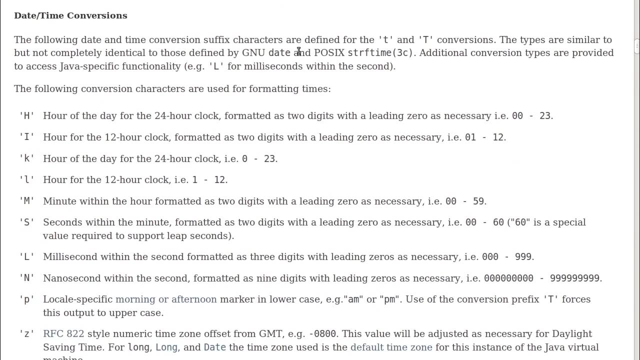 we used small s, but you could also have b for boolean, c for characters, d for decimal integers, o for octal integers, x for hexadecimal integers, f for floating point numbers. we could have n for line separators. we could also use date and time conversions, say, for example. 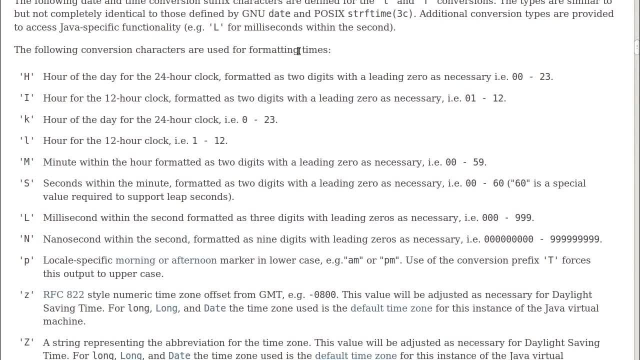 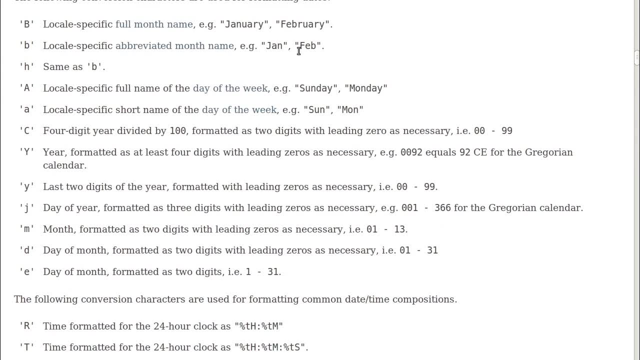 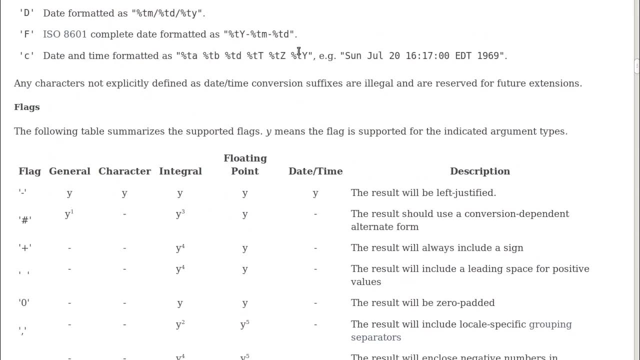 h for the hour of the day, i for the hour of a twelve hour, clock z for time zones, q for milliseconds, and on and on. there's capital b for the full month, name y for the abbreviation of the month, capital y for year, and you could also have different flags. 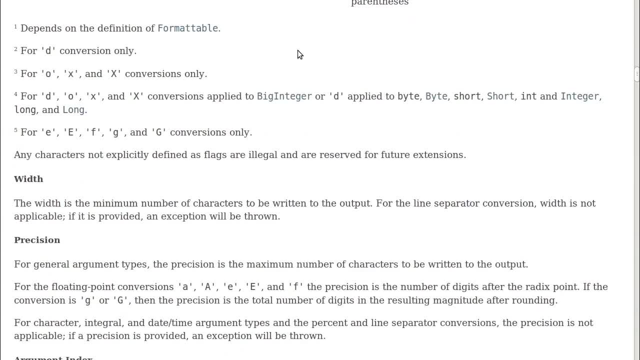 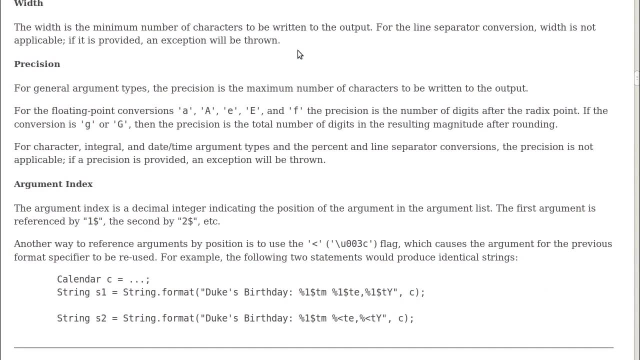 to change the way things are formatted. so go to this website for a reference, and what I'd like to do is use that reference in our code. let's go back to our editor now. let's try a Commodore's classic. actually, I'm not sure if it's Commodore's. 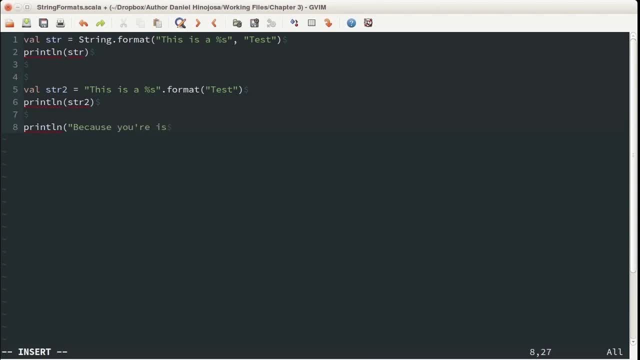 or just Lionel Richie, but it goes because you're once, it's generally, you're once, twice, three times a lady. now let's say we want to use format here. now what goes on here? some of the Java programmers will call this var, args or variable arguments. we in Scala call it repeated parameters. 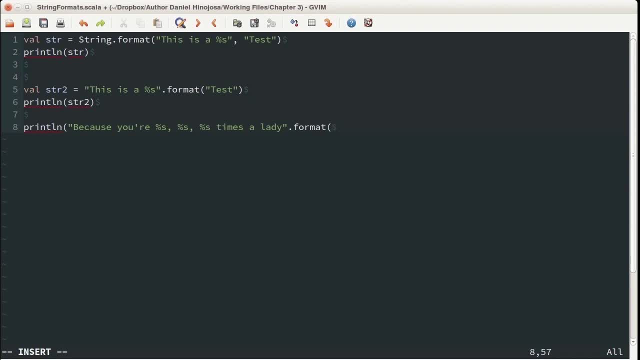 but the notion is the same, that within this format we can have as many number of parameters as we would like. so the first percent s, let's say we'll do this in reverse- three, twice and one. this is already in a print line. now compare that with the previous. 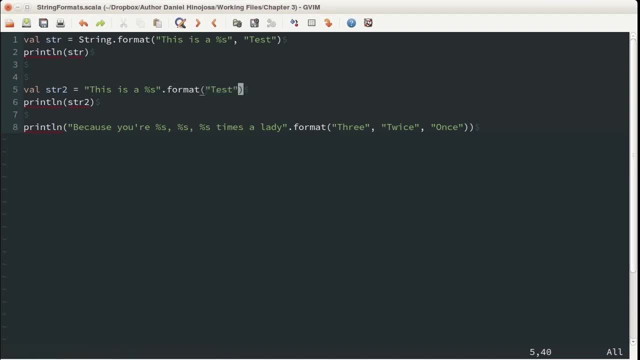 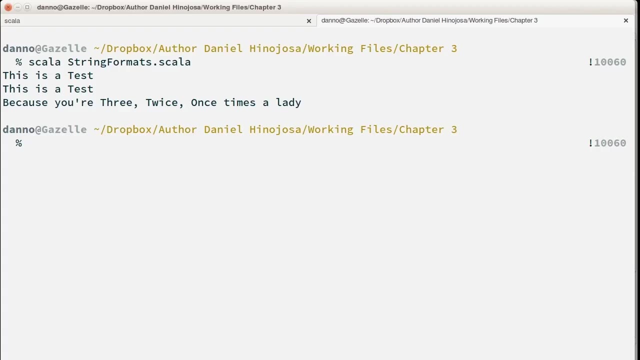 example we had where we had only one parameter. format accepts variable parameters. so if we want to use one, that's fine. if we want to use three, that's fine, if we want to use ten, that's fine. it will allow any number of parameters. let's run this. 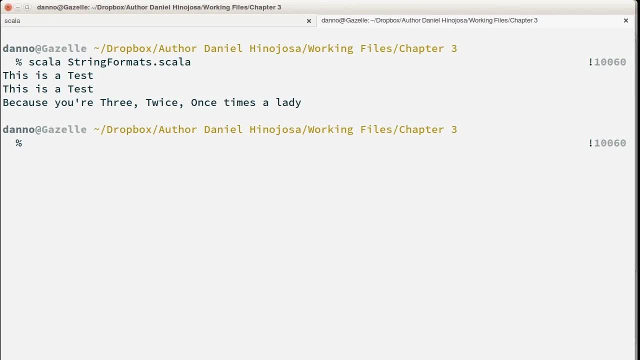 now it does it the order that it's specified. if we just leave it as percent s, it's always going to choose the first one by default for the first percent s, the second one for the second percent s and the third one for the third percent s. 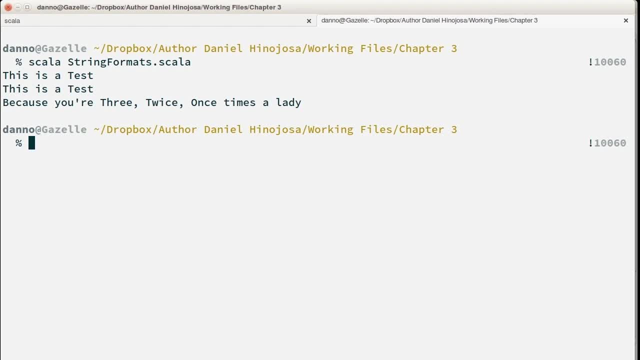 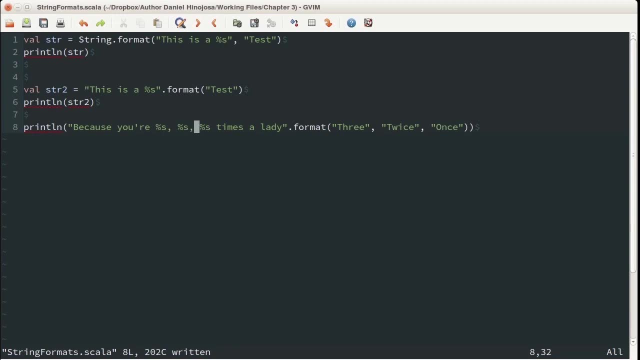 but if you cannot change the order, we can change the string format. let's give that a try. I'm going to head back over to the editor. let's say the third one needs to be the first one. so what I'm going to do is specify here, after the percent, that we want. 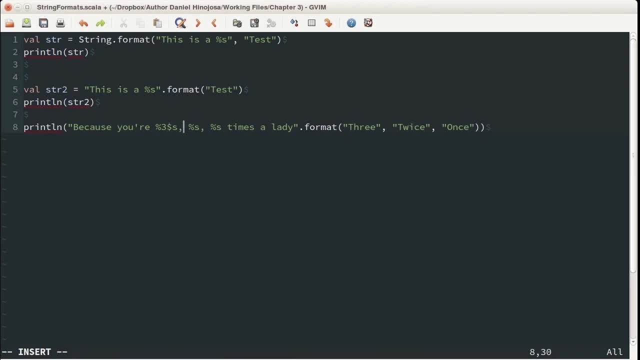 the third argument and we want to make that a string. for the second percent s, we want to make that the second argument, but we still want to maintain that as a string. and then, finally, for the third one, we want the first argument and still maintain that as a string. 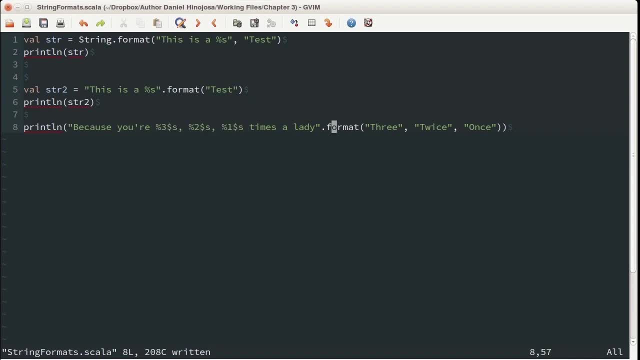 again, the percent three states that we are going to get the third argument, which happens to be once. the percent two states we want the second argument, which is twice, and finally, the percent one here represents the first argument, which is three. let's run. it works in the format that we need. 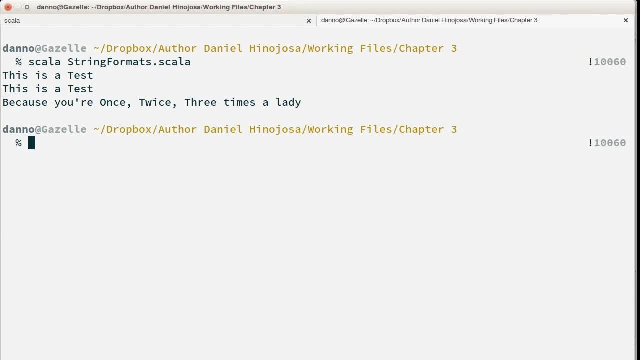 let's get a little fancier this time. I'd like to use java time. if you're not familiar with java time, it used to be called a library, called jota time. if you're using a project that is jdk7 or less, I highly recommend. 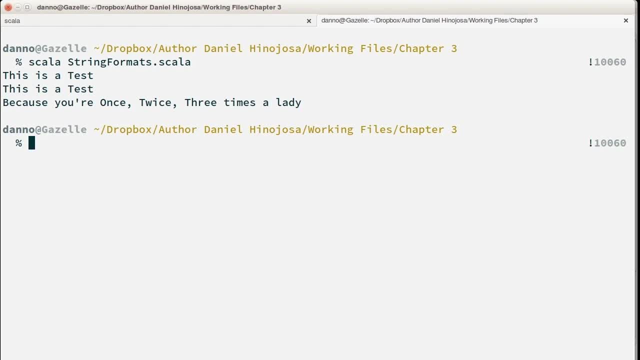 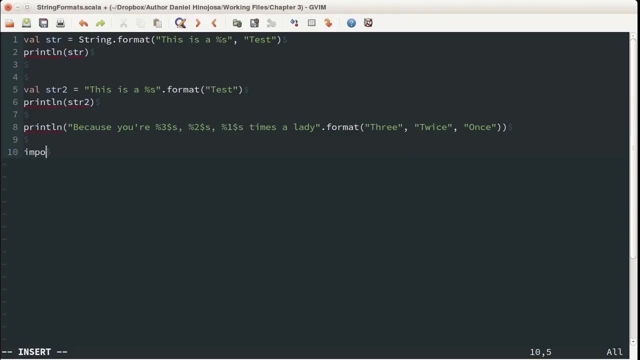 that library, the creators of jota time were brought over to oracle and they created a fantastic package that is now a part of java 8 called java time, and I'd like to use java time in our next example. let's go back to our editor, so what I'd like to do is 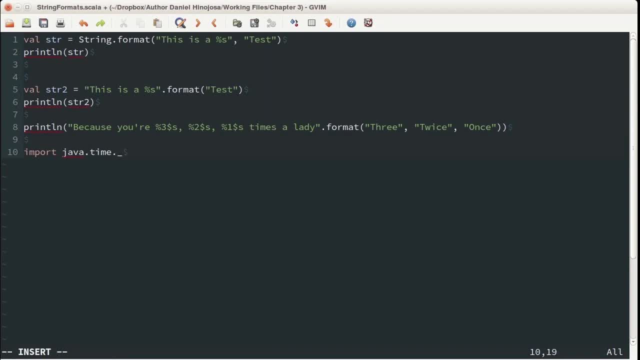 I'd like to import the package again. it's worth reemphasizing that, this java time underscore that I'm bringing in, by the way, this underscore means bring me everything within java time. but again, this is with java 8, and what's really great about this? 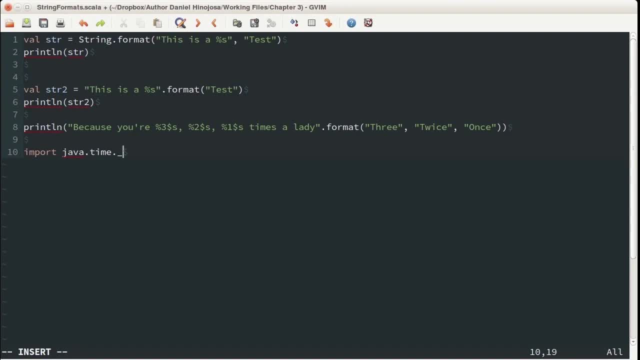 is that it is immutable, very much like everything by default is in Scala. we embrace immutability. so let's create a print line on this and say we will be eating lunch. and in our example, let's say I want to bring in one date item and it's going to be called local date. 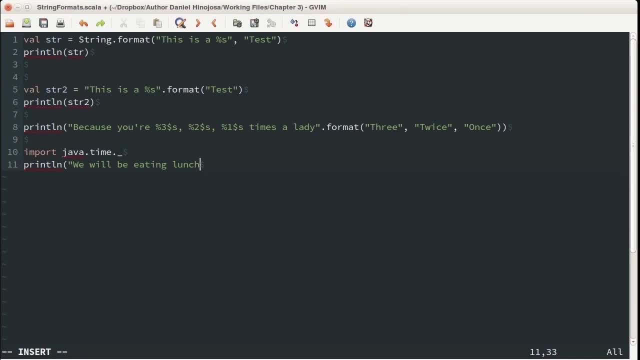 there are four different ways to create dates using the java time API. one is called local date, one is called local time, one is called local date- local time and the other one is called zoned date and time. local date is just the date, with no reference to. 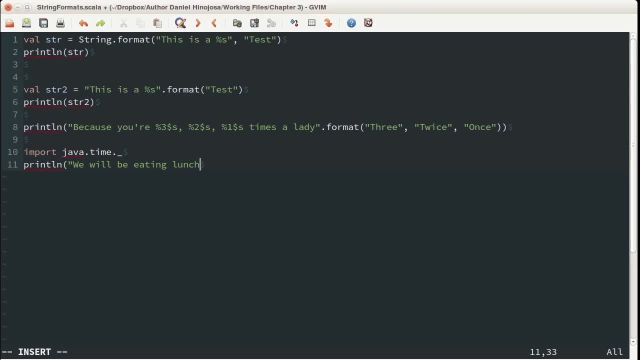 time zone. local time is the time, with no reference to a time zone or reference to a date. local date time is the date and time, but no reference to a time zone, and then zoned date and time is everything: the date, the time and the time zone. so 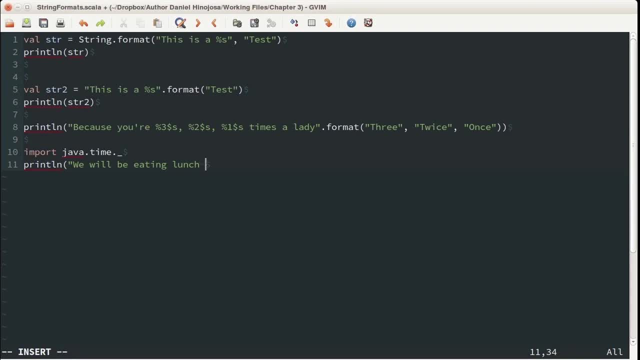 let's say, in this case, here I want to say, we will be eating lunch on and let's say, for this example, we only have one argument, but we need to use it three different times. so percent one, and we need to specify that this is a time element. 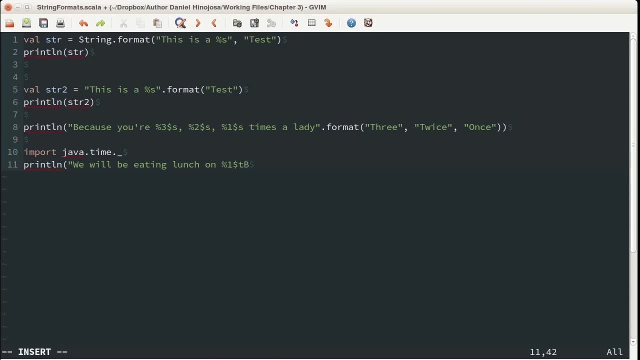 and b is going to be the month, so we will be eating lunch on month. the day will be, let's say, we want to use percent one. this is a time and if you take a look at the reference at the website, this would be the date e. 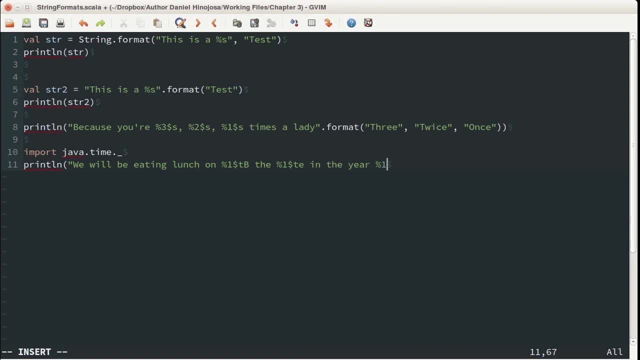 in the year, and now we want to specify the year. we still want to use the first argument: it is a time element and here is the year. so b is the month. if I said that was year, that was incorrect. this is the month. this is the day. 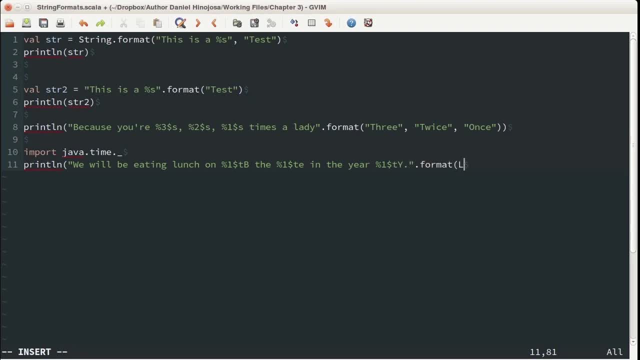 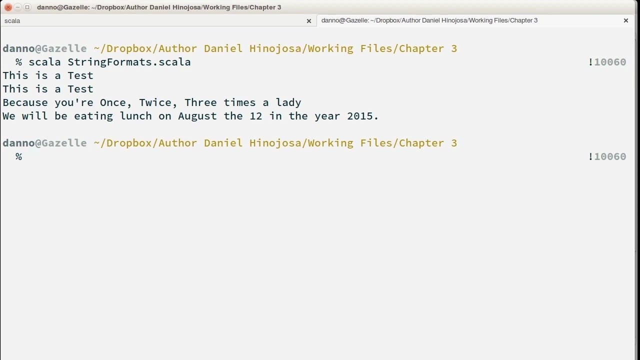 and this is the year. finally, we will format the whole thing and provide it with local date. local date now says: just give me the calendar of whatever it is on my system clock. let's run it, we will see here. it says we will be eating lunch on August the 12th. 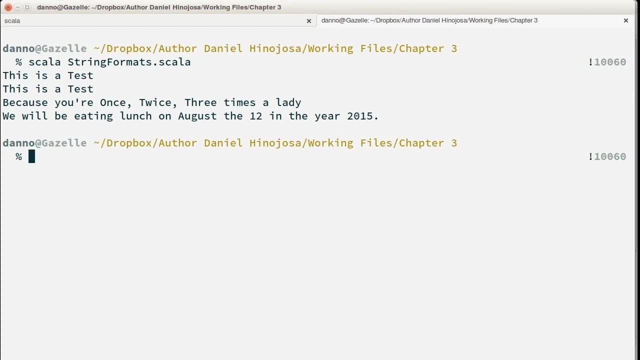 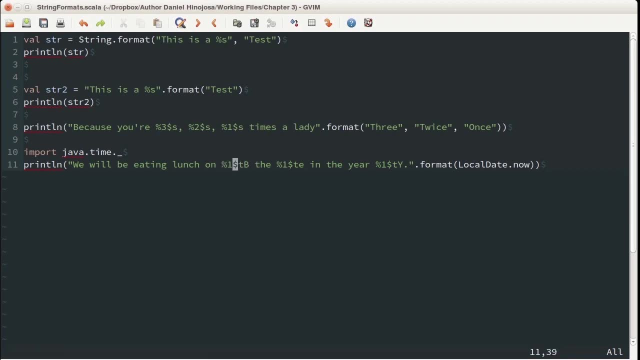 in the year 2015. this just happens to be the date this recording was made. let's go back to the code. here it is. there is only one argument. that's why we have percent one here, we have percent one here and we have a percent one. 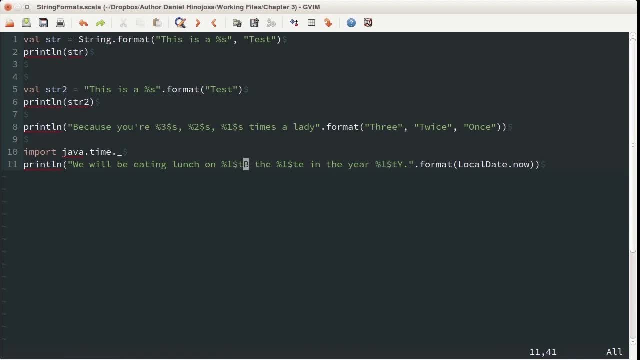 here. all of these are time formats, which is why we have a t under all of them. capital b is the month, e is the day, and capital y is the year. it is worth noting, though, that all of this could also have been rewritten using printf and instead. 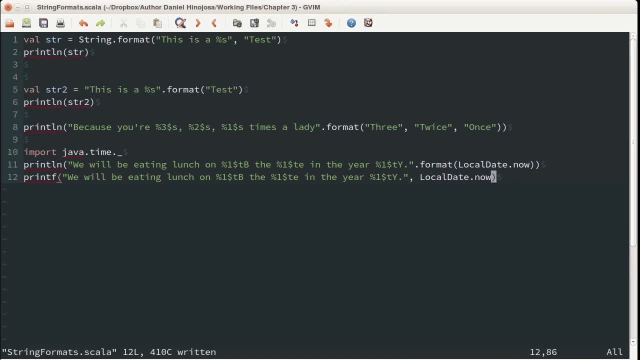 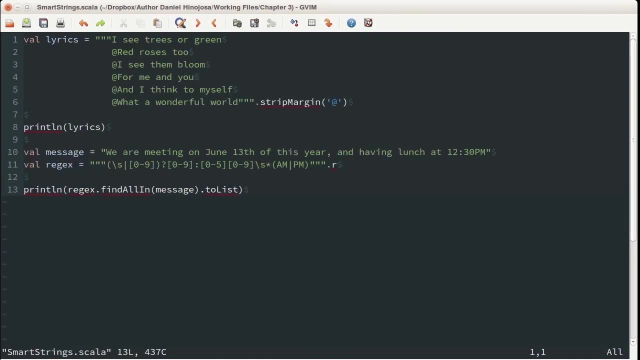 of the format. we just need to include the variable that's going to run this now as a well rounded discussion. in our previous session we talked about smart strings, so let me bring up the item we had with smart strings and we had these lyrics from Louis Armstrong: 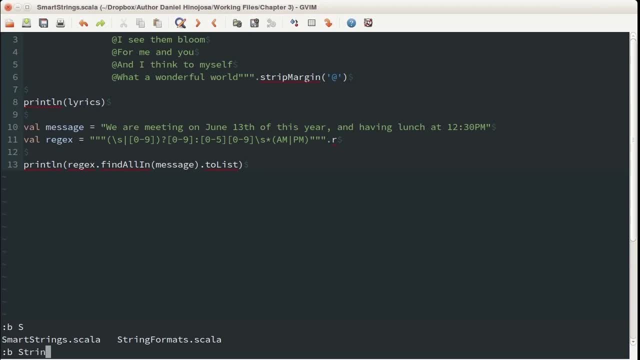 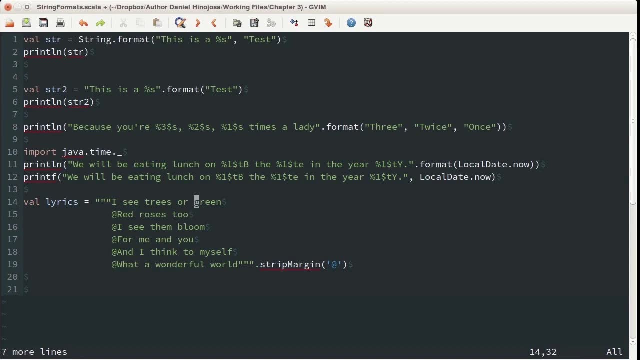 and let's go back to our current file, and what I'd like to do is bring those lyrics in here, and here they are. by the way, in the previous session I had misused this word. that should have said of, but let's say given this string. 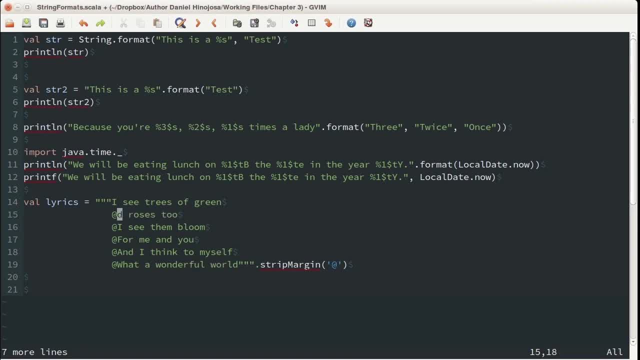 what I'd like to do is everything that is a color. I'd like to do a variable replacement of that. so I'm going to do a percent s here and, of course, for the green, which is also a color, do a percent s. so if I want to do substitution, 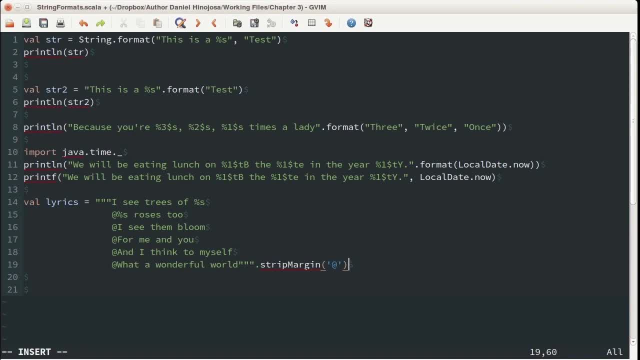 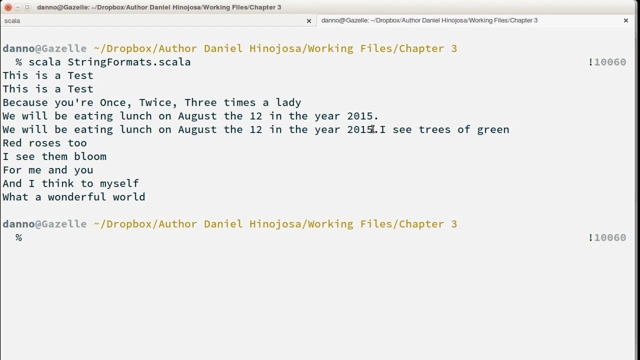 everywhere where I have a percent s. I could also do this on a smart string, so I'm going to call format with green and red. let's print out these lyrics and let's take a look at the end result. now. everything is caught up here to the top, because we needed. 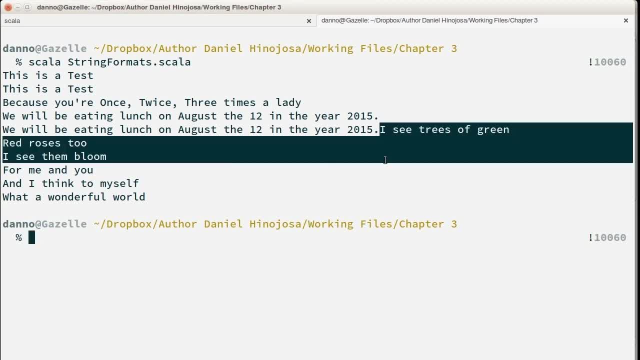 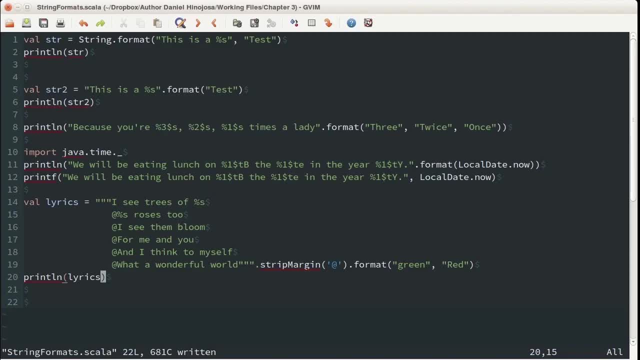 to do a new line at the end of the previous one, but we get the idea. here I see trees of green, red roses too, and so on. let's go back to our source code and do a review so we have string format. this is the java way. this is the older. 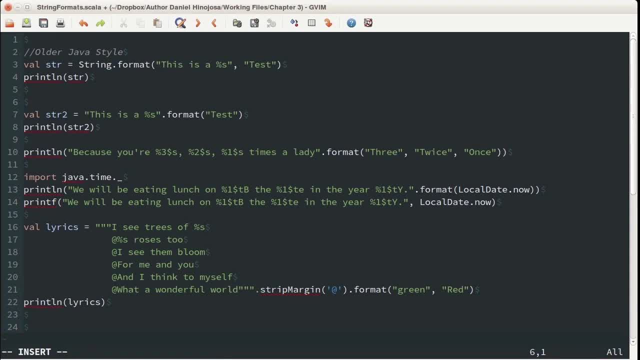 java style under the. this is a percent dot format. this is Scala's style, this format. we are using positions because your percent three would be the third argument. percent two second, percent one, the first argument. in our fourth example we used time to do formatting. we used the. 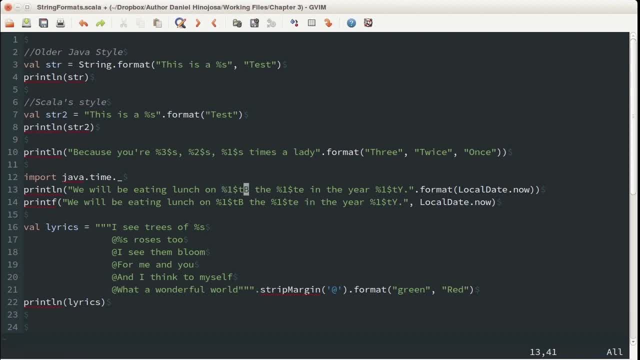 first argument over and over, because we wanted to separate the month, the day and the year. and in our final example we used a smart string from our previous session and this time we replaced all the colors with percent s. so if we want to change the colors on a whim, we can do so. 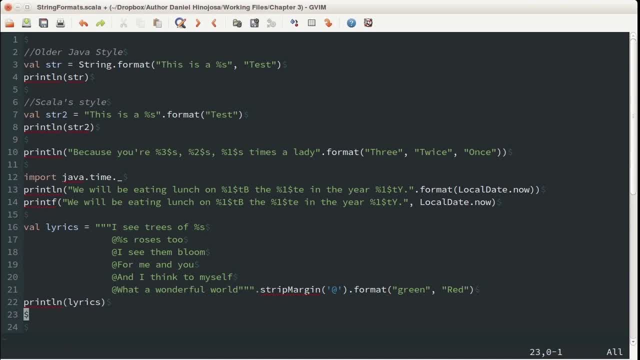 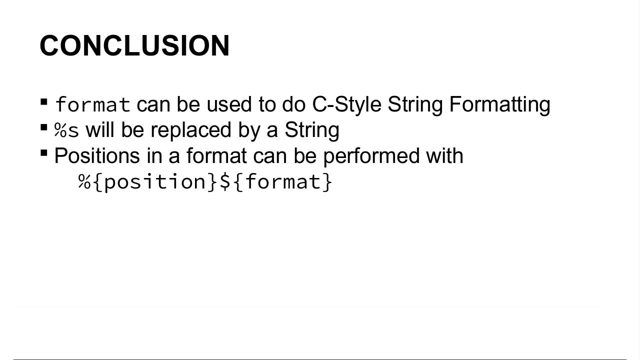 using a format method, call and finally, we printed out the lyrics. so, in conclusion, you can use the format method on any string to do any c style string formatting, or if you want to call it java style string formatting, you can do so. percent s is probably one of the more popular. 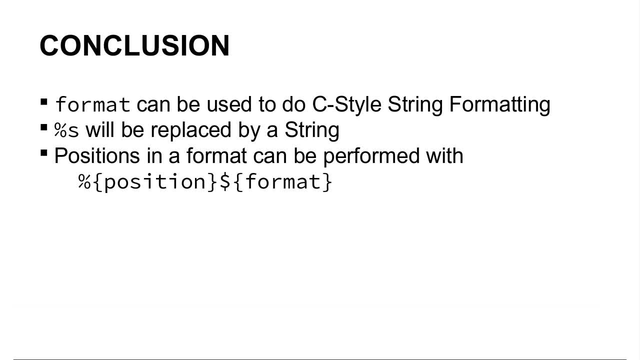 ones. percent d is probably the second one, and this will cause a replacement of the percent s using whatever repeated parameters that you use in the format method. positions in a format can be performed with percent and then you place the position dollar sign and whatever it is the format. 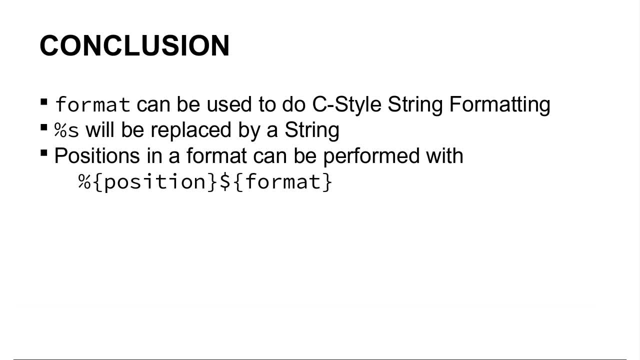 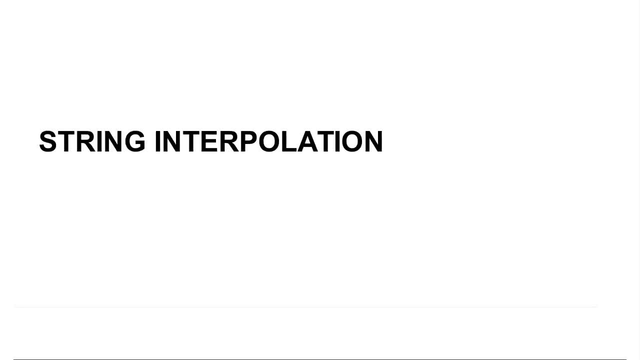 that you want. this is no different than it is in java. in this section we'll be covering the wonderful world of Scala, string interpolation, big word, basic idea. with string interpolation we can replace any word from within a context. the context could be a class, it could be an object, could be a. 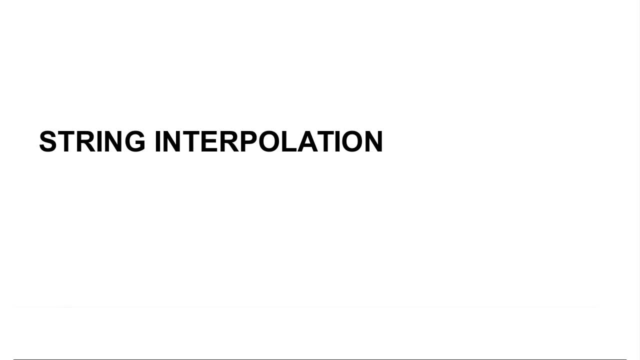 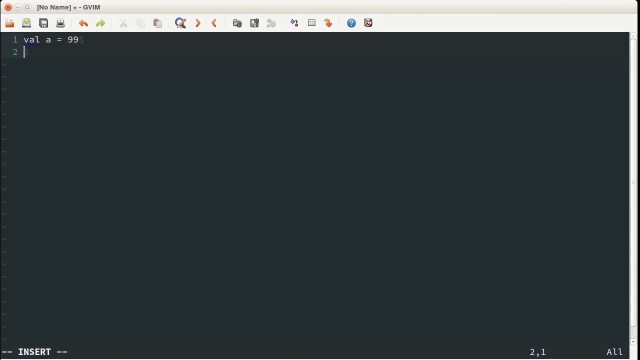 script anything that is outside of its line. so let's create a file called string interpolation, dot Scala, and try some of this string interpolation out. let's set up a vowel. a is equal to ninety nine, and some of you may be familiar with this song. this is a lyric from a song. 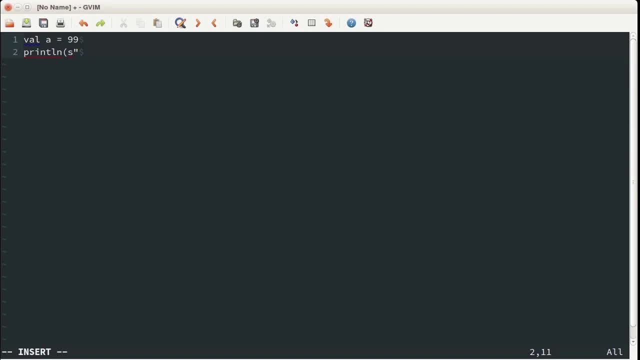 called ninety nine love balloons, and we are going to start off with the letter s. this s comes before the string and in order to use string interpolation, we require this s. now that we've established that this is going to use string interpolation, I am going to bring 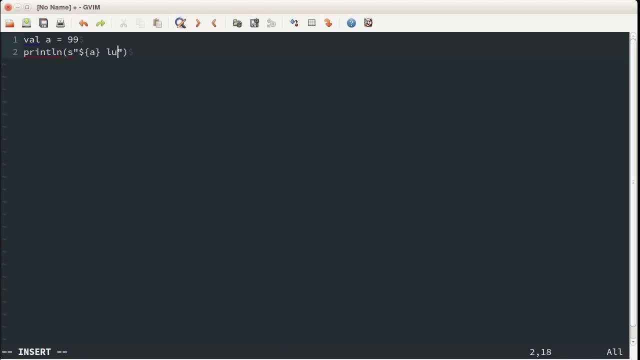 in an, a surrounded in braces, and the rest of the lyric goes: ninety, nine love balloons floating in the summer sky. this almost looks like formatting. the only difference is that we are going to use a dollar sign, we may or may not use braces, and we are going 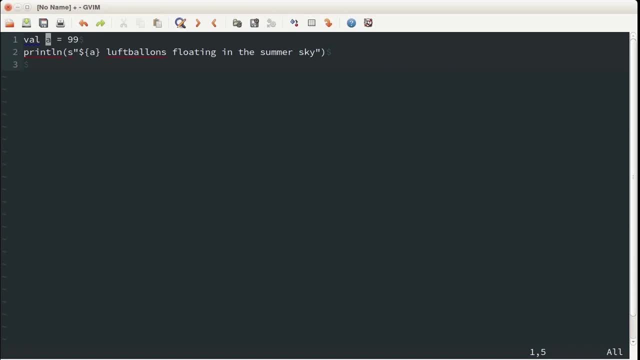 to replace a with whatever a is within the context of this line. so in the context, meaning around its general area, there is an a. we are going to take that a and it will be replaced right in here. let's save this file again. we want to call. 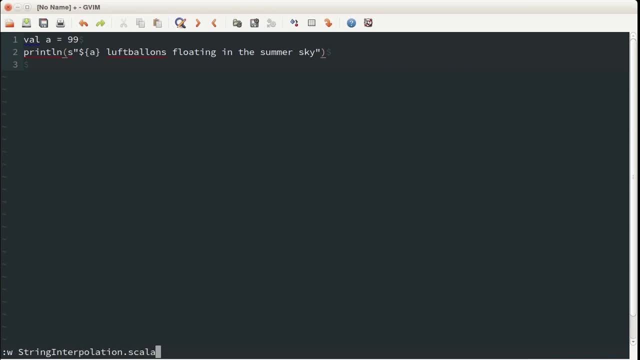 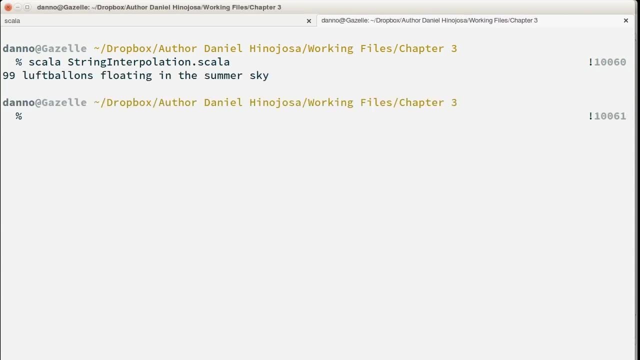 this string interpolation, dot, Scala, and let's run it as we see here. the ninety nine which was val a is equal to ninety nine, which was in the context. I am going to take that ninety nine and replace the a with that particular number, because we are only referring 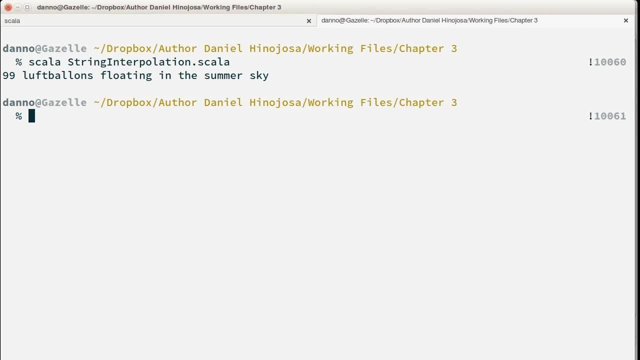 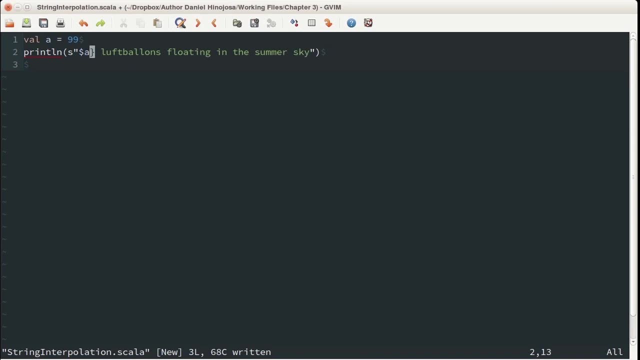 to one value. we can omit the braces. let's go back to the code and show you what I am talking about. I am only referring to a, so the braces aren't absolutely necessary. we could just simply say: dollar sign a. let's save it and run it now on the console. 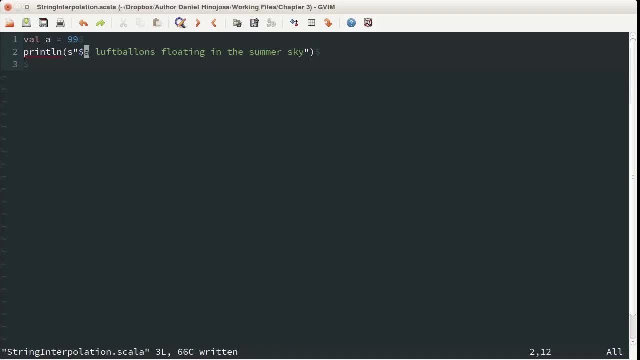 shows the same thing. let's go back to our code. be warned, though, that once you try to call any method on the interpolated object, perhaps things can go wrong. and let's say that for this particular number. let's say I want to add three, and because we are doing, 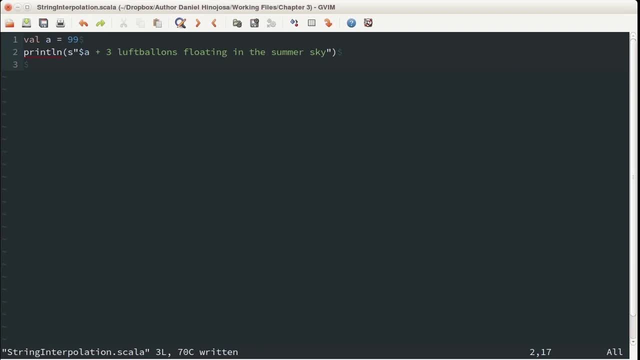 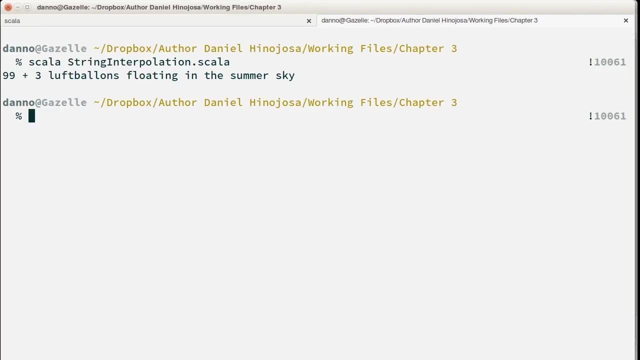 it this way, we are going to get a result we are not expecting. I went ahead and saved this. let's go over to the command line and see the results. it says here: this is ninety nine plus three, but what I really wanted to do is I wanted to add the 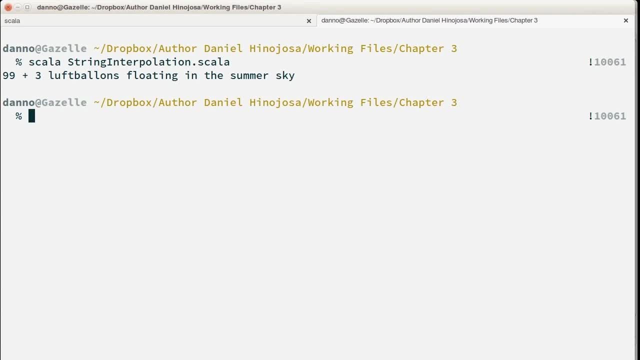 three to the ninety nine. so that did not work. so let's go back to our code and put braces around there, save it, and let's go to the command line and run it and finally we will have one hundred and two love balloons floating in the summer sky. 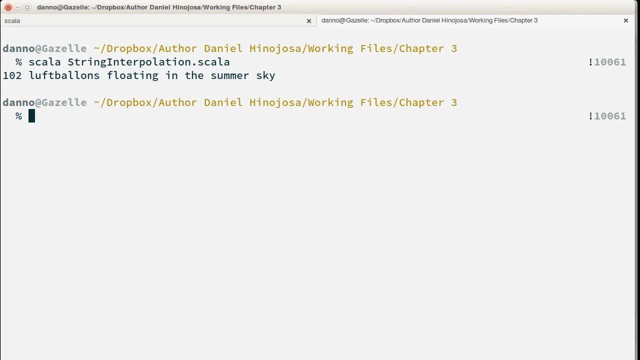 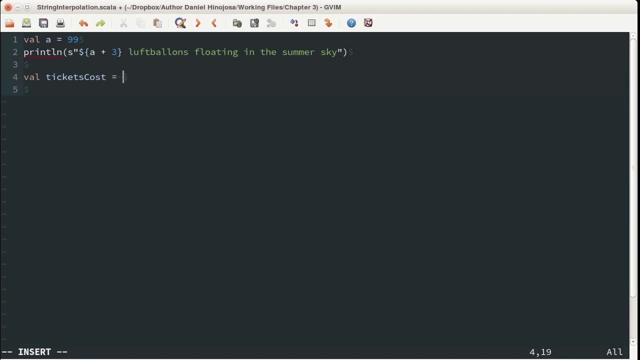 there is also a way to format a string using the string format rules that we did in our previous section and interpolate that in one fell motion using what's called the F interpolator. so let's go back to our code. in this example, I'd like to set: 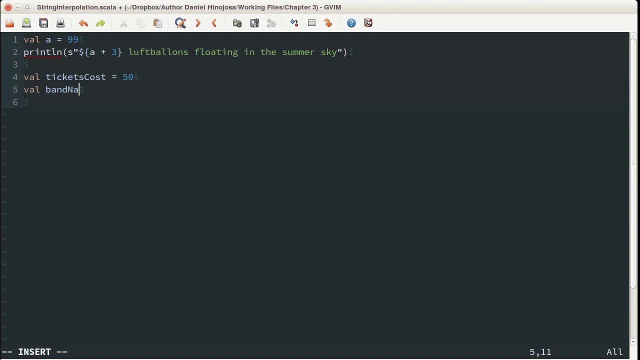 up a value called ticket cost. this will be an int. I'd like to set up a band name. bring in an eighties band and I would like to do an interpolation. so I'd like to print line F. now, this is going to be a little bit. 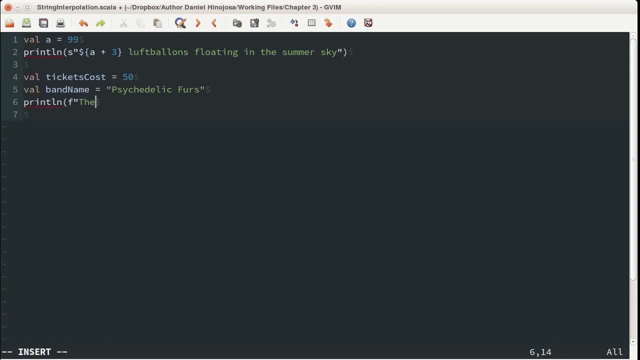 different. take a look here. I am starting with an F, I am not starting with an S- the band name- and I want to interpolate this as a string. I can use different formats with the F interpolator. tickets are probably, and for a dollar sign now a dollar. 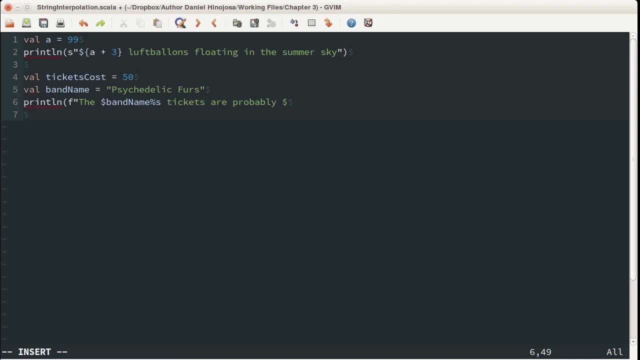 sign is going to be tricky, because a dollar sign is the character that escapes for string interpolation. so in order to create a dollar sign, I need to put two dollar signs in order to create that. then next, I want to bring in the ticket cost, but I want to format. 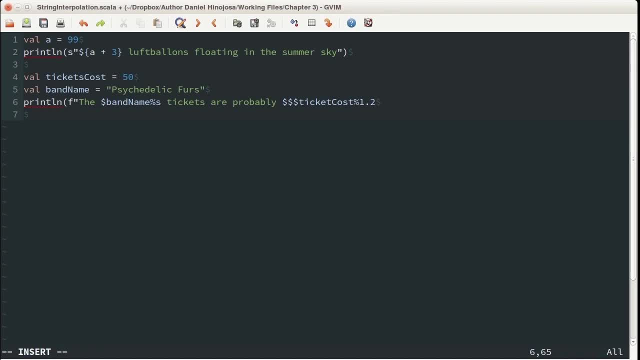 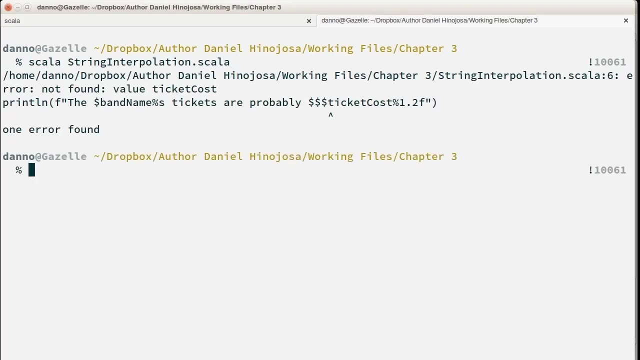 this as a float. so let's say one digit, dot two for the decimal point and as a floating number. this is the F interpolator to do formatting. let's save it and let's run it to see the results. I have an exception here. ticket cost is 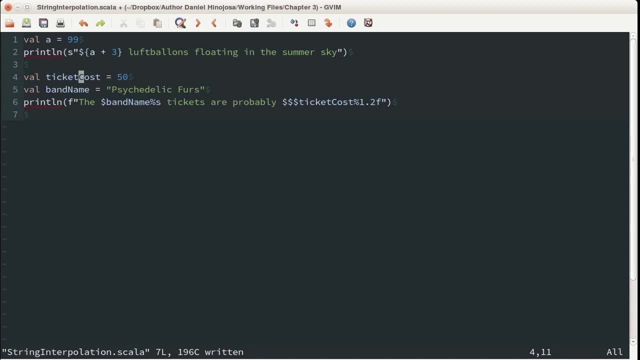 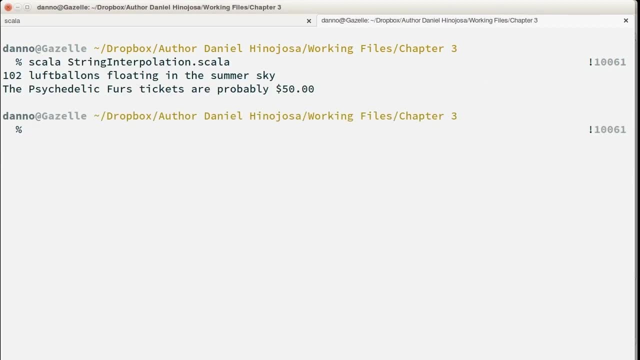 not found likely because I called it tickets cost. let's save it. fix the issue, run it again. so with the F interpolator, we were able to bring in the string and we were able to bring in the number value and we formatted it using the F interpolator. 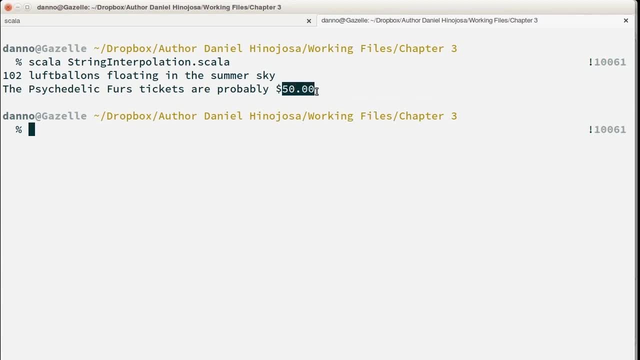 and using this format. so we wanted to interpolate fifty, which, if you recall, was an integer, but we wish to format that using a decimal point, so using one dot two F, the one dot two F created for us this fifty dot zero zero. let's go back to our code and review. 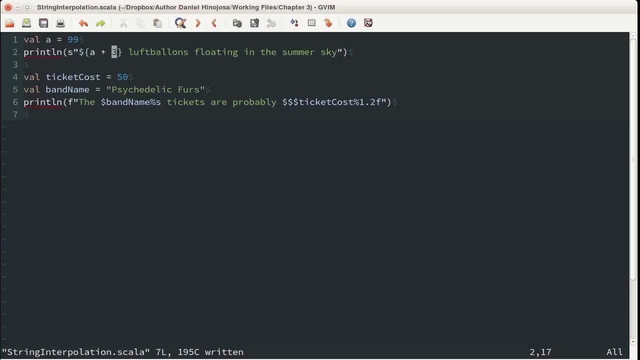 and these are two different interpolators. one is just an S interpolator, where we get the A and we do something with it. the F interpolator: we can still get information from within the context, but what's different about this is that we can format it according. 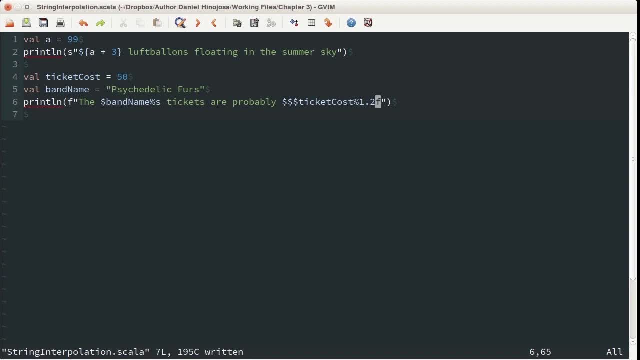 to the formatting rules of string format. now let's change things up a bit. let's say we have the ticket cost, we have the band name and what I'd like to do is let's do a percent, change things up a bit and I'm going to have a percent increase. 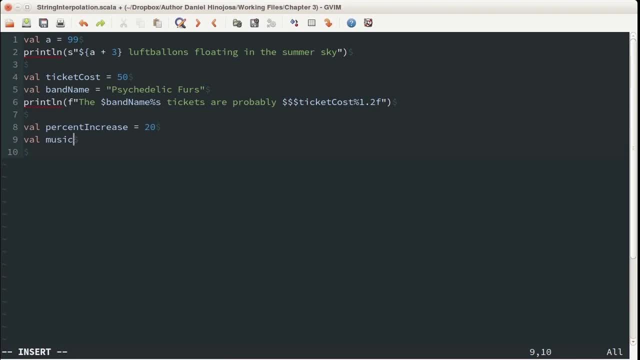 let's say a percent increase of twenty. and as the music genre, let's say that this would be new wave. I'm going to bring that print line down here, but I'm going to change things a bit. let's say we want to say the band names. tickets are probably. 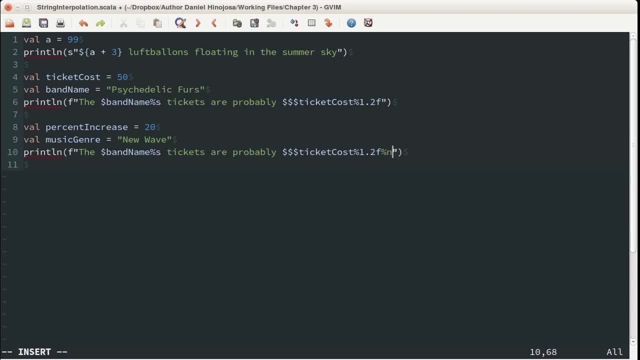 this cost and after this, let's create a new line and I'm going to say that's A. let's bring in our percent increase. here I need to do two percents in order to create one percent name, just because percent is used for formatting. so two of them is going to be the. 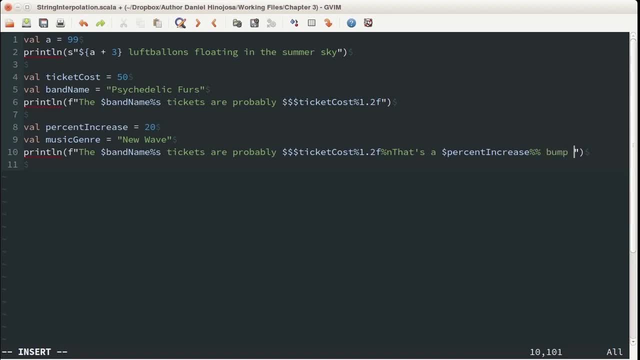 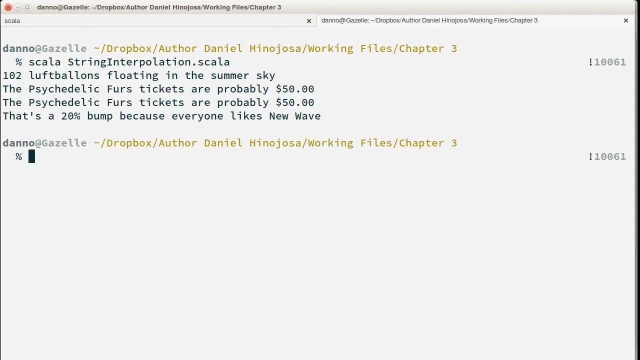 escape to create the percent, and I'll just say this is a bump because everyone likes this particular music genre. it's a fairly large format we have here. let's save this and run it and let's see the result. so we have our new line. we use percent to end for our new line. 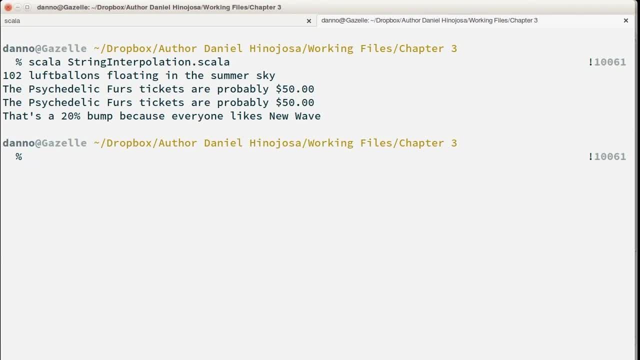 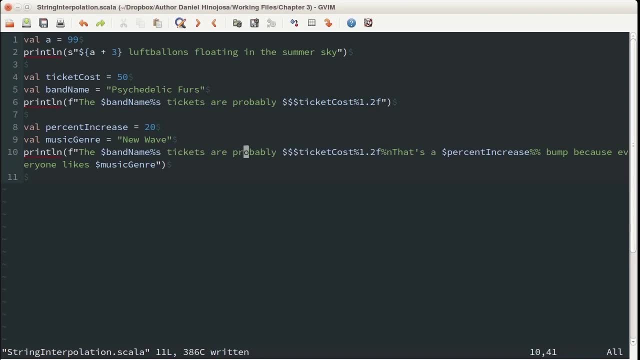 it states here: the psychedelic furs tickets are probably fifty dollars. that's a twenty percent bump, because everyone likes new wave. now let's say we didn't want to do the new line. let's say that we wanted to separate this up a bit. in fact, let me go ahead. 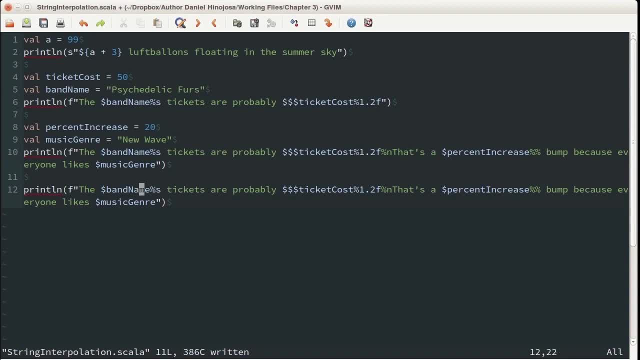 and bring this down and show you how to do this with a smart string. so this will be an f interpolator using the f interpolator, using a smart string. now, whether we're using an s interpolator or we're using an f interpolator, we can use a smart. 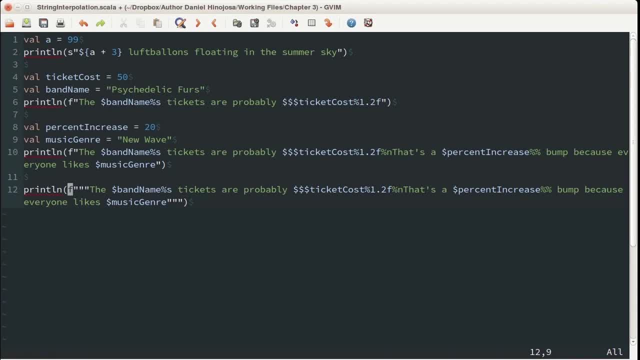 string with those interpolators. so I'm going to use the f interpolator using a smart string, and in our case here, I don't want to do this percent n, I would just rather use a smart string to format it. let's put a pipe there and: 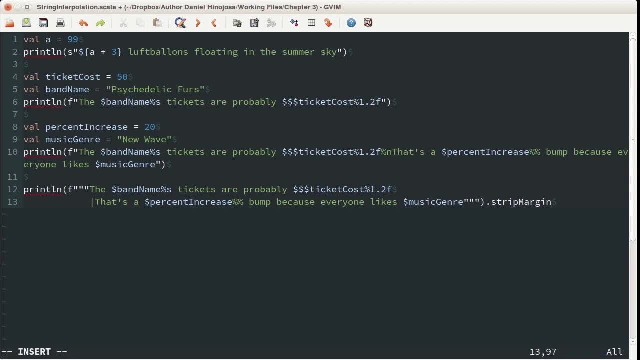 finally call strip margin, and this says that's a percent increase bump, because everyone likes a certain music genre. we'll need one paren here, we'll need the strip margin to apply to that smart string, and there we go, let's run this so again. what's different about this one is: 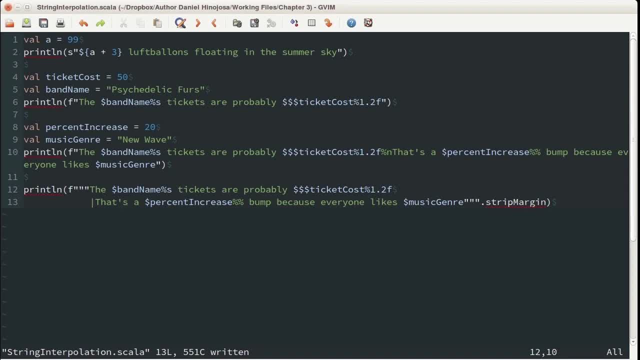 instead of using that percent n, I wish to use a smart string. I am preceding all of this with the letter f, causing this to be an f interpolator, and everything will be replaced by what is in the context. band name is from the context. ticket cost is from the context. 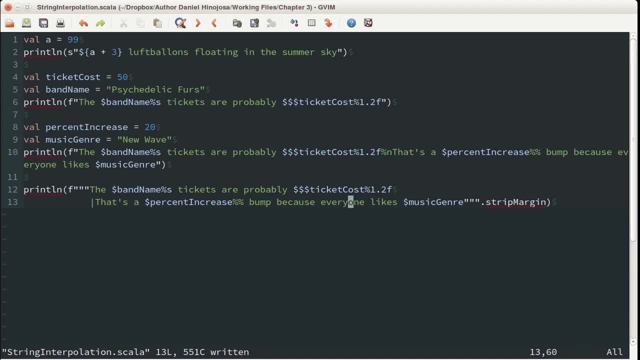 percent increases, and so is music genre. it's a little cleaner, and this just goes to show you. we have a lot of tools at our disposal to display output. let's save it and run it. let's go back to our code and review. we have multiple ways. 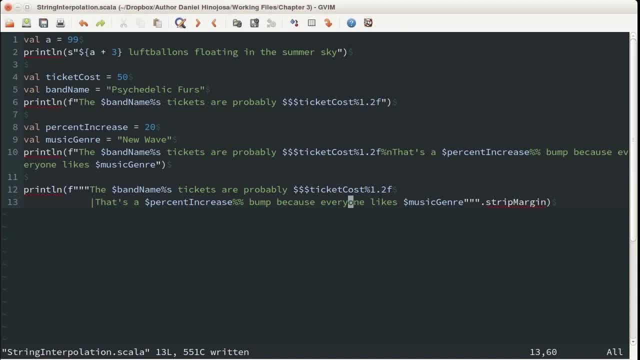 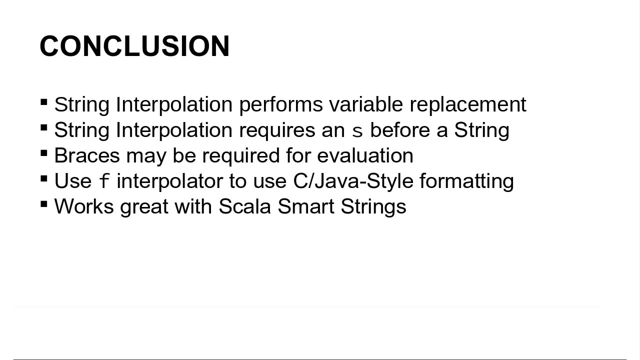 to run the string interpolator. one is the s interpolator that just brings values in from the context. f interpolator brings values in from the context and we can format it along the way. we can also apply this using a smart string. so, in conclusion, string interpolation performs variable. 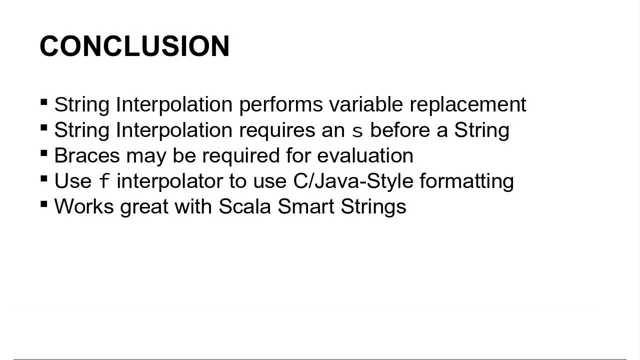 replacement within a string. all that is required is an s or an f before a string. braces may be required to surround an evaluation. we saw that with our a plus three example. you can use f interpolators in conjunction with the classic c style or java style string formatting. 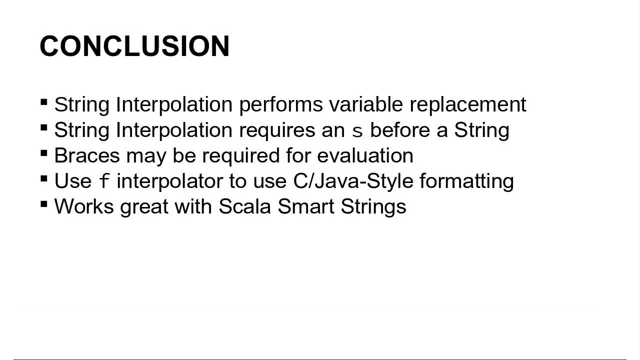 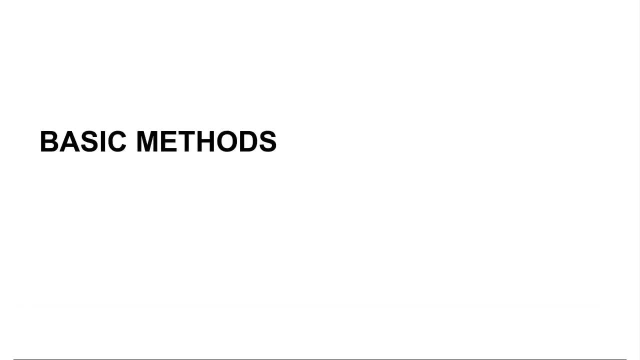 and string interpolation also works great with Scala smart strings. in this section we'll be covering basic methods. in java, there is a differentiation between methods and functions. in this session we're only going to be talking about methods. methods belong to a context and in an object oriented programming language, 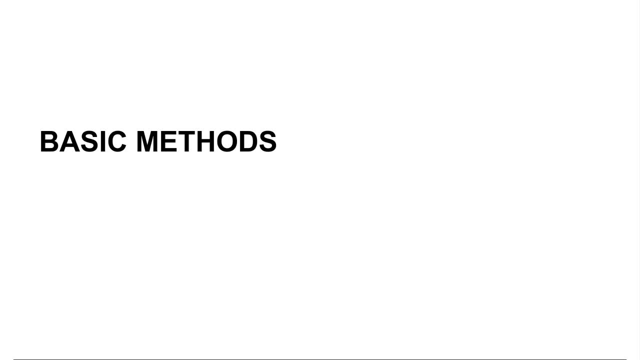 like java, that context is a class. there are different contexts. actually. in Scala a class an object, a script or another method. in Scala, a method starts out with a keyword called def. a method will always start with def. in our example, we're going to create a file called 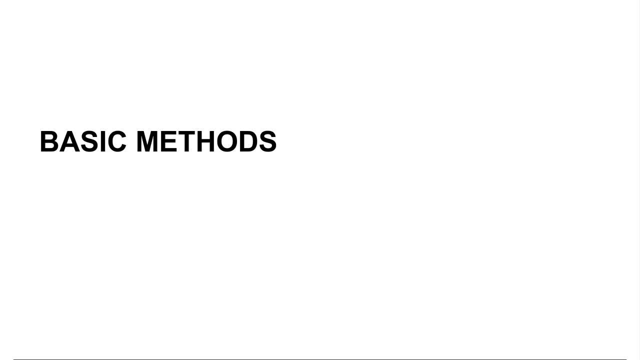 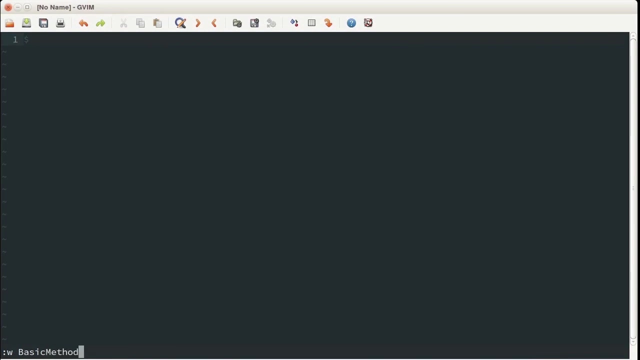 basic methods, dot Scala and we'll be creating a method called add that will add two integers together. what we're going to start off with is we're going to do this in the most inefficient way possible. let's get started this method. we are going to create a file called basic methods. 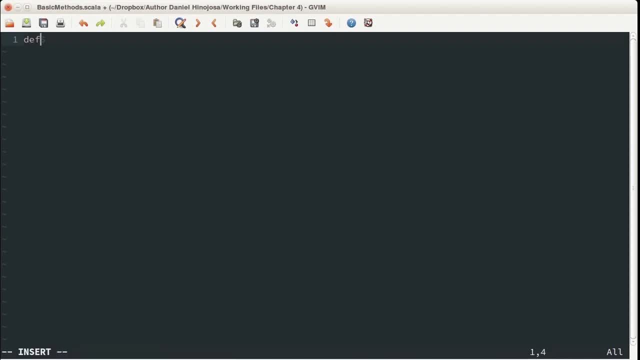 Scala. and here we are, and we're going to start off with the keyword def. again, def is the thing that starts off every method. we're going to give our method a name called add and now we're going to add it with some parameters. so how do we do parameters in a method? 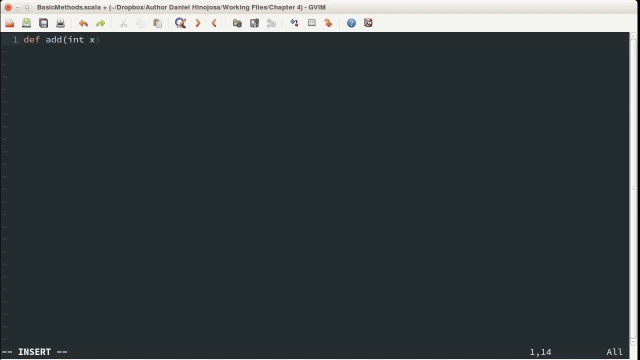 well, if you're coming in from java or perhaps some other language, you're probably used to something like this, where you specify the type, space and the parameter name. in Scala, we're actually going to do the reverse. we're going to do x, the type comma, a new parameter. 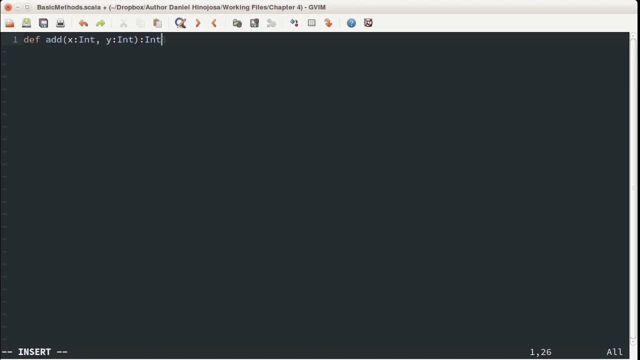 name and the type. what comes afterward is the return type, and in this case the return type is int. if you're coming in from java, you're going to expect that the return type come over here, but that's not the case in Scala. in Scala, the return 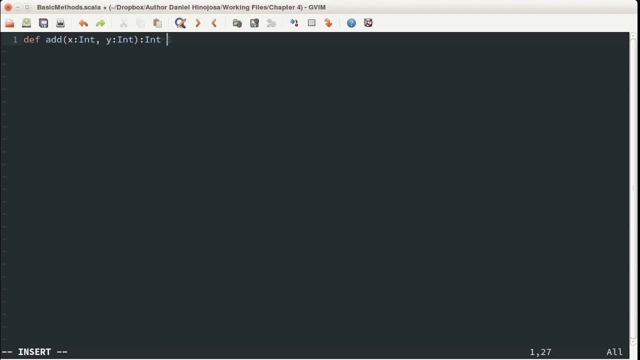 type comes at the end. now as a warning. this is the most important part of a method and it is the equals. that means that we are stating that this method is going to return something. now let's go ahead and add a brace and we'll give it a return. 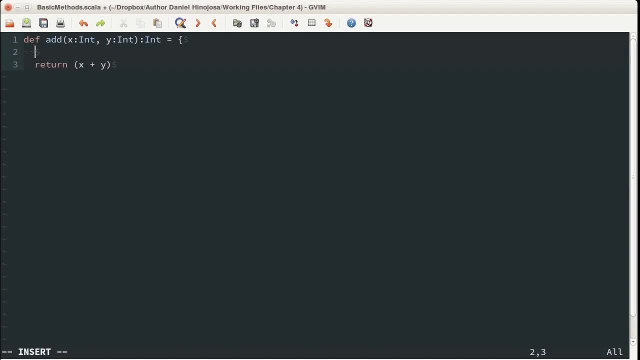 x plus y. everything that happens within here is the body of the method. the slash. slash is the way we do comments and finally we're going to close the brace. next we'll go ahead and print line and let's see what happens when we add six and seven together. 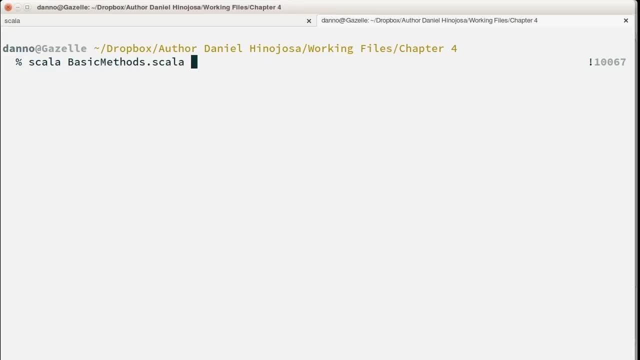 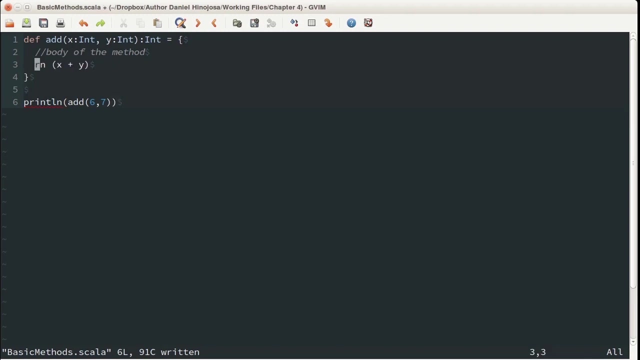 save the file. now let's go over to the terminal and let's see how this looks. looks like we're on the right track. now let's go back to the source code and get rid of some unnecessary items. first off, the keyword return is actually unnecessary. Scala programmers- hardly ever. 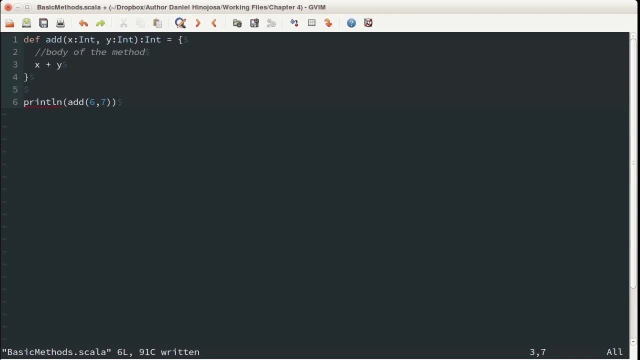 use it. we could also get rid of these parentheses. they're not required anymore. there is really only one line in this method, so we could bring that up to the top. let's get rid of this comment. these braces are unnecessary and the return type can also be inferred. 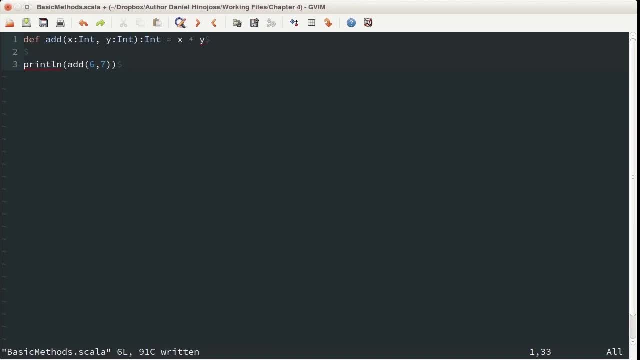 since x is an int and a y is an int and the operation of adding the two together will also return to an int, the type inferencer during compilation will already know that the return type is an int. therefore, the return type here is absolutely unnecessary. be careful. 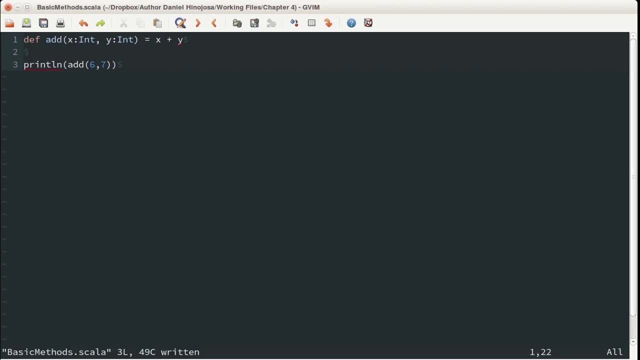 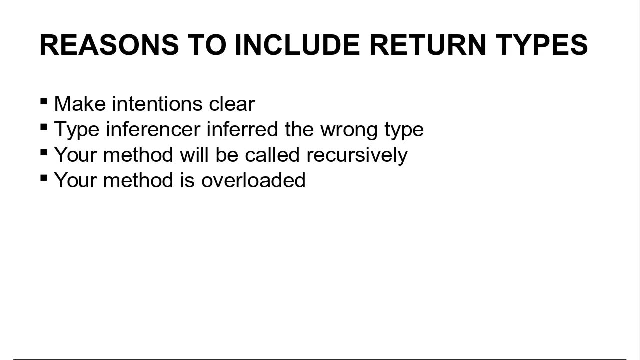 though there are times where we will actually need a return type, and those required times are the following. here's a slide called reasons to include return types. one is: perhaps you want to make your intentions clear. two, perhaps the type inferencer will assume the wrong type and it will be up to you to. 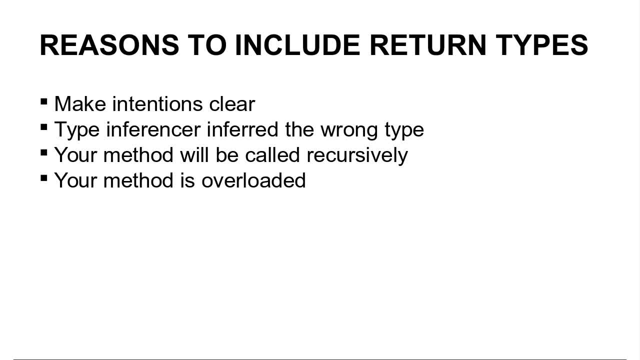 settle on a type. the method is being called recursively and, finally, your method might be overloaded and a return type is required so as to distinguish this method from other methods with the same name. now, since none of these reasons are applicable to our method, let's get rid of the return type. 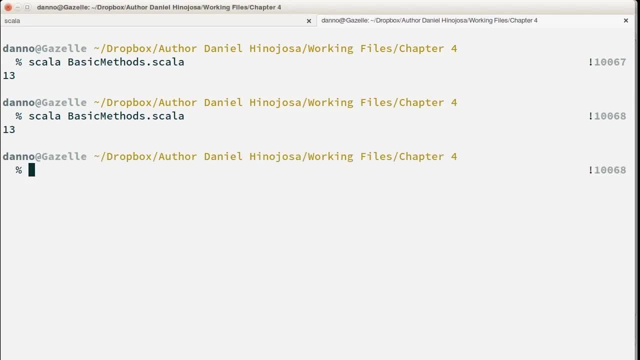 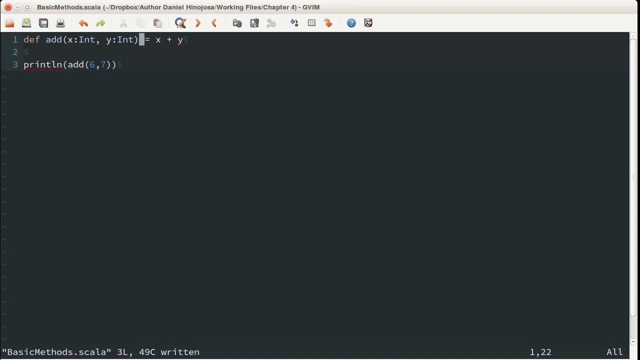 let's save it and do a sanity check. fantastic. let's go back to the source code. now. let's add a little complication to a method. let's bring in an if statement from a few sections back and make that into a method again. I'm going to start off with def. 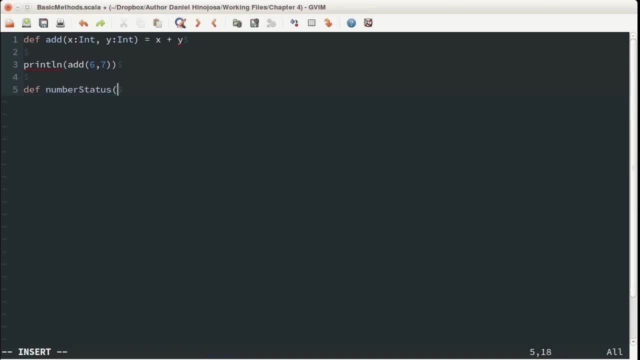 this is a different method and I'm going to call this one number status. it has one parameter called n. so if I type int- and again the important part- I need an equals. let's do a brace first and do an if statement if a was less than. 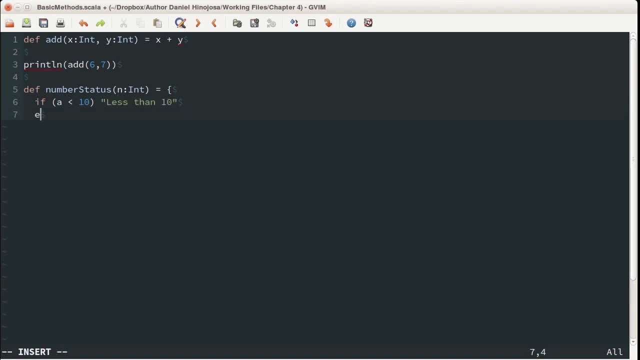 10, then we returned less than 10. else, if a is greater than 10, then we have greater than 10, otherwise it is 10. we had something similar to this a while ago, and I'm going to finish off with a brace now. we didn't. 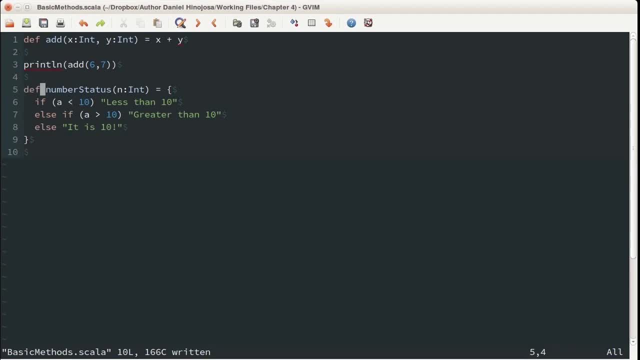 specify a return type and in fact, we don't even need these braces. remember the if statement? we could just treat it as one single statement, but in this case we have an if statement and the last evaluated statement, as I mentioned before, will determine the return type. this isn't a trick question. 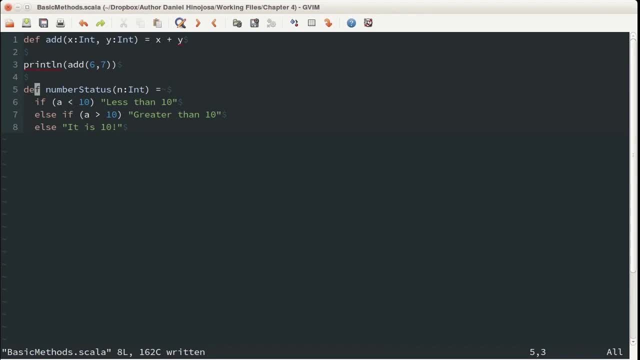 the return type will be a string in three different branches. as you see, here we have an if, an else if and an else. these are three different branches and in each branch we are returning a string. therefore, this method will take a int type and return a string. 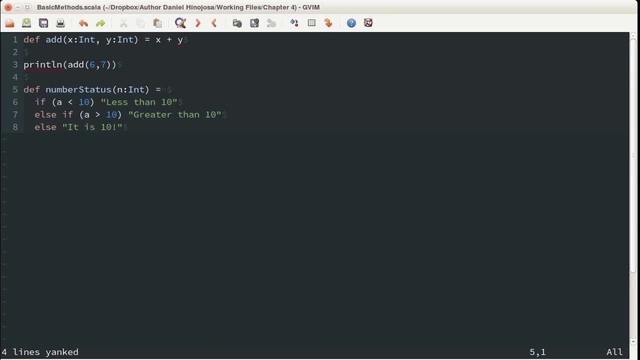 in fact, if we copy this code and bring it over to a repl. what I like about the repl: it always shows what the compiler is doing and what it's looking at. let me show you an example. so I'm going to copy this code and I'm going to bring it over to the repl. 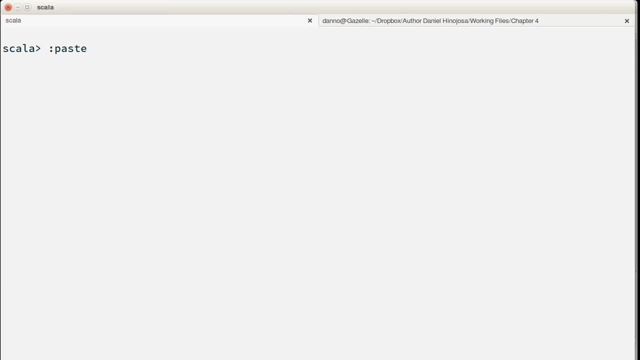 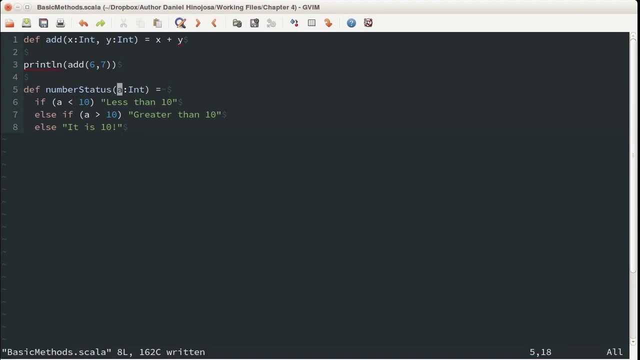 I'm going to call paste in the repl. this is paste mode and I'm going to bring the code in here. here's the number status as stated. I'm going to hit control D to finish. ah, I called it A instead of N. let me go ahead and just change that to A. 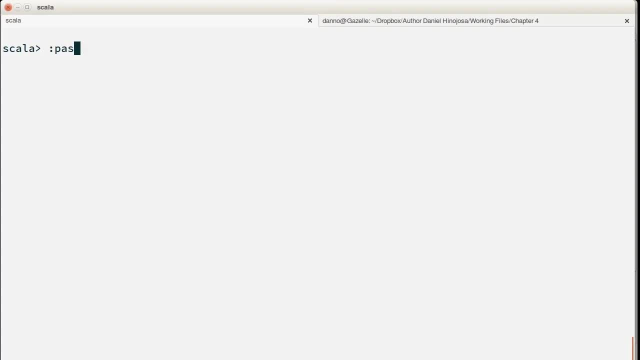 embrace our errors, recopy this and do it again. okay, as you can see here, we have a number status, we're bringing in an int and we are returning a string, even though I didn't explicitly declare it, as you can see here, since there are three branches and all of those last, 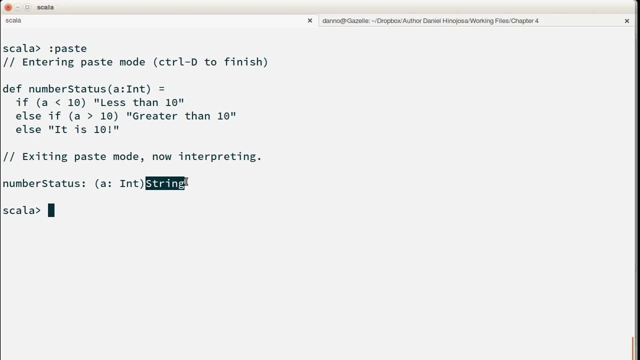 evaluated statement under each one of these branches will return a string. therefore, the type inferencer is going to go ahead and strongly assume that this return type is going to be a string. let's go back to our code and let's see what we've done. so we create a method called 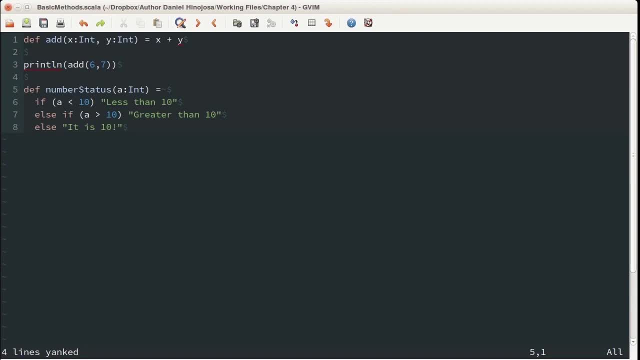 add takes two ints. we have the equal. we need the equal because this specifies that we are returning something and we're adding x and y together. the next thing: we have a number status, where we bring in an int, and we have three branches: an if, an else if. 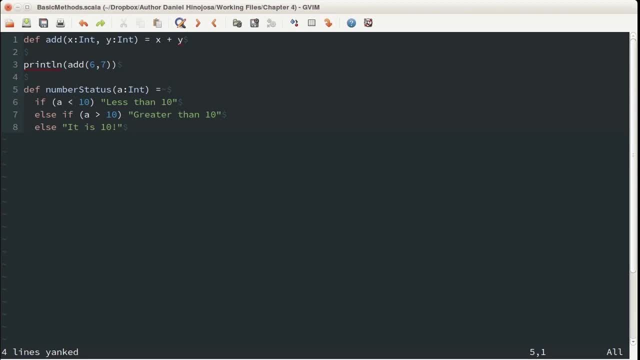 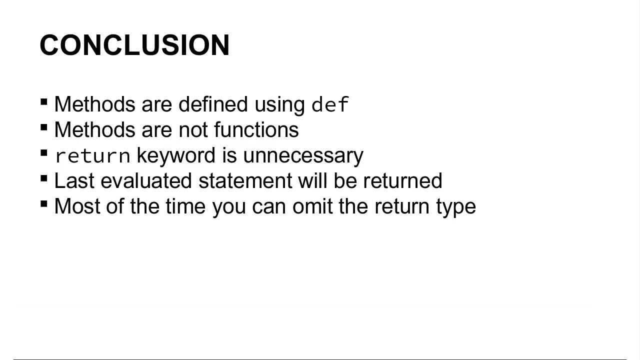 and an else at the end of these branches. each branch, the return type is a string. therefore, the return type for the entire method is a string. so, in conclusion, methods are defined using a def and they're always defined using a def. methods are not to be confused with functions. 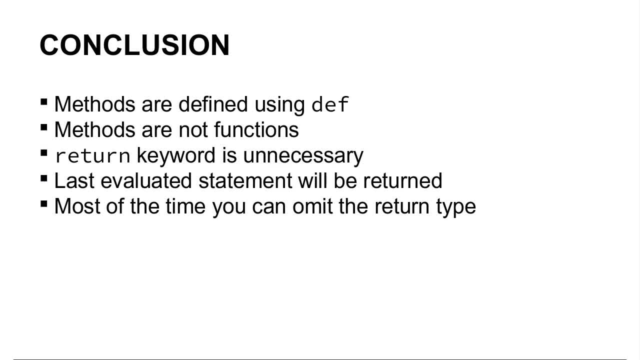 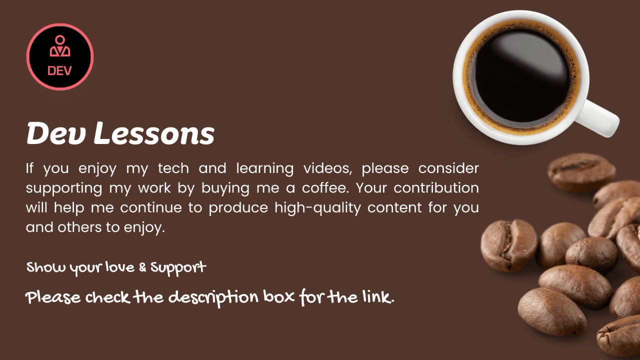 the return keyword is unnecessary because the last evaluated statement will be returned most of the time. you could omit the return type in methods unless you needed for clarity to override the type inferencer, whether you're using recursion or whether you're doing method overloading. in this section we need to. 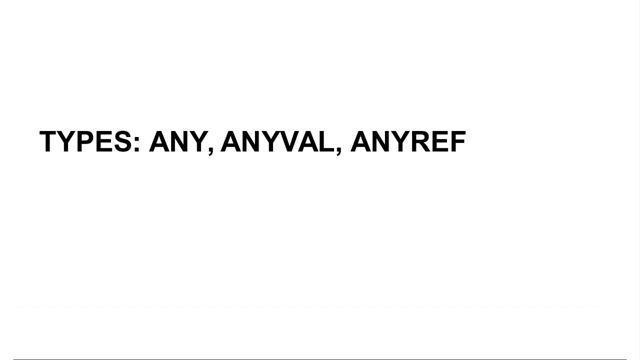 understand a little bit of types before we can discuss more about methods and return types. a type is a class, trait, primitive or an object. in Scala, a class- for those who don't know- is a code, template or blueprint that describes what the objects created from those blueprints will. 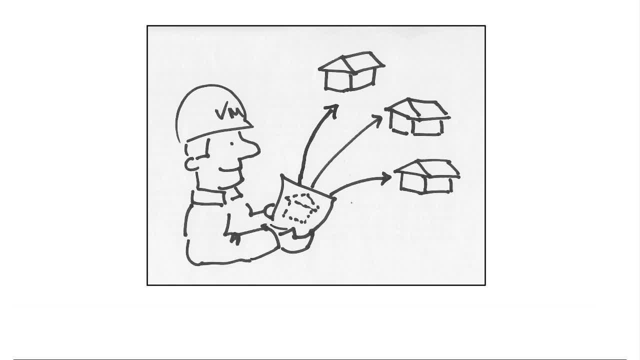 look like. here's an image of an architect. this architect is the virtual machine, and what the virtual machine will do is it will class load a template or a blueprint from either the file system or the network. the whole process is called class loading. once the class is loaded onto. 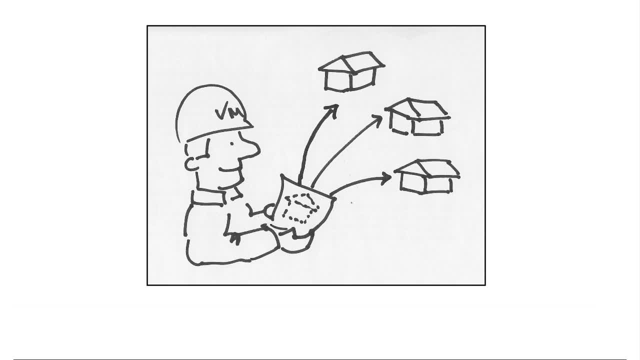 the JVM. given that blueprint or class, the VM can create multiple objects from that particular template. that template is a type. therefore, what else is a type? an int is a type. string is a type if we create a class called car. car would be a type if we 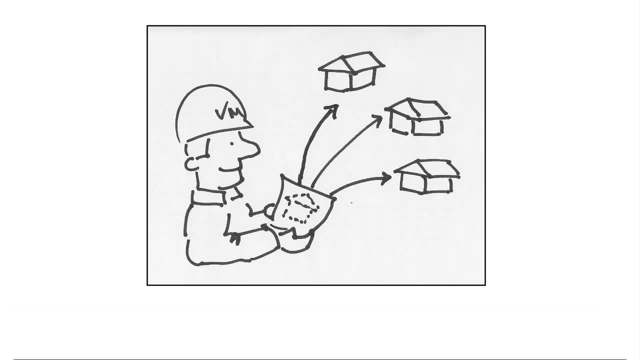 create a class called invoice json serializer, then invoice json serializer would be a type list set, a map serializable interface. those are all types. Scala is a static type language and all types need to be known at compile time and all types are under the control of what is called the type system. as 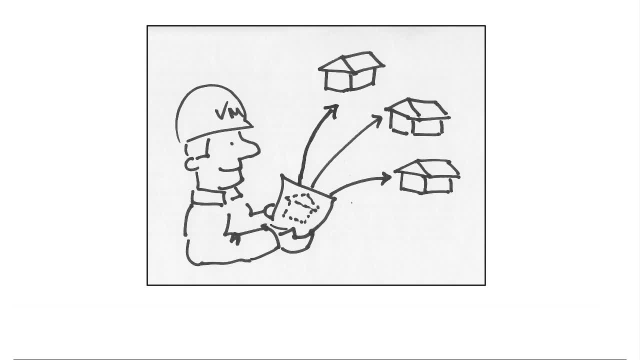 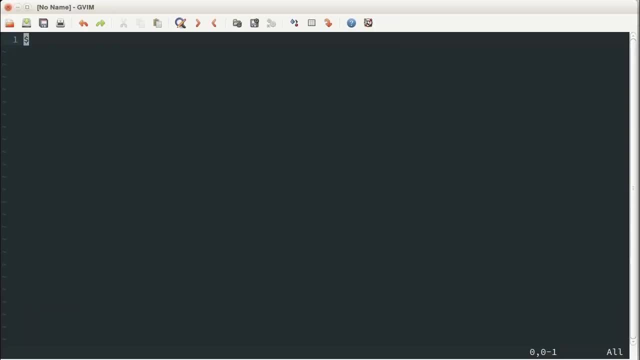 a Scala programmer, it is up to you to make sure that all the types match. very much like a puzzle. let's do some code. I'm going to head over to the editor in this file. I'm going to create a method called add which will take in. 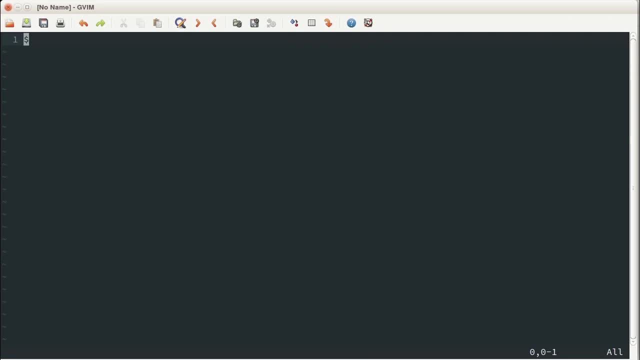 two ints and return an int and obviously it's going to take those ints and add them. I'm going to create another method called subtract, which brings in two ints and returns an int, and I'm going to use these methods together and I'm going to match the types. 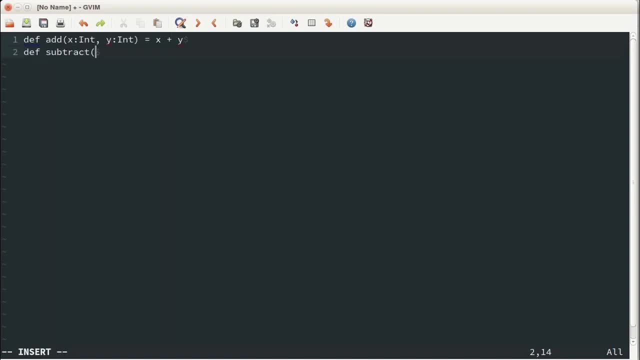 I'm going to do this all in a file called typesscala. okay, so again, here we subtract. the subtract returns an int. therefore add requires two ints. so we know that add requires two ints. subtract is going to return int. therefore, the type system got us is pleased with our design. 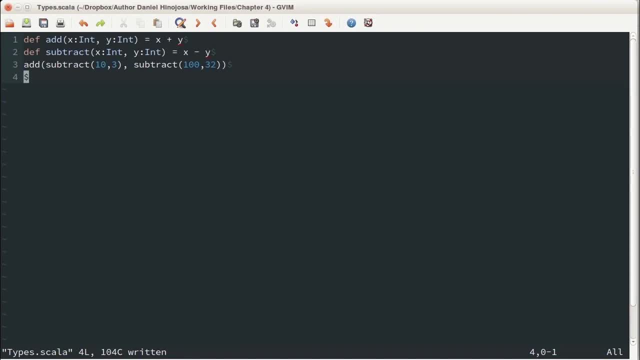 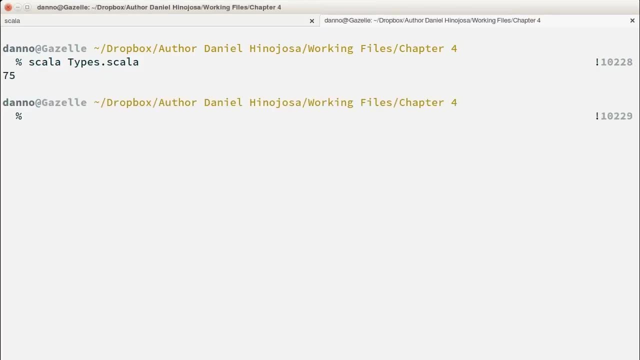 and will not destroy us in hot molten lava. so let's go ahead and run this and let's see what this gives us. okay, so we have our number. now let's change subtract to take in different types and return a different type. see what happens now. what we're doing is we changed int. 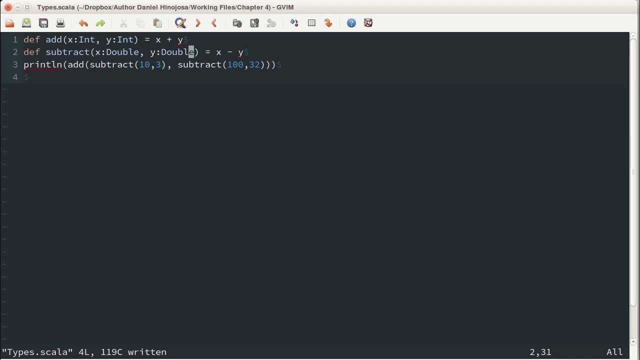 to double. that means via type inference, the x minus y is going to return a double. so therefore the types are not going to match because subtract returns double, and what we're trying to do is we're trying to give, add two different doubles. let's run it. 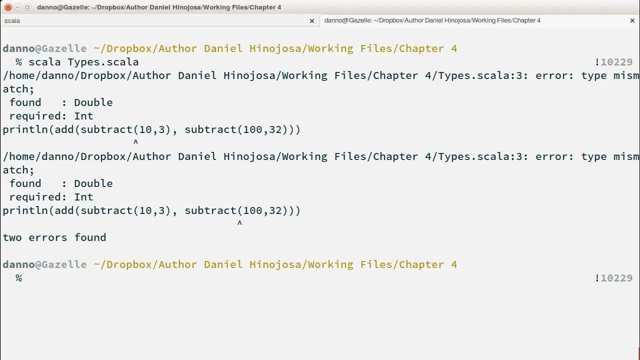 okay. so we end up with a couple of type mismatch errors. type system got us, is displeased with our attempts and punishes us with these particular exceptions. so types are good. it keeps us from making mistakes in our logic. in a moment of reflection it could be. 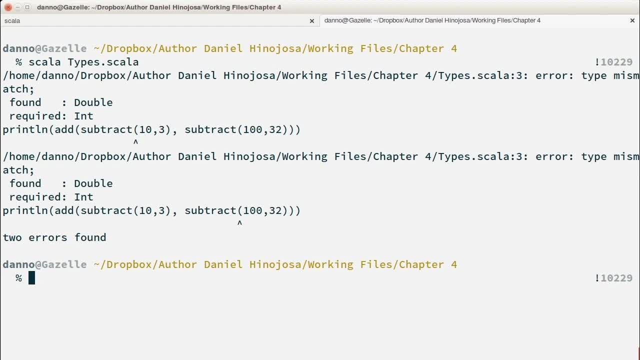 that we didn't want to perform this operation. after all, we're trying to take the double type from a subtraction and shove it into a method that takes an int, so maybe we wanted to take the double and either truncate it or round it while we're thinking about it, and this is why 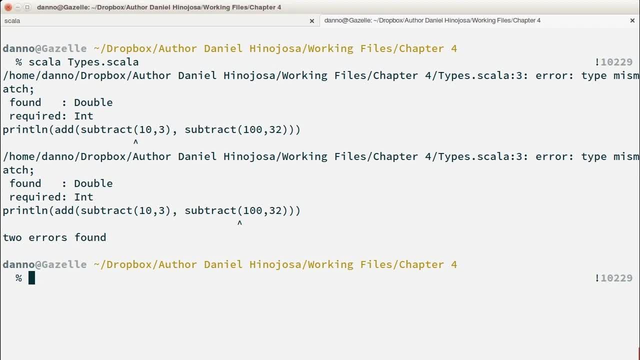 static typing is so important. it allows us to reflect on our code. maybe it is something we wanted, maybe it isn't something that we wanted after all, so let's go back to our code and try to make these types match. now, this is just an example, and 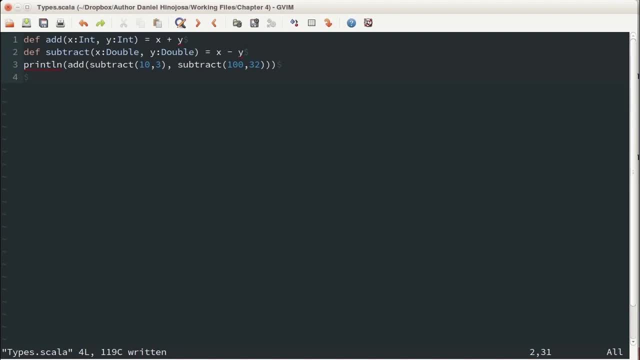 yes, the obvious answer would be: why don't I use ints to ints? but let's say, for the specification for subtract we could only use doubles and we need to find some way for these two methods to work together. so let's try perhaps a truncation here. 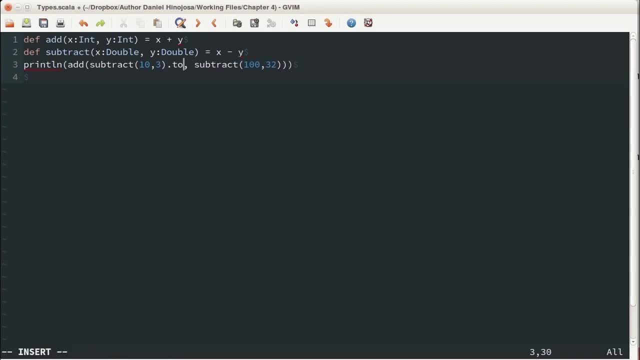 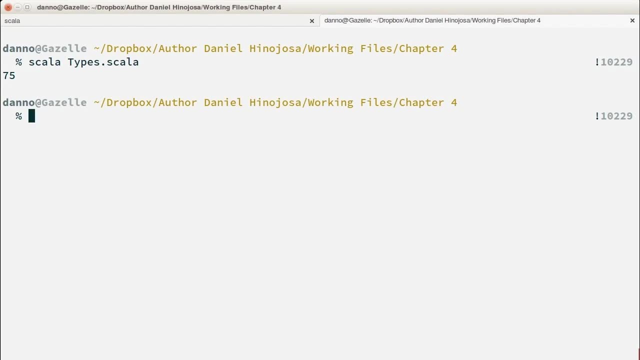 so let's say within the subtract I want to do a two int. let's run it. that works. every number type has a method that converts from one number type to another: two byte, two short, two int, two double, two car, etc. for a conversion from a double to an. 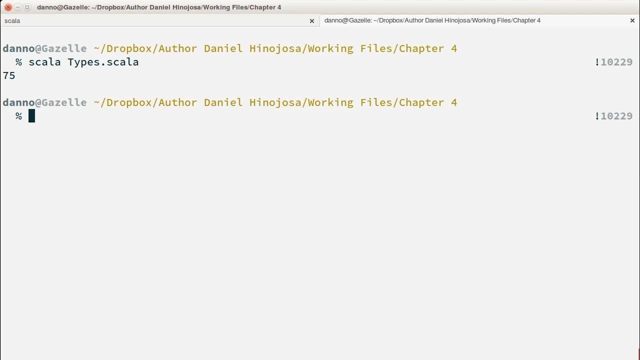 int. this is purely a truncation. let's go over to the REPL and let me show you what that means. so let's say that we have 10.0 and this is going to be a double, and let's say that we're going to take. 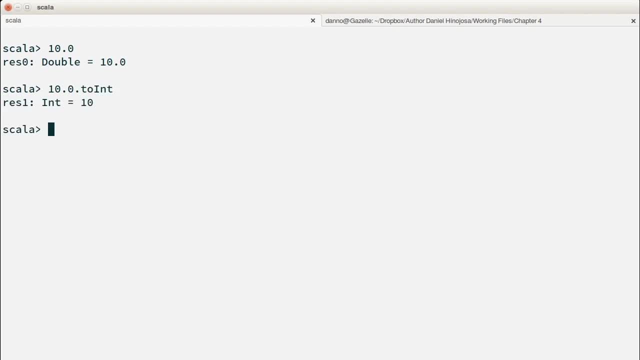 10.0 and we are going to truncate it. if this looks confusing, let's wrap the 10.0 in a paren. so we're going to take a double and call to int. that looks great. so this is a truncation. we could also do a round. 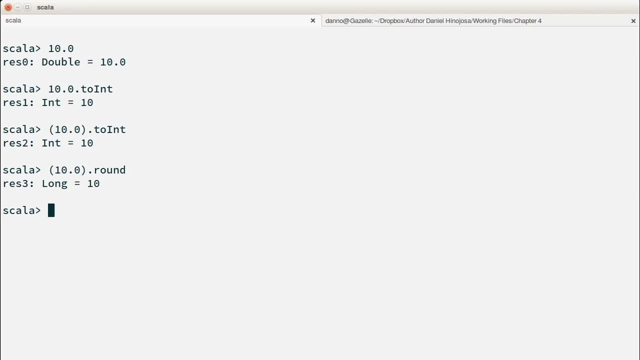 there's a problem with this. this 10.0 dot round is going to return a long and remember. the type should match what we want out of this is an int. one thing that we could do is we could possibly do a 10.0 round that and then do a two. 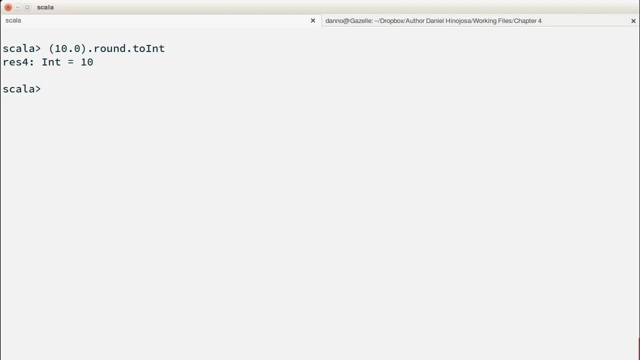 int, and this will give us the number that we're looking for and the type that we are looking for. but this comes with a warning: long is 64 bits and int is 32, so we may lose some information if we do this conversion. for example, let's 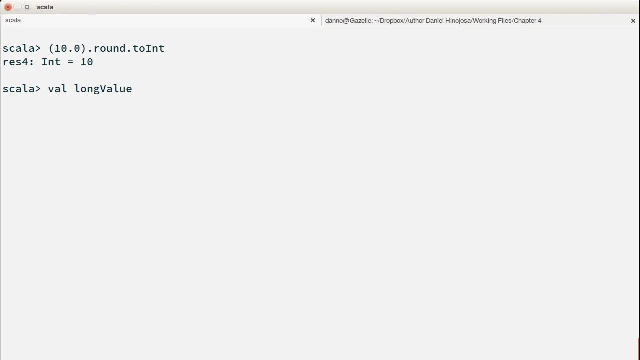 say, I have a val called long value. so what I'm going to do here is I'm going to take this long value and create a very large number and round it, and then I'm going to call to int. okay, so we have this long value, 203 949. 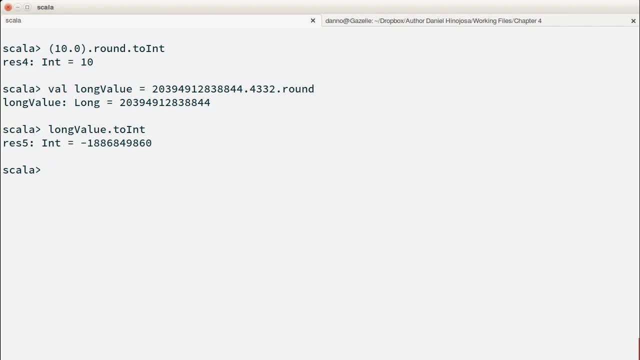 etc. dot 4332, then we call round on it. so it's going to round it out and it does so fairly nicely once I have the round number. remember this is a long. but if I call to int on this then we have an issue because int only takes so much. 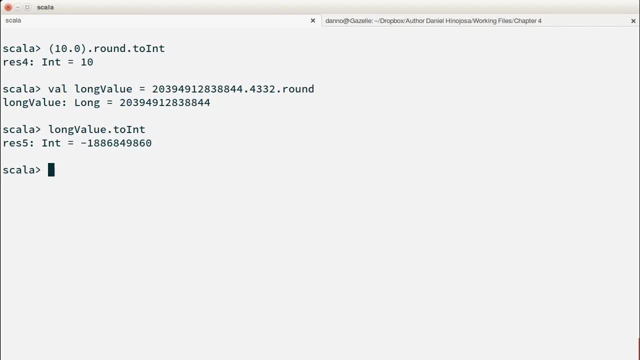 space. it takes 32 bits. long is 64 bits, so there's going to be a loss of information and because the first bit is likely going to have a sign on it, this is why the number is negative. so do we have another choice? well, there's something called 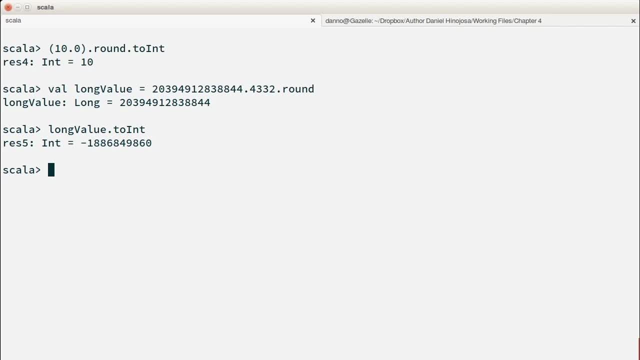 method- overloading- that we could perform to accept different types so that it wouldn't lose any of the data. there are some other types, like big int and big decimal as well, so we can cross that bridge a little bit later when we talk about overloaded methods. but back to our problem. let's say that 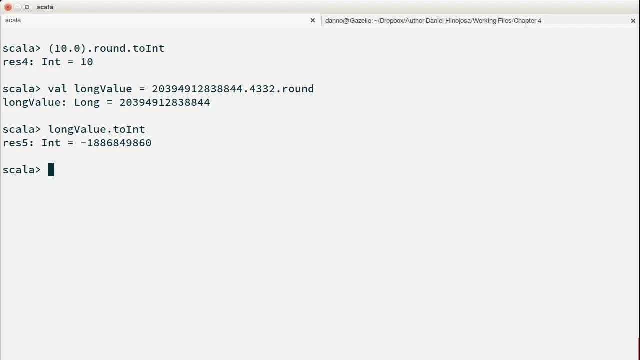 we're okay with this. let's say, we'll run the risk that some of these values would be too large and therefore it's acceptable for now. so let's go back to our code and make that change. remember, the whole point of this lesson is about type matching. 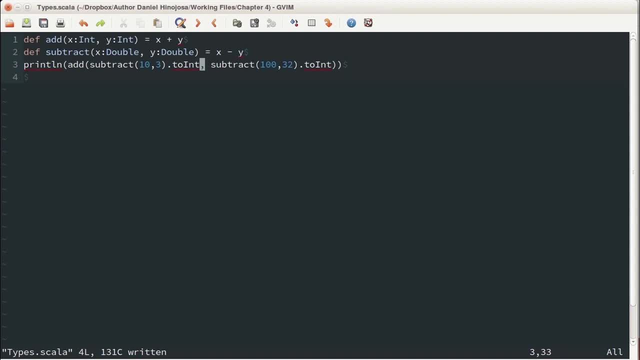 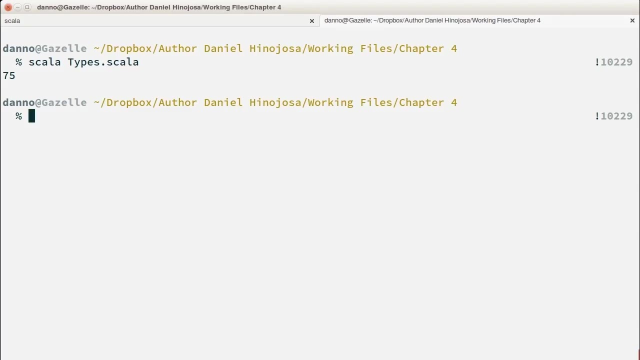 not particularly right now about whether we're getting the right answer or not. so, given this add, I have the to int. this is truncating. let's say that I want to make all of these a round and a round, let's run it okay. type: system got us is most pleased. types. 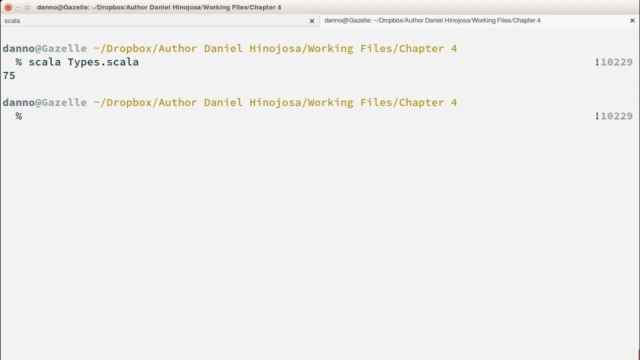 match whether your program works to your specification. again we are running the risk of possibly taking a really large number and not bringing it down correctly. but as far as the types matching, let's go back to our code and review that it works correctly again. add takes two ints. 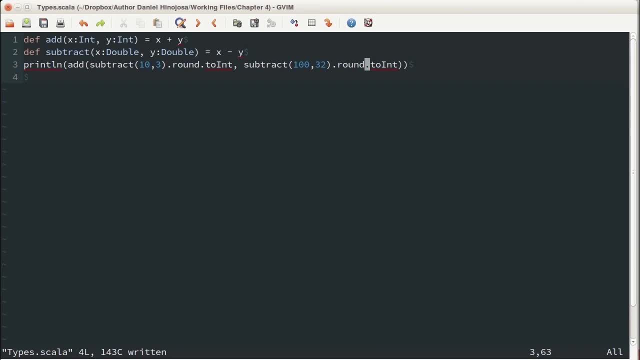 subtract returns doubles. therefore, we need to make the types match. types have relationships. scala is not only a functional programming language, but it's also an object oriented language. in fact, I'd like to argue that it's even more an object oriented language than java. in java, there are objects. 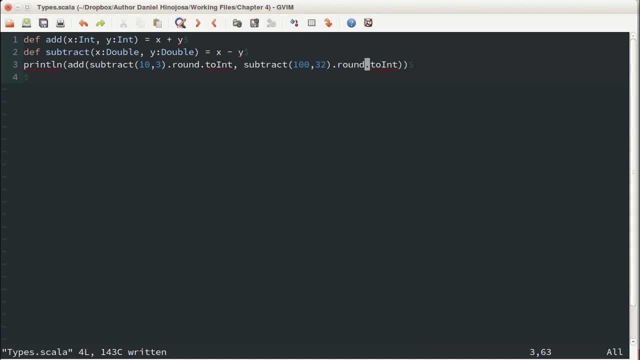 and there are primitives in scala. you can treat everything like an object and if you can do that, you can treat all numbers, characters, booleans, as types. every type has a relationship and is a member of an illustrious family tree. so let's take a look at this family tree. 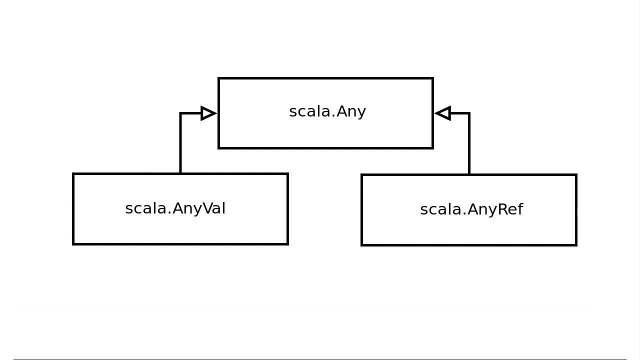 unlike humans, procreation, an object oriented system, does not require two parents, just one. in scala, any is the parent of all types, any val is the parent of all numbers, booleans, characters. for the java people migrating to scala, that means that all your primitives have a parent and that parent. 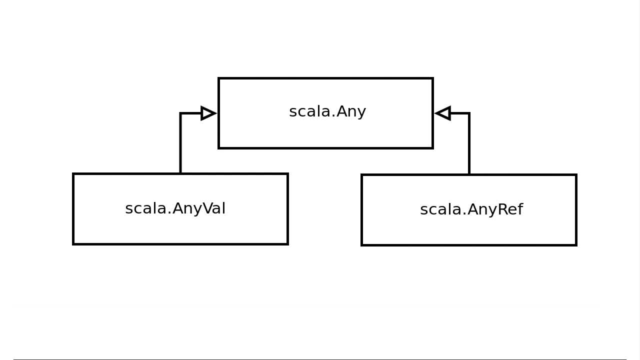 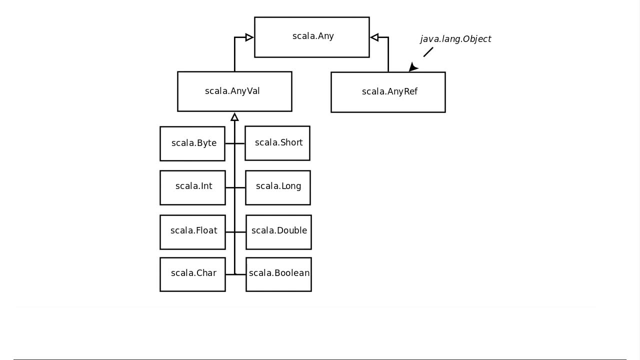 is any val. any ref is any other type that has a class, whether scala created it, whether java created it or whether you created it in either java or scala. here's a fuller graph again. any is the top most parent. any val is the parent for all primitives. 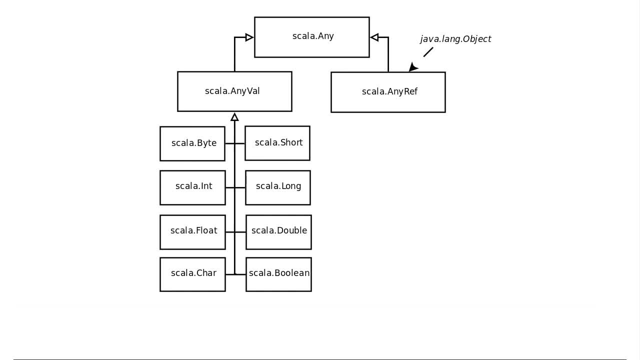 and any ref is the parent of all objects. it's also worth noting that for the java programmers coming in, java lang object is going to be semantically the same as any ref. again, here's any val. that is going to be the supertype of all primitives. 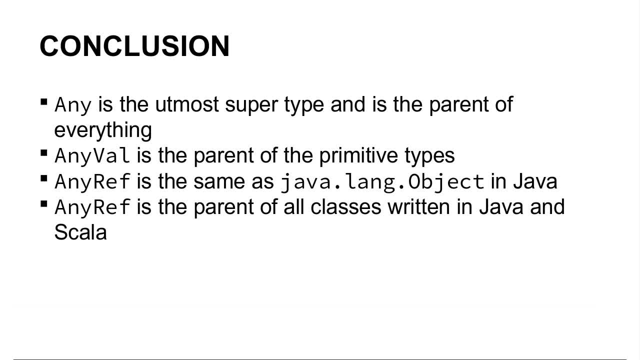 so types are templates that make up an object. primitives are also types in scala, in short, by character, booleans, etc. types need to be matched up like a puzzle. if it isn't, the type system at compile time will tell you there's a type mismatch every type. 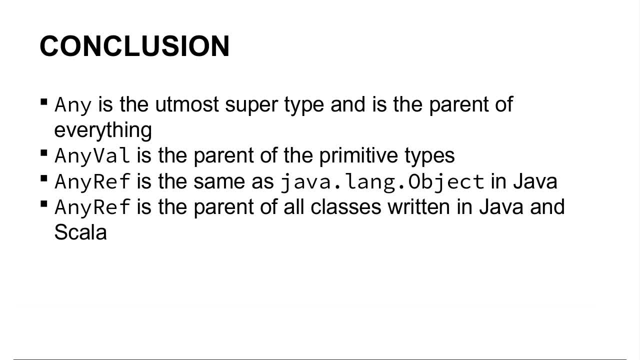 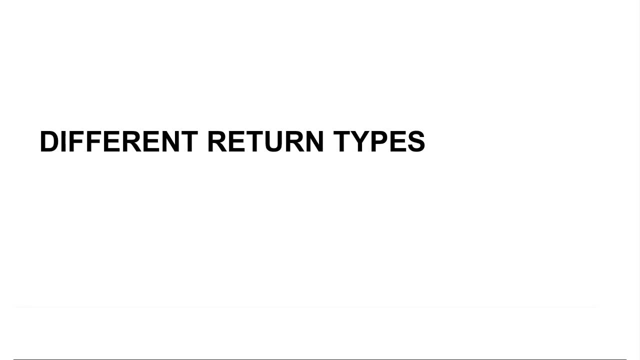 is in a relationship: any is the parent for all types, any val is the parent for all primitives and any ref is the parent for all scala, java and custom objects that you create. in this section we'll be discussing methods returning different types and what the type inferencer will decide is the best. 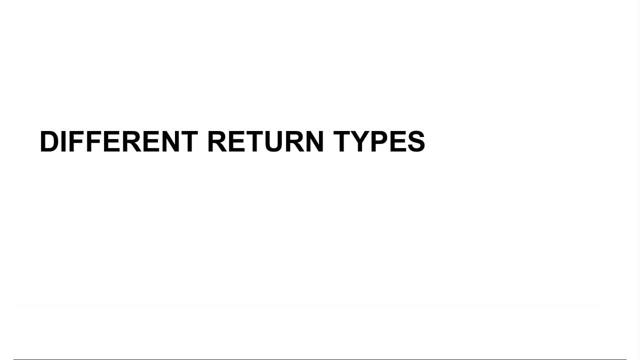 return type. scala's type inferencer will always make the best choice given the information that it has, since we know how return types work with methods and we generally know about types in scala and how everything eventually extends from either any val or any ref, and we also know that any val and any ref 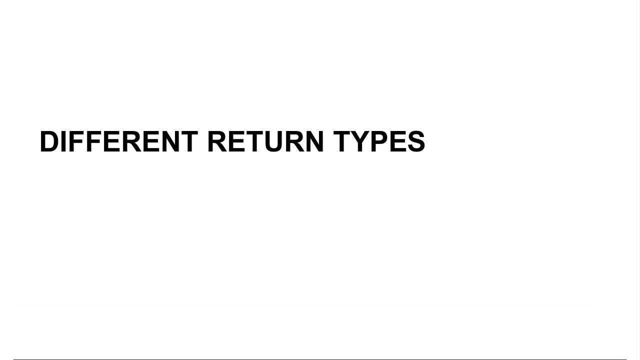 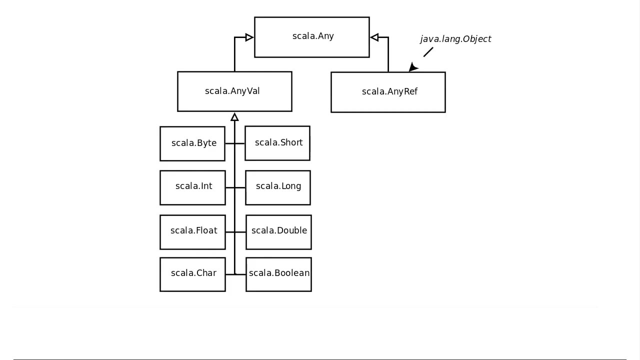 extend from any. from the previous session. here is a class diagram from the previous session as a reminder. any val extends from any, any ref extends from any. any val is the superclass for all primitives and any ref is the superclass for all classes. here it is again. here is any, any val, any ref. 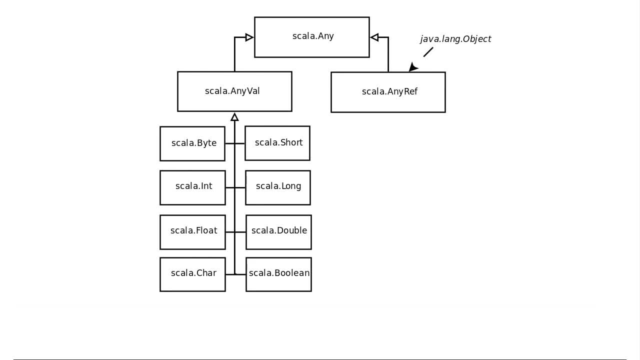 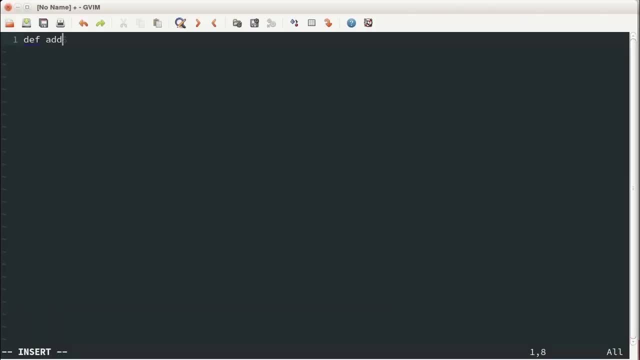 again, any val is the superclass for all primitives. given this now we'll understand what will happen if we do something like this. so let's go over to the editor and give this a try. let's say i want to create a method called add. given two ints, what i'd 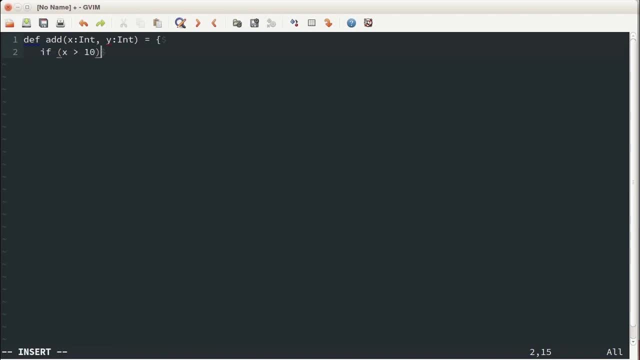 like to do is i'd like to ask the question if x is greater than 10 and i'd like to return. okay, so i have method add, bringing in two ints. if x is greater than 10, then do the summation, but return it as a string. otherwise. 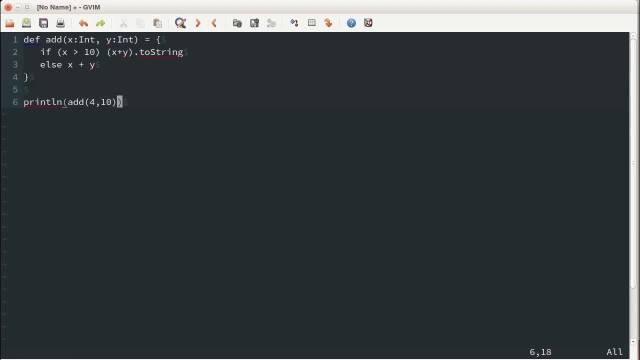 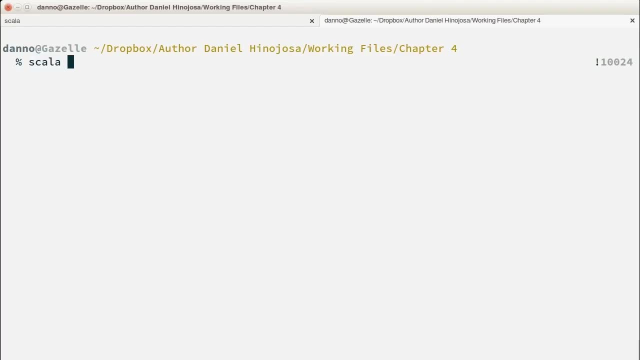 do the addition. finally, let's do a print line and save this in a file called different return types, dot scala. now i'm going to run it, so it does what we are expecting. we don't know, though, if this 14 is really a string or an int. 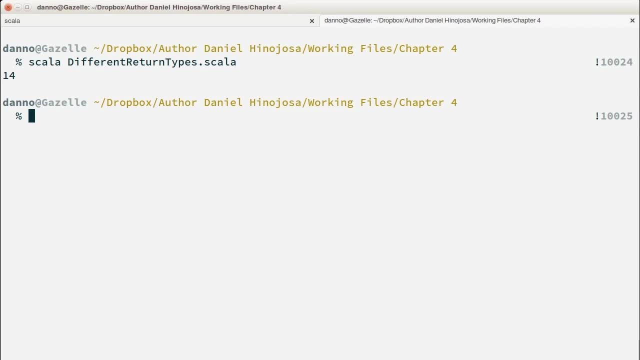 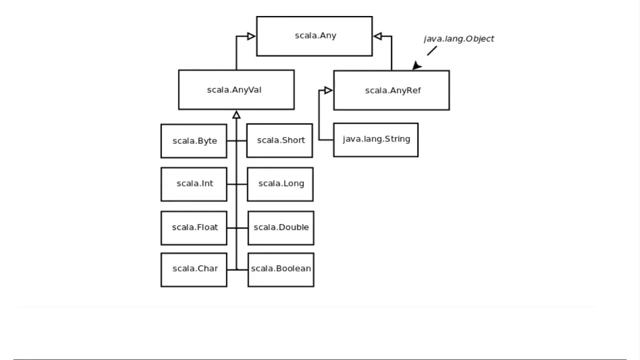 what do you think the return type of this actually is? in order to do that, let's look back at our chart, but this time let's include string. here is string. remember. any class will extend from any ref and, of course, any ref is a child of any. int is a child of any. 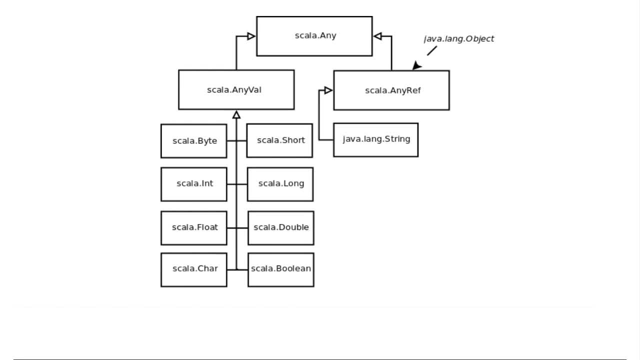 val, and that is, of course, a child of any. now we have to determine what is the common parent for both string and int. well, that would be any. therefore, the return type for the method we just created is any. to verify that, let's copy the code and: 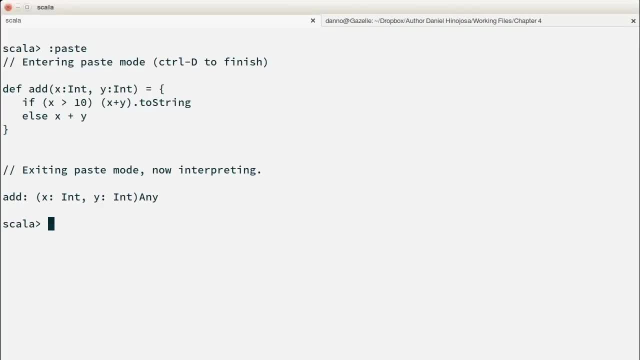 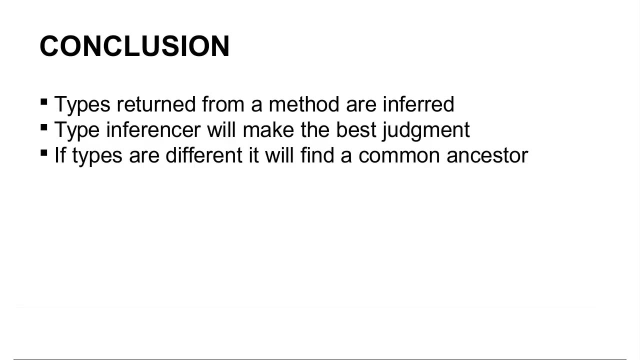 put that into a repl. as you can see, the return type for the add is any. so in conclusion, types inside of a method- this could also be applied to functions, as we will discuss later- will be inferred the type. hamster will make its best judgment based on what is available. 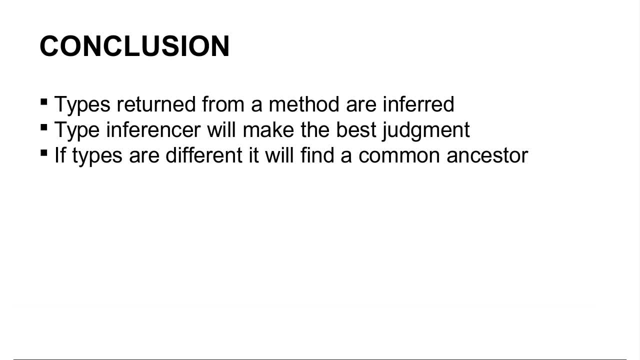 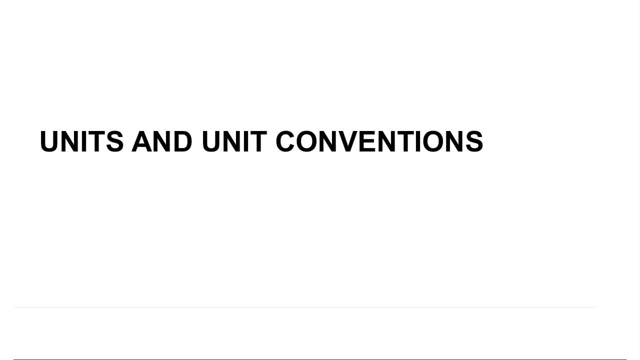 if types are different, it will find a common ancestor and use that type. in this section we will be discussing unit, what it means and its conventions. let's go over the repl and get started with unit. there is a value we can create. it's an open paren and close paren. 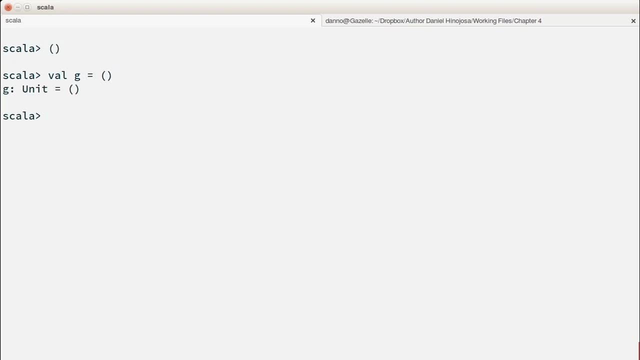 this could be assigned. now this type is inferred and it is called a unit. we could be explicit about it if we want to. unit is something that you get when there is nothing to give. the analogy in java is that this is a void, or what you consider to be. 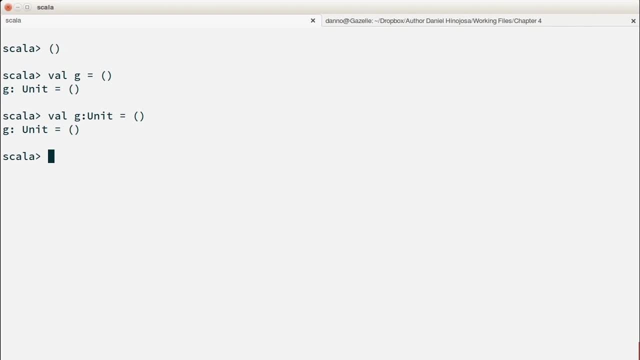 a void. when would we use unit? well, you've already used one, and it's called print line, so let's go over to the documentation. by the way, if you want to take a look at the documentation, it's at this address. the api is at scala-langorg. 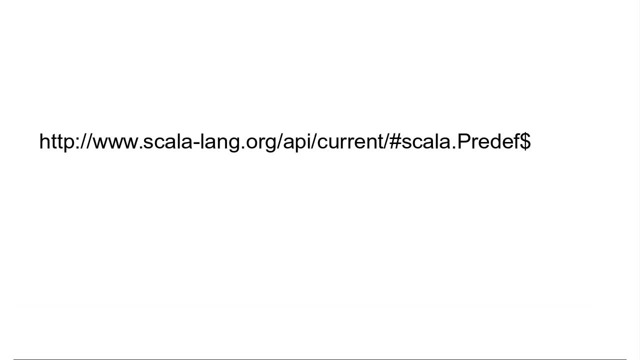 slash api. slash current. current will get you the latest api for your perusal, and what we're going to look at is called the predef. now, predef is an object- we haven't discussed objects yet- but a predef is something that is inherited in every. 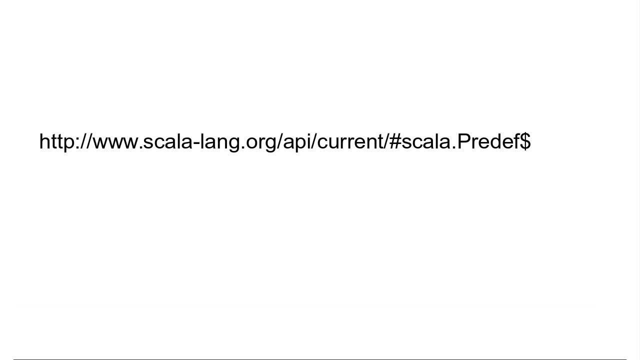 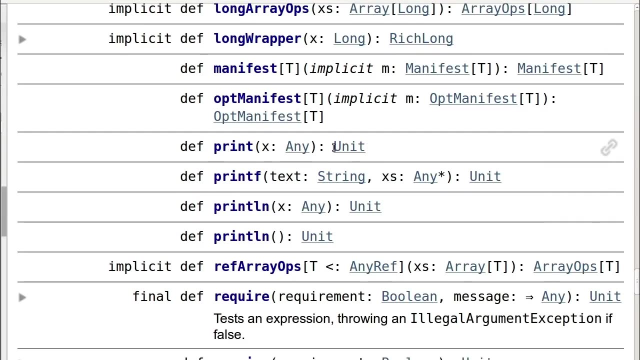 scala class object file that there is out there, so it's automatically imported. so let's take a look at the predef, or a little bit of the predef. as you can see, there is print that takes an any and it returns a unit. we did print line before. 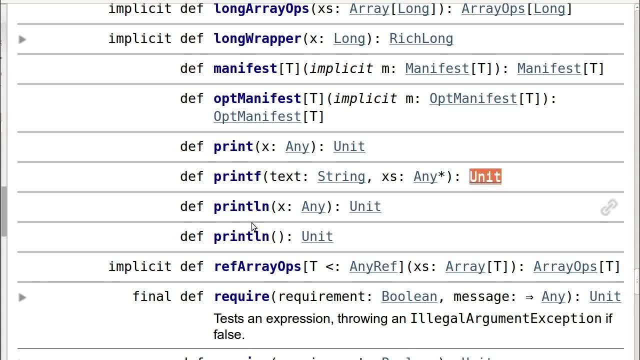 there is printf. we also did that one before. this one shows a unit. here is print line. this takes an any. you know what any is? now, that is the parent of everything. so that means that we can give print line any type that we want and it's going to print it out and this is going. 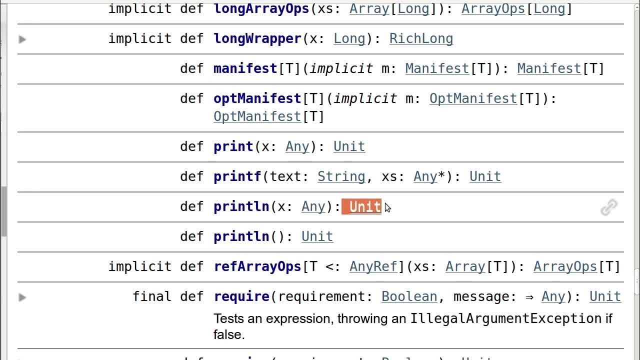 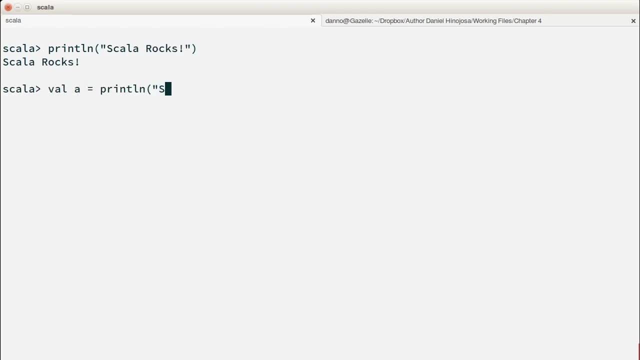 to return a unit- the type is unit, meaning again it's analogous to void- we're not getting anything in return. so, in fact, when we type this into the REPL, let's go back to the REPL. if we type in print line, scala, rocks in fact, instead of just that. 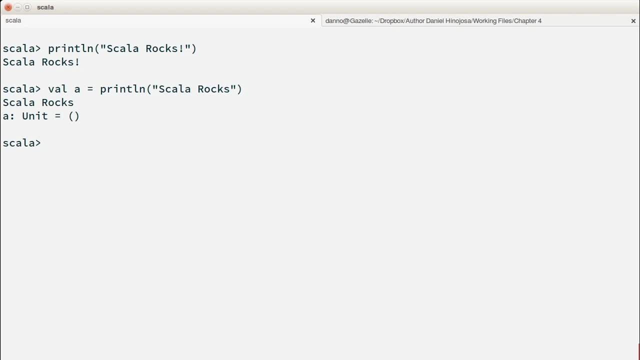 let's assign it to something. we see that the return type- after we did a print line scala- rocks and assign it to a, we see that a is of a type. that type happens to be a unit. if you go to java, for example, you can't do a system. 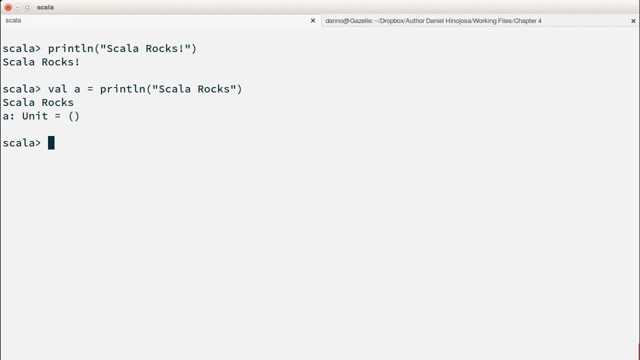 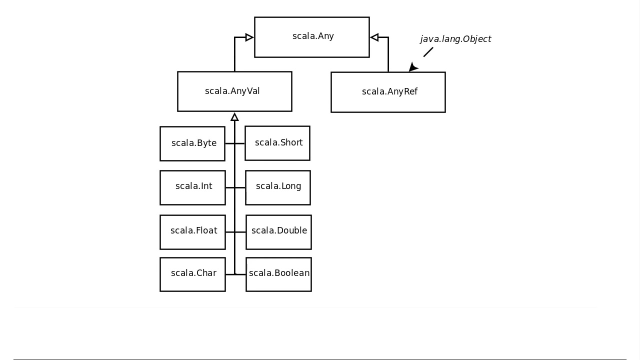 out print line call and assign it elsewhere. but in scala you can, because unit is a type, it is a sign able. so where is unit in our hierarchy chart? there it is. it's actually thought of as a primitive and it is a subtype of any val. so keep that in mind, let's do something. 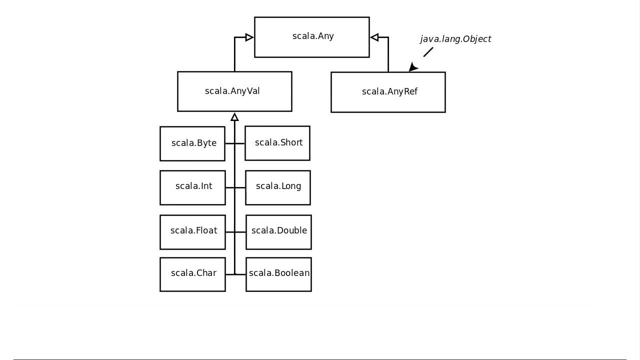 else I'm going to go back to our REPL. so again, remember this: right here we have scala unit and that is a child of any val. it is considered to scala programmers a primitive. so in our REPL I'm going to do an add much like the tire. 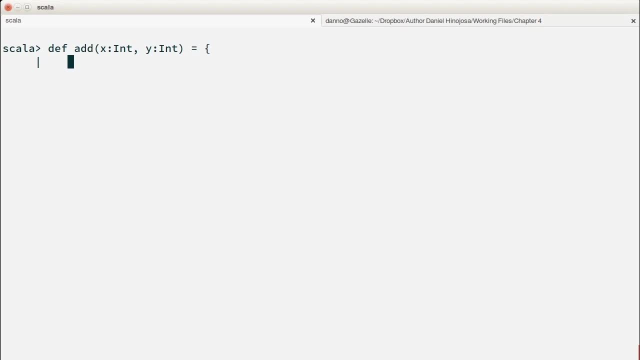 old example. we've been doing up to this point. but what I'd like to do inside this method is ask: well, if x is greater than 10, then we wish to return a print line again. may seem kind of strange that we're returning a print line, but since we 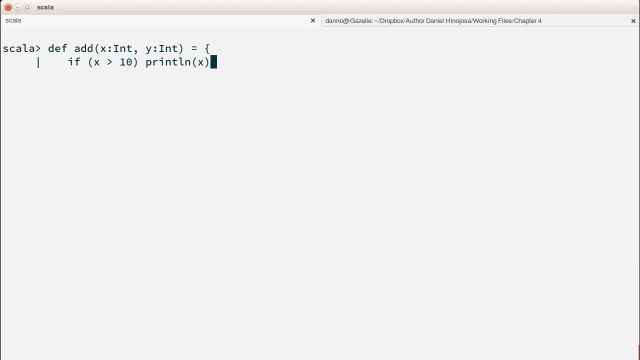 know that print line is returning a unit, we know that that unit will then be the return value from it. I'm going to have an else case: in case it is not greater than 10, then we'd like to return the summation and we'll close that. 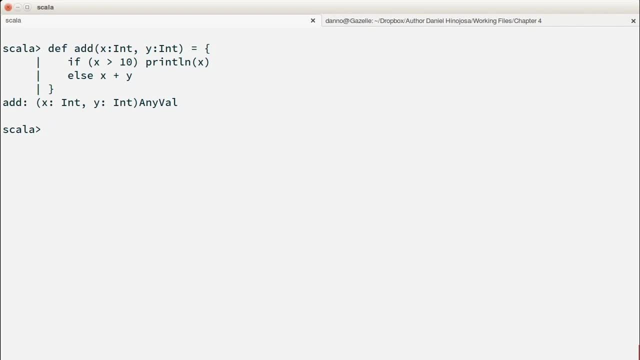 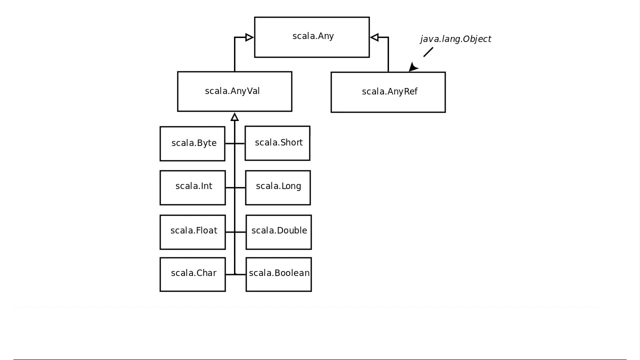 up. so again, print line returns a unit. x plus y naturally returns an int. and what do we have here? any val? let's go over to our hierarchy chart. take a look at this again: both unit and int. remember int would have been the type given x plus y. 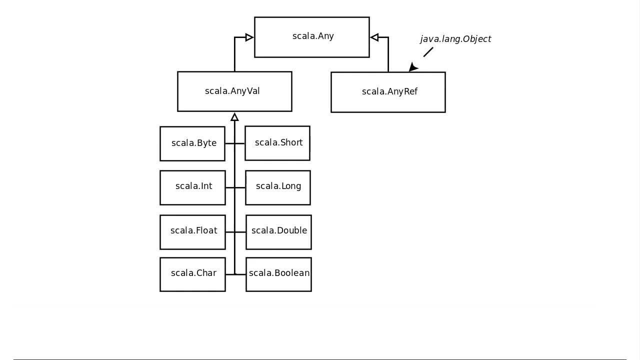 x plus y would have returned an int, but print line returns a unit. remember, unit is something that is assignable. so therefore, in something like this, if we're giving two different types, then the return type of the method said it was any val. why is it any val? 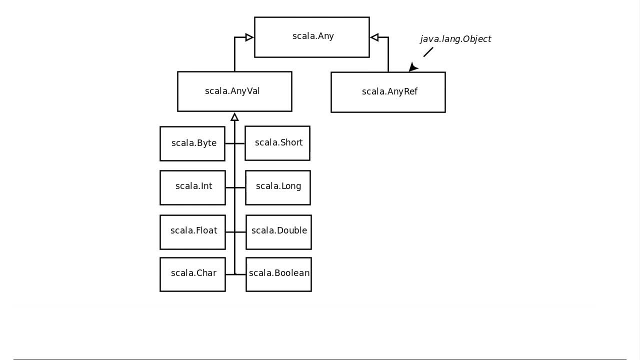 because it is the parent of both int and unit. programming to a type system is all about putting the pieces into a puzzle. if the types match, then it will work. so let's get a little crazy for a no real life but purely academic example. let's give something. 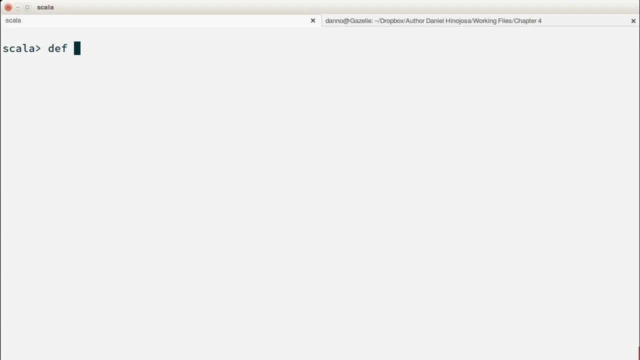 else a try. I'm going to go back to the REPL and create a method called nonsense and we're going to bring in a unit and we're going to return an int in this case, and the return will be a 40, as you can see here the signature for: 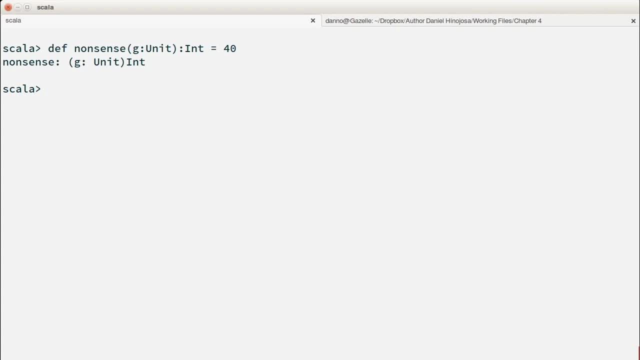 this method. nonsense is that we are receiving a unit and we are returning an int. so if we wish to call it, we'd have to call it with the parens and we would have to make sure that we tell Scala. what we're trying to do is. 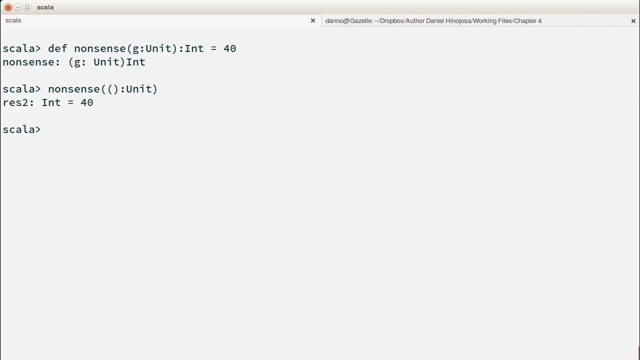 we're trying to give it a unit so we get a 40 out of it. we're giving it the value of the open paren and close paren and we're getting 40 back. now why did I do such a dumb example? to show you that unit is an object and it can be. 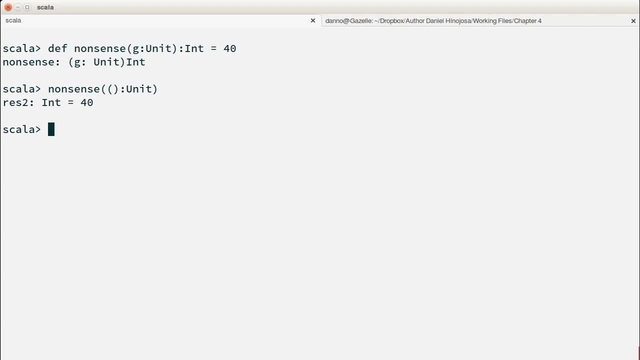 used anywhere. so imagine putting void into a method. in a programming language like java, it's not going to work. but in Scala, if you want to think about it this way, unit is an object and it has a type, and we can just treat it like any other object. there isn't. 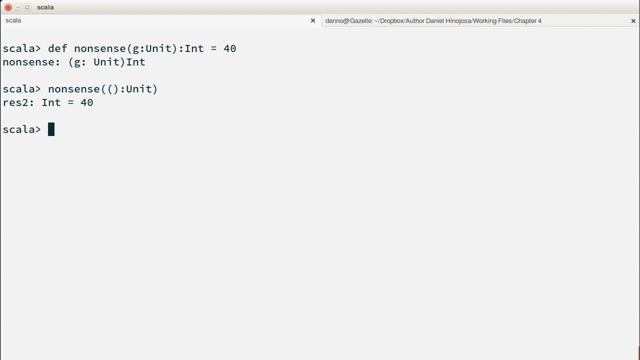 much you can do with unit, it is what it is. it's just this plain object that you can move about. it is just a representation of the of a no value. so let's go back to a simpler time, when we worked on a basic method, and try something else. 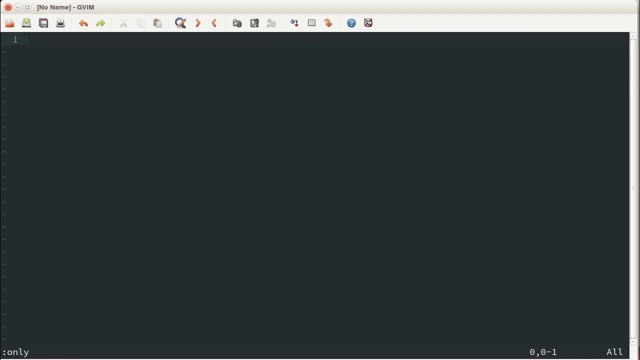 let's go to our editor. so I'm going to create in our editor. I'm going to create a method called add, which takes two ints and obviously returns x plus y. I'm going to save this in a file called unit methods- dot Scala. now, this is a simple method in Scala that adds: 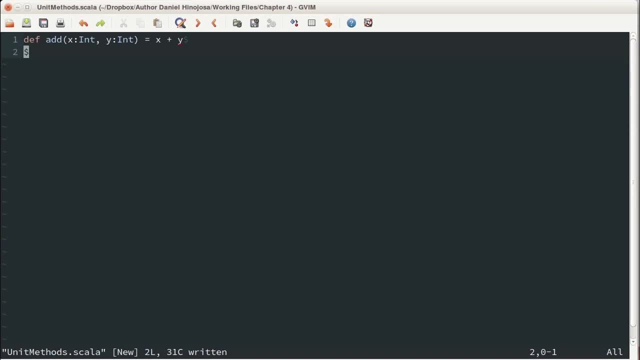 two numbers- I mentioned this in the basic methods video- that and an equals is used. that it states that we want to return something. let me add some braces. the reason I brought this up is because a common mistake for Scala programmers, especially those that come from the land of java, is that they often 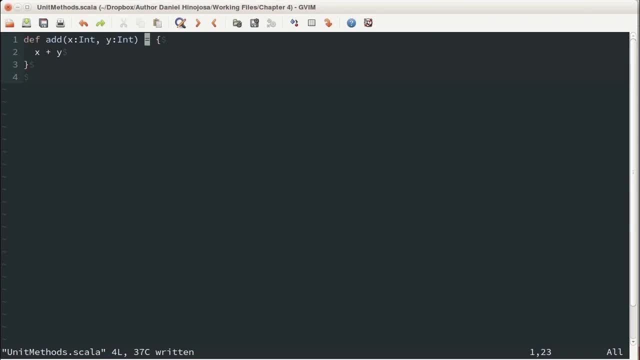 forget to include this equals at the end of the method. remember, equals means that we want to return something from a method, so let me do a bad add. the method up top is correct. the method down below, called bad add, is incorrect. I'm going to do a print line on this. 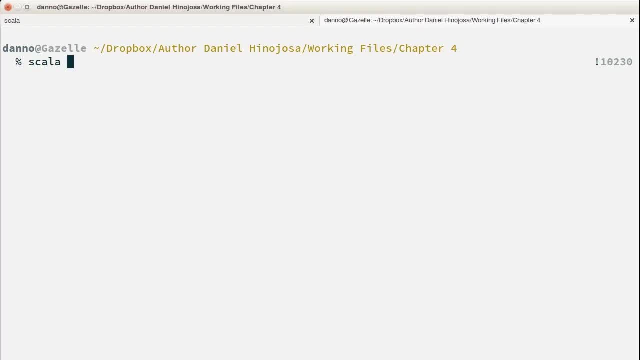 bad add. now I'm going to run it. okay. so this returns an open paren and a close paren. you know what that is. that's a unit, remember. I mentioned the open paren and close paren is the value for the unit type and when you see that, don't panic, it's just an. 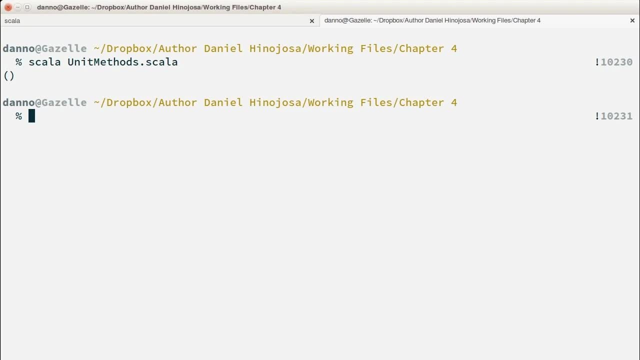 object that tells us we got nothing from it. in other words, it is a void. if we wanted to be explicit about our bad add, let's say it was intentional that we wanted to return a unit. we could just say: well, we want to return a unit, let's go back to our 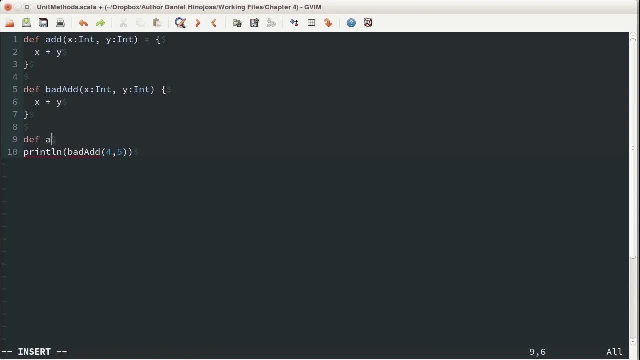 code again. if we wanted to be intentional about it, let's call this one something different. I'm going to call this add unit that takes a x and a y, but this time what I want to do is I want to be explicit about it and state I: 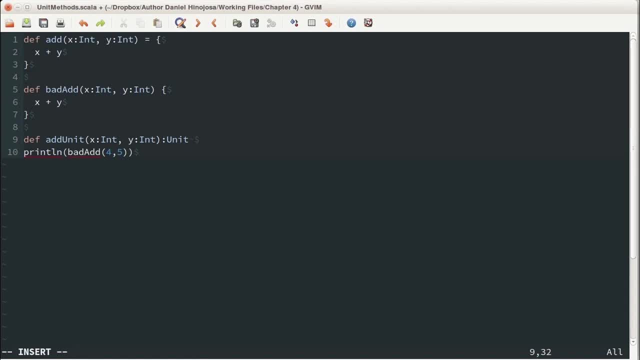 know what I'm doing and this is going to be returning a unit. in fact, I could use the equals here. I am returning something and in this case what I'm returning is actually a unit. so in my case, now I have add unit, takes in two ints returns. 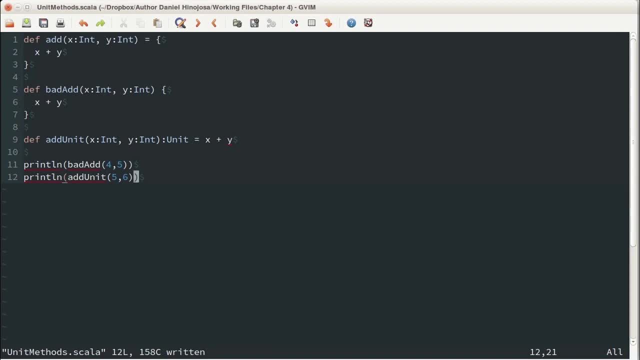 a unit. I am being explicit about that. I am using the equals. I am returning something. remember. unit is an object. I can return it. I'm adding x plus y, but that's irrelevant, because what I'm returning out of here is nothing. let's run this same thing. 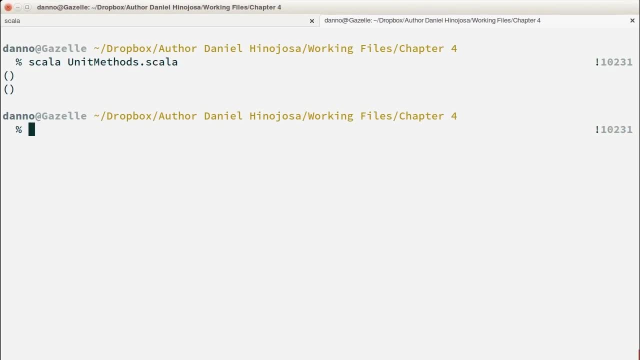 when we run it again. I didn't call it bad add because this was intentional. I did do it on purpose. I called it add unit. but remember the point here is: whenever you see the open paren, close paren, it is a unit. the type is unit, there is only one. 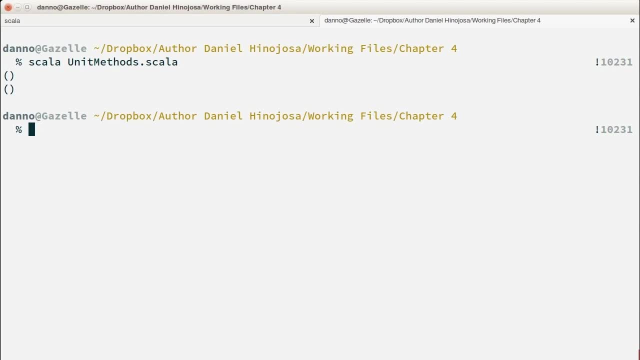 value for unit and that's the open paren and close paren. unit will be used sparingly as a return type in Scala. in pure functional languages you won't see it at all. whenever there is a return type of unit, it likely has a pure side effect. this has nothing to do with pharmaceuticals. 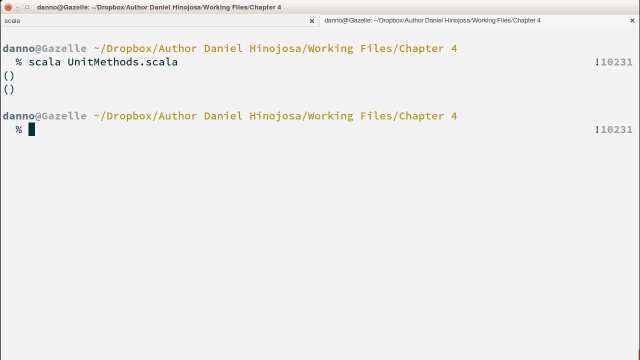 a side effect is something that happens to the outside world, perhaps something like printing to a screen, writing to a file system, sending items over a network. when we are printing to a screen, that's the case of a print line. that is a side effect that happens. sometimes we are even. 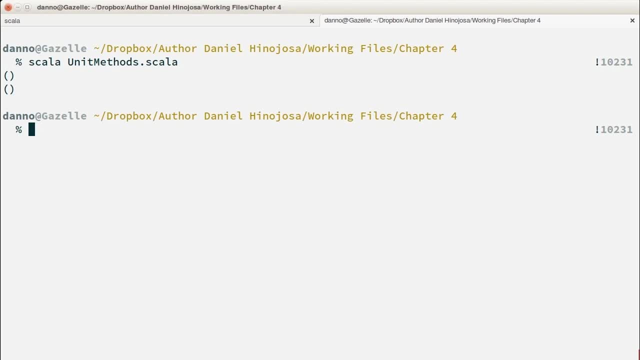 changing the state of an object. changing the state of an object is also considered a side effect. let's try another sample of code. let's go back to our editor. I am going to create a new file called side effect state, to show you what I mean by state. 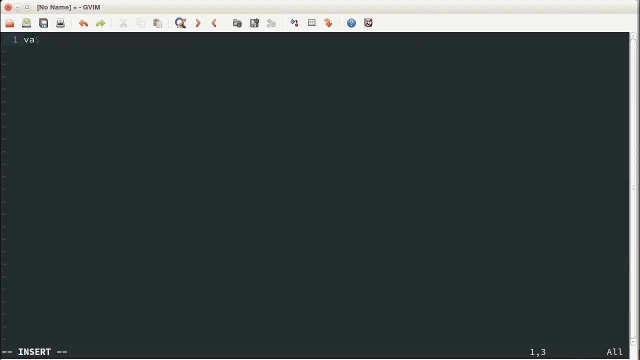 in this example, I am going to create a var. remember: var means that there is a side effect. there is something that is mutable. create a var. a is equal to zero. I created a method called side effect. in fact, take a look here- I did not include an equals. this is going to. 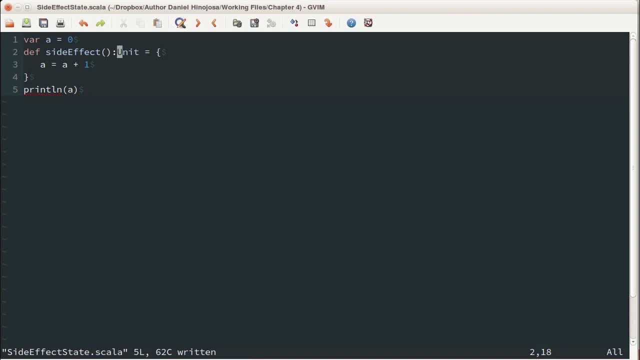 return a unit. as I mentioned before, it is up to me whether I want to declare this returning a unit or I could just leave the return type out. and if I am returning a unit, I can leave the equals sign out. this is changing the state of an object again. 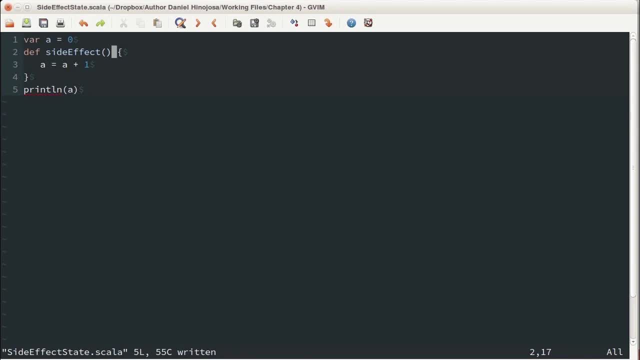 I have a var. var is usually an indication that something is mutable. also an indication that sometime down the line there is a change in state. now you don't have to be too stringent on avoiding state, although some functional programming purists may disagree. there is a topic called state monad. 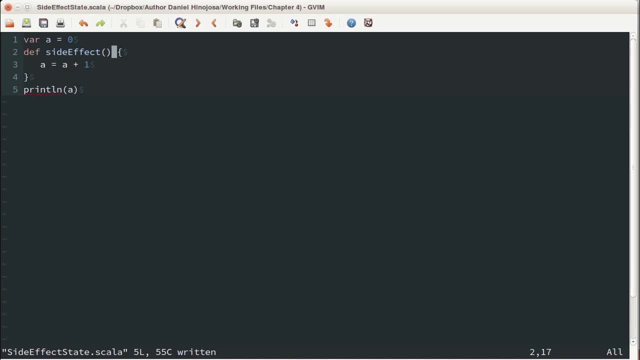 which is a functional design pattern that you can use to hold state by avoiding a lot of these side effects. that is not covered in this series, but in time it may be something you want to learn up on after you get some more functional knowledge in that squishy brain of yours. 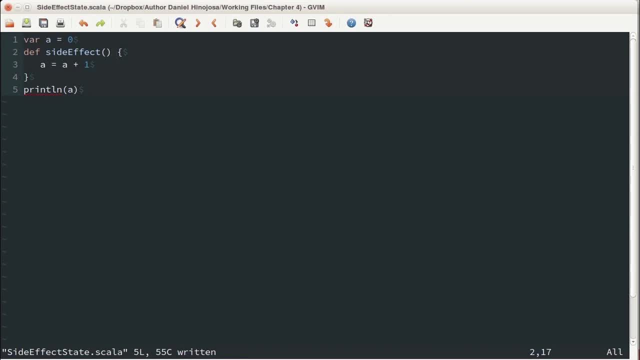 I will mention this. the whole idea for Scala is to bring over Java programmers, to make it comfortable for Java programmers. so keep that in mind. you are not doing things wrong if you are bringing in your object oriented knowledge over it. you are bringing your mutable knowledge over. 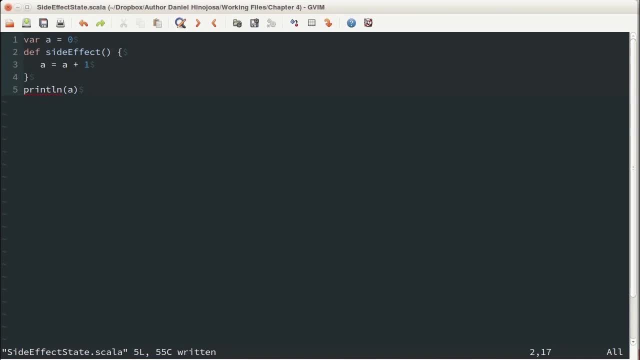 to work with you again. over time you are going to learn some other concepts and once you learn those concepts, it could very well be that you don't like these side effects and you wish to implement a lot of these functional design patterns to avoid them. so, in conclusion, units: 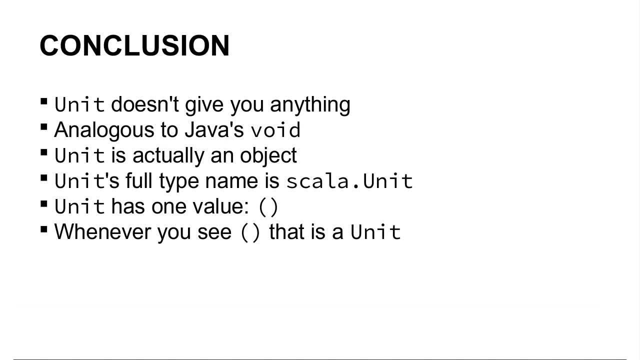 don't give you anything. they are analogous to Java's void and units are actually objects. the unit full type name is Scalaunit from the Scala package. unit has one value: the open paren and close paren. and whenever you see the open paren and close paren, that is a unit. 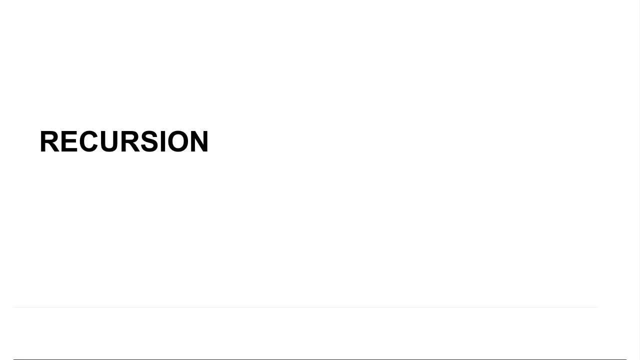 recursive programming is essential in functional programming. it is strategically recalling a method to perform a task, and this section will create a method that is called recursively onto itself. let's start off with a file. we are going to call it basic recursion- dot Scala. let's create a simple recursive method to do recursion. 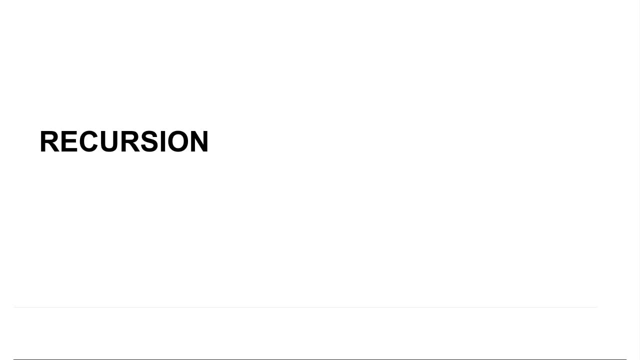 I think maybe most of you will know what a factorial is. but if not, factorial is the product of all the positive integers less than or equal to n. given whatever n is, a factorial is usually denoted as a number with an exclamation point and as a special rule. 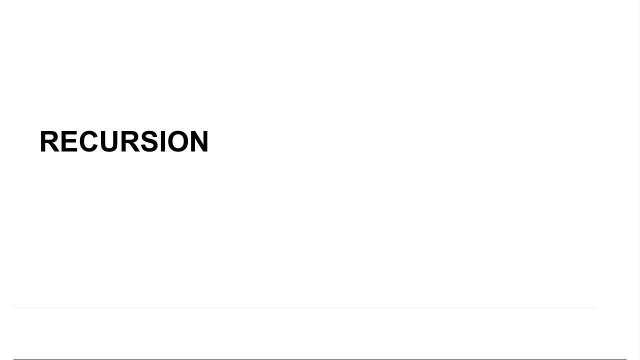 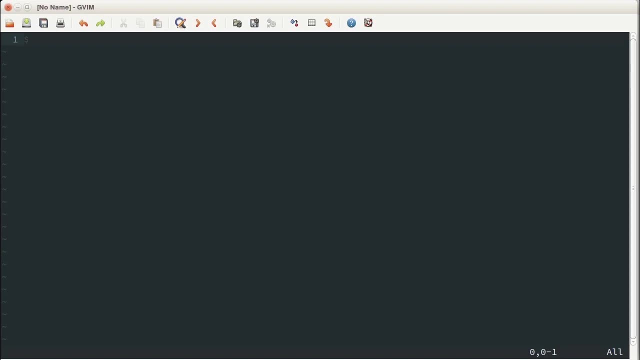 the factorial of 0 is 1. so let's get started. I am going to head over to the editor again. if we have a factorial of 5, that is going to have to be 5 times 4 times 3 times 2 times 1. 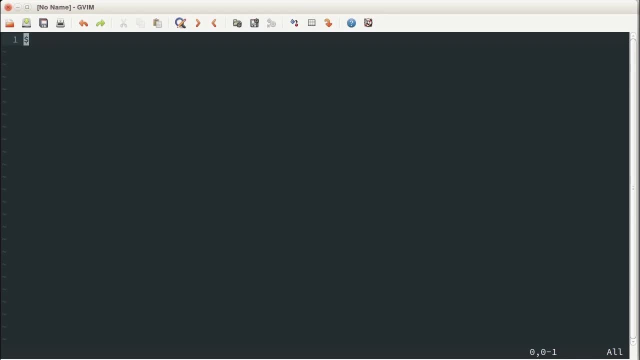 factorial, again, of 0 has to be 1. factorial of 1 is going to be a 1, so let's get started. ok, so here is the first line: def: factorial. we are going to bring in an n, it is an int and we are going to 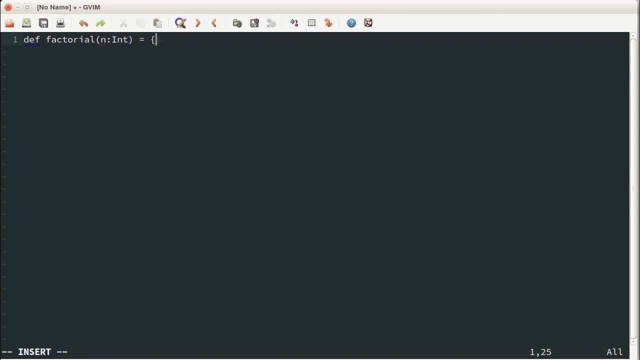 return something. but first of all, we need a base case, and the base case is the simplest thing that we can do. how do we code that? well, our base case is whether it is 0 or if it is 1, then the answer has to be 1. 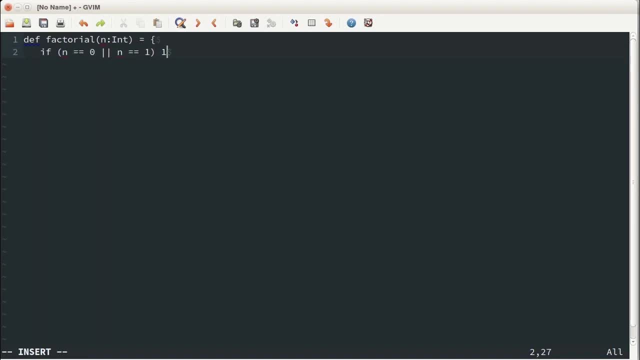 so let's do that. so in case it is 0 or in case it is 1, then it will be 1, otherwise we are going to take n, whatever number it is. so if we give it 5, we are going to say 5 times now what we are going to do. 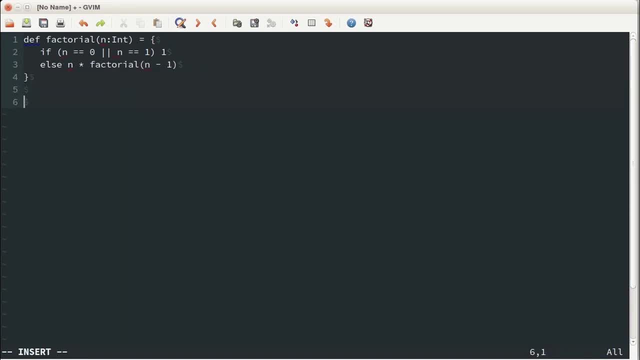 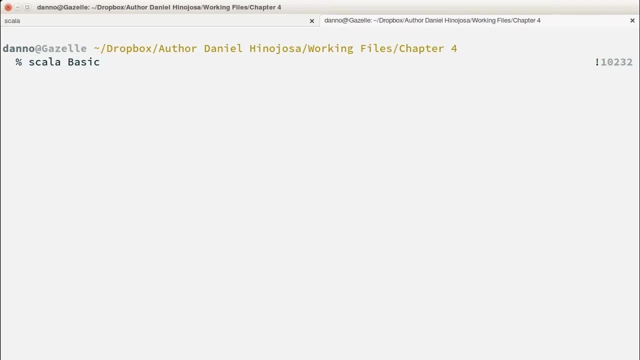 is call factorial with a deduction. let's do a print line and save this. 5. let's run it ok, so we end up with an error. recursive method: factorial needs a result type. this happens to be one of the rules for recursion: return type must be declared. let's fix that. 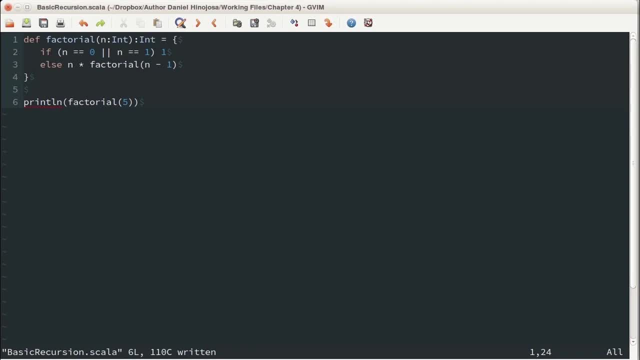 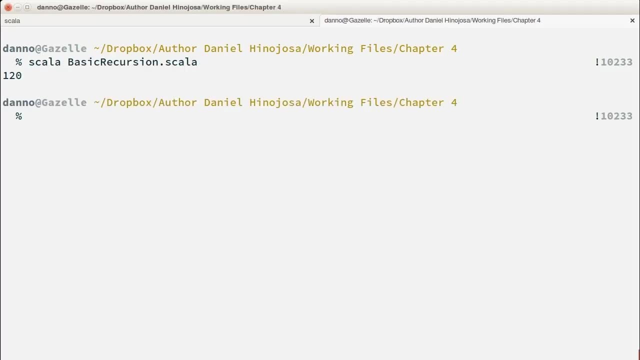 we do need an int. we do need to declare the return type. let's save it and run it. that's fantastic. it works. we have a recursive method. only problem now is that this doesn't go very far. let's add another item. let's go back to the editor. 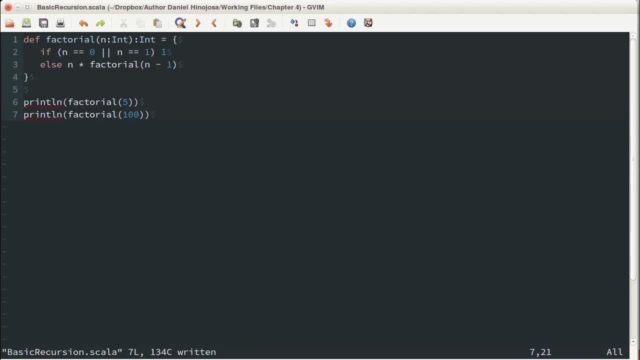 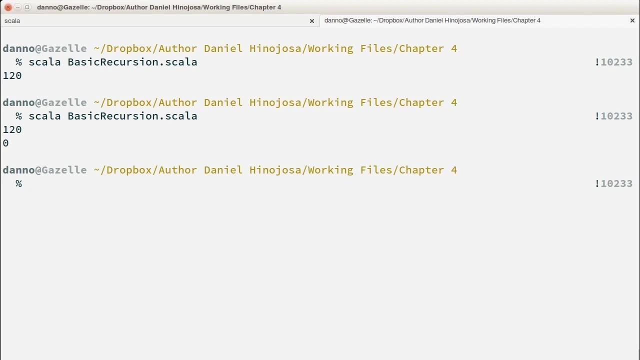 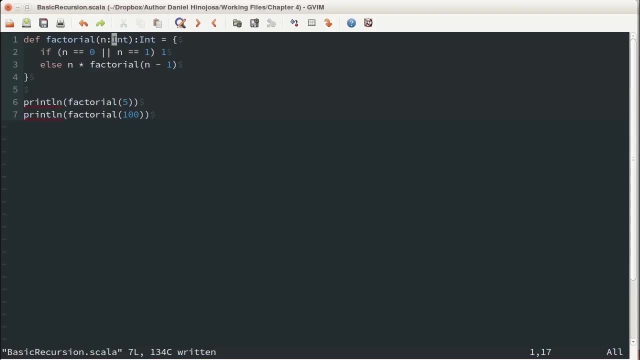 instead of 5, let's do 100. not a huge request. let's give it a try. interesting: 0, it overflows and this is not right. so let's change things around. let's do a big int. big int happens to be a class that has storage. 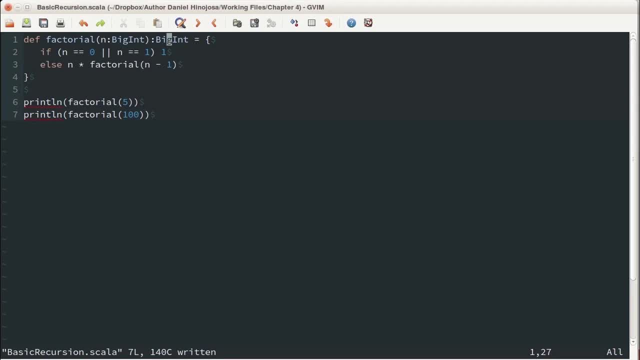 and enough storage that we can store very large numbers, just holds more information and, believe it or not, this is all that is required. just change the types. though it is tough to see right now, there is something good happening at the compiler level and for those coming in. 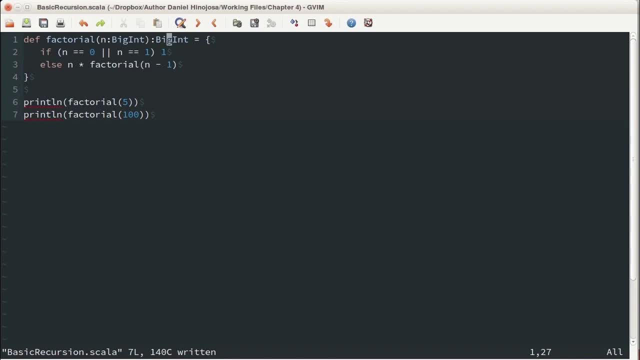 from java, you would understand. we didn't have to change the methods or the structure that much of the method, because big int has the same method names as int. in other words, big int has a star, big int has a subtraction, big int has a quality, it can also convert. 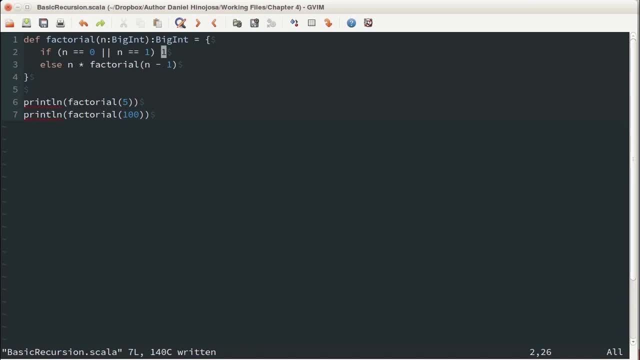 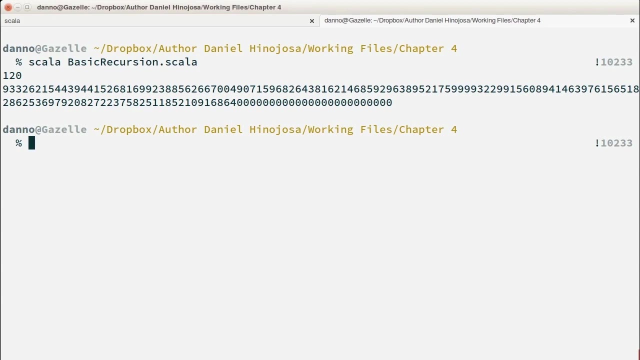 the one into a big int one automatically. what that means for you is you can express yourself faster without paying too much consequence on changing the type being used. let's run this nice, we get a very big number. so therefore the factorial for 100 is 933, etc. 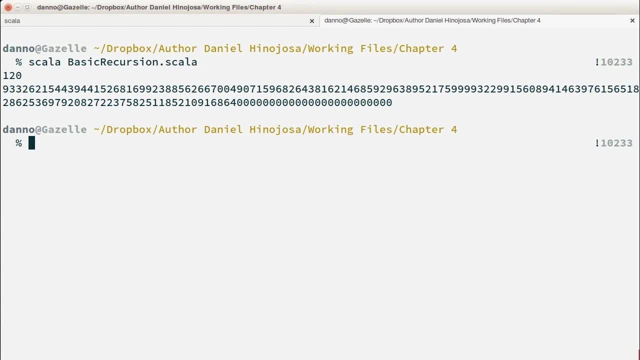 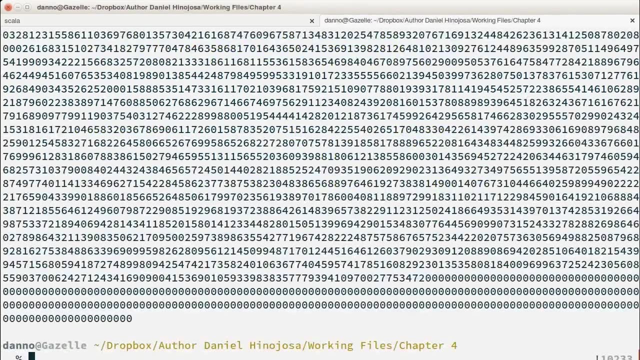 now, let's give it something harder to work on. let's go back to the editor. just one more 0. let's run it looking very good now. of course, this is the factorial of 1000. of course, this is going to be a much larger number. 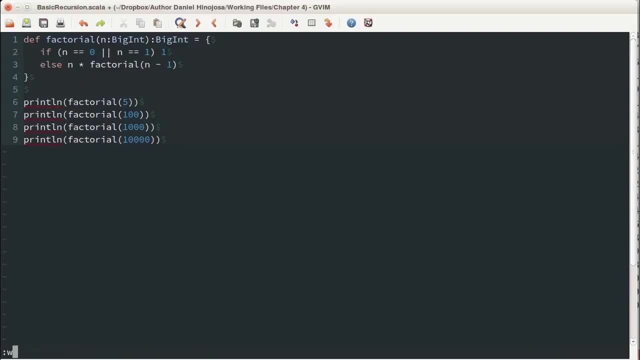 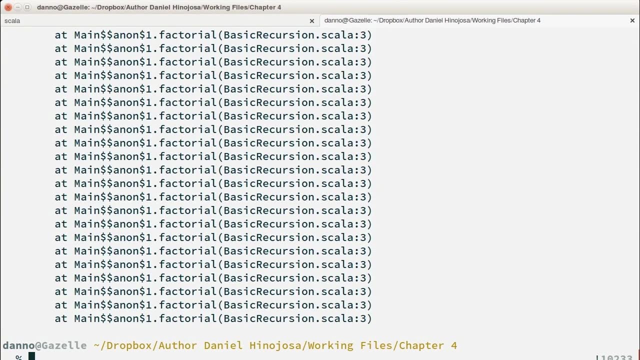 let's give it even something harder to work on. let's go back to the editor and kablooey. at some point we blew the stack. recursion only goes so far. before the stack that handles the recursion blows up, you could adjust the stack at the command. 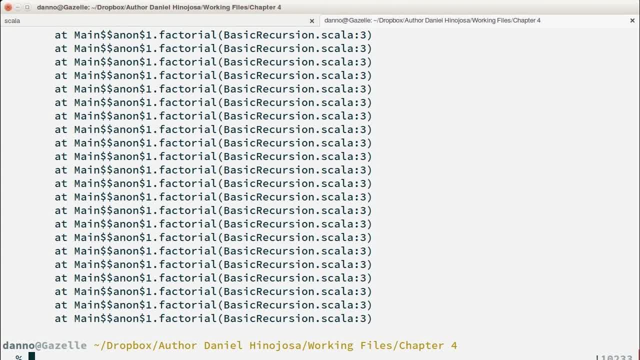 line for the size of the stack. but that is unnecessary because we have another strategy. we'll rewrite this in something called a tail recursive optimization in the next session. let's see if we can scroll up. it could very well be that we aren't going to be able to see the first. 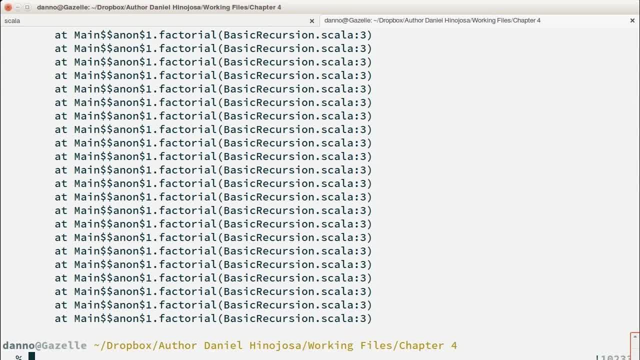 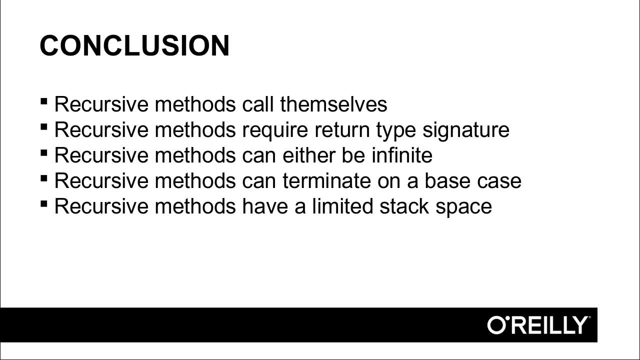 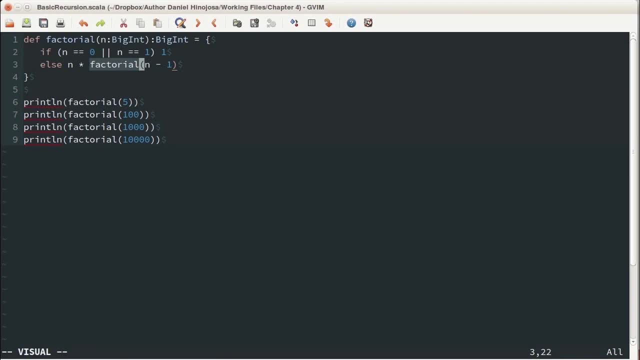 part of this error, but it is a stack overflow exception. so, in conclusion, methods can be recursive and call themselves. let's take a look at that again. it's worth looking at this again. right here is where the recursion happened. we're calling factorial, but with a different number. 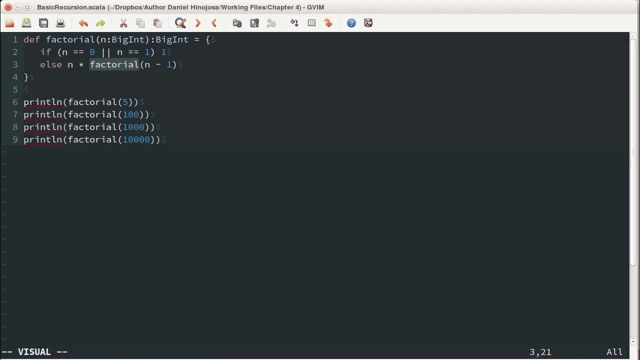 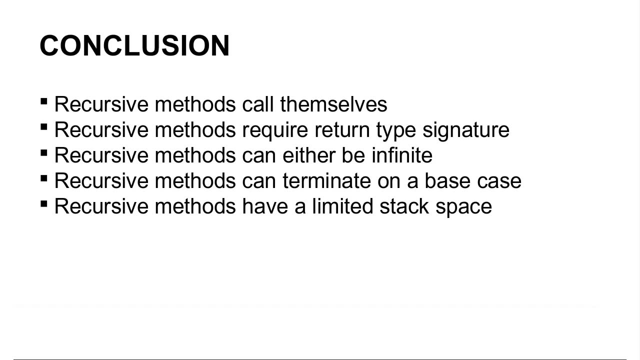 we're subtracting 1 from it, but this is a method calling itself, so recursive methods call themselves. they require the return type in the method: signature. recursive methods can be infinite if written correctly, or have a base case where everything stops. recursive methods have so much stack to use before it blows up. 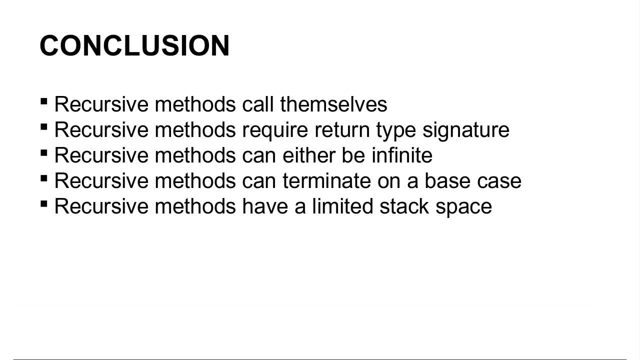 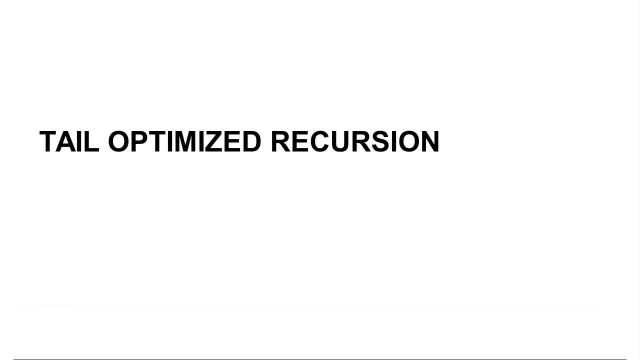 there is only a limited amount of space and you may need to reconsider the decision to use tail recursive calls. in our last session recursion, we created a method called factorial. if you're just joining this session, a la carte review the last session. what we'll be doing in this session is: 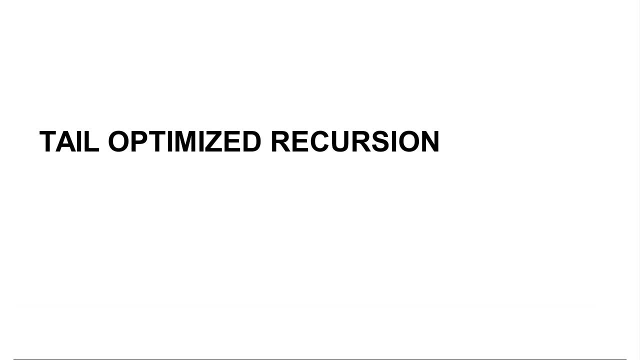 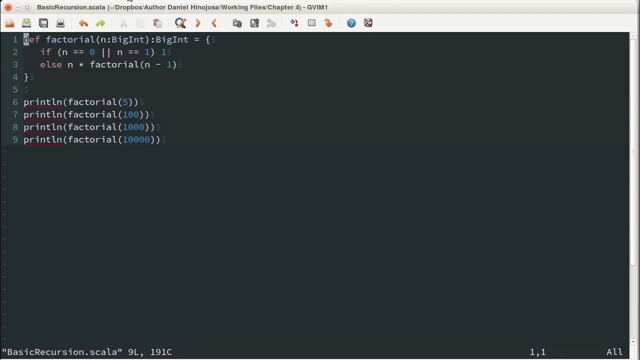 redesigning the factorial method to be a tail recursive method. let's go back to the file called basic recursion dot scala. it almost worked well until we called it with a fairly large number like 10,000. if you recall, phi worked out really well initially. we had problems with 100 and 1000. 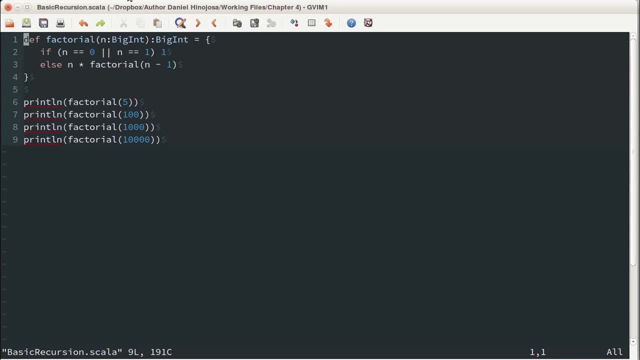 mostly because we were just dealing with int, and int only has limited size to work with, so what we had to do was beef that up to a big int, which is an object that stores more information and represents an integer. now, what I'd like to do is save this. 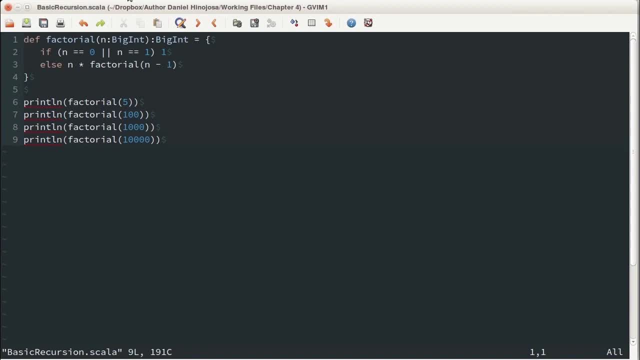 file as another file called tail. call recursion dot scala and open that file so we can make changes. ok, everything's saved. now, before we begin, there's an annotation we can use, called scala annotation- tail. rec annotation is a metadata that the compiler uses so that we can 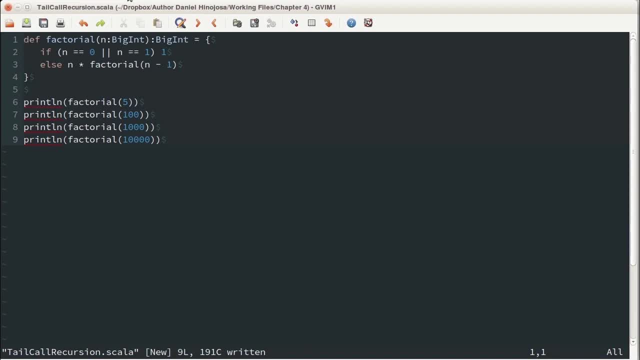 change the way the code is compiled or used at run time. annotations will not have any direct effect on how the code operates. so let's get started. here's the at annotation: scala dot annotation. dot tail rec. the scala dot annotation. you see, there is a package packages. 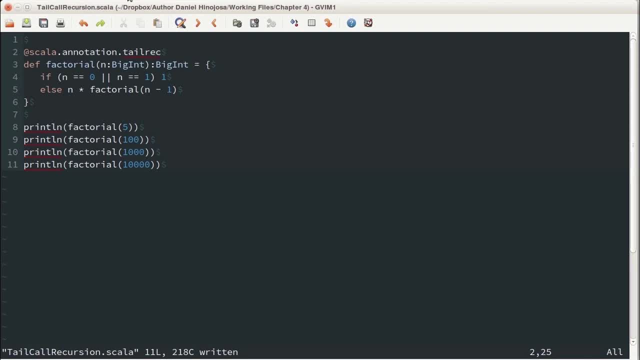 for those who don't have a java background, are addresses of the class, much like the addresses of your home or place of business. in other languages, like ruby or haskell, they're called modules, typically in the jvm world they are the reverse domain name of the company or 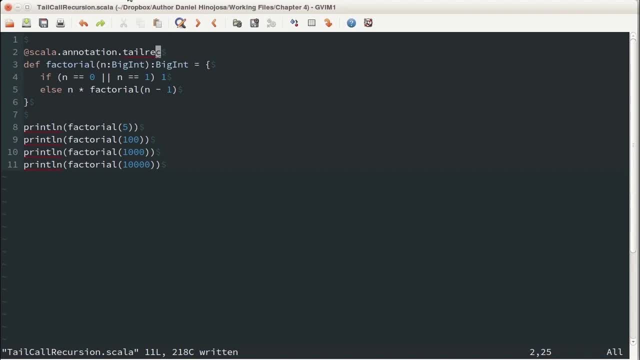 entity that created the code. if you work for a company called xyz corp, for example, then the package would likely be called com xyz corp. if you work on a project called project a at the xyz corp company, then a possible package would be com xyz corp, project a. 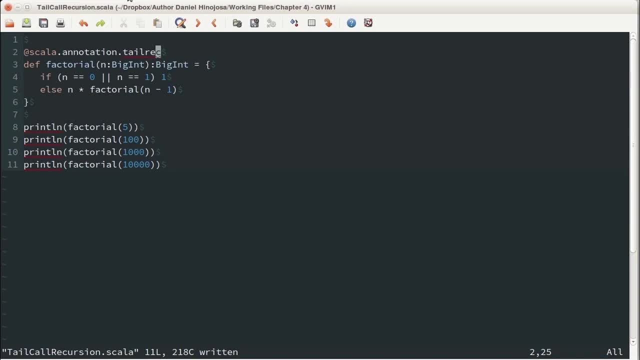 at compilation packages are made into folders where the class or, in this case, the annotation would be called in scala. all constructs are a member of the scala package, either directly or indirectly. the full name for scala annotation, tail rec, is called the fully qualified name of the annotation. 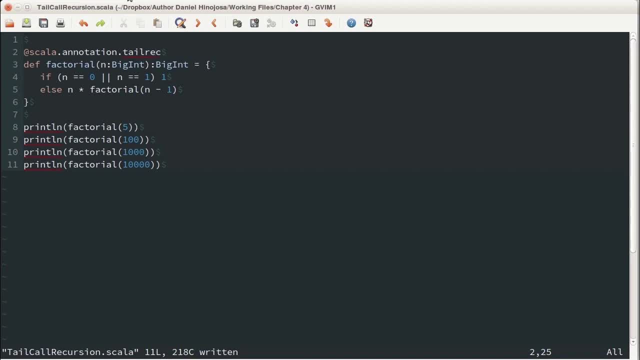 if we don't want to include the fully qualified name of the annotation above the method, we could import the annotation so that we just call the annotation name without including the entire package. so let's go ahead and do that now when we try to compile this or run it, since it is a 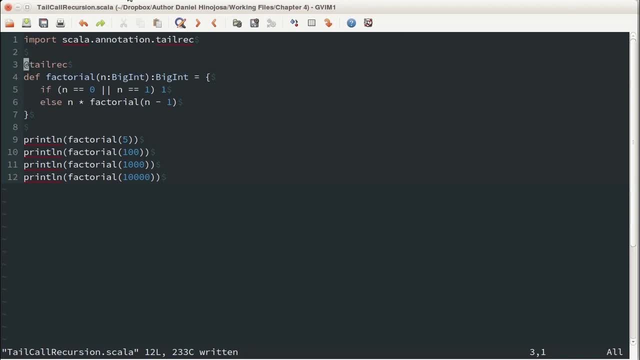 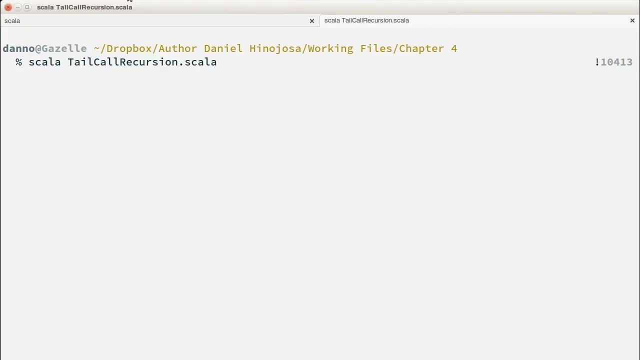 script we get to see what a nice, handy utility the at tail rec is. it's going to tell us that this code does not meet a requirement. let's give it a try. it tells us that this code is not tail recursive. to make this tail recursive, we need to ensure that after: 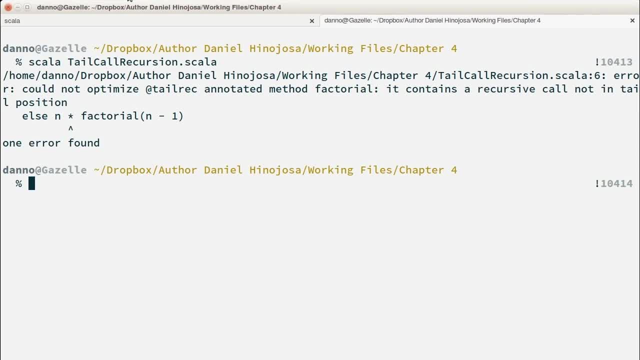 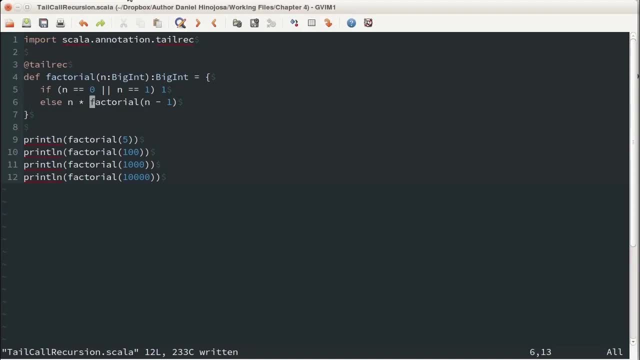 the recursive call has been made that there are no further operations on what has been returned, we obviously violate this rule. let's go back to the code and take a look. we violate this rule because we are calling factorial and right after we're calling factorial, we are multiplying. 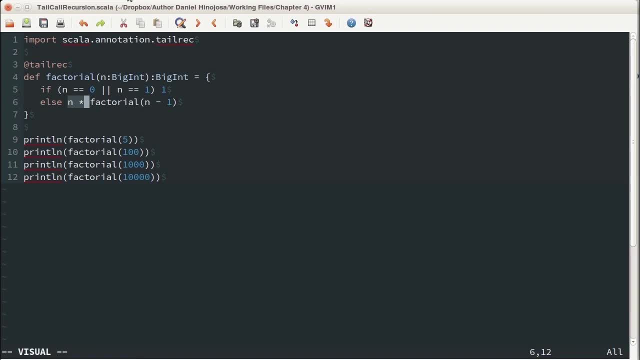 we're doing an operation after the factorial is returned. we have to make sure that whatever factorial returns is immediately returned from the method. we can do this with an accumulator. an accumulator is an object that will hold the running total, in this case the running factorial, with each recursive iteration. 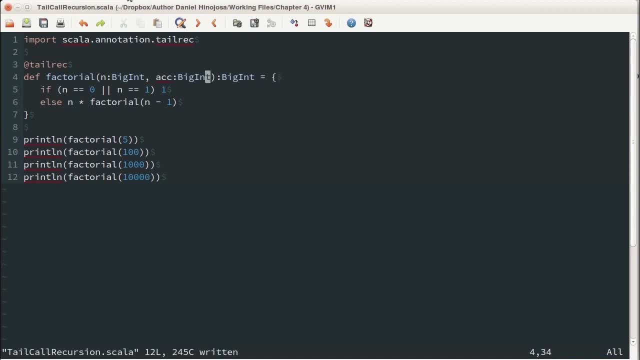 so let's change this code around. so I'm going to add the accumulator. this is an accumulator that has a big int type in our base case, whether n is 0 or 1, what I'd like to do is, instead of returning 1, I would like to return the. 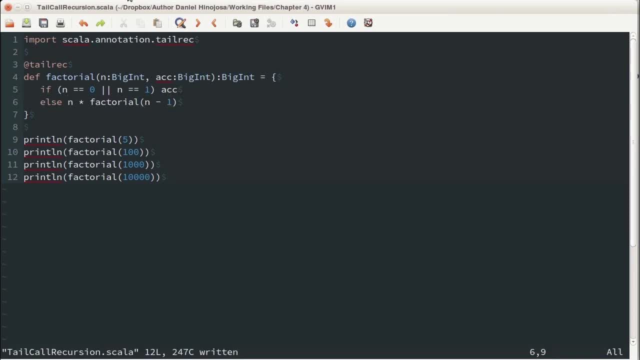 accumulator. now, when I call factorial, I am going to get rid of the n star, because we want to make this tail call recursive, and what I'd like to do here is multiply the accumulator by n. since we made changes to the method parameters, we also need to make 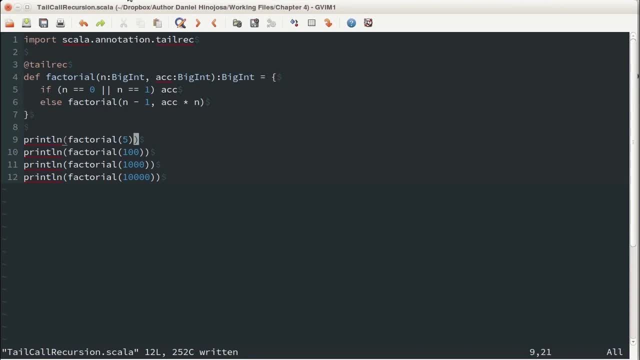 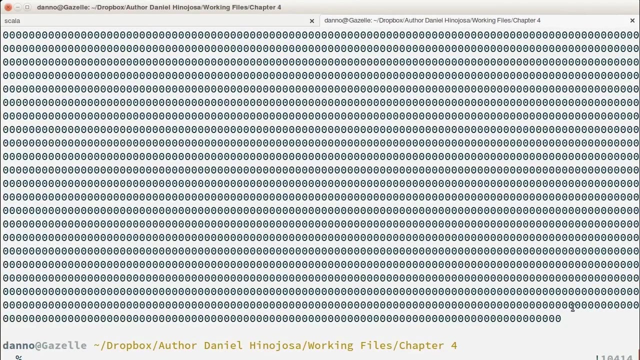 change on how the factorial method is invoked. now that factorial requires two parameters, I need to make sure that there is a second parameter to each one. with those simple changes, we can run the script and see what happens. this works. let's take a look. the bottom one right here is: 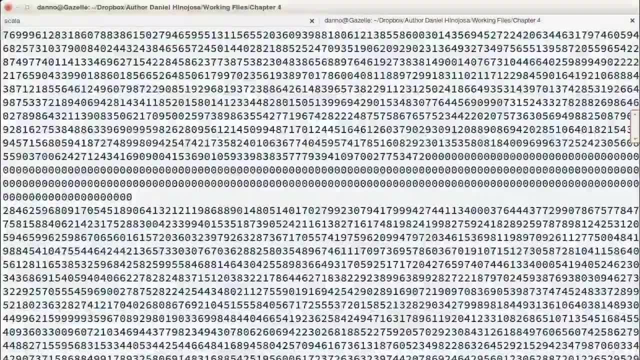 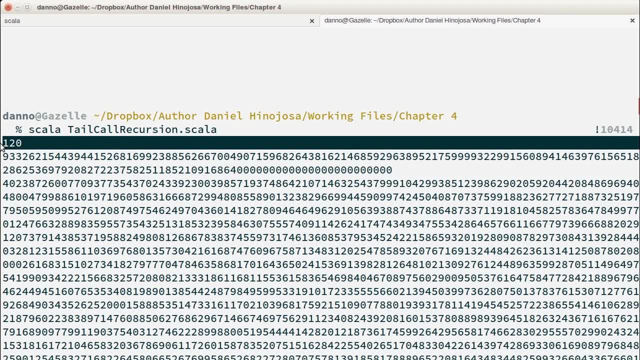 the factorial for 10,000- pretty big number. here's the factorial for 1,000, here it is for 100 and here it is for 5. this works and this is just another way to look at the same problem. what happened? let's take a look. 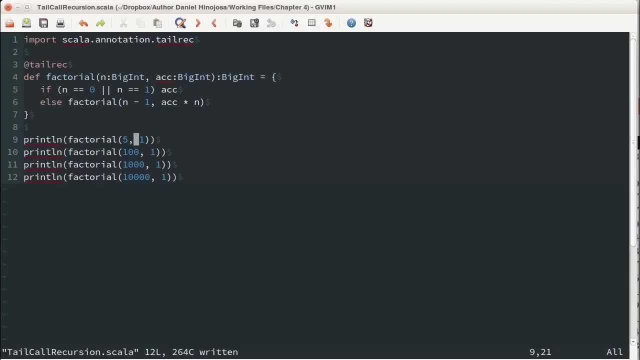 back at the code. this is a compile time trick. if your recursion is modeled in a tail recursive way, then the Scala compile will optimize the code for you in a loop so that the stack is rarely filled. this process has an acronym: TCO or tail call optimization. 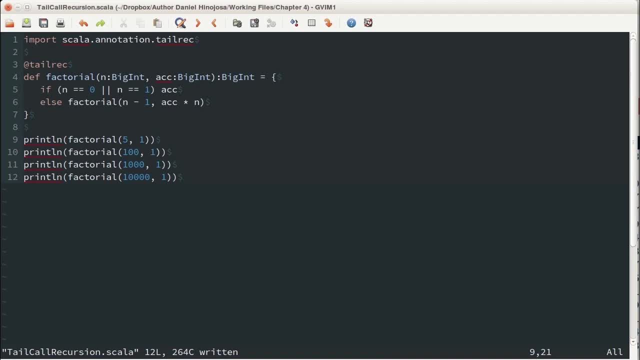 of course, one problem that we have is that we have to keep calling our factorial method with 1 every time we want to call it. in other words, we have this 1, this 1, this number 1 and this number 1. let's create a method that. 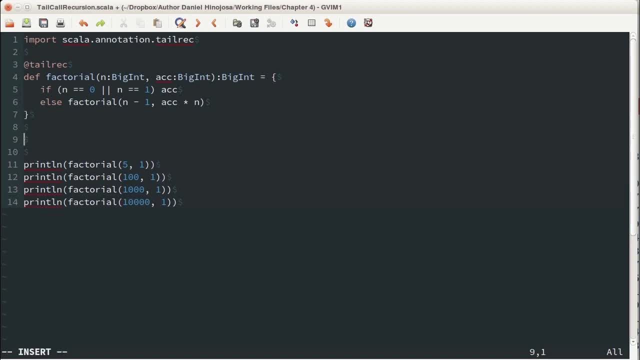 does this for us, so that we don't have to call it over and over again with the number 1. in order to do that, I'm going to change the factorial to a method name called fact. that way, the main method that we usually interact with will still be called. 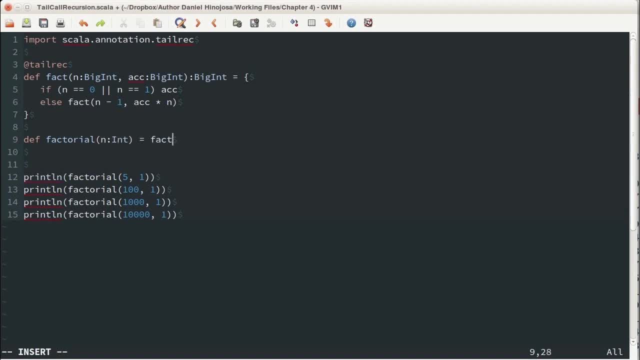 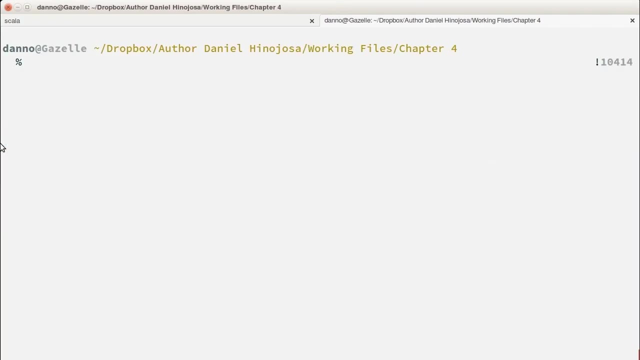 factorial. factorial will bring in a number and when we call that number, we will then call the method with that number and the number 1. now we can get rid of the 1's. let's run it and make sure all this works. looks great, we have our 10,000. 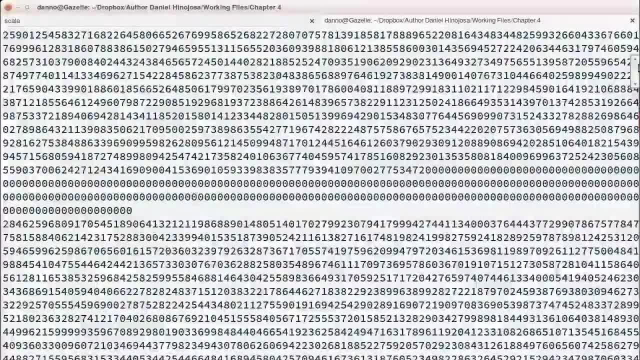 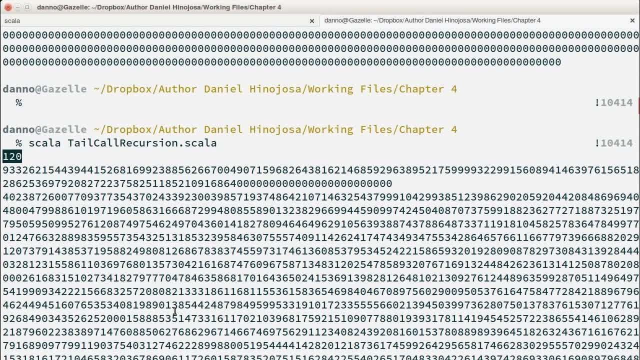 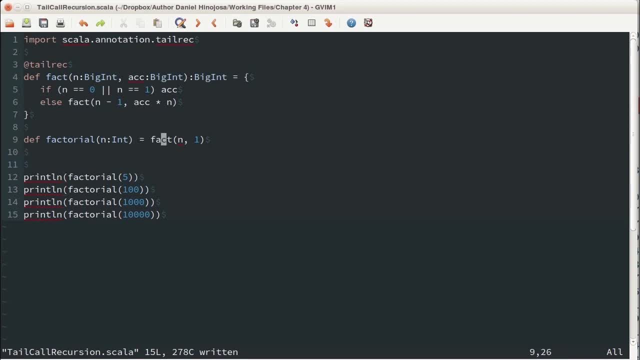 again. here's our 1000 coming up here soon. there's the 1000, there's the factorial for 100 and finally the factorial for 5. looks great, let's review the code. so we have our factorial method that brings in an int and we call fact. 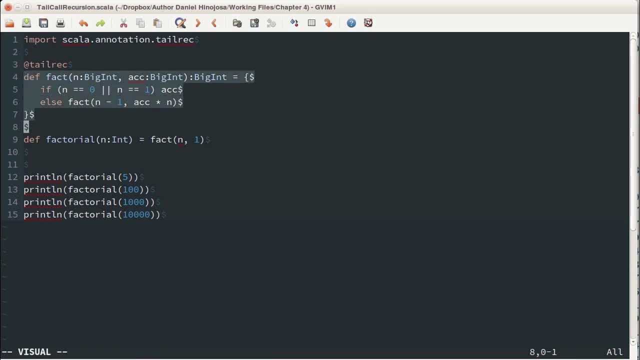 now up here under fact. here's the method fact. this is our recursive call. we refactored it to make it a tail recursive call. there are no operations being made on this method after it returns. and here is the tail rec annotation. in the next section we'll do some other. 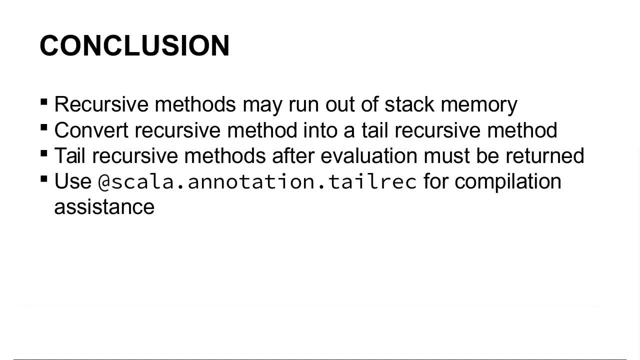 refactoring by putting one method into another. if your recursive method continually makes calls to themselves, they may run out of stack memory. a strategy you could use is to convert your recursive method into a tail recursive method. the recursive method, after being evaluated, must immediately be returned. and finally, a conclusion: you could also 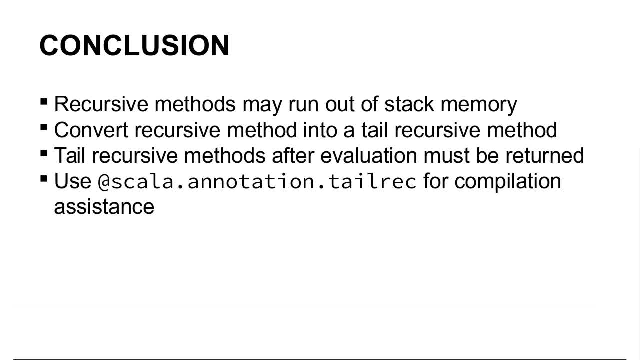 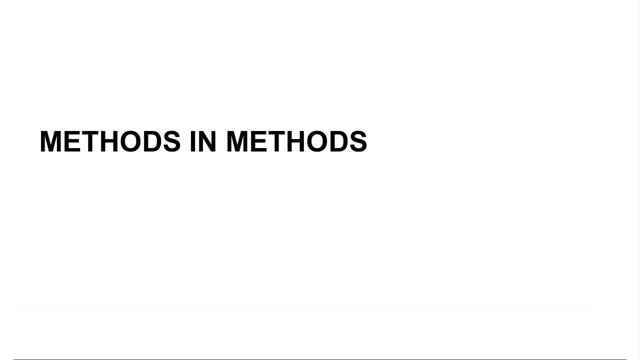 use an at tail rec annotation from the Scala annotation package for any compilation assistance into making sure that your method is indeed tail recursive. in our last session we have a tail recursive method called fact and that is used by another method called factorial. fact is our tail recursive call. 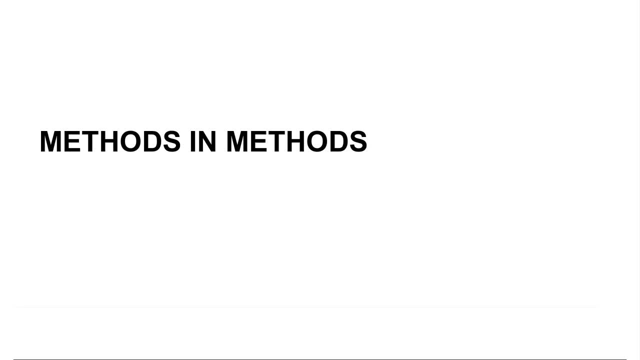 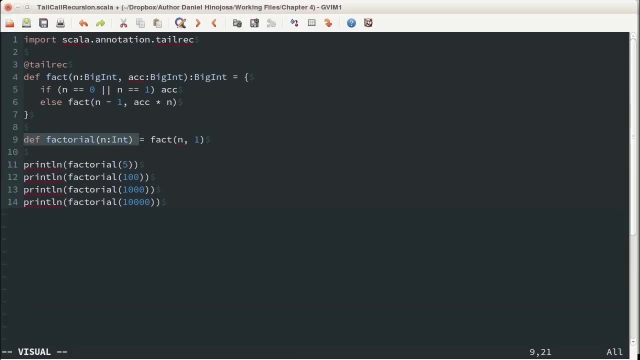 and all this was in a file called tail call recursion dot Scala. let's open that up and review. so here's that factorial method that I was referring to about. this brings in an int. we take that int and we call the method fact once we call the. 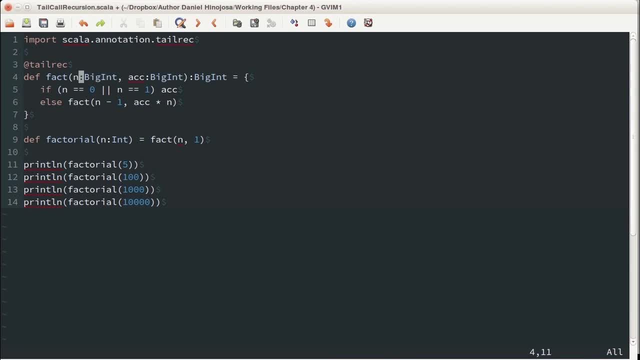 method. fact: we have the number that we wish to get a factorial of and we have an accumulator that is going to keep our running total. for us, if n is zero or n is one, the base case will state that we will just return whatever has been accumulated up to this point. 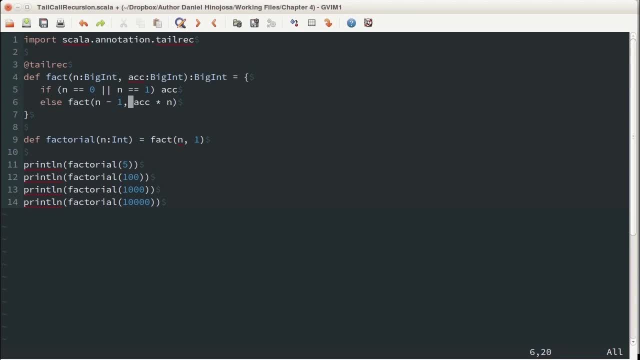 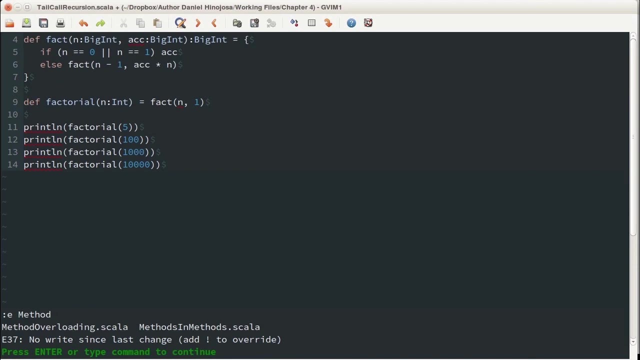 otherwise we will deduct one from n, and for each succession we will multiply the accumulator times n. so what I'd like to do is refactor this a little bit and I'm going to save this into a file called methods in methods dot Scala, a feature that I 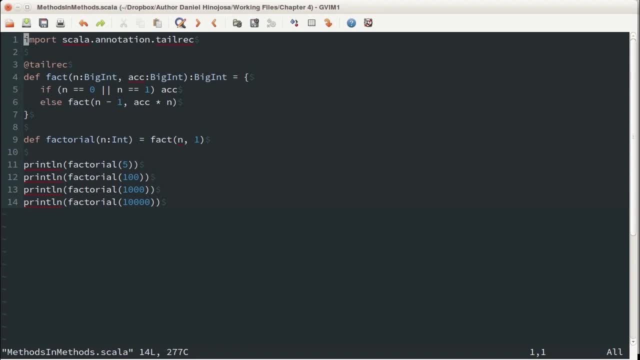 really like about Scala is the ability to take a method and shove it into another method. use case would be: if you have a method that says purely with one method and nothing else, one such method would be our fact method, it is not needed anywhere else and all the interaction. 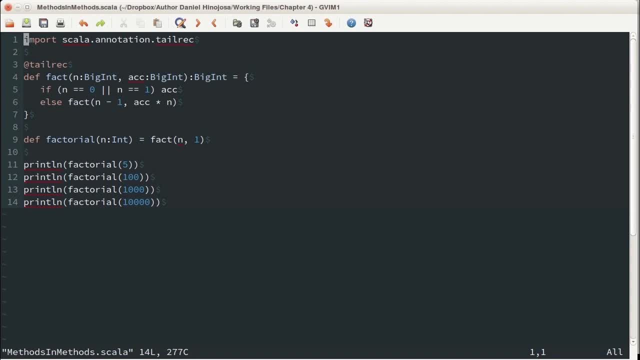 can be done by our factorial method, since that is the public interface, so let's try that. okay, did some clean up along the way, and what we did is we took one method inside of another method. again, factorial is going to be the public face in all this. the 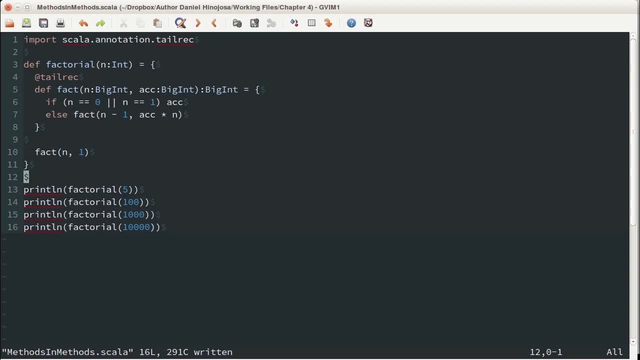 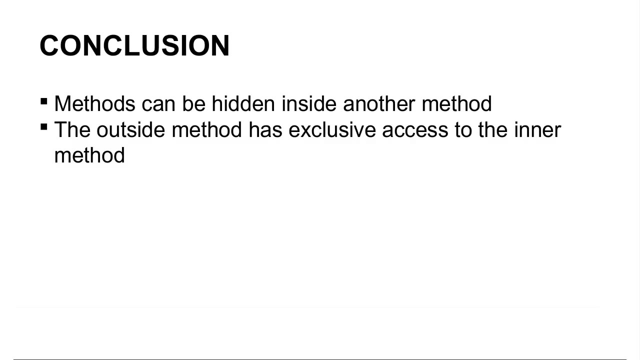 fact, can be hidden away inside of another method. it looks great, everything in its place. so this may be a feature that, for the Java programmer, you'll not see in the Java programming language, but this makes things a lot cleaner. so, in conclusion, methods in Scala can be hidden inside of another. 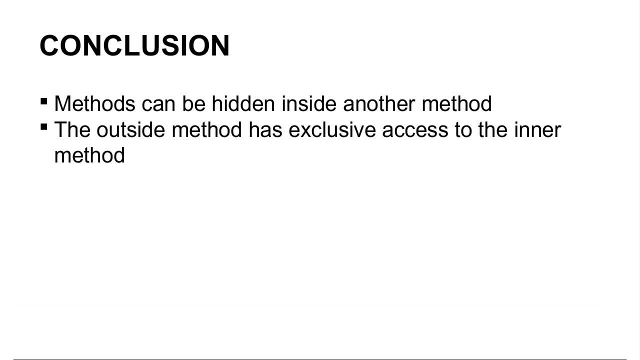 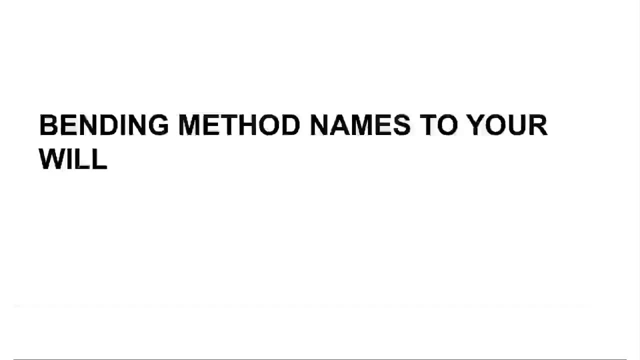 method use case would be: the method inside does not interact with the outside world and it is only for exclusive access to that inner method. in a previous session, bending val and var to your file, we created some values and variables with some nifty tricks that allow us to express ourselves when it. 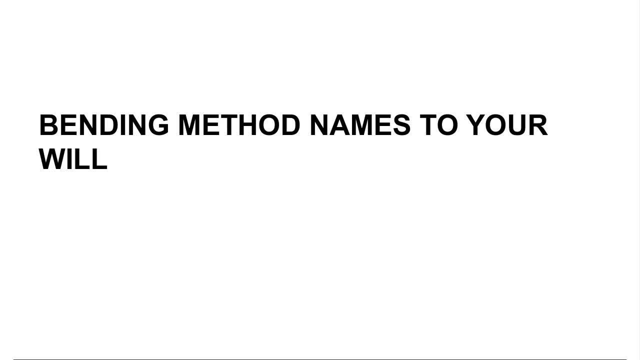 came to naming. we can take those tricks and apply them to methods. now, much like val's and var's, we also have spaces and other what are called opchar, or operational character codes in a method if the method name is surrounded by a back tick. now, if you need a reminder before we do, 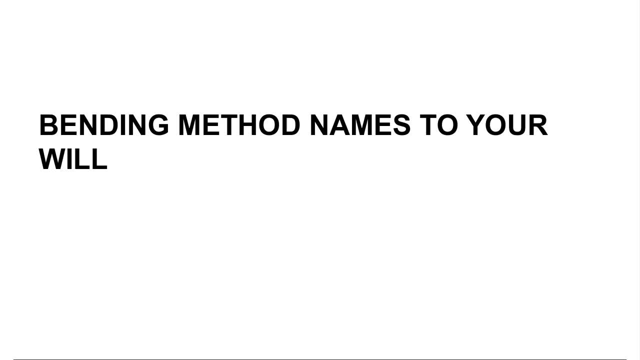 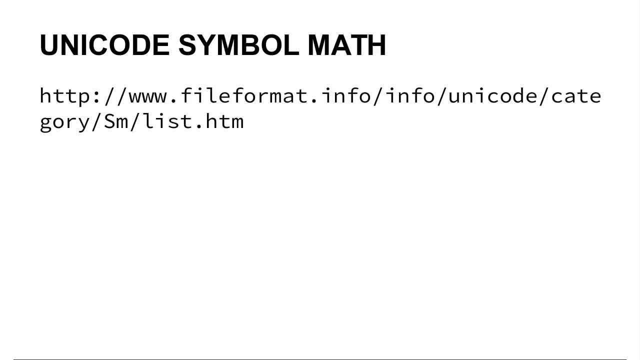 this what an operational character is or an opchar is. there are a few links you can visit. this is from unicodeorg, so a valid operational character is a unicode character from u0020 to u007f. you could also include unicode symbol math, and here's the. 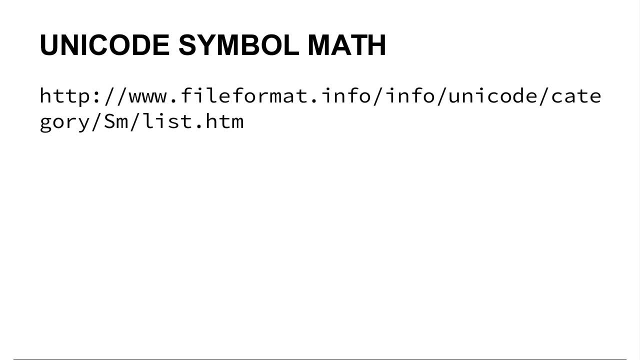 category. visit this website to see all the unicode characters under the unicode symbol of math and here is the url for unicode symbol for other. so these characters are legitimate operational characters as well. so let's go to repl and try some of these out. so let's say, i want to create a 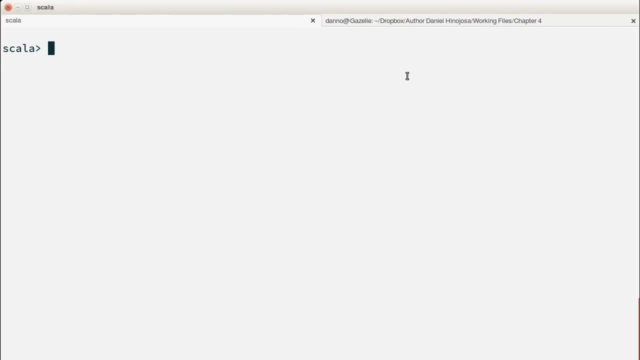 method called summation of, and let's say i want to have a space between the words summation and of. here's the method. there's the method name: summation of between two back ticks. the reason for this is because i have a space between summation and of. 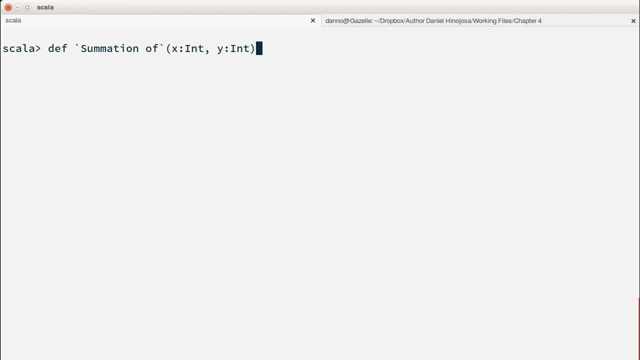 i'm bringing in two parameters, both are ints, one's called x, one's called y, and, as part of my implementation for this method, i'm just going to add them together. now i need to call it. so i cannot call it like this. it's not going to know. 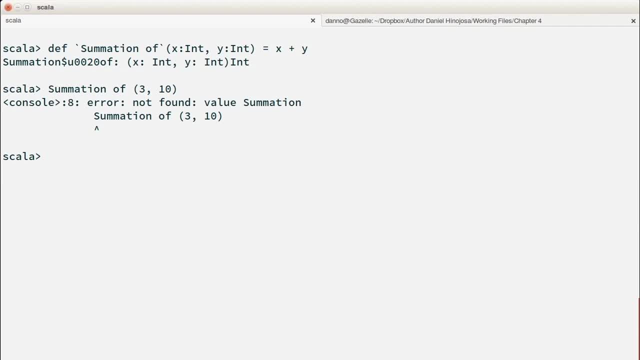 where summation is, so use the of there, but it's going to interpret it as there's an object called summation that has a method called of. so that's not going to work out. so if we want to call it, then we'd have to include the back. 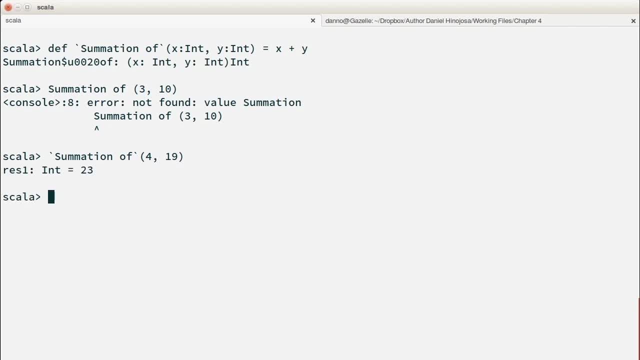 ticks. now, if you also recall, we have an underscore and anything after the underscore could also be an operational character. let's try a sample of that. i'm going to hit control l to clear out my repl. i like to create a method, this time called are we liking scala? 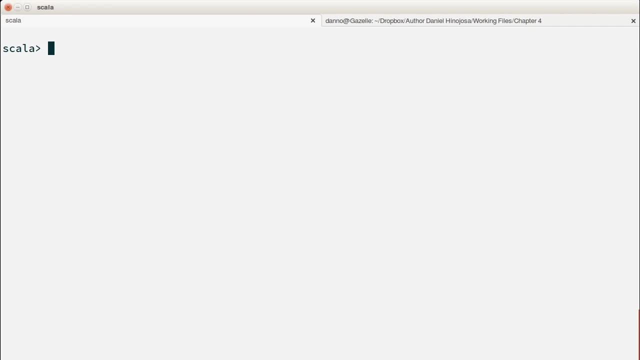 with a question mark at the end. now, in the java programming language a question mark is not allowed as part of the method, but in scala we can. but as long as we establish the underscore first, then we can use the question mark. so this is being interpreted, as are we. 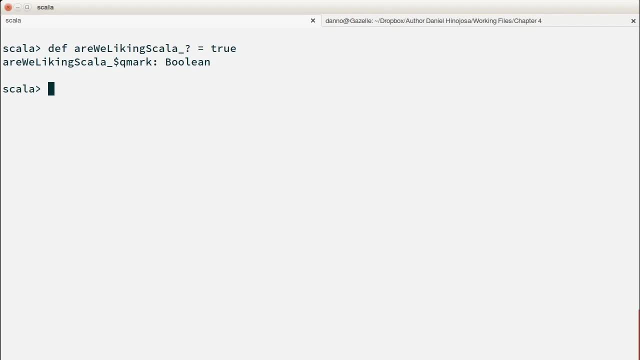 liking scala. underscore. dollar sign. q mark. as you see here, this is a method, a method that doesn't take any kind of parameter, but it is returning something, and in this case it is a boolean of true. it looks like a val or a var, but it really is a method. 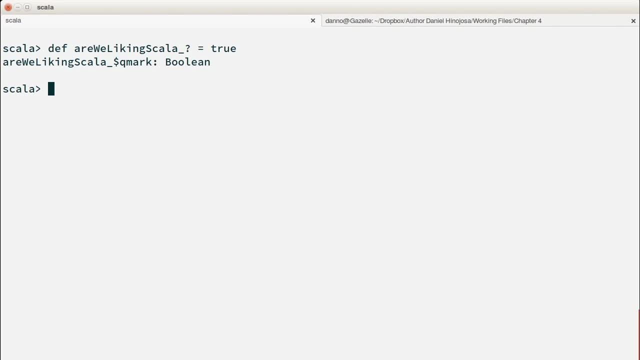 and at the java bytecode level, it is going to be considered a method. given that this is a method, we can attach this to a status, so we're using. are we liking scala as a method? the method is going to return a boolean, placing it in an if clause and 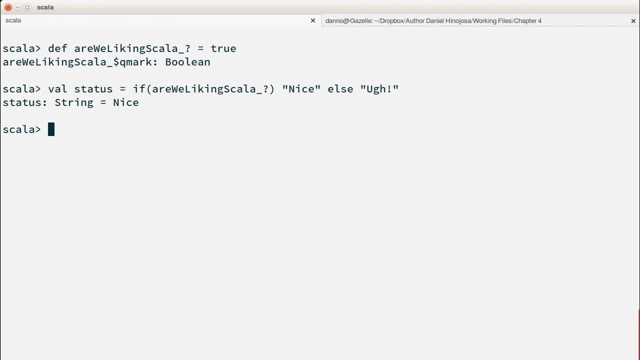 if it is true, then we'll return nice, otherwise we'll return a. of course, we'd be remiss if we forgot to mention that if you want to make a reserved word and method name, you could do so, albeit it may be doing yourself and your team a disservice. 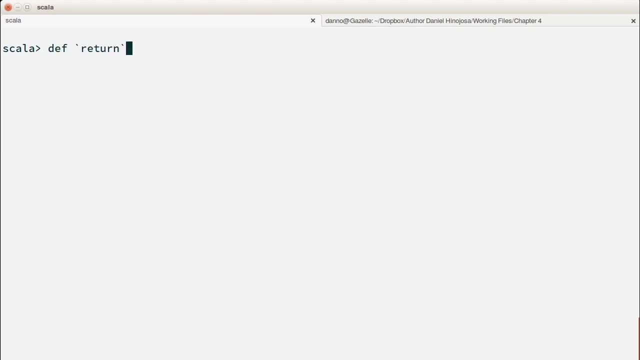 but let's give it a try. obviously, in this case, i'm going to create a method called return, but obviously this is a reserved word in both the java programming language and in the scala programming language. so let's say, i'm going to be careless, i'm going to use a reserved word for 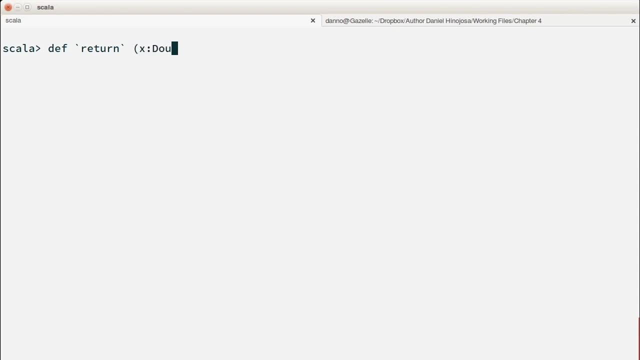 a method and this is going to take two doubles. once we bring in these two doubles, i am going to take these two doubles and, let's say, add 4.0 and convert it to a string. so there's the method, name, called return. if i wanted to, 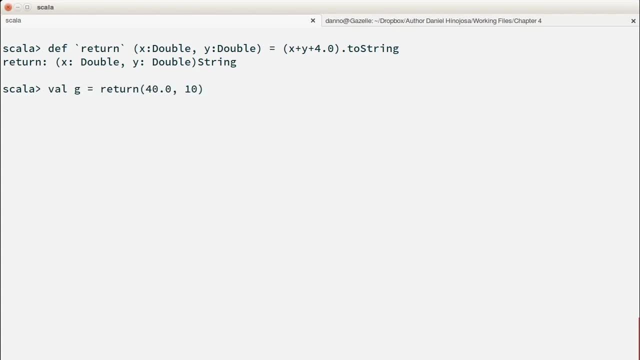 make use of it. obviously, doing this may not work because scala still sees return as a reserved word. so if i want to call the function instead of having it interpret as a reserved word, i would need to surround that with backticks. so, in conclusion, methods can have: 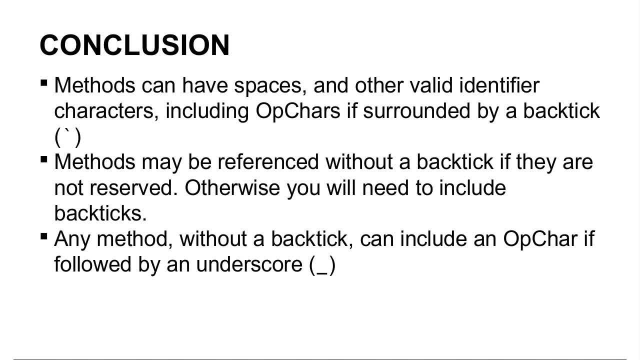 spaces and other valid identifier characters, including operational characters, if they are surrounded by a backtick. methods may be referenced without a backtick if they are not reserved or due to not contain any spaces. otherwise, we'll need to include the backticks. any method without a backtick can include: 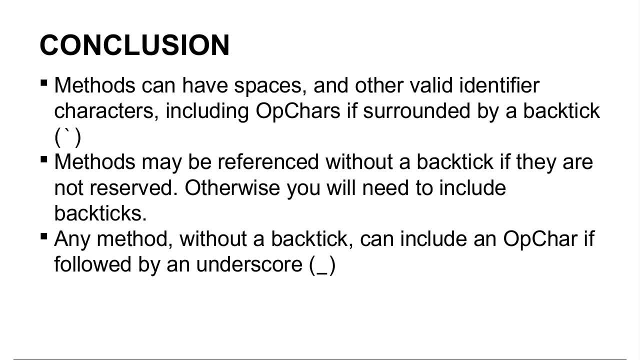 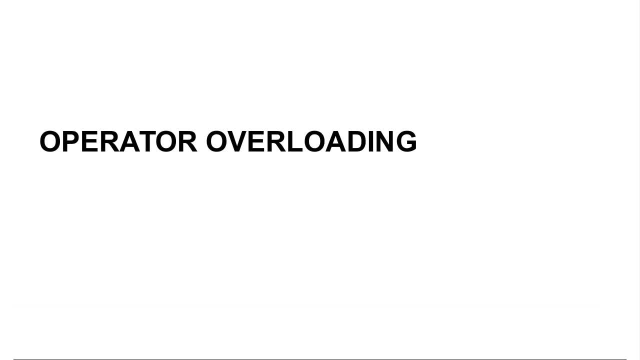 an operational character if followed by an underscore. in this session we will discuss operator overloading. as in languages like c++, operator overloading gives us the power to name our own methods as operators like plus, minus, multiply or asterisk, or slash for divide. this power comes also with scala, but 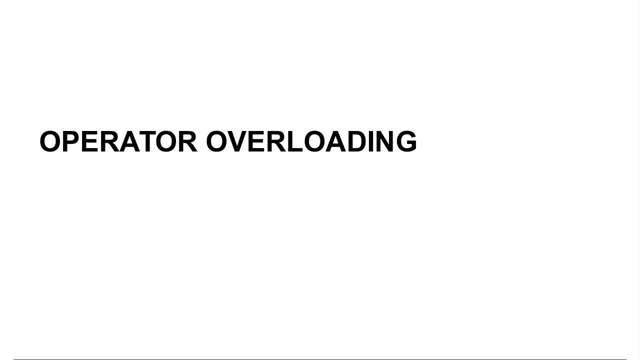 be warned: with great power comes great responsibility. operator overloading should semantically make sense to your domain, typically without having to look up its meaning. so let's go to repl and give this a try. all right, here we are in the repl, and let's say i want to create a method. 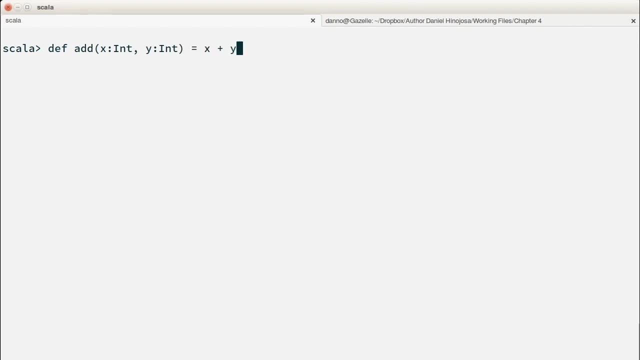 called add. done this method over and over, so that works out fine and of course, we can just call add with it. but what if, instead of add, i wanted to call it plus? i can do so now. there are better ways to go about this, like using an infix method. 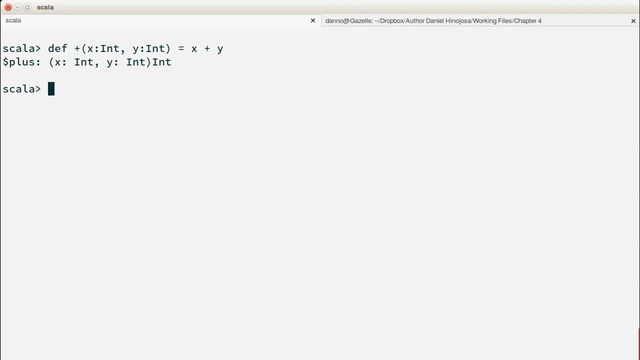 which we'll cover a little bit later, but as it is currently, this works. we know what plus is, we know the semantic meaning of it and we can intuitively make sense of what it is. i also brought this into repl for a reason, because we get to see the type. 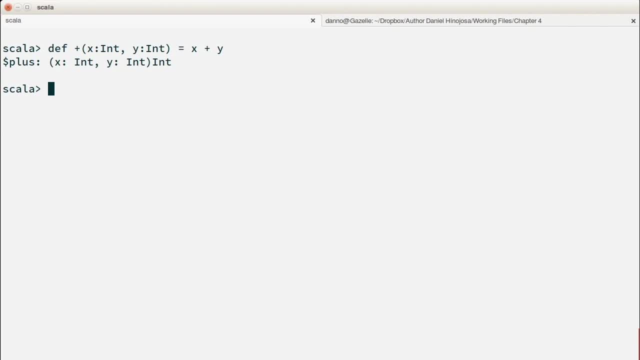 and here's the type signature of the method. see that: dollar sign plus the plus is actually the name of the method. internally to you, the programmer is just the plus sign, but internally it's called dollar sign plus. let's take a look at another example. this works, but this is just me. 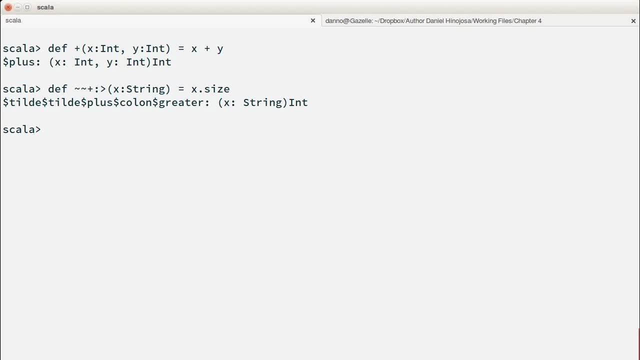 semantically it doesn't make much sense. no intuition can help, and try looking this up on a google, yahoo or bing. when someone wants to try to know what this is, this is invocable, but again, this is something that's really hard to look up. so what can we use? 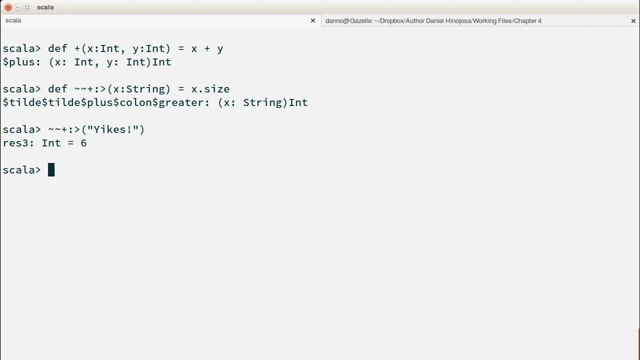 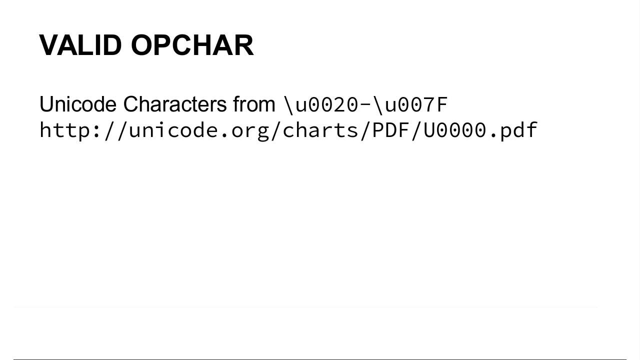 well, we could use all the operational characters, or obchars, as method names. and here again, just to jog your memory, are the references as to what obchars we can use again: unicodeorg. the unicode characters from 0020 to 007f are valid operational characters you could. 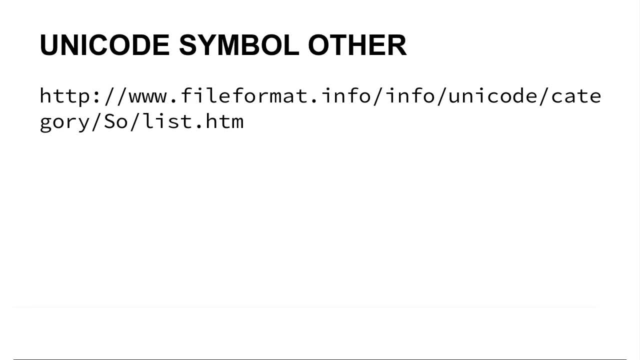 also use symbol math, and you could also use symbol other. any symbol that is listed on here can be used as an operational operator overload. by the way, did you know you are already using operator overloading? let's go back to the repl. let me hit control l. 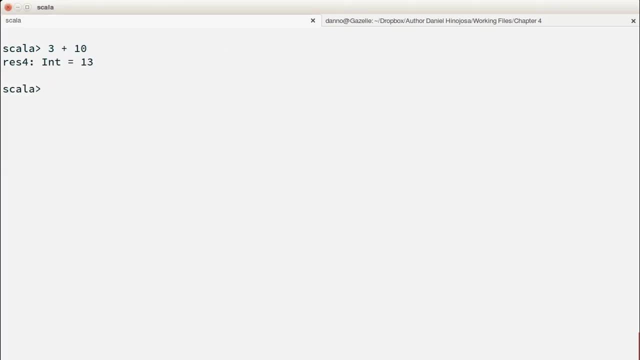 clear up the screen. remember this. it just seems like we're adding 3 to 10. but remember that we could treat all of scala as if it were an object oriented language. in other words, that means, from our point of view, we are using the plus method. remember. 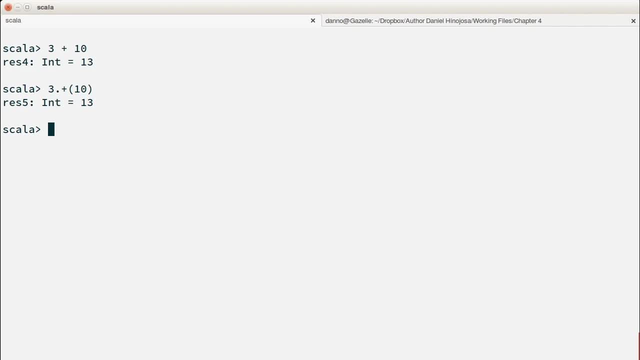 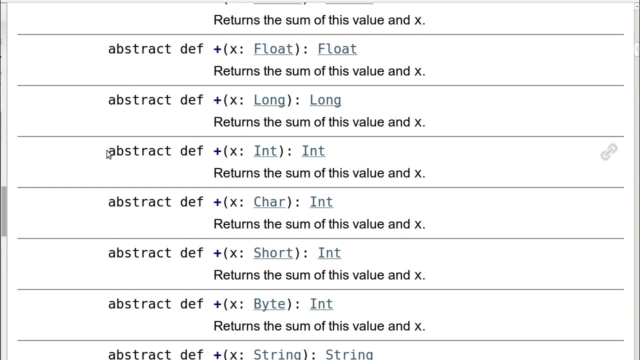 operator overloading plus method on the 3 object and calling it with 10 as the method parameter. in fact, this is listed in the scala documentation. here is scala int in the scala api. this is from scala int, from scala langorg api current. and here it is. this is a method. 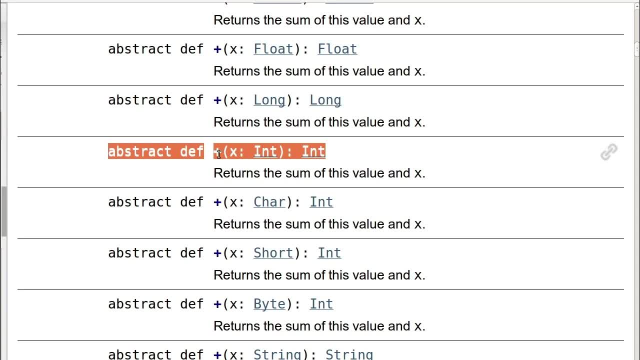 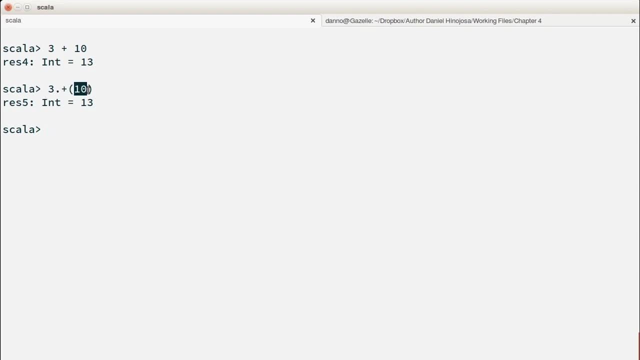 plus, which is inside of a class called int- we'll discuss classes shortly- and this takes a method parameter called int. again, the plus sign is a method. so let's go back to that repl, and here it is. int has a method call plus and we are merely invoking 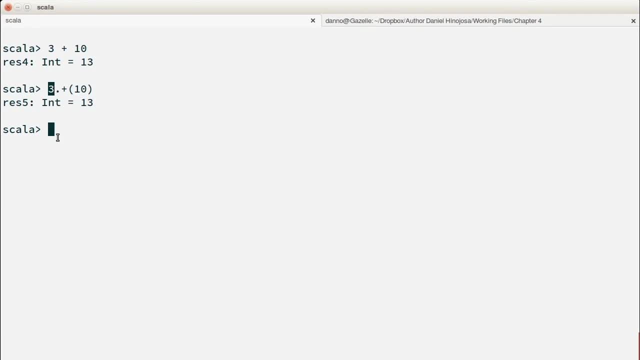 10 to the object 3. remember our recursion method that we completed and refactored in methods and methods. it was the factorial for a certain number. we used recursion and we put a method inside of a method. we also used tail rec and designed that using a tail recursive call. 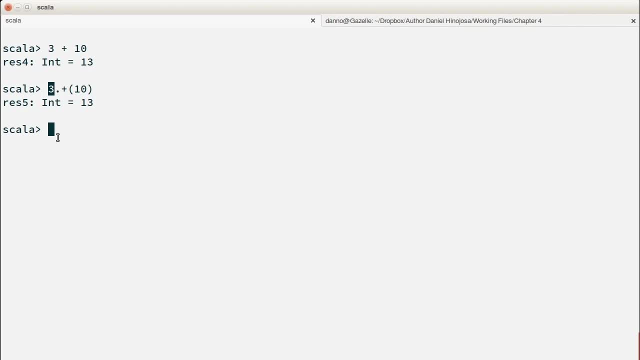 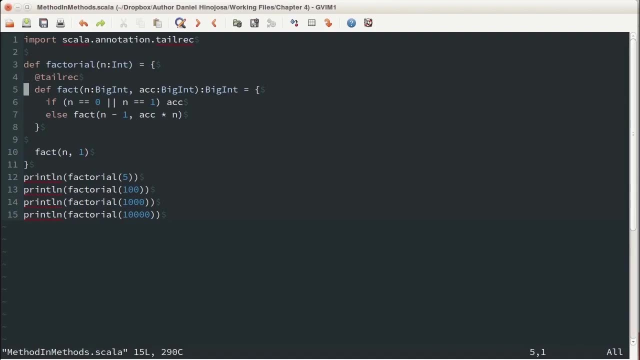 remember how we didn't have to do much when we changed from an int to a bigint. let's reacquaint ourselves with that file called methods in methods. here it is again. remember we had int before, but all I did was change it to a bigint. 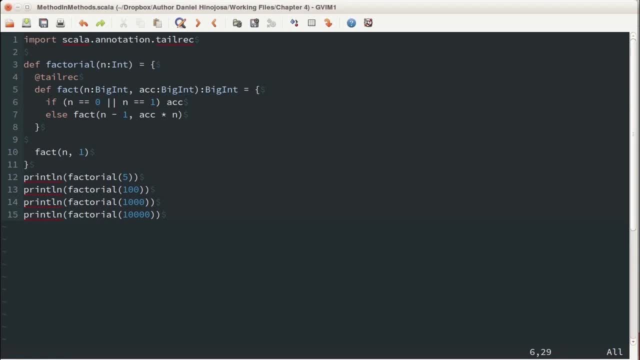 and, if you remember right, this didn't take much effort. I didn't have to change the method signatures, and the reason is bigint also has a plus operator, a star operator, a slash operator for division and subtraction, etc. the same methods that were in int were also in bigint. 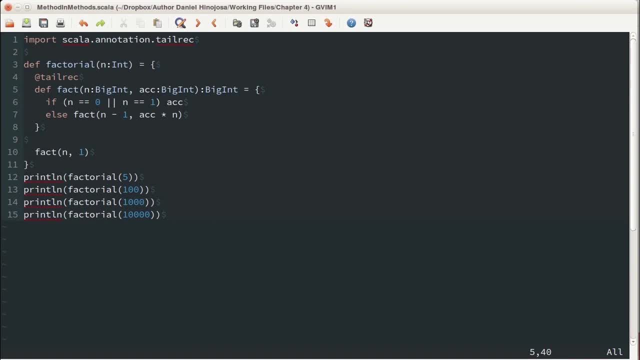 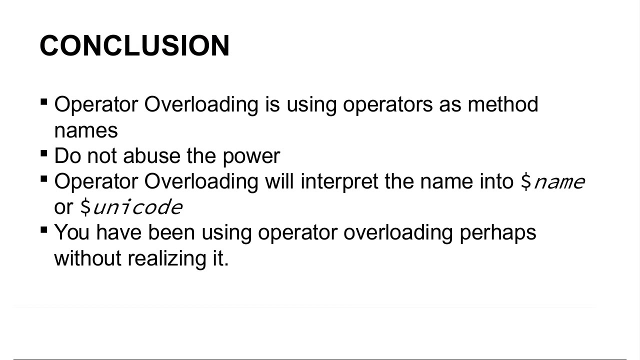 and that too was operator overloading. in other words, this minus right here happens to be the minus that is inside of bigint. the star right here happens to be the star that is inside of bigint. so, in conclusion, operator overloading allows us to use operators as method names. careful not to 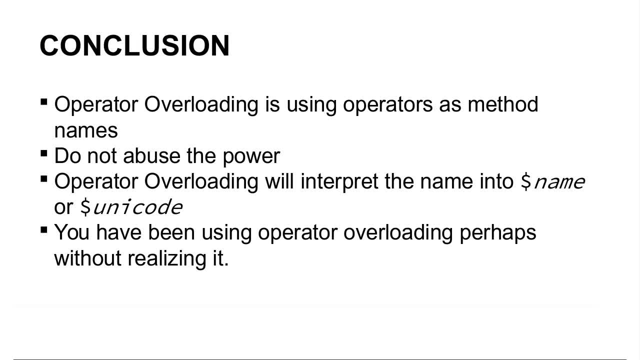 abuse this power, operator overloading will interpret the name into a dollar sign with a suffix, so dollar sign with a name or dollar sign with a particular unit code. and finally, you've been using operator overloading up to this point, probably without realizing it, in the case of int, in the case of double, 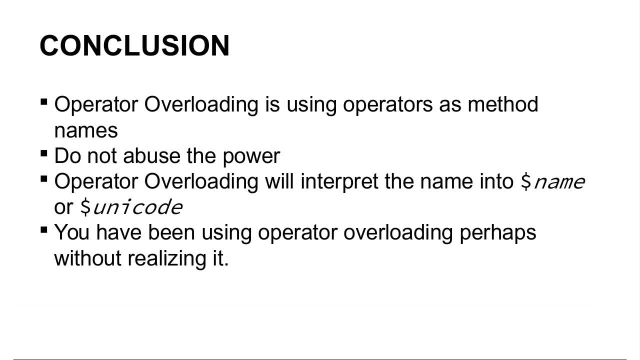 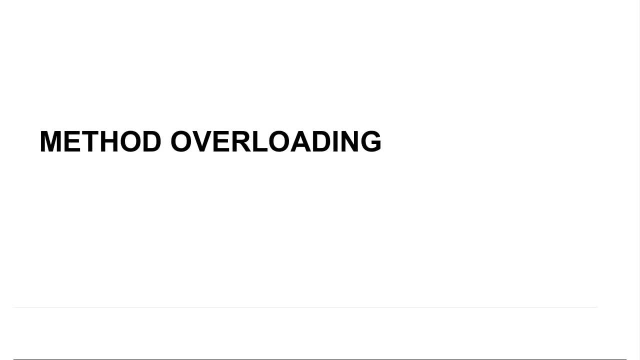 in the case of bigint, there are a lot of operators that are being used as an operator overload. in this session we will discuss method overloading. method overloading has the ability to use the same name for a method, though not law. you would typically do so if the method performs the 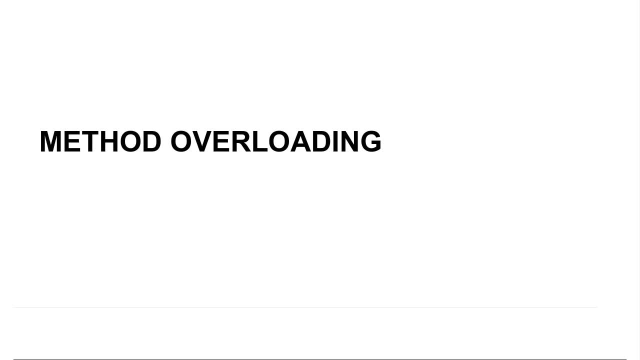 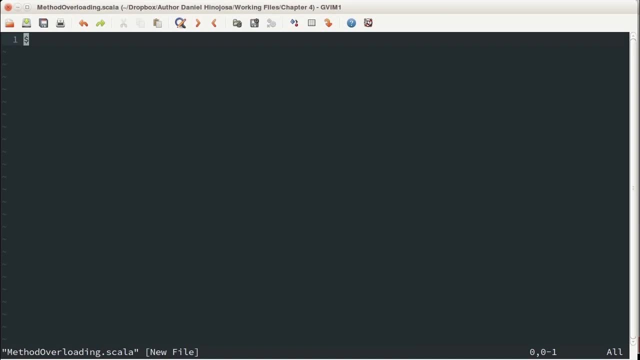 same operation, but with different types. so let's create a script called method overloading dot scala, to see how all this works. we created our file. now what I'm going to do is I'm going to create three different methods, all with the same name. here's the first one. 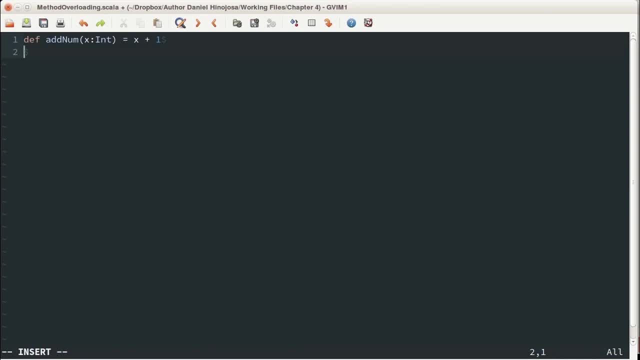 add num. this will bring in an int. once we take that int, which is an x, we're going to add one to it. okay, so we create three different methods. one will bring in an int, one will bring in a double and the other one will bring in a string. 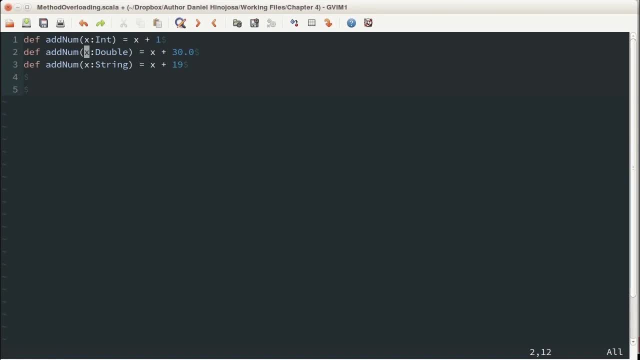 they all are called x. they don't need to be, in fact. why don't I just change that around so it's less confusing? it could be whatever you want to call it, and these are still overloaded methods. now I'm going to invoke these. let's create three print lines. 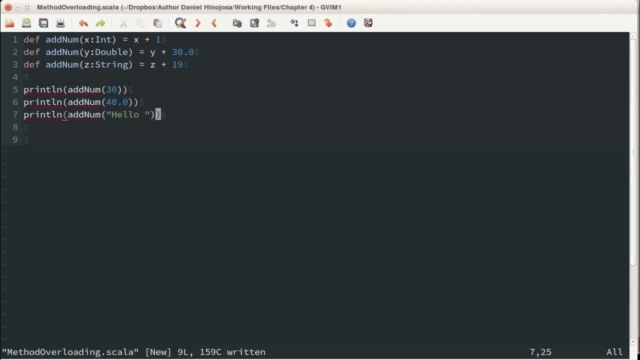 so I have three print lines. one will call with 30. that means the first one will be invoked. if I call the second one with 40.0, since 40.0 is of a double type, the add num, the second one on my line 2 will be: 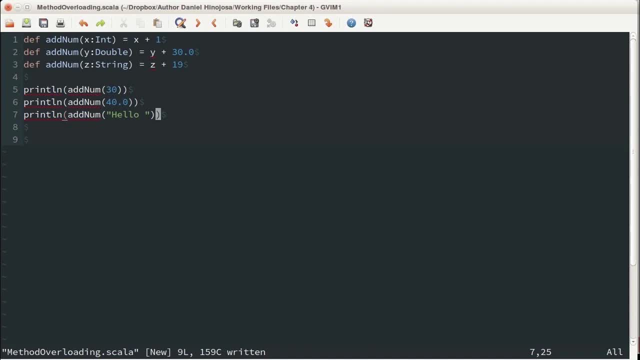 the one that's called. and for the third one, since I am invoking it with a string, the add num with a type of string is going to be the one that will get called. this is all based on types and it's all based on parameters. let's run. 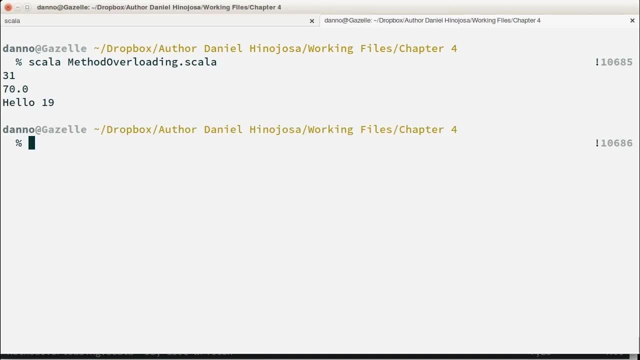 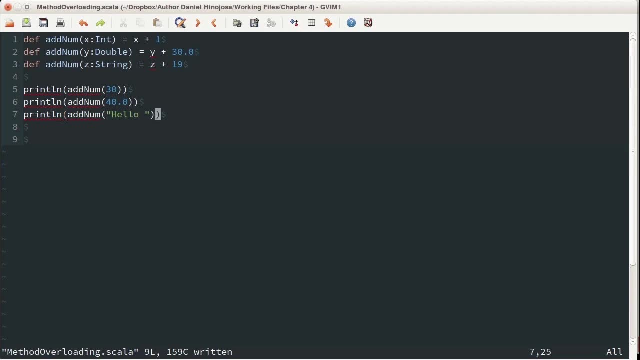 it and give it a try. we see here that it's 31. let's go back to the code and the reason it's 31. we're calling add num with a type of int and since 30 is of a type of int, the first method is the one that gets called. 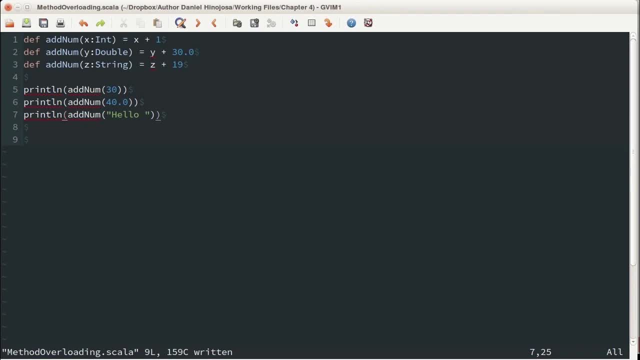 therefore, we're just going to add 1 to it. let's take a look at our second answer. our second answer is 70.0. let's go back, and the reason for that is that on our second call, we are calling 40.0, which is of a type double. 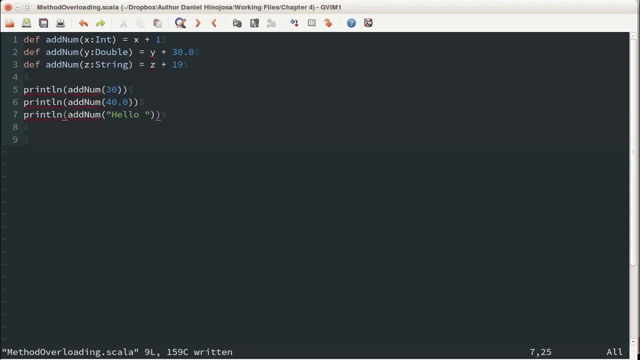 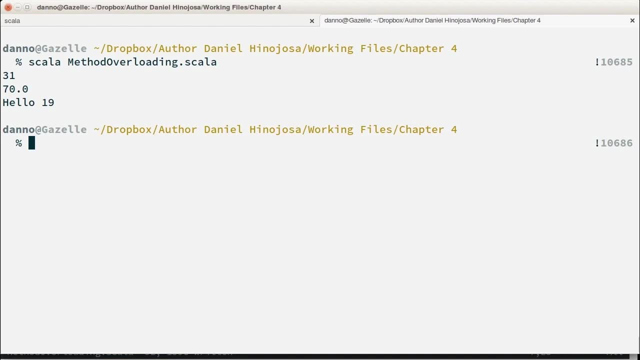 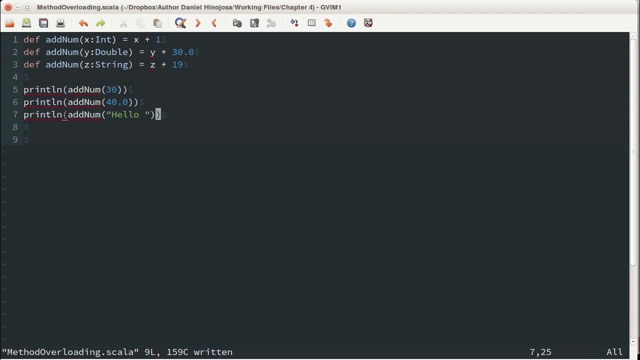 therefore, the second method on my line 2 is the one that gets invoked and we are adding 30 to it. let's go back. 31 says hello, 19 the reason: let's go back to the code. we are invoking it with a string now, coincidentally, I put this: 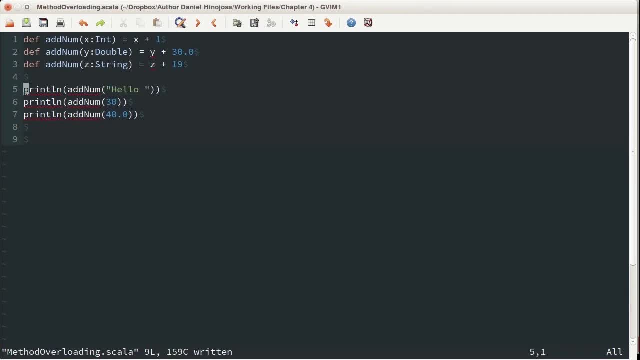 in order. but the order really doesn't matter, it's all based on type. again, as long as the method parameters are different, you could use the same method name each with different implementations. now, if the parameters are not different, the compiler will complain that the method names are ambiguous. 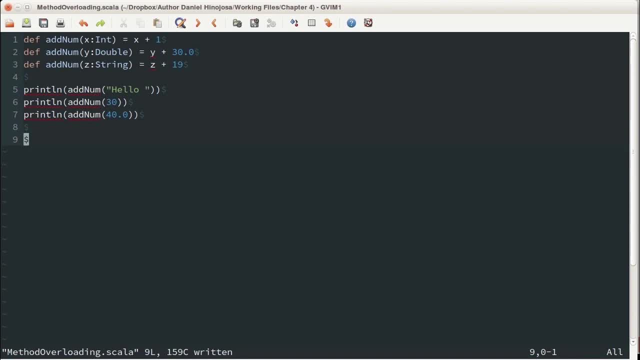 and that they are defined twice. so let's create some bad code. next, let me create a couple methods. both of these will be called add 10 and both of these will receive an int type. what's going to be different about this one is that the second add 10. 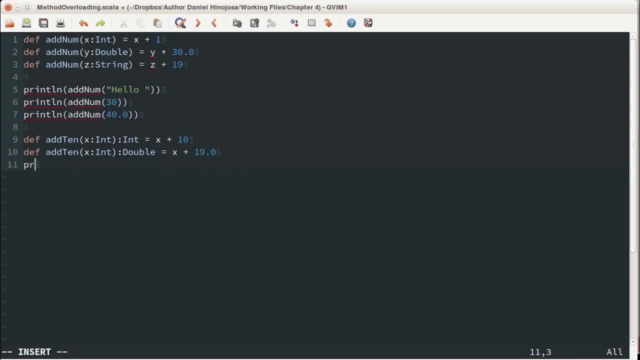 method will return a double. so if I try to invoke this kind of see what's going to happen. I'm calling add 10 with 40. problem is Scala doesn't know which add 10 to call both of them except an int. let's save it and try it. 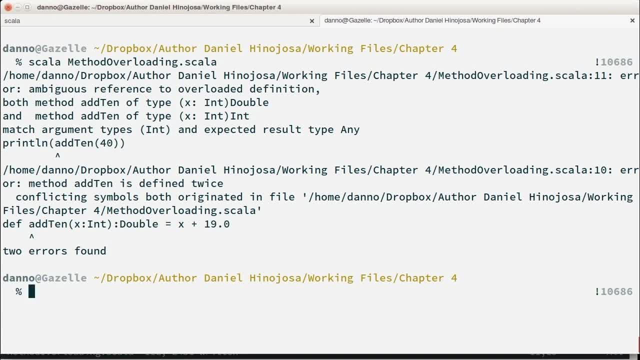 first error says ambiguous reference to overloaded definition. both method add 10 of type int to double and add 10 of type int to int. the second one states that the method add 10 is defined twice. as far as the Scala compiler is concerned, it does look like that. 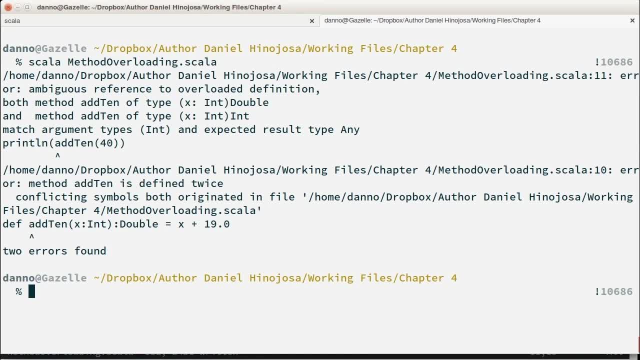 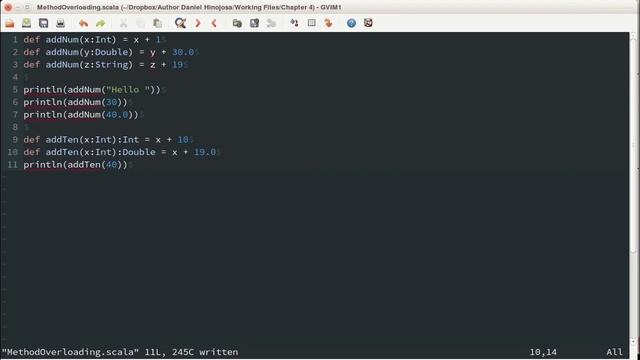 there are two. add 10s. both that, except an int. of course we had enough information on the type signature that would allow method overloading, so let's go back and change that. so what I mean is if there is enough information enough for it to be different. 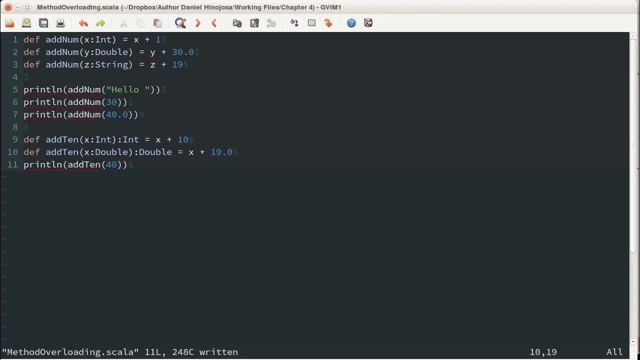 then it would know what to call. and in this case let's say: I want to change that second parameter in the second method to double save it. let's go back and run. it looks great, we get a 50. let's go back to the source code and see why. 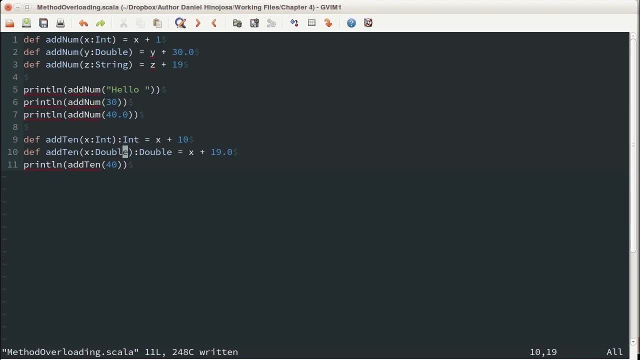 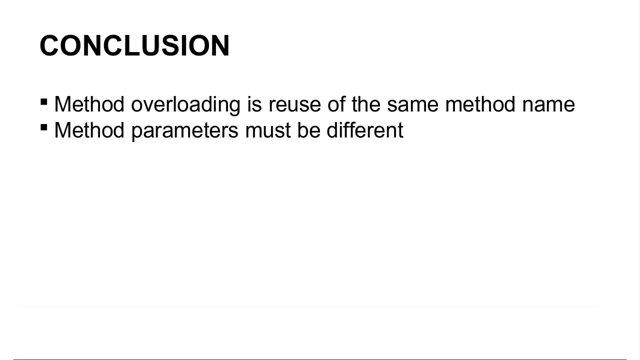 we're calling 10 with 40. very much like add num example we had up there, we're calling it with 40. once we call it with 40, we are adding 10. so method overloading allows us to reuse the same method name for different reasons. 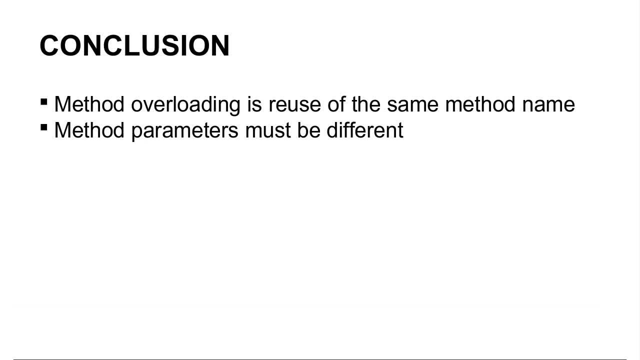 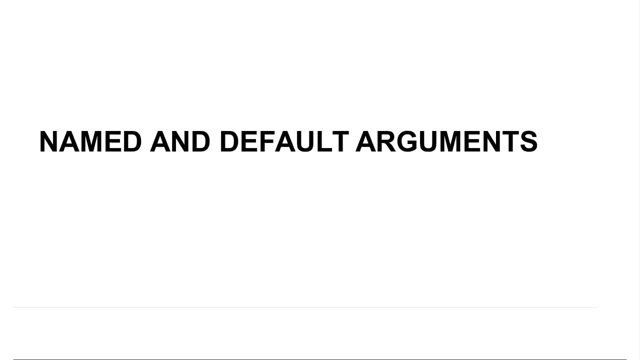 the only thing is method parameters must be different in order to avoid any such conflict. in this section we discuss named and default arguments. others may call this named parameters or default parameters, according to the Scala specification. these are going to be discussed using the terms named and default arguments. 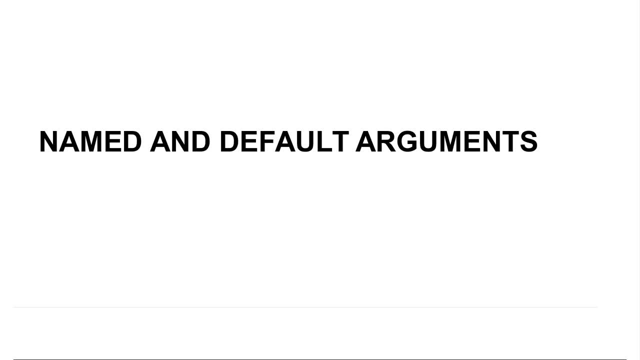 named arguments are a way of calling a method with our own order. so let's take a look at an example of a method. given a method that accepts a Boolean and returns two ints, and we'll call this process numbers, and let's see how this works. I'm going to create a file called named. 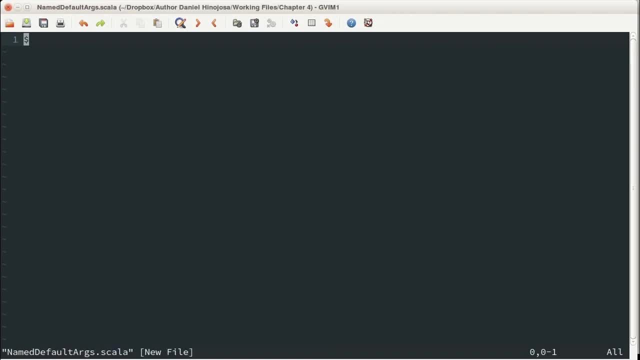 defaultargsscala. and in here I'm going to create a method called process numbers, and in here I'm going to ask the question: if b, then x, otherwise y. ok, fairly straight forward, let's do a print line just to get things going. ok, I'm going to call it process numbers. 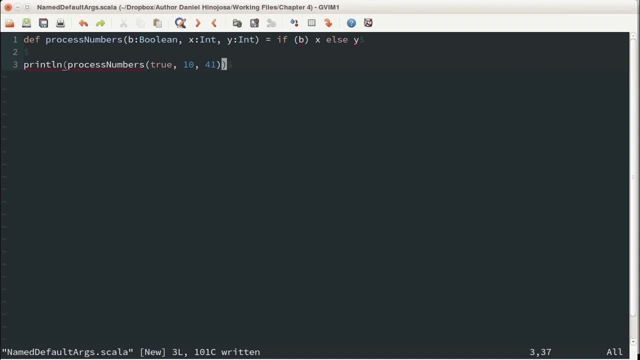 I'm going to give it true, I'm going to give it 10 and I'm going to give it 41. given this example, what should happen is that this should return 10. if it's true- in this case it is- then we will return 10. 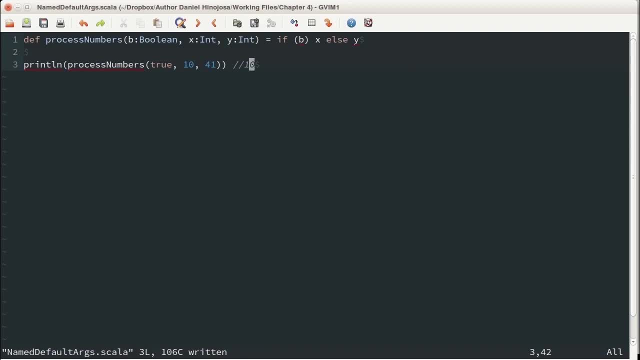 ok, let's save this. let's run it as a sanity check first. alright, we got our 10. now let's go back now. let's say, for a particular reason we did not want to call the method with those arguments in that particular order. in Scala we could specify the order. 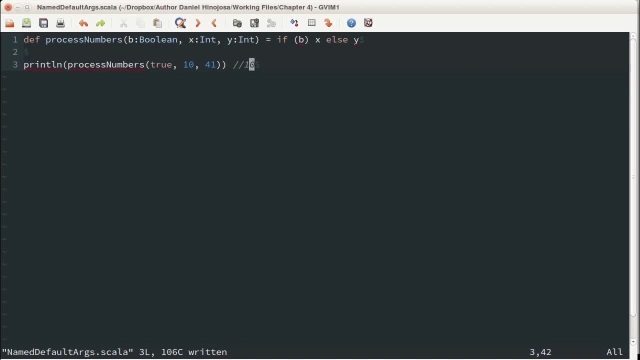 with what are called name arguments, merely state the name of the parameter name at an equals and provide it with the value in any order that you want. so, for example, if I wanted to do- let's say I didn't want to do the boolean here, but I wanted to specify that this will be- 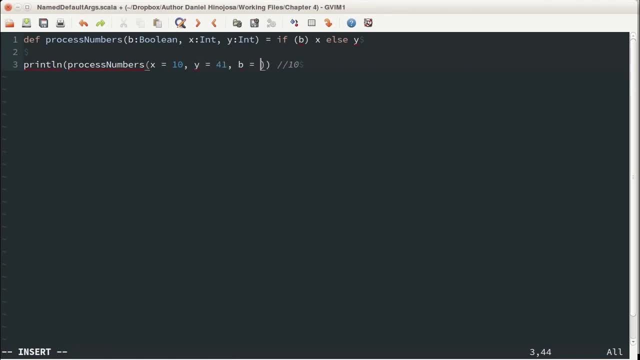 x, this will be y and this will be true b. this b right here corresponds to this b right over here. x corresponds to x and, of course, y corresponds to the y method parameter. this will invoke the method in order with the values given. let's do another sanity check. 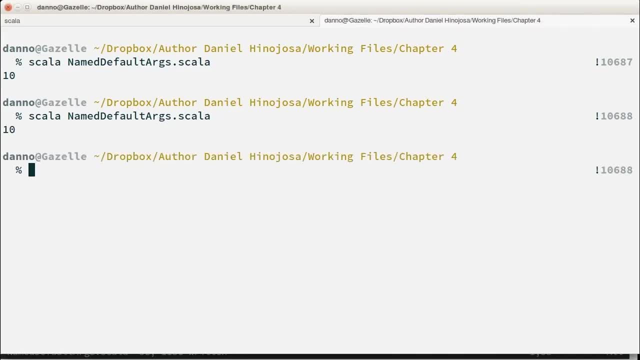 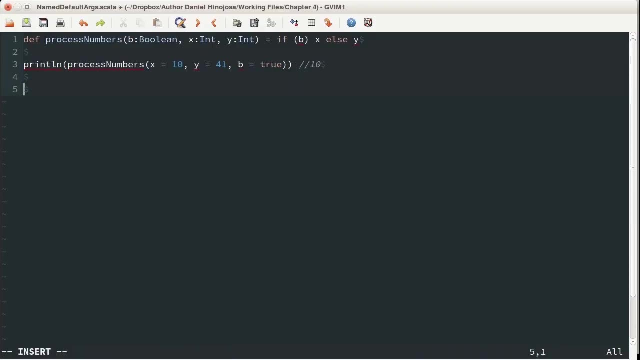 save the file and I'm going to run the file. great still 10. this again is called named arguments. now Scala also provides what's called a default argument. let's show an easy example. I'm going to create a method called add. takes two numbers. we've done. 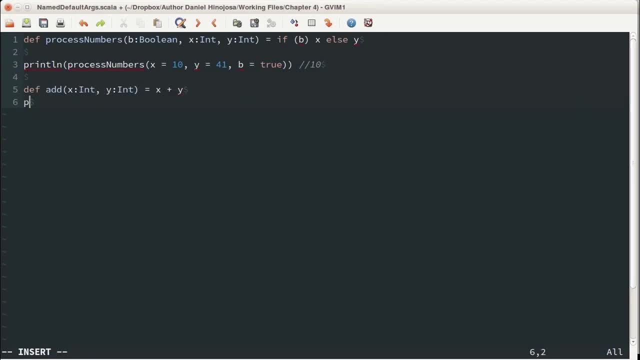 this one plenty of times before and, of course, if we want to invoke it, nothing too crazy here. but what I could do is give it a default argument and because I give it a default argument, I can call without it. let's run it first. 10 was from the previous. 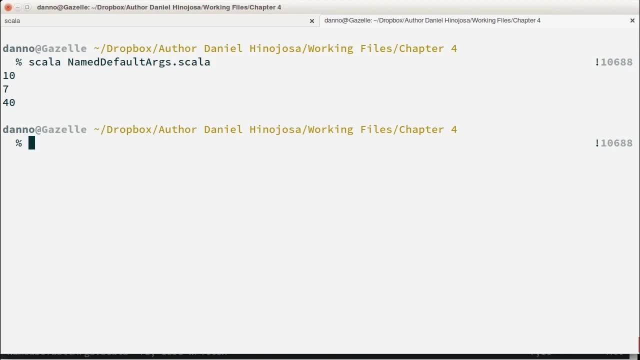 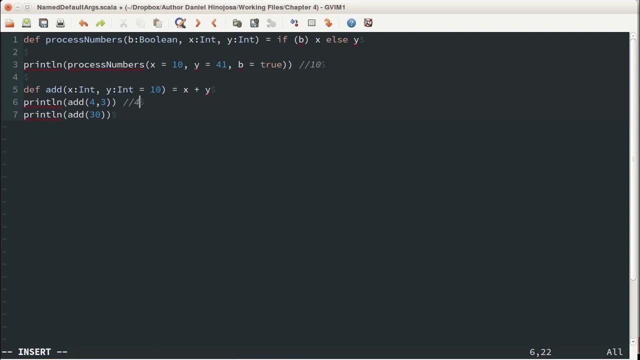 example, and we have a 7 and a 40 for this example. let's go back the reason this was 7, because obviously we're just adding 4 and 3 together. the method is called add. it's going to take 2 ints and add them together. 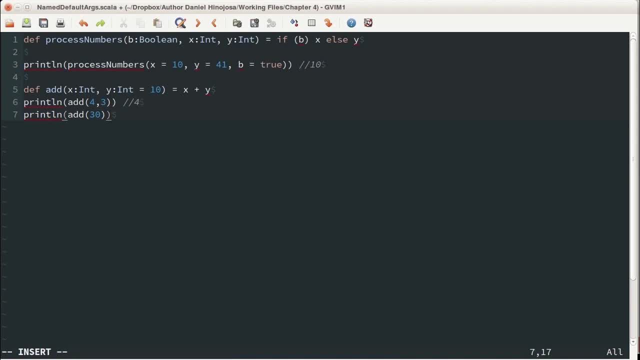 on the second one, though, we give it a 30, and what happens is that, when we call the method add, x is going to be assigned to 30, but since we did not explicitly call y in this example, y is going to be assigned to 10. 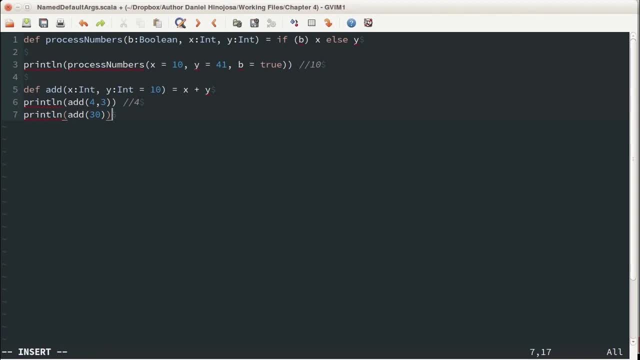 therefore, 30 plus 10 is equal to 40. the y colon int equals to 10 is what is called a default argument. now, where things get complicated are when the default argument is not the last parameter, but somewhere in the beginning. so let's revisit our process numbers. 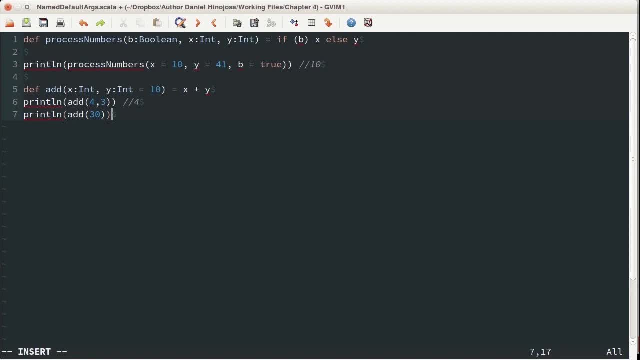 example from above and give our boolean method parameter a default argument. so in other words, coming back up here, let's say in our process numbers we have a boolean and we're going to set that equal to true. so how do we call that? well, if we call it with just the int values, 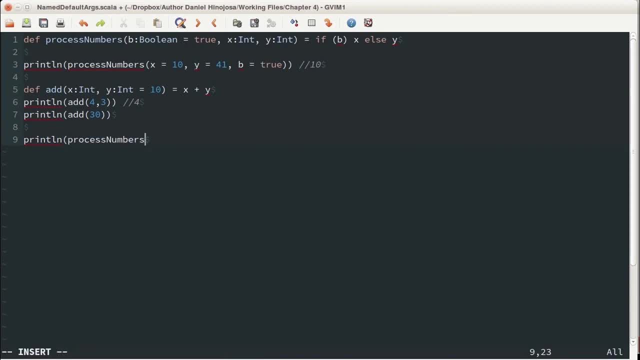 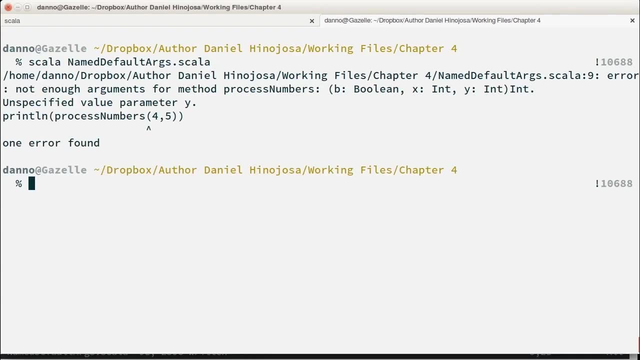 something is going to go wrong. so let's give that a try. we're just handing it over two numbers. let's save it and let's run it. not enough arguments for the method process. numbers doesn't know how to fit that in or make sense of it. 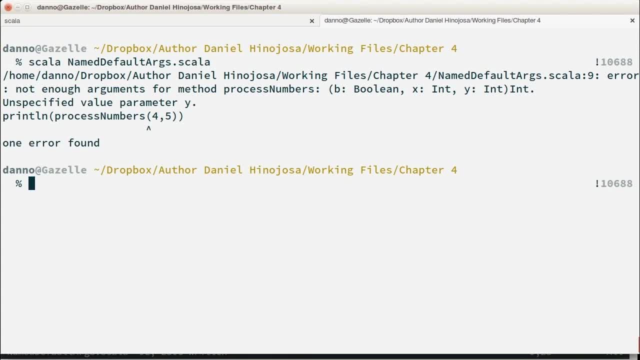 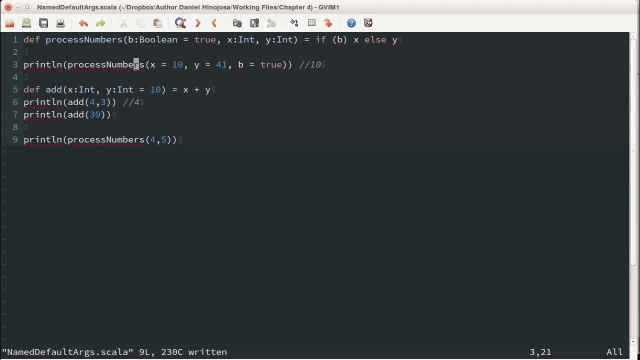 in this case, it's saying: unspecified value, parameter y. it's a little bit confused as to what's going on. let's go back to our code. we're giving it 4 and 5 and, because this is the way this is structured, I think what it's doing is. 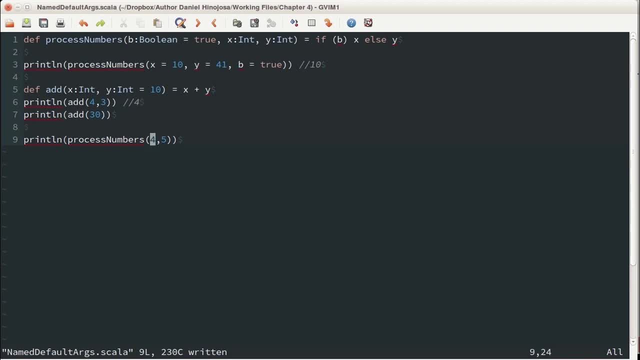 thinking that the 4 is a boolean and the 5 is trying to match up with the x and, I'll be honest, this is an educated guess on my part. as to what the compiler is doing, all I know is, yes, the compiler is confused, but let's go back. 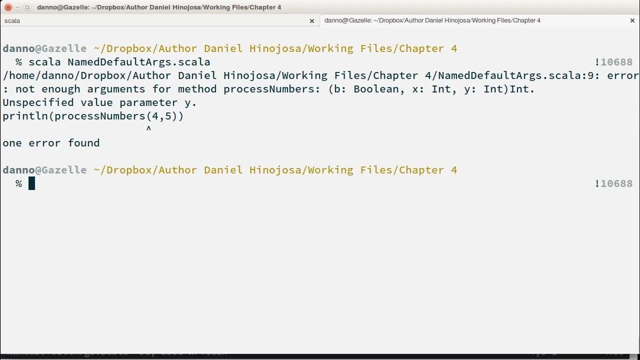 to our output again, and this says: unspecified value, parameter y, so it has no idea where y is coming from. types don't match, so the answer to this is a combination of named arguments and default arguments. so let's go back to our code and make this work. 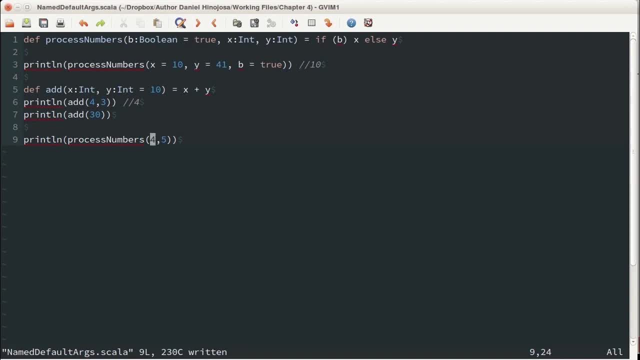 so here in the process numbers, we're giving it 4 and 5 and the compiler is confused, doesn't know where to put the 4, doesn't know where to put the 5, and what we could do is use named arguments to help it out. 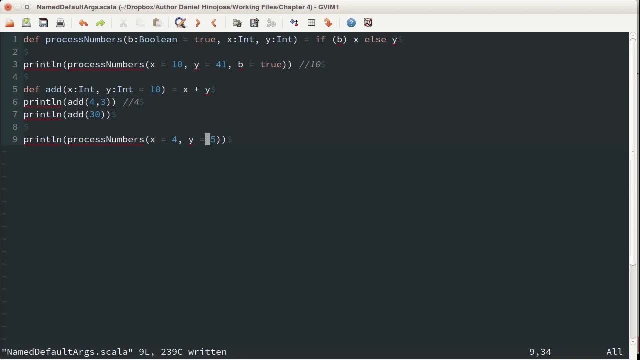 now the compiler knows how we're calling our method, with only the int and all the time knowing that it'll be accepting the default argument of true for the boolean. so let's save this and let's see where we're at. comes out as 4. let's see the reason why. 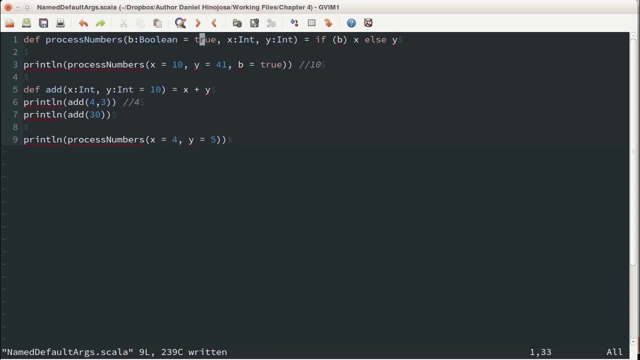 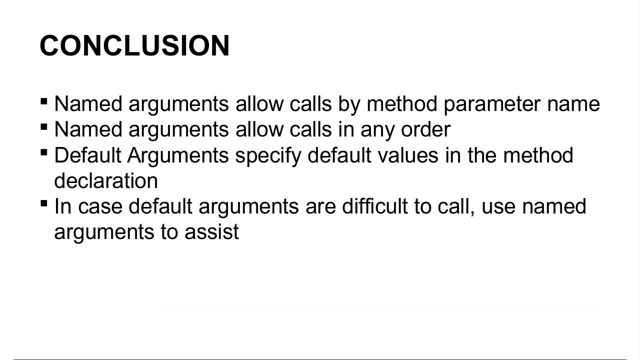 x is 4. y is 5. by default, the boolean is true. since it is true, what will be returned is x. so, in conclusion, named arguments allows us to invoke our method by method arguments. named arguments also allows us to call our methods in whatever order we please: default arguments. 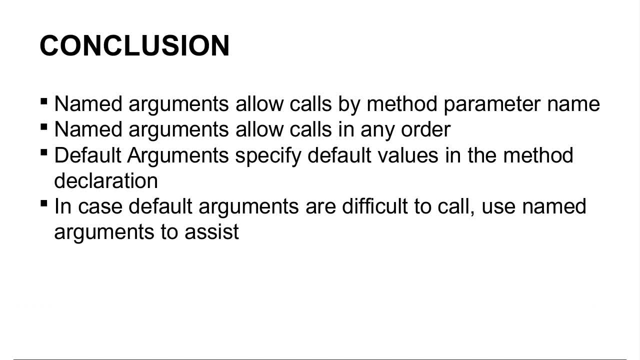 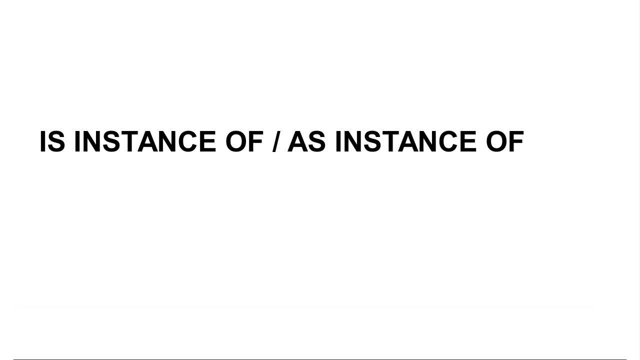 gives us the ability to specify default values for our arguments and, in case default arguments are tough to invoke by regular means, we can use them in combination with named arguments. in this session, we're going to discuss two methods that are a necessity in learning. Scala is instance. 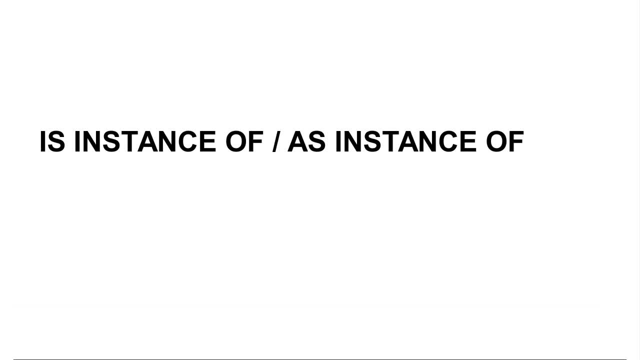 of and as instance of both of these methods are in the superset of all classes called any. for information on the any type, please refresh your memory: in the any any val any ref session earlier in this chapter, since is instance of, and as instance of, is a method from the type any. 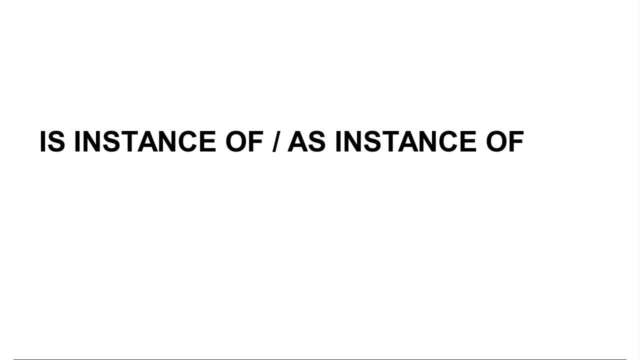 that means that those methods can be used on any object and any primitive. let's go to the REPL and try this out. we could do. 3 is instance of int. now these square brackets are what are called a parameterized type, and we'll be discussing that in the next session. 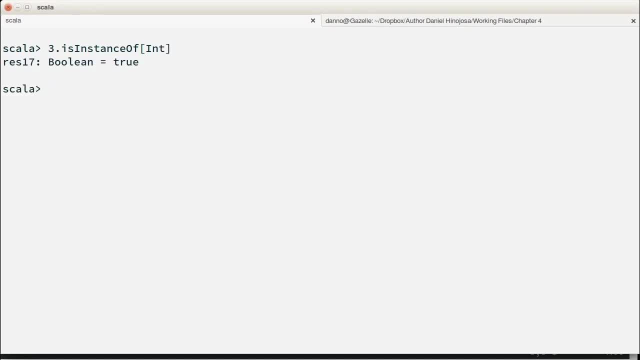 if I hit enter, this is going to return a boolean whether 3 is an instance of int. if I do 3, is this an instance of boolean? this would say false. I mean, obviously the number 3 is not an instance of boolean. if I did, is 3. 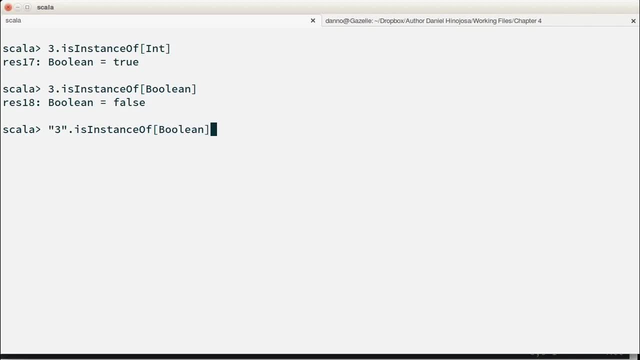 is that an instance of boolean? of course, this would be false as well. but if we did, 3 is, I'm just doing a tab completion here by hitting the tab key. is this an instance of string? this would return true, but it goes a little deeper than that. 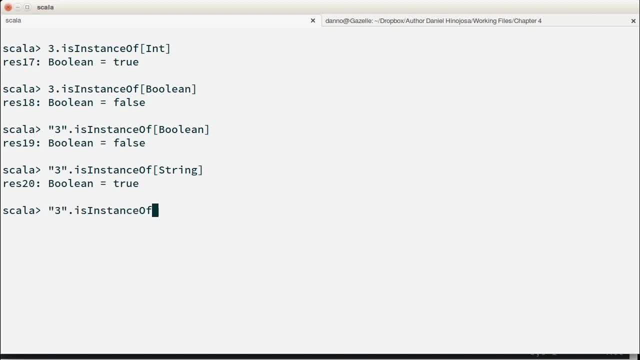 if I do string of 3, is this an instance of car sequence? this would also be true. car sequence is a super type of string. that's why this worked. so therefore, is instance of car sequence returns true for a string and a car sequence. here's the family. 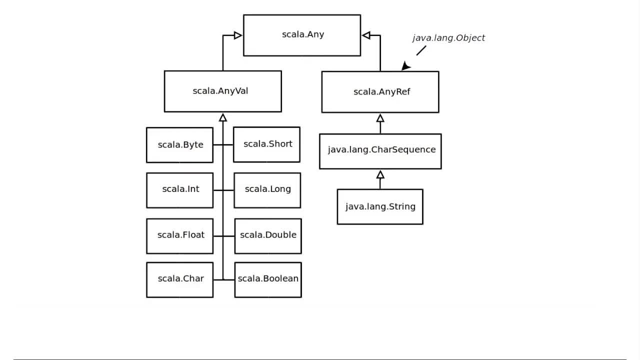 tree for string, any type that makes up your object will return true if it inherits from that type. a string is a car sequence, it's also an any ref and it's also an any. it's worth mentioning that all these types come from java and for those coming in from java, 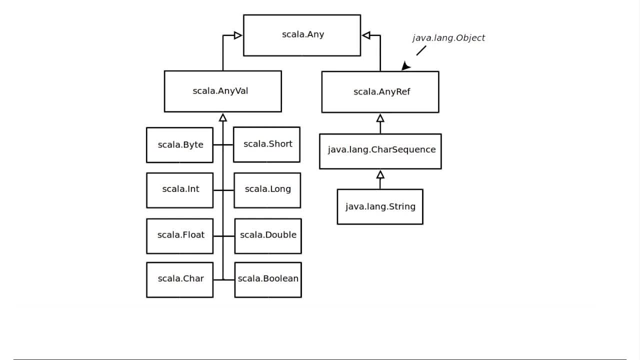 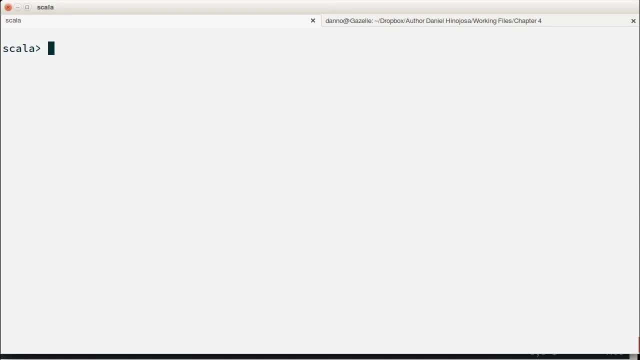 this is going to be a replacement for the instance of keyword. now let's go back to the repl and let's talk a little bit about casting. casting is forcibly converting an object from a super type to a more refined type. I know it sounds like a lot. 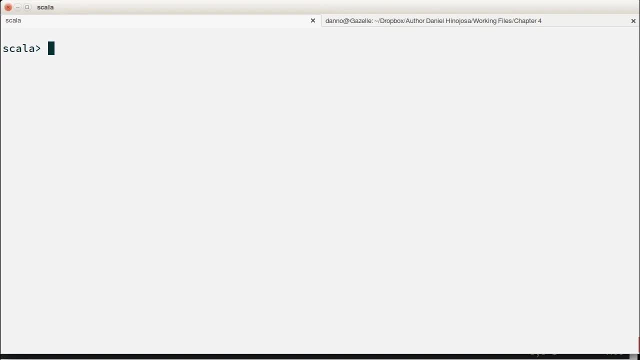 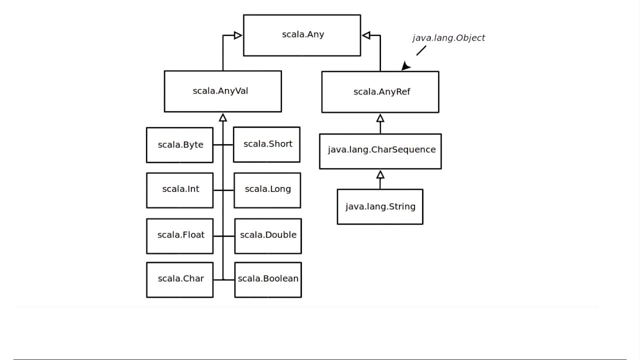 of nerd talk. so let's show an example. we know that string car sequence, any ref and any are all in a linear relationship. again, let's take a look at that family tree: string car sequence, any ref and any- they're all in a linear relationship. assigning a super type to an object. 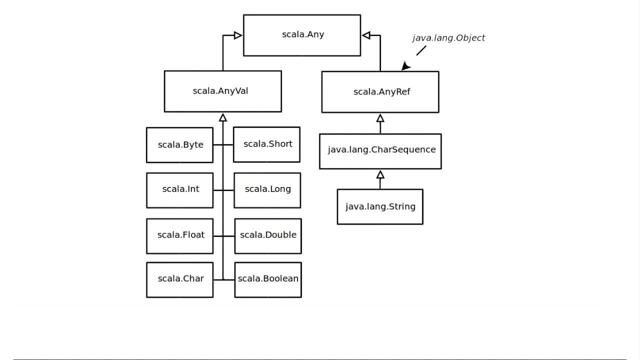 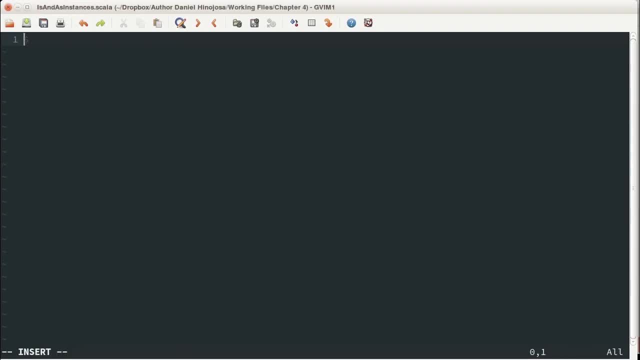 is no problem. so let's get started with an example. I'm going to create a file called is and as instances: dot scala. so let's say we start off with val g and let's make g of a type any and let's assign this to alright, kind of a silly one. 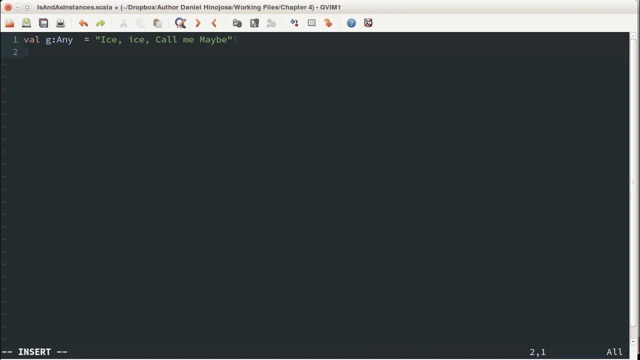 any is the super type and string, if you remember, is a subtype and therefore this assignment does not require any cast. we're taking the more broader type- here- it is any- and assigning it to a more refined type. now, going the other way, assigning an any object to a string. 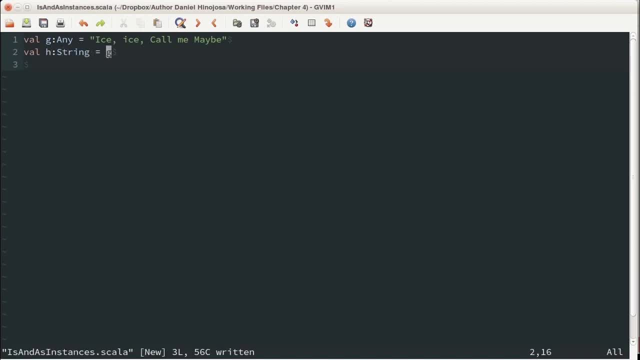 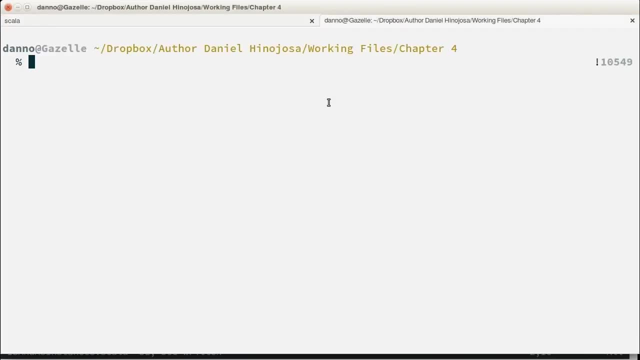 will cause issues and this will not work. g is a reference to type any. h is a type that only refers to strings. we save this and if we run it, this will cause a type mismatch again. we're trying to take something of an any type, which is: 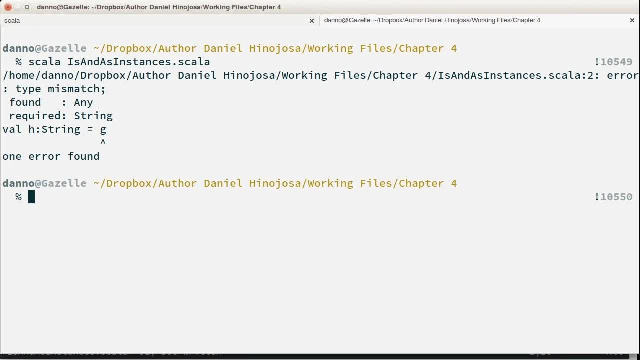 much broader and we're trying to show that into something more refined, the string type. going the opposite way, and because we're assigning that broader type into that refined type, we need to cast. but scala doesn't have a cast like c, c++ or java. our cast is actually a method called. 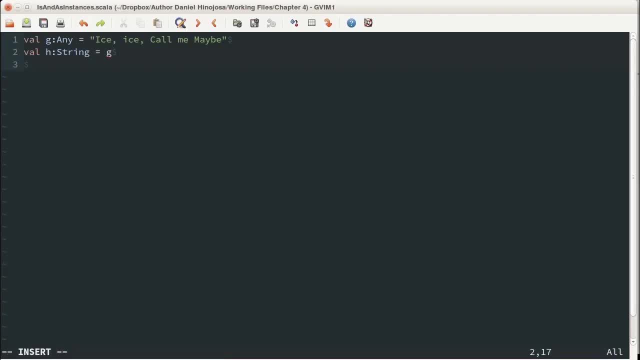 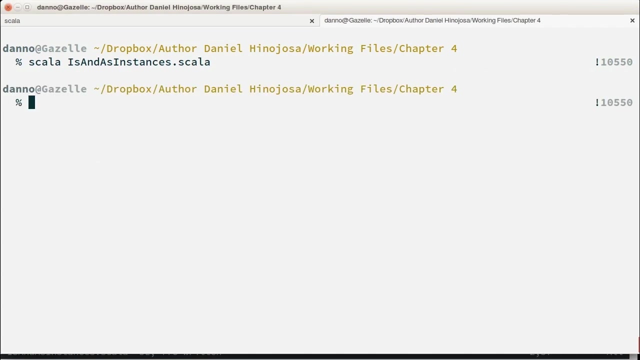 as instance of. so let's give that a try. so I'd like to take g and convert that, using as instance of with a type that we wish to convert to. let's save this and run it. okay. success. we didn't have any print line, just knowing that it compiled. 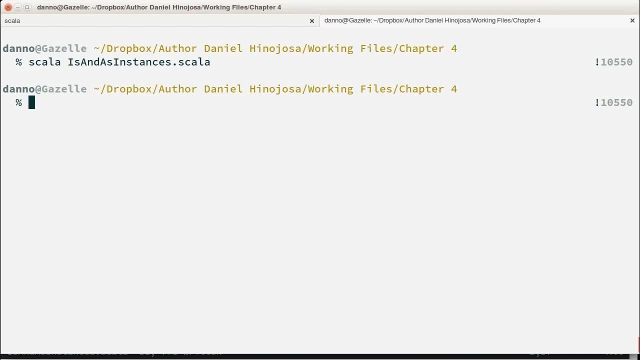 and ran means that it was successful. the two methods is instance of, and as instance of, go hand in hand. it's usually very dangerous to perform an as instance of on something that you don't know the type of. therefore, the methods will usually work in combination. I'd say usually, because under most circumstances, 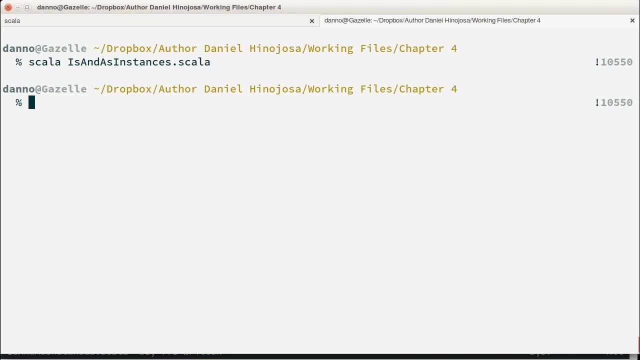 you will need to do this, but there may be a time that you are in complete control of a particular situation and you may not need to convert to another type. let's do an example for that. let's say I have a method called decide, and decide is bringing. 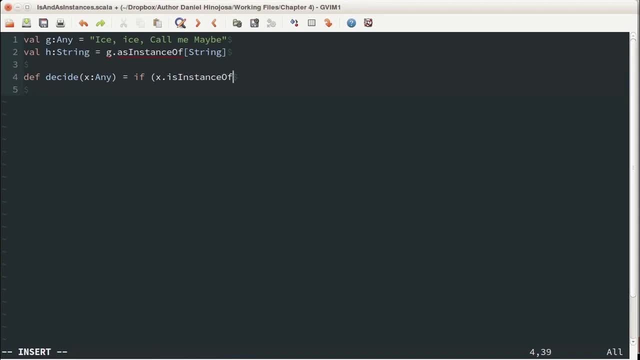 in any, and I'd like to ask the question. so this is a method called decide. it has one method, parameter x, which is of a type any. in other words, we can call this method with anything that we'd like, and the implementation for this method is if. 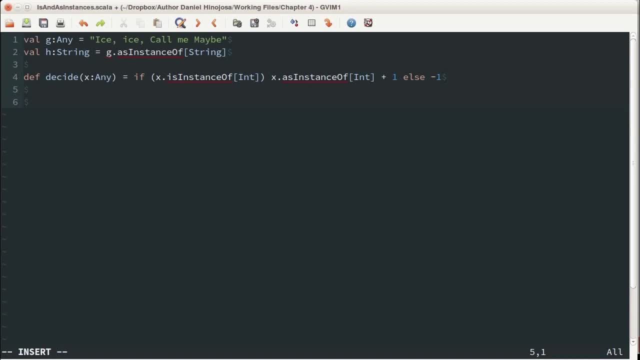 x is an instance of int, then what I'd like to do is convert that x to that instance of int, very much like in our line two. we took something and converted it into an instance of string. in this case we want to do essentially a cast to an int and then add one to. 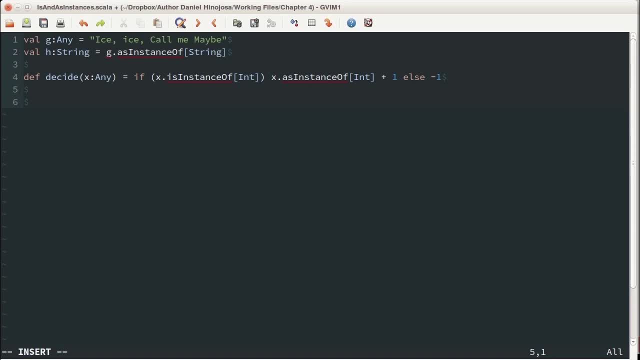 it, otherwise we will return negative one. and this is determining the instance x first, before performing the cast. once we determine that x is an int, we can say: alright, I know it's an int, convert it to an int and add one. so let's give it a try. 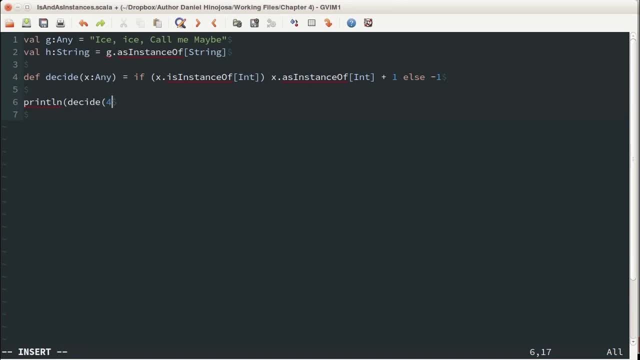 let's do a print line decide, and if we give it something that is a int, then we will add one. otherwise, if we give it something that is not an int, we should end up with a negative one. so the answer on this should be a five and a negative. 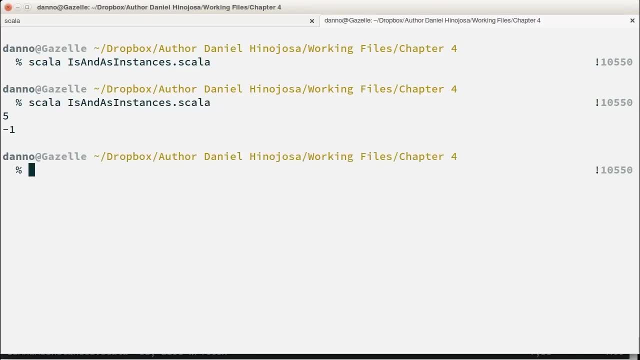 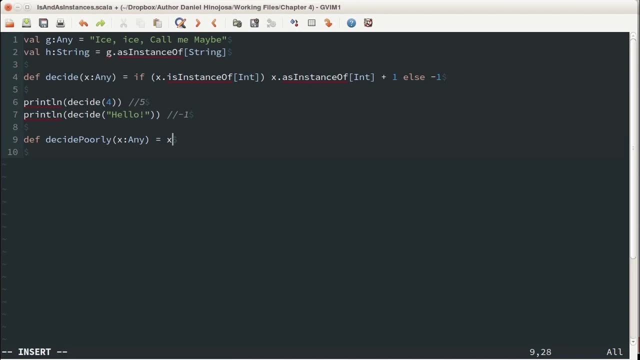 one. let's run it now. let's say we didn't write it correctly. let's go back to our code. I'm going to create another method called decide poorly. in this case, I'm giving decide poorly an any and I'm going to make a strong assumption. 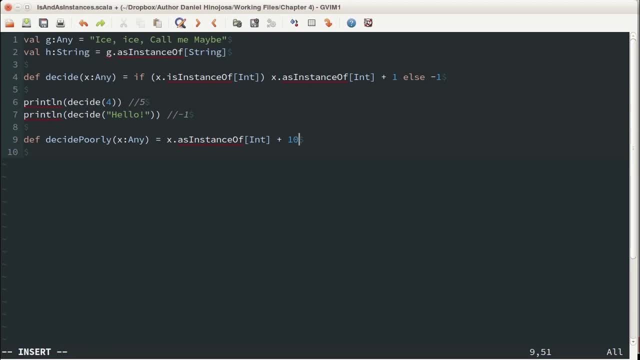 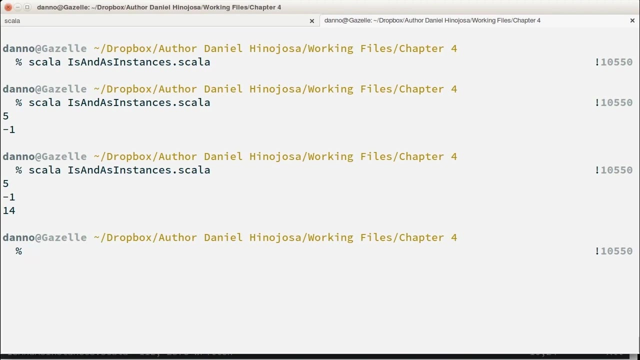 that anything that is given to this method is an int. so if we do a print line decide poorly with a four, let's run this. that will work just fine. we're adding ten to it, we give it a four and what we get back is a fifteen. that works great. 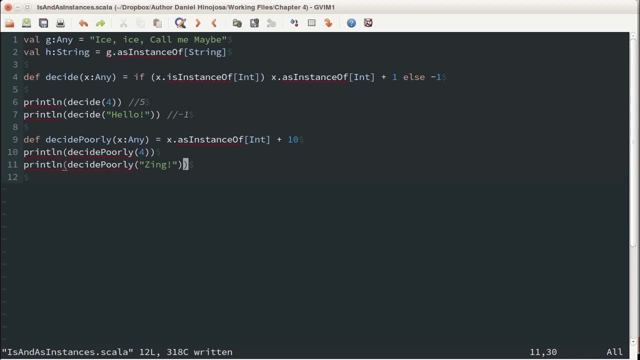 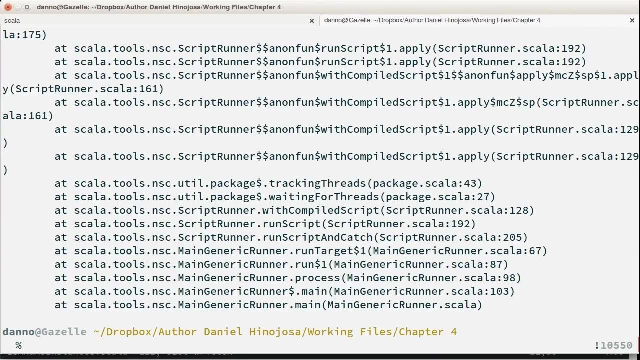 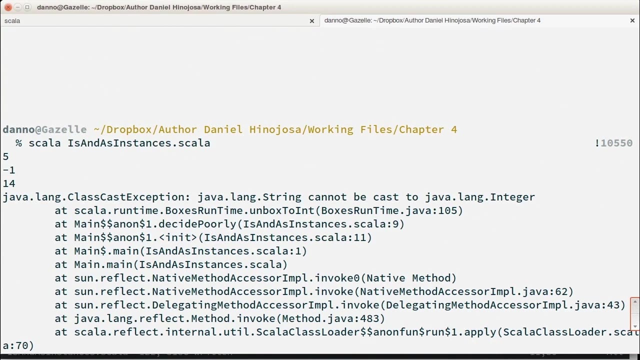 but where things go wrong is if we give it something of a type that is not expected. if we don't do our due diligence, things are going to go really wrong. we get an exception. the exception is called a class cast exception- java lang- string cannot be cast to a java lang. 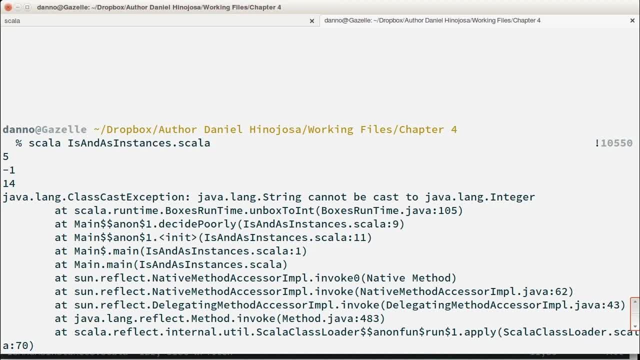 integer- and for those coming from java, you likely already knew this- and this follows the same rules in Scala. for those who are really paying attention and wondering why I didn't talk about the square brackets again, these are parameterized types on a method and we'll cover that. 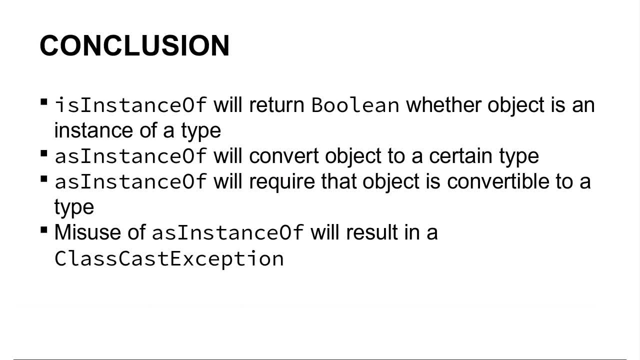 in the very next section. so in conclusion, is instanceof will return a boolean whether the object in question is truly an instance of that type or supertype, as instanceof will convert the object to any other type. as instanceof will require that the object is convertible to that type and any kind of 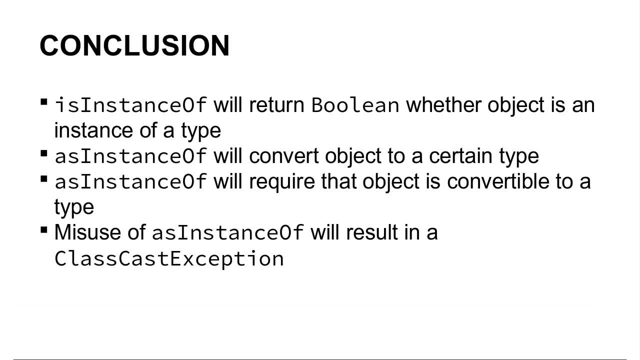 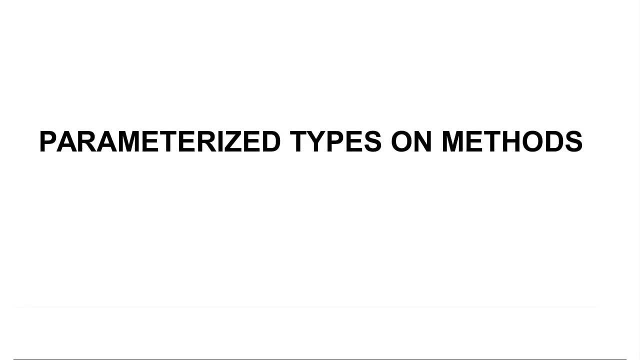 bad call to as instanceof will result in a class cast exception. in this section we discuss parameterized types on a method. parameterized types gives us the ability to maintain type safety when calling a method. this keeps us from referring to an object by its supertype. parameterized types in. 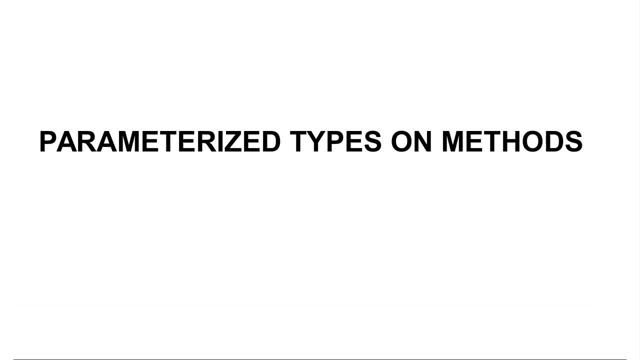 java are known as generic types. parameterized types in C++ are called templates. they're not the same thing. both C++ and java have their own rules when dealing with generic programming. in this section we'll perform generic programming, but we'll do so the Scala way. so let's get. 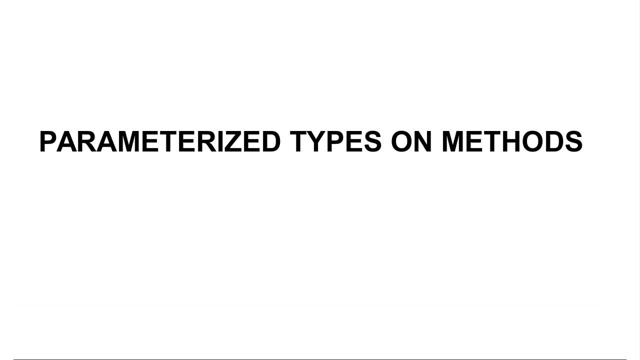 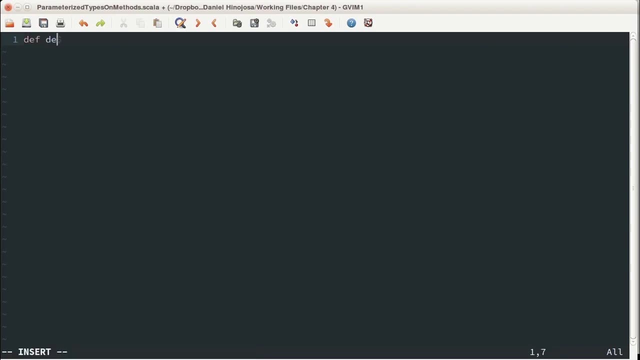 started. let's create a file called parameterized types on methodsscala. and for our simple example, let's say we want to call a method with a boolean and two items, and those items can be anything. so let's get started. I want to create again a method called decide. 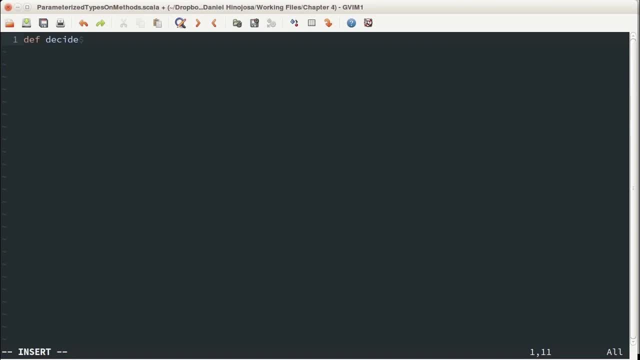 this has three parameters: a boolean and two items. that could be anything, and in our first example we're going to use the any type. this can return an any and the implementation is so again, we have a method called decide. it's bringing in a boolean and bringing in two any's and returning an. 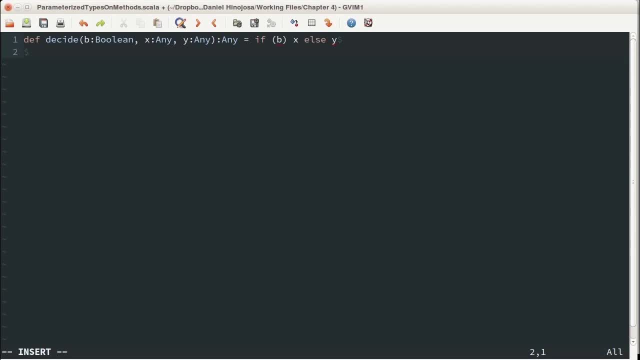 any. if b, b is the boolean. so, given that boolean, if the boolean is true, return x, otherwise return y. now we're going to create some print lines, so let's say for the first one we're going to call decide. if it is true, then return the string of a. otherwise, 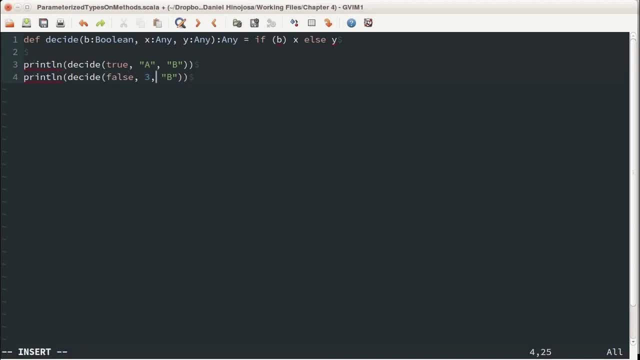 return the string of b. in the second example we'll have false, therefore ten will be returned. and in our third example, if it is true, return the character of c, otherwise return the character of d. now let's go ahead and save this and let's go ahead and run it to see. 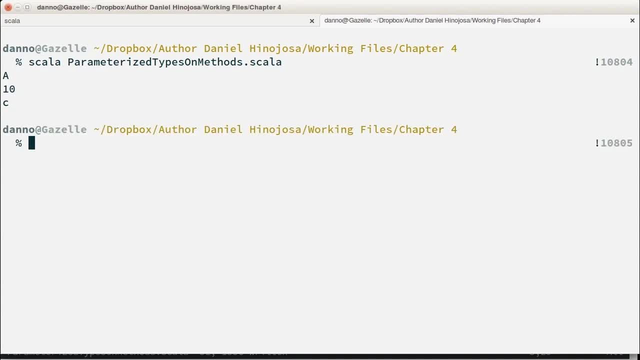 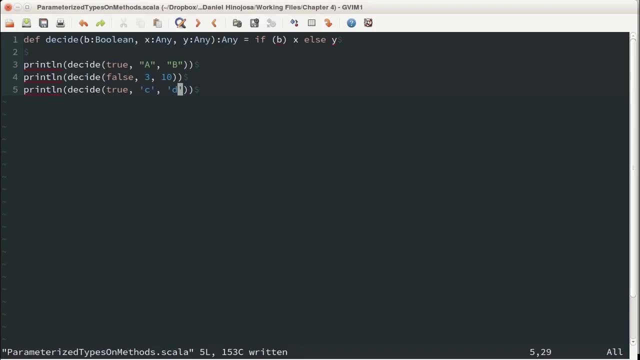 what happens? okay, so we are returning a string of a, a number ten and a c. let's go back to our code and that works. it works just fine. decide takes a boolean and two of any item. remember, any is the super type of all objects and primitives. we're also 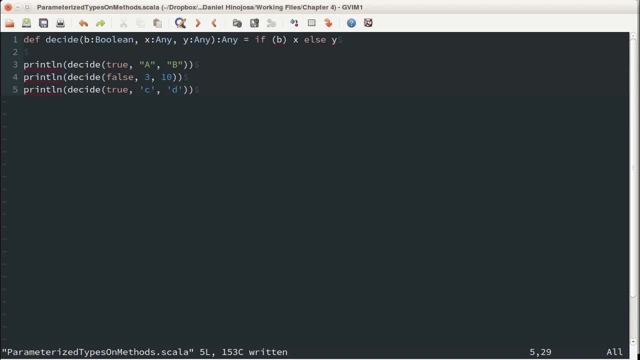 returning an. any problem is that? it sure be nice to maintain that type when invoking the method. what do i mean by that? well, let's take this line right here and let's bring it over to a REPL to see what i mean. okay, so i'm bringing. 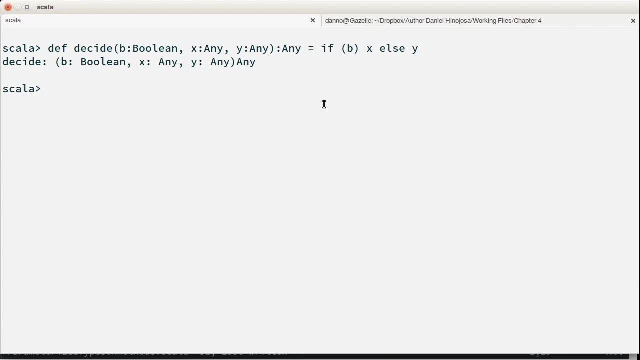 in that decide method. it's bringing in a boolean and two of any item. now what happens if i call this method? let's use the characters. in this case, this returns a, c, but the problem is this is returning an any type. it sure be nice to have this return a character. 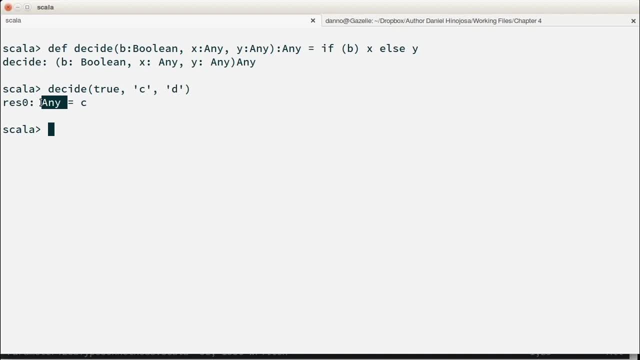 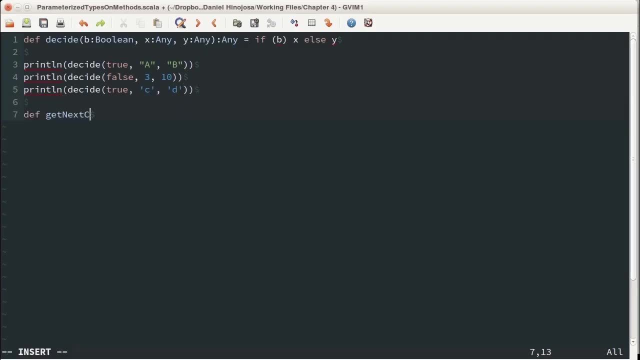 type. there's another problem with this. let's go back to our code and add a few more items. let's say we wanted to add a method called set next character and this receives a character and the implementation is: note: we have to add the to car. reason is that any JVM language. 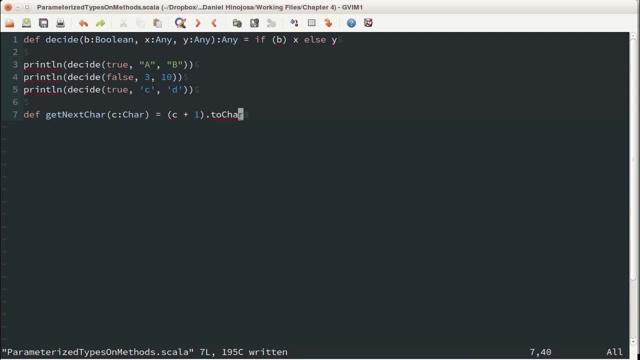 if you add a number to anything that is smaller than 32 bits, the result is going to be promoted to an int automatically. character is 16 bits and since we're adding a one to that character, the result is going to be an int to make sure that it's. 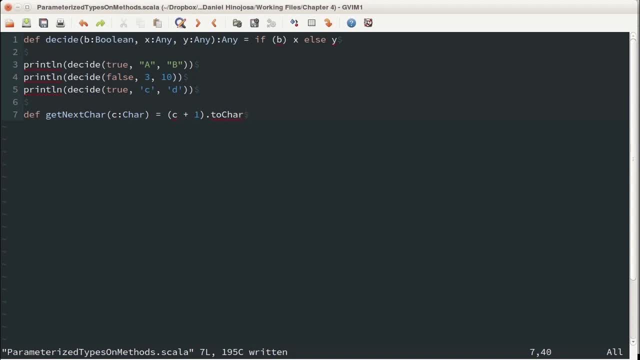 not going to return an int, i have to call to character to make sure that it is a character. now, focusing on this method, this method is something that takes in a character and returns a character. now, if we want to call get next character, we have to provide it a character. 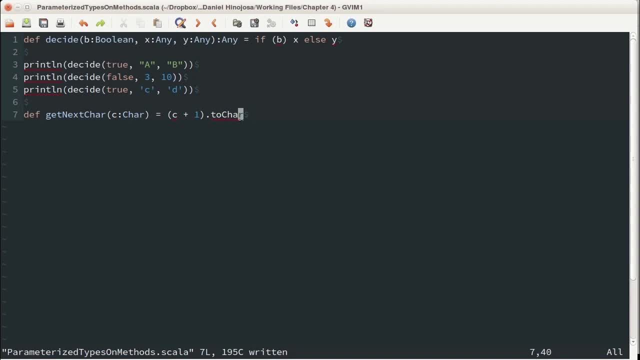 and i'll state that again. we have to provide that a character, the method get next car, and there's no going around that. in other words, if i add the following line, in other words we're doing a print line, we're calling: get next character which accepts the 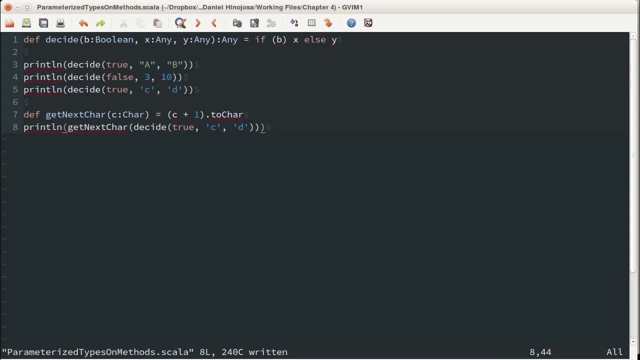 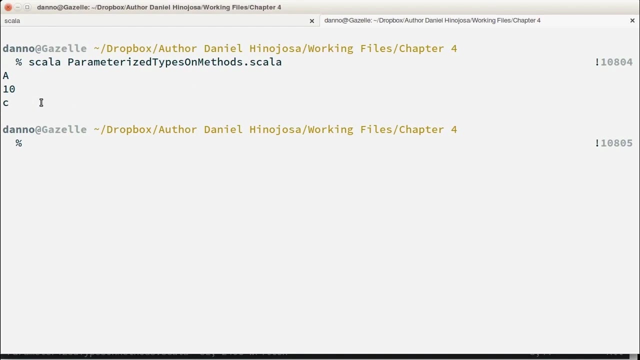 a character- and we're calling it- with whatever gets returned from decide. decide is going to either return a c or a d, depending on the boolean. so let's save this and let's go ahead and run this to see what happens. we have a type mismatch, remember. 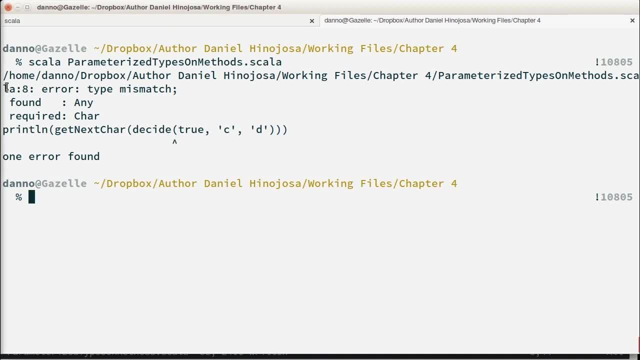 decide is returning any, but what was required was a character say so. right, here we are expecting a character. now we could do a work around, so let's go ahead and do that work around. let's go back to our code. so let's say, in the meantime, we cannot. 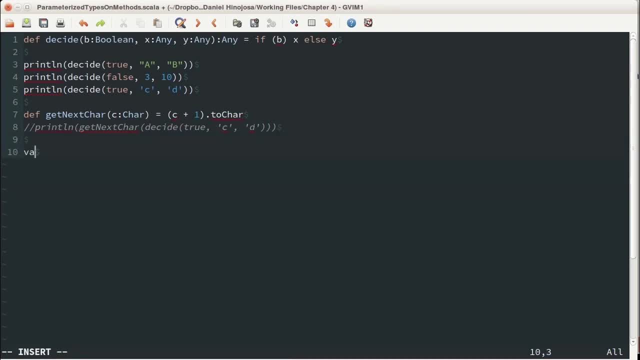 do this? what is our work around? well, we can create, let's say, a result, and let's say we're going to call our decide method with the values that we tried previously and call if. and do you know what this is now? if you don't go, 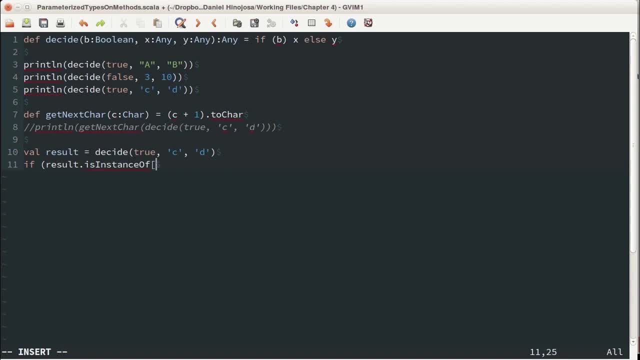 back and take a look at the video series, for is instance of, and as instance of. so if this was a character, and what I'd like to do is I would like to do a cast. remember casting. what we're doing on line 11 is making sure that result is an. 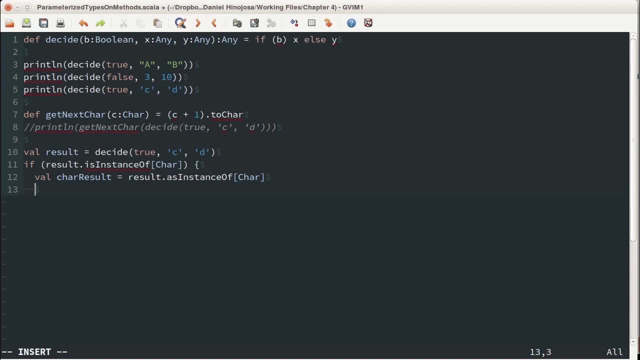 instance of character. if it is, then we want to cast that into a character. remember, results is of a type any. that's why we need to do all this. finally, now that we have this particular result, what we can do is we can call our get next character. 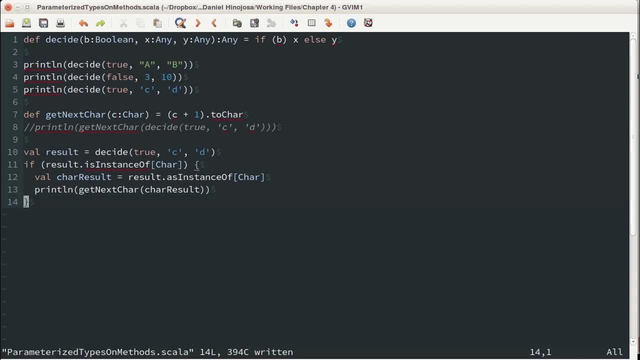 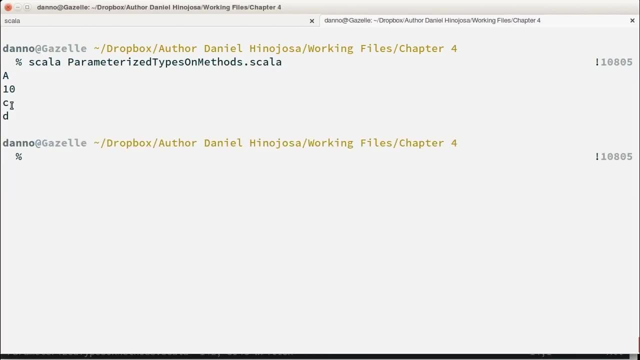 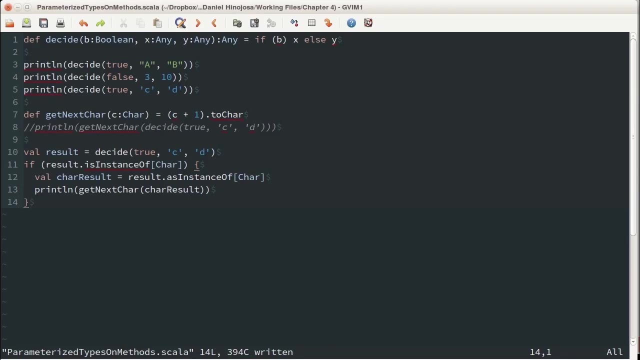 with the result: let's go ahead and save that and let's go ahead and run it. so the first three items was from our first example, but the d here is what we want. go back to our code and here's the d. this is the reason why d was. 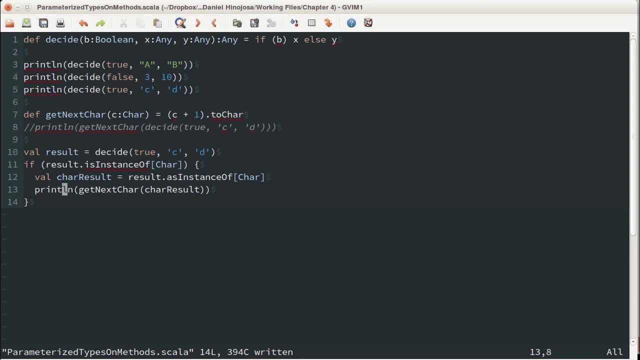 printed out, but already I'm kind of sad. this was a lot of work. I had to ask the result whether it was actually a character, and if it was, then I needed to cast that over to something called car result. car result could be whatever name I wanted to. 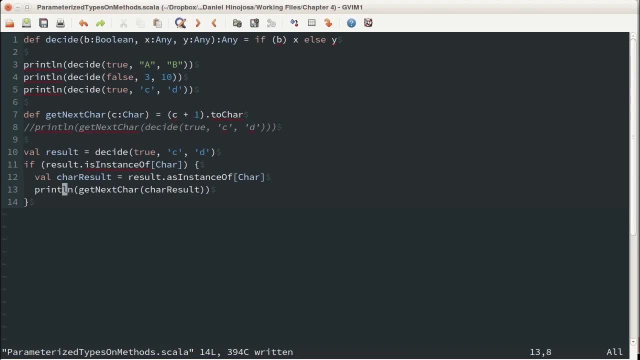 it was just a name that I made up. I had to call is instance of and as instance of, and then finally get the result that I want. now we have parameterized types and we've used them already. in fact, these brackets right up here are actually parameterized. 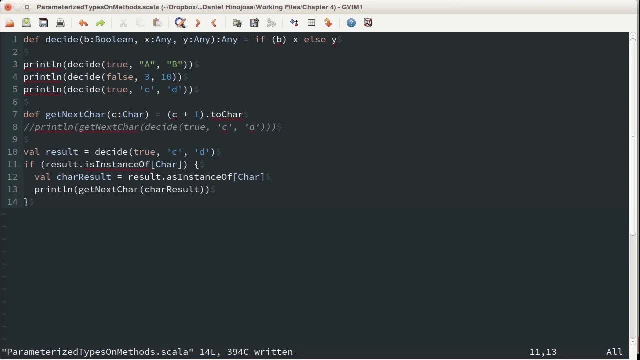 types themselves. this is a method, is instance of, and, as instance of, they're just using parameterized types. now we'll be nice if we can do a parameterized type on our own method on decide. so let's go up here and let's say we want to convert. 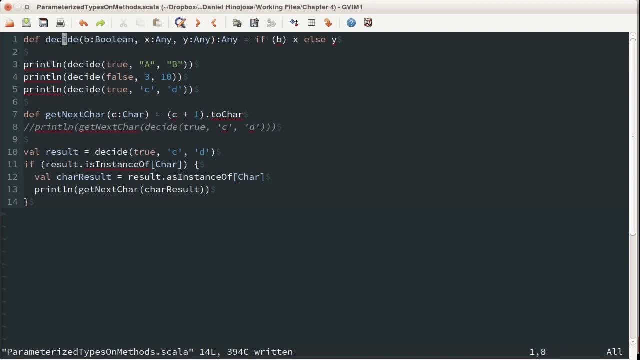 this decide method to use these parameterized types. that way we're a little bit flexible on the any, so let's change all any's to a parameterized type of t. this will return a t. and before we use these parameterized types, I have to declare: 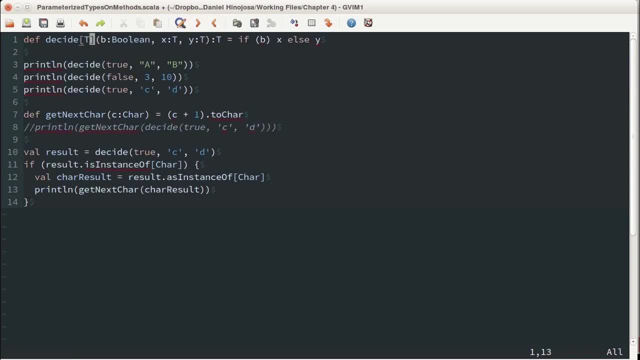 up front, in front of the method, that I am using a parameterized type t here. it is, it's worth highlighting: this is the parameterized type t. this is telling the method. I am going to use any type, but, whatever it is, keep that type around. this is the parameterized. 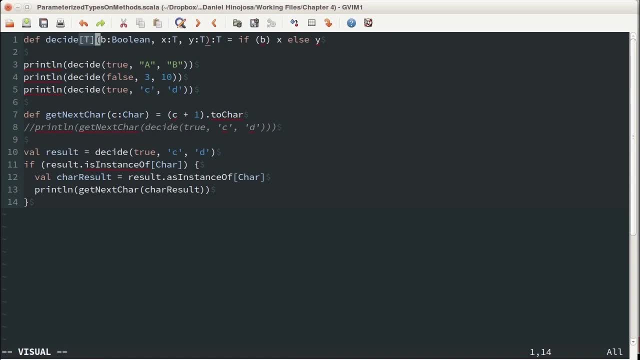 type. in other words, if you call this with int, it's going to maintain that t is of a type int. let's save this. what I'd like to do. let me copy this new method over to the repl. let me show you what I mean. let me call: 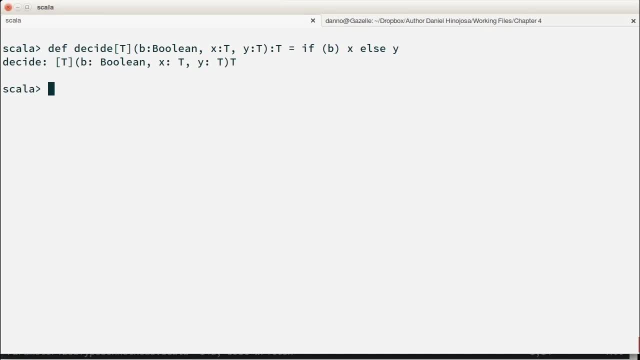 colon reset to clear everything out, and I'm going to go ahead and paste the new method onto the repl. so this is a method called decide. it is parameterized. t could be anything. we're declaring it up front that t is a parameterized type. so let's see how this 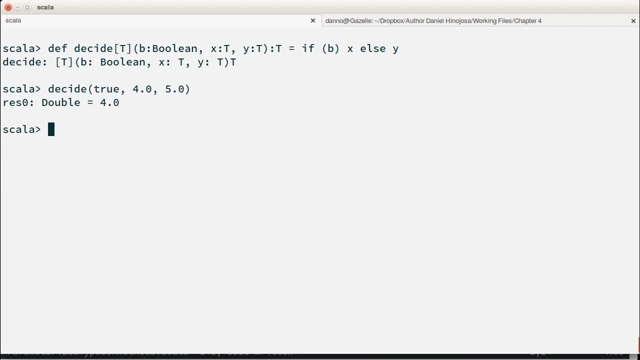 works pretty neat. this is not returning an any. this is returning a double. now, if we try it with something like this, what do you think the answer is for this one I'm calling: decide with a boolean and a double and a string. this will return an any. 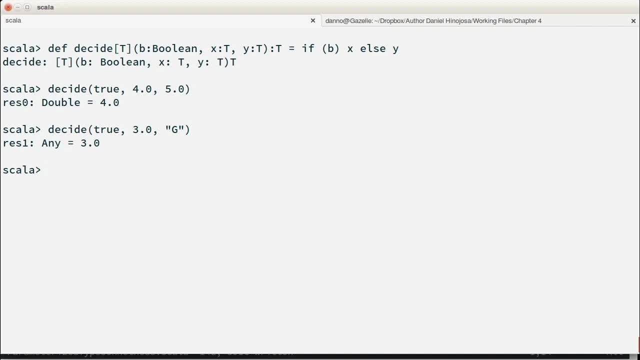 in this case, what the type system is going to do is: it's going to see a type of double which is under any val. it's going to see a string which is under any ref, going to find the common parent. the common parent in this case is: 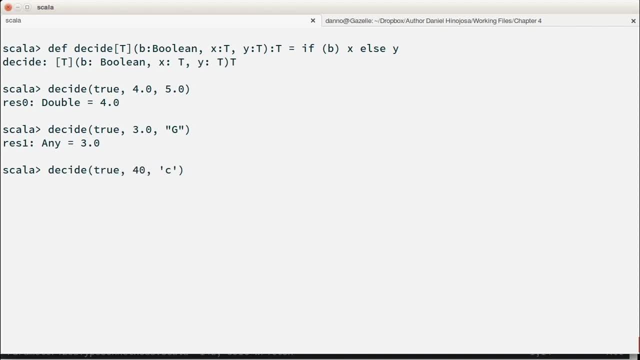 any, try something a little bit harder. this returns an int due to int promotion of the character. remember, behind the scenes, a character is a number, it is a 16 bit number and it interacts with an int. therefore, due to promotion, it is going to be converted to an int. 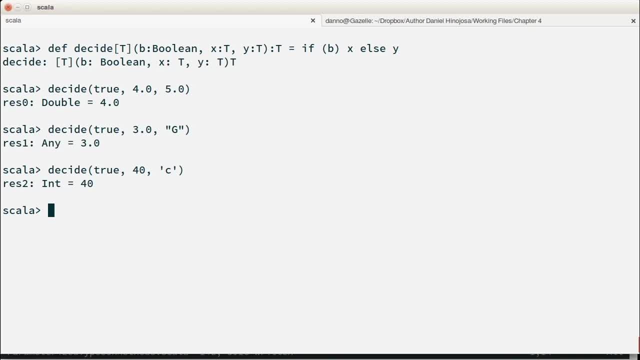 and again as a reminder, any numerical operation with anything smaller than an int will by default result in that promotion of an int. anything that involves a long as part of the operation will result in a long. anything involving a floating point will result in a double. greatest thing of all this: 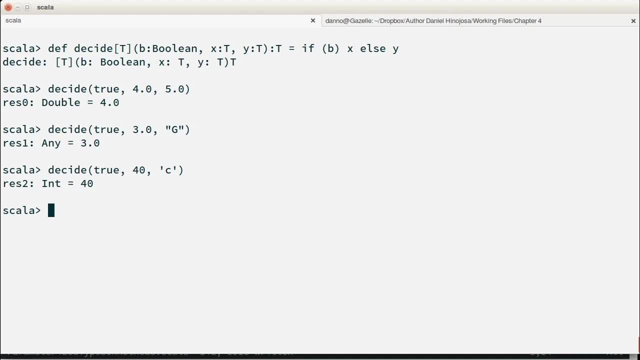 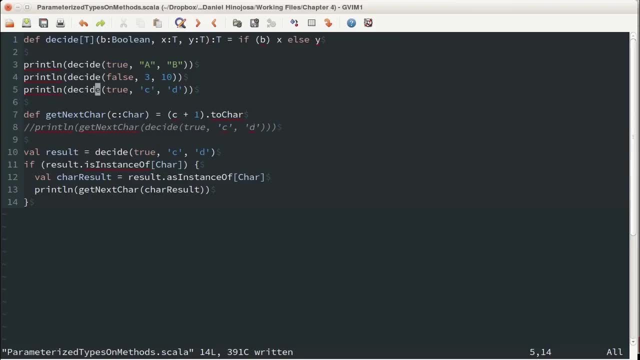 is that now we can call, get next character without any of the as instance of or the is instance of calls, as we had before. so let's go back to our code, and what I'd like to do is I would like to comment all this out and bring this back. 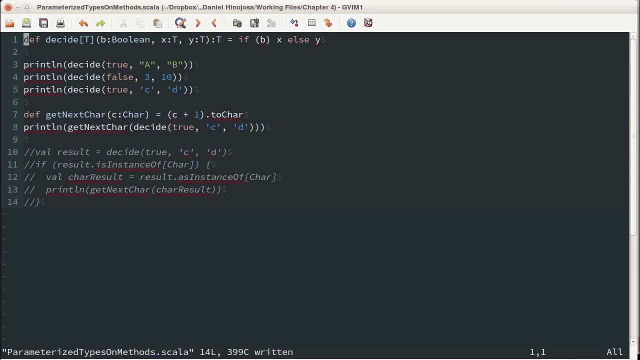 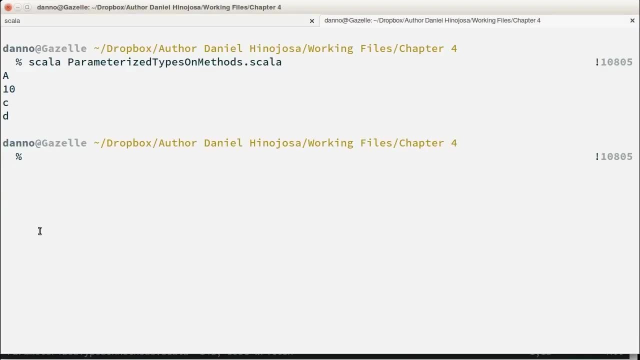 let's save it and remember we converted this to a parameterized method, using parameterized types, so let's save it. let's go back to our command line prompt. let's run it again. great, again, I didn't need to use all the as instance of or. 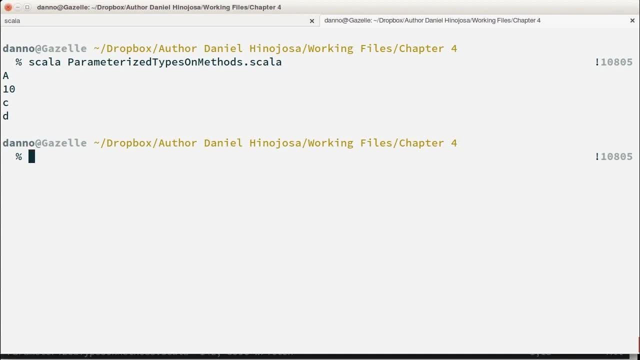 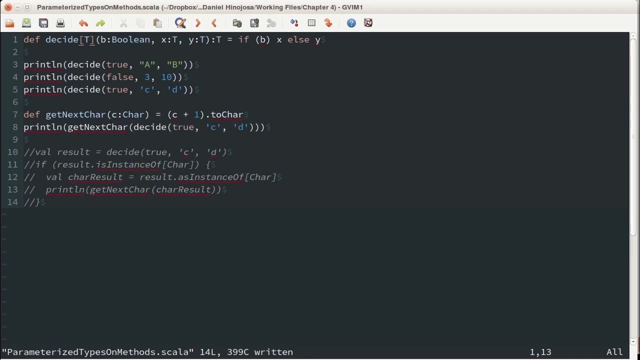 is instance of works out really well. why does it work? because the types match. let's go back to our code. decide now. can return a character. it doesn't have to return in any. we're not forcing it to return in any. this is a huge plus. it makes a huge. 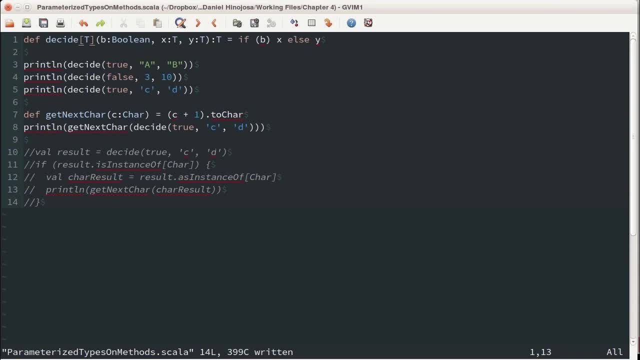 difference because we're giving it two characters for x and y. that means, since that is the same type t, we are returning that type t. and since type t is already established that it is a character, then we are returning a character. no weird. type checking- no weird. 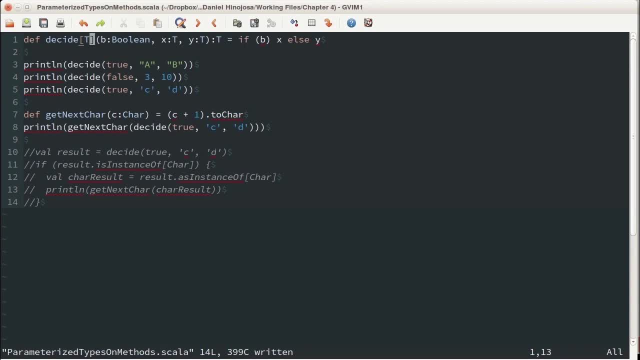 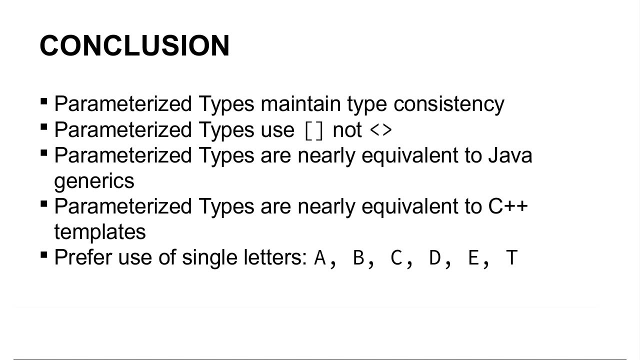 type casting is necessary and I think you'll agree. although it takes a little bit more thought and planning, it's a much cleaner solution. so, in conclusion, parameterized types help maintain type consistency. parameterized use brackets as opposed to the greater than or less than characters, as you saw with our 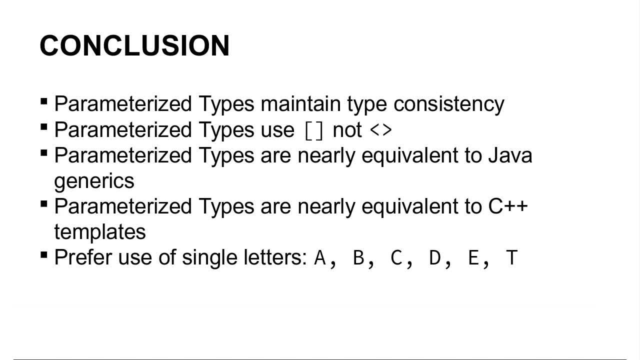 examples: parameterized types are known as generics in java templates and c plus plus. the implementation is different in Scala. it's preferred that you use single letters for the parameterized type. in our example you saw us use a- t. you could use a, b, c, d, e. 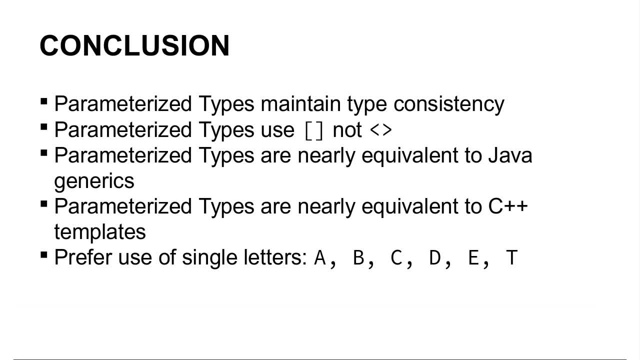 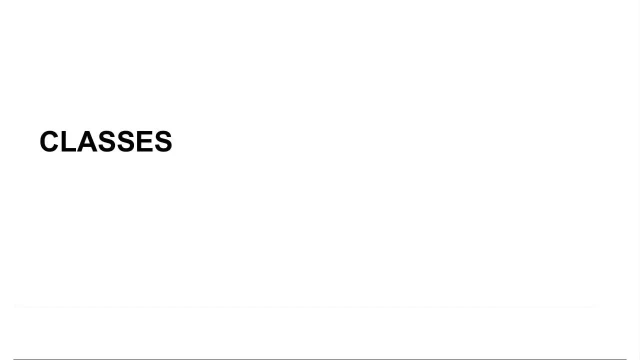 whatever kind of letter you want, you could have full names, although that is outside of Scala convention. in this section we finally talk about classes. classes are the templates or blueprints of a construct that encapsulates state and manages behavior. classes have been around for a long time and 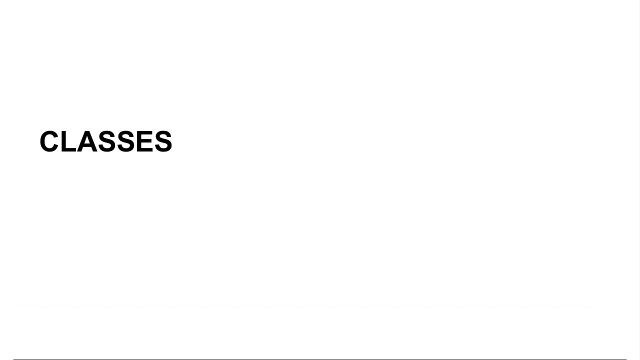 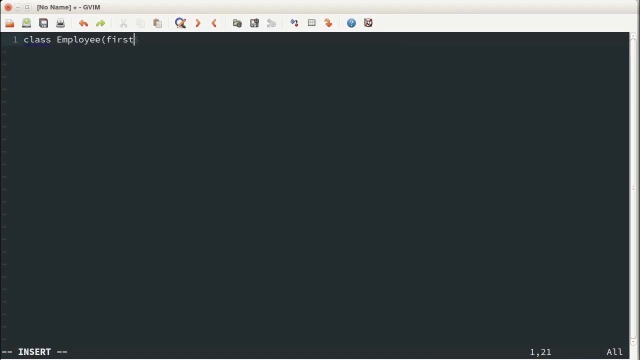 in every object-oriented language. since Scala is half object-oriented language, half functional language, there are naturally classes. so let's see what a class looks like in Scala. here I am in the editor and I'm going to create a class called employee, and employee will have a first name. 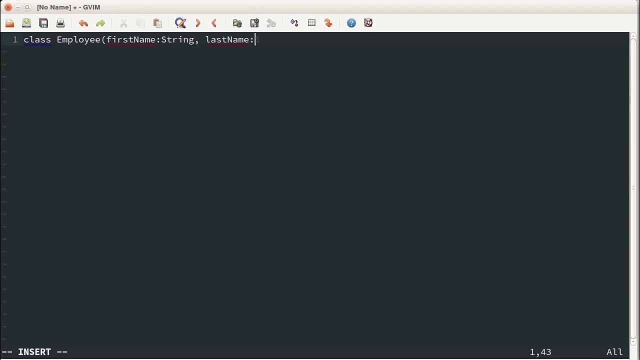 of type string and a last name of type string. I'm going to save this into a file called employeescala. now for the Java programmers among us, that is it. well, sort of. we have to add probably a few more things here and there to get what we want, but it isn't. 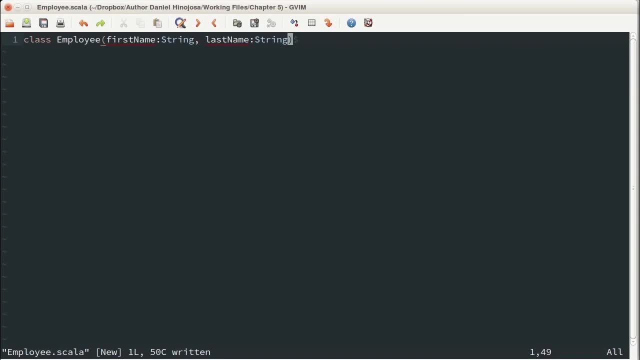 too much. in Java, there are all the ceremonial incantations we have to do in order to make this work, creating getters, creating setters, etc. whereas in Scala it is very straightforward and very to the point. again, for also the Java programmers among us also notice: there is no public the 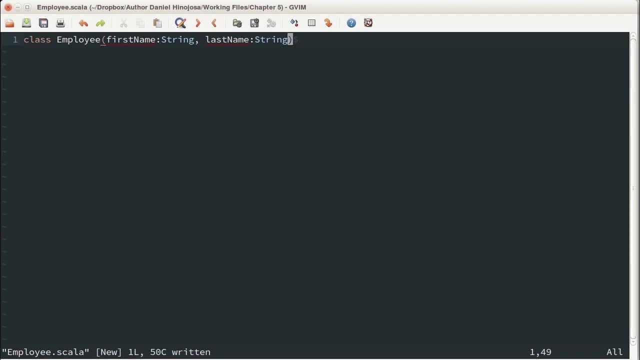 reason: everything in Scala is already public. therefore, the public keyword is not required. how does this look in the JVM? well, let's compile this, just make sure I save it. let me go over to the command line. here I am in the command line and I'm going to compile. 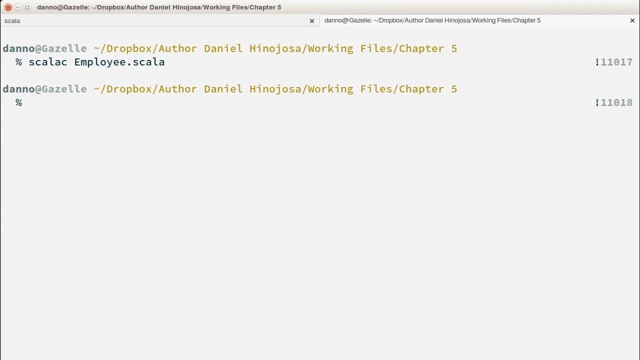 employeescala. now let's take a look at the bytecode using command called Java P. this comes from Java. this does not come from Scala itself. Scala C created a class file. in fact, before I even create this, let me just do a directory search, as you can see. 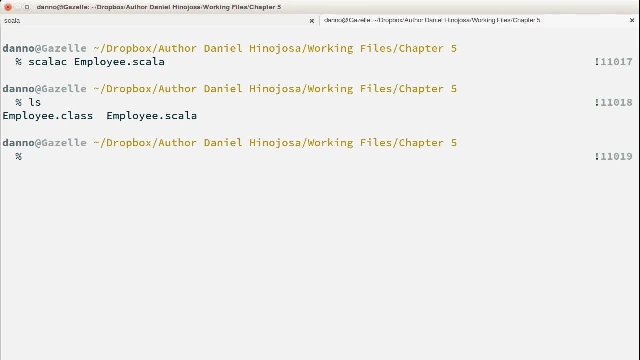 here we have an employeescala class, so I'm going to invoke Java P, dash P and the name of the class, and this shows what the Java equivalent of the Scala code looks like. if you ever need to see what Scala is doing, Java P is an excellent tool. the dash P that. 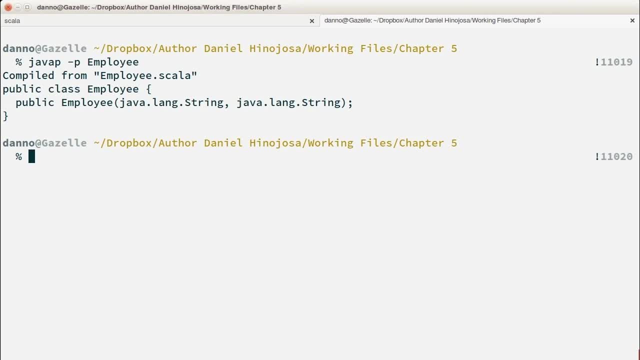 you see there stands for viewing the private member variables in the equivalent Java code. take a look at the constructor right between the braces. that's the constructor. it's called a Java constructor. it's called a Java constructor because it happens to have the same name as a class. 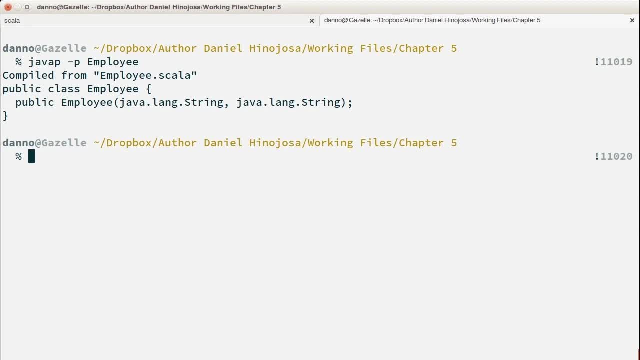 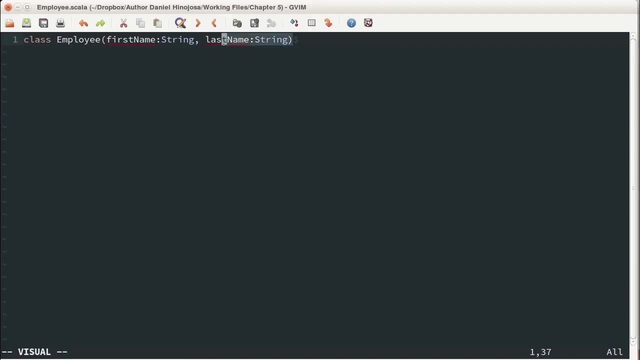 it's fairly interesting. it has a constructor that takes two strings. but where did we create that constructor? well, let's go back to our service code and look at that. the constructor happens to be right here. this is the primary constructor. constructors are quasi methods. that is in charge of setting up. 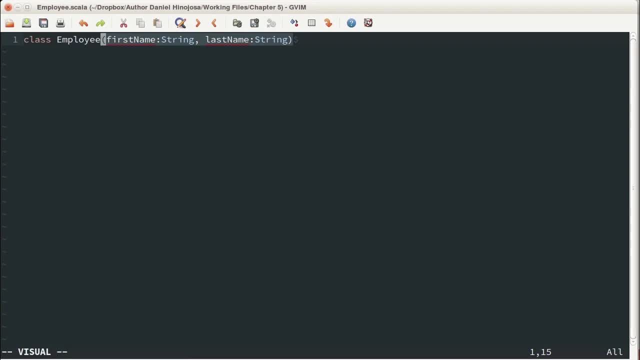 the state of the object. whenever we instantiate the object, it is the constructor that's in charge of setting up that state, as opposed to other programming languages that typically favor an empty constructor as the private constructor. Scala's primary constructor- the one you see here- is big and needs all the 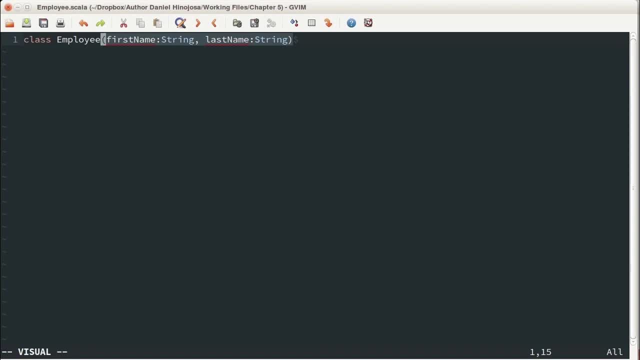 information. the reason: immutability. when Scala programmers change data, they usually get a copy in return, and sometimes copying can come at a price, and that price is memory. in order to avoid excessive copying of objects, we create objects by providing all the information to the class up front. 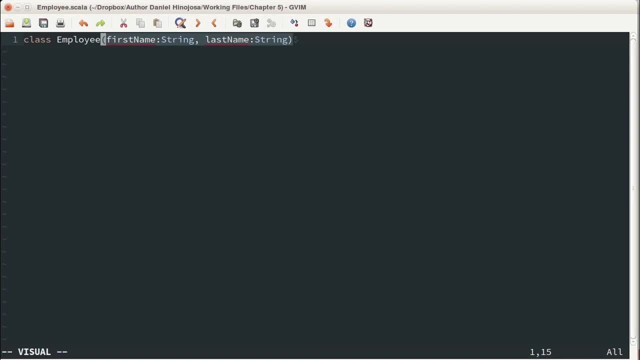 so, given this, now let's instantiate a class through the script. I'm going to create a file called employee script, dot Scala, and in this script I'm going to instantiate the employee object. and I'm going to instantiate the object with the very first computer programmer. let me add a print line. 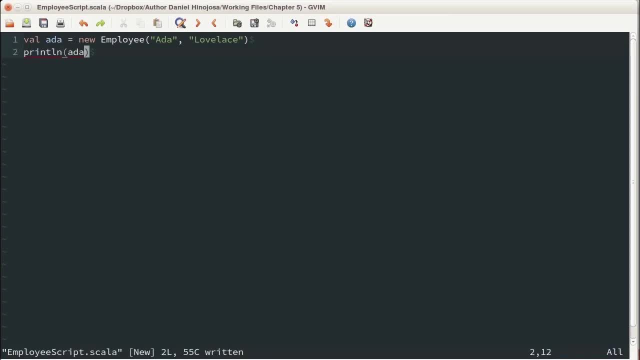 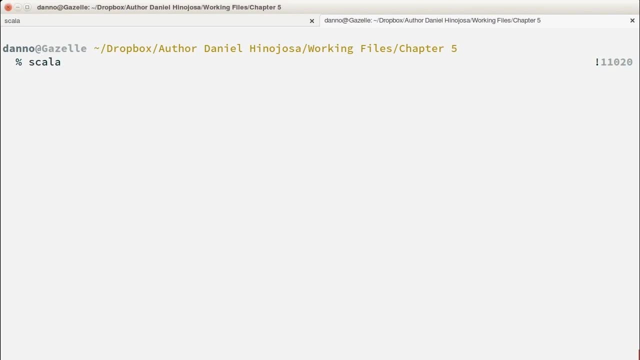 to make sure I have this correctly, and I will go ahead and save this. now let's go ahead and run it. I'm going to invoke Scala, just like I have done in the past with all these scripts that I've done, except this time I'm going to provide a switch. 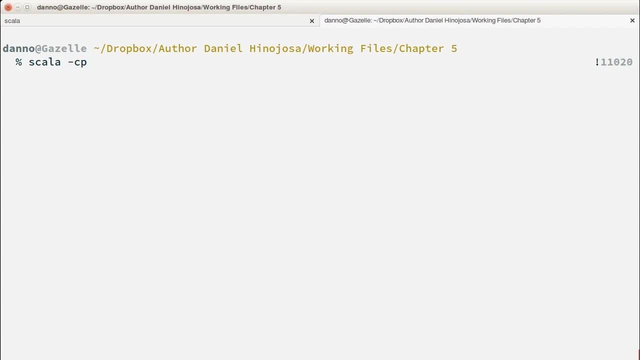 called class path and I'm going to state that in this directory there is a class that interests me, namely employee dot class that I wish to use in my script and we get the employee. now. if you're unfamiliar with JVM programming, this is the default to string. we'll correct this. 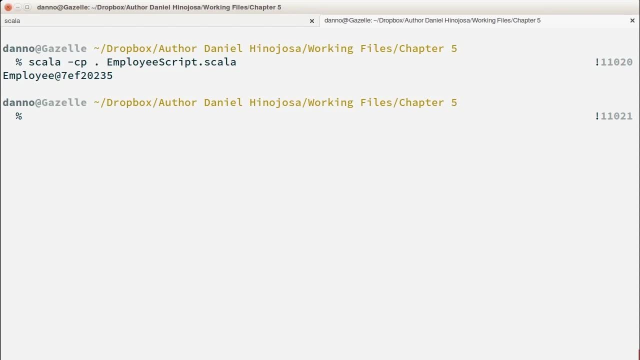 a little bit later. but we get the employee object in return. now what I'd like to do next is I'd actually like to get the first name out of this particular employee. let's give that a try. go back to our code. so, inside of the script, I'd like. 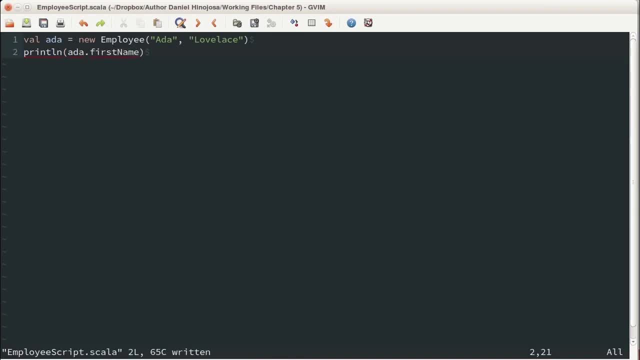 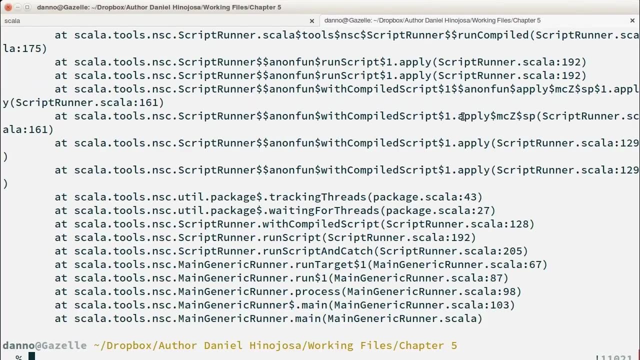 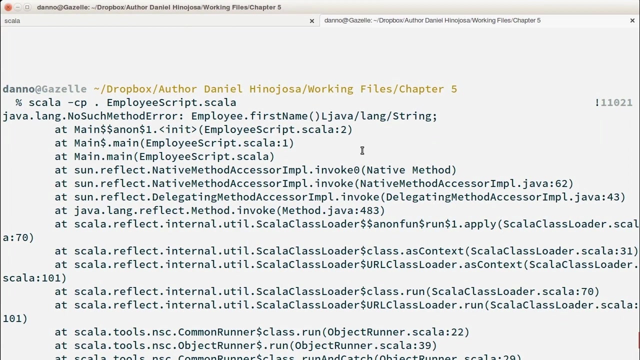 to get the first name. this is an accessor in Scala. it allows me to access the information within the object. let me go ahead and save this and let's run it and we end up with a big stack trace and this states here that no such method error employee dot first name. 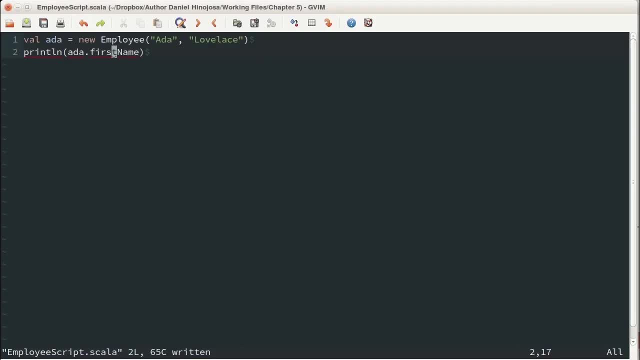 does not exist, so let's go back to our code. and first name does not exist, but believe me, this is an accessor in Scala. this is the way we access information for the Java people. you may be a little bit startled by this. why am I accessing the field directly? 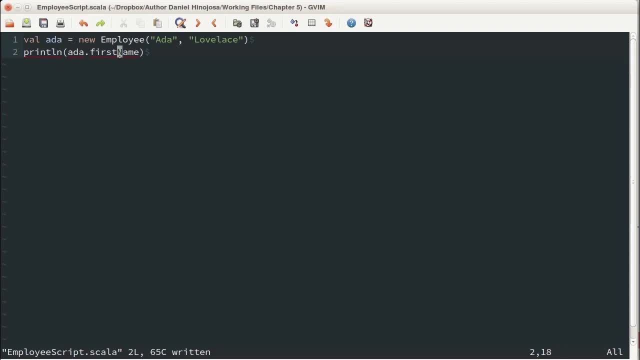 I'm not, nor am I trying to do so. accessors are not in the same style as in Java, also known as getters. you merely call the method, as it has the same name of the member variable. in other words, the method name and the member variable are the same. this is what's called. 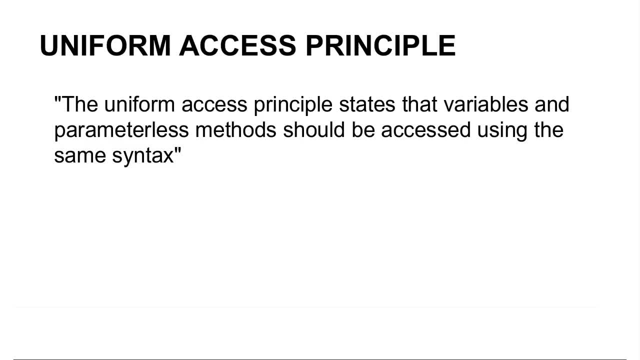 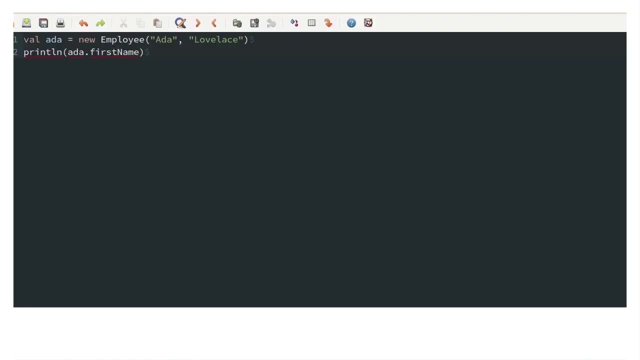 the uniform access principle. the uniform access principle states that variables and parameter list methods should be accessed using the same syntax. in other words, the field and the getter are going to have the same name. let's go back to our code, so simplifying that uniform access principle. that means you. 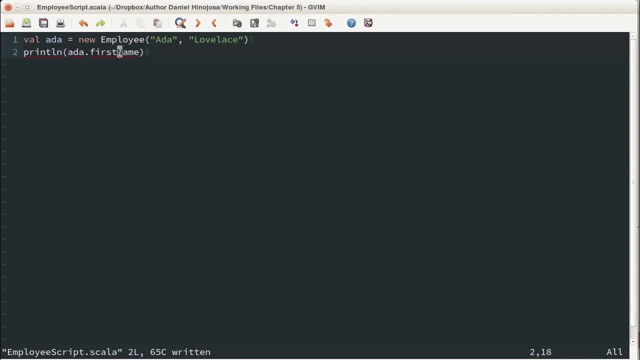 don't know if you're accessing your data directly as a field or from a method. benefit of that is that you can make changes without adversely changing how people interact with your code. to make this work, we need to add an accessor, and we do this by putting a val in front. 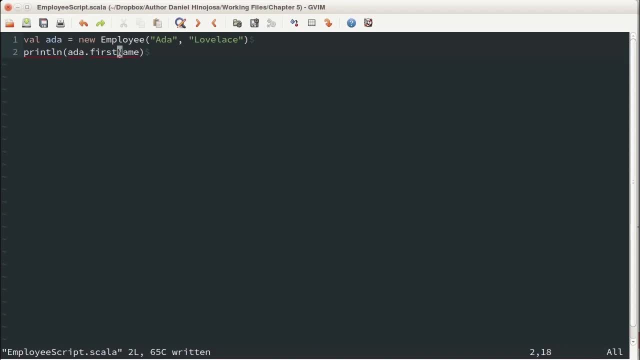 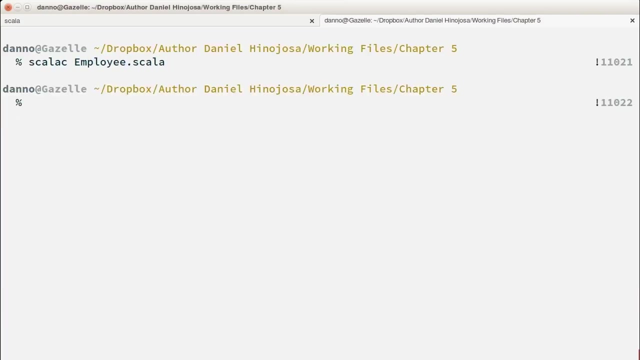 of the constructor parameter that we need to access. so let's go back to our employeescala and in front of the member variable for first name, I'm going to include a val, I'm going to save it and compile it. now I'm going to run our script. 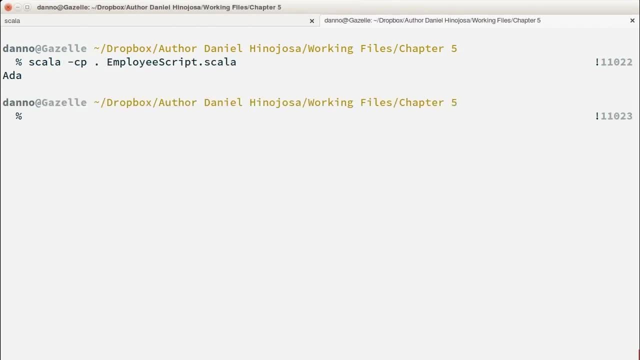 and we get in return Ada. this looks fantastic. so what happened? well, let's take a look at the bytecode. remember our bytecode. in order to take a look at our bytecode, we're going to use java p, dash p and our bytecode says: well, you have a private member variable. 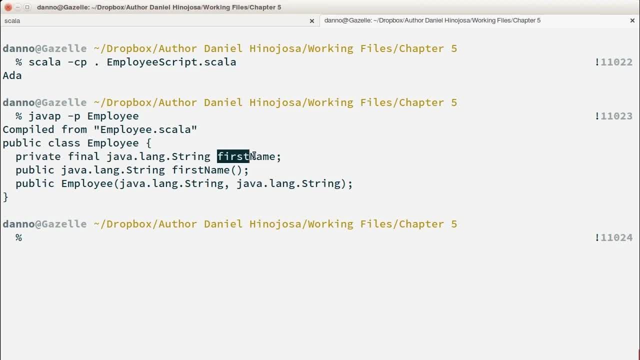 happens to be final because it is a val, and the name of the private member variable: first name. the name of the method: first name. this is the uniform access principle. the return type for this method happens to be a string. let's take a look at the employee script, that's: 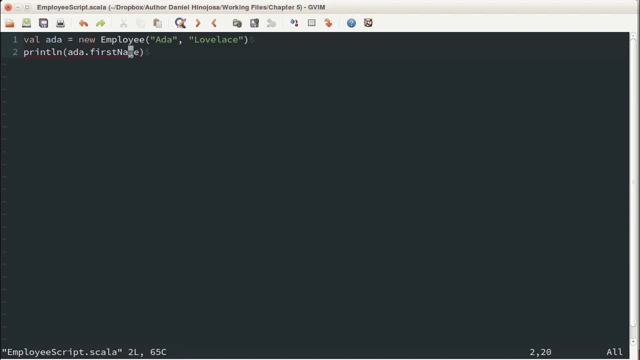 why, when we access this, we don't know if we're actually calling the method or the private member variable. so this worked out great. now you could probably imagine what happens when we add a var. so let's give this a try. so for last name, what I'd like to do in this example: 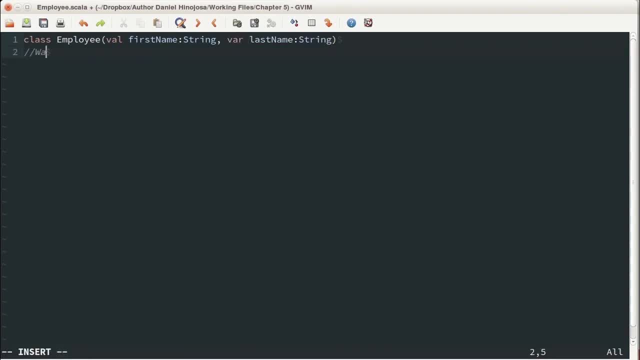 is make last name a var. now let me place a warning here. it's worth emphasizing this again. we particularly don't like vars, but we're just learning right now, so let's go ahead and create the last name as a var. this generates a Scala mutator. so let's go back to 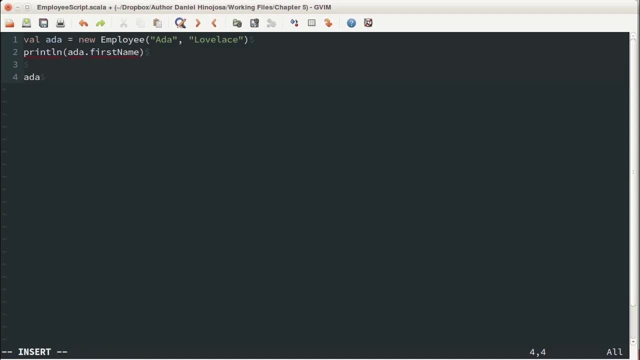 our script and mutate the employee we'll call Ada. last name is equal to: and let's give Ada Lovelace her full name, Ada Byron, Countess of Lovelace. this is the way we change our object, so we're changing Ada Lovelace's last name. 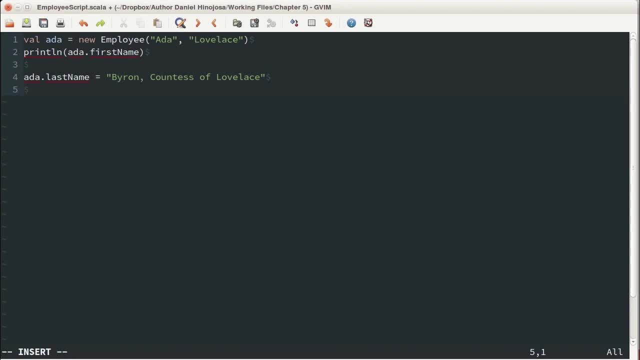 to Byron, Countess of Lovelace. let's do a print line to see if all this works, and I'm going to print out the last name. var works as both a read and a write. everything that is writable is also readable, so if you put it as a var, 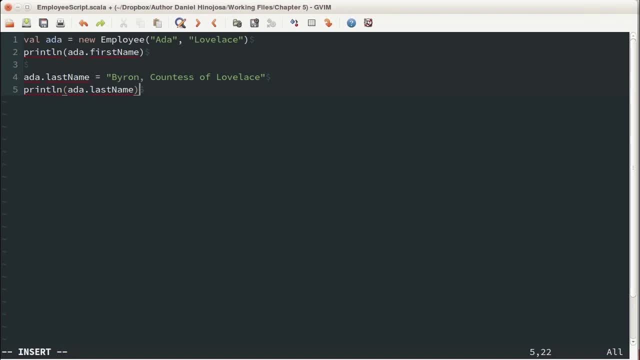 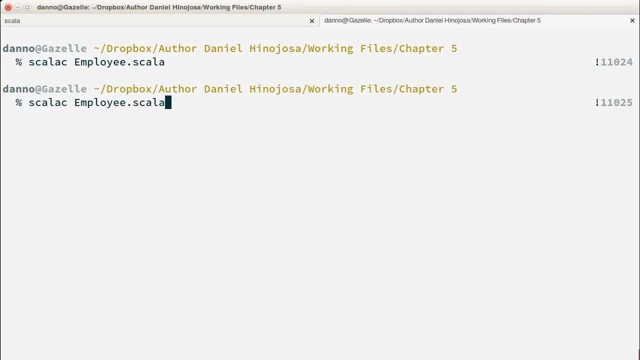 that means not only can you set it, but you could also read it. let's save this and let's run it. first off, let's compile the code, then let's run the script. we're able to see now that we can change the last name, and we could. 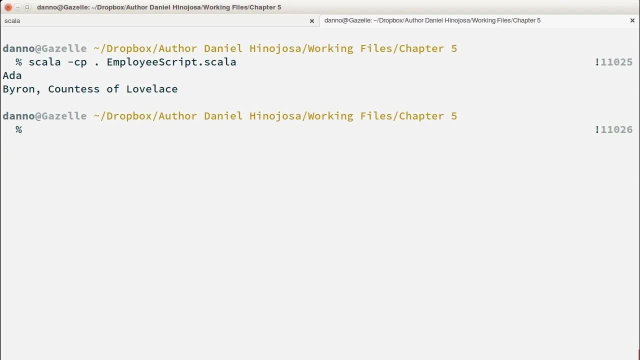 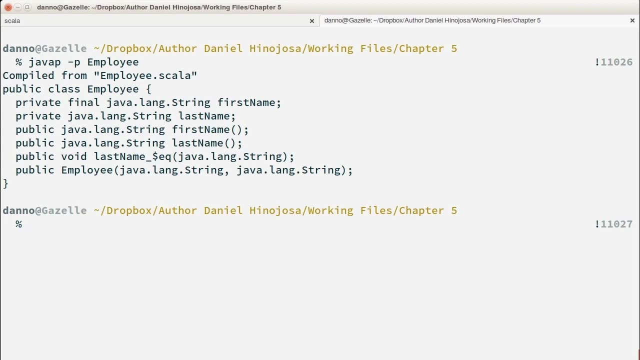 do that because we listed last name with a var. let's take a look at the byte code again. things have changed, though let's see what we have. this contains a method def last name, which is the method where we get the last name, but def last name. is this method right here? 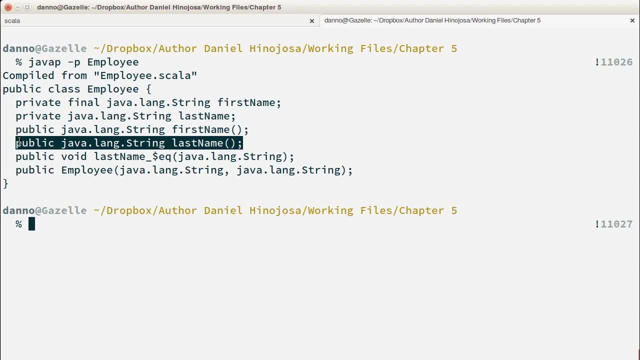 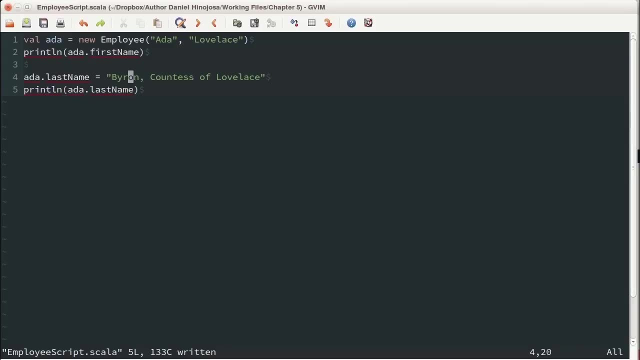 just called last name, which returns a string. but we also have another method, killer one too. this is right here. public void last name underscore dollar sign eq. this is that equal that we used to set the last name. let's go back to our code so you can see that here it is right. 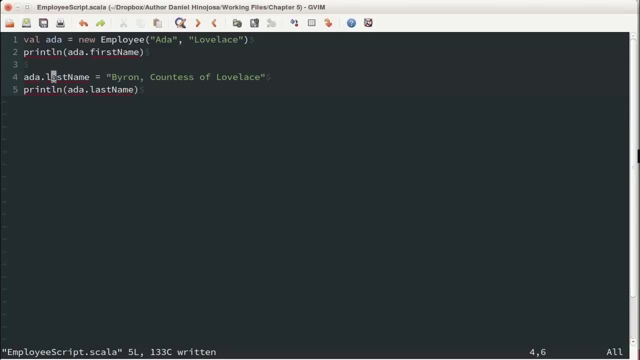 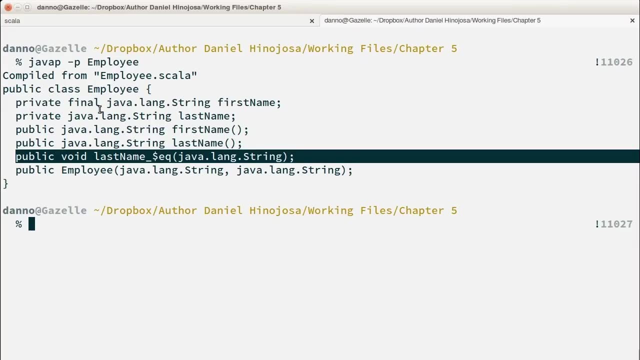 here. this is that equal that we're referring to. so this is actually a method, a method called last name, underscore eq. let's go back to the command line, and this is what we're actually using. remember that once the underscore is established, you could add any character that you want. 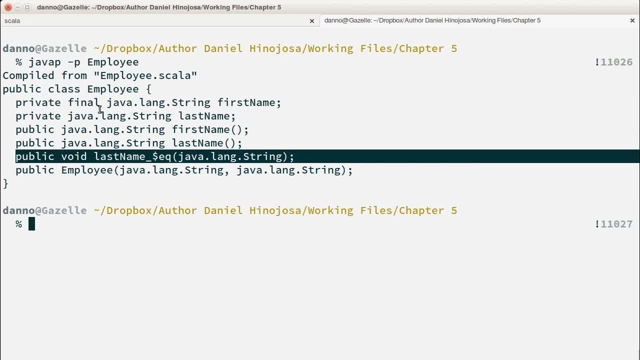 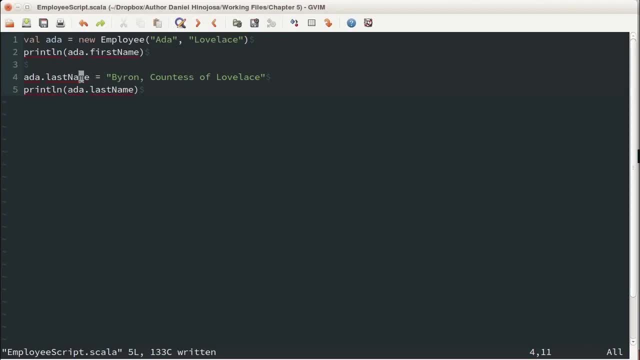 the Scala compiler will just go a little bit further and name your method with an underscore- equal- and you can call it without the underscore. so let's go back to our script and this is the equal that we're referring to. it's very important to note that. 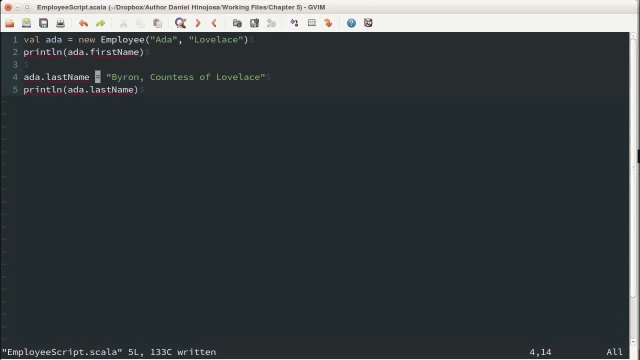 Scala programmers rarely use var again because we prefer immutability in all our code. it's very typical for us to use val consistently, so let's go over to the REPL. try something else out. so this is the way that we typically do things we'd like to. 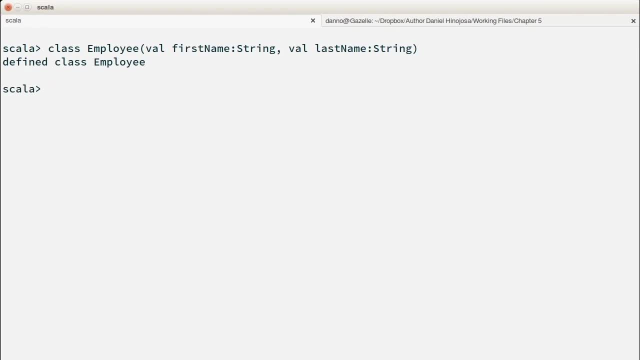 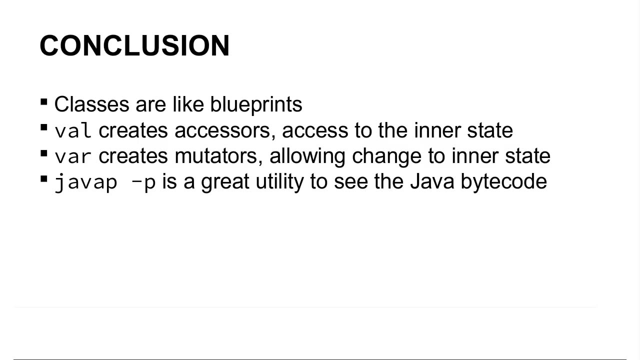 have vals for each member variable. if all this seems like a lot of syntax sugar, it is may look like it, but this is actually common form. so, in conclusion, classes are templates or blueprints. val creates accessors methods that will allow us to access the interstate var. 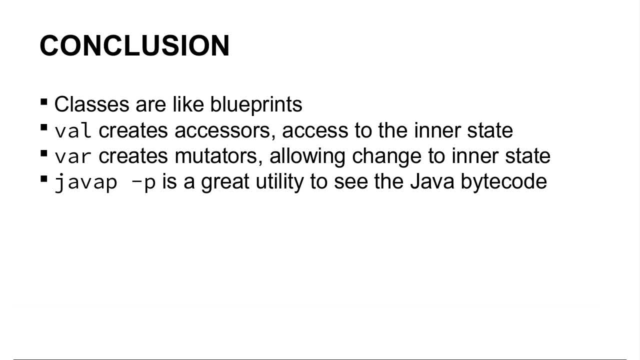 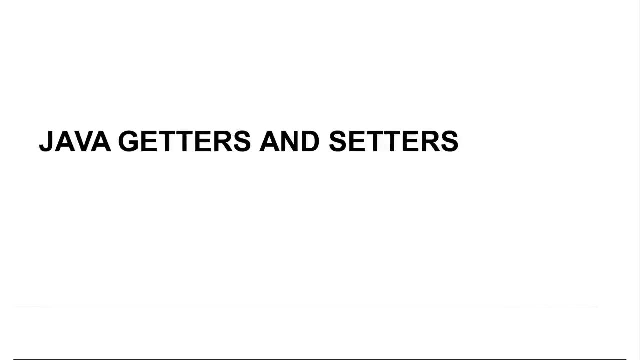 creates mutators and accessors. mutators allows us to change the interstate. very important to note. we rarely use var. it's also worth to note that java p space dash p is a great utility to view how Scala compiles to java. in the last session we created a class called 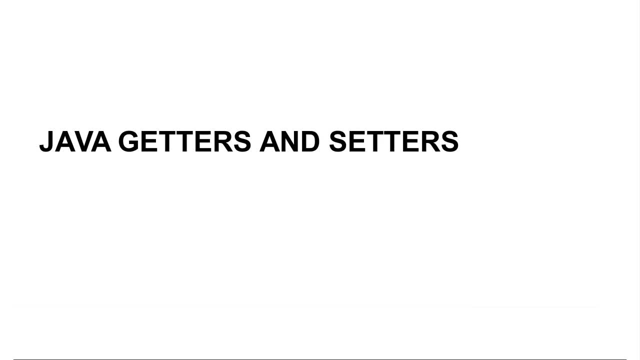 employee in that class. we also had accessors and mutators, and accessors a method to obtain the internal state of an object, and a mutator is a method that can change the internal state of an object. those forms, though, were unfamiliar to the java programmer, since the java programmer 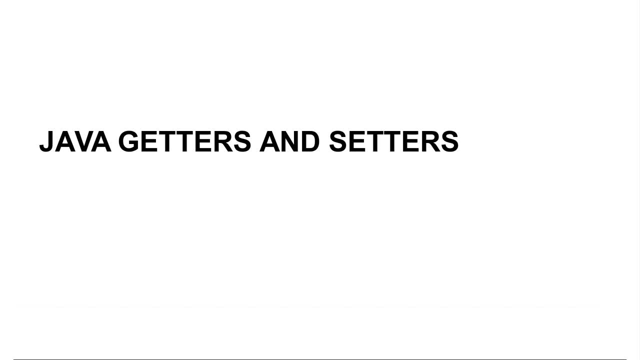 deals with what are called getters and setters when it comes to integrating their code into a java framework. in this session, we're going to talk about creating java style accessors and mutators called getters and setters, and when we do so, those getters and setters will coexist. 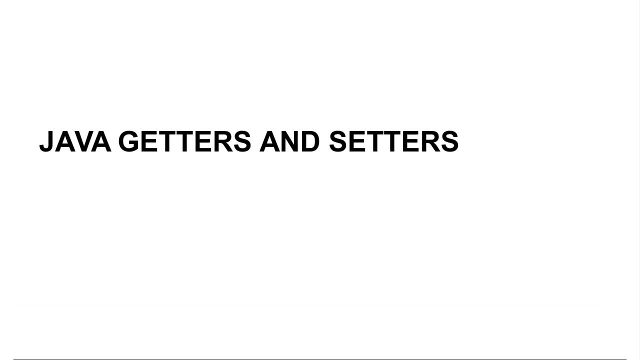 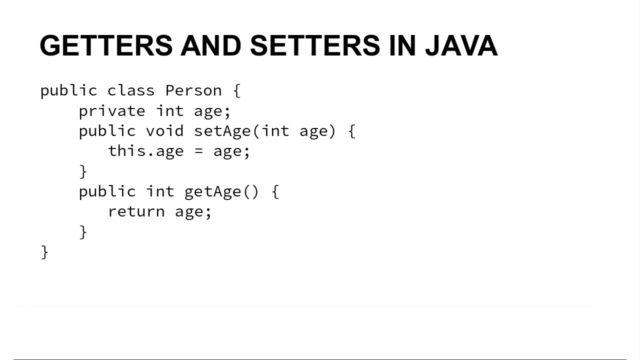 with the Scala accessors and mutators that we already have. we start off by looking at an example of a getter and a setter in java, using an example class called person, and here it is given a property age of primitive int. the java bean convention is that in order to access the property, 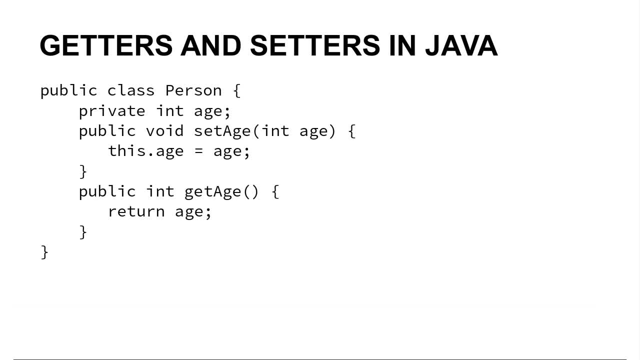 you provide a getter in the form of get age and that is the method down at the bottom: public int get age. internally, we are returning the internal state. we are returning the parameter int age for a mutator. it takes the form of set age with a method: parameter of age. 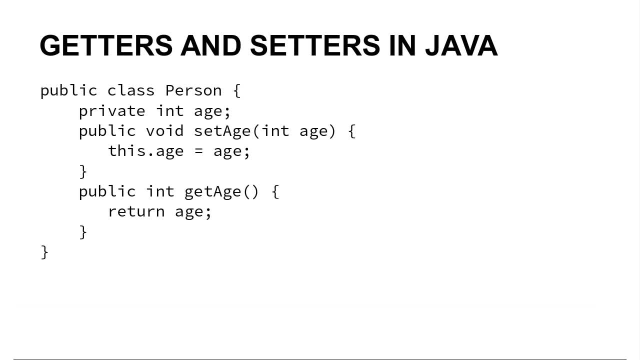 public void. set age again. method parameter: int age. once we obtain this age via the method parameter, we are going to set that to the internal state, calling this dot age and setting that to what comes in from the method parameter, the private access modifier on what's called the member. 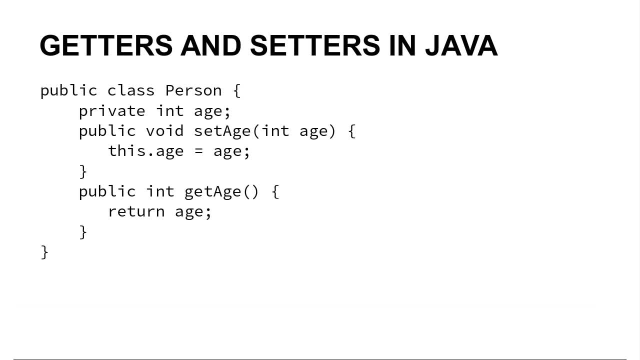 variable private int age close to the top of the class. declaration states that direct access to this field cannot be done from the outside of the class. i did say class and not objects, since objects that are created from the class can access each other's private fields, and 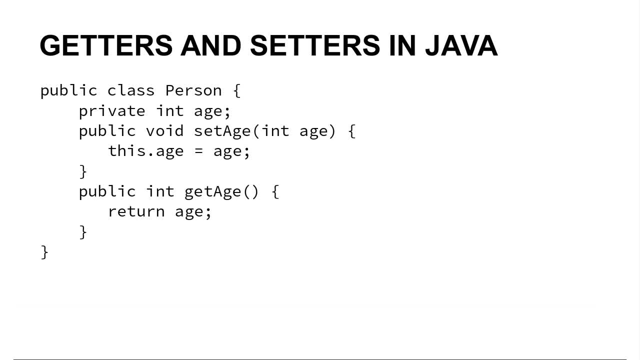 methods now, because we love java and because we are aware that we have to interact with java frameworks, since java is so dominant in the enterprise. there is a quick way we can get these creators and setters in scala, and that is done using an annotation called bean property. the bean property annotation. 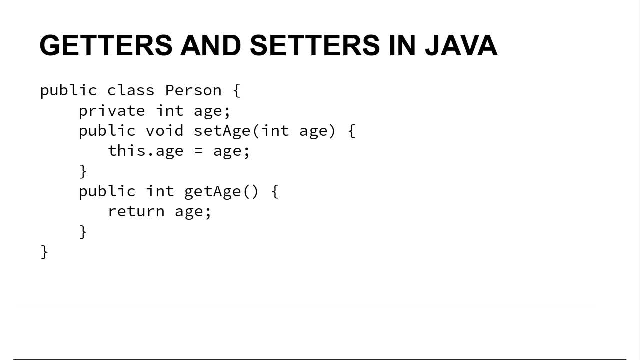 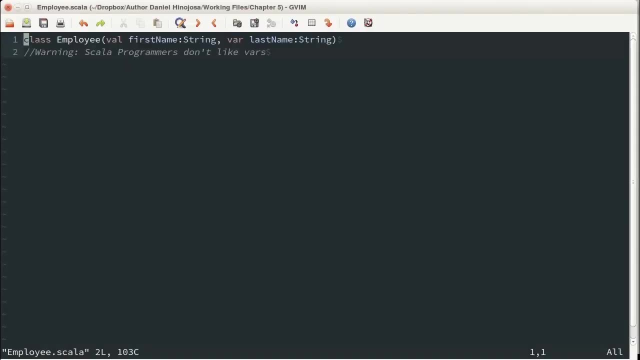 comes from the package scala dot beans, dot bean property and when applied to the property name of the primary constructor, it will create a getter or a setter, depending on whether the property is a val or a var. let's go to the employee dot scala file that we created. 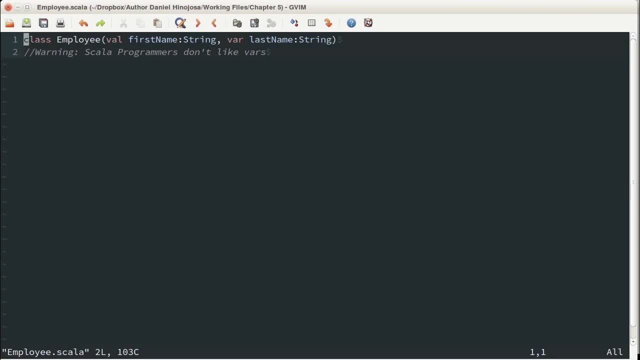 in the last session. here it is class employee val, first name of type string and var, last name of type string, the comment here stating that scala programmers do not like vars and particular. but this is a learning video series, so we will just keep that in there. we will now import. 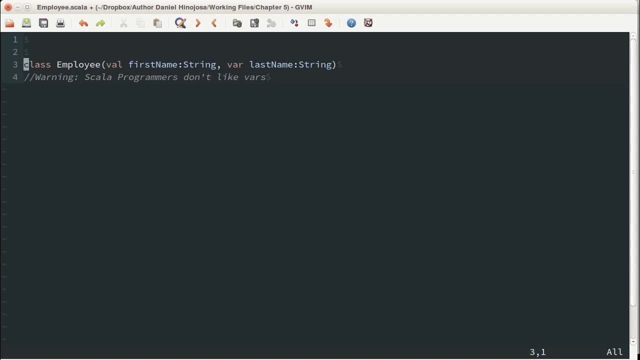 the scala beans bean property annotation, so that way we don't have to litter our class with fully qualified names of our annotation. now that we import it, we can apply that annotation on the property that you need a java style getter and setter for. but let's try this. 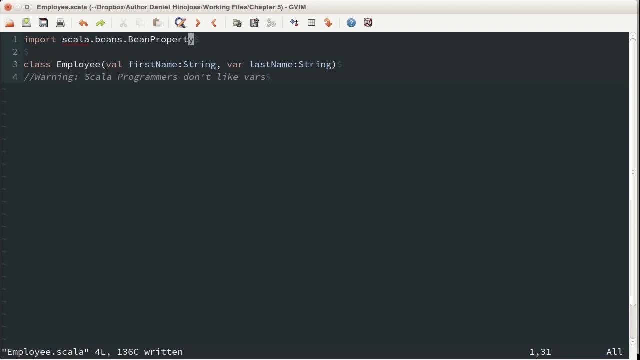 a property at a time, by applying it to the first property first name and using java p to view the outcome. all right, so we applied the bean property annotation to the first property first name and we're applying it right in front of the val. now let's compile it and 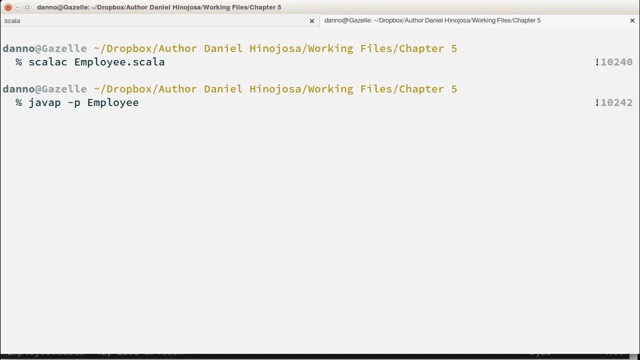 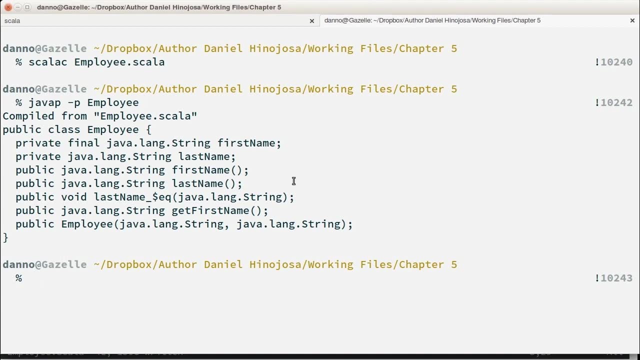 now let's run java p space dash p on the employee class. we then see that there is a getter for first name in the java format, and here it is: also note that the first name property only has a getter. there isn't a method in here called. 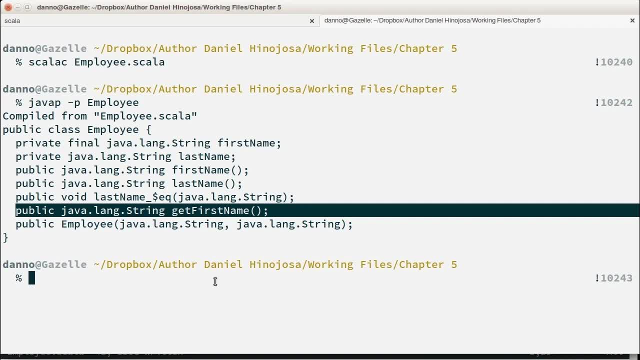 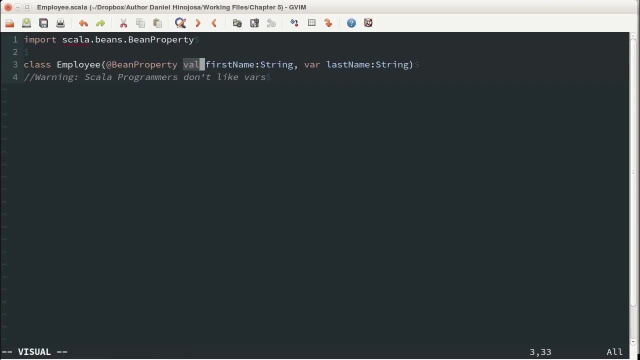 set first name, and the reason is, of course, is that the first name property has a val. let's go back to the source code again. this has a val and not a var and, as we know, val means that once it is set, we can no longer change it. so it stands to reason. 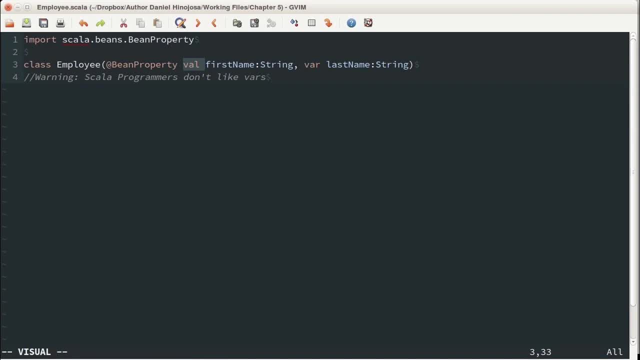 that, since we can't change it, there will not be a setter. now, since we're back in employee scala, let's add a bean property to the last name property. this time, though, it has a var and not a val, so we should expect that last name will not only have. 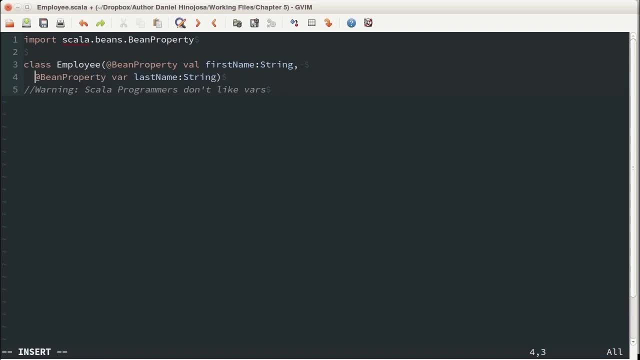 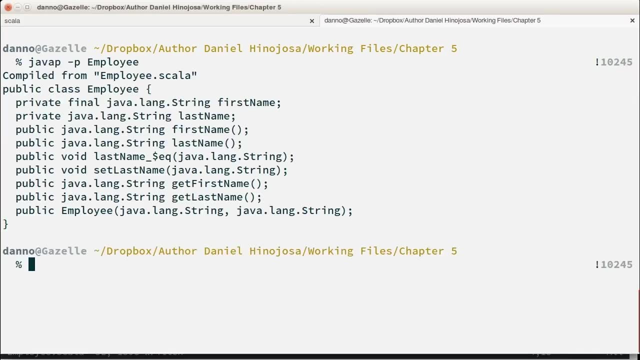 a getter, but a setter. if you want to make this cleaner, you can put a new line inside of the primary constructor. let's compile it and view the results with java p. alright, so here we go. this time we have a getter. here's the getter for last name. remember last name was a var and not a val. this is our getter and here it is our java setter: getters when the property is a val and a setter when the property is a var. so, in conclusion, if you need java style getters and setters, use the annotation scala. 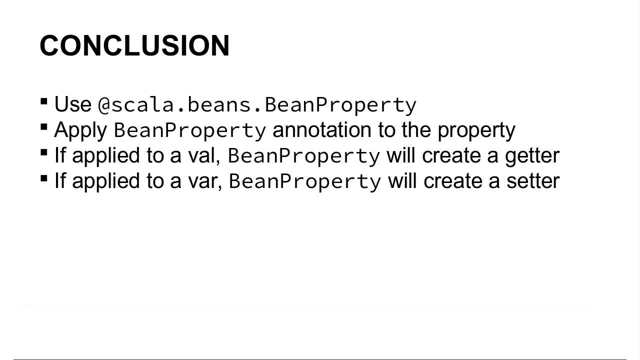 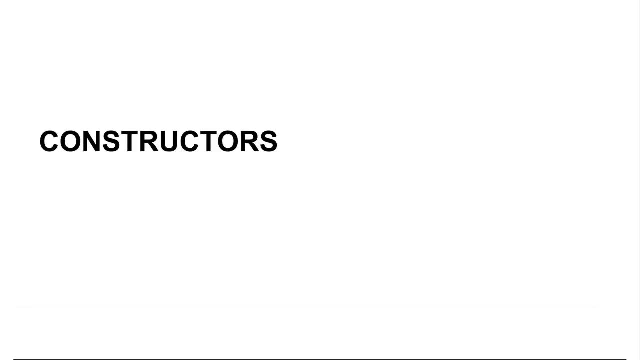 beans- bean property, then you apply the annotation to the property. you need a getter and setter for if applied to a val, you'll get a getter. if applied to a var property, you'll get a setter. in this section we will discuss constructors in scala. constructors are specialized methods. 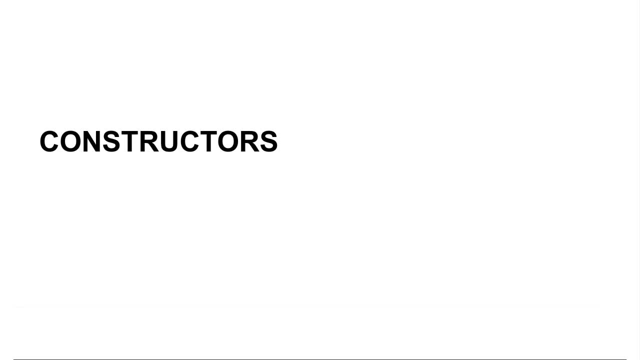 that are invoked to construct an object. it is the primary opportunity to set up state. in our session, we will re-emphasize immutability, revisit the primary constructor and create ancillary constructors that support the primary constructor. so let's get started by reopening our employee class that we created in our previous. 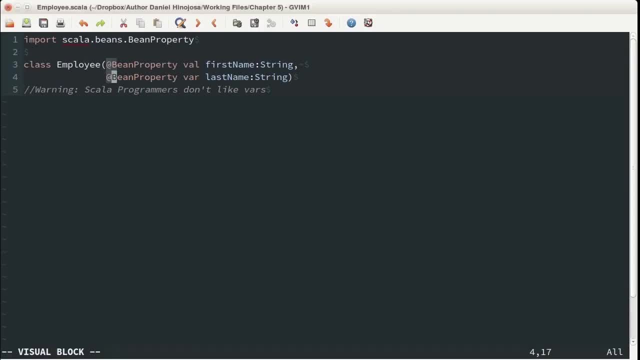 session. what you see between the parentheses is the primary constructor. when we create an instance of an employee, we give the constructor a first name and a last name. let's also open up our employee script that we created in our previous session. here we use the keyword new to. 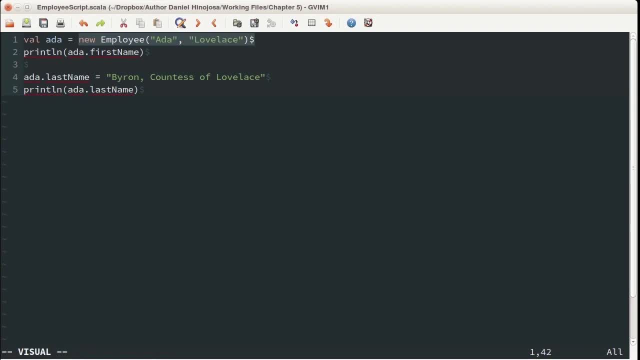 instantiate the employee and we're giving it two items: ada and lovelace, both strings. the first one is the first name, second one is the last name, and this in turn calls the primary constructor. now we know that, because of immutability, everything must be called in the primary constructor, since 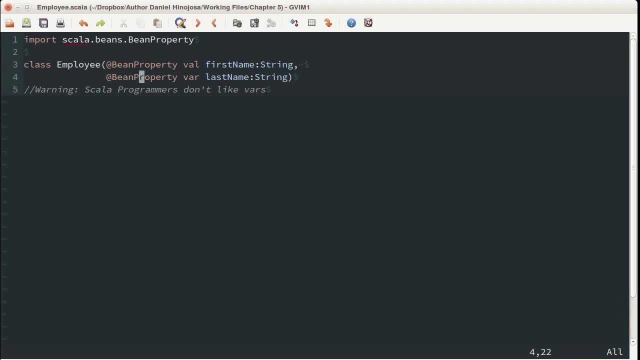 creating an object with little or no information in an immutable language will result in excessive copying and memory consumption. so let's change things up. let's say, for our example, we want to add some new data, a title for the employee. because we made this change, this will affect our script. 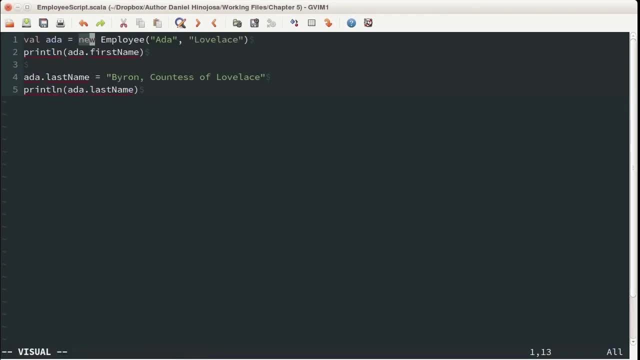 that runs it. let's open that up again. this line right here will cause an error because we're giving it two items, two strings. problem is now because we added the title. we have three items on the primary constructor, two items being given and here we have three items. 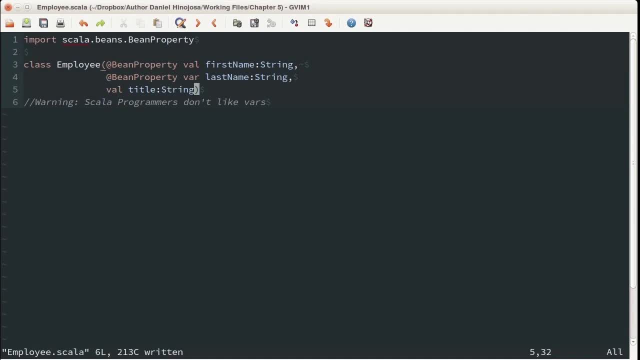 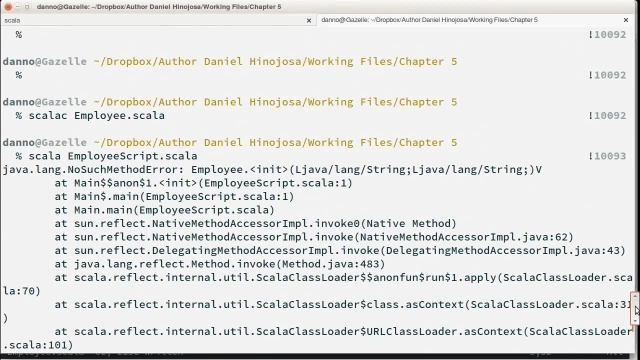 so let's save this, compile it and prove that we get an error. first we will compile our employeescala, now we will run our script. so we get a no such method error because our script is looking for employee, a constructor that takes two strings, but it does not exist. 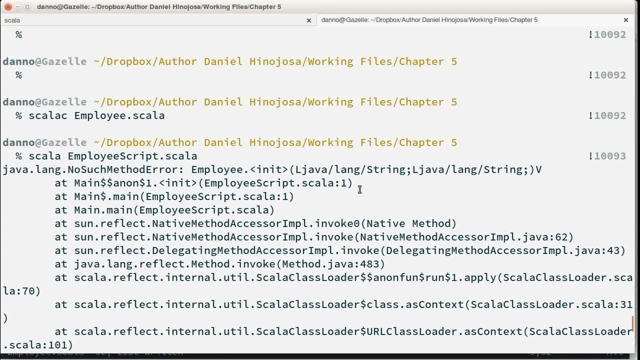 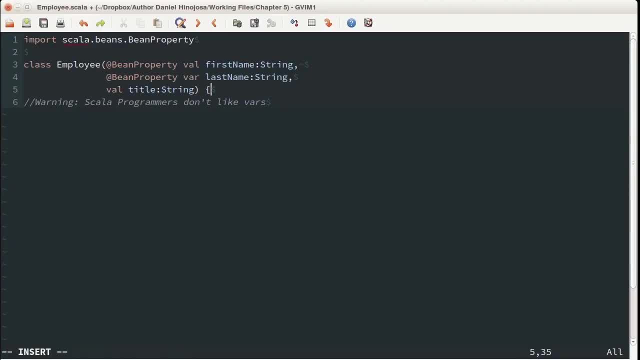 if we don't want to affect other people's code, we can add another constructor, an ancillary constructor, to maintain the interface that others expect. so let's go back to our code and fix it. so I'm going to create a body of the class and I'm going to create an auxiliary. 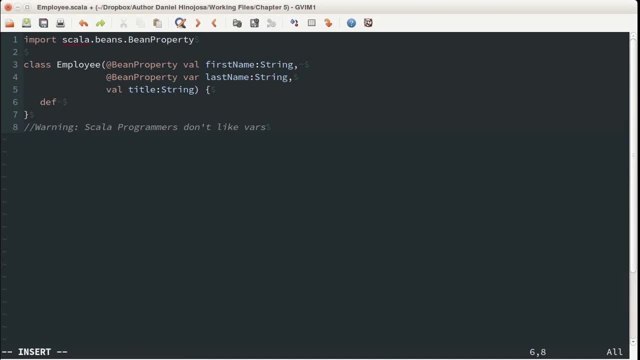 or ancillary constructor. I'm going to start off with the keyword def and the method name is going to be this: it's going to take two parameters. given those parameters, I'm now going to defer this call to the primary constructor. I'm going to use the first name that was given. 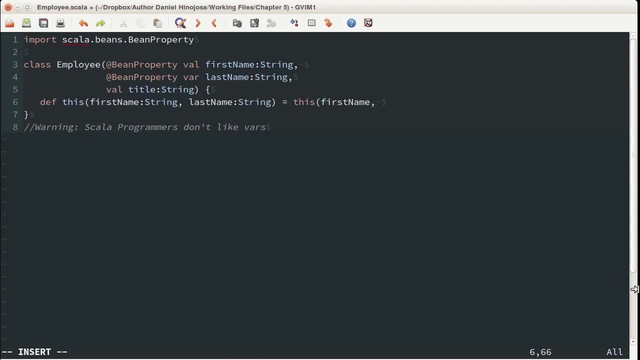 over here. I'm going to give it a call to the primary constructor with that first name and that last name. what am I going to do with the title? well, at this particular moment, I'm going to give it a particular value. the default value I'll choose. 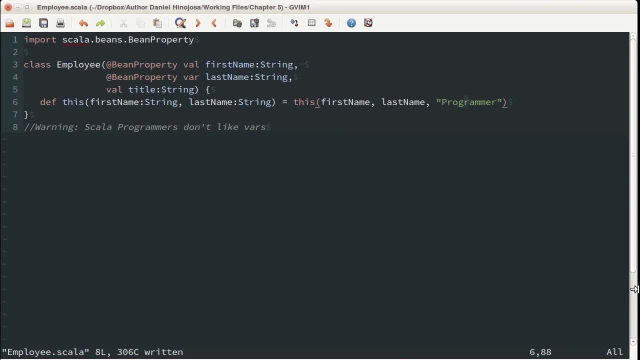 is programmer and we start off with what looks like a method named this. this is no method, it's another constructor. we create an employee object with this alternate form. the word. this signifies that it is a constructor. this is unlike other object oriented languages that use the same. 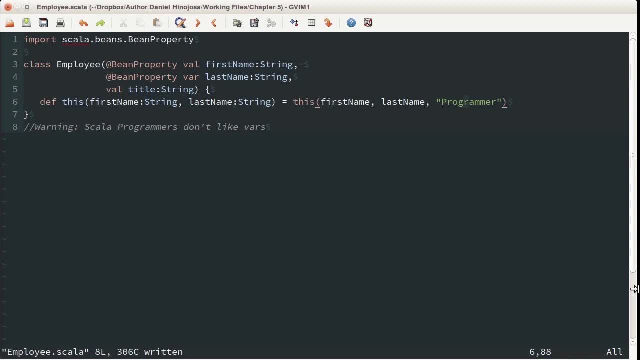 class name to signify that it is a constructor. like a method, though, the constructor accepts parameters, and we are accepting a first name and a last name. once the parameters are obtained, they can be plugged back into the primary constructor by calling this: we'll take those parameters and send them. 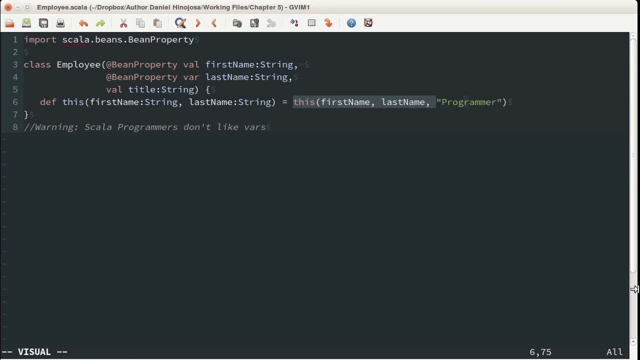 to the primary constructor. notice, though, that because the primary constructor is the dominant constructor, we have to provide a default value for the title. this entire line is an alternate or ancillary constructor. notice also that our constructor parameters are a subset of the primary constructor. ancillary constructors. 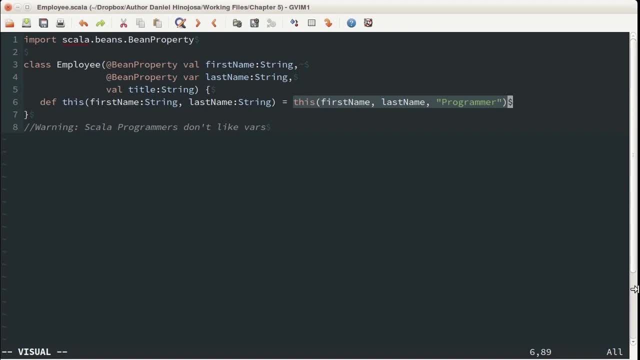 are always going to accept a smaller number of the parameters than that of the primary constructor. as another rule, every ancillary constructor needs to find a way to call the primary constructor. this will look a little bit different than what you're used to, in a more mutable language, where the 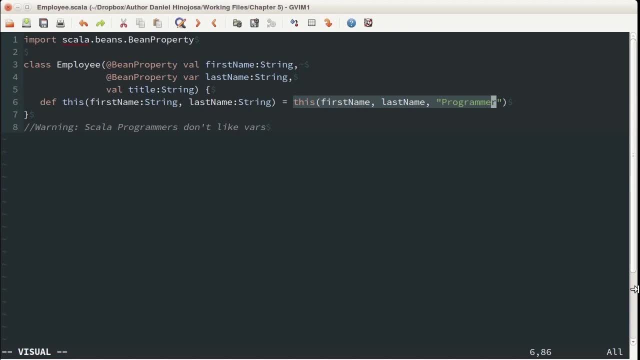 constructor with no parameters will call one of the ancillary constructors with more parameters. this is essentially flipped in Scala. primary constructor is the one with the most parameters. all others must support either directly by calling the primary constructor, or indirectly by calling the primary constructor from one of the other. 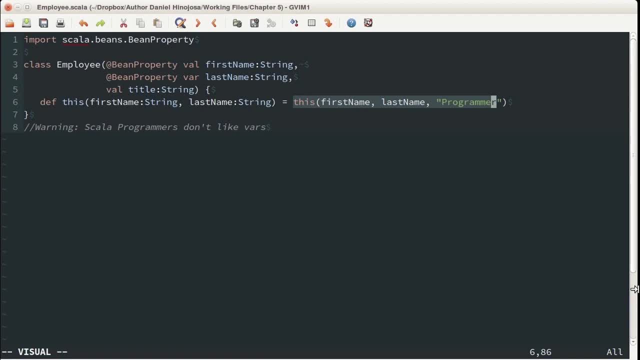 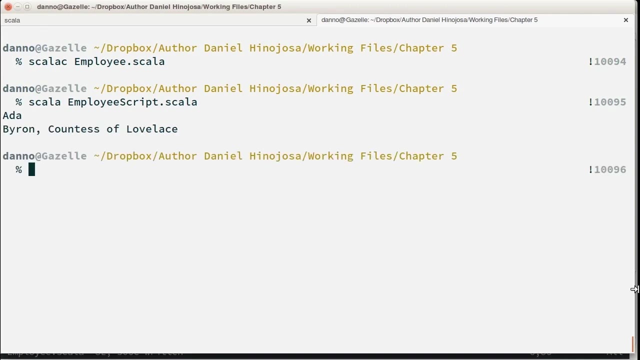 ancillary constructors. this is the typical form of ancillary constructors that we use to call the primary constructor in Scala. now, when we compile the employeescala file and run the script, this will now work. so let's go ahead and write this, compile and run the script. great, now let's go. 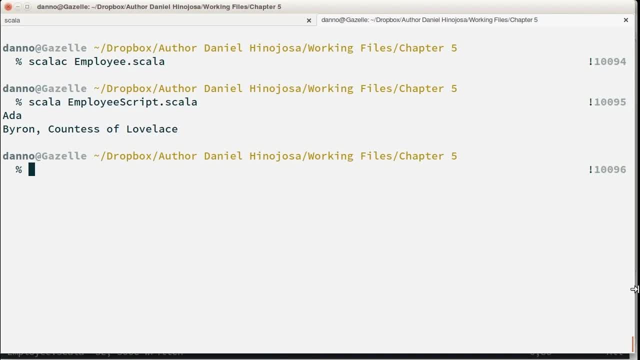 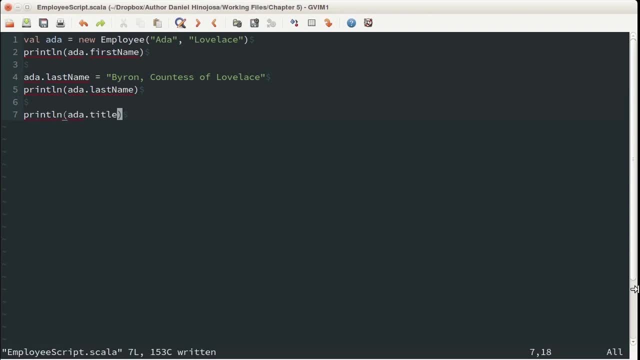 to our script, because what I'd like to see is: I'd like to see what the title for Ada Lovelace is going to be, so I'd like to do a print line again. I did not explicitly state her title. I'll save it now. I'll go to the command line by. 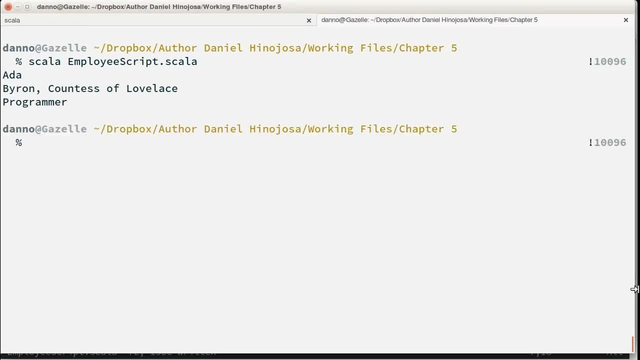 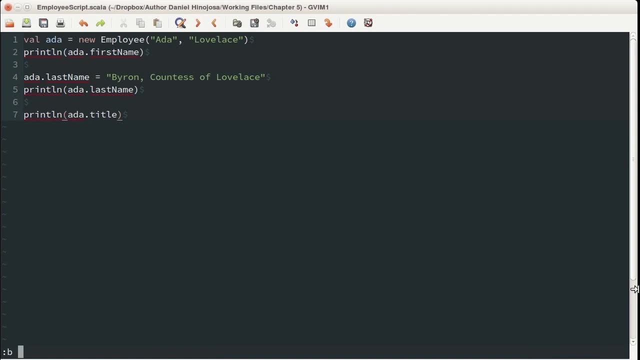 default, she has the title called programmer. now it's worth noting that the constructor can be written in the same way and differently. what we did is the common way. let's go back to our code. I'll go ahead and make a note here. this is the typical form we could write. 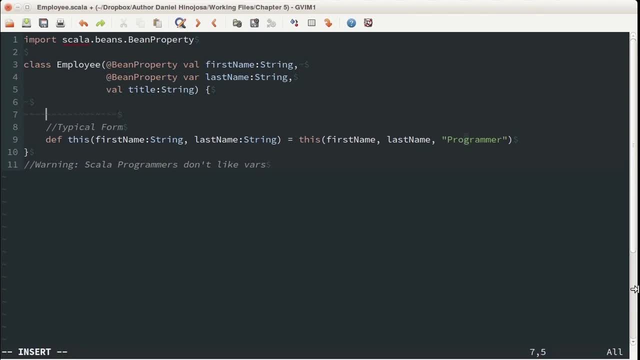 other forms for these constructors, for example. it's going to comment this out and rewrite it in a different form. nearly the same initially, in fact, very much the same initially, except this time we can call it with a block. this isn't too out of the ordinary. let's save it. 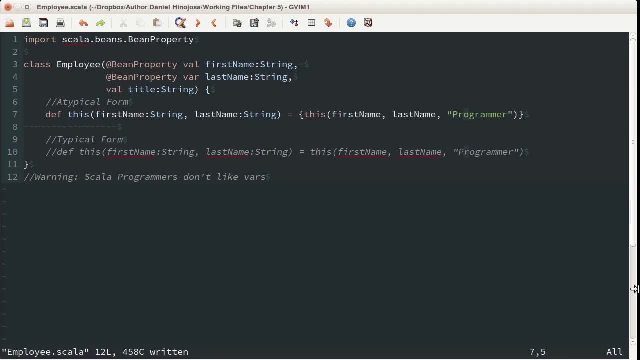 and let's give it a try once again. works out great. let's go back to the script now. let's go back to the constructor and let's go ahead and rewrite it into the code now. what's great about the block is that if you have other statements and you want to, 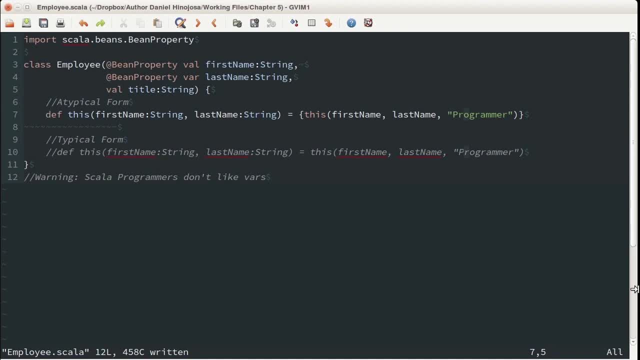 include some side effects. let's say printing to the screen or setting state. you could do so after the call to this, but you do need the block first. anything that is a multi-line would require a block. so let's try another form, this time with a side effect. so here I'll. 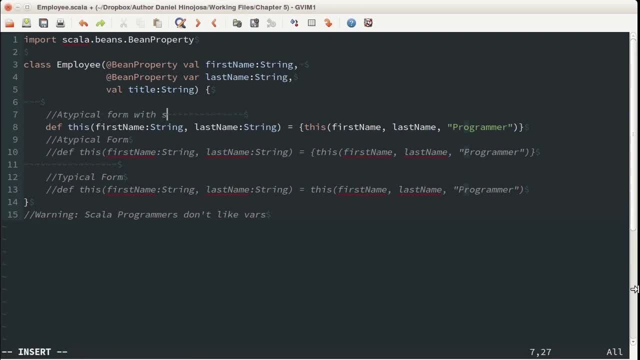 state a typical form with side effect and in this example I'm going to place a semicolon. any time there's a multi-line in the same line, I'm going to put a semicolon and I'm going to put a semicolon in the same line I could use. 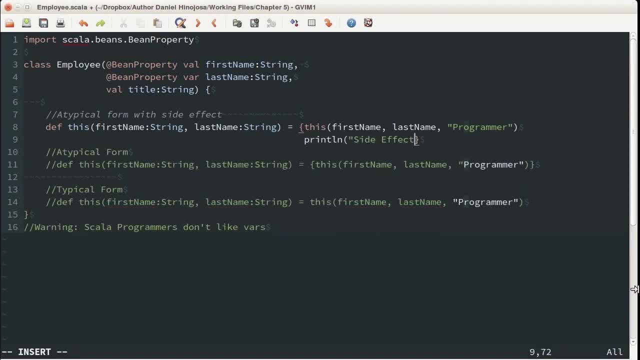 a semicolon, or I can just do my side effect here without the semicolon. okay, now it's worth warning that a call to this needs to be done first. so let's try this code first, and then what we're going to do is we'll flip these lines. 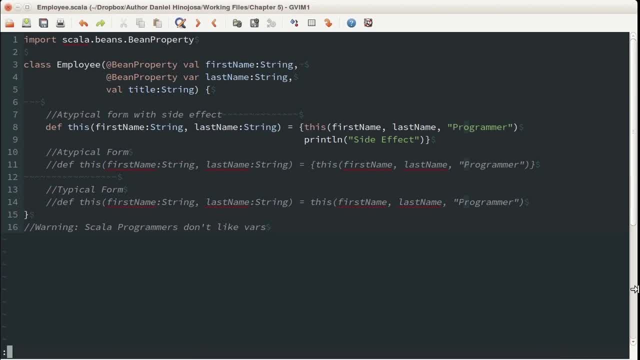 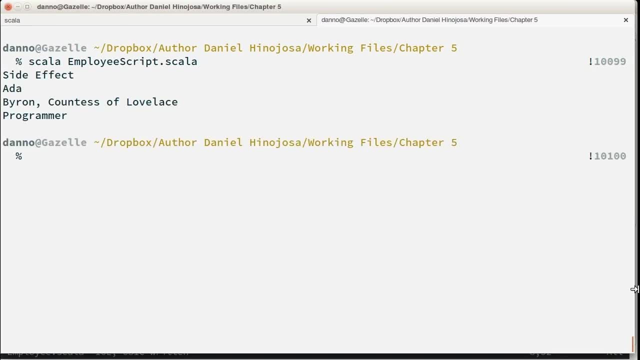 next. so, first off, let's go ahead and save that. I'm going to go over here and just check to make sure that everything will work. here it is, there's a compilation and let's go ahead and run the script, so everything works great, and also we have this side effect. so 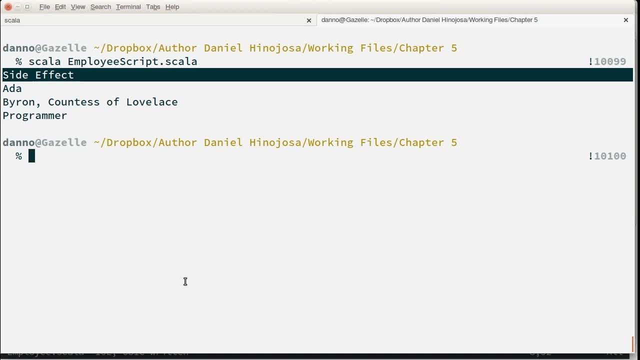 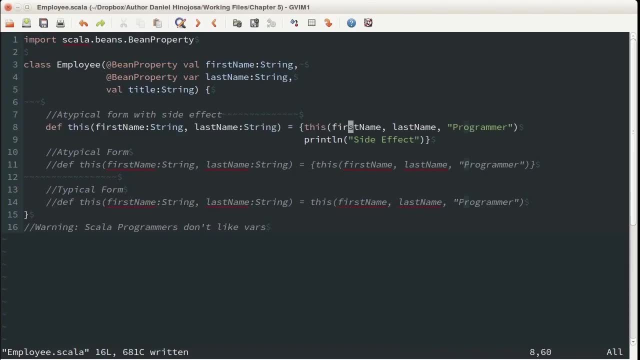 let's go ahead and run the script and see what happens. so, as I mentioned previously, the this call needs to be the first call. if you're going to have other lines within that constructor, let's go back now. what if this was not the first line and the call to this was: 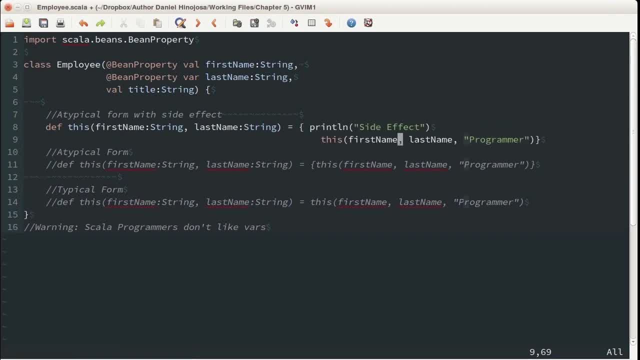 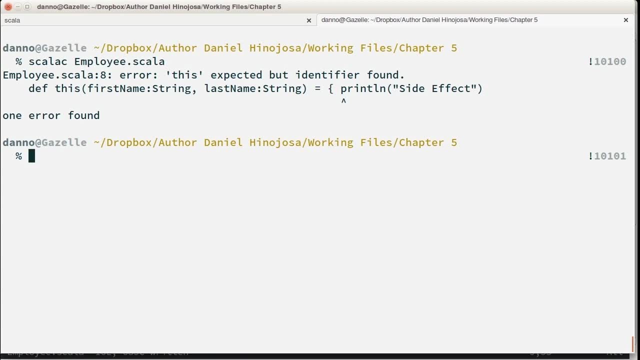 on the second line. the compiler will not allow this, so let's go back to our command line. this will say error. this expected, but unidentifier was found. so let's revert back to our correct state now. in none of these circumstances do you even require a command line, if you. 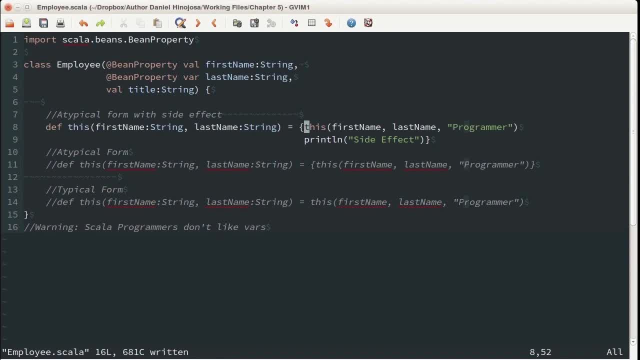 don't require a command line. let's go back to our command line. let's go back here and enter the same code again. this time. here we're going to have two lines. we have a capital letter and an equal sign. I prefer it because it is convention. so the first couple of 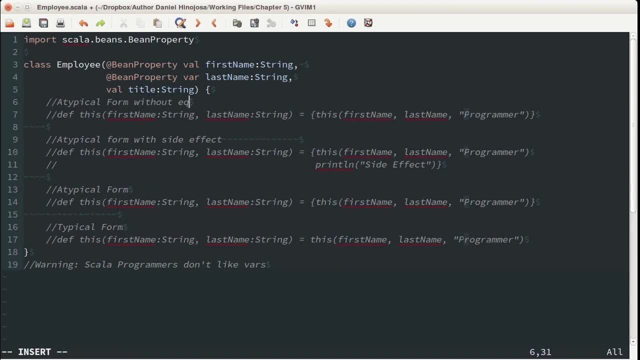 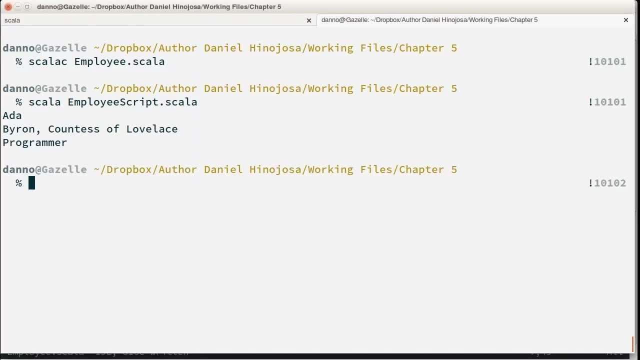 atypical examples, we can get rid of the equal sign. so let's just copy and paste some of these examples and try them in turn. let's try this one, and this would be the atypical form without equals. let's see how this works. saved it, compile it, running the script: everything. 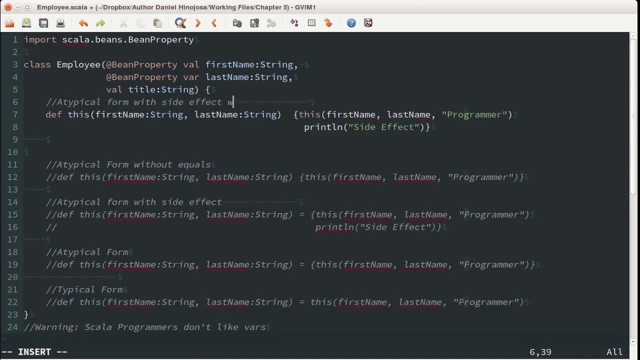 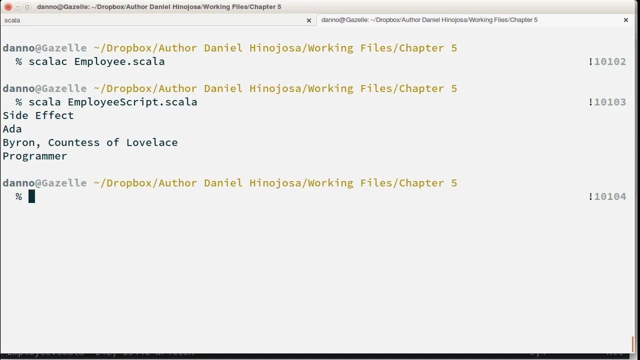 works great. let's go back to our code now. let's try the multi line with the side effect- this time, though, without an compile, and run the script. as you can see, everything works great. now. I'm a sucker for convention. I don't particularly like performing any side effects in the constructor. I'm not going. 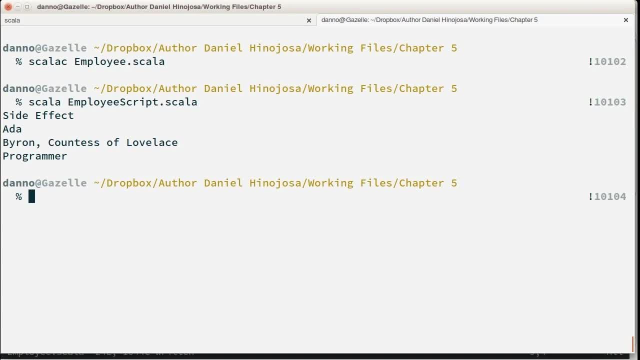 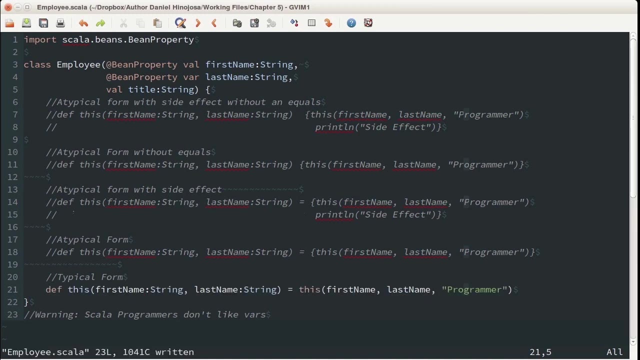 to say I'm never going to do that. there may be a circumstance where I would, but something like that is typically a code smell, so what I'm going to do is I'm just going to go back to the correct form. it is again worth re-emphasizing a few points. one is that the line here, this one that I'm 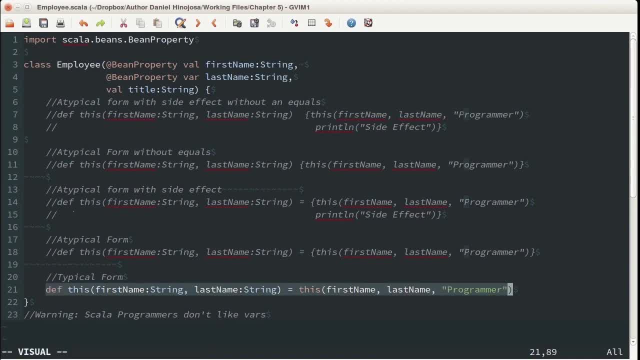 showing you is the typical form and this is what you'll mostly see from Java programs throughout the internet. the other thing is that side effects that you see here are many times frowned upon. we have two different examples with side effects, so that's something that you won't see very much. I 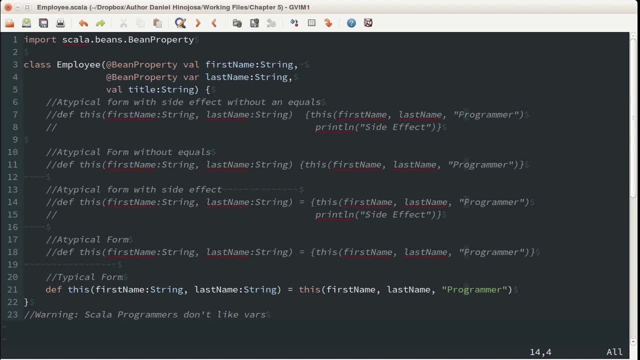 did these examples just to show you the language flexibility purely academic. also, another thing to mention is that when multiple ancillary constructors are in use, you can chain multiple constructors until the primary constructor is called. in other words, if you have a primary constructor and another constructor, we'll call it a and another construct or will call it B. you could have be call a and then a. 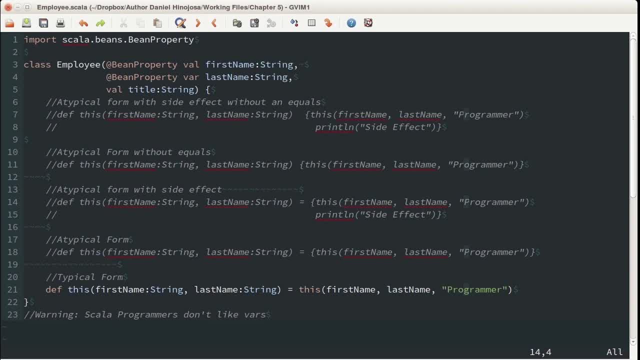 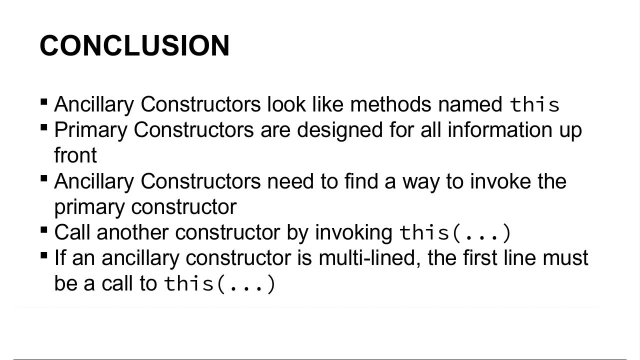 call the primary constructor, although we can force an example here. we have an excellent example for you when we cover options in a few more sections. so, in conclusion, ancillary constructors look like methods named this. primary constructors are meant to ask all the information up front, and so there. 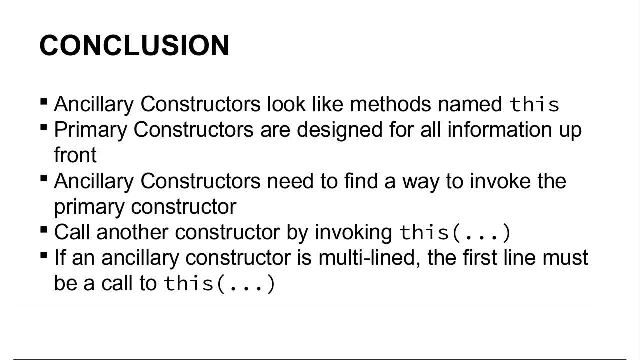 a constructors, once called, need to find a way to the primary constructor, either directly or indirectly. The call to another constructor uses a method. call to this, The call to another constructor, needs to be the first line within the constructor body, otherwise you'll get. 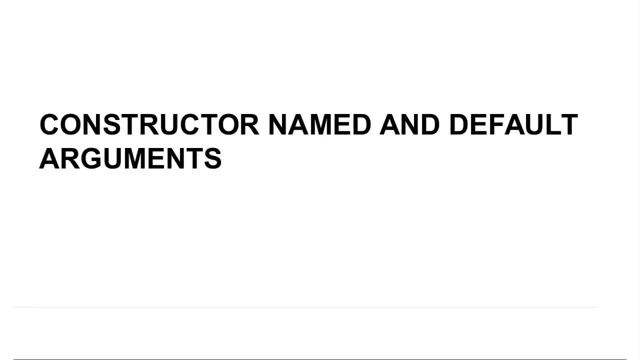 a compilation error. In this episode, we take the knowledge of what we learned about default and named arguments and use them in constructors. In the session Default and Named Arguments, we learned about default and named arguments in methods. This session is to inform you that the same rules 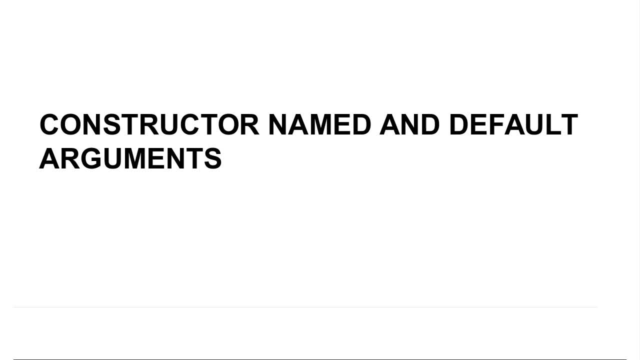 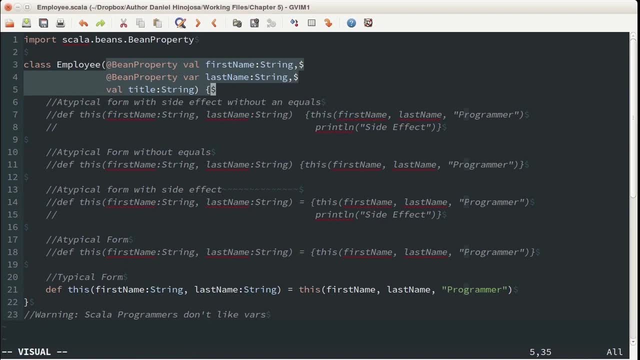 used for methods can also be applied to constructors. Let's take a look at our employee class that we've been working on for the last few sessions. We have two constructors. The first one is the primary constructor. It takes a first name, last name and title. The second constructor is one that takes a first name and a last. 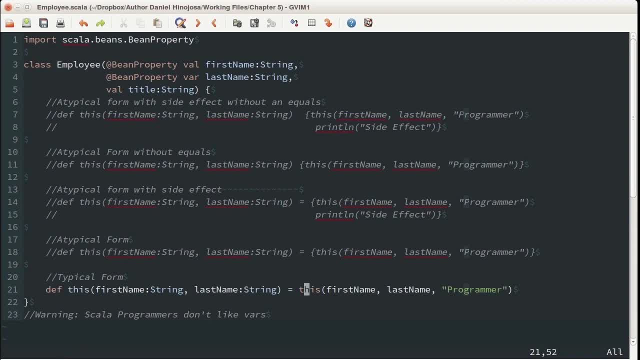 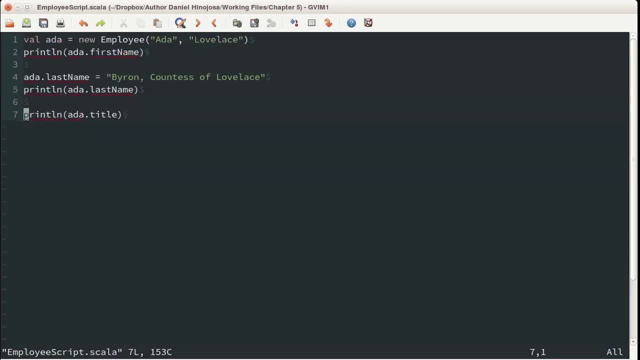 name, but it feeds it back up to the primary constructor with a default string of programmer for the title. Let's go to our employee script. Let's start off by invoking one of the constructors using named parameters in the employee script. So I want to instantiate a new employee, but this time I want to specify my own order. 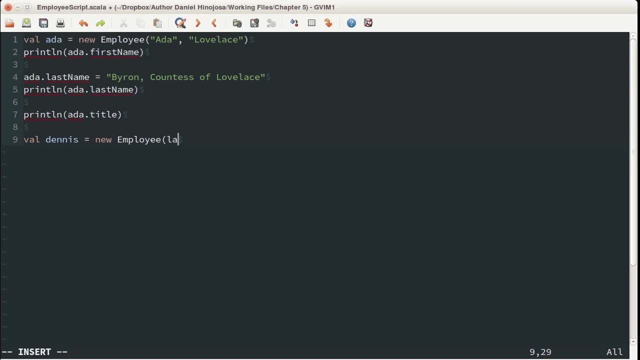 so I'm going to use named arguments. So I'm creating Dennis Ritchie, famous for the C programming language, and we want to call our constructor with a name parameter. Again, we want to decide the order. We have the power. So I'm going to go ahead and save this and before I continue on, let's add some print. 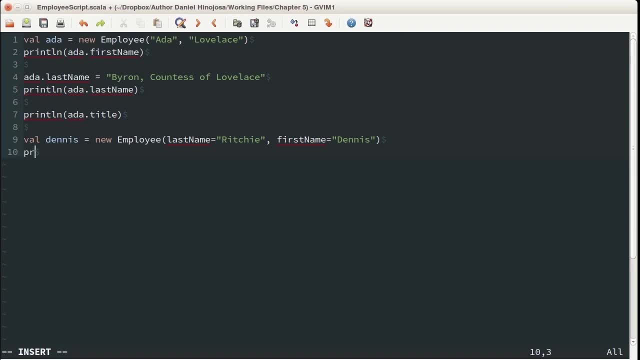 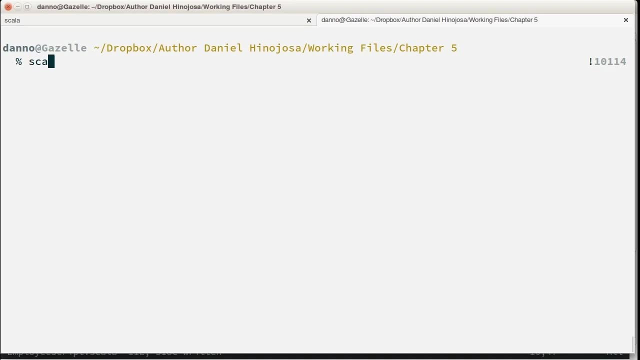 lines to this. Let's make sure that we have the correct values. by doing a couple of print lines, We saved it. Now let's run our script. We do not need to compile employeescala, since we've made no changes to it. Great. 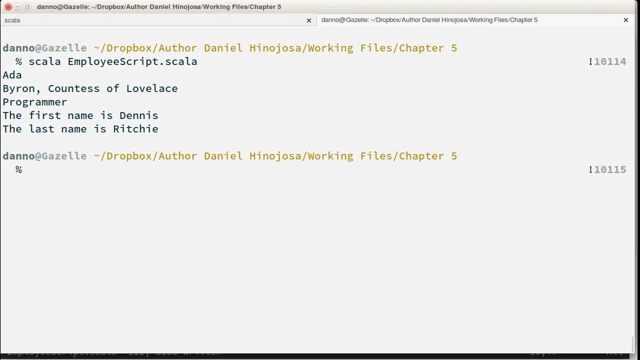 First name is Dennis, Last name is Ritchie. That looks fantastic. So again, named parameters can be used for methods and constructors. What about default parameters? Remember from the previous session, named in default arguments. we used default arguments, default values, so that the invocation of that methods parameter, remember we're talking about. 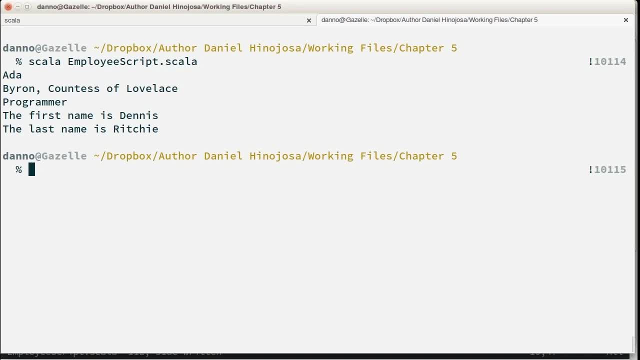 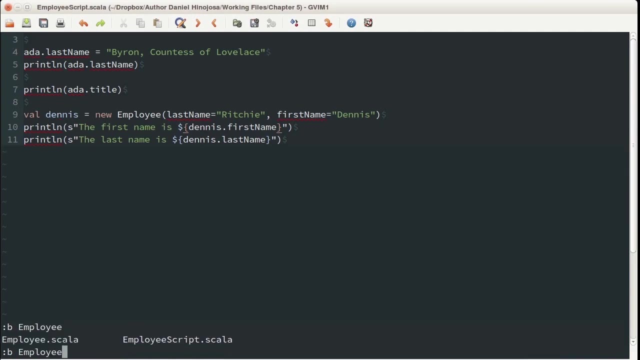 methods at the time that could be optional, because we provided a default value to that particular argument or parameter, however you like to call it. So let's try doing this for a constructor. So let's go back to our code, And what I'd like to do now is for the title. I would like 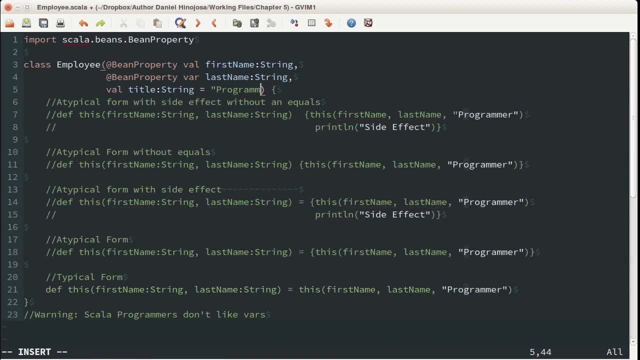 to provide this with a default title of programmer. Well, this makes things interesting, doesn't it? So what does this mean? This means that the title has a default, in case we don't call it, And it also means that we don't need our ancillary constructor. In fact, we don't need any other. 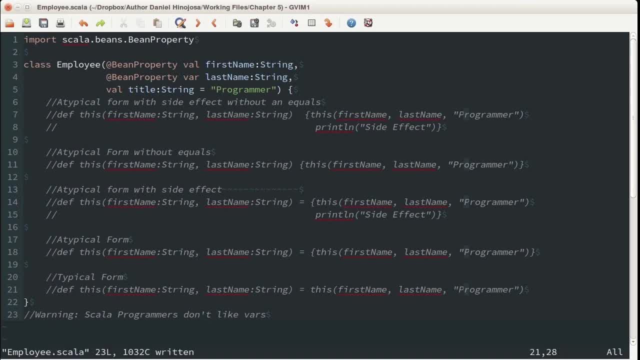 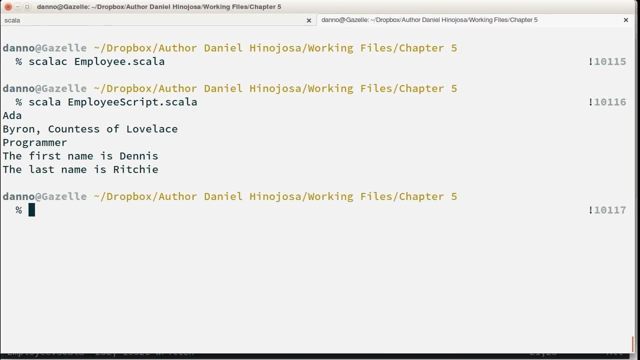 constructor. Very interesting. Now let's save this, compile employee Scala and then run our script. This works With Scala. you have a lot of different choices. You could either use a constructor or you could use a constructor. So let's say that we want to use a constructor. So let's say that we. 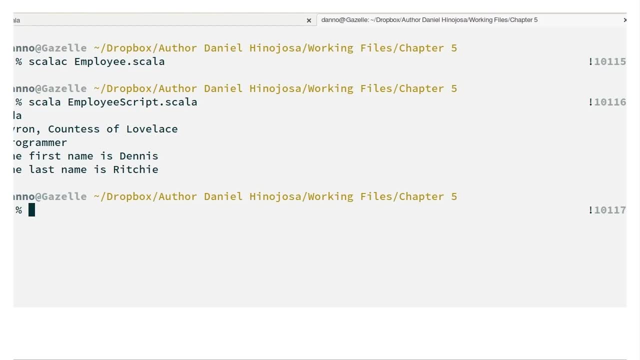 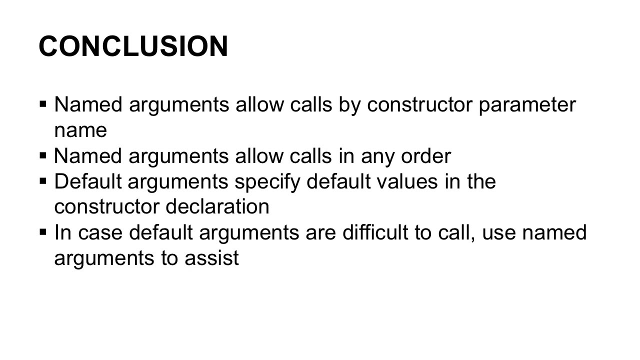 could use a default parameter to achieve the same effect. So, in conclusion, named arguments allows us to invoke our constructor by constructor or the parameter names. Named arguments also allows us to call our constructors in whatever order we please. Default arguments allows us to specify. 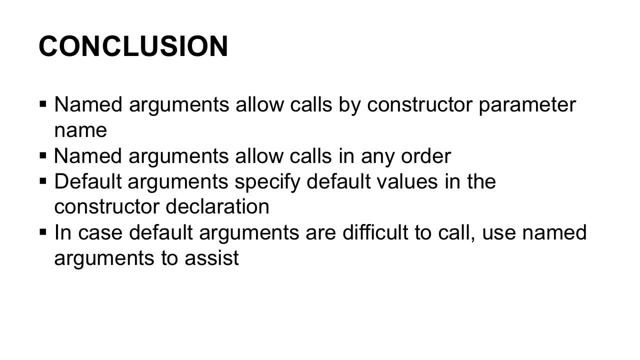 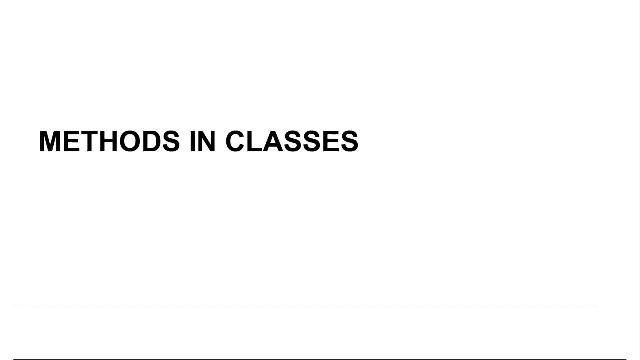 default values for our arguments, but this time in constructors. We did it before in methods, We did it now with constructors. In case default arguments are tough to invoke by any regular means, you can use them in combination with named arguments. In this session we'll talk about 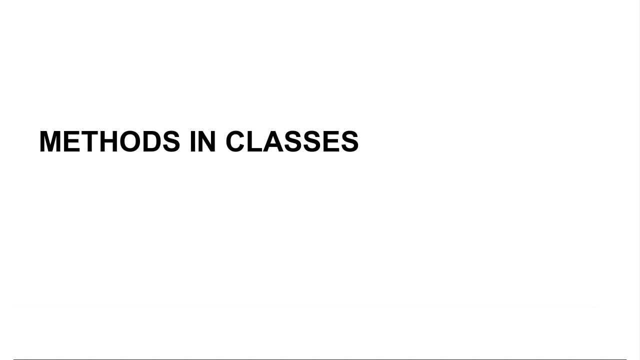 methods within the confines of a class, And we will also address an issue of a bug that may occur when running a script, And we'll talk to you about how to overcome that issue. Now we've discussed methods, how they work, but we've done it in isolation, So we're going to bring those into a 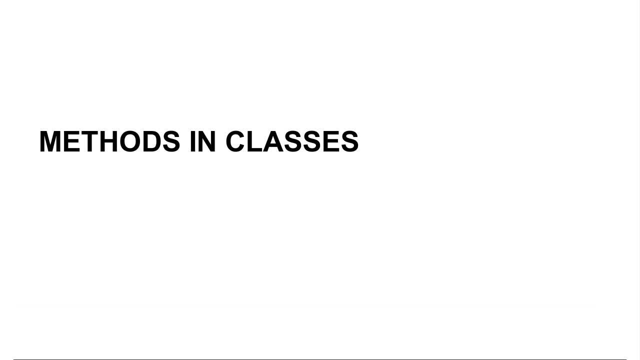 class And, as you may have already surmised, this works inside of a class and works to add functionality to the class, So we're going to bring those into a class And, as you may have already surmised, this works inside of a class, So we're going to bring those into a class. So 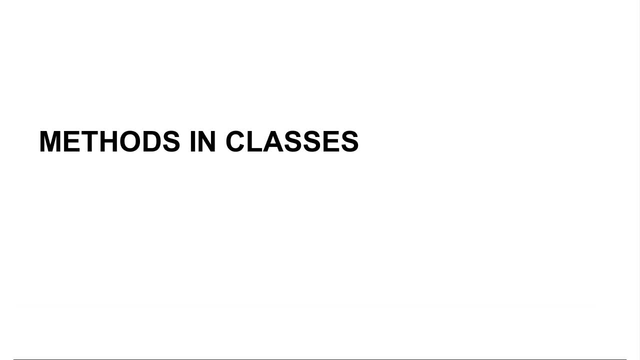 let's get started with our employeescala file that we've been working on for the last few sessions, And this time what I'd like to do is add a method called full name that returns the concatenation of our first name and our last name of our employee. So let's go back to our code and 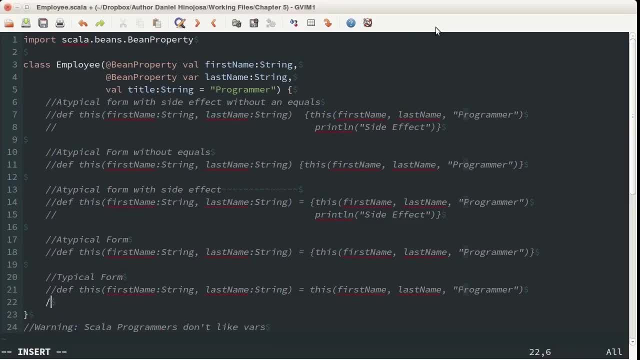 see where we left off. So here's our code, And what I'd like to do is add another method onto here. This would be our first method. the rest have been commented out, But we like to add a method called full name And the return value we're going to put in a method called full name. 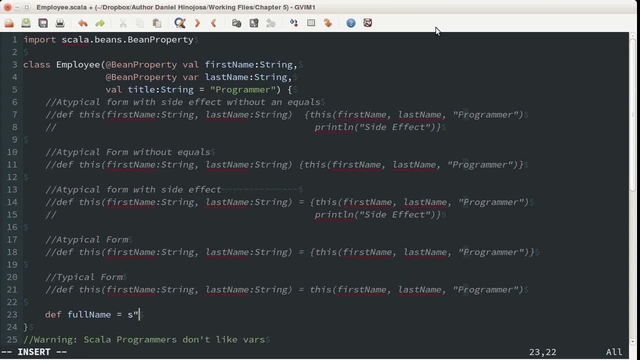 We don't have any parameters, So this is just something that we purely return. Let's use string interpolation. we'd like to bring in the first name and the last name. Great, So here's our method. Now let's go to our employee script and invoke our method. So here's our employee script. 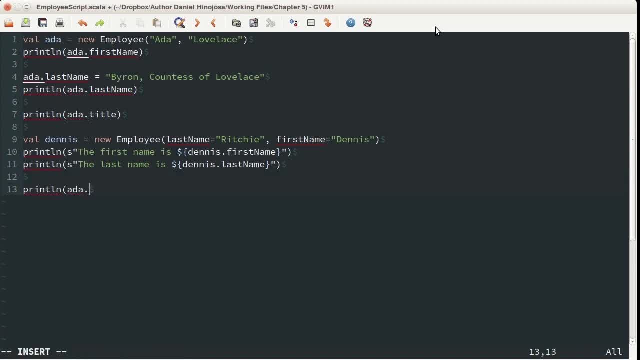 from what we had last time, And what I'd like to do is add a couple of print lines: One. I'd like to see Ada Lovelace's full name, And I would like to see Dennis Ritchie's full name as well. We're. 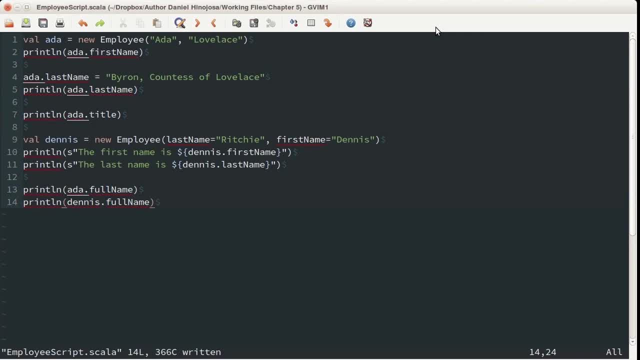 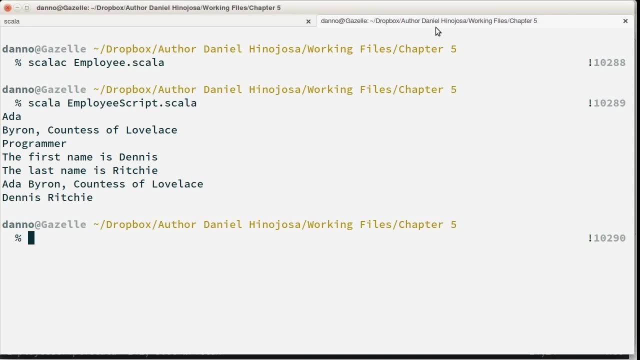 going to save that file. So we saved our employee. we're saving our employee script. Now let's compile Employee Scala And let's run the script. This looks great. Our last two lines show the full name. One is Ada Byron, Countess of Lovelace. The reason why it says Countess of Lovelace is because we've 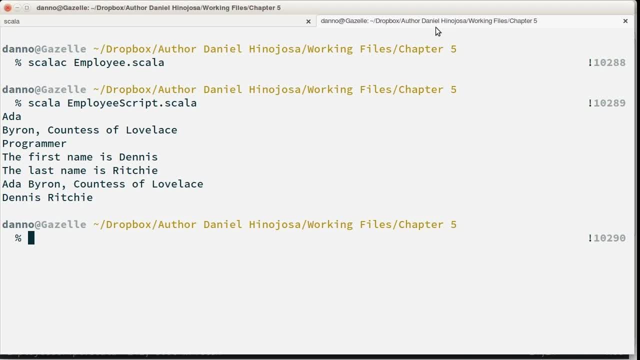 changed the last name And then finally we have Dennis Ritchie worked out great. The method inside of the class is in a support role for the class and its member values and variables. Now let's go back to our code. Let's try something else Now within employee. 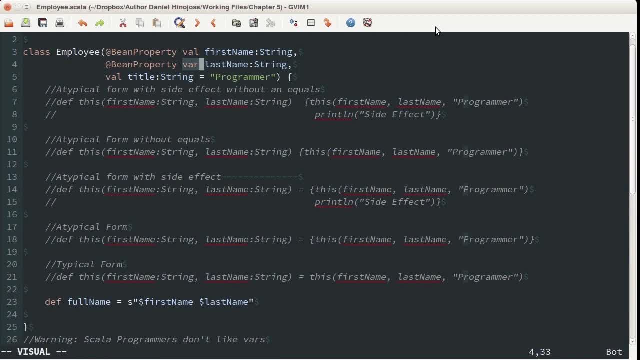 we have this var And if you take a look at my line 26,, it says right down there warning Scala programmers do not like vars. We particularly don't like vars because every time there's a var there's something mutable going on or changeable. Now let's say we want to change this var, Let's go. 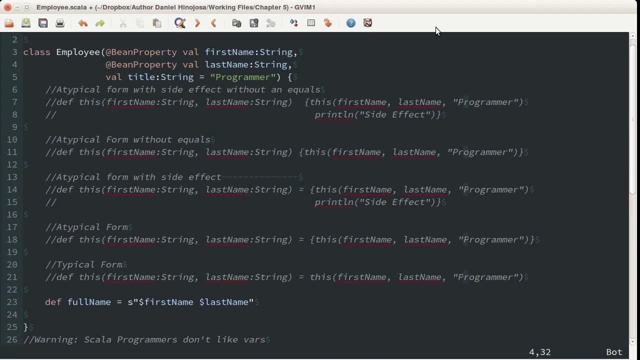 ahead and do it now to a val. Question is now, since this is val and unchangeable, how do we update the last name member value when these member values are unchangeable? Well, the answer to that will be a method, So let's create a method called. 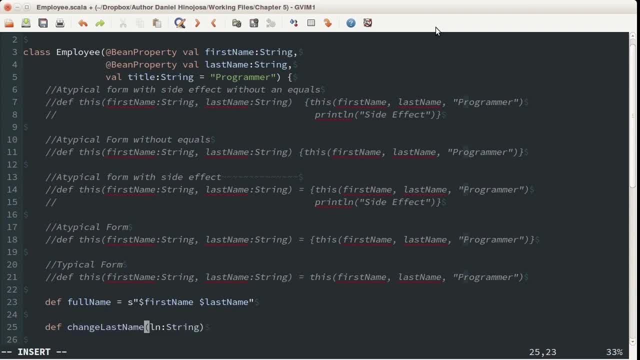 change last name. I'm going to bring in ln. This is of a type string, This is a method parameter, And what we're going to do is we are going to return a new employee object. This employee object will bring in a first name, But what we're going to do for the last name is we're going to 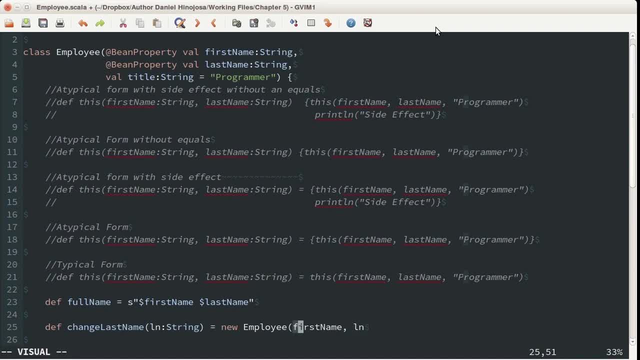 take this ln and plug it into here. The first name that we created happened to be the already established first name that is in our object as a predefined state. Then we will add last name, And this to is also predefined from what is within the object. So again, we're taking a string. 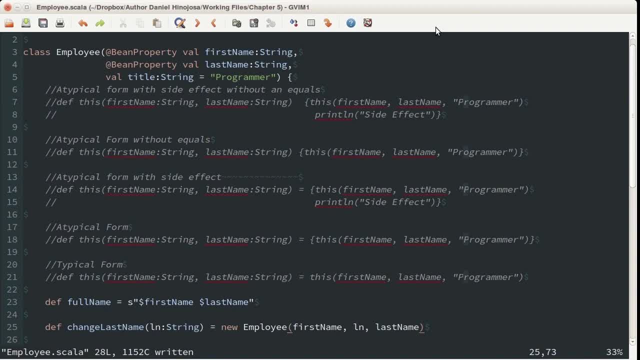 and we're using it in the construction of a new employee. object. the key to immutability is: never changed the original state, But to make a copy. And what we're doing here is we are returning a new employee, which is a copy, But except this time, with our copy, the last name has changed. Now let's 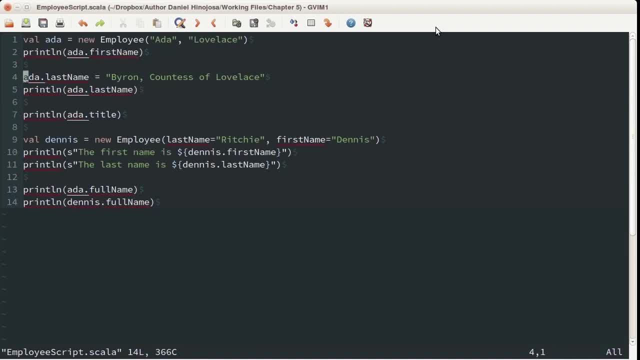 to our script and update that. now, right up here on my line four, i am calling. adalastname is equal to the new string, but what i'd like to do is i would like to change this to the new method that we just created, called change last name. the thing about this call, though, is we are returning an 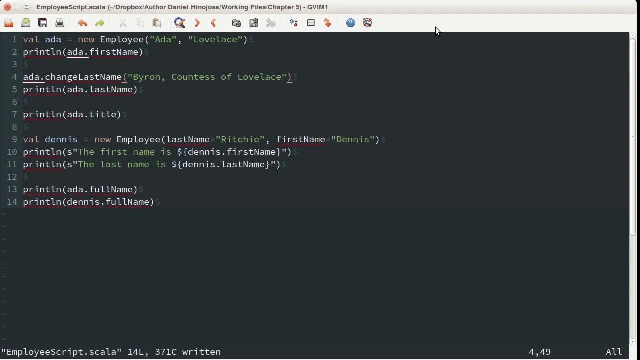 object: we are returning an employee from change last name, so we need to assign this to a new value, preferably a val, of course, because vals are rarely ever changed. but because we did this, we have to change every other reference that happens afterwards. so what i'd like to do is: i'd like 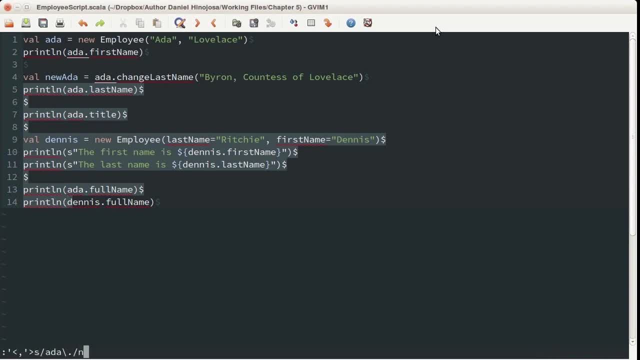 to change ada period to new ada, which is the name of the new reference period. so we'll change this, this and this. now what else i'd like to do is add another print line here- adafullname, because ada is the original reference. so what we should be expecting here is that the third from the bottom. 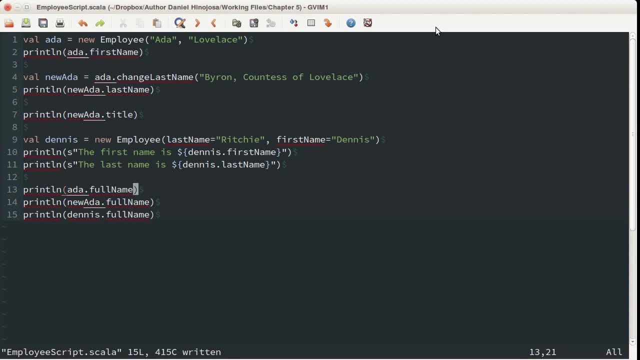 of the line should just be ada lovelace, the second to the bottom line should be byron countess of lovelace, and then finally, the third to the bottom line should be byron countess of lovelace and then finally, as the last line, that should just say dennis ritchie. so we saved our script, let's. 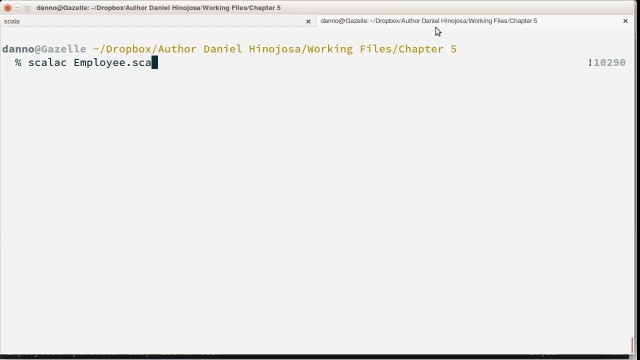 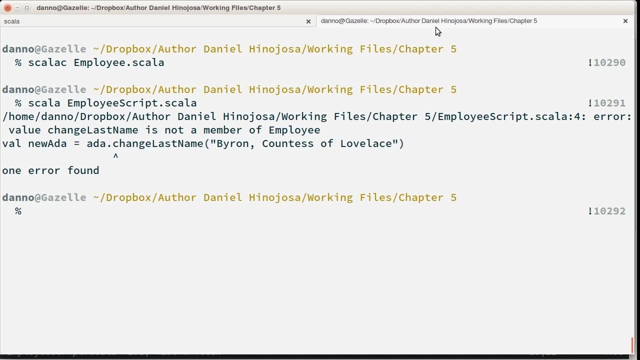 recompile and let's run our script. there's our recompilation, now let's run our script. so what we end up here with, unfortunately, is a bug. i'm fairly confident what we did will actually work and this states right here that change the last name is not a member of employee. but we did. 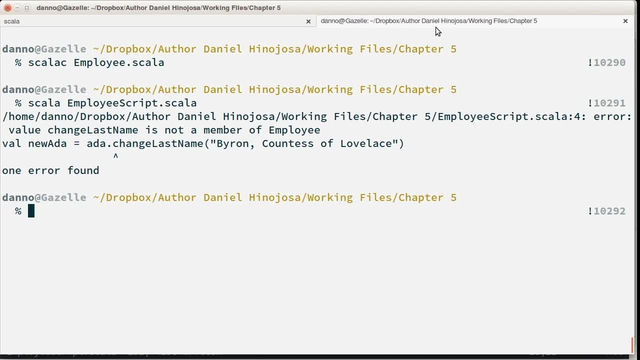 save our file, and so i'm pretty sure that this is going to work. now what i'm going to do is i'm going to impossible, but i'll work here what i learned with photocopier. it says something about the ней battlefield, them, the pieces that we were looking for, but actually they all work together. 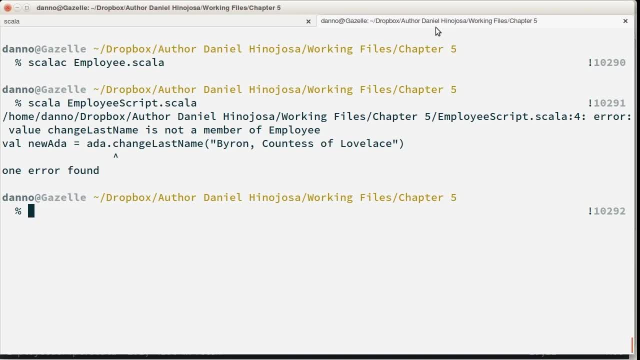 so we're just going to call it: psh, fill out your machine code now. it will just go kind of redone. there's a couple их and what's kind of fun about these specs. it just kind of puts us under control. okay, now let's go ahead and run another test. wonder, with msc, what the new code is. hmm, balth 영상. 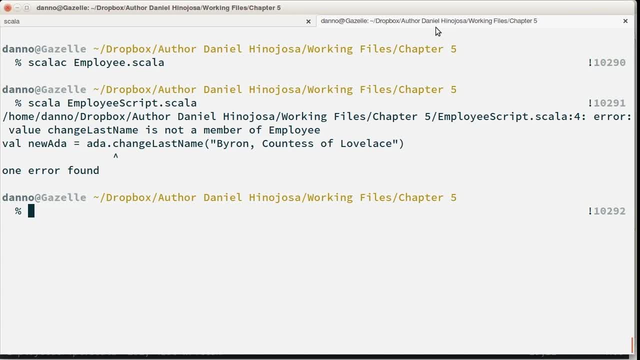 what comes across is that this is the code that appears in the máximo and this is the room. the code is the common code. as you know, it's compiled into code-based code. the other thing is that if the version 211.7, although I've seen this in 211.5.. In a future session we'll be using something. 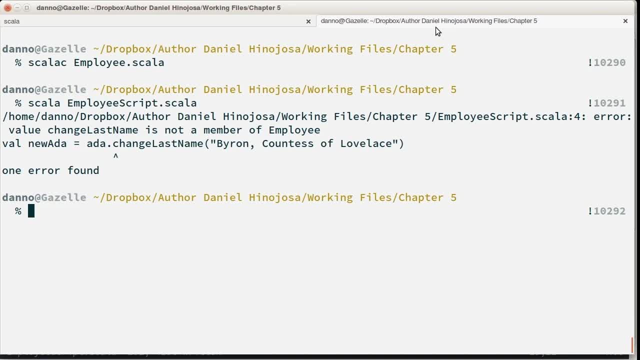 called an object to run our code, but right now we're just dealing with scripts, So I still do consider this a bug at this time. but our workaround is: I would like to run the script using something called the dash and C switch. The dash and C switch prevents Scala from accessing classes. 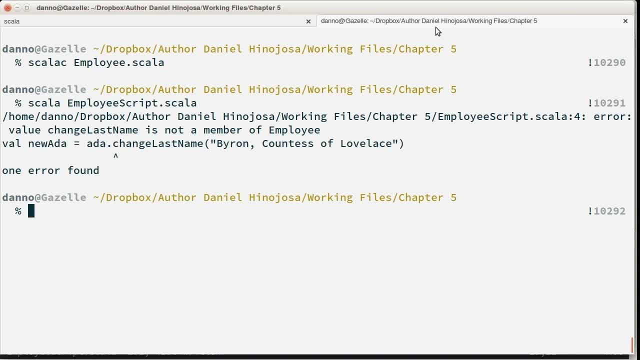 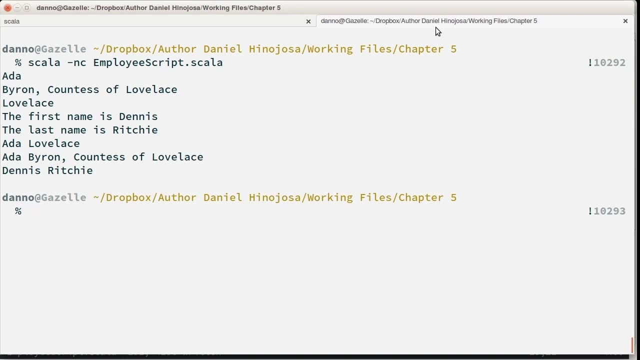 from the FastCompiler cache and will use the class files directly. So what I'd like to do is run Scala, this time NC. Again, don't use the FastCompiler and let's run our employee script. So we are using the classes from the class path directly and the bottom three state Ada Lovelace. 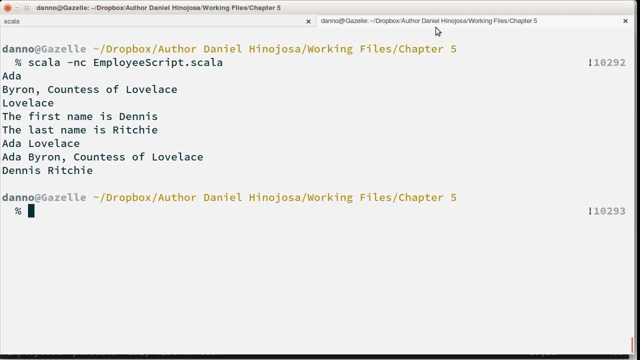 Ada Byron, Countess of Lovelace and Dennis Ritchie- Exactly what we were expecting. This is really neat. Also, note again that the original Ada contains the original information, while the new Ada contains the newer information. Now, what's really great about immutability and creating? 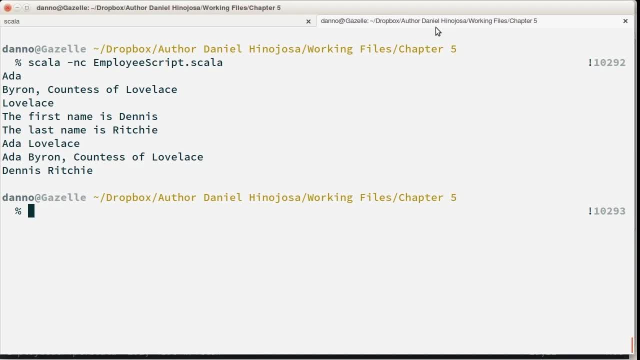 copies is that you don't have to worry about it. You don't have to worry about it. You don't have to worry about it. We have a code that changes every time we make a change. This code is called item, And what we do is that we get an automatic design pattern from the original gang of four. 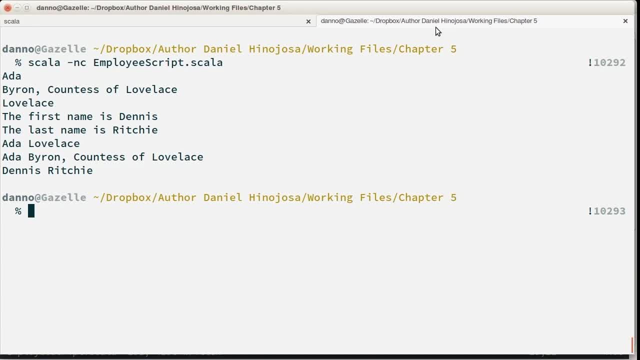 design patterns, called the memento pattern. We get to see what happened in the past because we have a copy of what happened in the past. Not only that, but immutability is safe for concurrency across multiple threads, since there's no need to synchronize change in states. 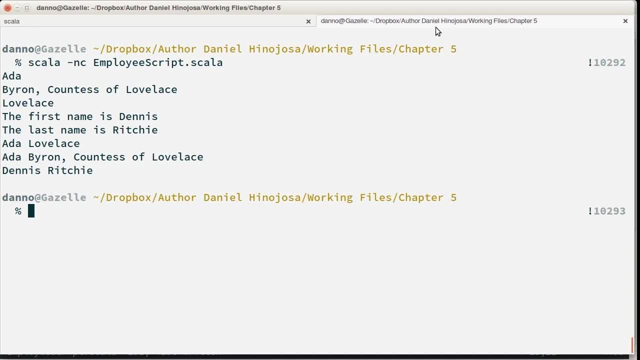 particularly in processor. Now let's go back to our code. The ChangeLastName method is a bit. can update our object for us in an immutable way, but this will use default and name parameters to implement. so let's go back to our code and get started. all right, so here's our change last name. 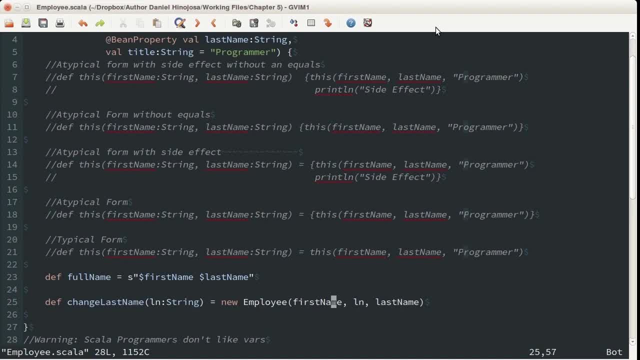 method. so what i'd like to do is change this around and create a one-stop shop for immutability by making something called a copy method. so our change last name is no longer there, and we're going to create a brand new method in its stead, and this will be called copy and what we're going. 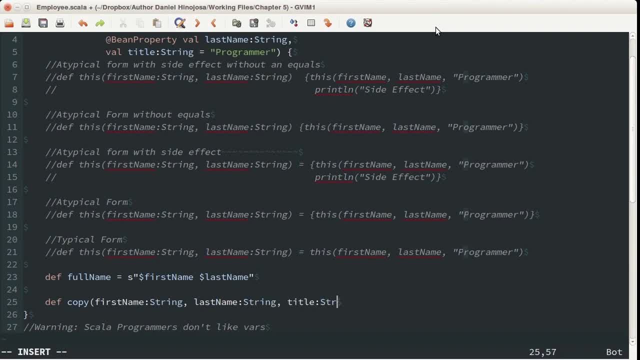 to do is we're going to bring in all the parameters from our primary constructor. what we're going to do is we're going to use default parameters here. so first name is going to retain the state that we already have from within the object. we're going to make a call. 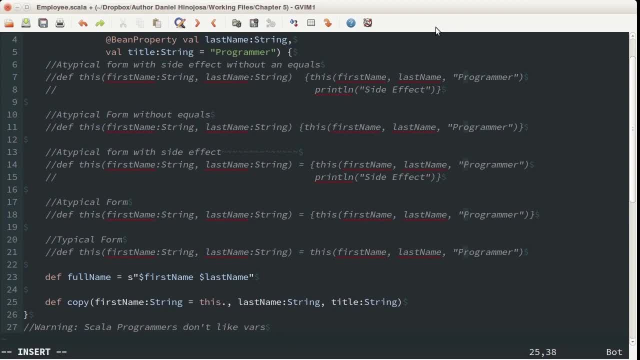 to this. this just means within the object itself. give me the state of first name which is a property internal to this object. for last name, we're going to bring the already established last name and for title, we'll go ahead and bring in the already established title. 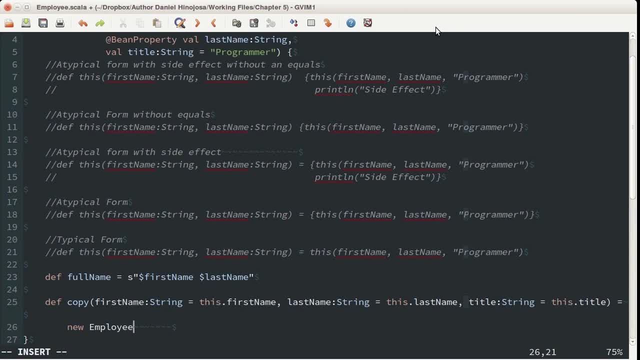 and what we're going to return is a new employee object. we're using the same methodology as we did before, and what we're going to do is we're going to plug in the first name, the last name and the title. let's clean this code up a bit. that way we get to see how everything's working. we can create. 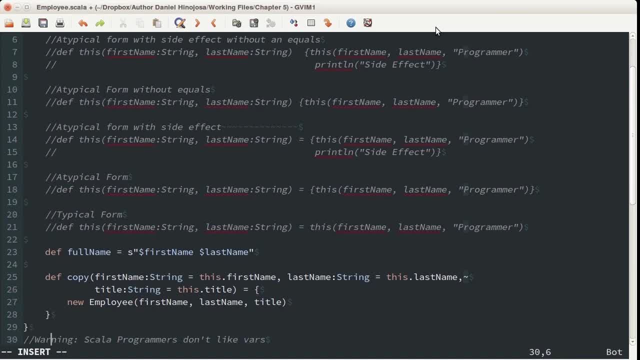 a block here if we'd like just to make things a little bit cleaner. all right, so there's our copy again. we're bringing in a first name. this will use a default parameter. this will use the state that's already been set. last name, the default parameter. and we're going to bring in the first name and we're 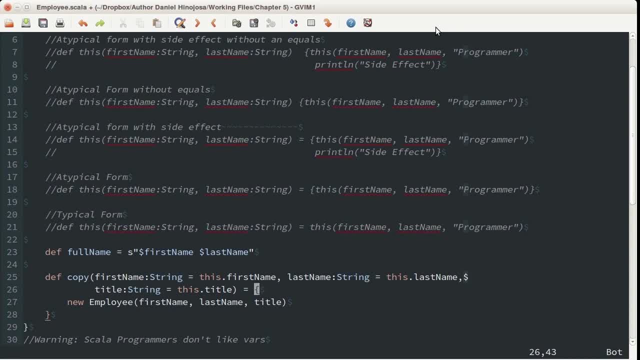 going to create a new property. that will be the default parameter, that will be the last name that's already set and title will have the property that's already been set within our object, and what we get in return is a new object, a new employee with those new fields. so let's try it out. i'm 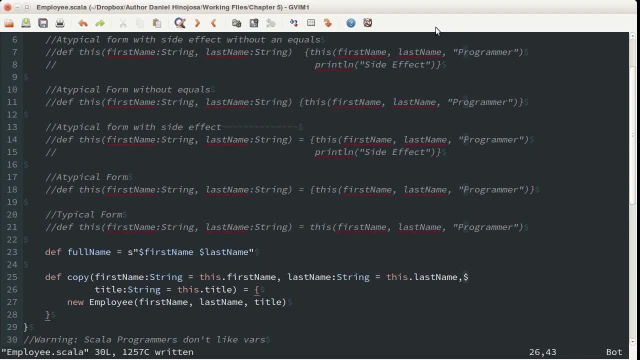 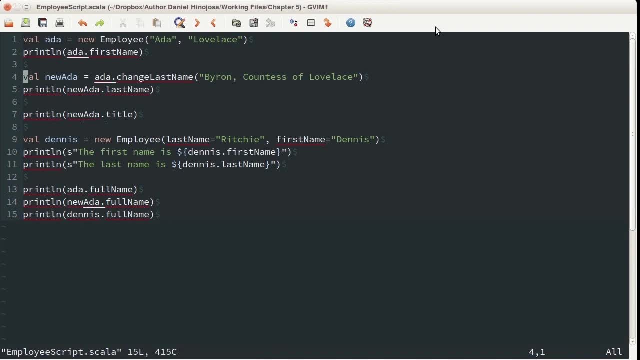 going to go ahead and save employee scholar and let's go to our employee script and this time we'd like to use name parameters to specify which parameter it is we wish to copy. so here we are in our employee script, but on line four change. last name does not exist anymore, so let's get rid of it. 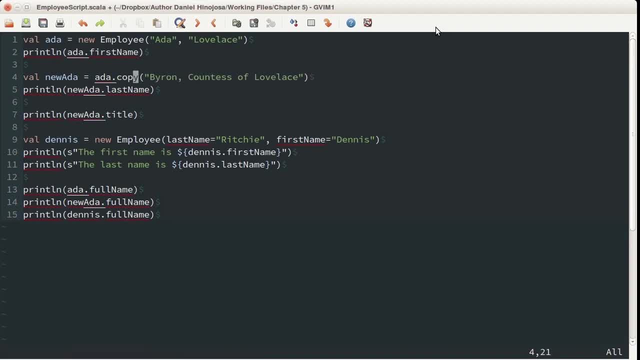 and what i'd like to do is i'd like to invoke the method copy, but we have to use the name parameter now, and what we're going to do is we're going to state that the thing we wish to change will be the last name. so i'm going to change this to state last name is equal to byron countess of lovelace. 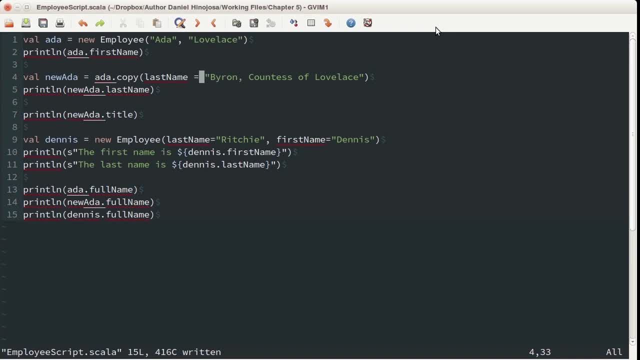 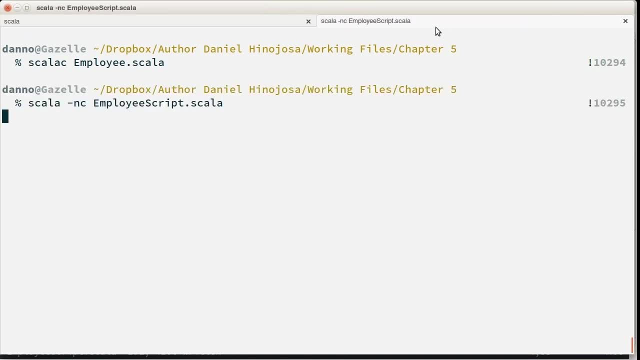 now let's compile our employee skull and let's run employee script, of course with the dash and c flag, because we don't want it to use the fast compiler anymore. and now let's run our script. great, remember, we have to do the dash and c just to avoid the fast compiler issue we were having earlier. but 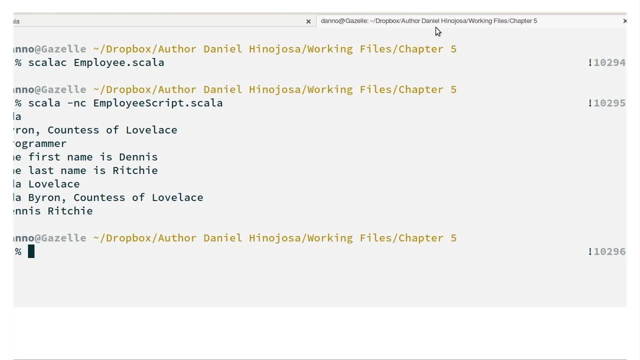 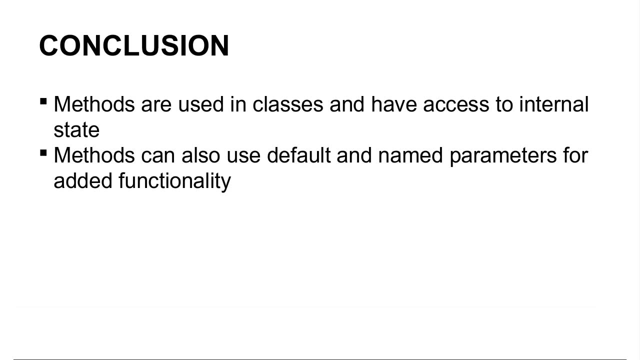 there we go. that looks great. we have immutability and we have our flexibility. so, in conclusion, methods are used in classes and they have access to the internal state. methods can also use default and name parameters for better functionality, and we did so with that copy method also when running. 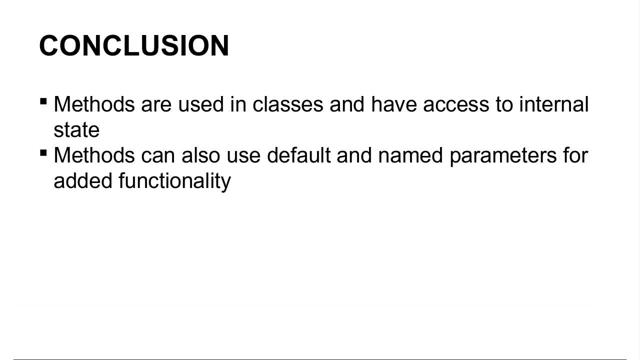 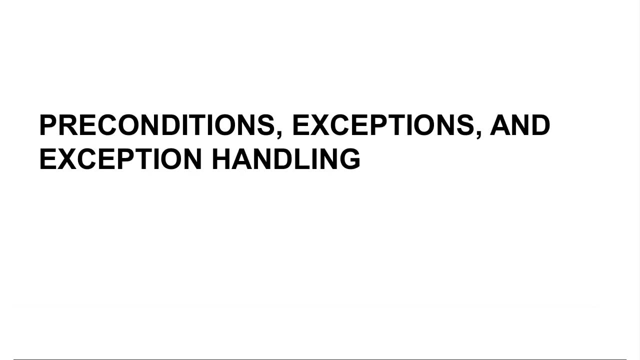 a script. we talked a little bit about the fast compiler, what it does again. nothing wrong with it, just moving a little bit too fast currently, and if we want to avoid using the fast compiler, we can run our script using a switch called dash and c. in this section we introduce preconditions. 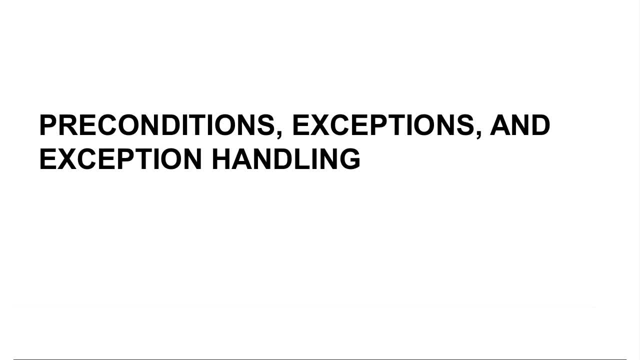 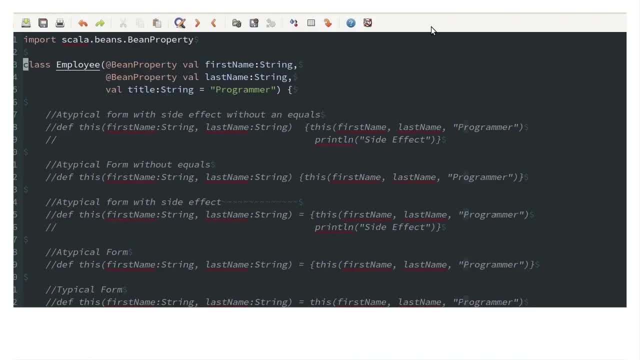 to ensure that no one will give our class any information that will affect our internal state. let's go to our employee scholar, the same one we've been working on for the last few sessions and the problem currently right now let's go to our code: check it out. 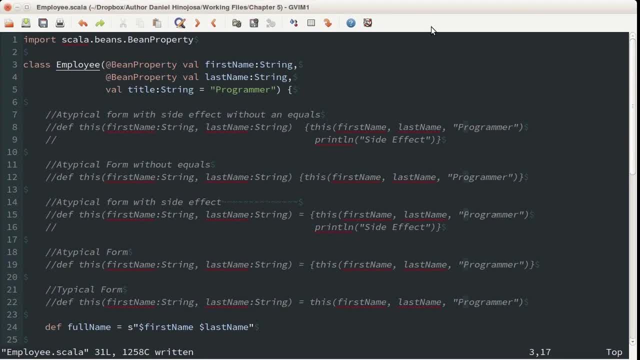 now let's say: this is our documentation and we want this to have an empty string. let's let's make some gray 삶 Herr, feel that for use p.2.0 or p.2.0 now, if we need to do all the things we just made wh vir to permissive users of our code. 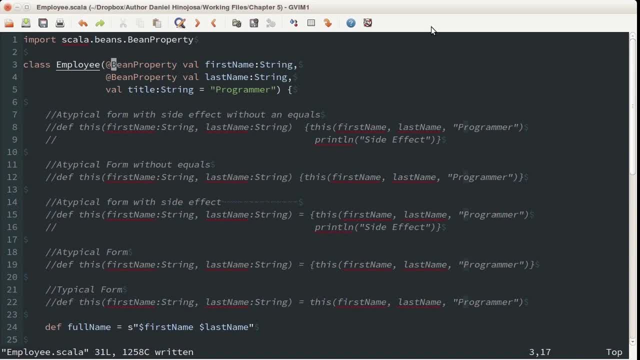 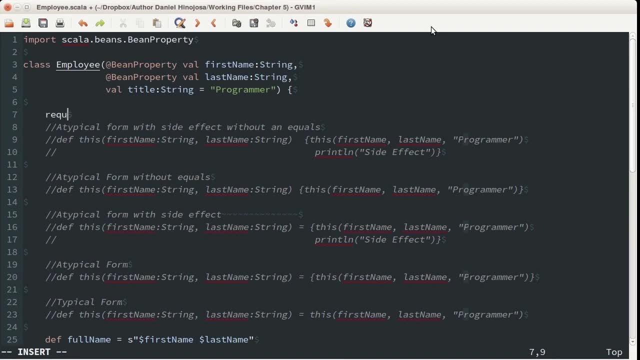 can actually provide an empty string, if they feel like it, for our first name, for our last name and for our title. if we want to go on the defensive, we can do so with a method. this is actually a method called require, so let's put some requires in for the first name, last name. 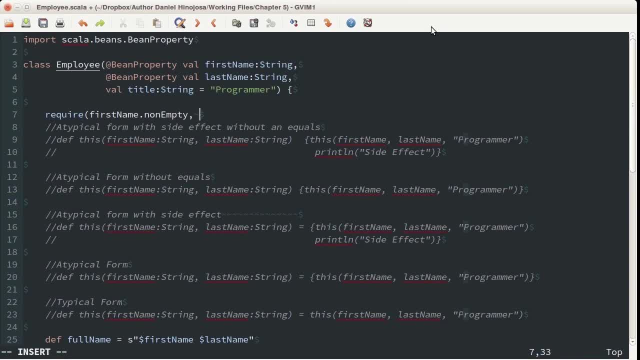 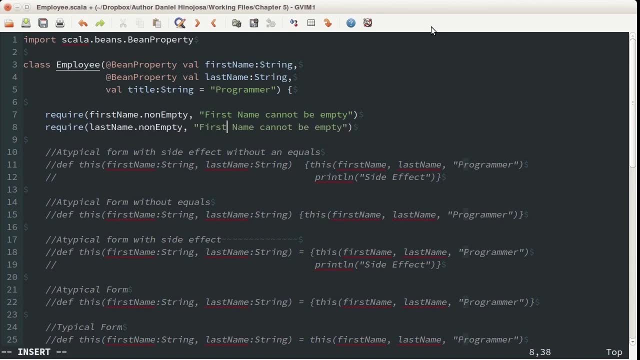 and title. so here's the first one. require. next part has to be of Boolean or something that evaluates to a first name, is non empty. but if this condition is not met, a message will be displayed. let's try that again for last name, and in this case last name cannot. 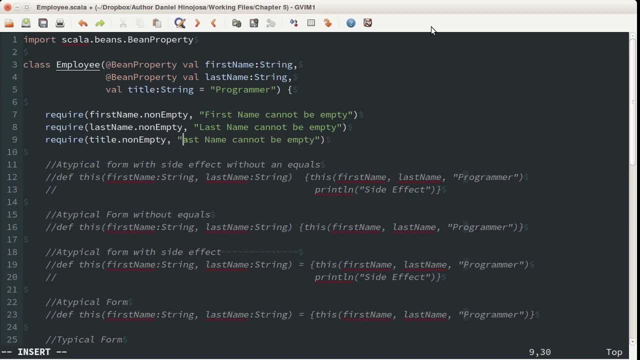 be empty, and we also want to make sure that the title cannot be empty. so we have three requires. now there's something peculiar about the placement. the first time you look at this it's gonna look a little bit weird. these lines are a part of the primary constructor. they're not inside of any. 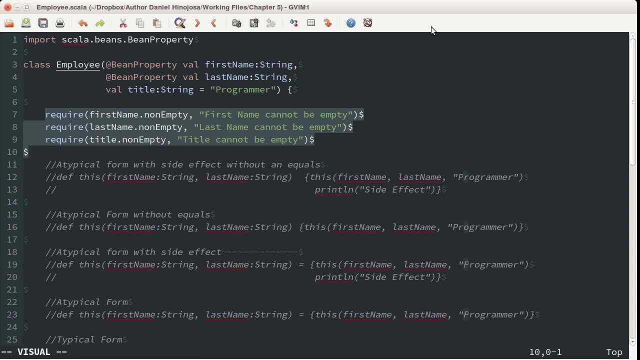 other method. this entire space that you see here is invoked when we call the primary constructor. it is essentially the primary constructor space. now, these require statements, all require that the entries of first name, last name and title are not empty and, to re-emphasize, this needs to evaluate to a boolean that 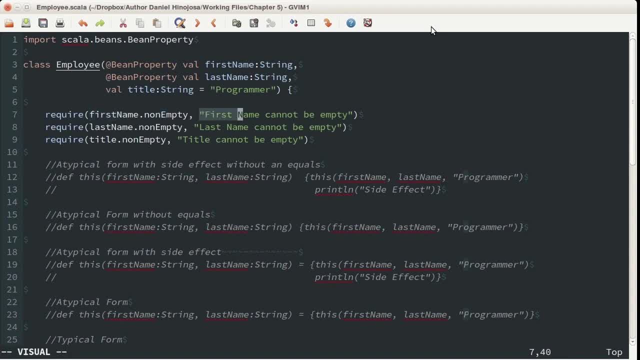 defines whether a certain condition has been met. second parameter is going to be the message, and that's the one that would be generated if the condition is not met on the first parameter. now let's try it with some bad code in the employee script, dot Scala. let's save this and. 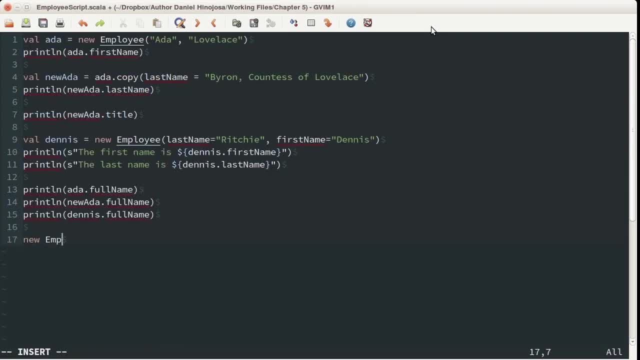 let's go over to our script now. what I'd like to do is create an employee, and we're going to create an employee called Bono, with no last name, his stage name has no last name and his title will be singer. so let's save this and run it, and 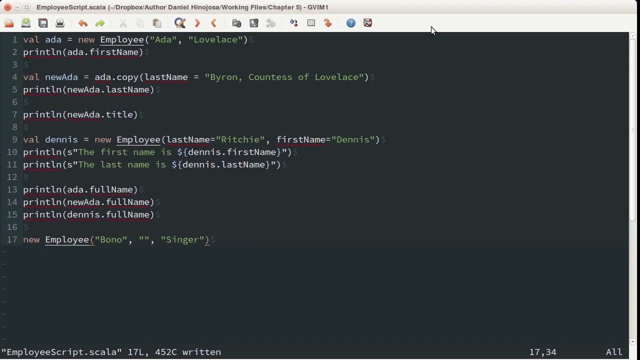 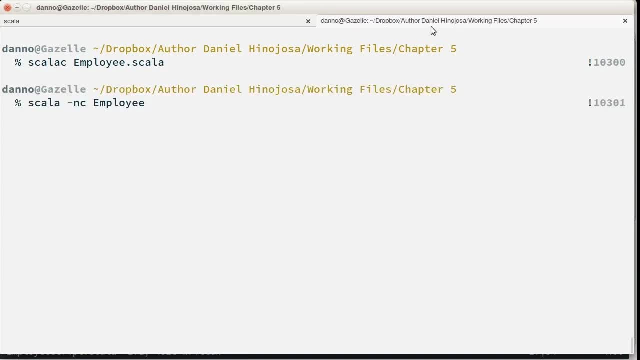 let's see what happens, and last name is going to be the empty string. and now let's run our code. I will be using NC just in case there are any bugs, and we had referred to this in our previous session. this way, we don't have our 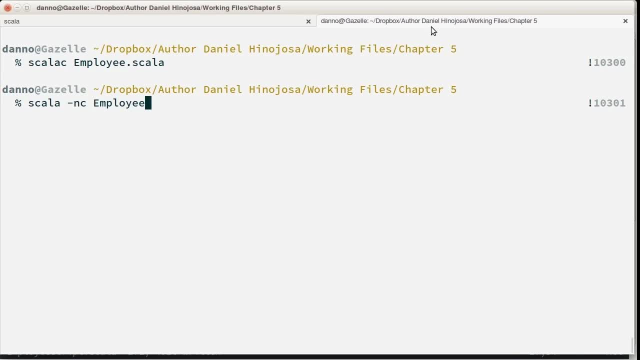 classes go into the fast compiler. this will just use the classes that are already in our class path, so I'd like to run employee script dot Scala and let's take a look at the results. this is going to produce a stack trace and if we scroll a little bit up, this is going to stay right here. legal argument. 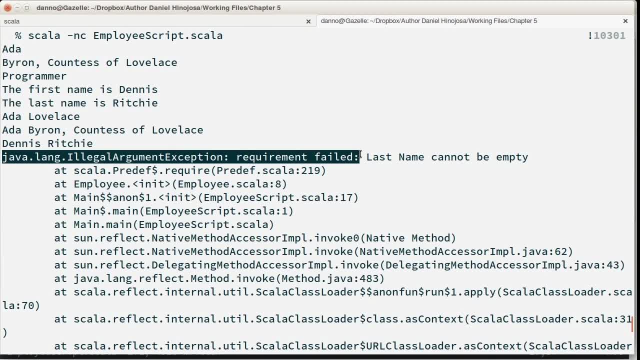 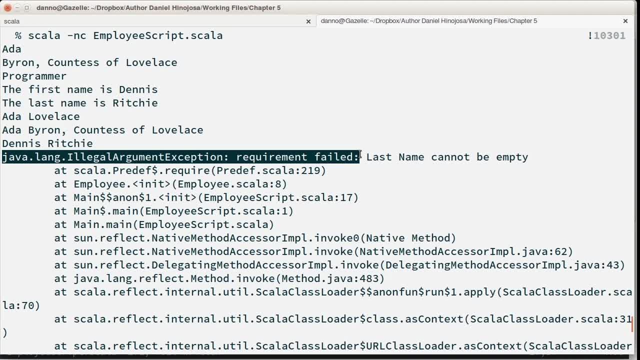 for posterity. and what hate for this exception to keep hanging around and busting up our code. so let's wrap it up in a try-catch block. that way our program runs and we are able to tell what the reason is for this program failing. so let's go back to our code. and since we know bondo is going to cause, 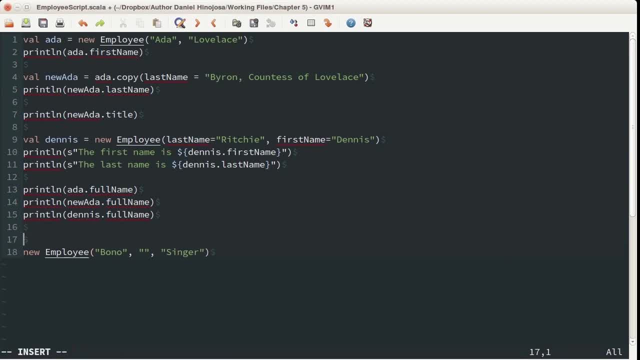 trouble, let's surround them with a try-catch block. here's the try, here's the block, and I'm going to call it the try-catch block and I'm going to call catch. now, what's going to be different in Scala is that I'm not going to declare. 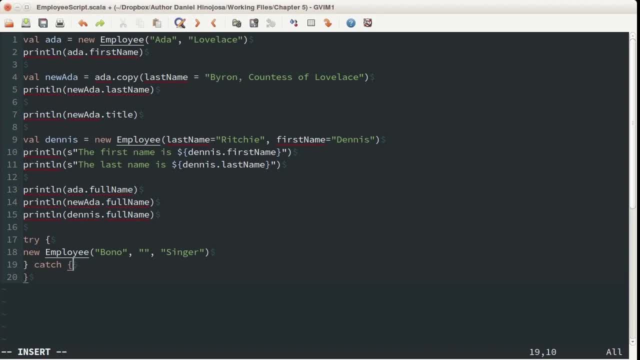 the exception here, but inside of the block right after catch, now try catch block. for those who are unfamiliar with them, is like a bomb container system that the bomb disposal technicians use to either diffuse or detonate the bomb. if something ever happens, then this reinforced barrel will take up all of 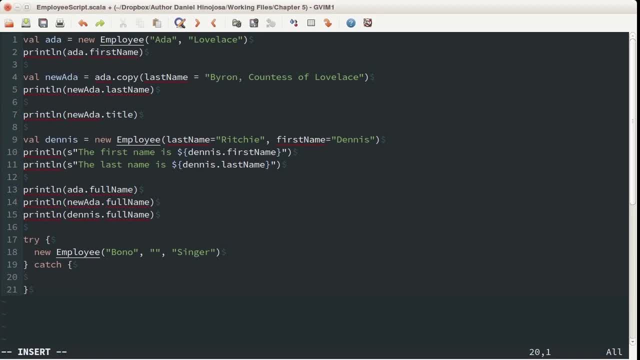 the blast same type of situation here. we know that when we instantiate the employee on line 18, this can cause an issue. so what's going to happen is the try-catch block is going to catch this particular exception and, since we're able to handle the exception, we can safely continue with our program all right now within. 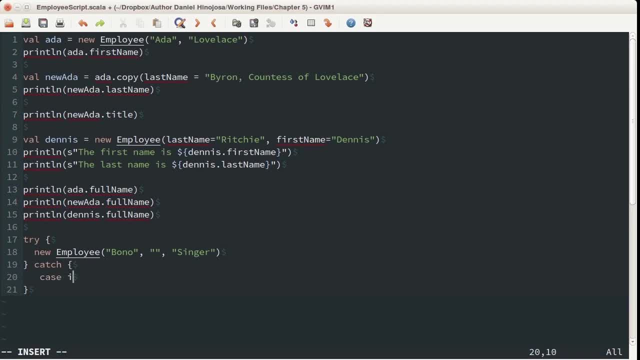 here I am going to add a case and a value, name IAE, followed by the type. what kind of type am i expecting? and the type is going to be an illegal argument exception next time we use the implies operator or the rocket operator. what I'm going to do is I'm going to print line whatever the message is from this. 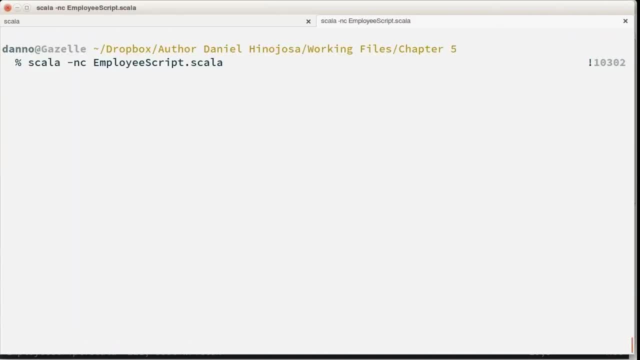 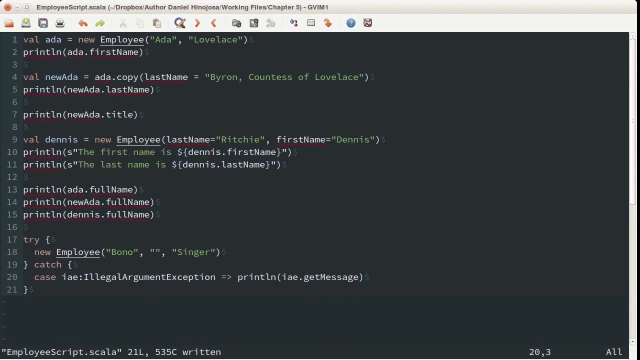 exception. so let's save it and let's run the script to see what happens. great, our program runs successfully and we have a requirement: failed message. last name cannot be empty. we're able to handle the exception. let's go back to our code now. the try-catch block looks slightly different from Java. in Scala you don't. 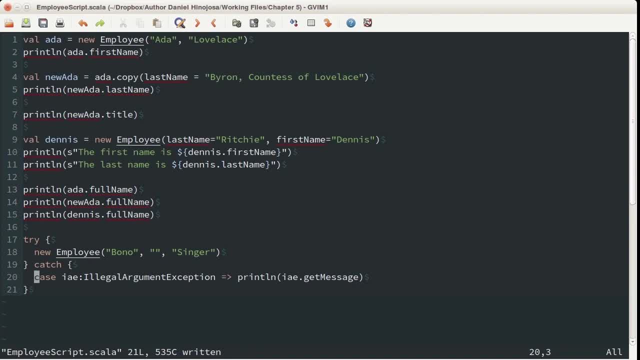 have the exception type and the assigned variable on the same line. the catch keyword stands on its own and here it is inside the catch block, and we're talking about this right over. here. we will use a little bit of what's called pattern matching. pattern matching allows: 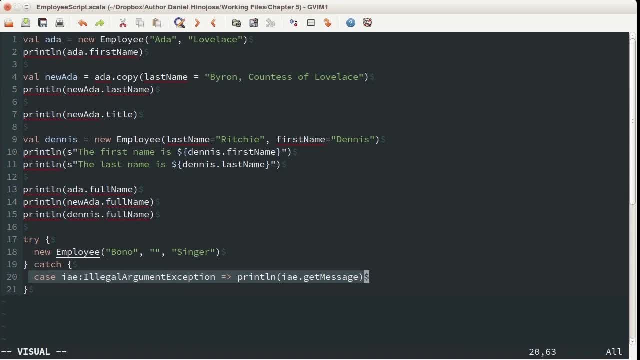 us to match the data with a match first policy based on either the type, which is what we're doing here. we're matching on the type- illegal argument, exception- or parts of that compose a particular object. if the IAE that you see here is of the type- illegal argument, exception, then we're going to proceed with what is. 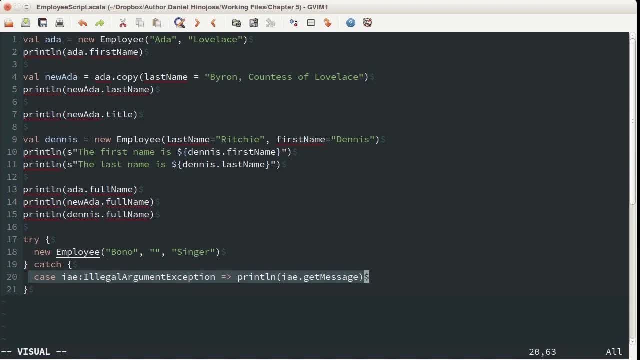 after the rocket operator. if it isn't the right exception, then the exception remains unhandled and it will bubble up to the console error panel or website error page. notice that after we match on the exception, we assign the exception to the value IAE, and here it is, once this assignment is made after the rocket. 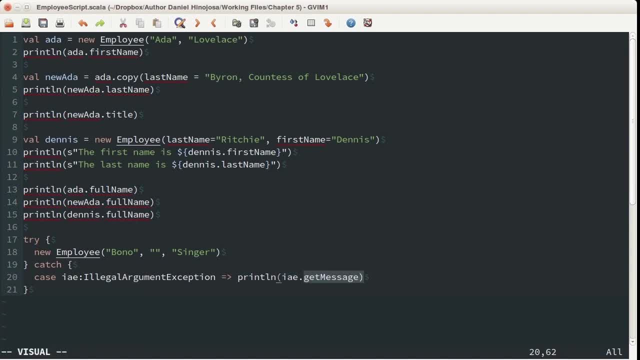 operator, we can refer to it and we can call methods that are a part of its object. this is a good thing now, as a best practice. exception should never be hidden and should appear if something is wrong, otherwise you'll never know how to fix it. so what we're doing here is not really a best pattern. all we're doing is taking 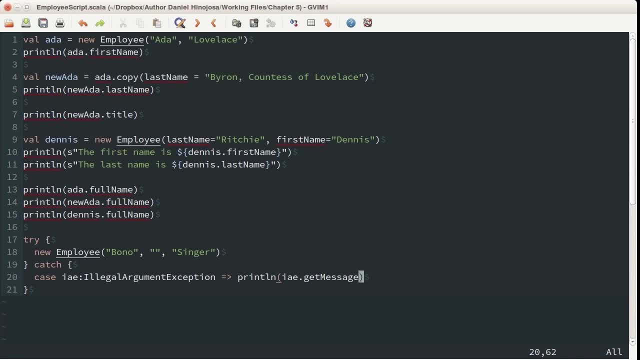 this exception and displaying the message on the system out. but we're only doing this for learning. it also needs to be said that all exceptions in Scala are runtime exceptions. there are no checked exceptions. checked exceptions are from Java. they are a kind of exception where the caller of the method is forced to 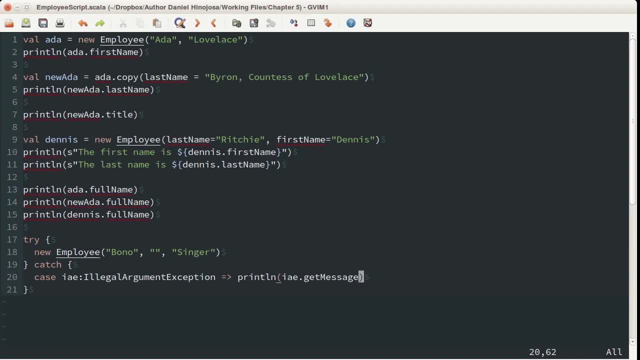 handle the exception at compile time. we don't need to worry about that in Scala, since they are all runtime exceptions. if an exception happens, you have to have the option to deal with the exception or not. you could just let it bubble up to the top of the call stack. so now let's run this. everything looks. 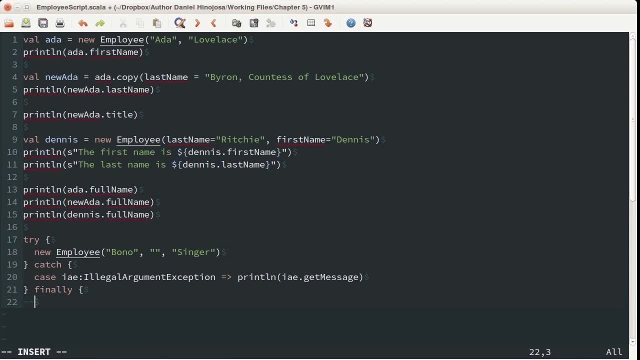 good, now one thing we could do is we can add a finally block. the finally block is optional and this is going to run regardless of whether an exception is thrown or not. it's used to clean up resources and perform other chores that you may have, so, as an example, let's just do a print line here stating that we are 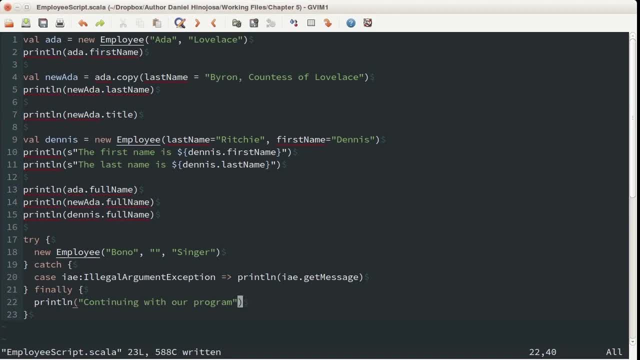 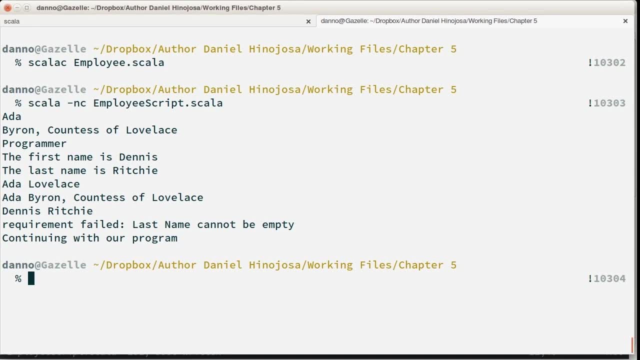 continuing with our program. now let's give it a try, no pun intended, compiling our employee and running our script. okay, as we see here, the last message states we are continuing along with our program. this is because the finally block kicked in now. require is just a nice way to handle preconditions without an if. 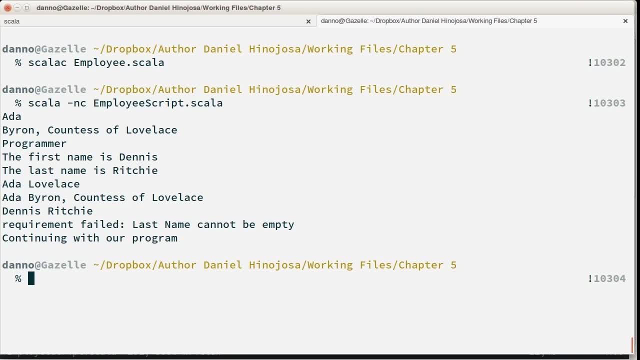 statement and creating an exception for ourselves. but let's write one anyway, just so. that way we get a flavor of what we would need to do. let's say, we have another requirement: that we don't want anyone giving themselves a title that contains the words senior or general. 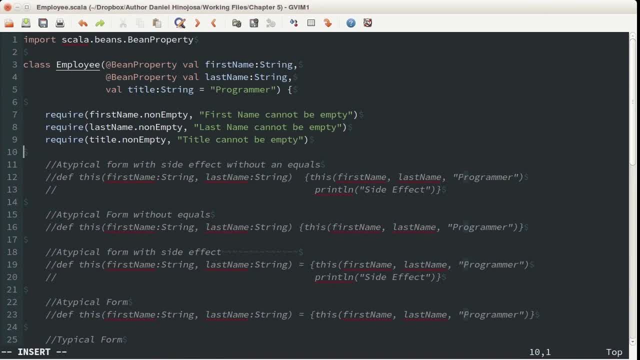 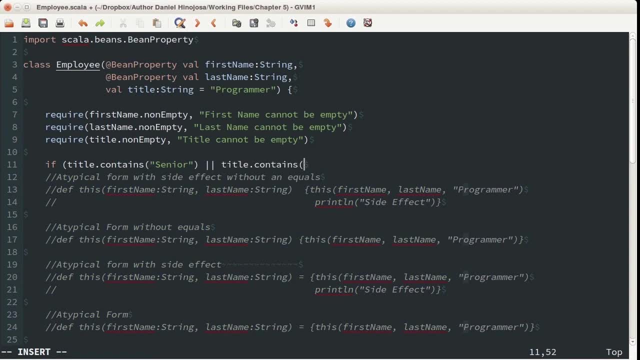 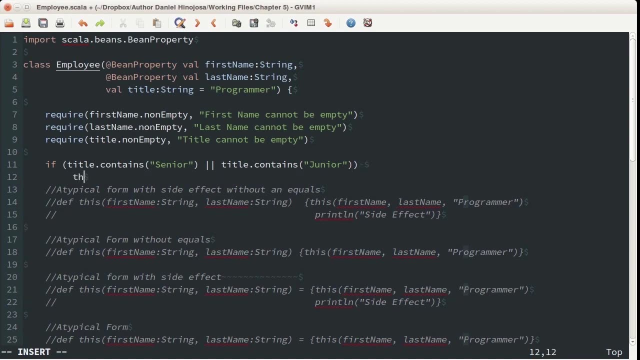 let's go back to our employee dot Scala and then the following line I'd like to add: if the title contains senior or if the title contains junior, then what we would like to do- and I'm just putting this on a new line just for aesthetic purposes- throw a new illegal argument exception and we'll state here: title: 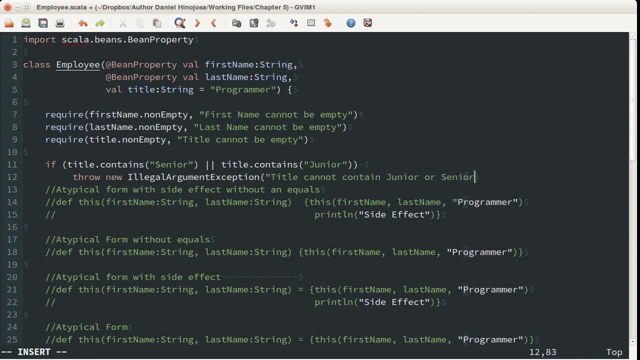 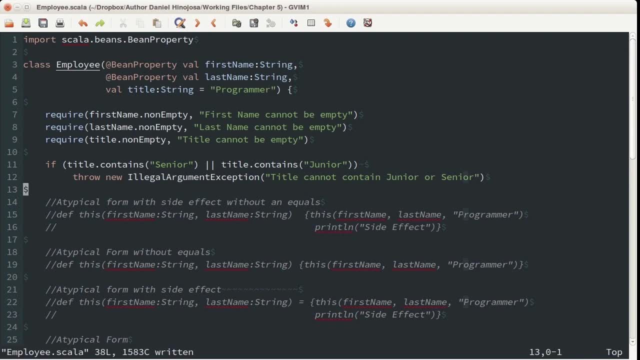 cannot contain junior or senior. alright, so we'll go ahead and save this, and this is the last line that we're going to need to do is we're going to go ahead, and this is how we do. a manual precondition check throw will alert the caller that 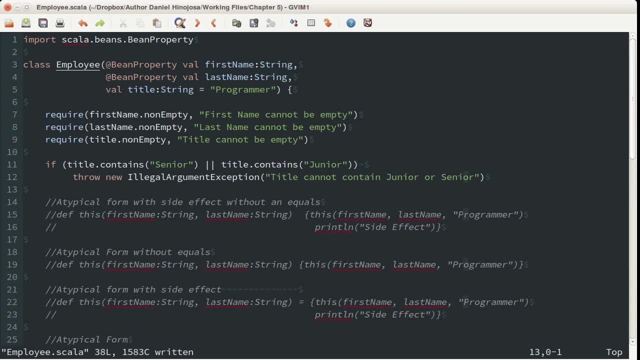 something bad has happened. there are many kinds of exceptions out there, but typically these exceptions- take a look over here: when you look up a pre-existing exception that you wish to use- will typically have a class name that ends in the word exception. find the right one that fits your scenario whenever you. 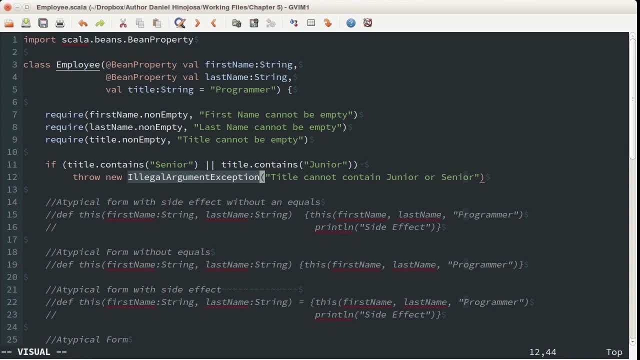 need to alert others of a problem within your code. now let's create a bad entry in our employee script with the title of junior or senior in that title, so we'll save this. let's go over to our script now. in our script, let's create someone. 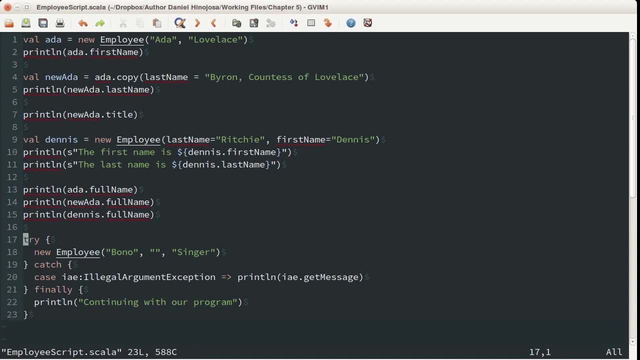 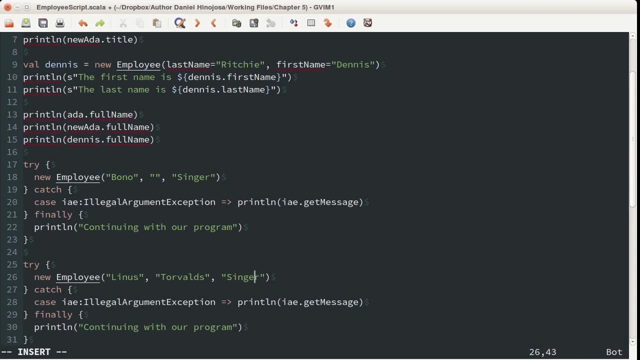 else and what I'd like to do. let's just go ahead and make a copy of that and instead of bondo, let's use Linus Torvalds. and this time Linus Torvalds will be not a senior, a senior C programmer. I am also expecting an illegal. 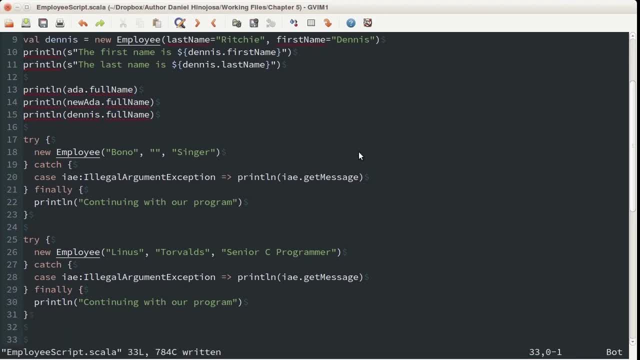 argument: exception. I don't want this employee script to fail, so I'm gonna put in a try catch block and I'll have this finally here to prove that we're able to continue along with our program. so we went ahead and save this. now let's go ahead and compile our employee Scala. 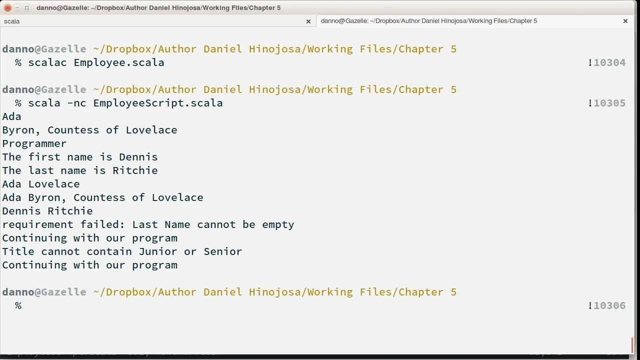 then we will run. our script works fine. so we see that title cannot contain junior or senior and we're able to continue along with our program. now we handle it in a way that was verbose and again I prefer to use the require. but this last example that we did just gets a point across as to what require does. 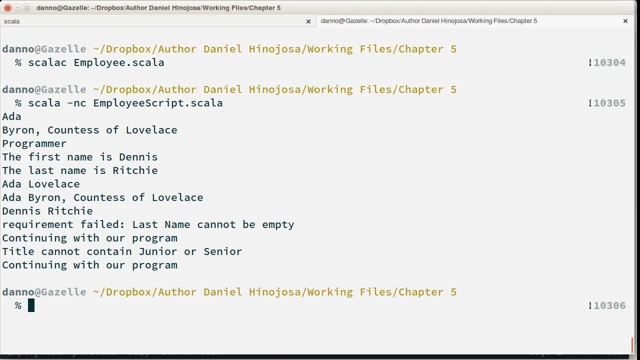 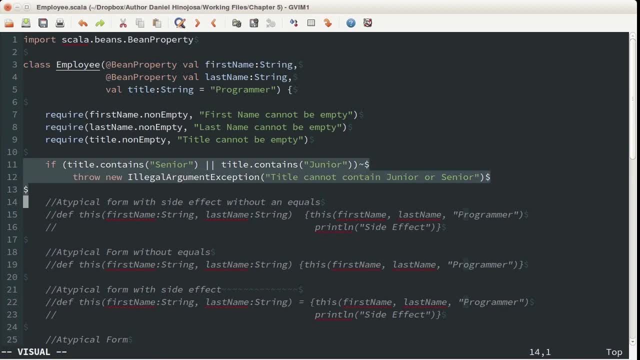 plus, we're able to dabble in throwing our own exception. let's go back to the code and take a look at that. so here is where we do our try catch and here is where we throw our exception. now, what about no? so in this scenario, it's very well feasible that first name, last name and title could be. 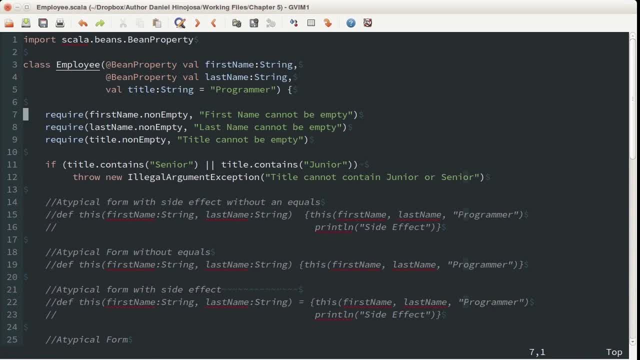 null, and I'm gonna leave this up to you. it's certainly up to you whether or not you want to check for. no, if you want to be aggressive- and again, there's nothing wrong with that- to make your class airtight, you can certainly check for. nulls. I will say this Season, Scala developers will regularly might leave your Jupyter data linux free if your script runs bad and sucks and we'rerewilded into a some way that makes senseént. I'm going to do a little fl 我們. 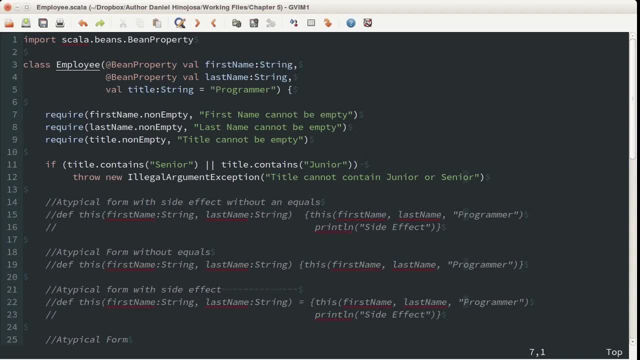 season scala developers finalize December school plan уверt��. rarely use null, if at all, So you may not have to worry about it Now. seasoned Scala developers will have to worry about null if this particular class is going to be interop with Java In other 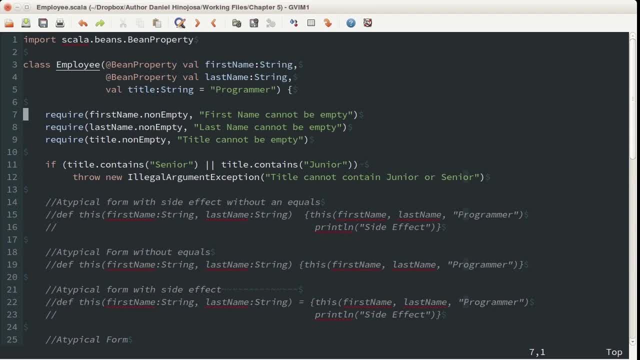 words, it's going to be working with some pre-existing Java code. Then there's also the other situation where novice Scala programmers, particularly from languages that use null consistently, will likely use null the first few times they use it in Scala. So I guess the answer. 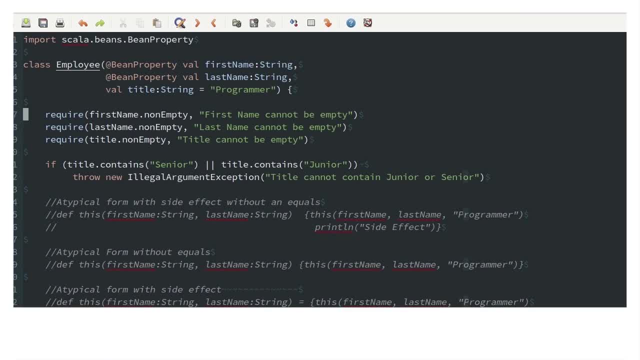 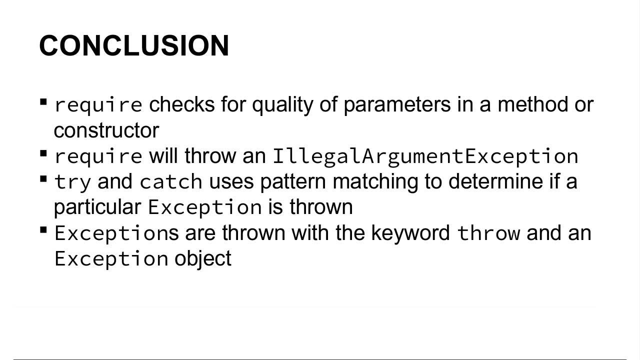 for this is going to be know your audience and I'll let you make that call. So, in conclusion, require checks for quality of parameters of either a method or a constructor. Require will throw an illegal argument. exception if the requirement is not met. Try-catch uses pattern. 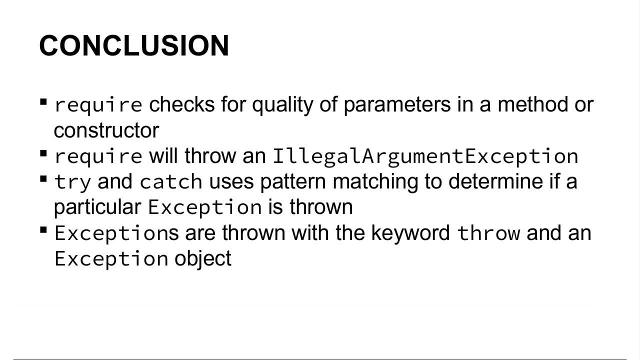 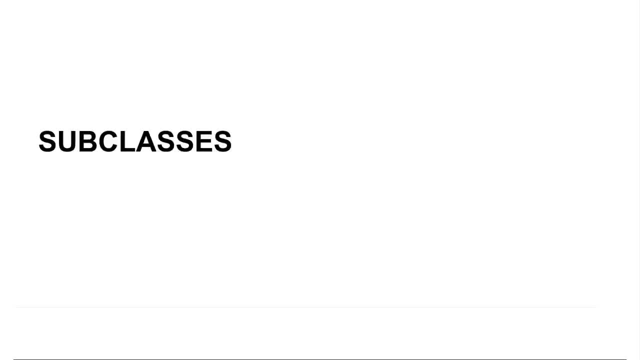 matching to determine if a particular exception is thrown And exceptions are thrown with the keyword throw and, of course, an exception object. In this session, we discussed subclassing, Scala being a true object. So let's get started. We want to go back to our employeescala file. Let's go ahead and make some. 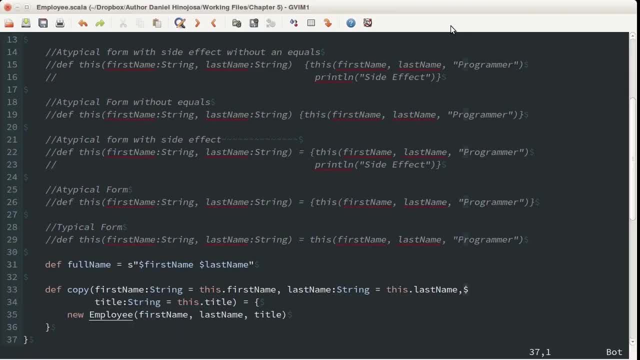 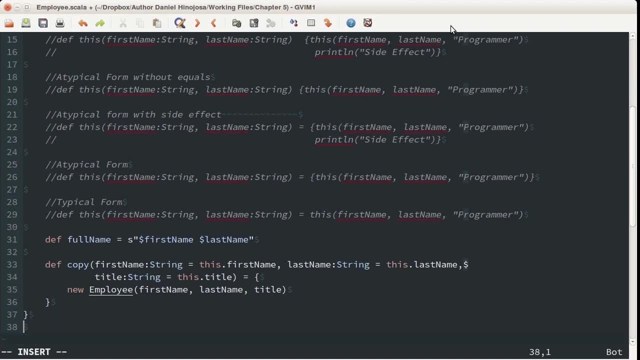 changes to that. So here we are in the employeescala file And, to start things off, I'd like to create another class called department. To keep things simple for now, in department I would just like to have a name And let's add a few lines. here I'm going to create a department. This will only 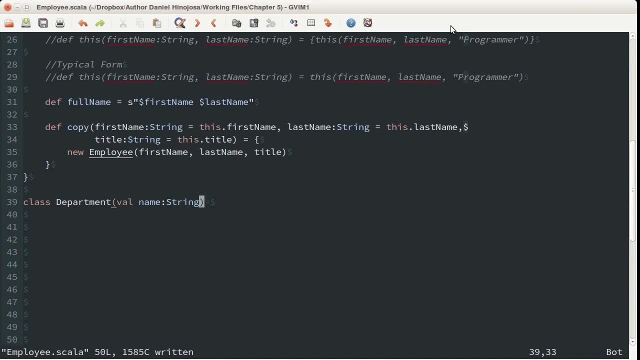 have one attribute And I'm going to create a department. And I'm going to create a department. Now this is in the class we'll be subclassing. Our subclass will come in with a new class called manager. So let's create that manager class Now. manager is going to have the same attributes as 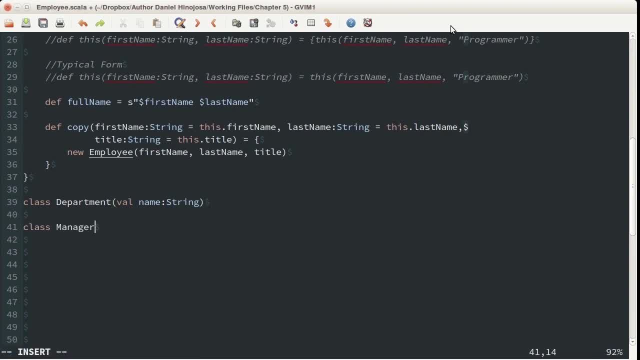 the class that it is inheriting from, And we're choosing to inherit this from the employee class, So we're going to have the first name, the last name title- This is new- the department. That's what's going to differentiate the manager from the employee. Next, the extends keyword. This is 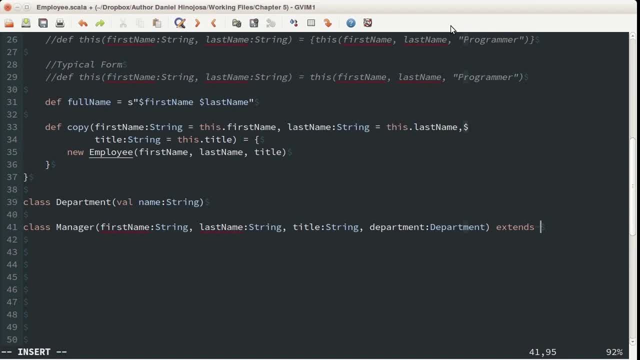 the name of the class that's going to inherit behaviors in state from a parent class. Then finally, employee. What we're going to do here is we're going to select the attributes. that comes into manager. that is handled by the superclass. So first name, last name and title are all handled by the 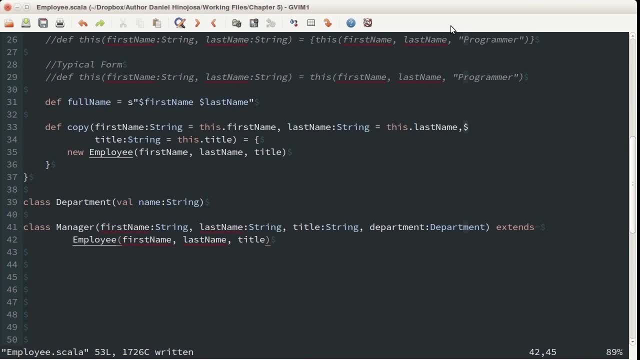 employee. superclass Department, on the other hand, is not. Now, manager is distinct from the employee because it has this department, But a manager is still an employee. A manager also has a first name, last name and title, Just like the employee, And the department, since it is distinct to the manager, will likely have a. 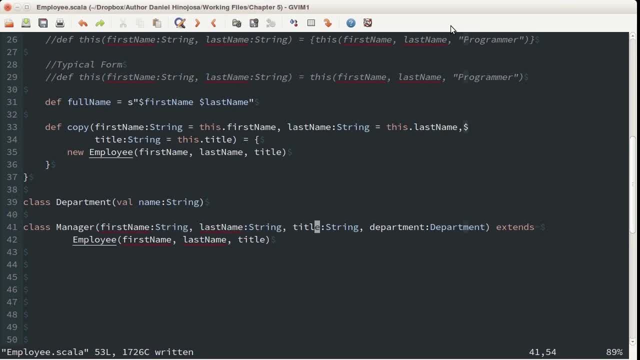 val in front of it. Now, we don't have to have a val in it. This is just so. that way we can get an accessor for this department. But if we just wanted to inject this value in and not have an accessor for it, we could just remove the val. We could also have a var, but, as stated before, we don't. 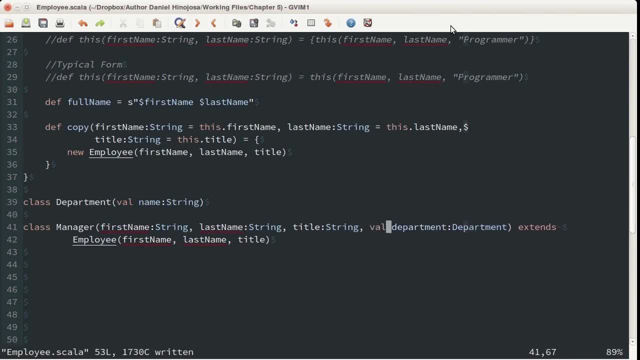 particularly like var. So I'm going to add a val in here and state right here that this val, since the department is part of a manager, we want an accessor. Now there are no vals in front of first name, last name or title, because they are forwarded over to the 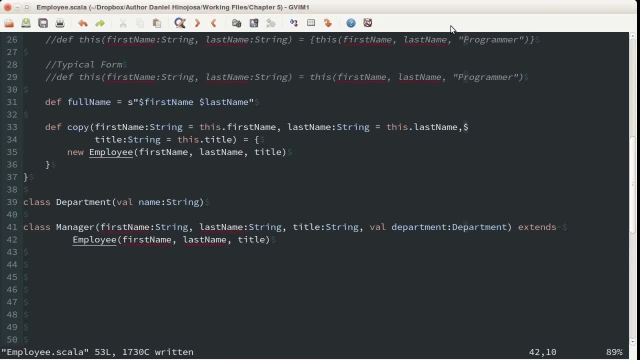 employee superclass via the extends keyword. The class name after the extends shows which class we are subclassing from And in this case that's going to be the employee. There is one very important rule when subclassing: When subclassing, it is important that the subclass has a is a relationship with a. 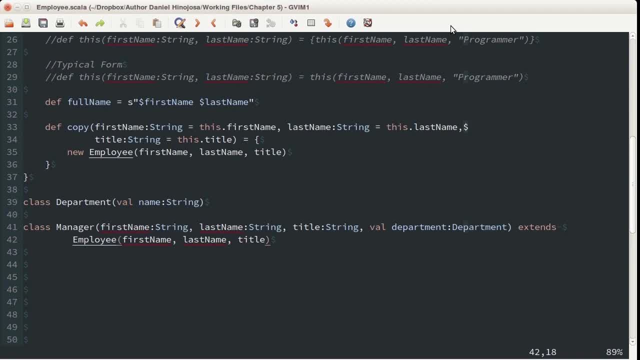 parent class In our example. is a manager an employee? The answer to that is yes. Therefore, that works. Many who are unfamiliar with object-oriented programming and design may want to reverse that relationship. The problem is that it doesn't adhere to this. is a relationship policy. Is an employee? 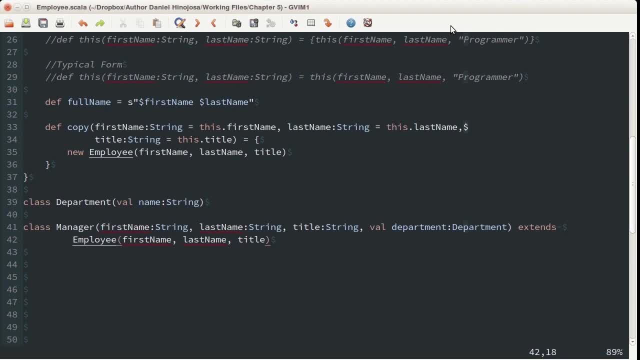 a manager- Well, not all of them, So therefore it does not adhere to the is a relationship policy. Be very worried about extending from classes like manager- And I'm not talking about the manager we're creating here. We're talking about the big manager classes that some companies tend to create. 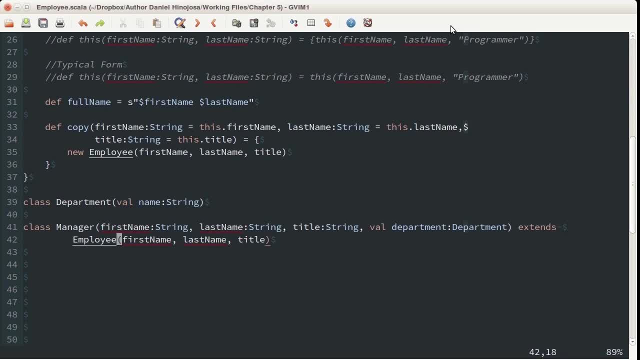 that encompasses everything, Every kind of business logic that the business does. Another violation would be a class called context. Context could be anything When you're using these broad terms and you're extending from these classes that are too broad or even creating classes with those names that are going to encompass just about. 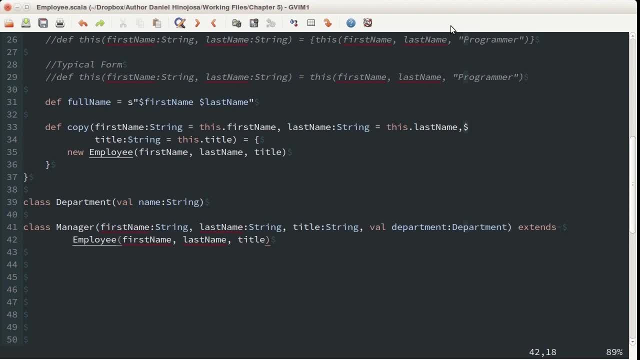 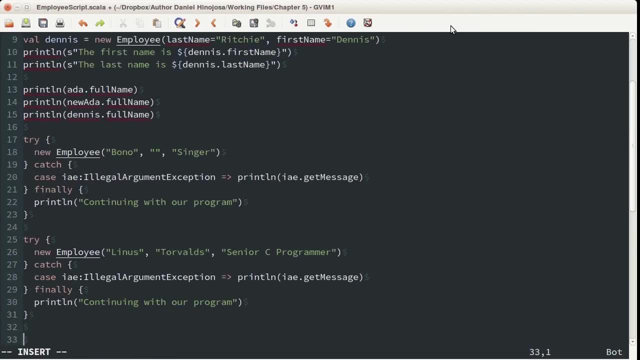 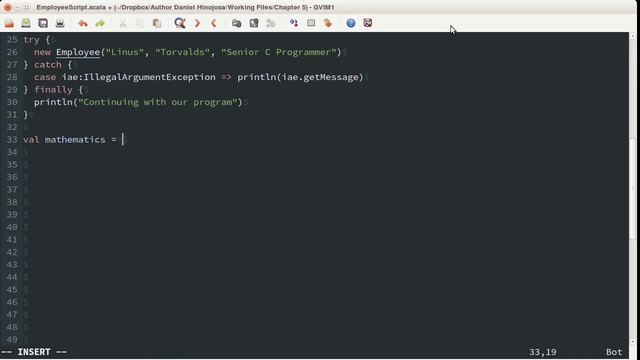 everything, you're likely modeling your application incorrectly. So think about your design. Now let's try this out inside of our employee script. Let's add a few lines here so we could see what we're doing. Now I'm going to start things off with a department, and this is the mathematics department, Since department has one. 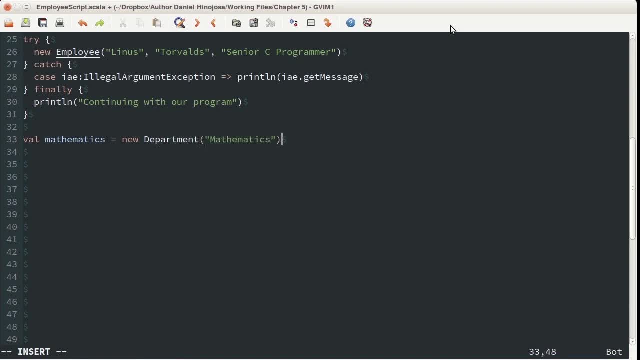 attribute called the name. we're just going to provide that with the name here. Next, I'm going to create a manager, and it'll be none other than Alan Turing, mathematician and logician, And then, finally, we're going to give him a. 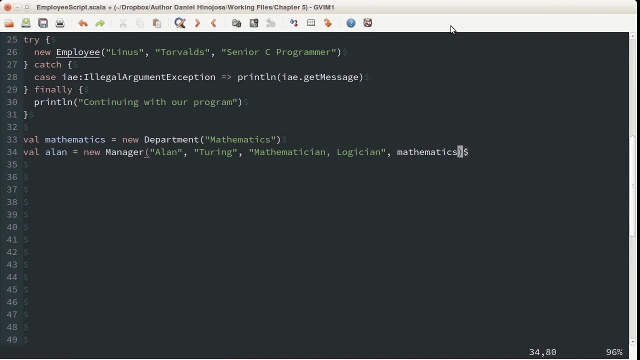 department. So we're going to take this reference and plug it into the constructor. Now, to test things out, Let's try a print line, And what I'd like to do is take Alan, take his department. Remember we created that Val. 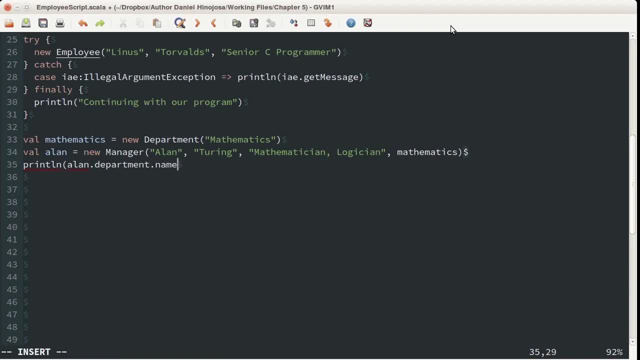 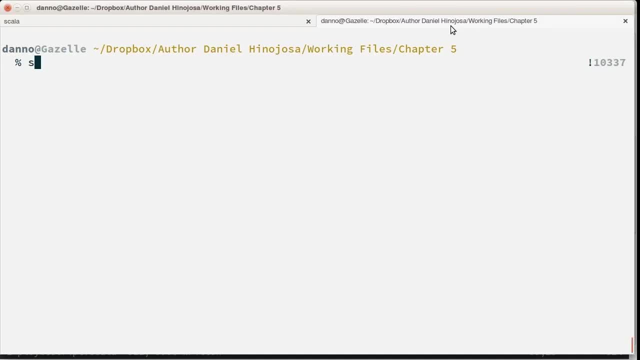 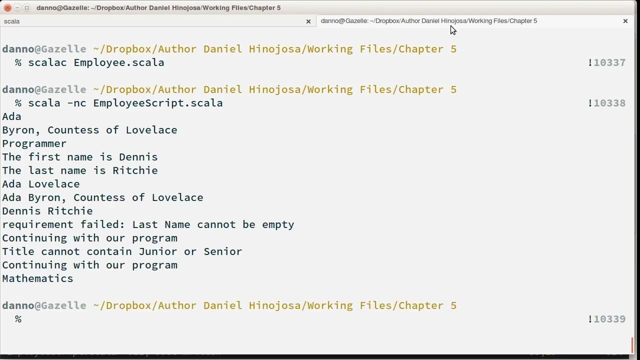 under departments. So that way we could do something like this and then get the department name. So we went ahead and save this. Let's go ahead and compile employee Scala and then run the script. So we're going to compile. Now we're going to run Again, I'm going to use NC. That way we don't use the fast compiler in our example. Here's the name of the: 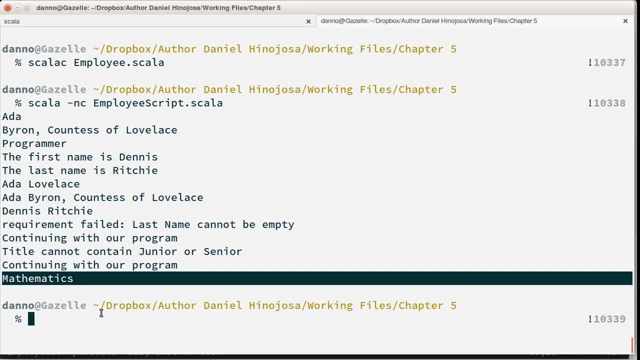 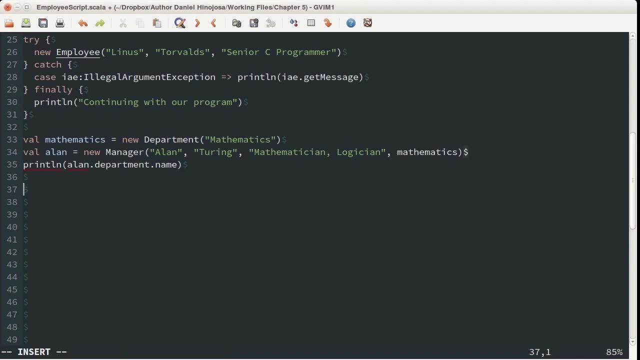 department. Pretty nifty: We can create managers. now, What we could also do is assign a manager object to an employee reference. So let's go back to our employee script and play around with some of these references And we'll assign Alan Turing as an employee. Now, in this case, right here, what I'd like to do is: I would like to create 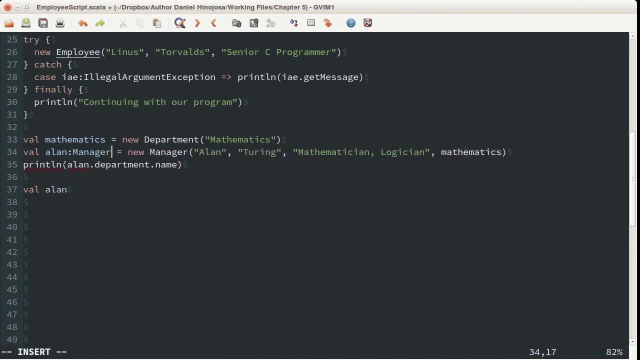 another reference. So this Alan right up here has a reference of manager implicitly because there is type inferencing going along. So we didn't have to declare that explicitly. But let's say we're going to declare that explicitly And let's create another reference called Alan employee And Alan employee is going to be an employee reference. 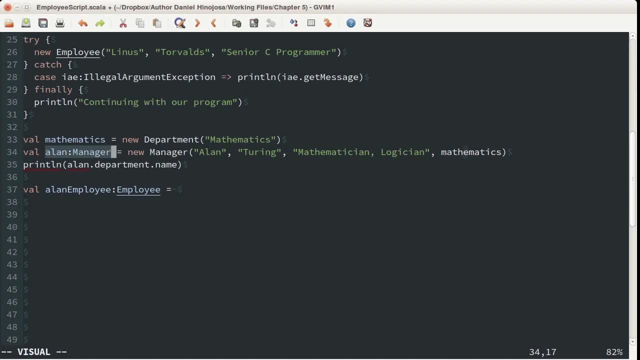 Alan's job. the reference I'm talking about right up here is to point to manager objects. Alan employee's job as a pointer is going to point to employee objects And what that's going to point to is the same reference as Alan. Now what we can do is: let's do some. 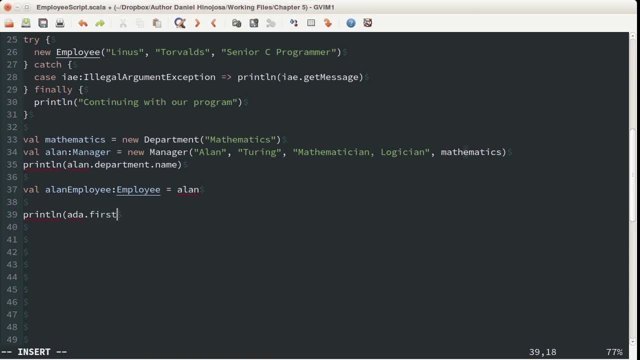 print lines. I'd like to ask Ada what her first name is, because this is an attribute of employees. I could also ask new Ada what her name is. I could also ask Dennis what his name is. I could also ask Alan what is his name And, finally, I could also ask Alan, as an employee reference, what his first name is. So let me save all this. 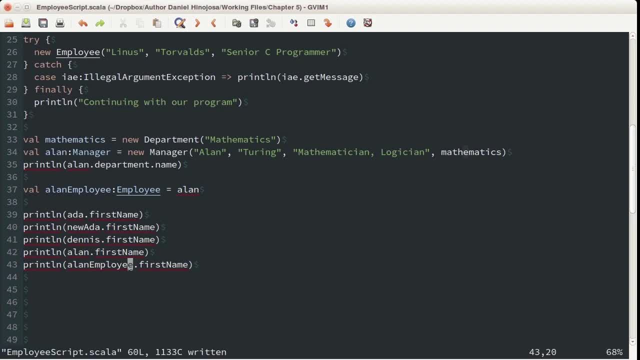 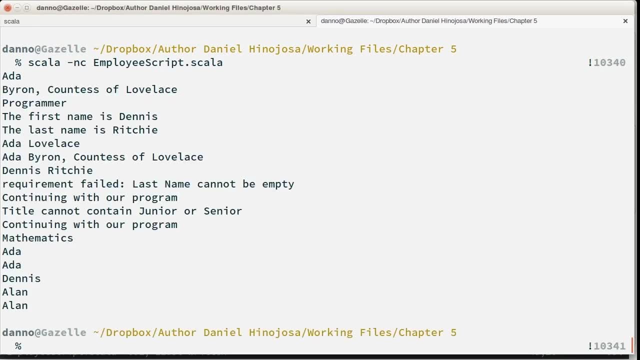 So I have five lines here. I'm just asking every employee object I created, whether it is a manager or an employee, what their first name is. So let's go over to the terminal and give this a try. Great, So we have Ada. Ada. This one is the first Ada reference. This is the new Ada reference. 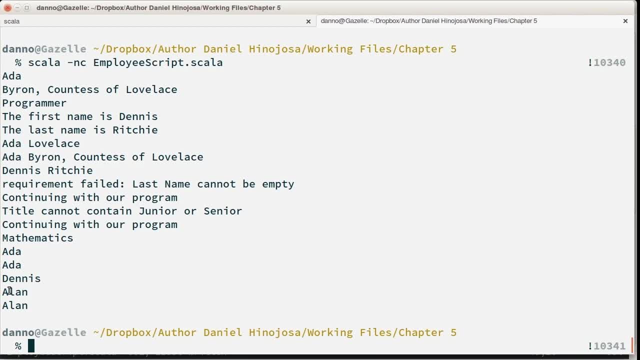 Here's Dennis and here's Alan. One, because we are using the manager reference. Two, because we are using the manager reference. Three, because we are using the manager reference. The other one: we're using the employee reference. Now, let's change things up. What I'd like to do is ask Alan. Let's try Alan. 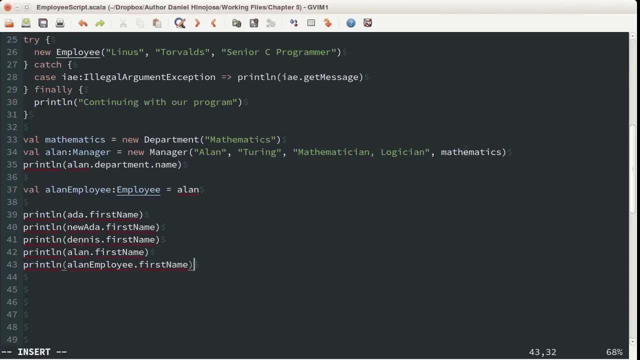 employee this time. what is department and name is- Remember Alan- employee is an employee reference, So let's see what happens when we call this. Now. we know that the object itself has a department, but the reference is an employee reference, So we're not going to be able to ask this. 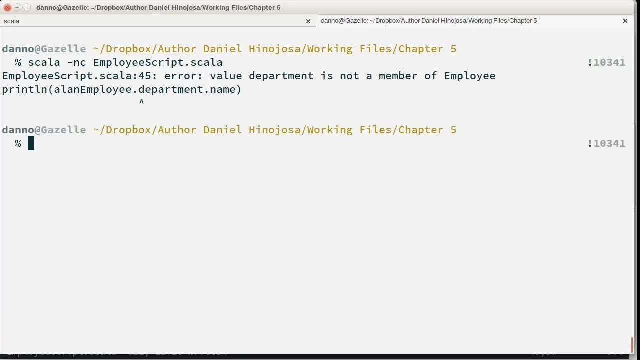 question And this will state right heremileau Department is not a member of the office. I can change it as client. I have to sit in this virtual device and perform job repair. Then I need to bring up what department I'm in And if that's the case I won't have just to connect with my administrative. 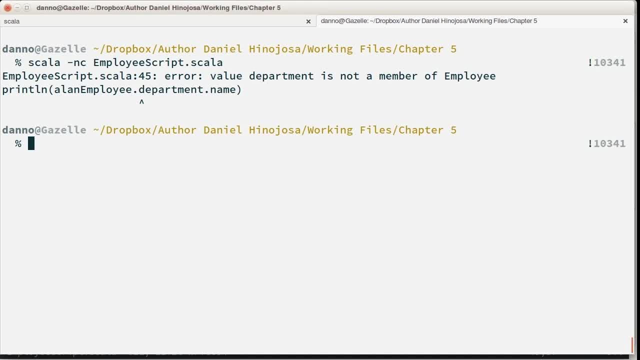 of employee. Remember all: an employee is an employee reference. Yes, it's pointing to a manager object, but the reference is an employee, So this is not valid. Let's go back to our code and fix that. Let's do a sanity run. Everything works. Now let's go back to the code. Now what? 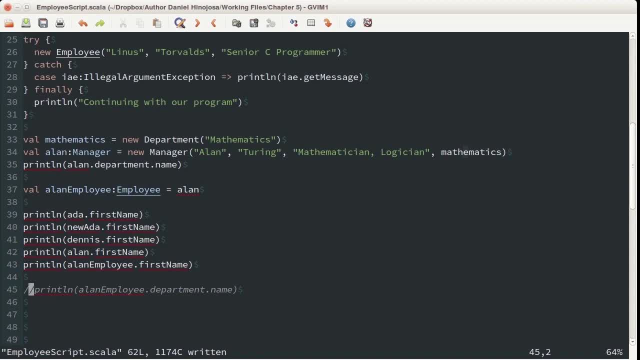 we're doing here is something called polymorphism, the ability to assign an object to any of its hierarchical supertypes. The type of polymorphism also applies to methods. So let's try some method polymorphism And we're going to add a method to the employee script to give it a try And the 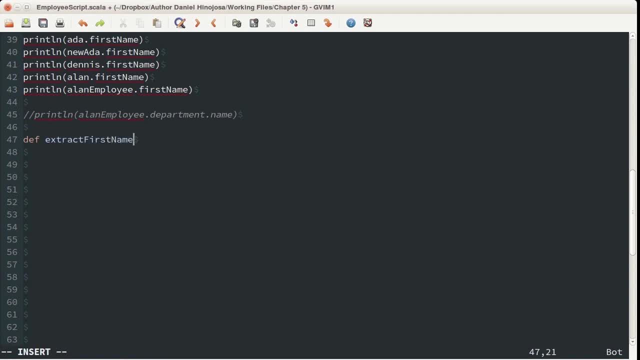 method I want to create is extract first name, And this method will only accept employees. But this will return a string, the implementation, the dot: first name. Now we can let type inference take care of this part, right here. This will still work. Now let's add a few items. We want to extract the. 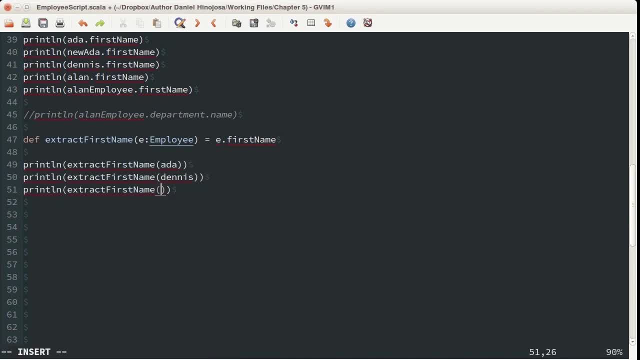 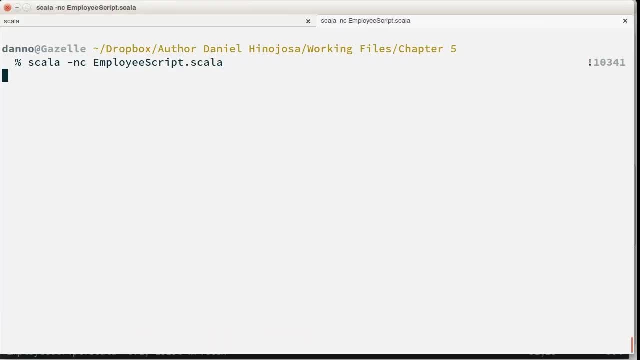 first name for Ada, for Dennis and for Alan. The first two are employee objects, The third one is a manager. So let's do that, And we're going to add a method to the employee script to give it a try. Let's go ahead and save this And now let's run it. There it is, We're able to obtain the first. 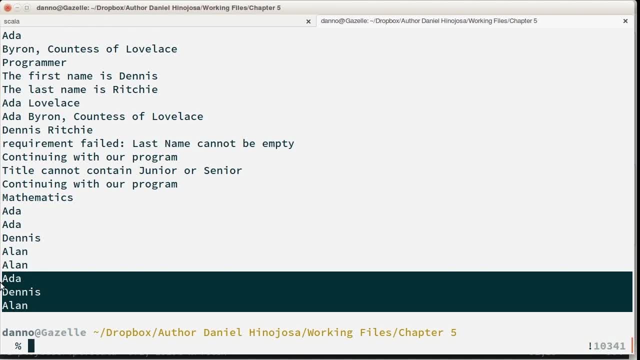 name, because the method accepts employees and every employee has a first name, whether it is a manager or whether it is an employee. Now something kind of weird is happening to our employee dot Scala. Let's go back to our employee dot Scala. We have a class here. we have a class. 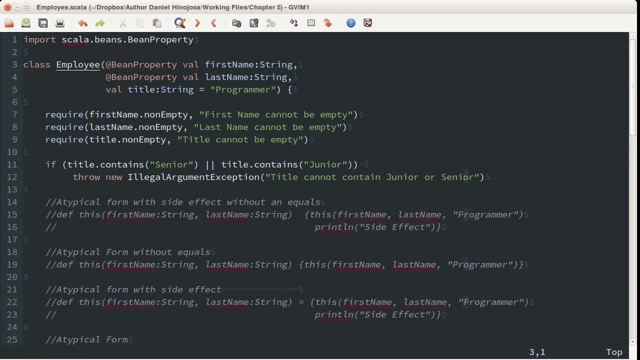 here and we have a class right up here. We have three classes in one file Now for the Java programmer. that is really weird. What did we just do? We have multiple classes in the same file. So no longer, especially for the Java programmer, for you. no longer do you have to. 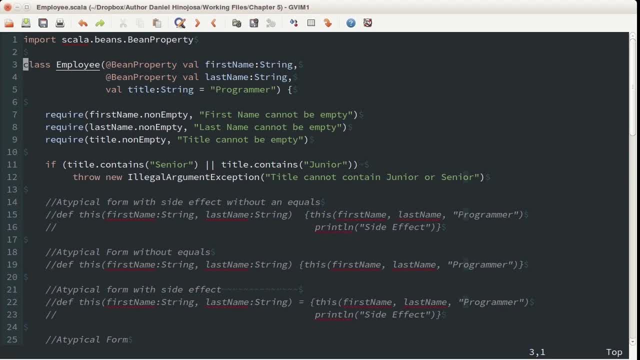 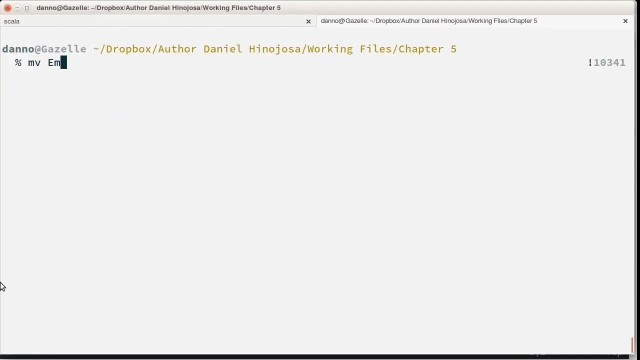 have one class per one file, nor does it have to be the same name as the file. And since we don't have to hold to any of these rules, let's rename our employee dot Scala file to models dot Scala, models being nouns. So let's head over to the terminal. So I would like to move employee dot. 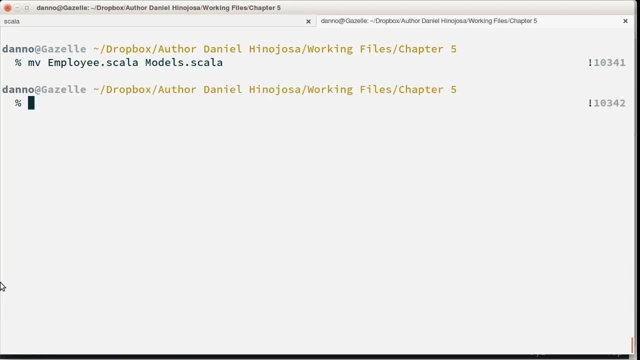 Scala to models dot Scala. Now what I'd like to do- let's remove all the class files that are in here, And this is what it looks like. I have models dot Scala now because we renamed that employee dot Scala to models dot Scala, And then we have our employee script. Now I'd like to 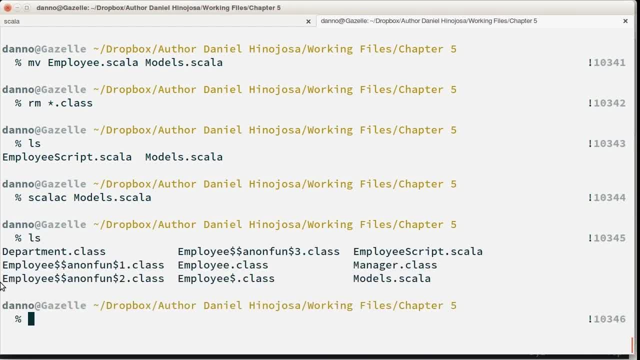 compile models, dot Scala. Let's do an LS here. Take a look at the directory. As you see, here there are a lot of class files and supporting class files And even though we had an employee class, a department class and a manager class inside the models, it was able to detect those. 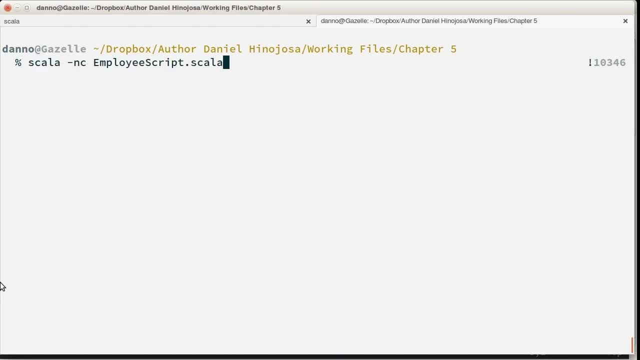 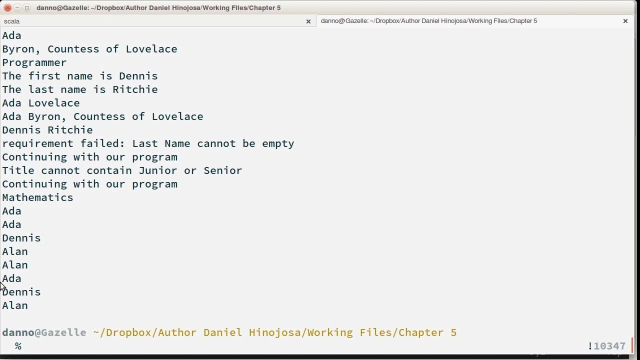 and then create those classes whenever we compiled. Now, when we run this, it works out just the same: Class files are class files. This flexibility, when used judiciously, can save the developer a good amount of time from file haggling. You no longer have to create the 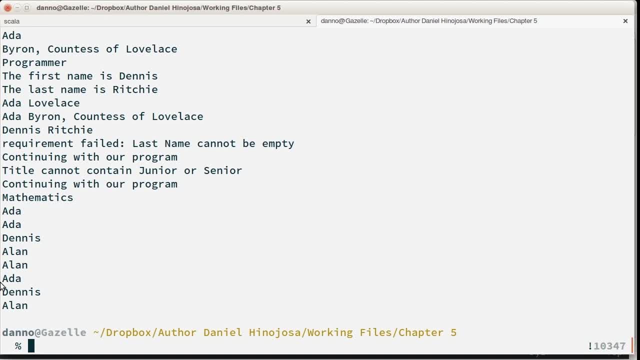 one class per one file. Some of you may view this as more difficult, since it is no longer obvious that classes are in a file just by looking at the file name. I'll let you form your own opinions whether you consider this a good thing or a bad thing. So, in conclusion, extends is a keyword. 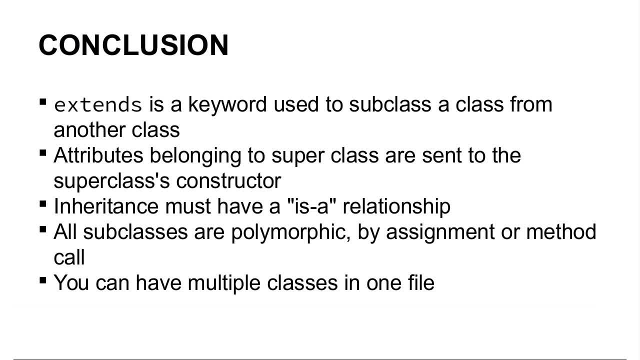 used to subclass from another class. Any new attributes typically will have a val or var, or you can leave them blank if you wish not to expose the property. But all properties that come from the superclass are sent to the superclass's constructor. Any inheritance from the superclass must have a is a relationship. 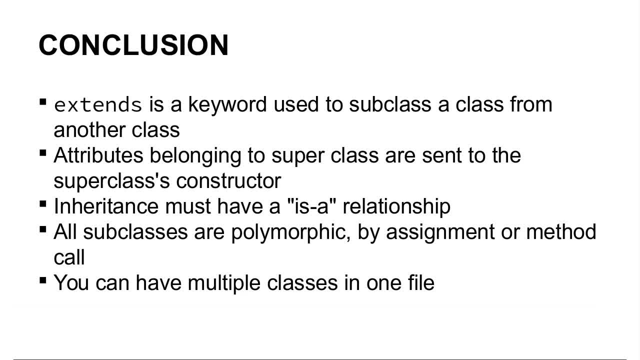 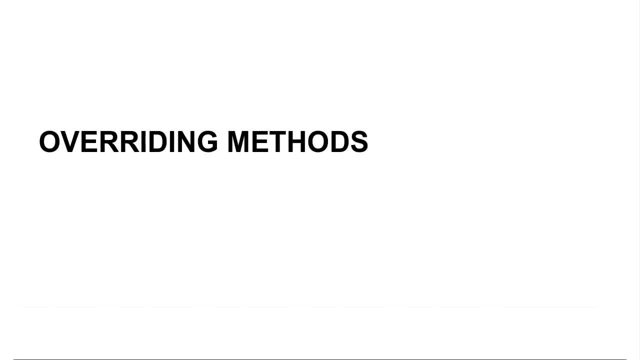 All subclasses are polymorphic, either by assignment or method call, And you can have multiple classes in one file. In this session we'll be covering how to override methods from a superclass. is a necessary procedure to redefine a method from a superclass with a refined implementation. 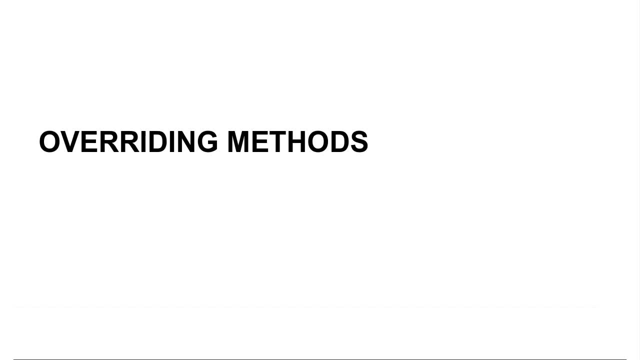 that fits your subclass's goal For this session. we'll keep it simple and override our full name method from employee and do it inside of manager. We'll also override copy and we'll also continue to use overriding in our next sessions when we perform equals hash code and two string. 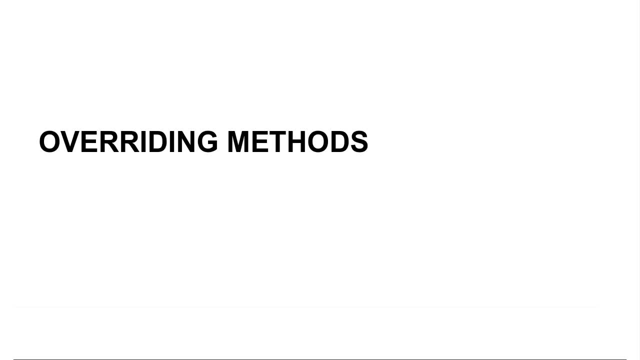 implementations In any object-oriented programming language. a method override allows a subclass to provide a detailed implementation of a method that is already provided by one of the parent classes. Given that we have a method called full name in employee, we could override full name to give it. 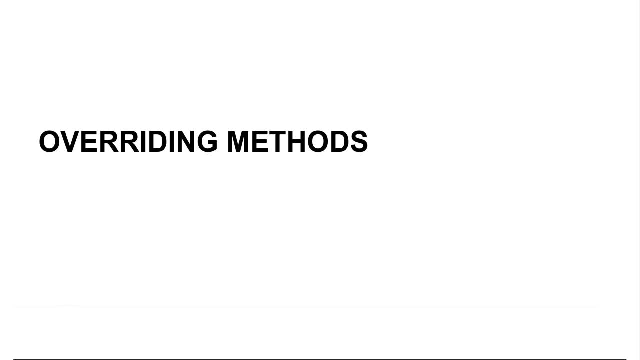 a different implementation in manager, one that reflects a more apt full name. In Scala, as in Java, an override must have the same exact signature. To get started, let's go over to modelsscala and override the full name method in the manager class And, for example, let's make that full name return. 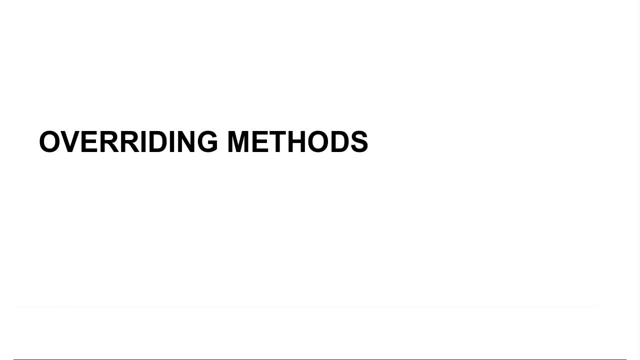 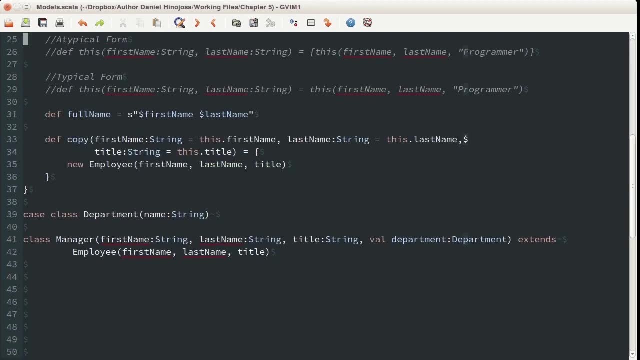 something different: The first name, the last name and the department name. Here we are at modelsscala and we have our case class department that we had last time, and we also have our manager class. that brings in a first name, last name, title and a department which. 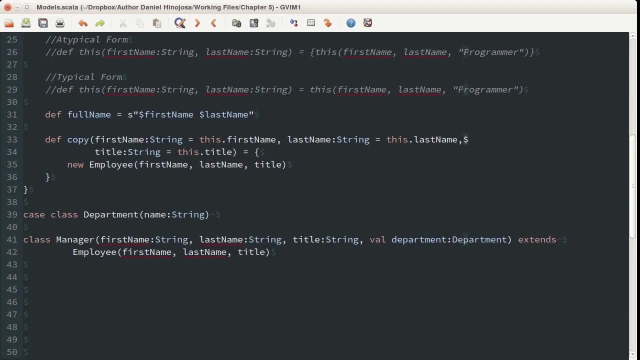 extends an employee, that will take that first name, last name and title from manager. But department has a val, so this is a property that belongs to a manager. What I'd like to do is override full name and on my line 31 here it shows that dev full name is equal to the first name and 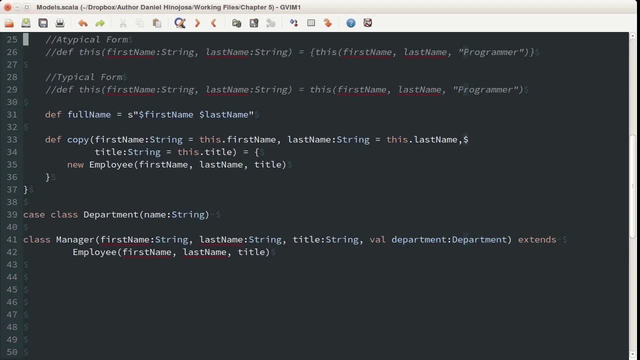 last name of the manager. So I'm going to override that and then I'm going to override the full name of the first name and last name. I wanted to add a little bit to this and create a different implementation for full name. Now, within here, I'd like to override the full name and give it. 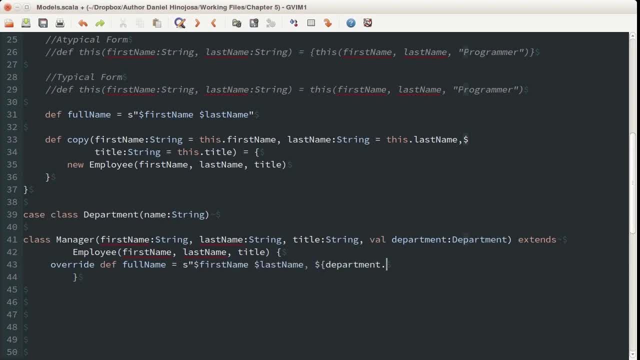 a different implementation. Now, one thing you'll notice with our addition is that there's a new keyword called override In Java. this is an annotation and it's used as a safety net on whether a method is indeed overriding a method from a superclass. Remember, an overridden method has to have the same signature as the parent class And this keyword. 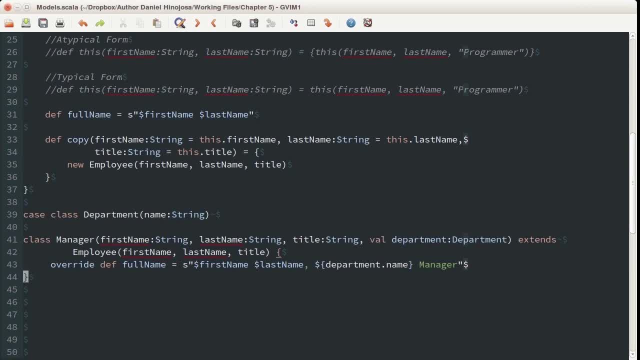 is an overridden method In Java. the annotation will ask the compiler to please check and make sure that we're following all the rules. In Java it uses an annotation and that annotation is optional, Unlike in Scala, which is mandatory. the override that you see here on my line 43: 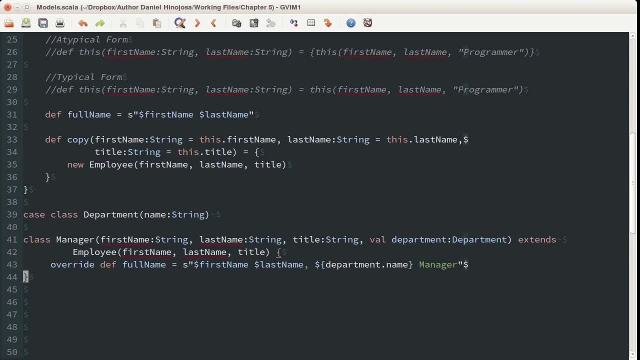 is actually a keyword, a part of the language. Not only does it check for being an exactly an overridden method at compile time by checking the signature, it's also a way that we could explicitly state that our intent here is to override. Now let's go to. 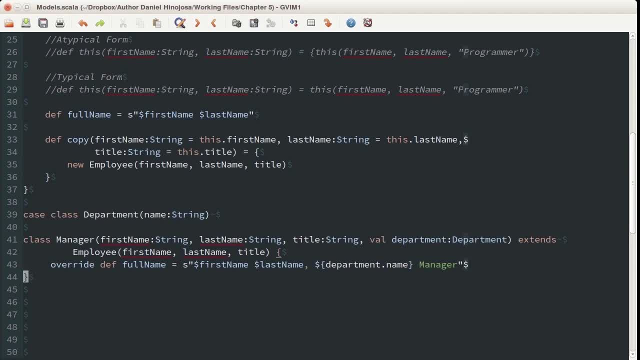 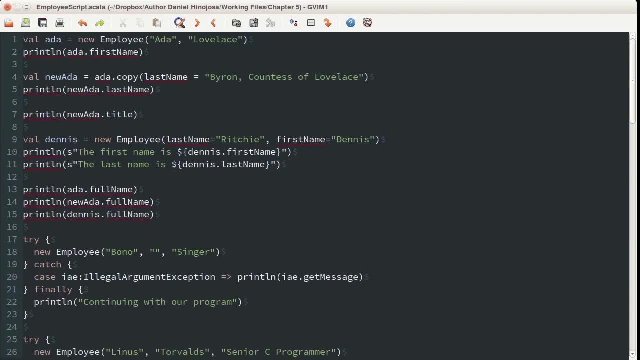 employee script and try out our full names once again, and within there, let's print out the full name for some of our managers. Okay, here we are under employee script and we've had this from our previous sessions. What I'm going to do is I'm going to copy these three right here, which print: 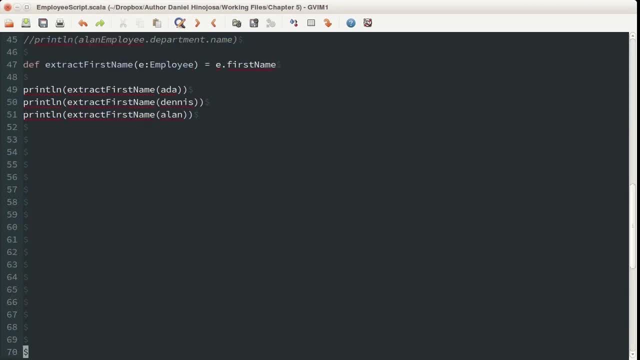 out the full name for Ada, new Ada and Dennis. I'm going to go down here to the bottom and paste them right in here. So I have Adafullname, new Adafullname and Dennisfullname And I'd like. 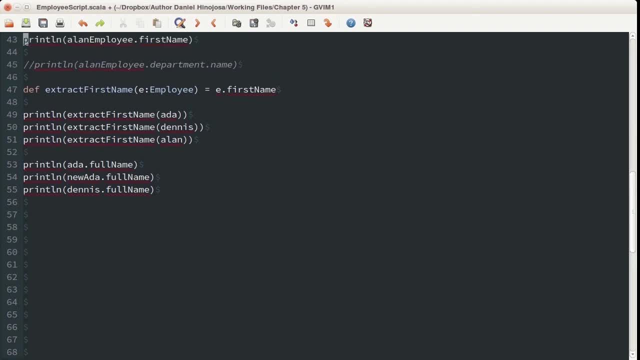 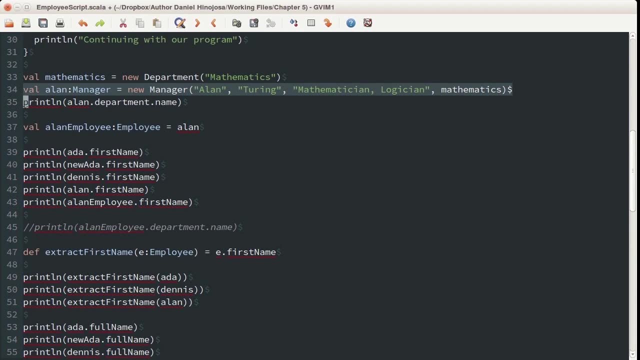 to add a couple more. Before I add those couple, let's refresh. right up here I have Alan, which is pointing to a manager, and this is pointing to a new manager that has the first name of Alan, last name of Turing, title of mathematician logician and is a part of the mathematics department. Now my line 37 here. 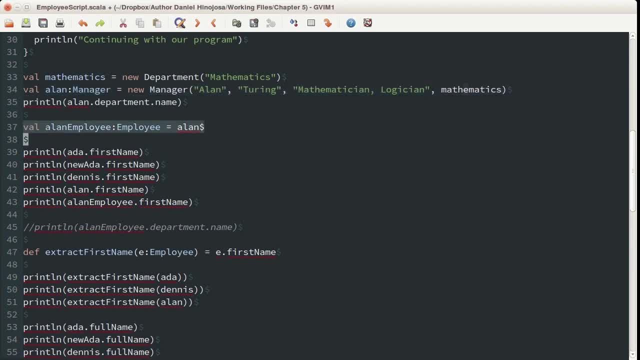 I have another reference called Alan employee, but this points to employees and this is legitimate because as an employee pointer, we can point to a manager. A manager is an employee, so this is okay. Now, at the bottom, I'd like to add a couple of print lines. Question is, what are the bottom two? 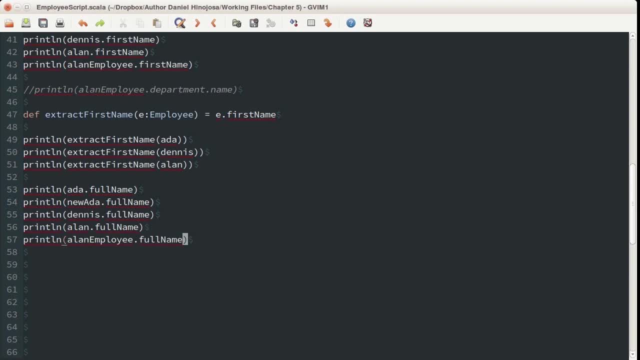 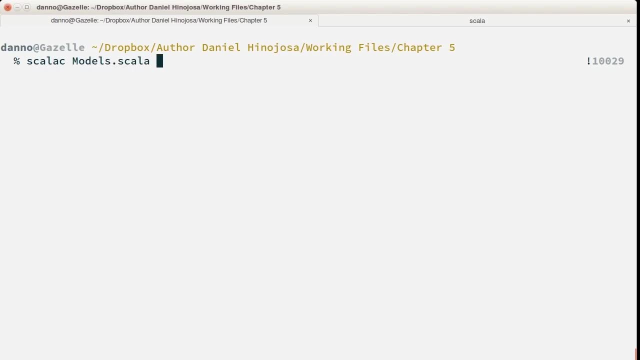 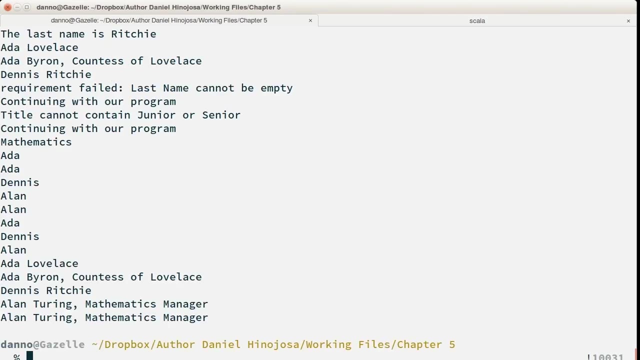 going to be. That's an interesting question. Well, I'm going to go ahead and save that and let's go over to the command line and give it a try. Here we are, the command line. First let's compile modelsscala, and now I want to run this script. Let's avoid any caching by using dash and c. Very interesting. 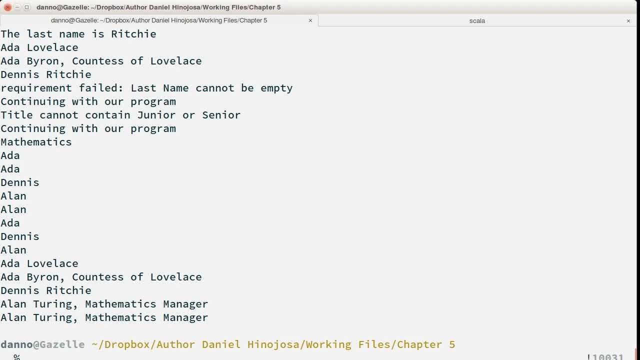 The last two are going to show Alan Turing, mathematics manager. Remember, mathematics is the department that Alan Turing is in. Alan Turing happens to be a manager of. Now we see that the implementation is different based on type. Last five we're actually looking at Ada Lovelace, Ada Byron, Countess of Lovelace, and Dennis Ritchie. 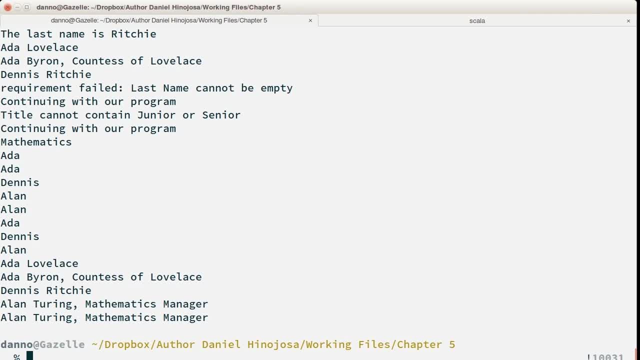 are all employees, but Alan Turing is a manager and even though the second to the last one is pointing to the manager and the last one's pointing to employee, the references that they're pointing to don't matter. What matters is the concrete implementation for each object. 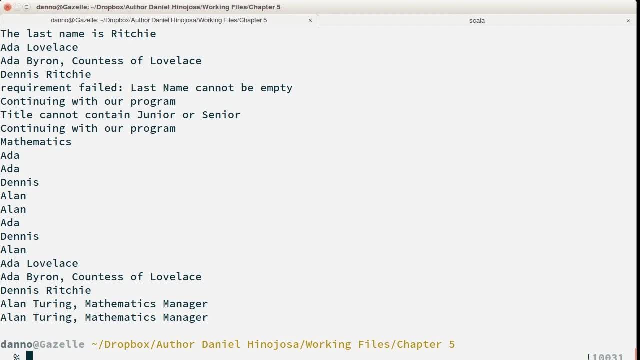 You'll notice that, interface wise, the last five all have a method called full name that looks and feels the same, And notice the strange twist at the end from our last session. We called Alan employee and noticed that we couldn't call department because we had an. 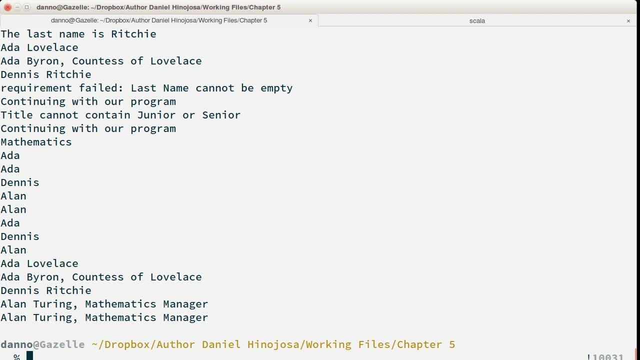 employee reference, not a manager reference. Now, this time, since both of them have full name for both the employee and the manager, the result is: what we're looking at is the implementation of a manager in the last two, not that of an employee. This should make us all at ease that it doesn't matter. 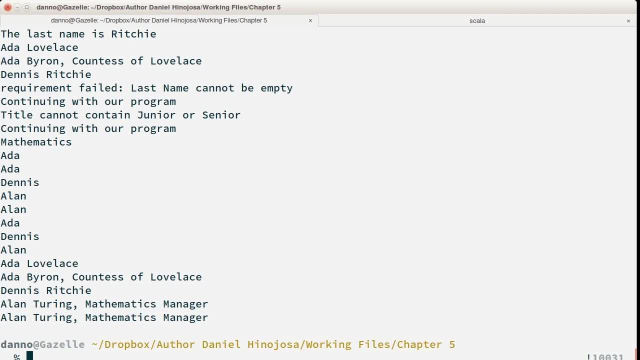 what reference we're using. We don't care if we're pointing using an employee reference or a manager reference. What matters is that we're pointing to the different manager references. So let's go over to the editor section. is the implementation of the object where this was created, Since Alan Turing's a manager when 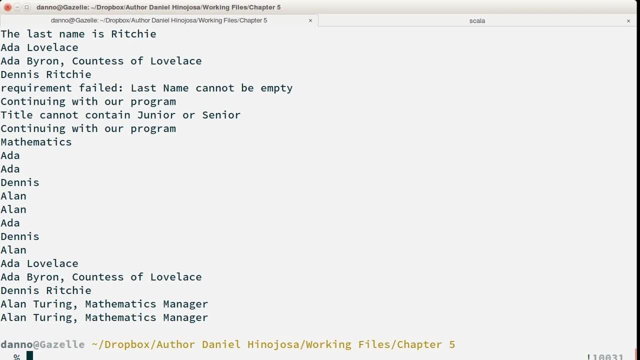 we call for his title. it's going to be his first name, his last name and the department that he is a manager for. Now, all this is method overriding, and we'll be using it extensively in the next few sessions when we discuss equals two string and hash code. Now we could also override the. 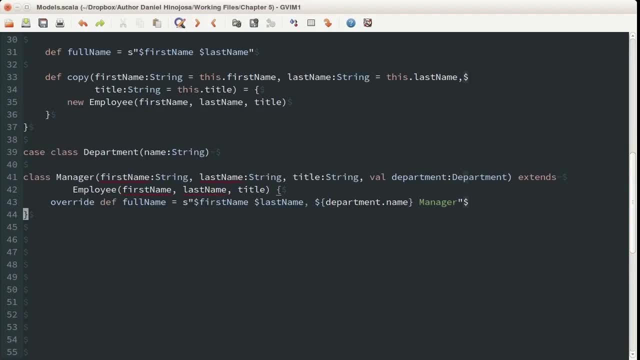 copy method. Let's give that a try. Here we are inside of modelsscala and what I'd like to do is override copy that I have here. So what I'm going to do is I'm just going to go ahead and copy this and save some time. Before I continue, the few things I need to change. First off, this: 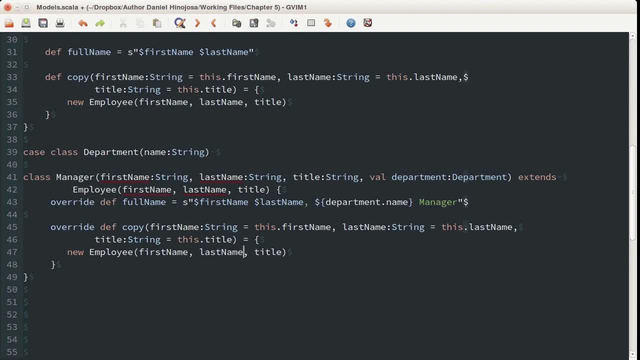 is an override. The arguments need to stay the same. This time, though, I'm going to be creating a manager, not an employee, and because it's a manager, I'm going to give it a department. Now, a true copy would allow me to include my own department right after title, right up here, but 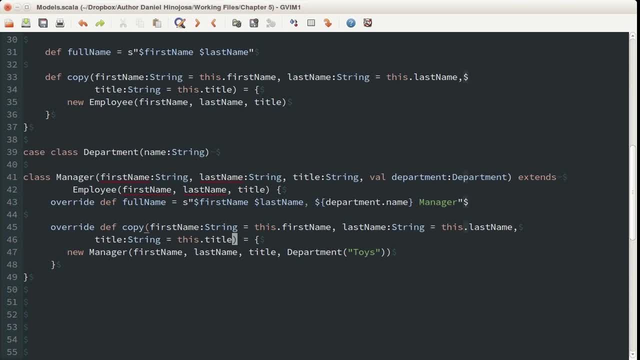 by doing that, I'm going to be able to create a department, So I'm going to give it a department, and by doing that, this is no longer an override but an overload. That's going to change things a bit, so let's do things a little bit at a time. And again, we're only talking about overriding, not 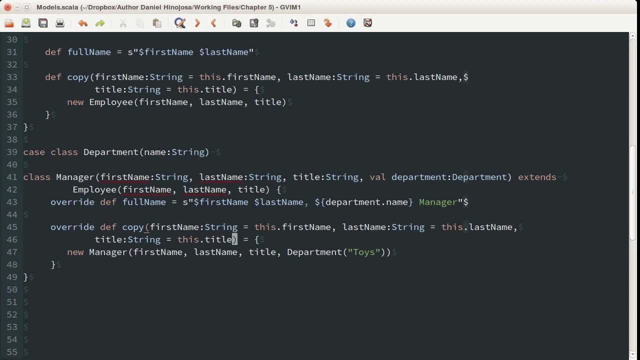 overloading. The moment we add a department to this, it's going to change things around. So let's stick with the override first, and what I'd like to do is let's go back to the employee script and change Alan Turing's title and see if the copy works. Here we are back at employee scriptscala. 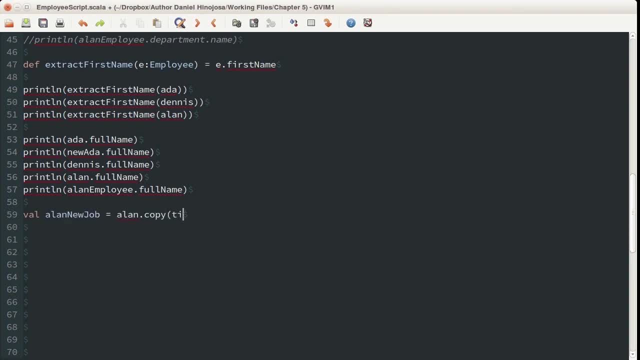 What I like to do is add the following: Let's give him a fun title. I'm going to take Alan, change the title around and change the title to Alan Turing. And I'm going to change the title around. This will be set to Alan new job, If all goes well. the last line from our output should: 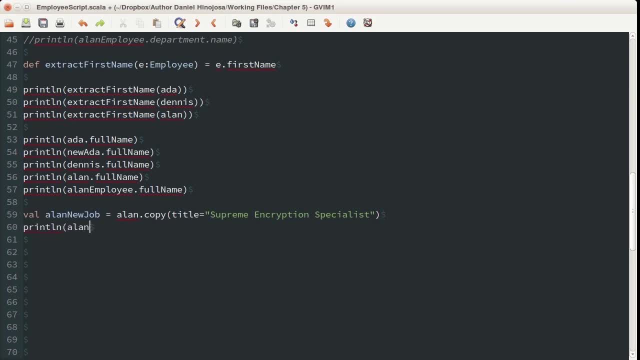 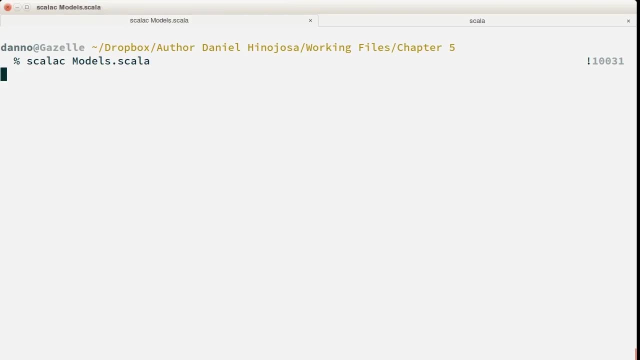 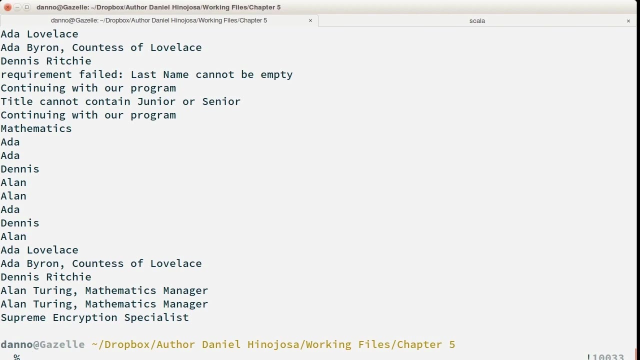 state that Alan Turing is a supreme encryption specialist. Let's go to the command line and give it a try. Here we are at the command line, So I would like to compile modelsscala. Now let's run the script. Great, there it is. The copy worked. For this reference, Alan new job, if we call the title. 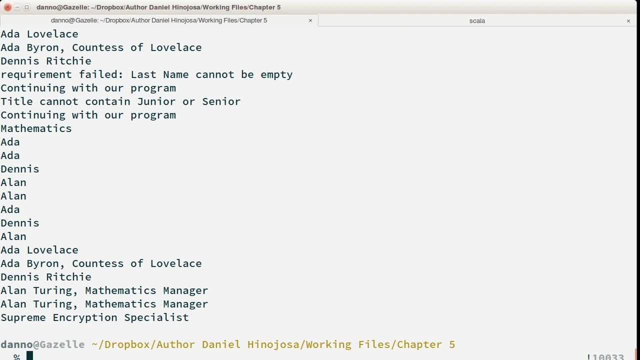 on it. this returns supreme encryption specialist. We could see that since Alan is of a type manager, the copy implementation of Alan Turing is a supreme encryption specialist, So I'm going to give him a fun title. Here we are back at employee script. Let's go to the command line and 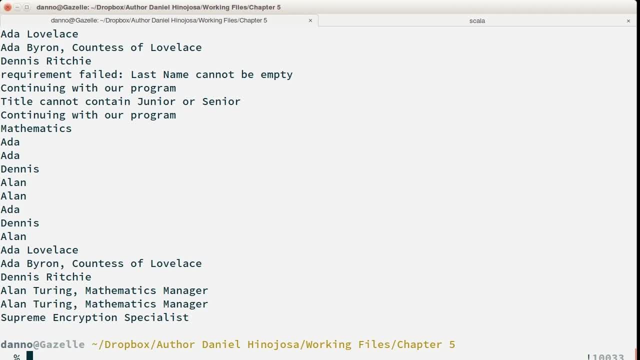 Now you may have noticed a peculiar problem, and we've stated this before: There is no department in our copy. So, to round this lesson out correctly, Let's change this from an override to an overload and talk about the difference, And this time I'm going to add a department. And, if you remember, 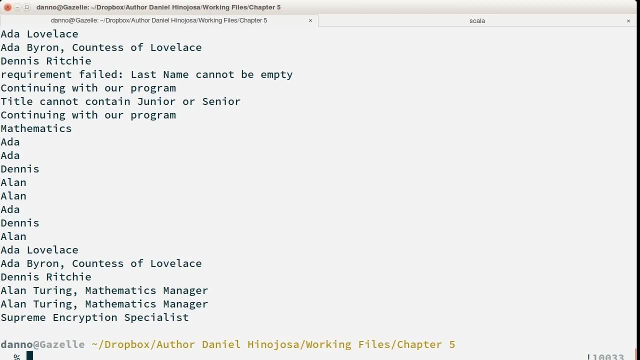 from the last chapter, and overload is where the method name is the same but the parameters, possibly the return type, can be different. And since we are adding that department, that is a significant change to make this an overloaded method instead of an override. First off, we need 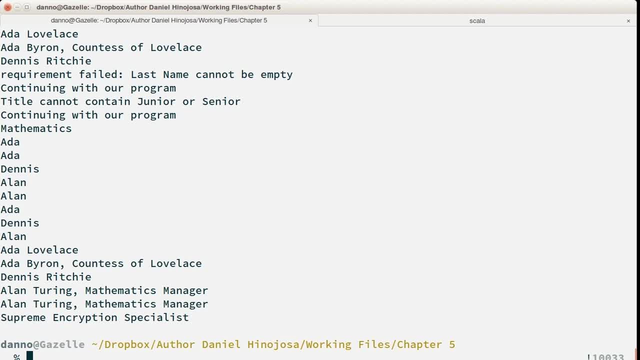 to get rid of the override keyword. Let's do so and change things up. Let's head back to our code. Okay, here we are, back at manager Few things that we like to change. Well, first off, let's go and 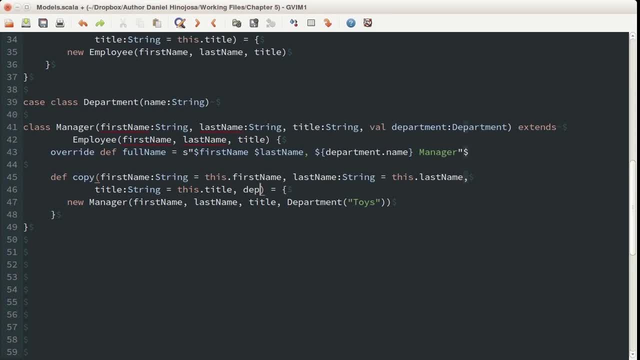 get rid of override. This is department, not manager. So we are going to add a department here And this will be the same as this dot department. Now, within here we don't need department toys. That was just a default filler because we were not accepting department. 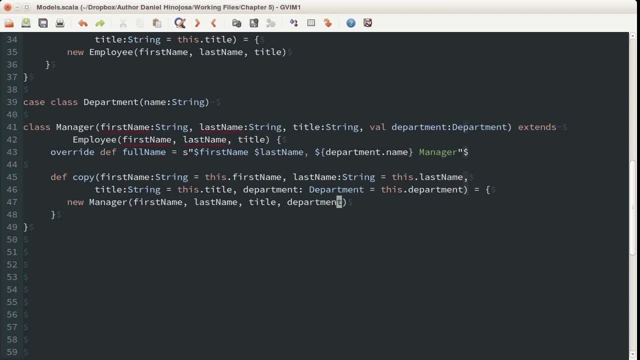 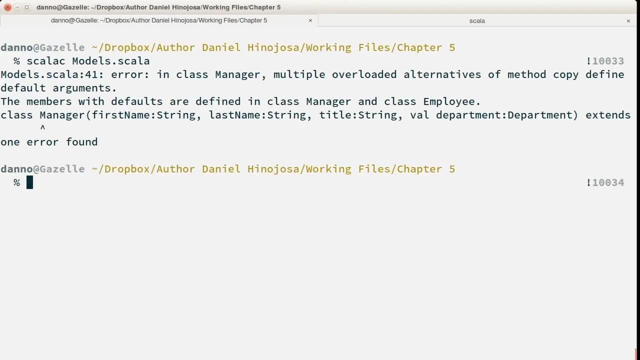 Before, And this time we will call department. That should do it. It's not going to work, But that should do it. Let's go ahead and save it and attempt to compile. This states right here that there's an error in class manager. multiple overloaded alternatives of method copy defined. 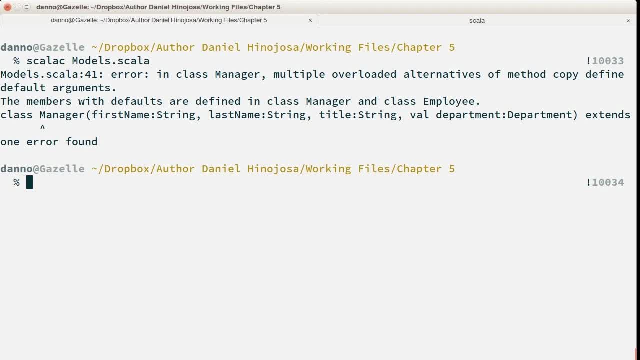 default arguments. I add this example as a warning that shows currently the fragility when it comes to overloading methods from a superclass that uses default parameters And again that uses default parameters. overloading is still okay, But it's not going to work. So let's go ahead and 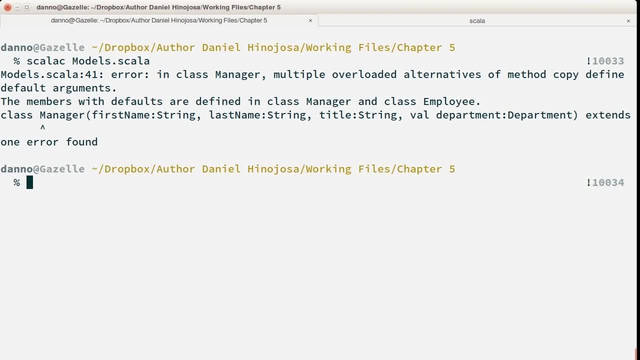 copy this one, And this one should be super class, So it will say: okay to do in Scala, except when it comes to default parameters. It shouldn't come up frequently And we also hope that the language authors, as clever as they are, to find some way to address this particular corner case. I just 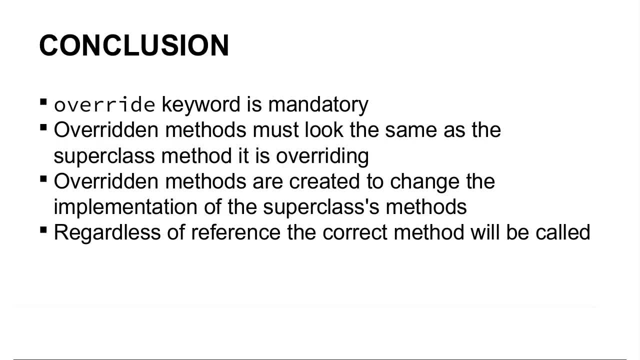 presented this as something to look out for. So, in conclusion, override keyword is mandatory in Scala And it's not an optional annotation like it is in Java. So if you are truly overriding a method, you have to use the override keyword. overwritten methods must look the same as the. 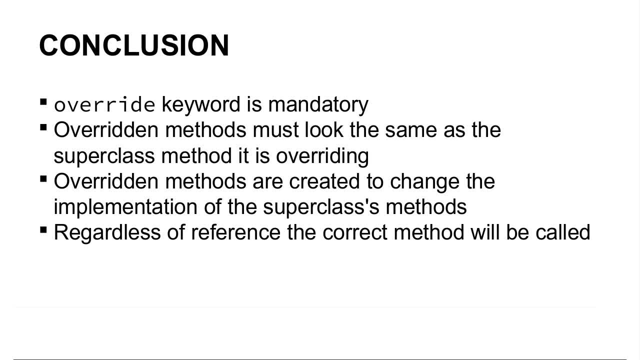 method that they are overriding from the class. Overridden methods are created to change the implementation for a subclass And, regardless of reference, the correct overridden method will be called. And again, just as an added warning, don't forget that overloading method is where the superclasses method contains default arguments. 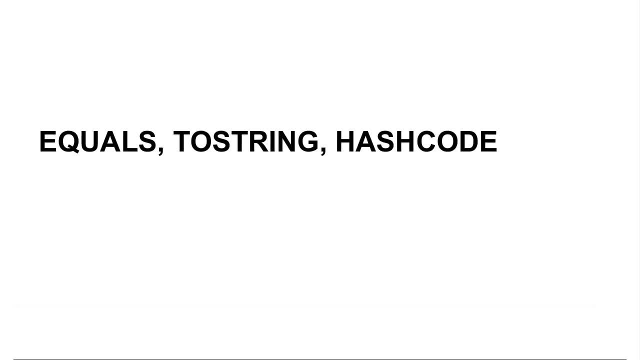 Those can cause issues. In this session we discuss equals hashcode and toString in an object. Every object-oriented language has logic to determine if two objects- or models, if you'd like to call them that are equal to one another. We must also create a number to efficiently store. 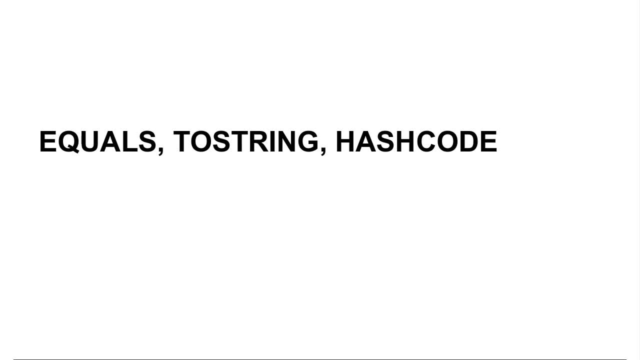 our object in certain collections like HashSet or HashMap, These are called hashcodes. We also need a string representation for our object so that it's not so cryptic when we place it on a system out. What we equate, create hashes and make string representations for is referred to as. 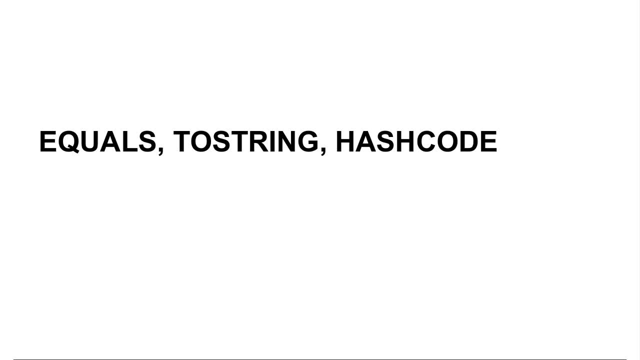 business logic in the domain models. Equals, hashcode and toString are in the AnyRef class and it is up to us to override these methods In our models to give it something with meaning. We start with equals In order to determine if. 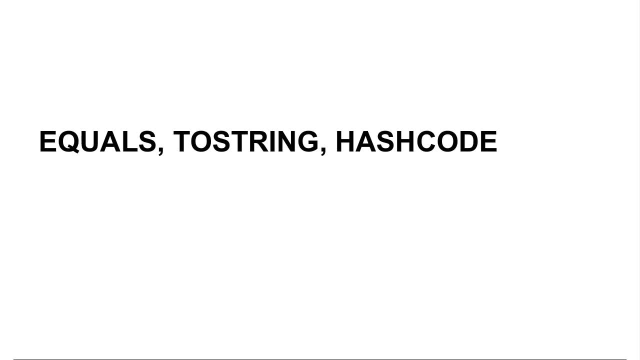 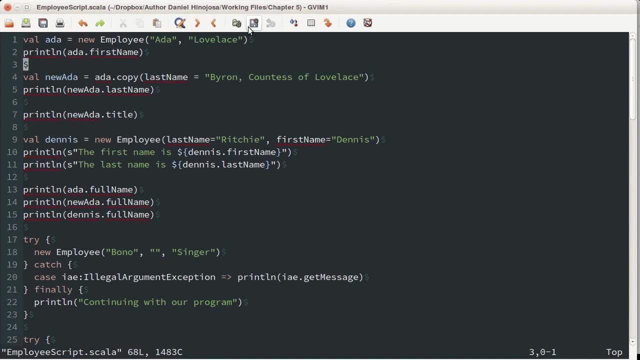 two objects are indeed equal to one another. we must override the equals method. Let's start with that First off. let's go to our employee script. We start off with Ada and new Ada. Ada has Ada Lovelace. New Ada we made a copy of by changing the last name to Byron, Countess of Lovelace. So 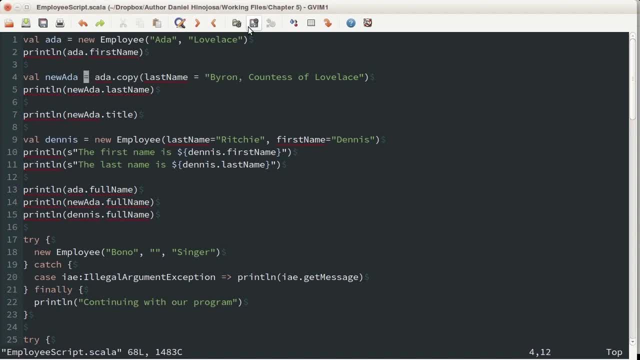 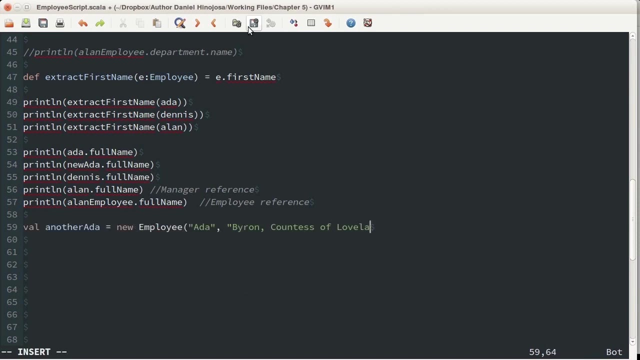 what I'd like to do is I'd like to create a reference called another Ada that is going to have a new Ada. Now remember, both of these have a title of programmer by default, So let's go down to the bottom of the file, And what I'd like to do is create another Ada. OK, so here we've created. 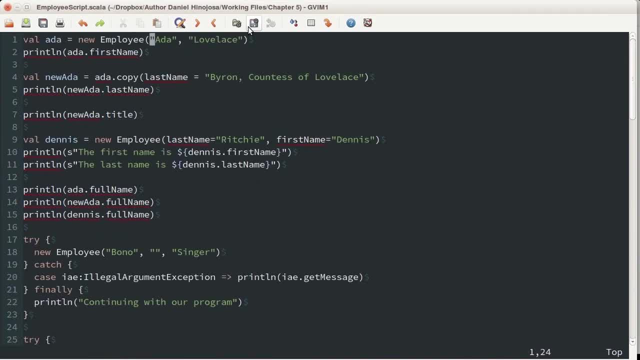 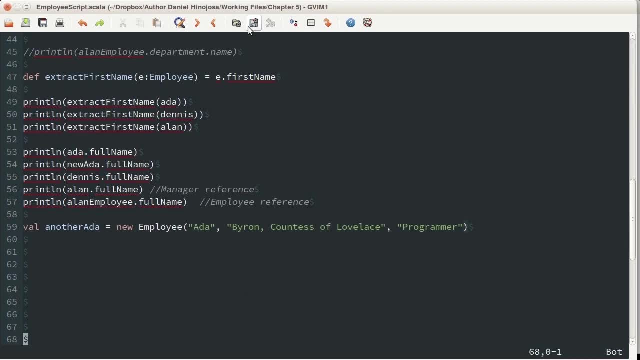 the employee. Let's go to the top to make sure that it's all correct. First name is Ada, Second part, last name is Byron, Countess of Lovelace, And finally programmer. And here it is. So we have another Ada. And now I would like to ask: is new Ada prcc granted, While other programs don't? 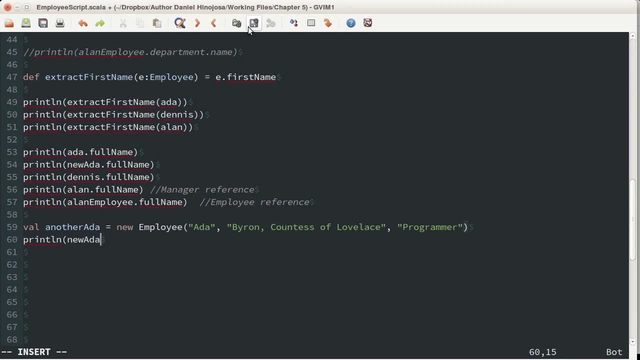 have this. we are going to create new Ada And remember you're already in the first section of this program, So let's go to the top and make sure that it's all correct. First name is Ada, Second part equivalent to another eta, given the business logic, given that the first names are equal. 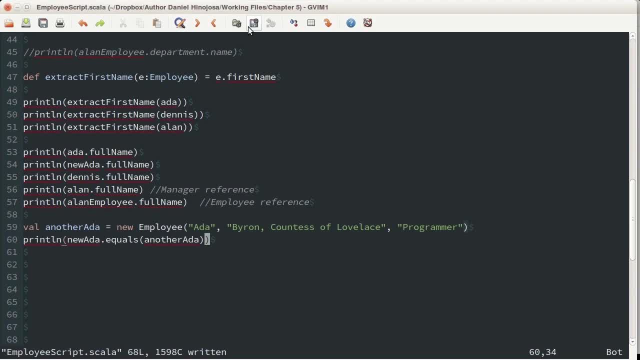 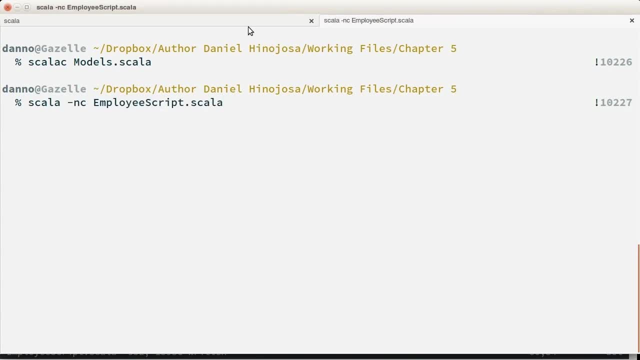 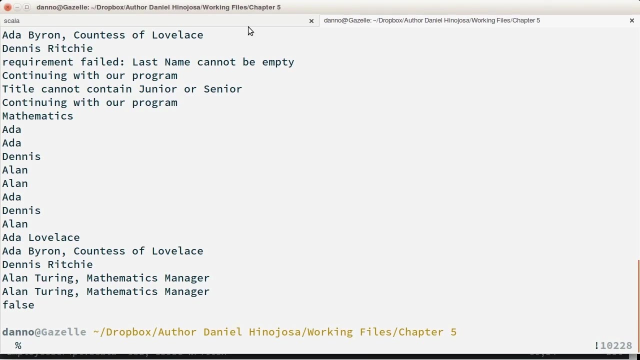 the last names are equal and the titles are equal, so let's go ahead and save this. go to our command line, compile modelsscala and run employees script. our script runs well, but at the end, right here, this says false. now the equals method that we call determines the equality of the business logic. 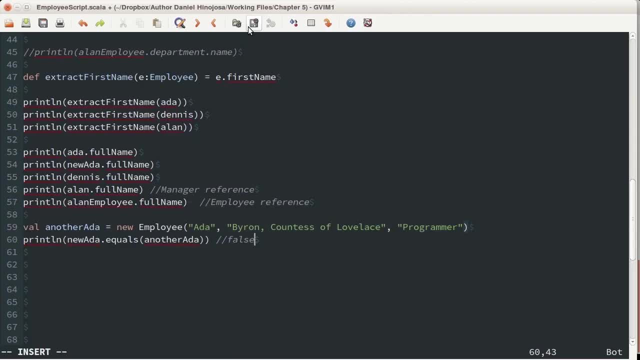 between two objects. let's go back to our code. so this rendered false. this should be true, because all the elements are the same, or we deem that it should be the same: first name, last name and title, since they're all equal. i believe, and maybe you do as well, that they should be the same, but it isn't. 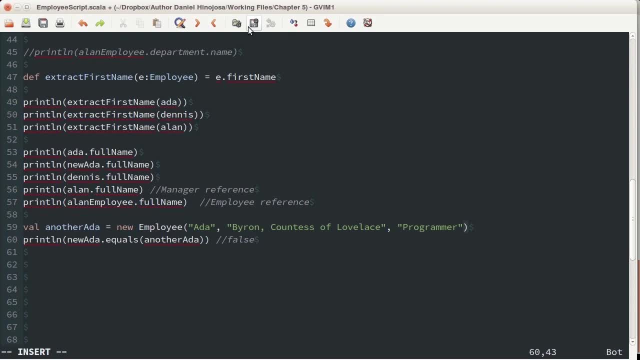 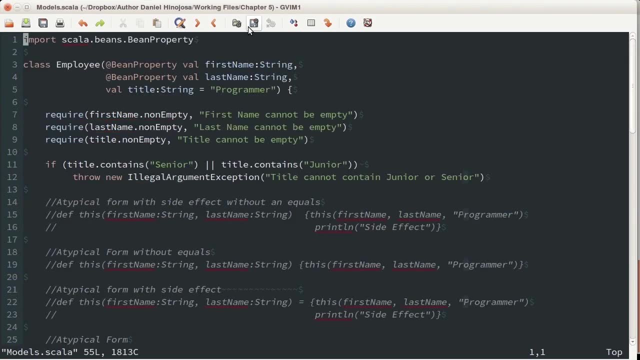 and that's because we did not program our employee class for equality. so what i like to do is go to the modelsscala file and add some equality logic to our employee class to make this work. so here we are in modelsscala and i have my employee class, and this is everything that we've. 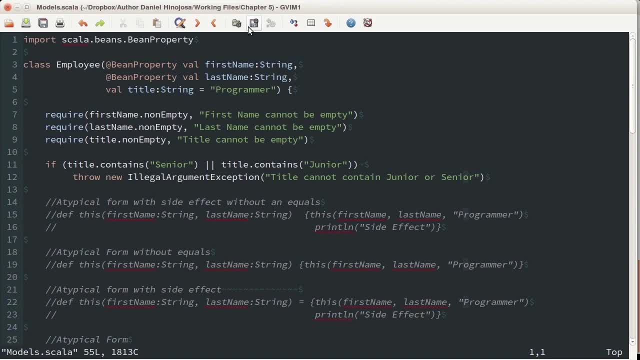 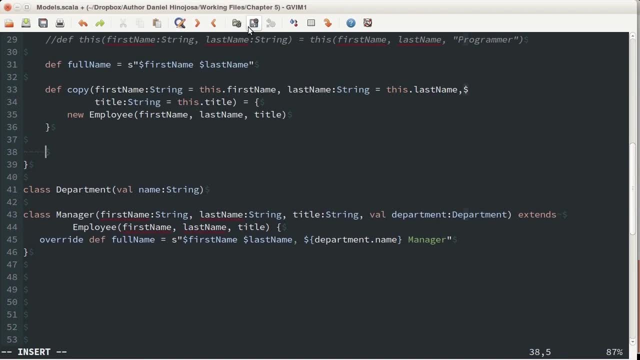 worked up to at this point, and what i'd like to do is create an equals method so that way we can make sure that equality between our adas actually works. so let's get started. i'm going to start off with the override modifier. this is a keyword, as we stated in our previous session. obviously, def- this is a method. 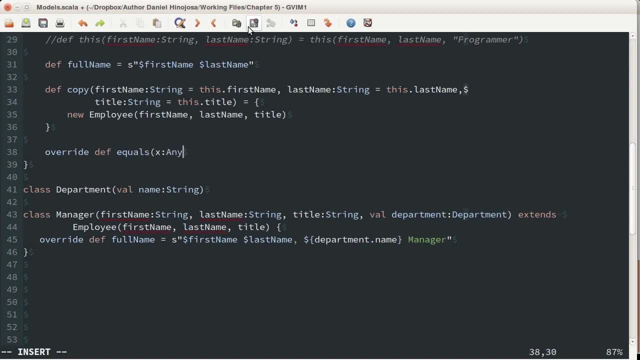 and equals. the method parameter for this will be any and the return type will be boolean, true or false. does this object equal to the other object? this x right here will be the other object that we're comparing against. now there are different ways to create implementations. i'm going to probably be a little bit verbose here. first i'm going to ask the 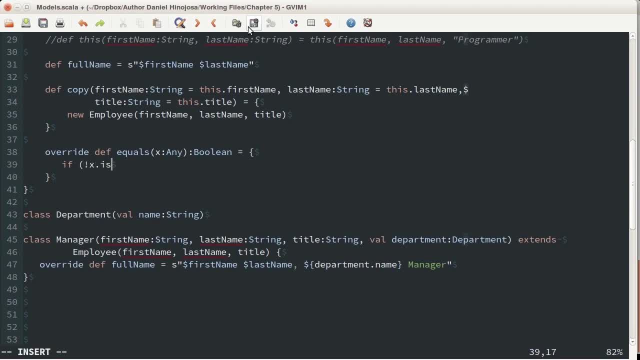 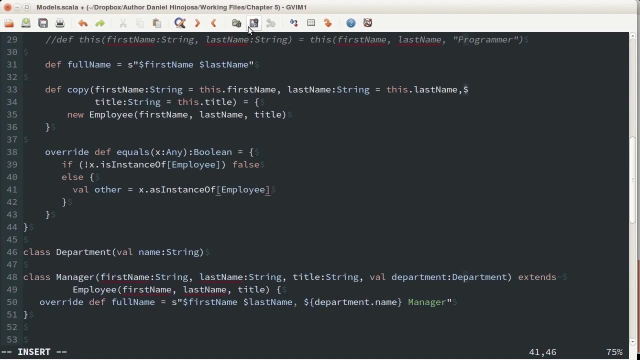 question: if x is not an instance of- we had talked about this method already- as instance of- if this does not equal to employee, then we will return false. so we have to test whether x is of a type employee. if it isn't, we'll return false, otherwise we will cast it and now other is of a. 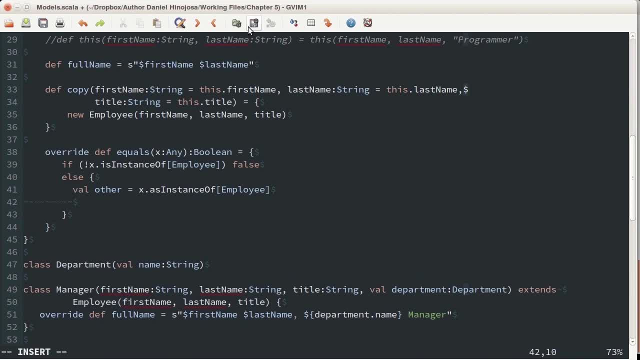 type employee. now we could ask questions like the following: is the other first name that's coming in, is that equal to our first name- and this is a boolean and we're going to be testing three different things- and is the other last name equal to this last name? and is the other title equal to? 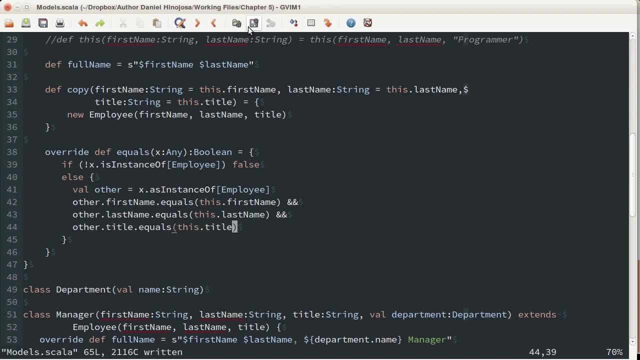 our title. this would be the last evaluated statement. this is one big statement and this is a boolean. now, since we establish this, we can then compare one object to another by calling the equals method again. this equal comes from the any ref. let's run our script. first of all, let's compile modelsscala. 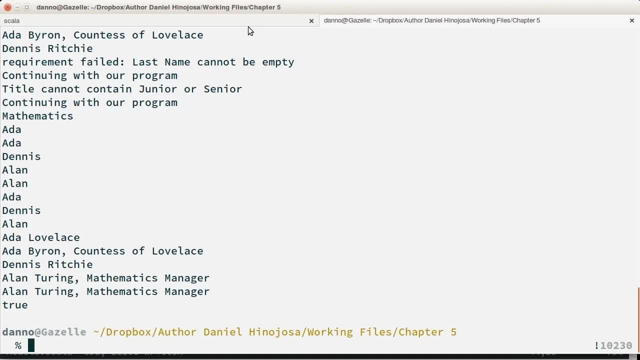 then run our script. great, take a look down here now, because ada lovelace's first name, last name and title are all equal. we deem that these two objects are equal to one another. now there's something really cool about scala. what it did is it took back the double equals operator and if 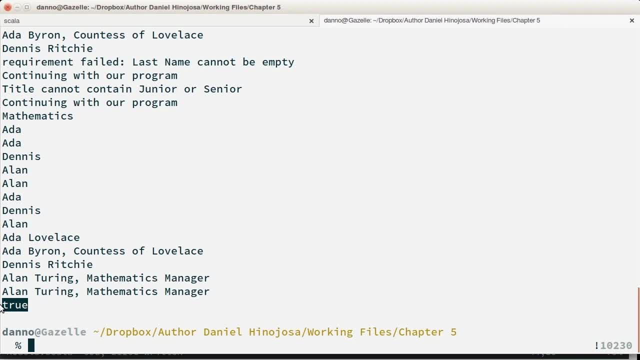 you're coming from java, you might be able to see that it took back the double equals operator. you might have a little bit of trouble breathing here. in fact, you are probably feeling a little bit confused. this means that everywhere that we used the equals, we can now use double equals, like the. 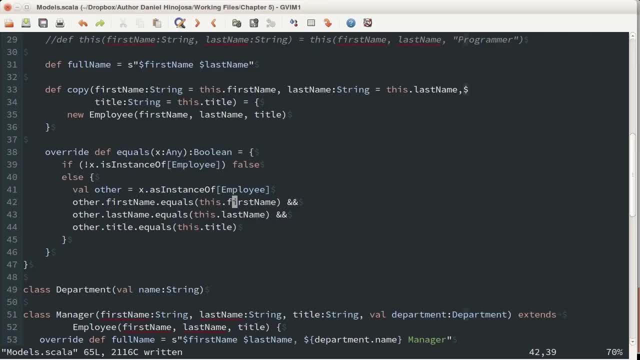 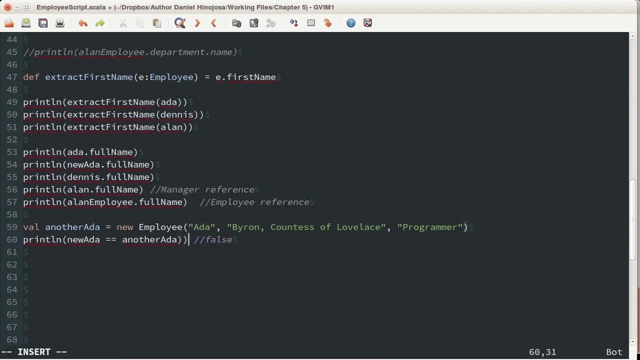 operator. so this is exciting. so let's go to our script and rewrite our equality checks, okay, so right in here we're calling the equals method, but we could forget all this and just state the following: we could also use not equals to as an operator. let's run the script again to make sure. 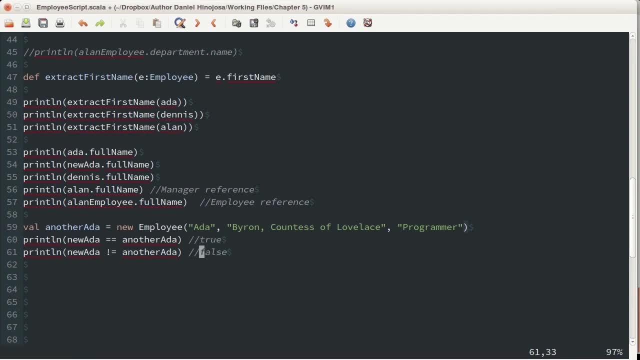 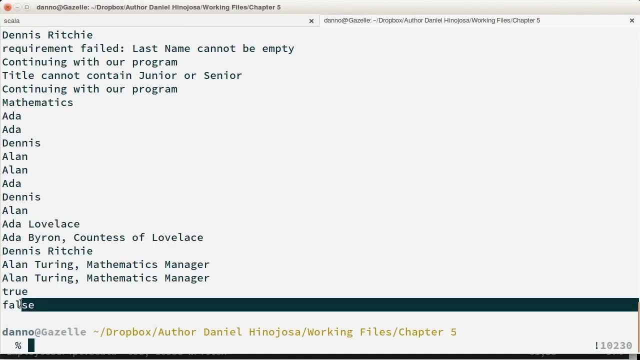 that we don't need to do anything else. now. this should say true and this one should say false, but what we're actually doing is we're actually using object equality, not reference equality here, as it is in java, this is going to be different, so i went ahead and saved this. now let's run our script again. 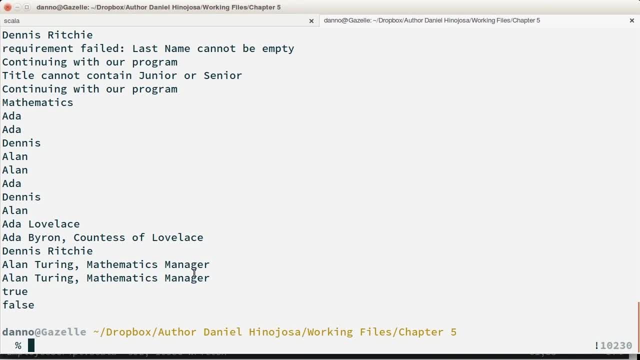 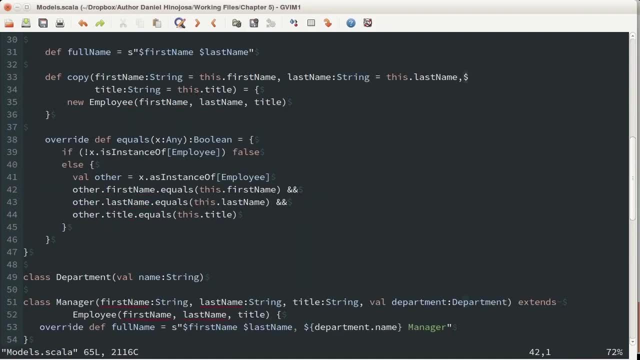 great, we see right here true and false. but wait, we could also change our code in our employee class in our modelsscala. so let's do that, okay. so here we are inside of our modelsscala and we have all these equals. so why not change these up? we no longer need that equals, we no? 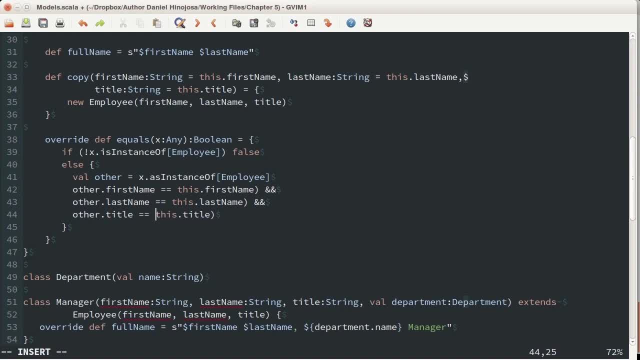 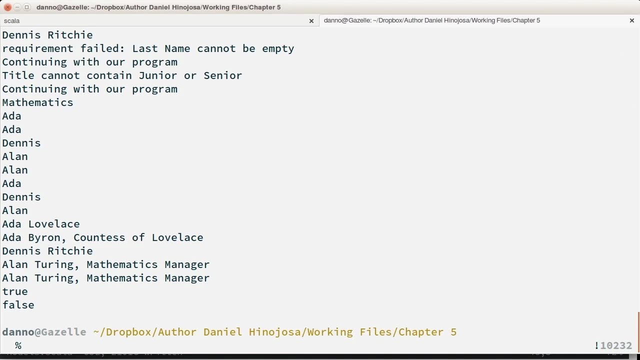 longer need this equals and we no longer need that one. you'll probably get rid of these outlying parentheses. that looks a lot cleaner. i'm going to save this. let's recompile and run our script. nice, i love you. scala, that's really great. now how do we test if two objects are pointed to the same? 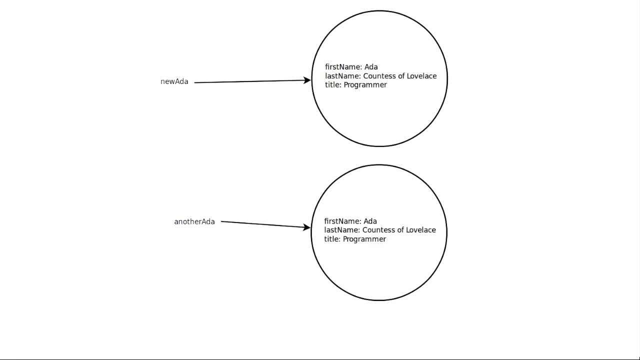 object. let's go to our employee script and see what is meant by references. so we see from this diagram that these two objects are equal. we created a new ada and we created another ada. first name, last name are the same, the title is the same, so these are actually equals, but they're not. 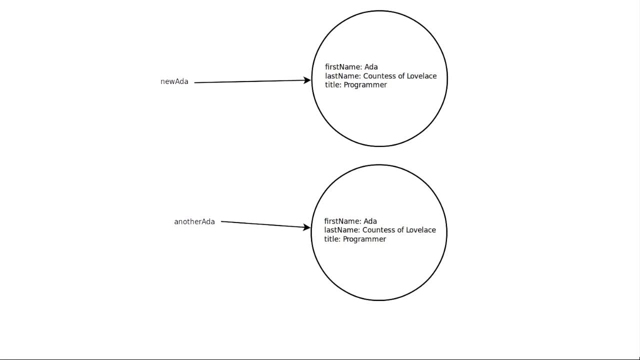 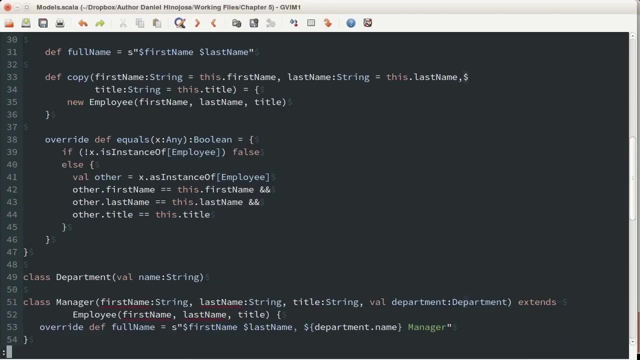 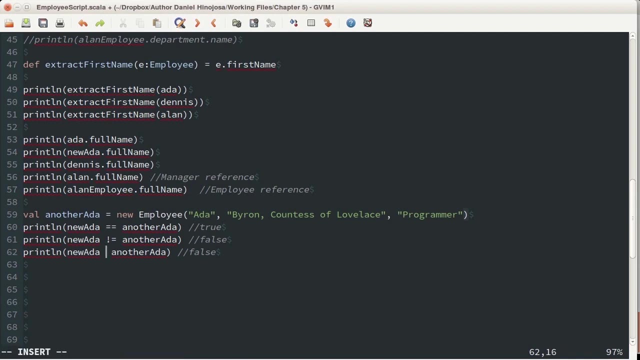 pointing to the same thing. the reason is we called it with a new keyword. in other words, we instantiated separate objects and references are going to be pointing to two different objects, so how do we test for each one of these is why we're going to use見てquipment. that means we tears away. an object and show you. so here we are, and what i'd like to do is show you how to test for equality. we're going to use method called eq. it's really an operator, not a method. this will test for reference equality. in java this used to be the double equals, but not anymore. this is now eq. this is a way we passed for references. these two are pointing actually two different objects, even though they are objects equal to one another. this should also be false. these are pointing to two different objects. so let's go ahead and'. 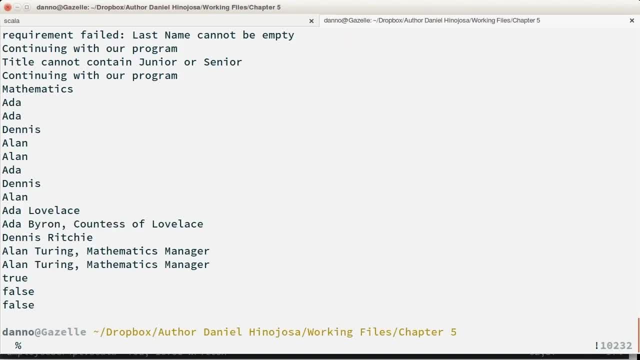 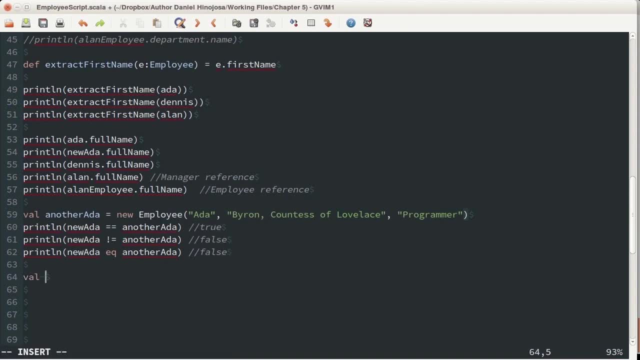 go to our command line and let's go to run our script. there it is, there's false. let's go back to our script. try something else. now we have another eta here. if we just so happen to say even another eta is equal to another eta and ask if these two are pointing to one another, 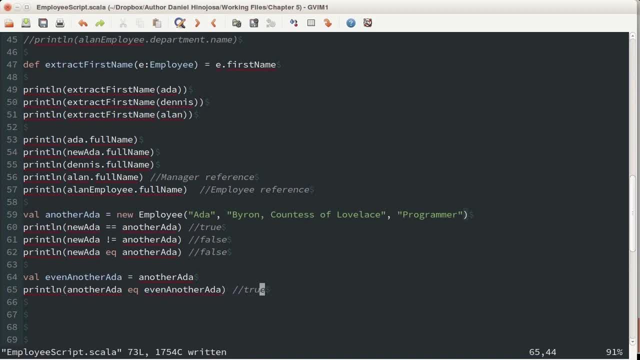 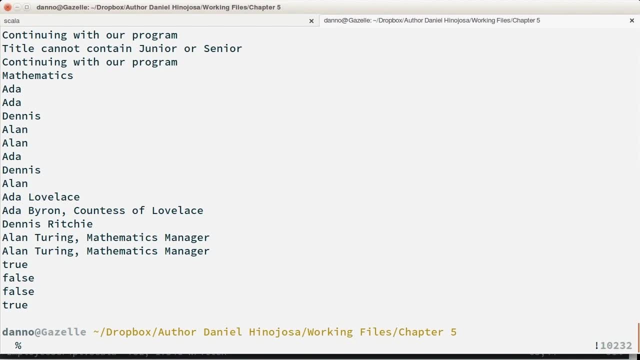 then this should be true, because we asked even another eta to point to the same object as another eta. let's save that and run the script. there we go. that is true. now let's try out our hash code. hash code is a generated number that is used to calculate where to store an object. 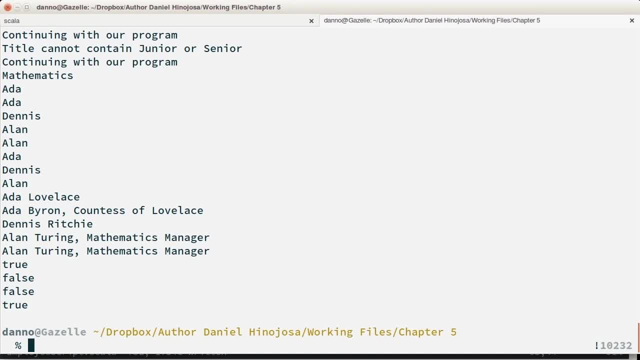 in things like hash maps and hash sets. many object-oriented languages has this notion for a hash code. hash code has to make every attempt to be as unique as possible and will need to return a 32-bit integer to identify that object. it's kind of like an employee number or social. 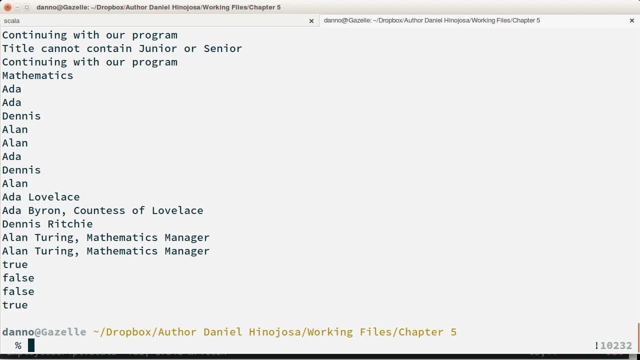 security number, some kind of number that identifies the object. i'll use josh block's recipe for hash codes from his book effective java, second edition. so we move on to the next step. we're going to need to do is we're going to need to do a. 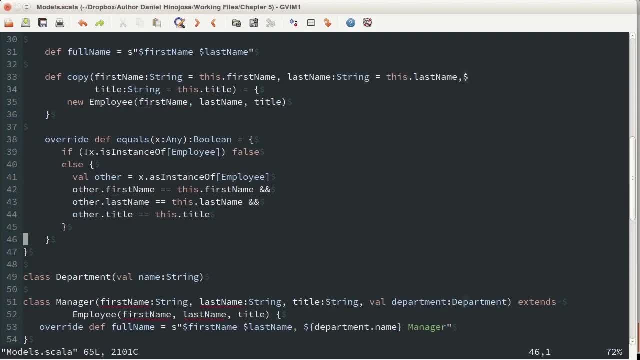 hash code. we're going to move over to modelsscala and add a hash code. okay, so we just got done with equals, so now let's create a hash code. this is an override def hash code. this will return an int. what we'll be doing? we'll be setting up a var here, even though using a var can be a little bit. 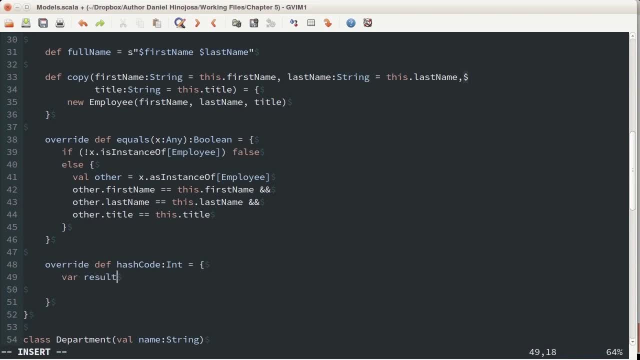 dangerous and over here it's going to be just fine. we're going to choose a constant, non-zero value and assign this to a result, and what we're going to do is we're going to change the result. we're going to take the prime number, multiply it by the result and add first name's hash code to it. take: 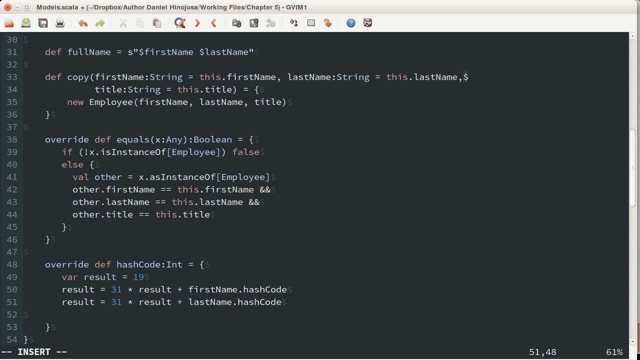 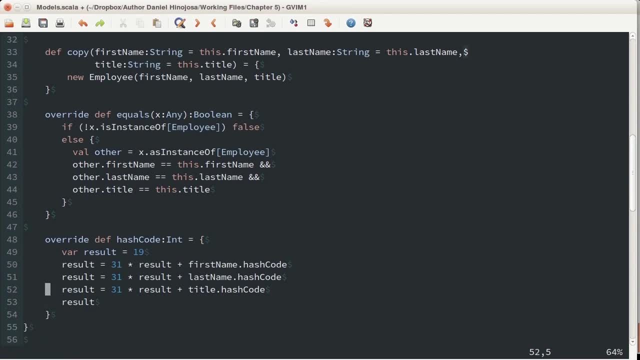 that same prime and we'll add last name's hash code to it. we'll take the title multiplied by 31 and then finally return the result. here's our hash code. now, once we return this number, it's no longer mutable. it was only mutable within the context of a method and that's why the var in this. 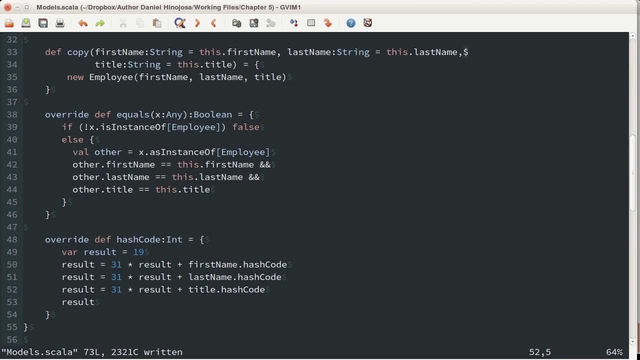 case is okay, not leaked outside, nowhere outside this particular reference, and we're going to need to put a solution here to作. Glenn, we don't have a2 key, we just want to take out the initial by the bothль alder. so what we're going to do here is we're going to take a new variable and let it. 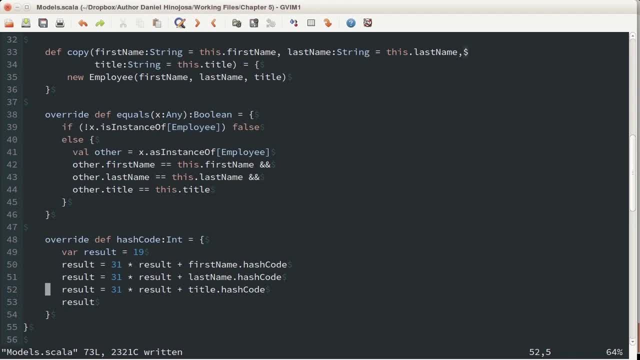 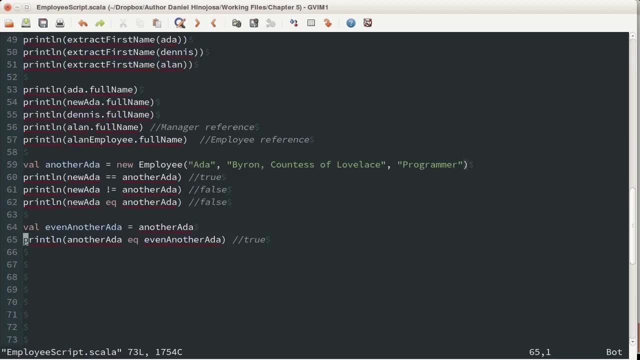 go to underscore the hash code, paste the new event and we're going to add it to our véritable hash code: tipセ squ пока, cplease test. in this example we're going to have a new, that is a field. there's going to be auarialять kind of a string. so here what we're doing is we're going to export it and with that. we're going to pick an int initial and let's have thatakhast ASMR. it's going to come to right's and we're going to nuet up and this will be one of the parameters. now, when flaws can, a second option and from here we could use and select, or with a way that it's what's元 the hard feature. 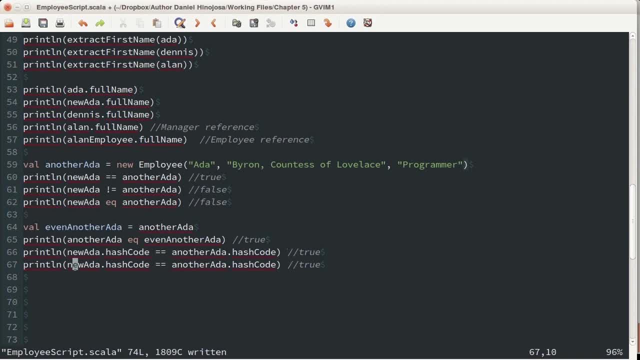 previously. we're going to so so that we had this one of the season test. let's use Ada, for example. Ada, remember, had a different last name, so this should also be true that Ada's hash code- remember she has a different last name- the Ada reference does and another Ada should have a different hash code. so 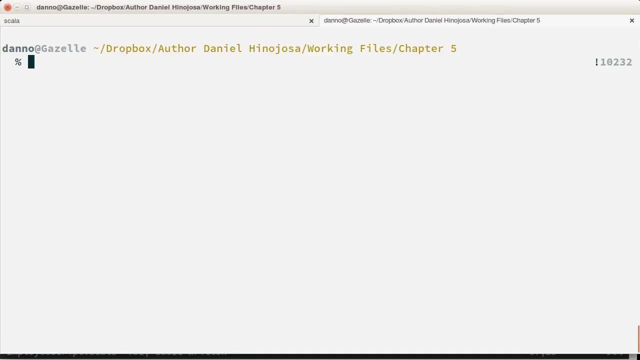 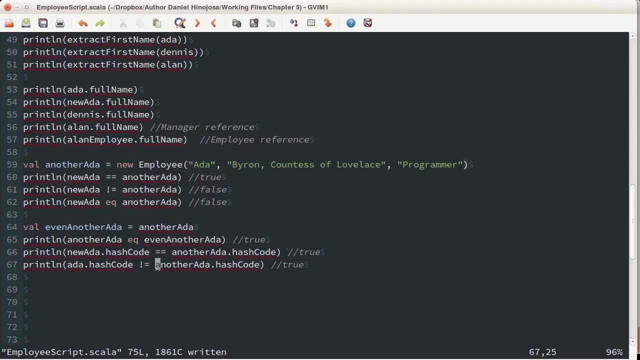 these two should not be equals. let's save this, compile our models, Scala, then run our script, so we have true and true. let's go back to our code. as the last two true and true, the hash codes work now because we have an effective hash code, we can then use our employee objects in collections like hash map and. 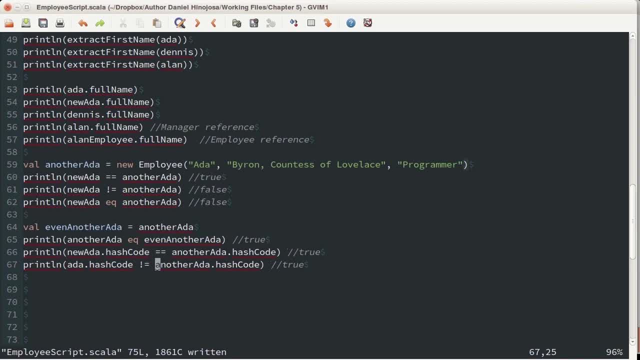 hash set. so, lastly, let's work up our to string and as it stands right now, if we print out any employee object, we get some sort of messy output. let's try it out first. so we're already here in our employee script, so let's add the. 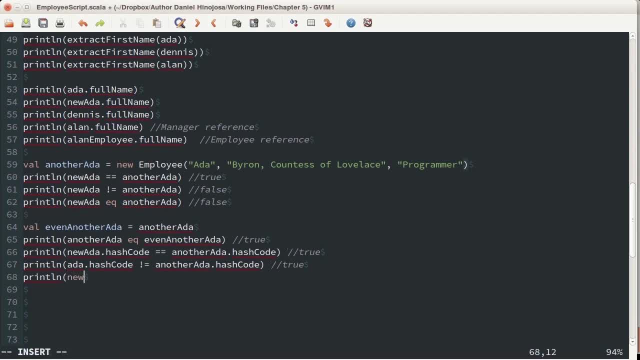 following line. in fact, I'm gonna do a print line, new Ada to string. but we don't actually need the to string right here, so I'm just gonna call new Ada. why? the default implementation for print line is that it's always going to call to string regardless. I could be explicit about it by adding to string if: 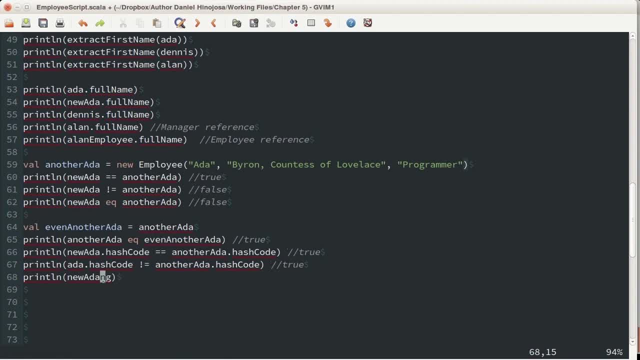 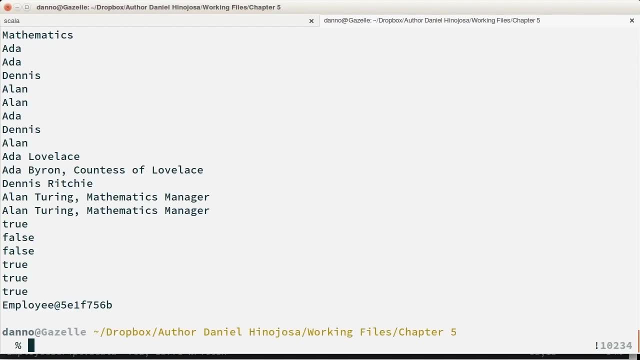 I wanted to, but I really don't need to, so I'm gonna go ahead and remove that. now let's run our script to see the result. so we see employee at 5e, 1f, 756 B- some sort of messy output. this shows the name of the class as well as an integer. 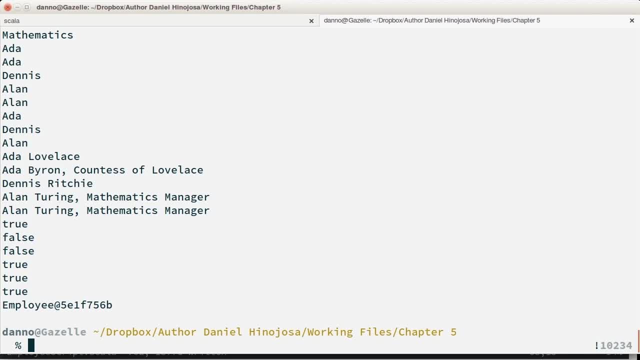 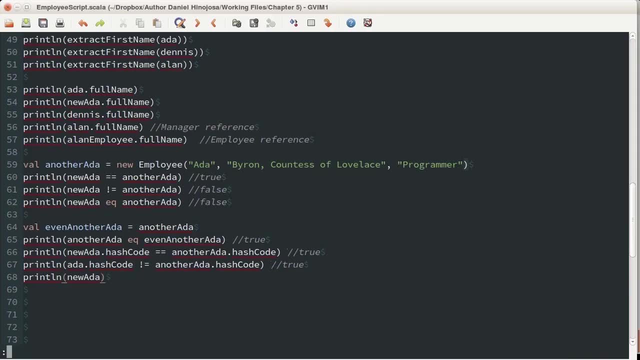 representation, really a hexadecimal type of representation of the object address. not very helpful. so let's create a to string method for our employee. so let's go back to models dot Scala. we're gonna do an override def to string and we'll use string interpolation for this. you. 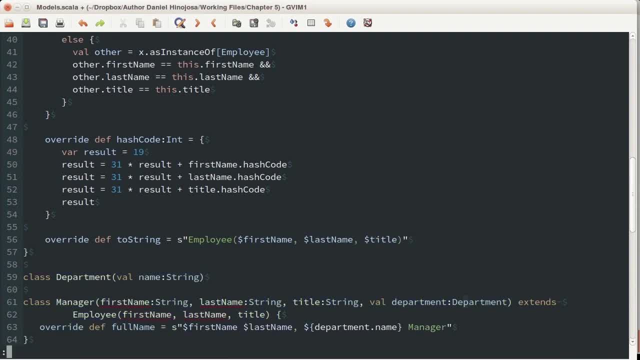 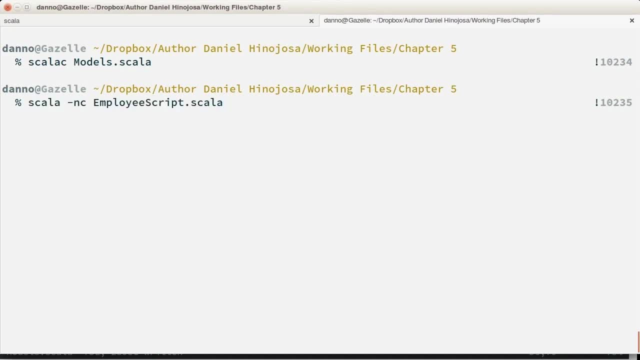 could do whatever you want here. whatever kind of string you wish to represent your object, you can do so here. it is all up to you. now let's compile models, let's run our script. keep in mind, I didn't change anything with scripts, so what should appear is the actual representation. 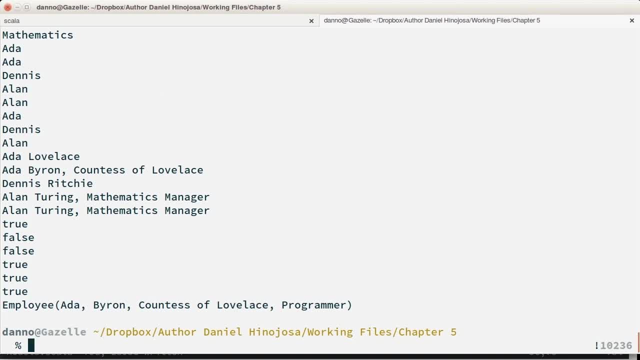 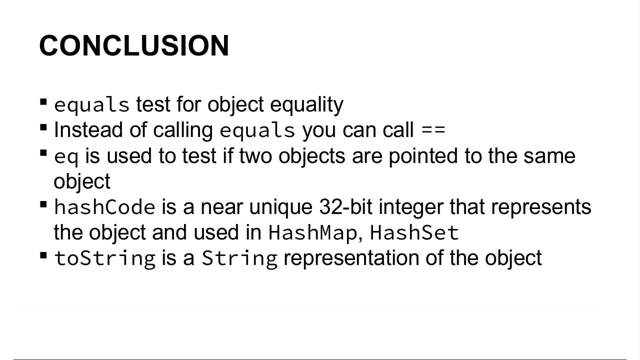 that we defined. now this is human readable employee Ada Byron countess of lovelace programmer. a nice string representation for our object. so equals tests for object equality and we would need to override this equals method. but when we call it, we don't have to call it with equals, we can call it with the. 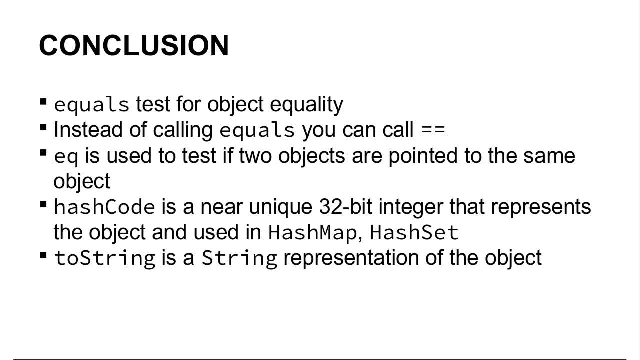 double equal operator. we can use EQ to test if two objects are pointed to the same object or if they're sharing the same reference. hash code is a near unique- and I do say near unique, unique. sometimes collisions will happen, but you should try your best and should return a near. 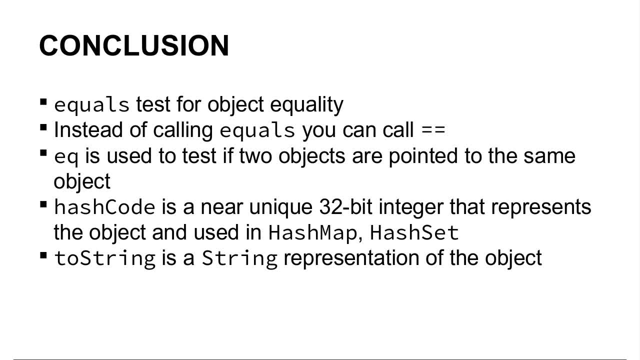 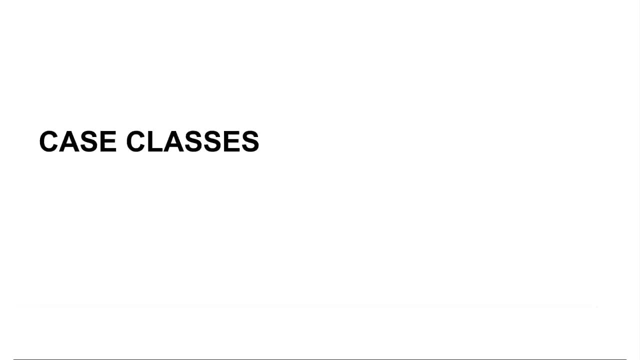 unique 32-bit integer that represents the object so that we can use in things like hash map and hash set, and two string is a string representation of the object and- just an added note- equals two. string and hash code are all overridden from any ref. in this session we discuss case classes up to 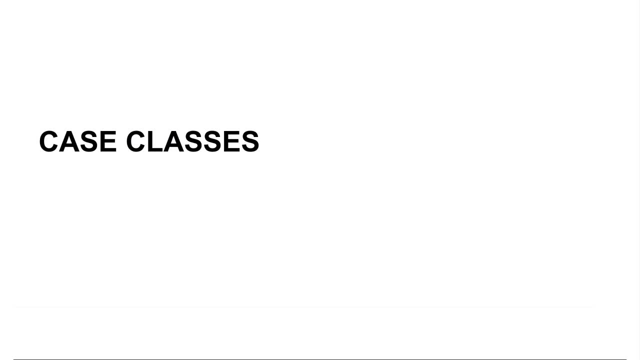 this point. we've been pretty hard on you, since we manually coded methods like copy two string hash code and equals case classes will do all of that for us. all we have to do is add the word case before the class keyword and we can forget all about that. equals hash code- two string mumbo. 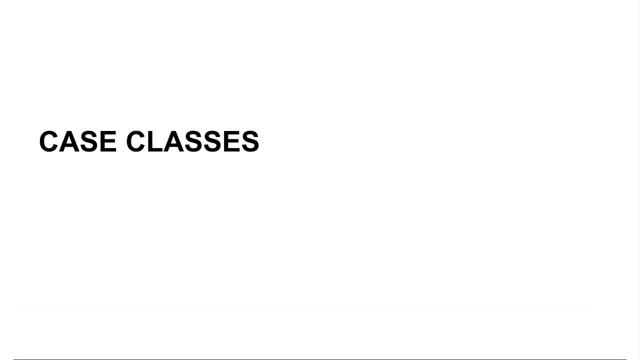 jumbo, since all of that will be created for us automatically. I will say: there will be some caveats to that, though, but we'll discuss that at the end of the session. but first let's try out our case class with department in our models dot Scala file. so let's head over there. 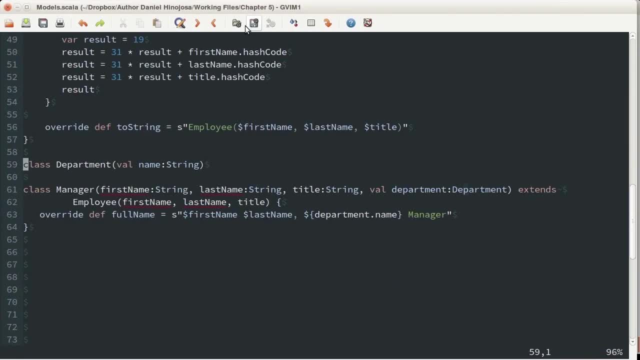 now, alright, so here is models dot, Scala, and what I'm going to pick on is I'm going to pick on department just because it's easier. we have department has one property name, so let's go to our script and we'll check to see that we indeed have a copy to string hash code and 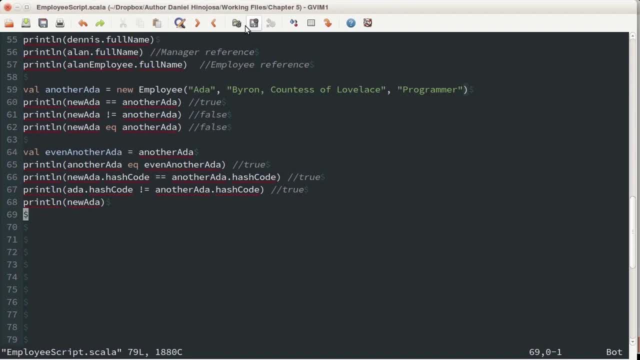 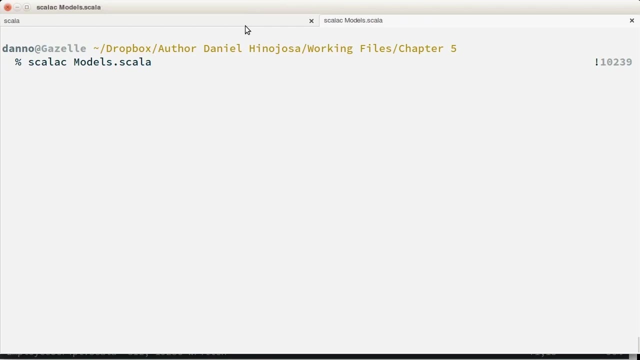 equals method. so here we are in the script. so what I'd like to do is give this a try. I'm going to create a toy department first. let's try out to string print line toys. now let's go to our command line. give this a try. so I'd like to compile models, dot Scala, first, since we made a 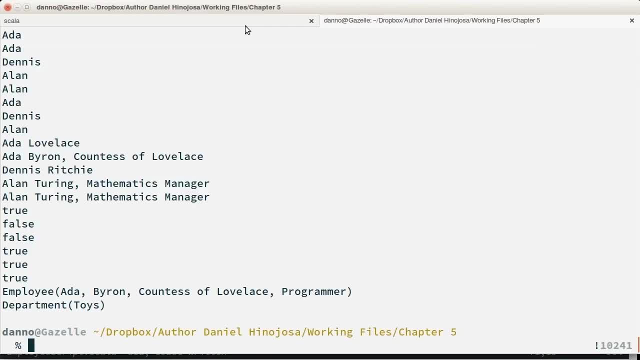 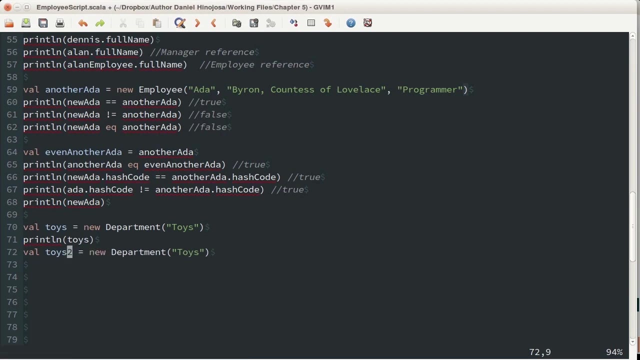 change to department. and now let's run our script. now, as we see right here, here is department, so it indeed created for us a to string implementation automatically for us. next let's try equals. let's go back to our code. so, given this, I'm going to create another reference, called toys, to this is: 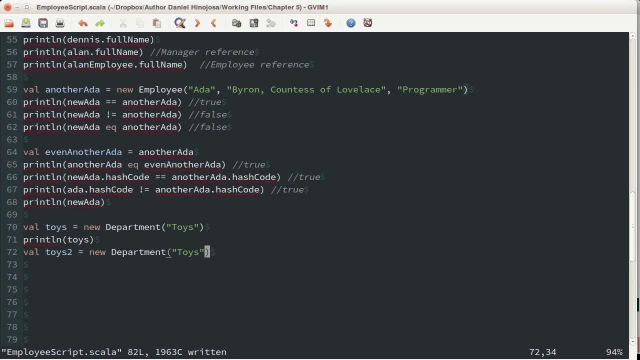 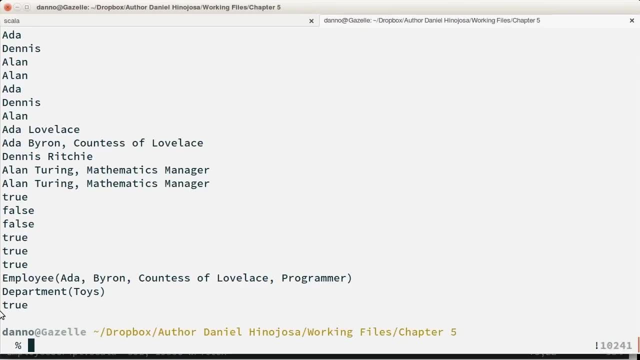 a different object called department toys- same thing, and we would like to make sure that we're going to save this to our code. so let's save this and run it right now. let's try to do this. let's save this and run it. that is true, really good. so now let's try hash code. remember that. 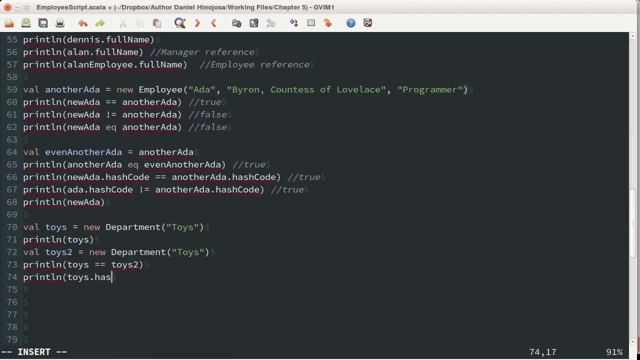 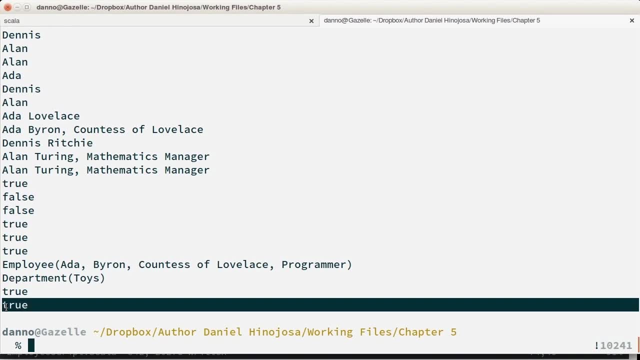 checking. two hash codes of two equal objects should be equal themselves. so let's verify that. so toys dot hash code should equal to toys to dot hash code. let's run that. so you see, right here, that is true as well. now let's try the copy method. the copy method is going to work the same way as. 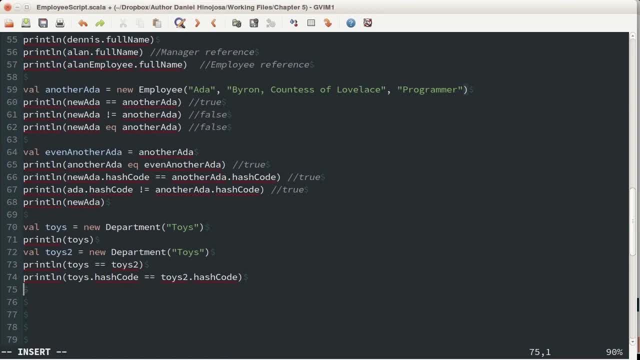 manually earlier, a few sessions ago. So let's go back to our code and give that a try. So this time I'd like to create hardware and we're going to take toys and make a copy of that, But in our copy 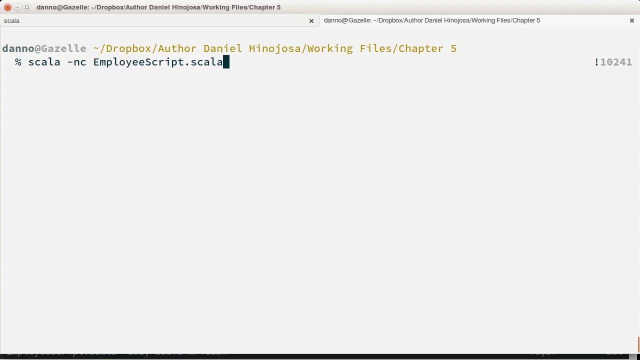 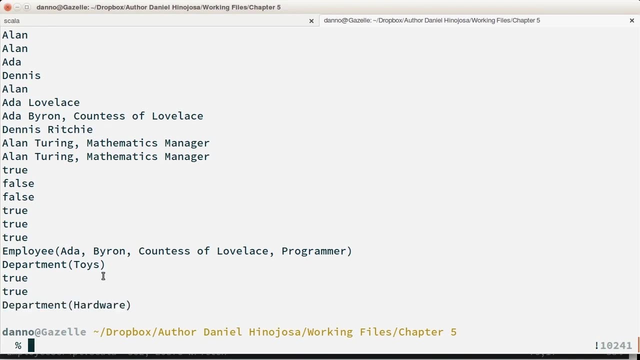 let's change the name to hardware. Let's go run our script. There we go, Department hardware. So we have two string equals hash code implementations. We have a copy method, case classes for the win. There are some other neat effects that case classes can give us. For one, we don't have to use the new. 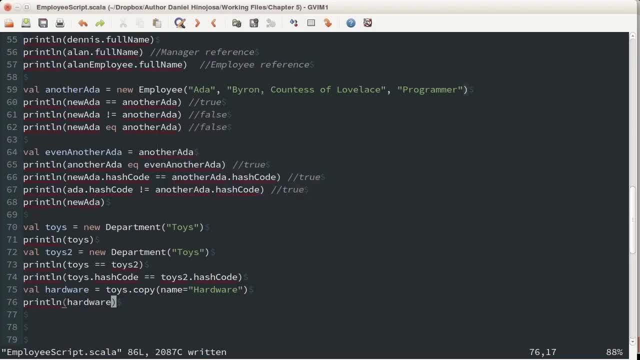 keyword anymore to create an object. Let's go to our employee script and try that out. So this new keyword: get rid of it. This new keyword: get rid of it. Let's save it and let's give it a try. 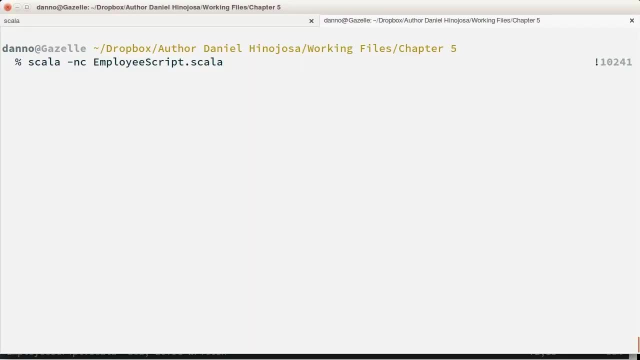 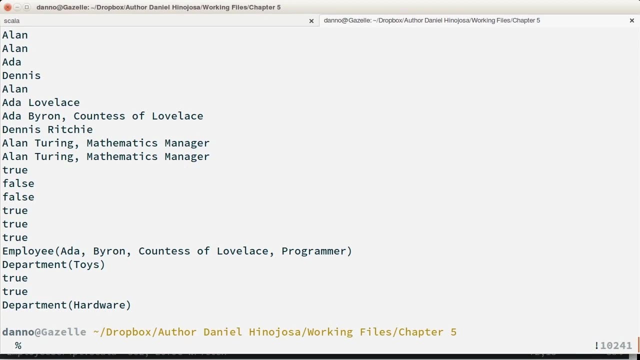 Remember: this only works for case classes. If there isn't a case in front of it, this will not work. Script works just the same Again, because we put a case in front of the class. the new is optional. One of the other neat things about case classes is that we don't need to declare. 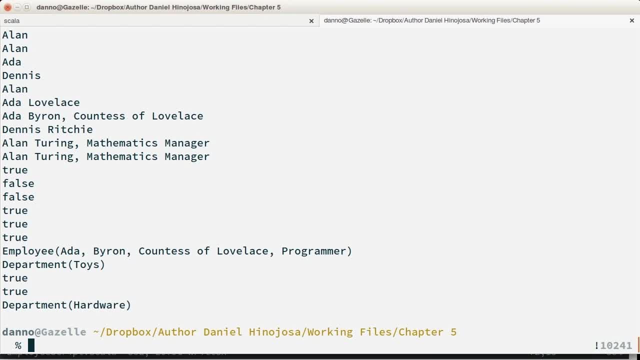 vowels in our primary constructor, since it's a case. So we don't need to declare vowels in our primary constructor. It's now assumed by default. So let's change the way our department looks by taking out the vowel for the name and to do so, go to the modelsscala Again. we no longer need. 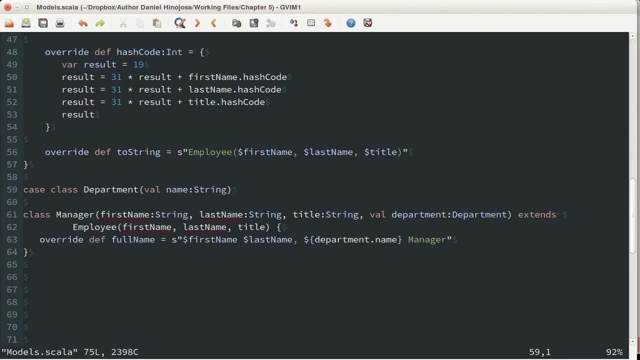 it if we're using a case class. So here we are under modelsscala, case class department, and we have vowel right in here. Do we need it? No, So I'm going to get rid of it, Save it, and now let's. 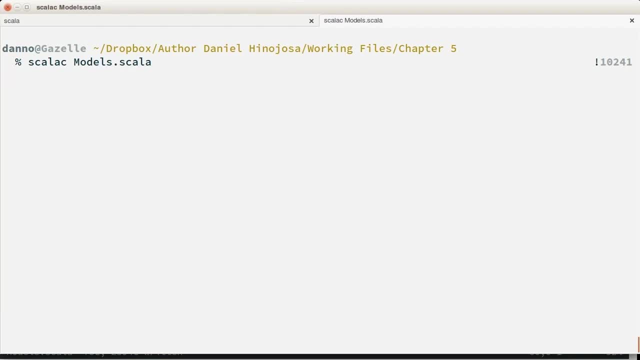 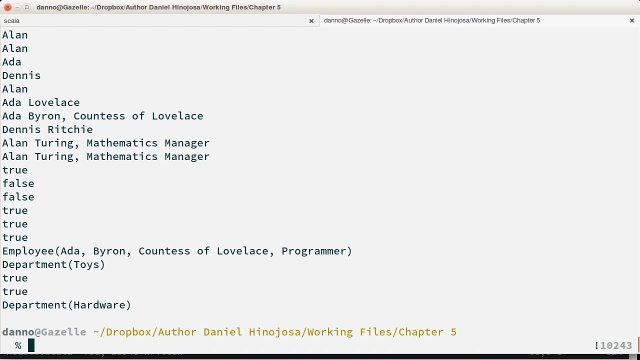 check that everything still works. First we compile modelsscala, since we made a change, and now we will run our script Again. everything works as expected Now, just so you know. if you don't like what is provided for you automatically, you could always override your own method while maintaining the other methods. 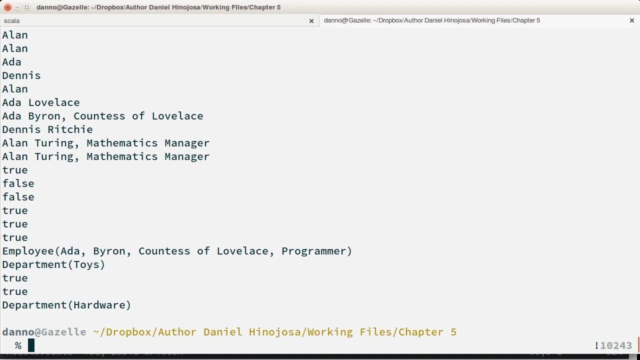 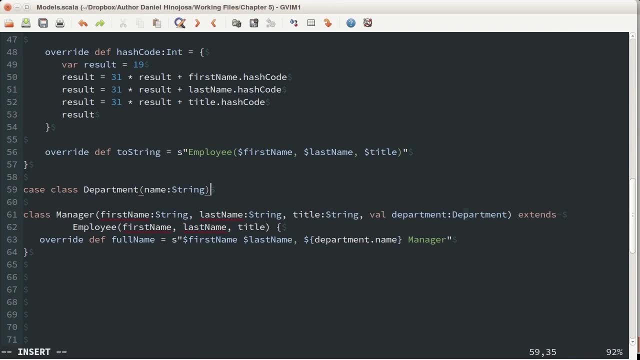 created automatically. So for this, let's say we want to create our own toString with department, while keeping equals and hash code, and copy the same. So let's go back to our models and what I'd like to do is override only toString Again, keeping the rest the same. So let's say 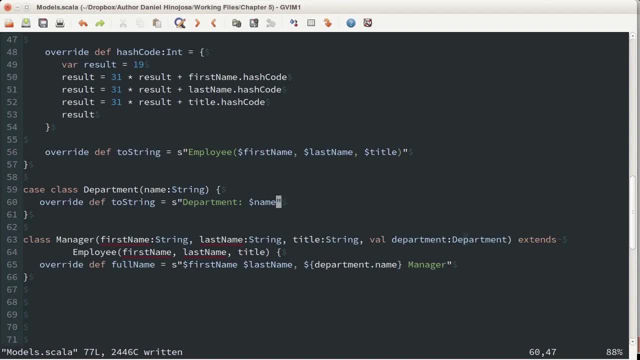 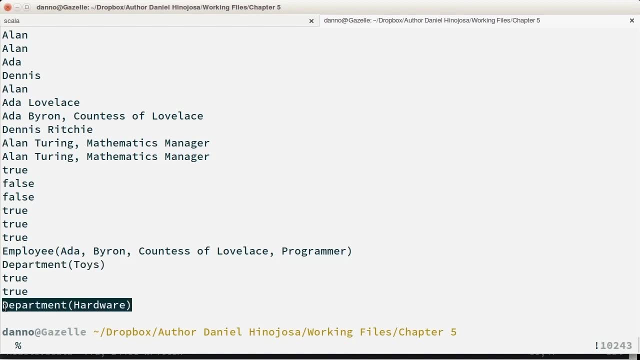 I don't like the way it looks by default. Let's go back to the command line just to show you how this displayed. So here's department toys and here's department hardware. That's what it looks like by default. States a class name parens and lists out all the properties for that one. 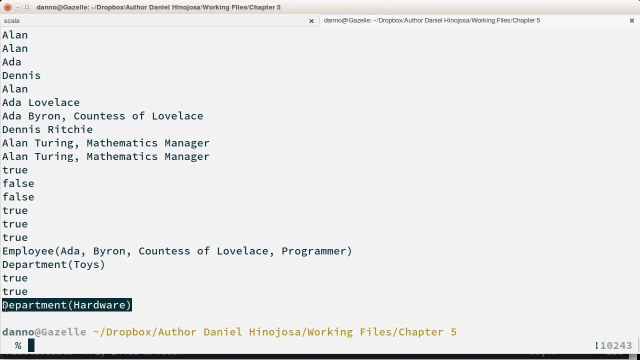 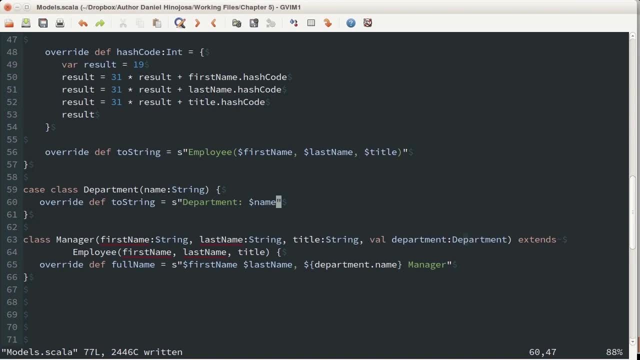 particular object. So what I'd like to do is just change the way this looks, Go back to our code. So I'd like for it to say now, department, colon space and then the name of the department. So I'll go ahead and save this And let's go back to our code. So I'm going to go ahead and save this And let's. 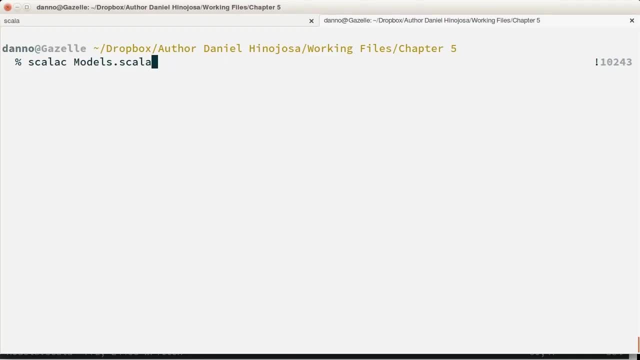 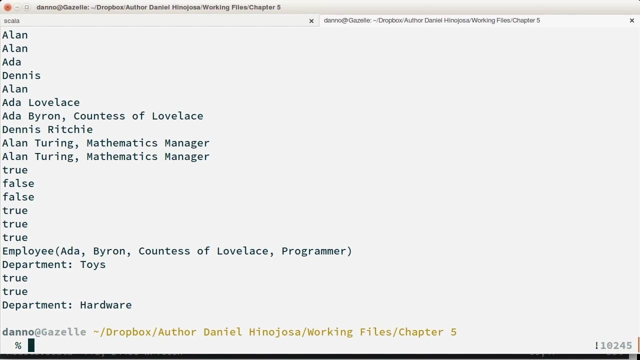 to the command line to see the effects of this. first let's compile models, dot, Scala. then let's run our script. everything's the same from our previous run, except the way we do a to string. so all the equals, all the hash code, everything else still stays the same. now case classes also. 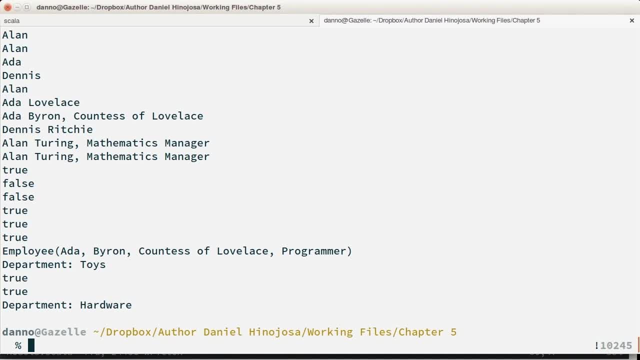 gives us the ability to unapply code for pattern matching, though pattern matching requires its own set of topics- topics that, unfortunately, we don't cover in this video series. but let's take a quick example of what pattern matching looks like. let's go to our employee script. let's say we want to. 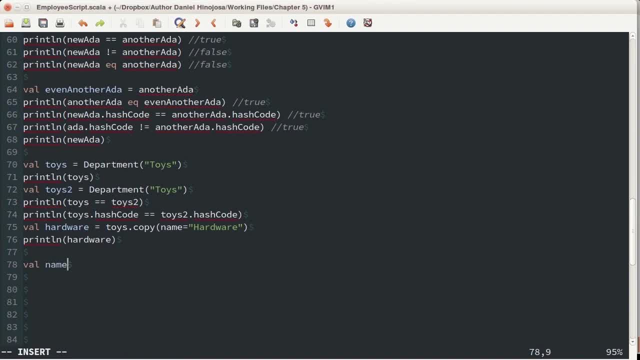 extract the name from one of these particular departments. I will choose toys for this example and I wish to match on this. this is a way we do pattern matching. pattern matching is very much like switch statements and other languages, simply a little bit more robust. we can do a lot more with. 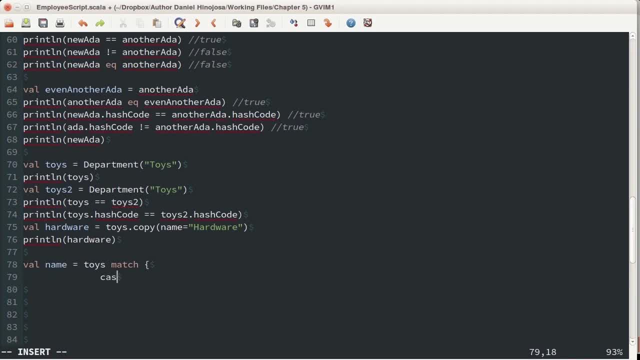 pattern matching. the way pattern matching works is: we're gonna put a case here. in this context, case means in case. this is a department and here I'm going to assign a variable. so whatever name is a part of this department, I'm going to assign this to n and if it just so happens to match this type, I wish to 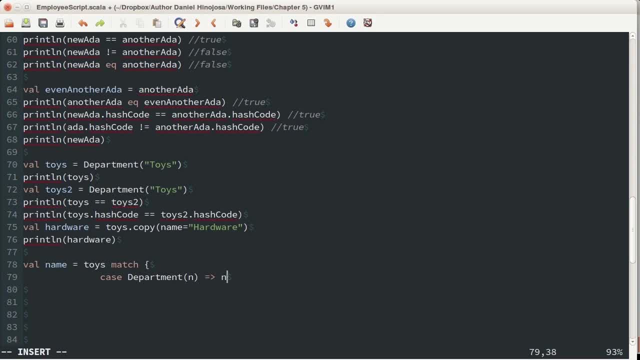 return that n that particular name. secondary case: this underscore means what default means in other switch statements in other languages. this is pattern matching, not switch statements. but the underscore here is the default, and if it is not known then we will return unknown. and then, finally, I'll close out the brace and in this case, here, what I'd like to do is just print out. 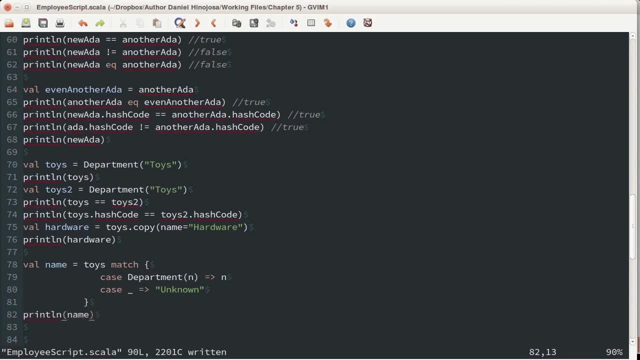 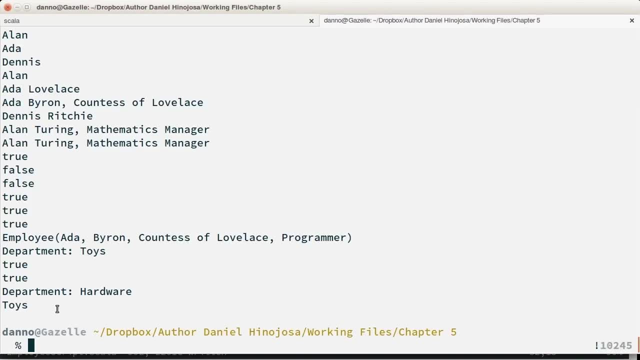 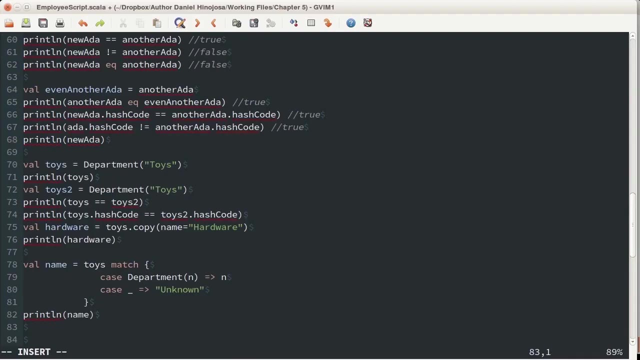 the name. I get all this automatically by using a case class, so let me go ahead and save this and let me go over to the command line and give this a try. great, there it is- toys. in fact, since we have that, we probably did too much work. we could also simplify it very much like this. let's go back to 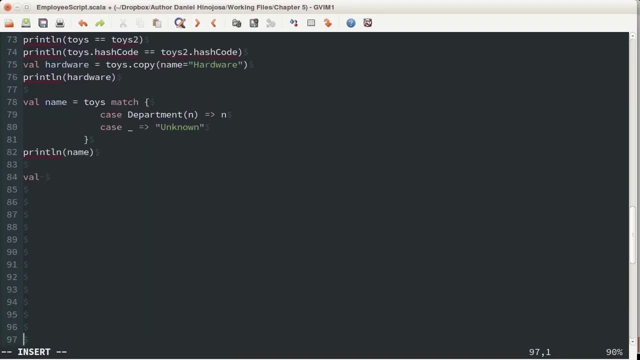 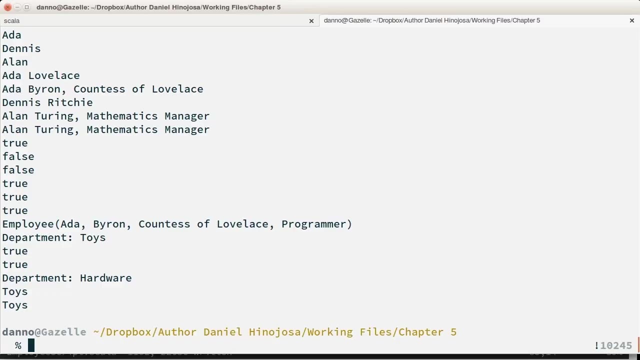 our script. it's at a few lines here, so that way it's not stuck down at the bottom. this is really what we're doing is we are extracting the name from toys and name two is going to be assigned to the name of the department. so let's save that and let's give this a run. there it is again. let's. 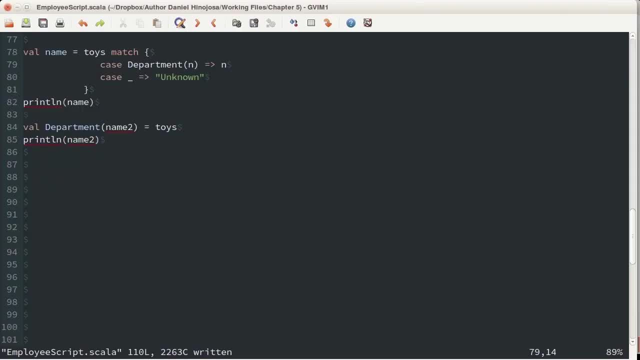 go back to our code: one line instead of four. this is the power of pattern matching. again, you get all this by using a case class. now, a lot of these neat tricks are tucked away in a construct called an object, and we'll discuss that in the next few chapters. so now let's talk about the caveats. I 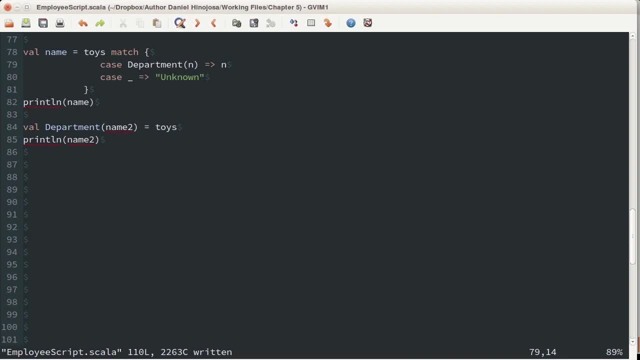 was referring to earlier. although case classes are wonderful, I'm going to do one more thing in this section. here is that cost case classes cannot be subclassed by other case classes. one of the reasons happens to be one we encountered when we created our own copy method: we cannot inherit from a method with default parameters. the other reason is back a. 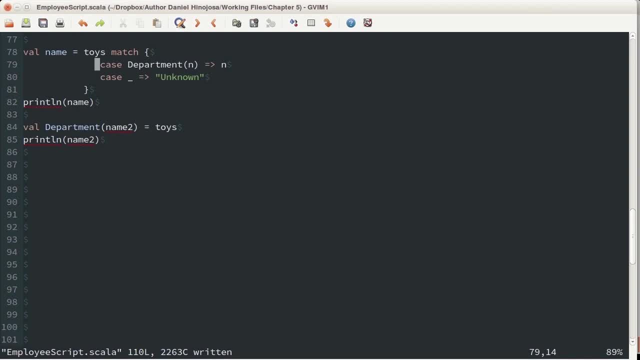 few years ago, when copy was being implemented, creating a copy method on a sub class returned an instance of the super class. of course that was incorrect. that was really tough to implement at the time. so there is that limitation. just be aware of this. sometimes you case class. sometimes there's no way around that and you're going to have to create your own two. 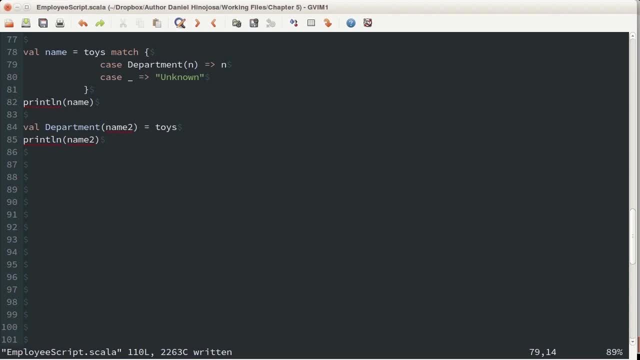 string equals hash code and copy methods. As far as pattern matching, you can create your own on apply. As far as invoking or creating an instance without the new keyword, you could also do that manually and we'll be discussing that in the next few chapters. But take heart, most scholar. 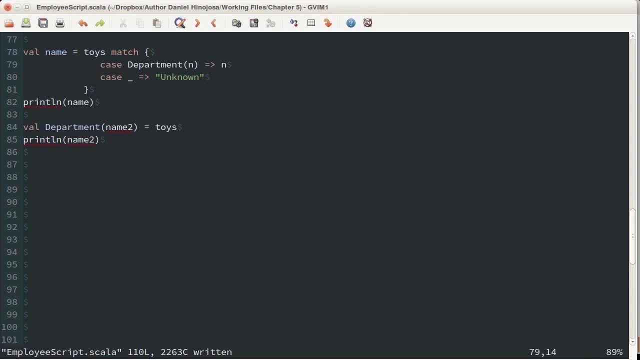 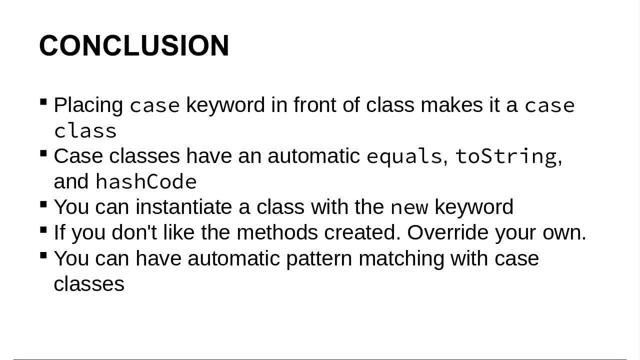 programmers will typically model a superclass as a regular class or abstract class, while the case classes will be the subtypes, and that you can do So. in conclusion, putting the case keyword in front of a class makes it a case class. Case classes have an automatic equals hash code two. 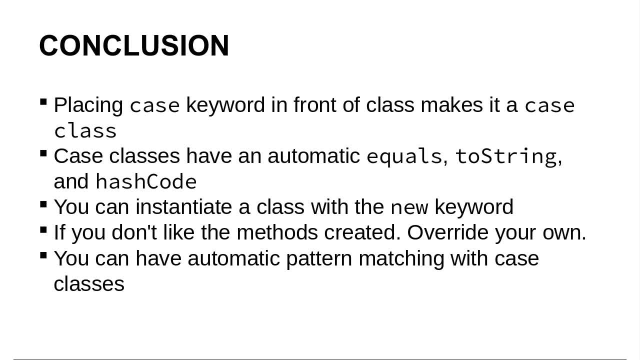 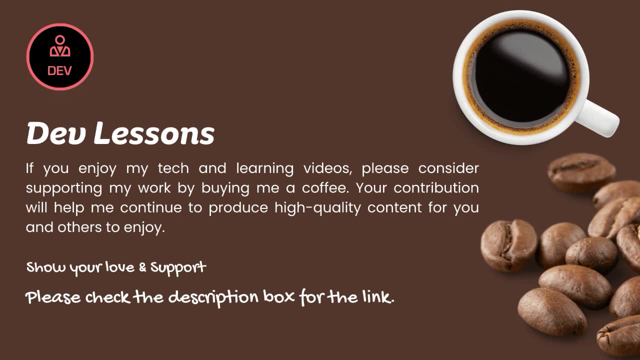 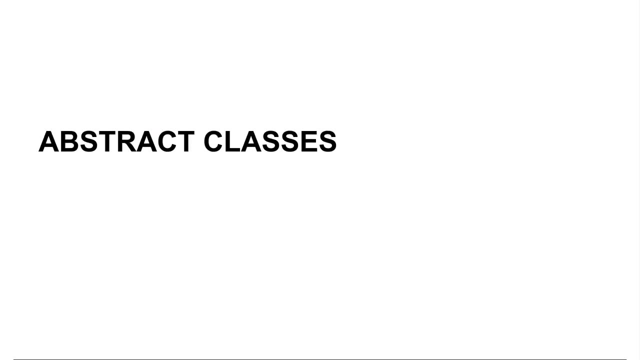 string. You can instantiate a class with a new keyword. If you don't like the methods that are created, you could override your own and you can have automatic pattern matching with case classes. In this session we discuss abstract classes. Abstract classes are classes that have zero or more. 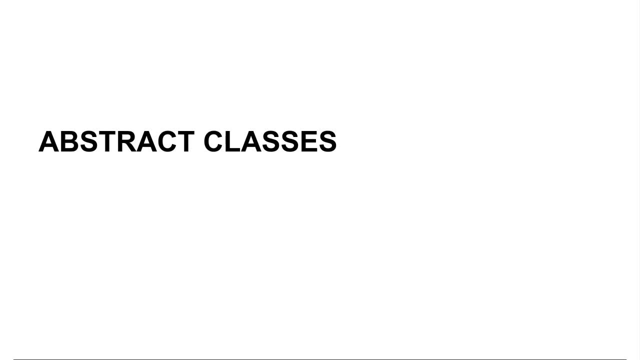 abstract methods. What are abstract methods? Well, abstract methods are methods that must be implemented by one of its descendants, since there are no concrete implementations for abstract methods in the abstract class itself. Furthermore, abstract classes cannot be instantiated, so you cannot use a new keyword to create an abstract class, Since it is a part of the abstract class. 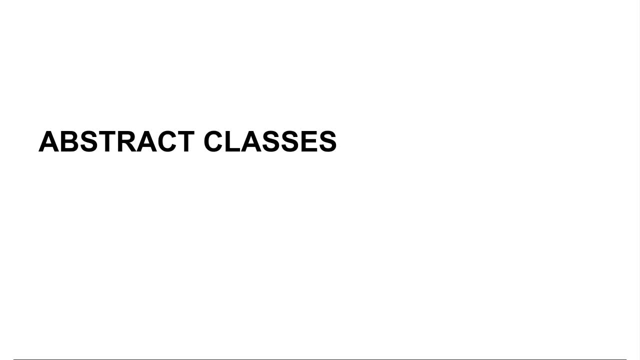 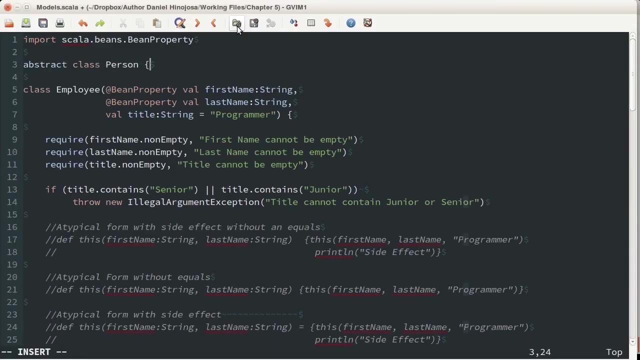 any subclass of the abstract class can be assigned to that abstract type. Now, that introduction had a little bit too many nerd words, so let's try an example in our modelsscala file. All right, so here we are in the modelsscala file, and what I'd like to do is I'd like to do the following. 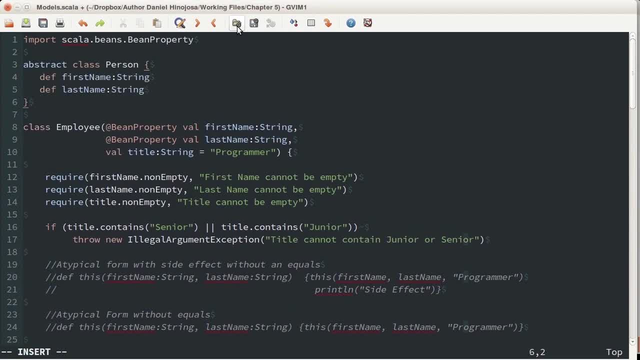 I'm going to be right up here at the top and I'm going to create an abstract class. So I'm going to go ahead and save this and this is an abstract class. I have abstract in front of the class definition and I have two methods. I'm going to create an abstract class and I'm going to 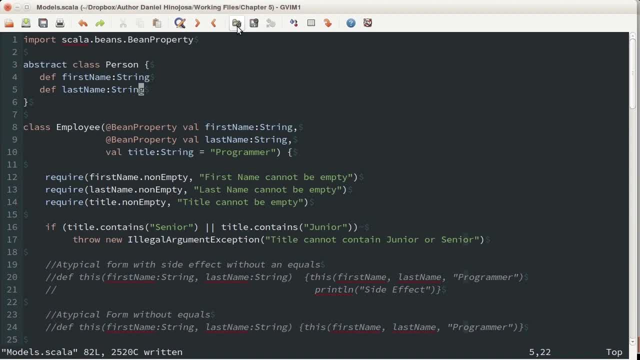 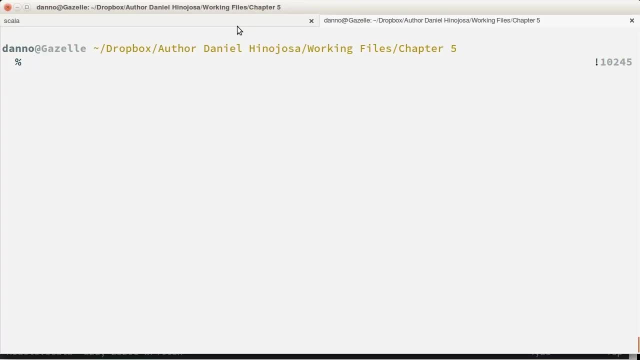 create an abstract class. One's called first name, that will return a string, and the other one's a last name that will return a string. Please note: there are no implementations. I don't have equal something. Now let's do a quick sanity compile to ensure that we wrote this correctly. All right? 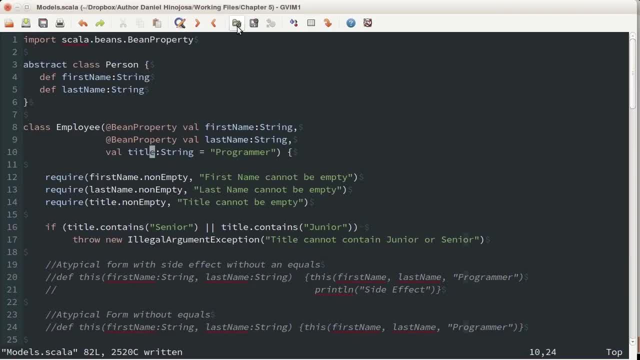 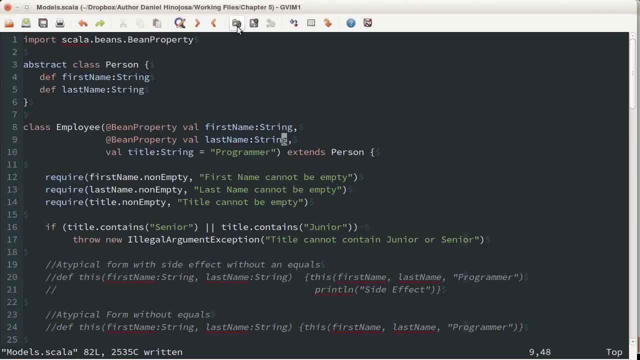 to our code. before we continue Now, remember we saw in our video session in the section classes that if we put a val in front of a property- and we're talking about these vals right in here- it automatically generates a method called the same as our property. We called it our. 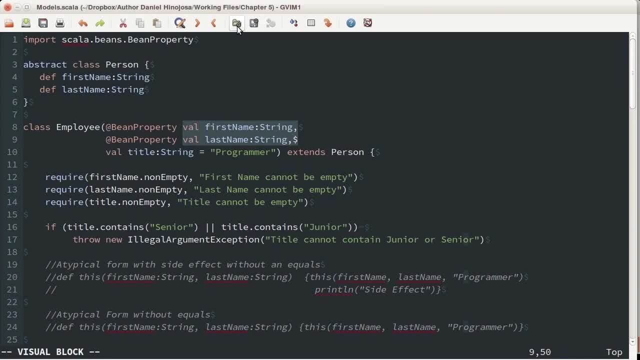 accessor method. In other words, the property first name has a method called first name because we put a val in front of that property. If we put a var, we'd have an accessor with the same name as well. Property last name has a method called last name, Again because we put a val in front. 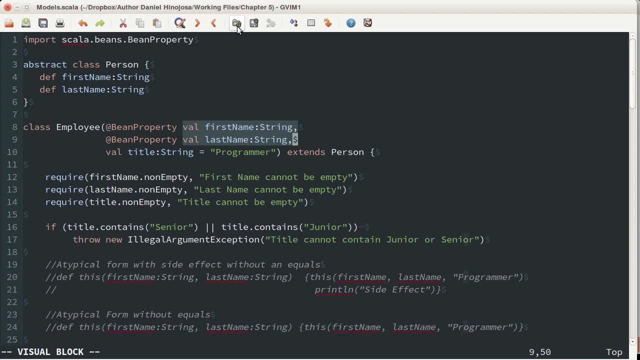 of that property. By that fact it is reasonable to conclude that employee does adhere to the contract, that it or its subclasses must have an implementation of the methods first name and last name. And if we compile we see that this is true. Not only that, we also see that from the 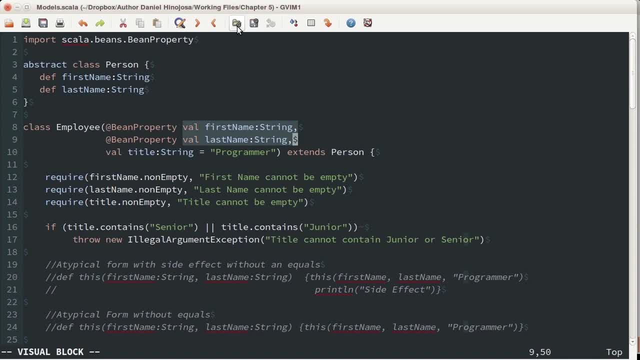 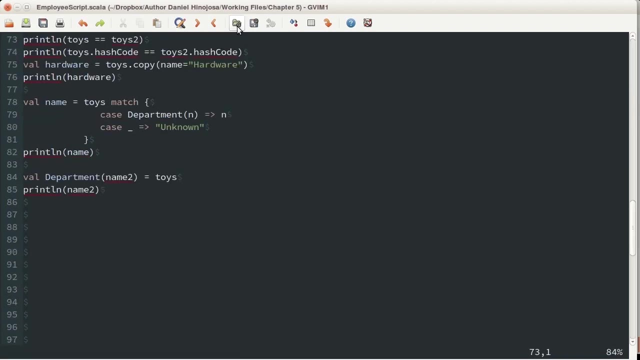 compilation that also manager adheres to the contract as well, because manager extends from employee and deploy extends from a person. Now let's play with our employee script And do some polymorphism with this. So here we are back again. we've already established that in our 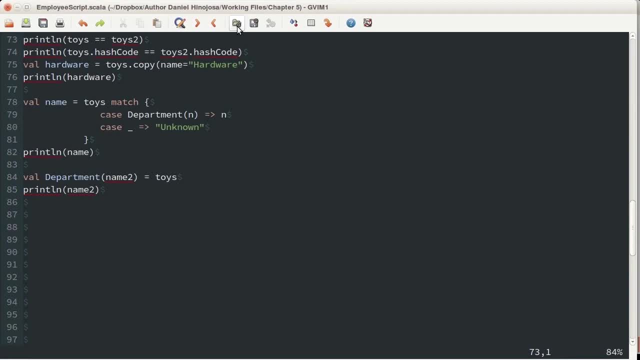 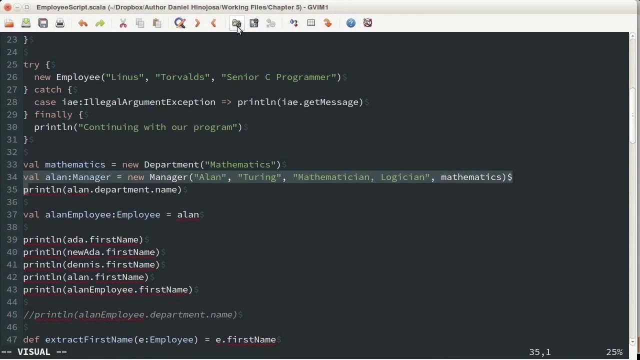 own little world that Alan Turing is a manager And that means that Alan Turing can be assigned to a manager reference, or it could be assigned to an employee reference, or now a person reference. So somewhere up on here- let's take a look back on here- we have a reference to Alan as a manager. 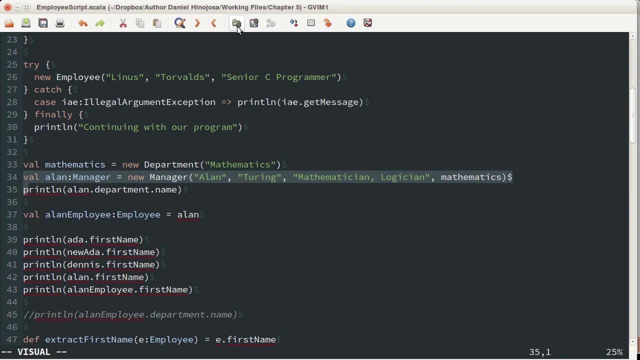 And here it is. we have Val Allen. the type of this pointer is manager and it is referring to a manager object, Since manager extends from employee and employee extends from person. what we can do is: let's give this a try. down here is that we can. 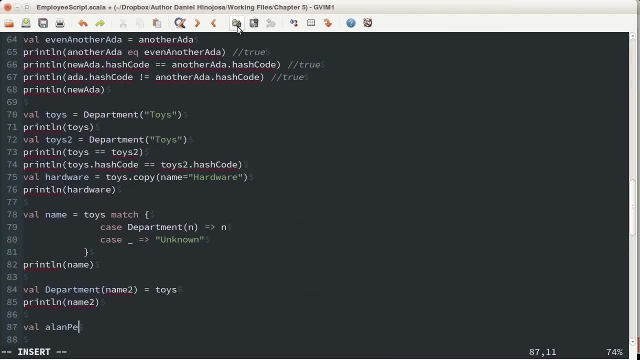 assign. let's say we want to create a reference called Alan person that only points to persons, and we wish to assign that to Alan. Will this work? Well, let's go ahead and save it and run our script. We didn't do any kind of print line, So just the fact that we're able to run it should. 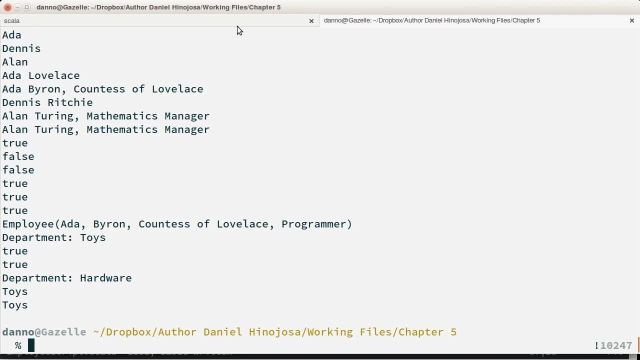 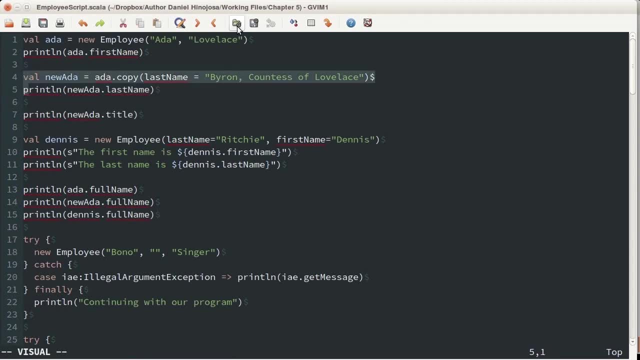 be good enough, And it does. it works out just fine, Otherwise we would have gotten an error. Let's go back to our code Now. given new Ada- remember new Ada- is this right up here? we're taking an Ada reference. 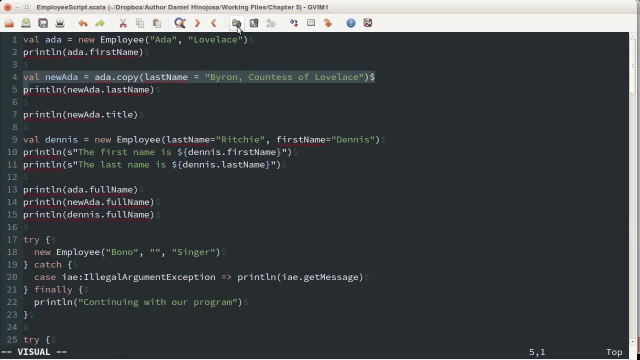 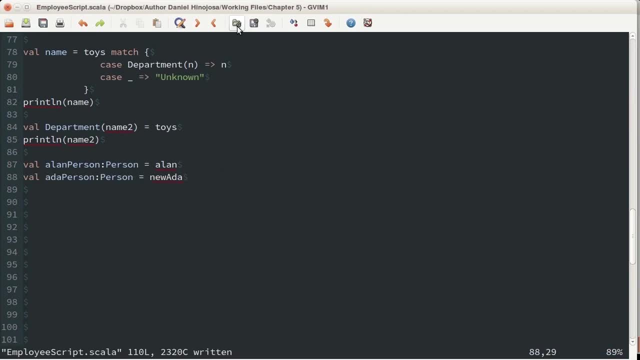 copying it, changing the last name, regardless of what happens. both Ada and new Ada are employee objects, So it stands to reason that we should be able to do the following: So we're taking an Ada reference which happens to be an employee reference and we're signing it to Ada person. 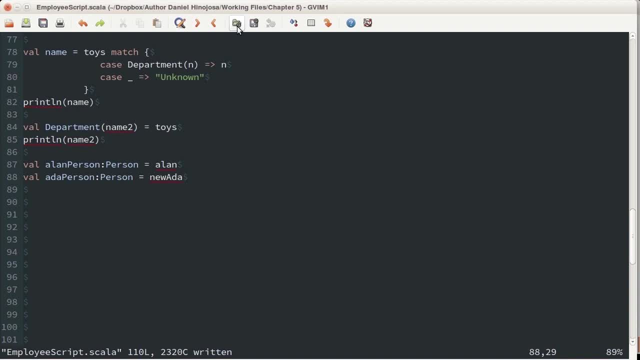 which is a pointer that points to person. Therefore, this is correct. this is just polymorphism And again, though we have no output in this example, the fact that we are able to run it as proof that polymorphism does indeed work. we can assign employees and managers. 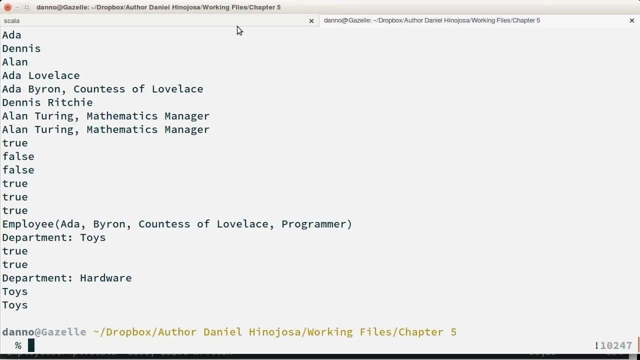 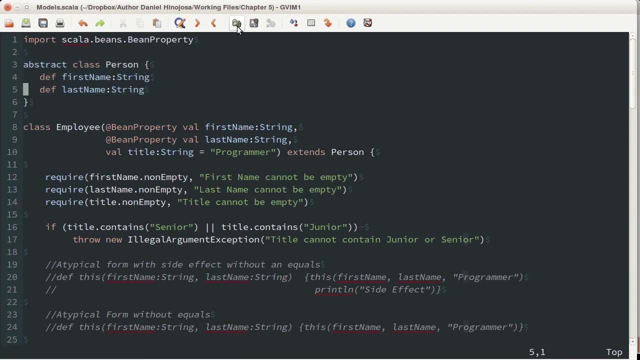 to a person reference. So we'll save it. let's go ahead and run it. Everything works out fine. Let's go back to the code and review. So here it is. abstract class has two methods. These are abstract, meaning there are no definitions. it is up to the subclasses to define these particular methods. But 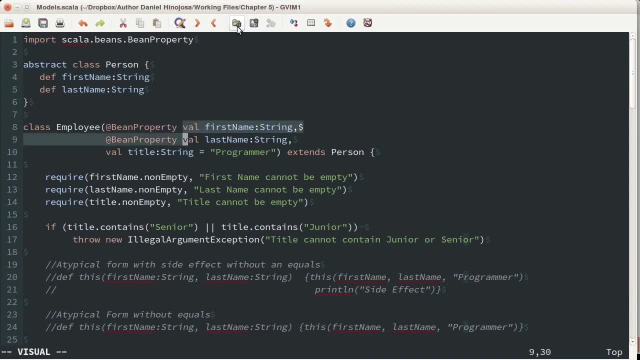 they are defined merely by the point of reference. So let's go back to the code and review. So here we can see, here let's say abstract is an abstract method, and in this case we're Days. And here we can see, our method has all the McKenzel starting and ending numbers, which indicates the 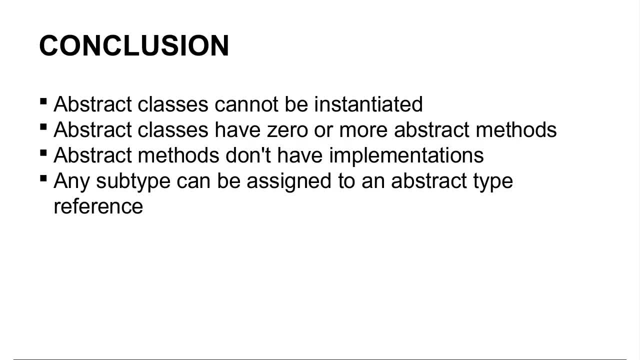 fact that they have vowels and because they are listed as vowels, a method is developed automatically for us for first name and last name, So it adheres to this particular construct. So, in conclusion, abstract classes cannot be instantiated. Abstract classes have zero more abstract methods: Abstract. 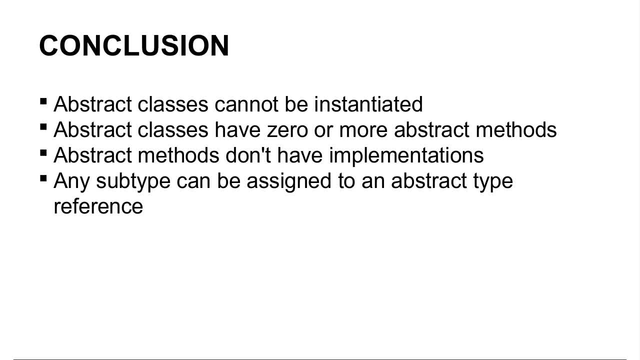 methods don't have the key word abstract implementation for it, and by that it is already an abstract method. since abstract classes are a part of the inheritance tree, very much like we had with person, employee, then manager, any object based off of that subtype can be assigned to that abstract type. in this session we discuss 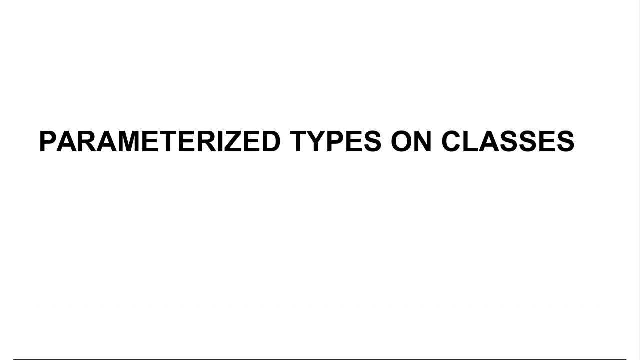 parameterized types on classes. we've already discussed parameterized types on methods, but now we discuss what happens when we apply them to classes. first off, we know that parameterized types use square brackets. we've seen that with methods. of course, the same holds true for classes. 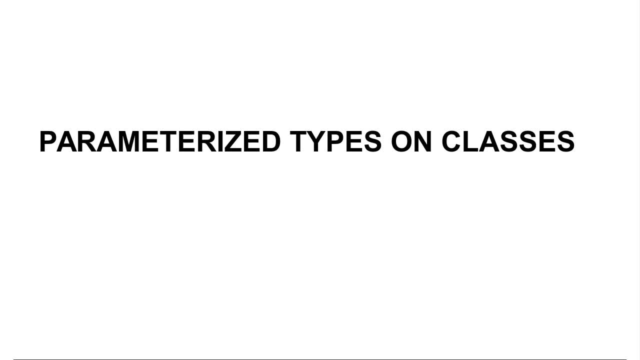 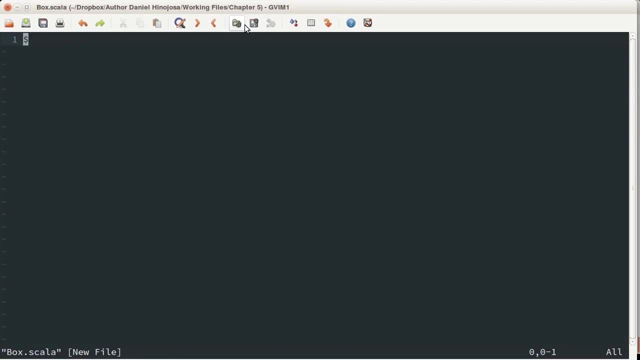 so, to keep things simple, let's create a class called box in its own file, boxscala. so here is our editor. we have boxscala, we've already created the file and i'm going to create a one-liner case class box, and here we'll have the parameterized type key, meaning we could put anything we want. 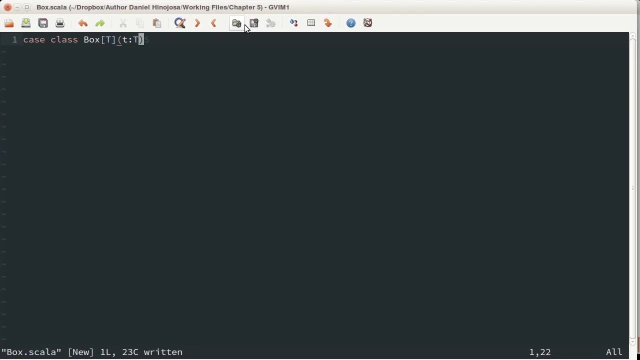 in the primary console. we could put in an int, we could put in a string, we could put in an employee, we could put in a date time. so we'll finish here. let's go ahead and save that. this is a complete line of code in the parameterized t states that the box can accept any type and that the scala's type system. 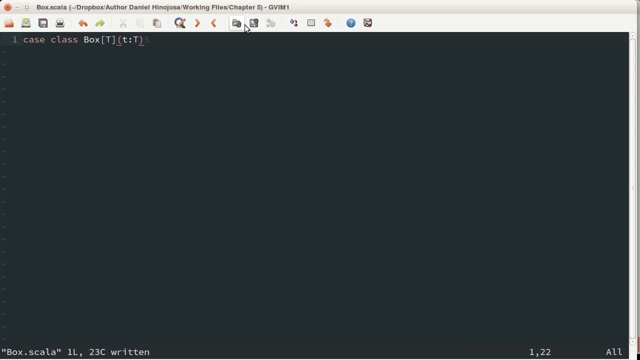 will keep track of that type. so if we extract t at any point, we'll have the correct type. now the same rule as applied with parameterized types. on methods, the parameterized type is always one letter: t, u, v, a, b, c, d. so let's create a script called box script that makes use of this box. 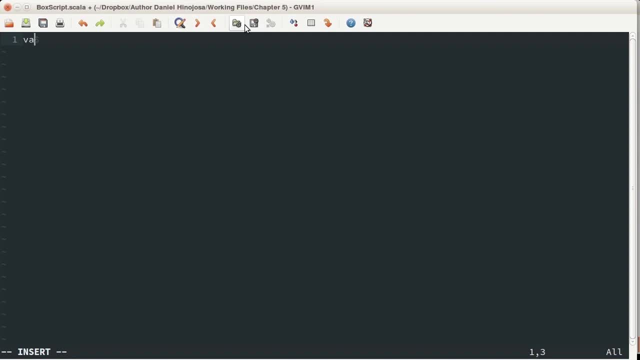 and in here let's create the following: i'm going to create one called int box and this would be equal to a new box of one. therefore, t becomes an int. so what is the type going to be a box event? let's try another one this time. let's be explicit what. 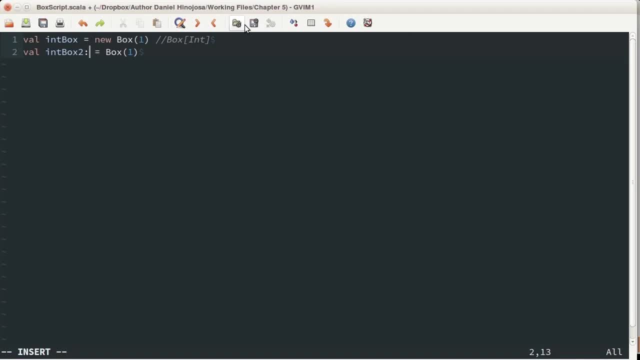 is the type. well, it's already listed there explicitly, but this too is a box of int. one thing: we don't have a new keyword that has nothing to do with a parameterized type. that has to do with the box is a case class. now, how about this one? now, this one's using coercion. 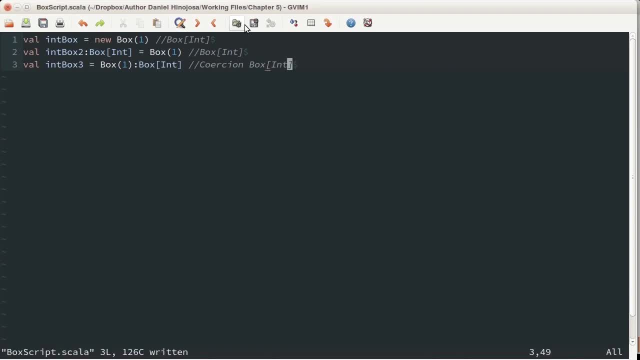 we're creating a box of one, although the type inferencer will already know what type this is, what we are coercing at stating that this is a box event, and do that before you assign it to N masse 3.. so this too is a box event. in fact, if i have int result of type ant, i call NB 3 and get t remember. 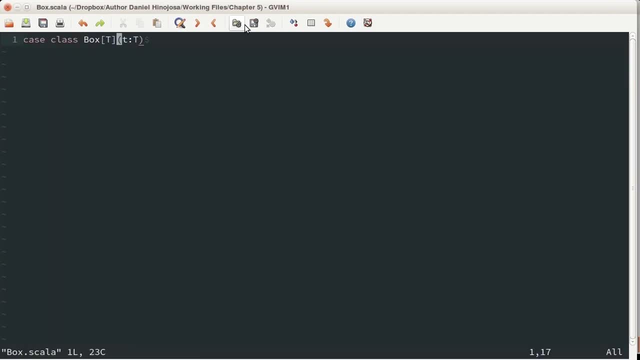 t is the property. let's go back to our box over here. here's that property. t is a parameterized type, so if we give it an int, t is now established as an int. so therefore, when we call t, remember this is also going to create a method. we could have had a val here, but we don't need to. it is. 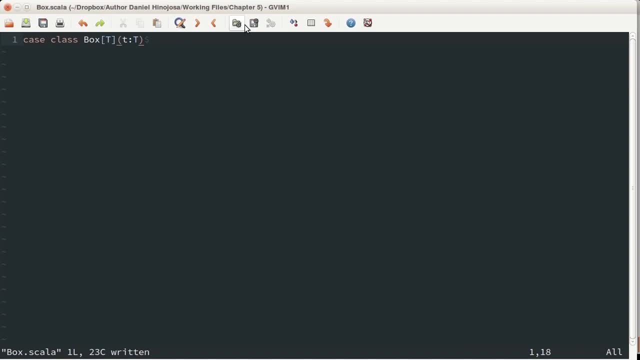 a case class. therefore, it's going to create a method called t and this method called t is going to return an int. if what was given to this box is a type of int, so let's go back. so therefore, when we call t, this is of a type int, so let's save this and let's run it out of a command line. so 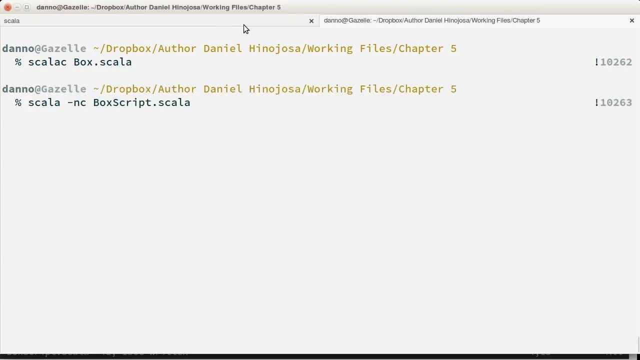 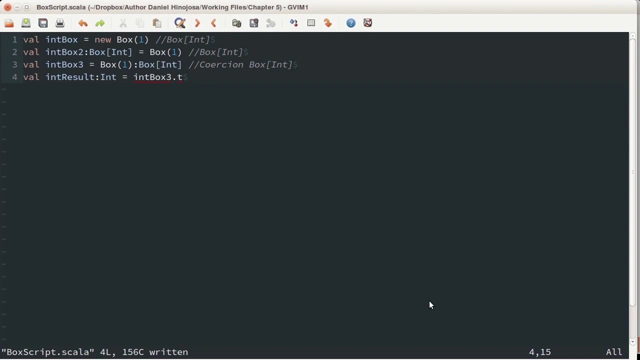 first off, let's compile, then let's run our script. okay, everything ran just fine. we didn't have any print lines. but because it ran just fine, we know that our assumptions are correct. let's go back to that script. of course, we could easily use different types in our box, so let's try some. we can create a. 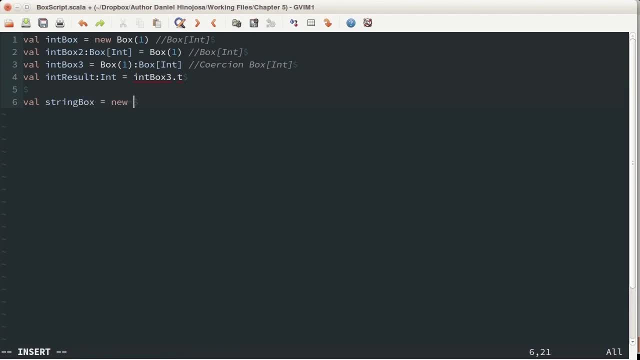 box of hello. we could do something like this to reinforce it: that what we want in here is is a string of hello. now for our next example. let's create a manager box again. with this box, we could put anything we want in it, and this will be a box of new manager. and let's try, Kathy. 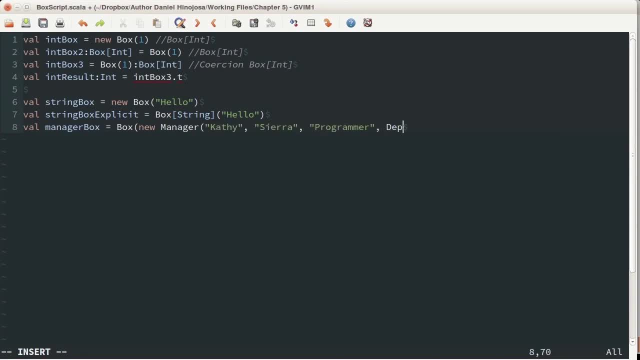 Sierra, who is a programmer and is with the department of programming, learning and fun, so this one is going to be a box of string. this, too, will be a box of string. and the last one, although this on multiple lines. let's clean it up so it looks like this: this will be a box of manager. 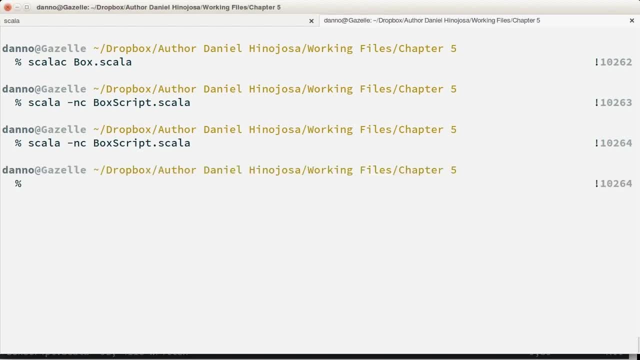 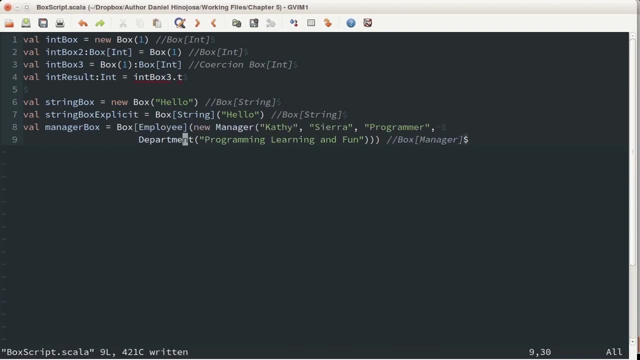 let's run the script to make sure that our assumptions are correct. works out great. if we wanted to, because manager is a subtype of employee, I could force it to make this a box of employee, where here the parameterized type is employee. that makes this box an employee. let's run the script to. 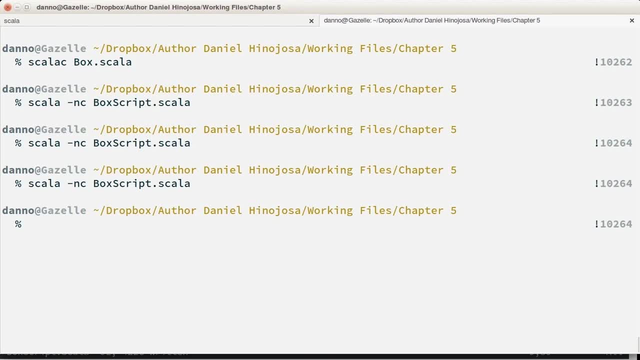 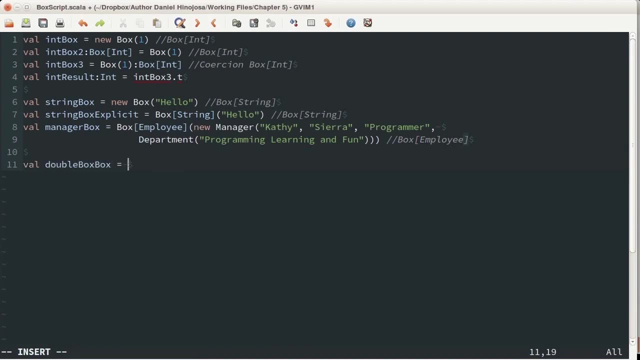 make sure that works, looks great. now let's even get fancier. how about a box of a box of double? sure, let's go back. let's call this one double box box and this is going to be a box of a box with 4.0. what is the type? this is a box of a box of double. so let's say: 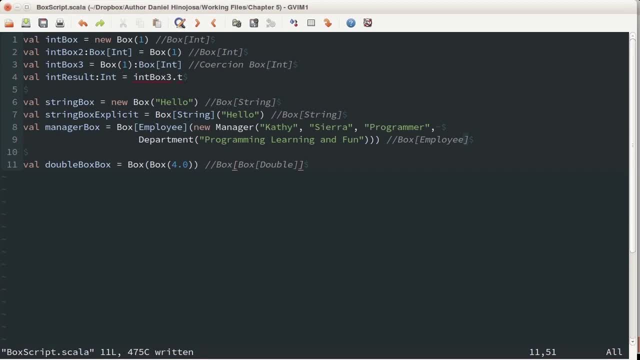 we want to fish out of here. so we have a box inside of a box. the box inside of the box has a value of 4.0. let's say we want to fish out that 4.0. what do we do? but we take double box a box. 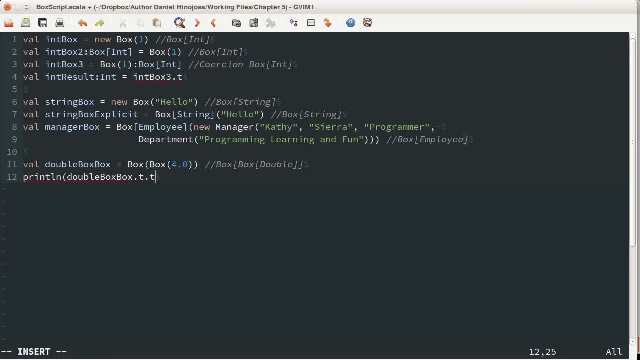 we'll get t. once we get t, this will be a box of double box and we're going to have a box of double and if we call t again, then we'll get 4.0.. In fact, just to make sure that the types carry along with. 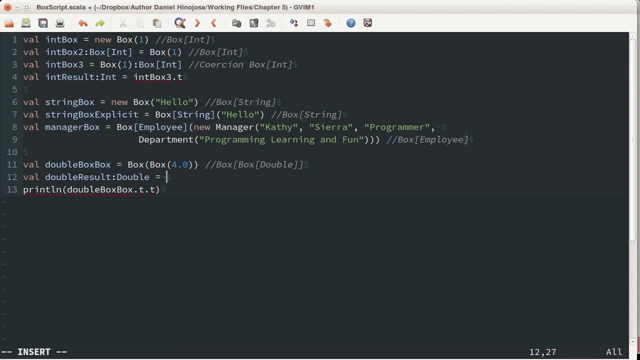 this: let's say we have a double result. this has to be a double, and we call double box box dot t, dot t. and what we'll do here is instead call double result. and again, this is the reason for the parameterized types we don't want to return in any or any ref. we want to return the actual type. 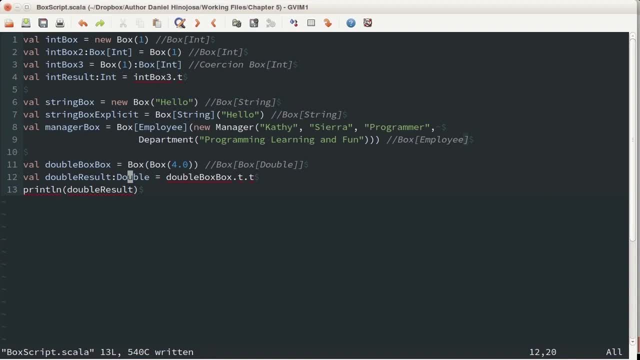 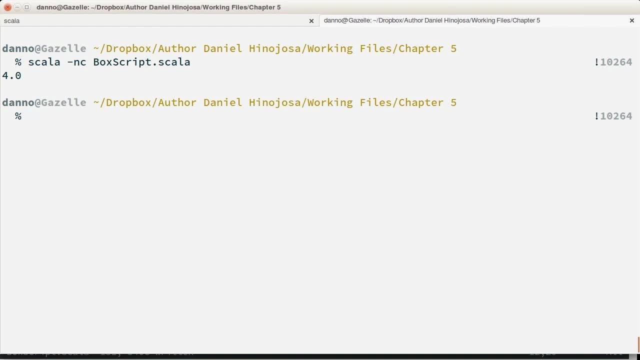 that is, within this box of a box. in this case that would be a double, so let's save this and run it there. it is 4.0.. Again, the parameterized type can be anything and in this case we have a type t. we could give it an int, we can give it a string, whatever it is we'd like, and the type. 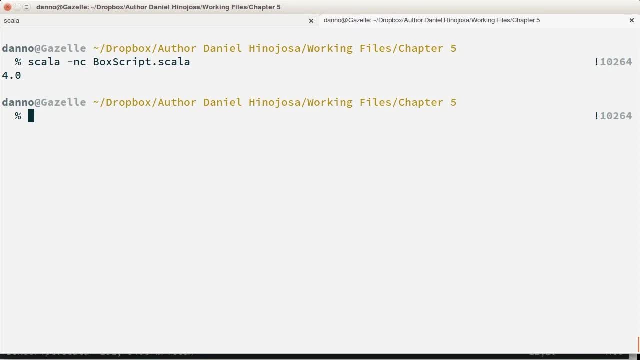 system will track all of it. It's very important that all functional programming languages, and really all static type languages, keep track of these types, no matter how many layers deep it is. So how about classes with two type parameters? Sure, so let's create another file called couple. 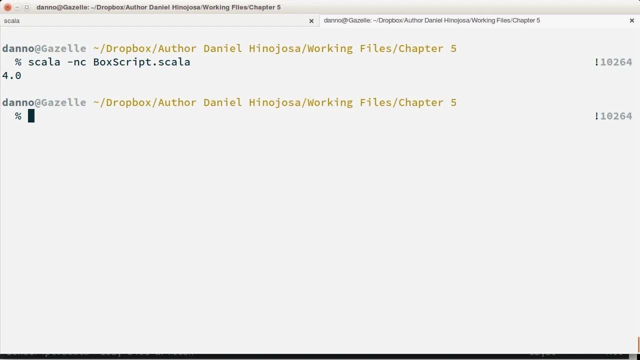 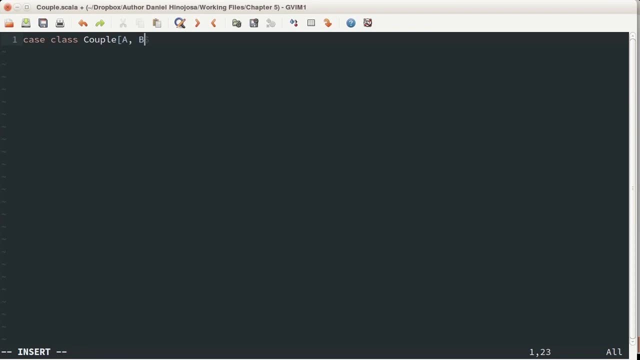 dot scala, and we'll create a class called couple, And this time with two parameterized types. Let's go back to our editor. So here we are at couple dot scala and a nice little one-liner, once again couple a and b, and we'll have one called first. this will: 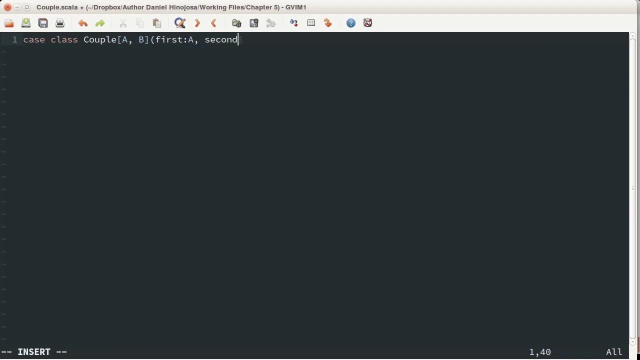 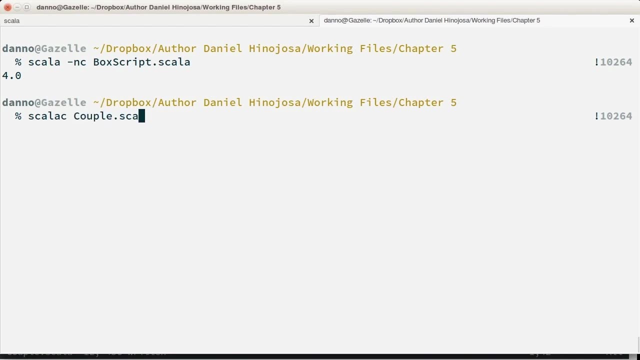 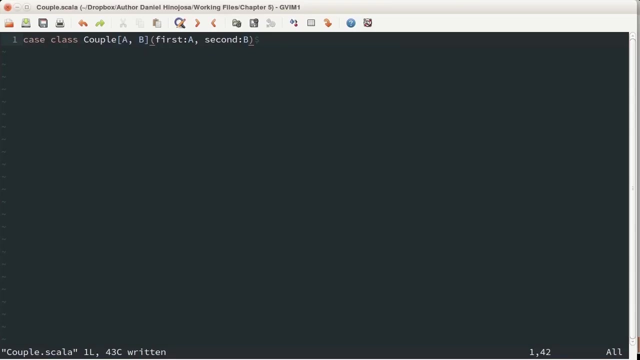 use the type a, and again, type a could be whatever it is we want, and second will be of type b, two parameterized types, whereas box only had one. so let's compile it. that looks great compiles, and type a could be anything, b could be anything and again, once established, type system will track those. 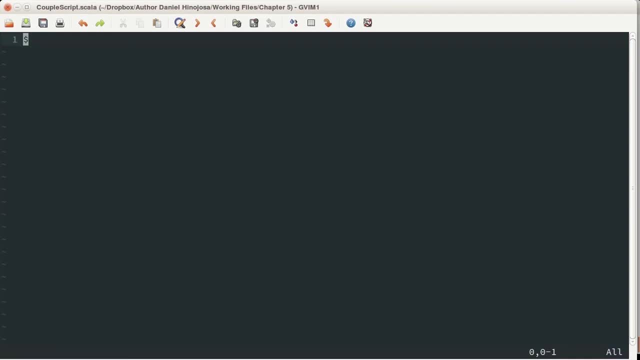 types. So let's create a script called couple script and let's give it a ripped and let's try a few different ones. Okay, this type is going to be a couple of int and string. This two will be a couple of int and string And in fact we could even make this explicit. Let's try another one. Okay, this: 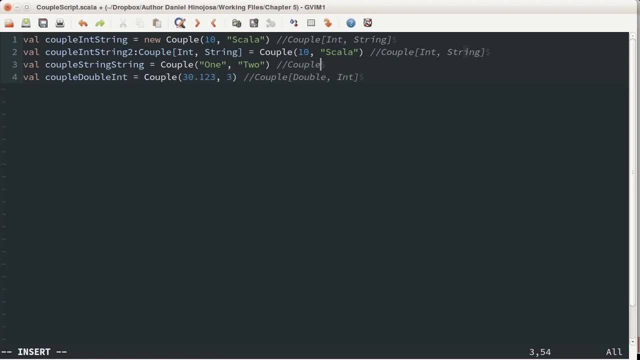 is a couple of double and int And this one is a couple of string and string. Now let's try a complicated one: couple of a string and couple of int and double Interesting on that one. So let's say that this one is going to be a couple of Hello and this will have a couple of three and 22.2.. For 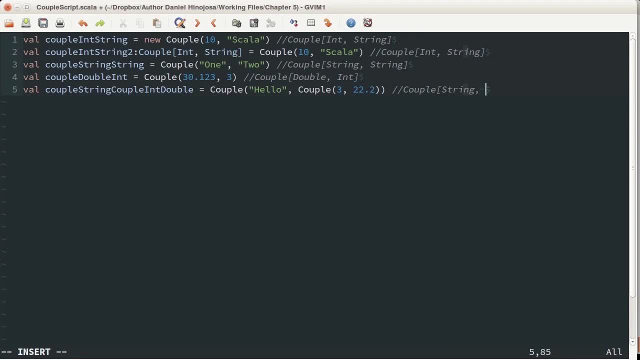 example, what is this type? This is a couple of string and couple of int and double Okay. so, as you see here, you can even place a couple inside of a couple. So, given all this, let's go ahead and save it and run.